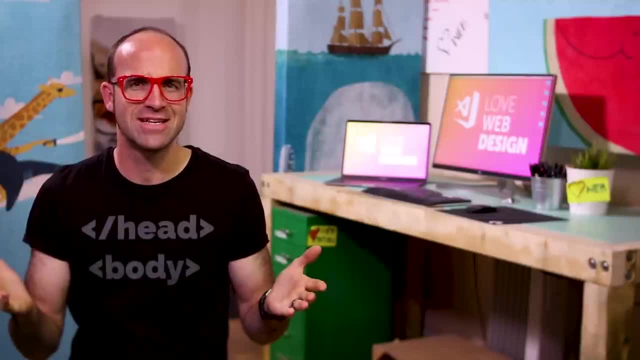 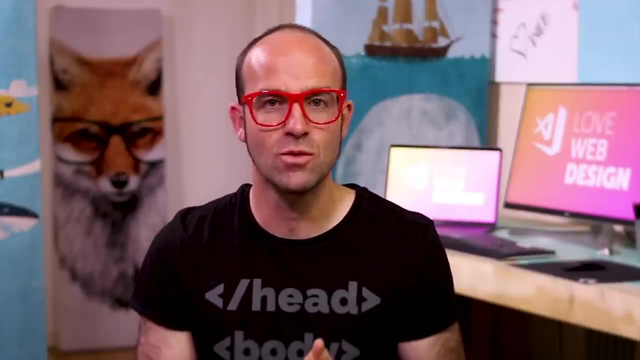 We're going to use the world's most popular and surprisingly free web design tool called Visual Studio Code. There are downloadable exercise files so that you can follow along with me in every video. At the end of each video as well, I'll save where I'm up to. 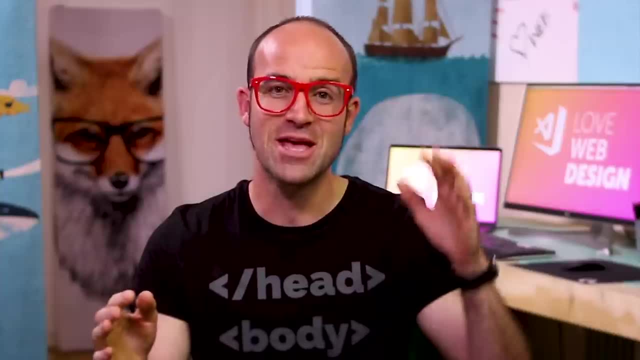 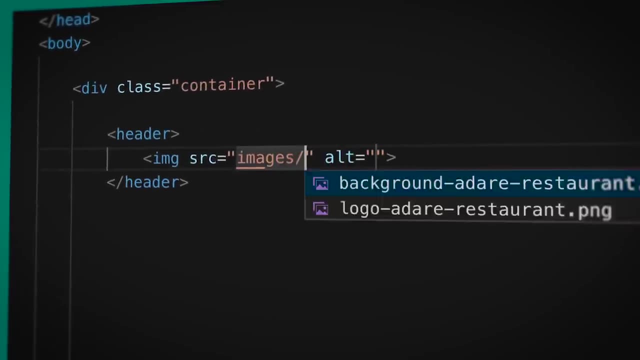 so that, in case you get lost or something's not quite right, you can compare your files with my files. It's a nice easy way to make sure you don't get lost. We'll start by working through some really simple HTML and CSS exercises. 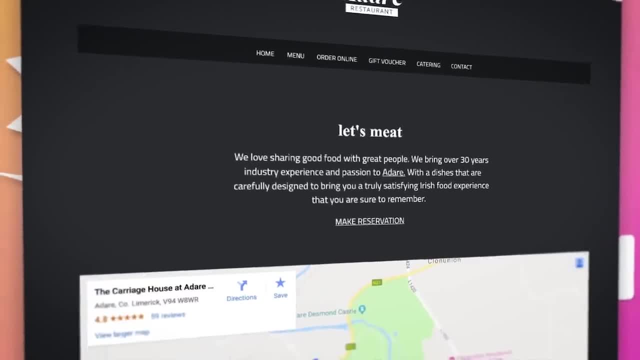 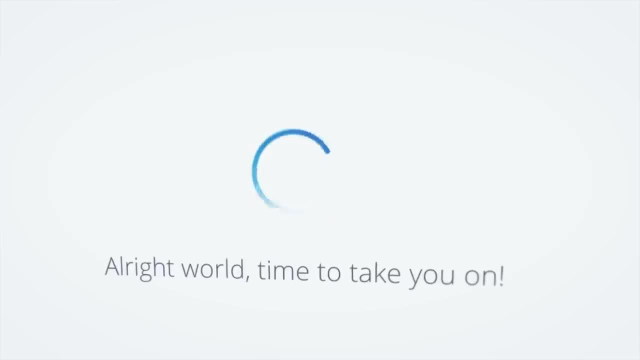 Learning how to create the structure of our website, then adding and styling text, working with logos and background images. you'll actually set up your own domain name and hosting and we'll upload it live to the Internet so other people can see your site. 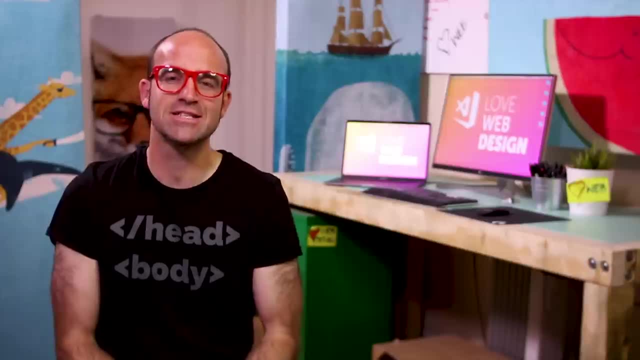 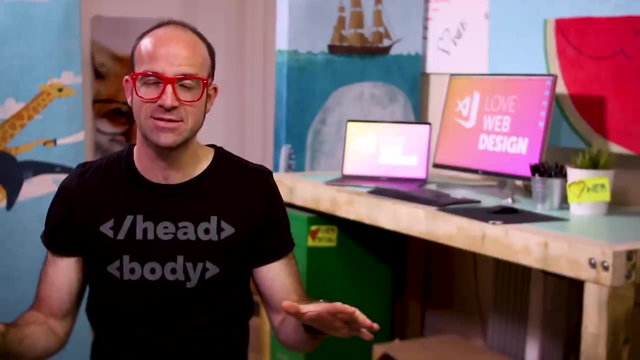 Throughout the course, I set some fun class projects so that you can practice everything you're learning in the course. So this is an introductory course aimed at complete beginners. So for people who have no experience in web design, have never written a single line of code, this course is for you. 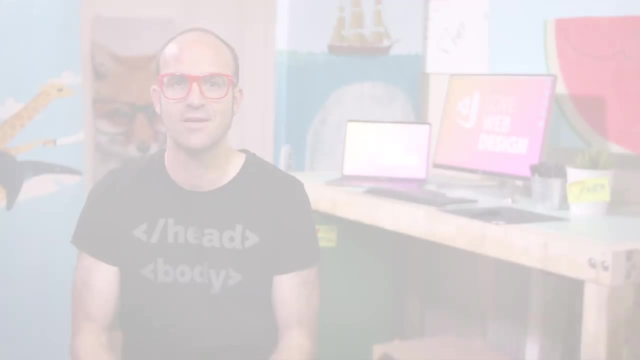 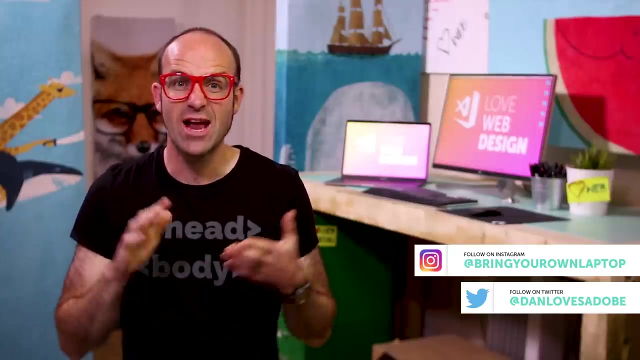 We're going to start right at the beginning and work our way through step by step. So who am I? Hi, My name is Daniel Scott and I've been a web designer for about 15 years now. I'm also an award-winning instructor. 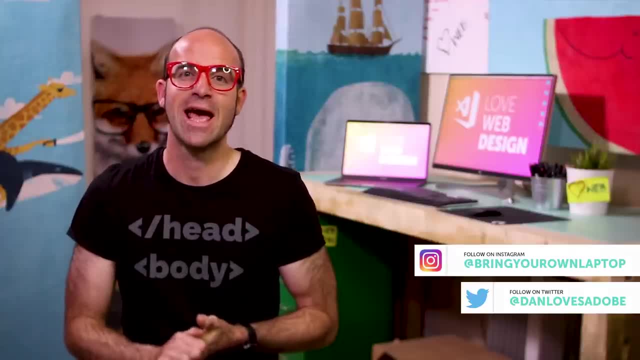 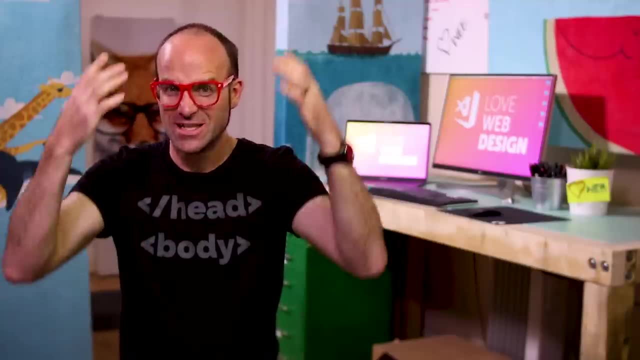 For the last two years in a row, I've won a Max Masters Award at the massive Adobe Max Conference. I also have red glasses and a cool T-shirt. I'm pretty sure just this combination on its own should make me qualified, Maybe. 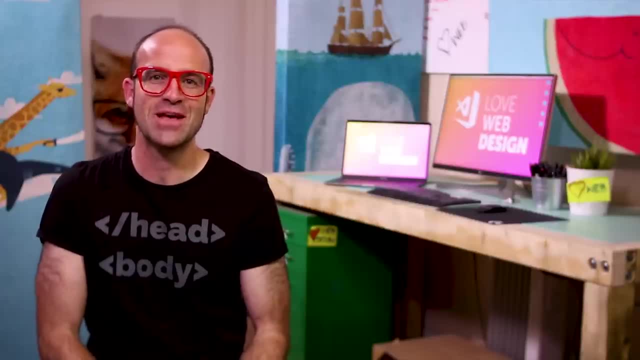 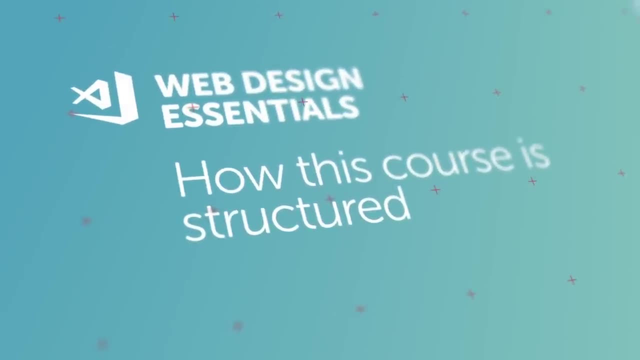 If you're ready to upgrade yourself, let's get into this video and learn how to build your very first website. Hi there, Welcome to the course, This video. I want to talk about how this course is structured, So it's broken into five parts. 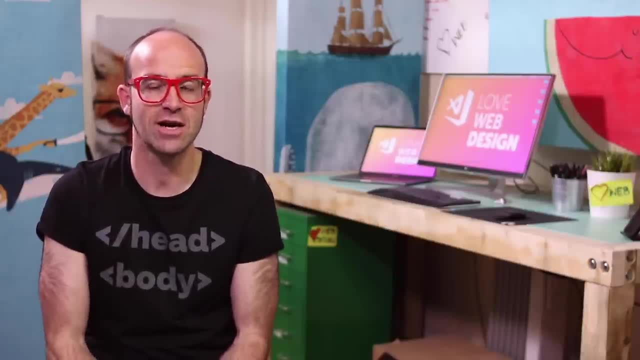 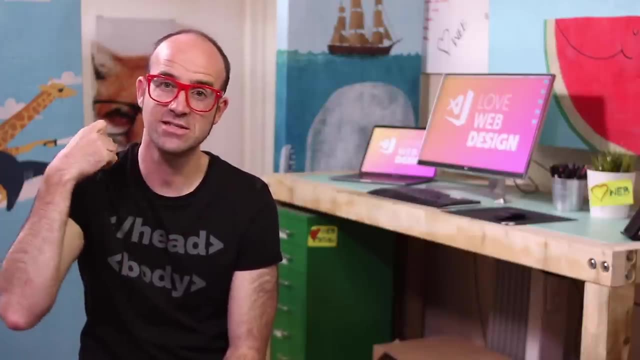 We'll start at the beginning with just a real basic introduction to HTML and CSS, And then we'll start our very first project. So phase one, quick introduction. Phase two: we'll build this website. So we'll take our kind of basic HTML and CSS introduction. 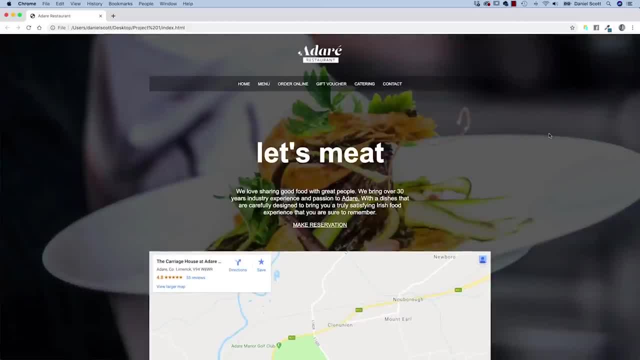 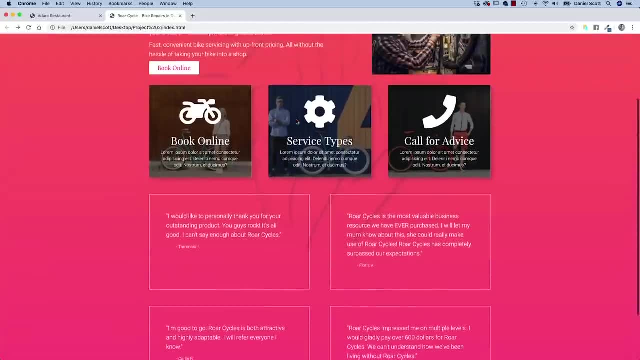 and turn it into this website here, Just a nice simple one to get started. The third thing we'll do is we'll create this Raw Cycles website. Now, this website is just a little bit more advanced. Let's say it's intermediate HTML and CSS. 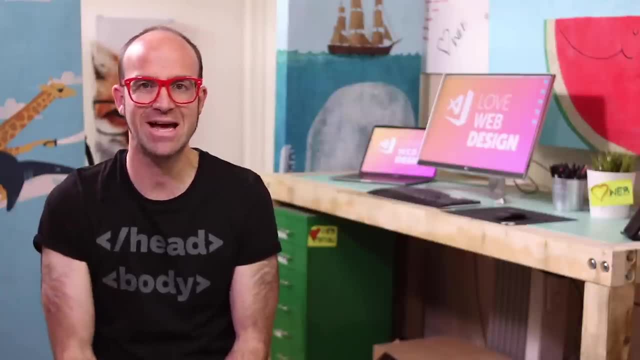 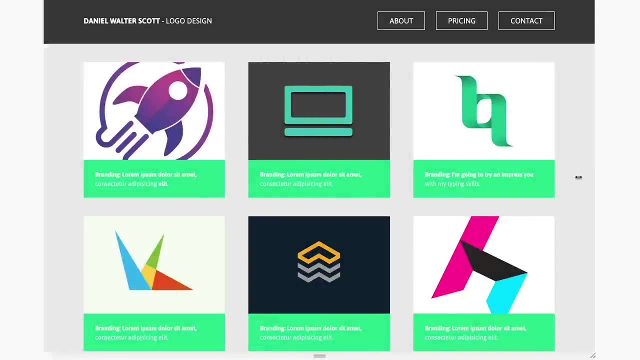 We cover the basics in the first one and then we get into a little bit more detail here. Third part is we will make our site responsive. Just means it's going to adjust for the different browsers, So mobile phones, tablets and websites. 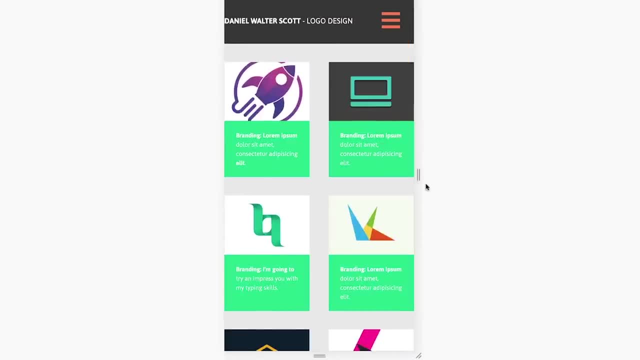 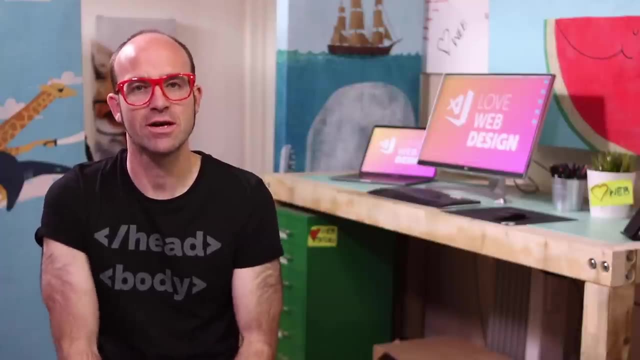 It's this one here. it's a portfolio site, Nice, simple one. You can see here it adjusts for different browser widths. And then the finale for the course is looking at a framework, The framework that we're going to be using in this course. 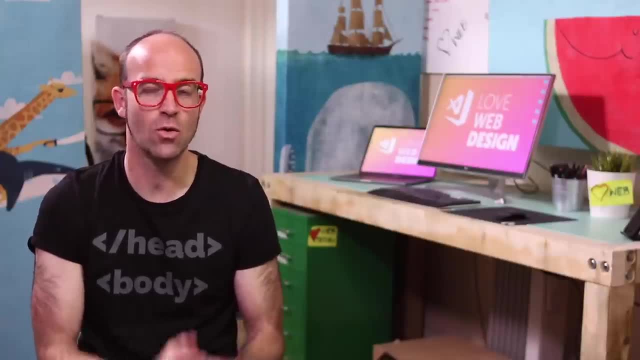 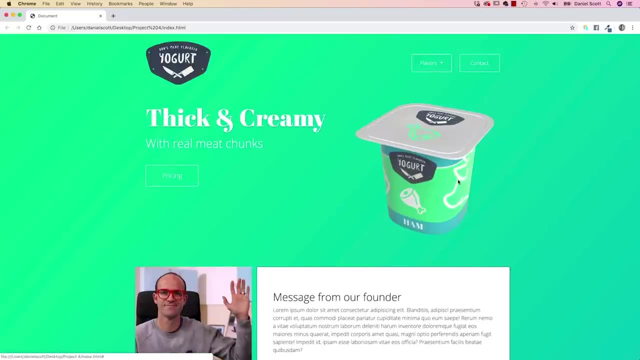 is called Bootstrap. it's super popular And it just means we can take all our knowledge that we know so far and kind of condense it down and use it really quickly to build sites. And we're going to introduce things like this jQuery slider here. 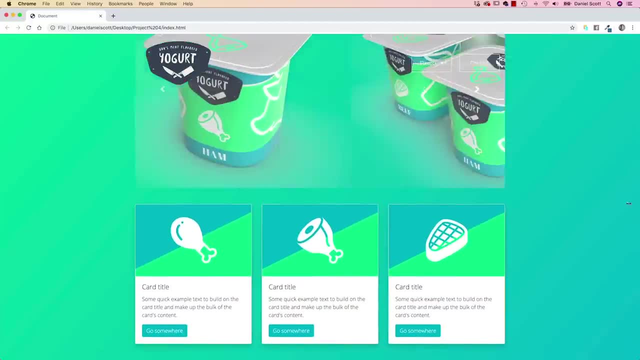 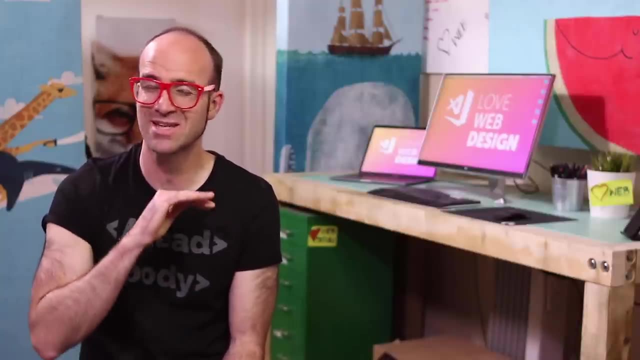 Images slide across. there's these cards. down the bottom There's an easy mobile nav. It's a really great addition to anybody that's building websites. A framework like Bootstrap is going to make you go super fast, make you look super professional, without you having to do all the heavy lifting. 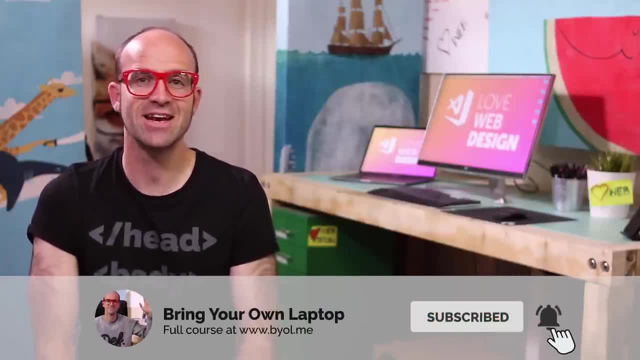 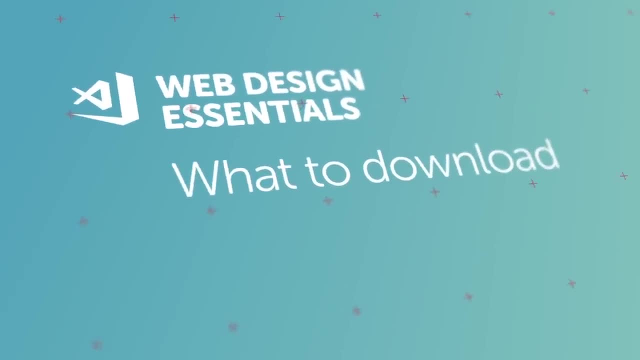 All right, I hope you're ready. It's time to get started and actually start building websites. I'll see you in the course. All right, let's talk about what you need to download and what you need to install. So downloading is simple. there are some exercise files. 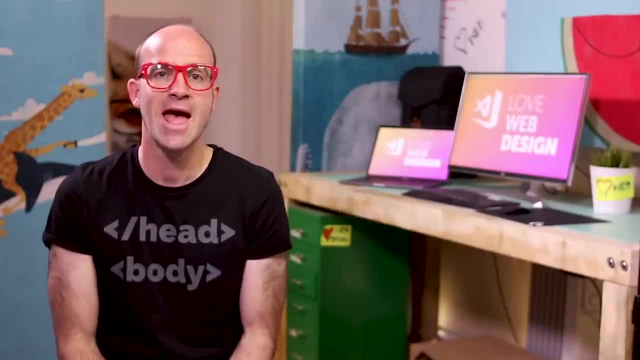 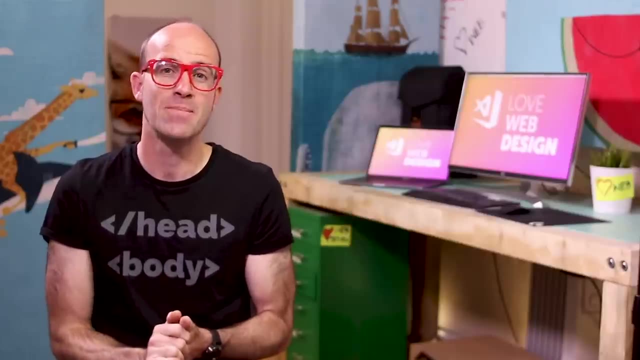 There'll be a link on the page here somewhere to download those And they will be everything that we'll use like images and text that we'll use throughout the course. So download those Inside that exact same file that you download. there'll be something in there called the completed files. 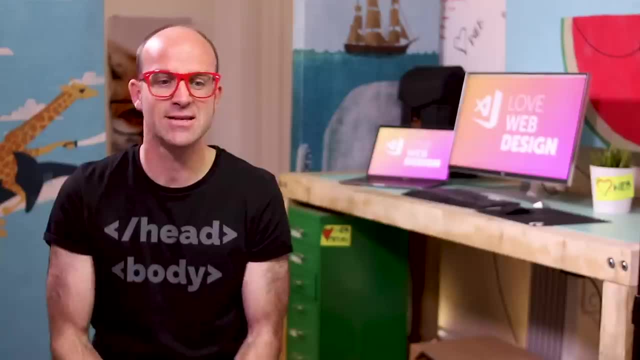 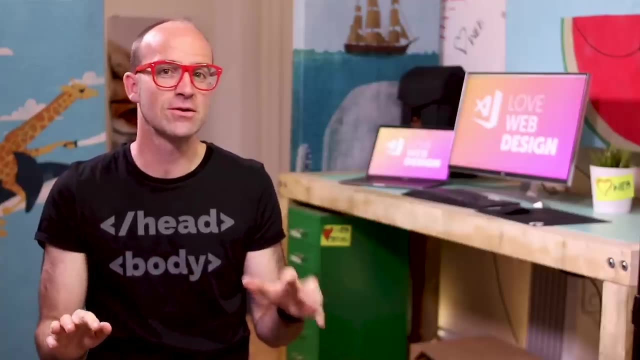 There'll be a folder inside of it And what they are is at the end of every video. what I do is I kind of save where I'm up to So that if you're following along and you're not getting the same results. 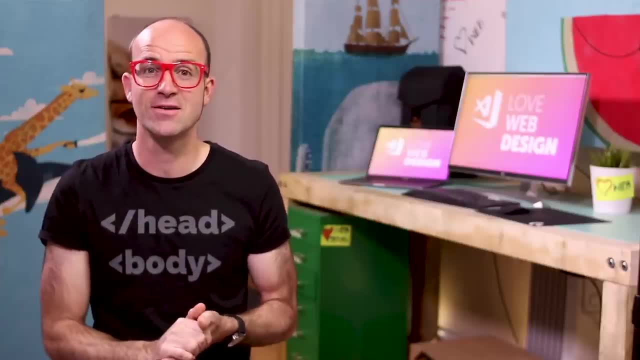 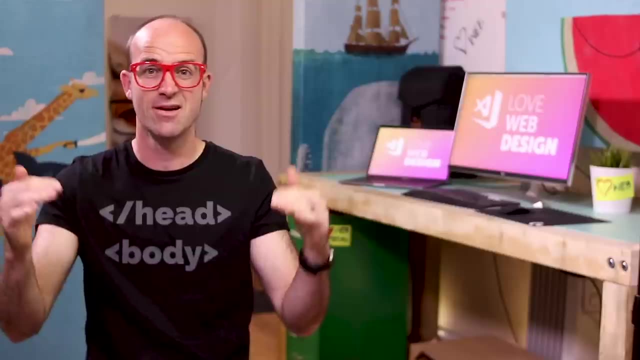 you can just look at the video number and then have a look at the completed files and just match my version with your version and go. often it's just maybe a spelling or a syntax error, but you can compare yours, that's working. 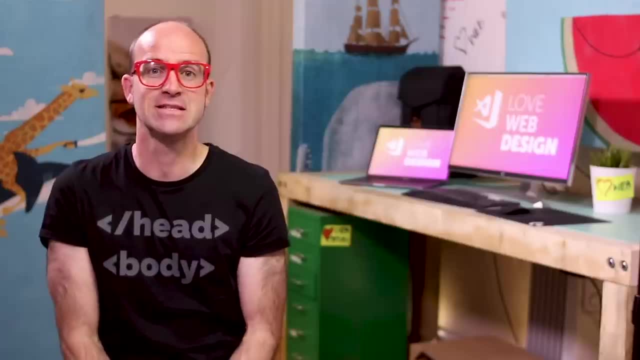 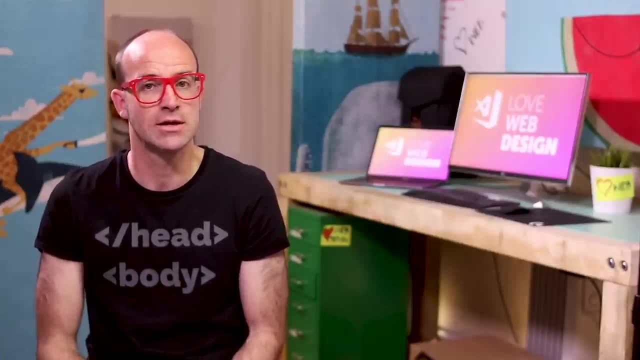 Or mine. that's working with yours. that may be not, So they're inside. the exercise files and completed files are all together. Other thing to talk about is what to download, So we will be testing our websites in Google Chrome, So make sure you download that. 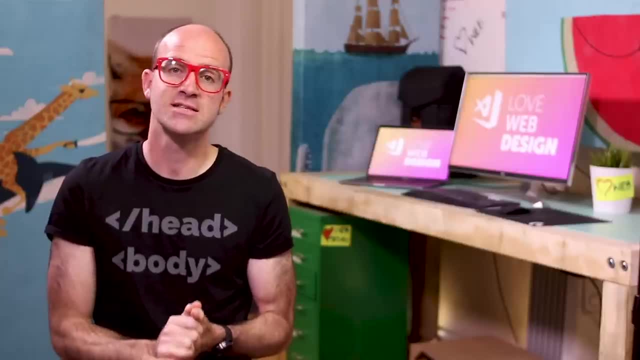 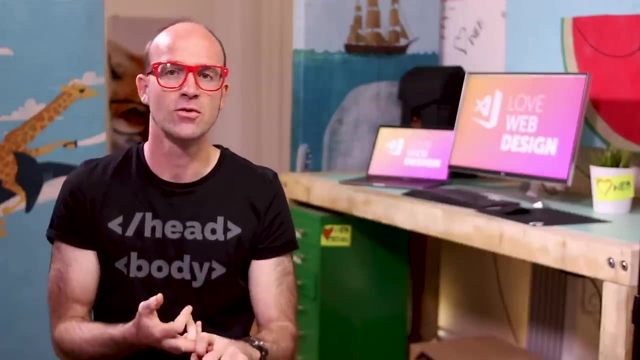 Google Chrome is by far the most popular browser at the moment, So download that and we'll do all of our testing inside of that. It's like Firefox or Safari or Microsoft Edge or Internet Explorer, But it's the most popular one. 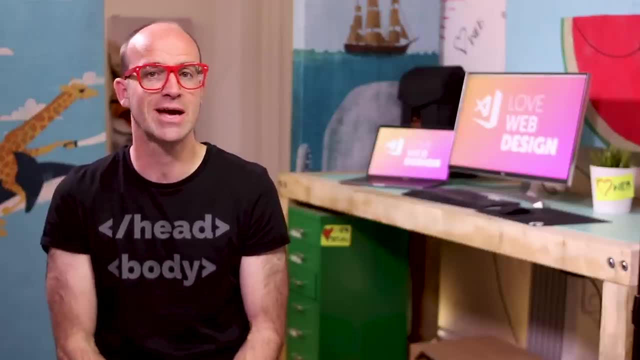 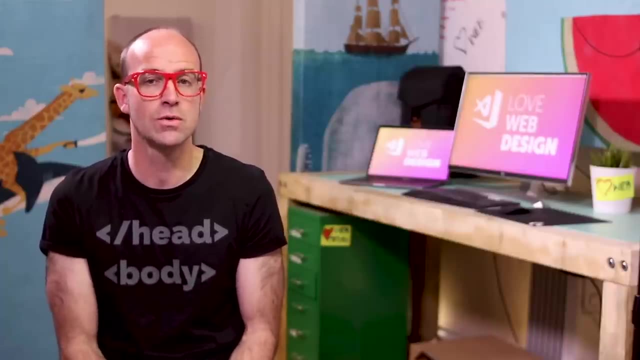 Go to Google Chrome's website and they'll show you how to install it. And the other thing to install is a code editor. So we're going to be using Visual Studio Code. Now why There's lots of different code editors. 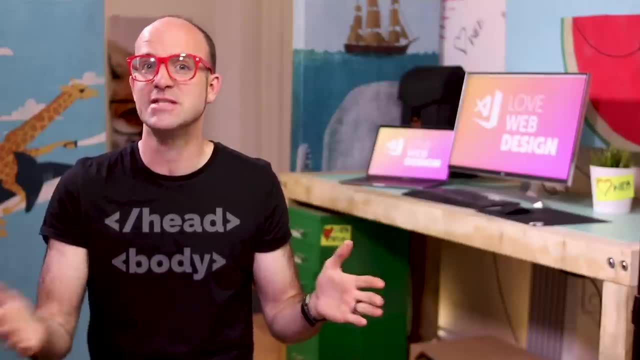 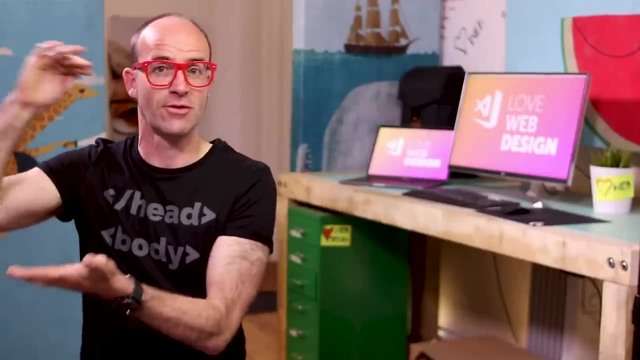 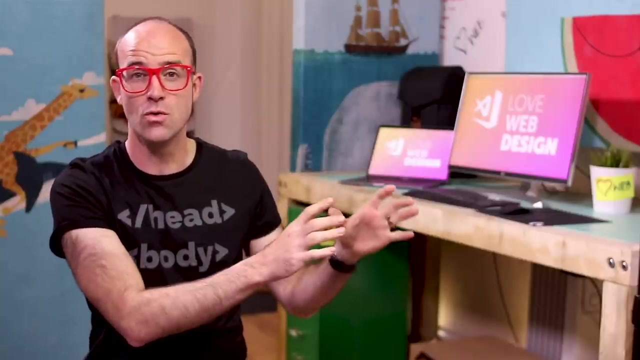 You don't need specifically this one, but you'll need it for this particular course Because basically, a website is a group, a mixture of HTML, CSS and JavaScript right, And you can use any code editor to make that. We're going to be using Visual Studio Code. 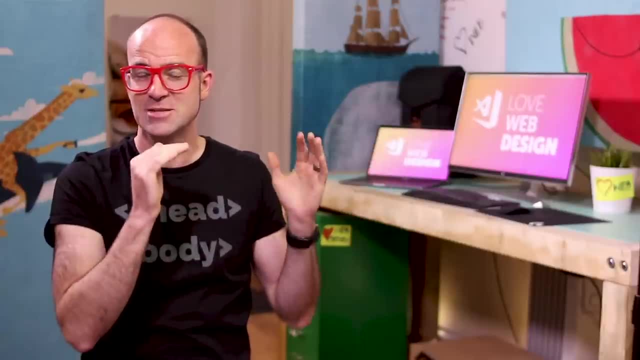 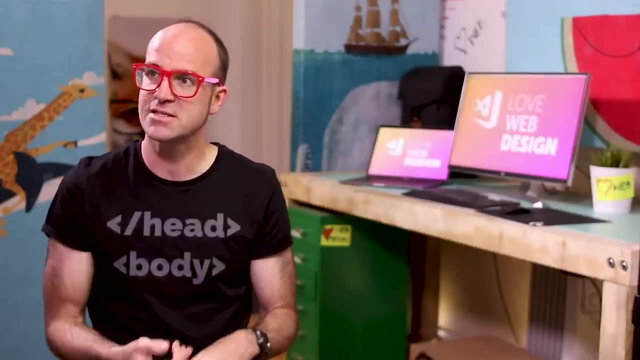 Not Visual Studio. that's a bigger product. You need the specific Visual Studio Code. It's free, it's made by Microsoft. And just so you know, though, I'm using that mainly because it's the most popular at the moment. So if you're looking to get work after this course, 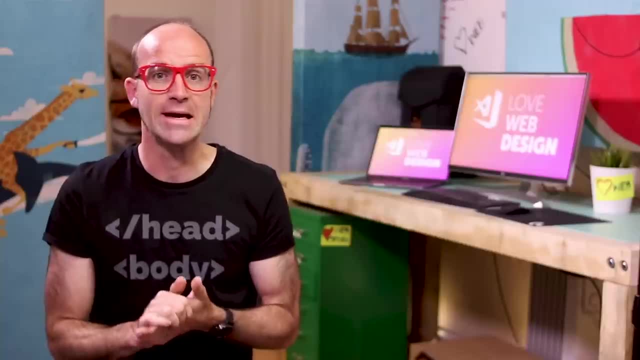 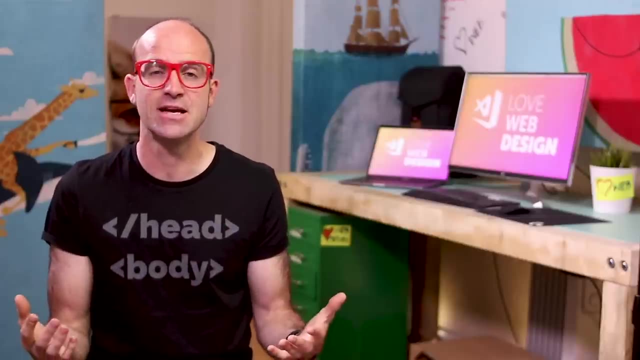 you're probably going to end up in a studio where they are using Visual Studio Code, So you might as well be learning the same one, But if you, the techniques and tools you're going to learn in this course are going to apply the same to if you're using a different code editor. 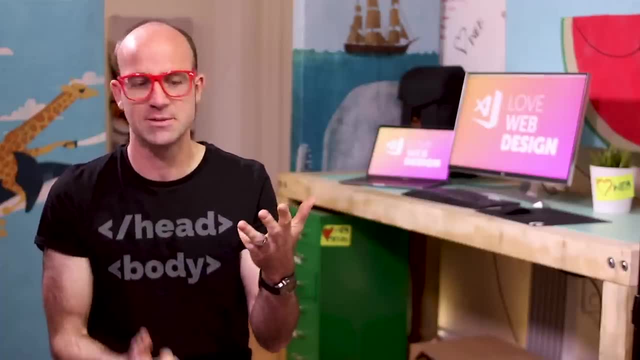 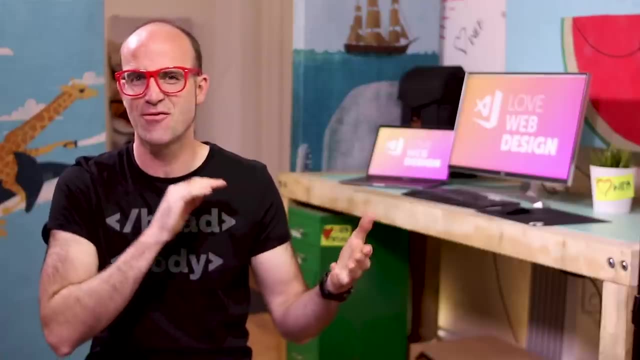 Let's say you're using Atom or Sublime or Notepad++. They're all really good editors, but they end up making the same thing. The shortcuts are different, They've got different ways of working, but the output is the same. 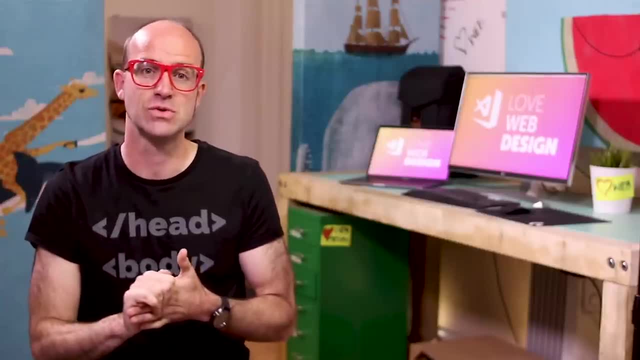 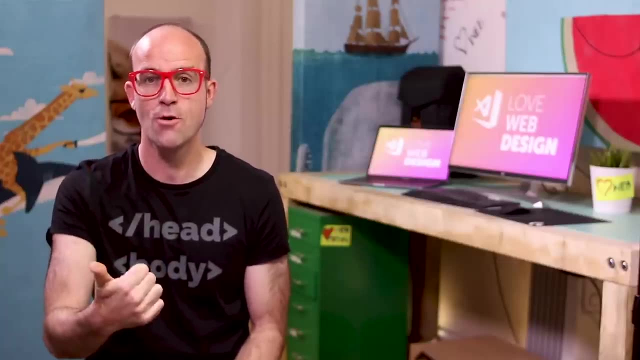 So don't sweat it if you learn all this stuff in Visual Studio Code and then you have to go and use another editor. Okay, They'll apply, lovely. but yeah, Install Chrome, install Visual Studio Code- Both of them are free- and I will see you in the next video. 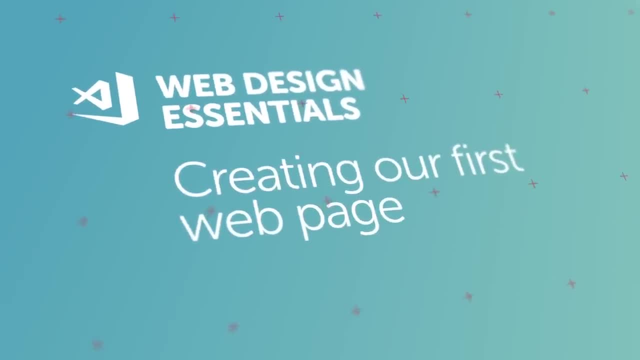 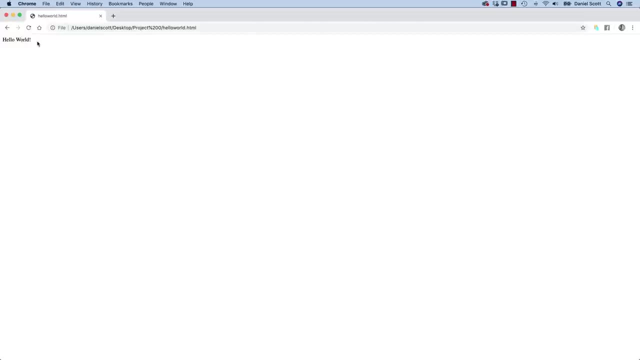 Hi everyone, this video we're going to make our very first web page. It's not going to be really exciting. It's going to say Hello World and in a browser it's going to show you Hello World. The course gets a lot more exciting, but we need to get the basics done. 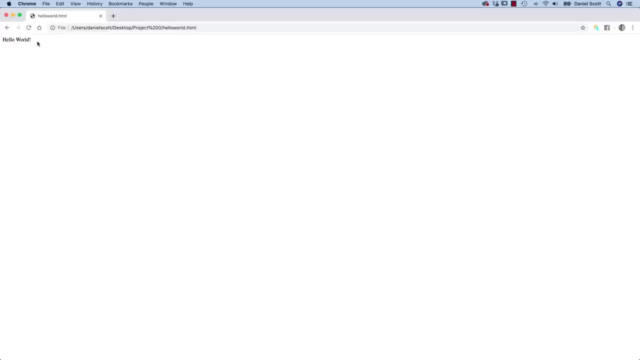 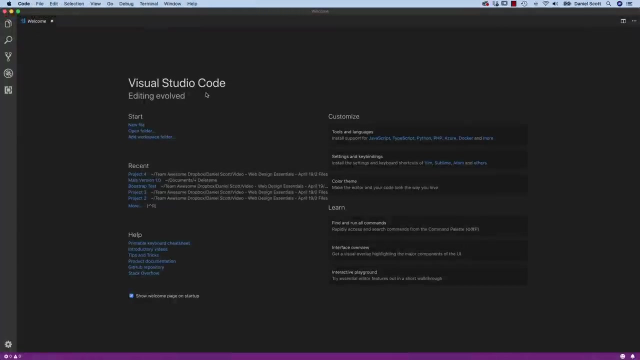 And that includes how to set up a folder for our website, how to create our first HTML page and how to test it in a browser. Let's do it All right. so we have installed Visual Studio Code and we have it open in front of us. 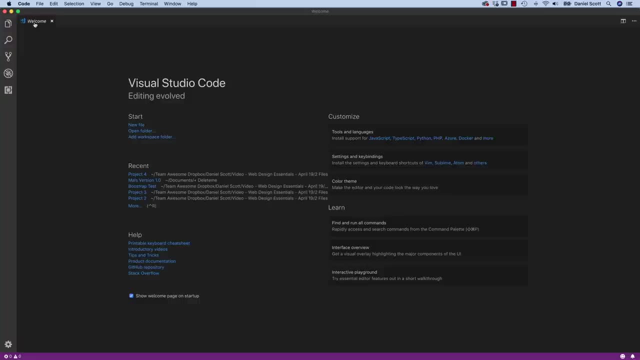 Now yours will look slightly different than mine You might have. we've got this welcome tab open along the top. You might have another tab open saying New Release Documents or something similar, And also yours might look slightly different because I'm using a Mac throughout this course and you might be using a PC. 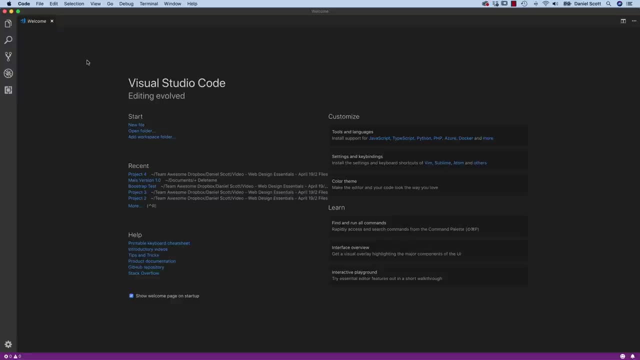 Don't worry, they work the same. Just some of the shortcuts are slightly different. but we'll cover those during the course. All right, it can be a little intimidating as well, this welcome screen and all the other kind of tabs on the top. 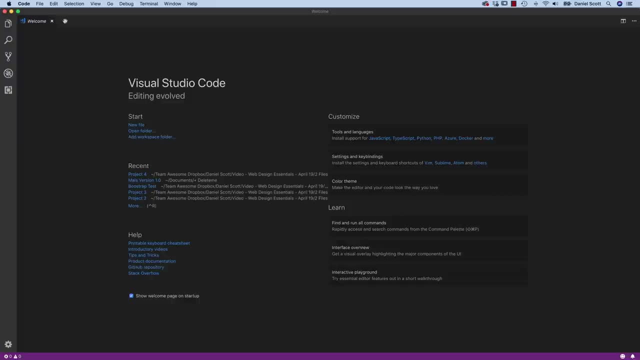 So just to make everything crystal clear and easy, close down any tabs along the top by hitting this little cross here. Click it once on all of them until you end up with this nice clean, clear application, The other difference you might have as well. 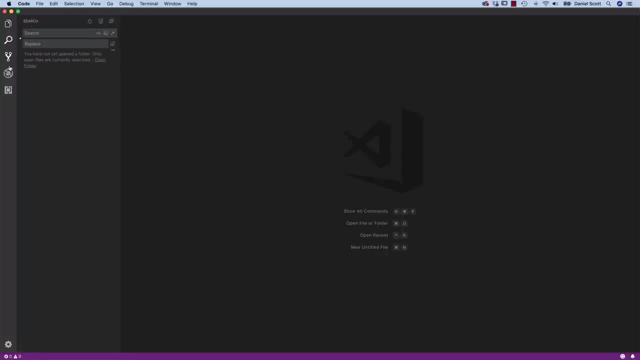 is along the side. here is a bunch of tabs. They're going to be helpful For the moment. if you click the top one once, twice, it disappears. It's all nice and clean. Let's go and create our first file. 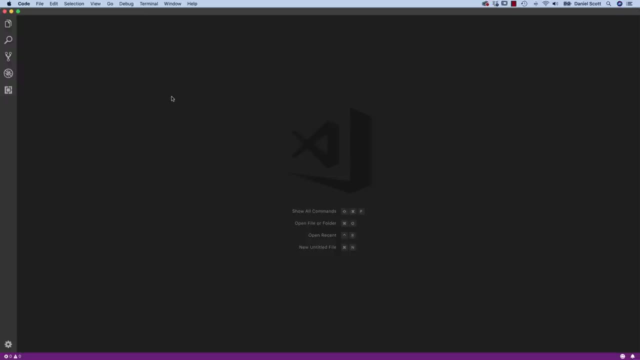 All right, to create our very first web page. it needs to go into a folder. It can't just be lying around in your Documents folder or on your Desktop. It has to go inside a folder And everything for that website needs to go in that same folder. 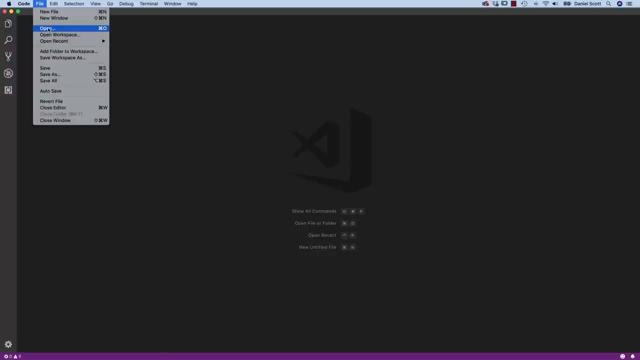 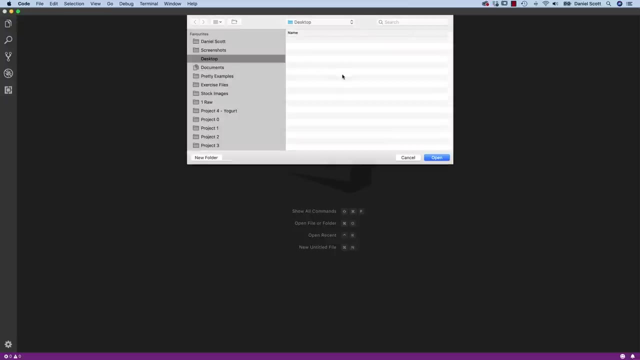 So to create that folder, let's go to File and let's go to Open, which is weird. Go to File, Open And it says: what folder do you want to open? We haven't created it yet, hold on. 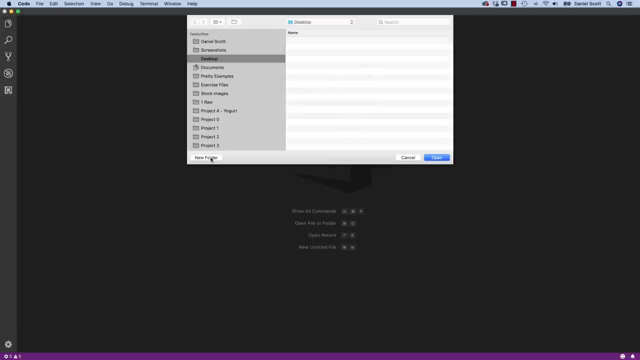 So what we do is on a Mac there's a New Folder button. On a PC it's slightly different. you're looking for that. it's a little new folder icon, I think it's a little yellow one with a little exclamation mark in the corner. 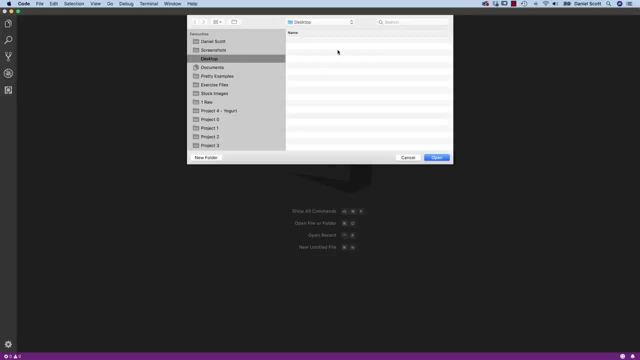 And decide where you're going to put it. For this course, I'm going to put it on my Desktop. Look how clean my Desktop is. I totally cleaned this up for this course. but anyway, Desktop New Folder- what are we going to call it? 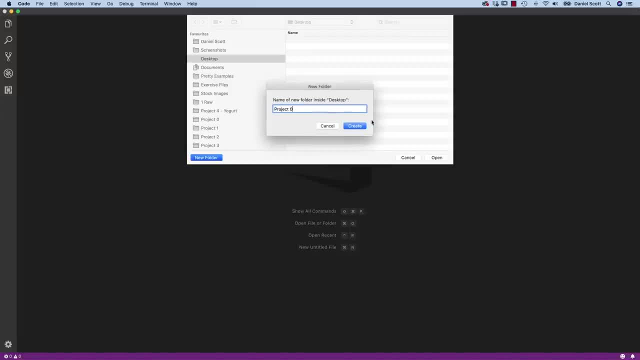 We're going to call it Project Zero, Click Create And that is my folder. I'm inside Project Zero. I'm going to click Open. Sometimes you have to kind of like select it and then click Open. You know it's right when you're on the top and it says: 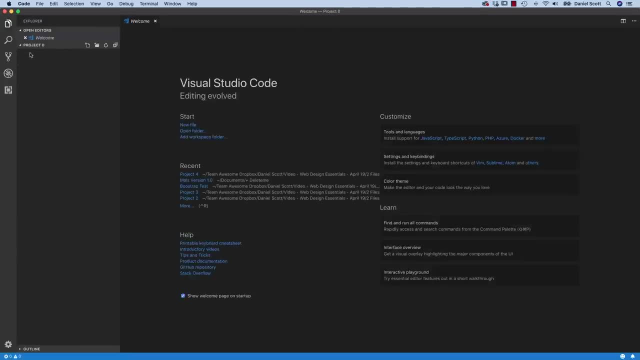 Welcome to Project Zero. along the top On the side here. it should have this option: Project Zero. There's nothing inside of it yet, But there's welcome screens. come back, go away. So we've got the folder and all it is on my Desktop. 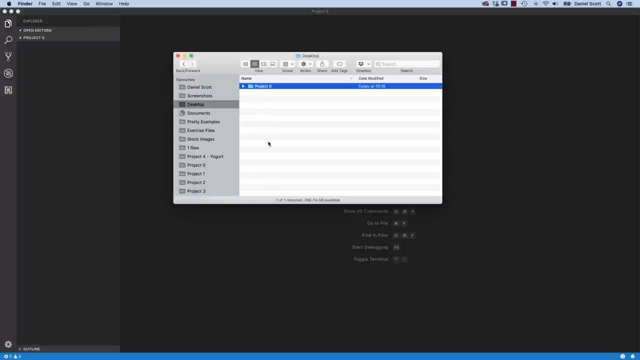 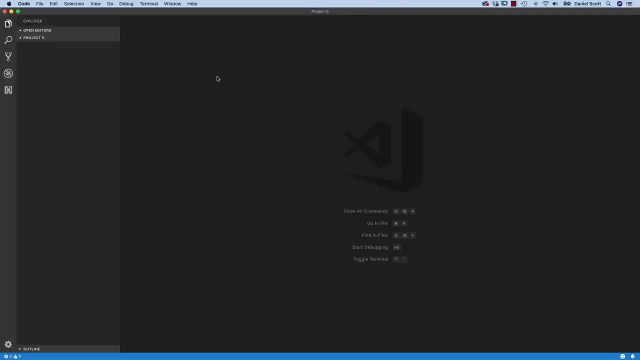 is, I have a folder with nothing in it, So we're just making a folder that way. It doesn't really matter how you create that folder, as long as it exists and you've pointed VS Code to it. Now we need to create our page. 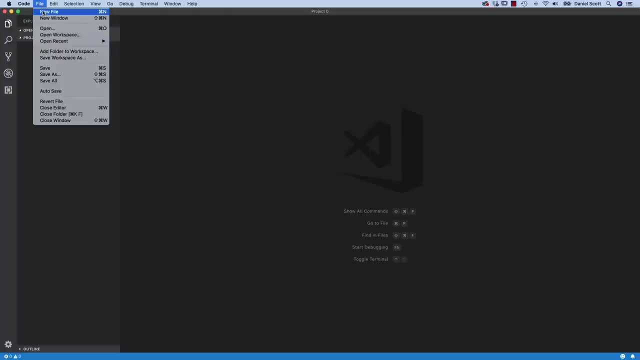 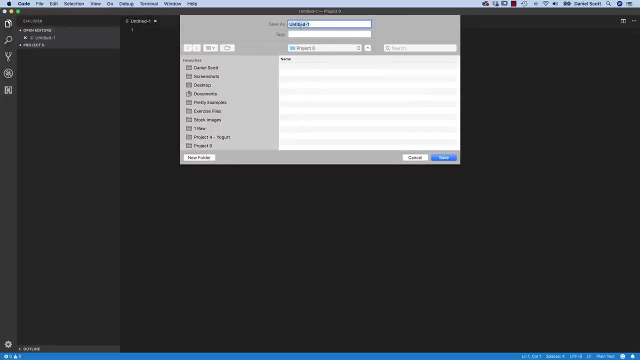 We're going to create our very first HTML page. Let's go to File. let's go to New File. We're going to save it. File Save. We're going to put it well. it should automatically know where to go. 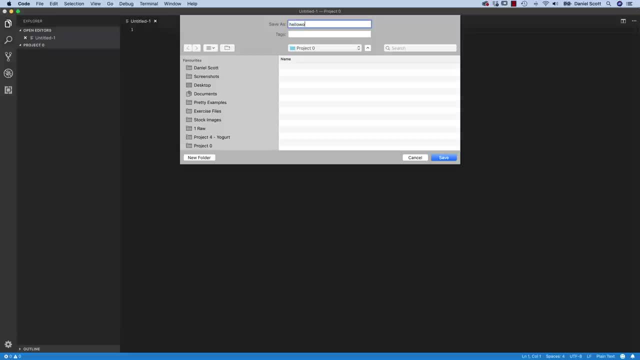 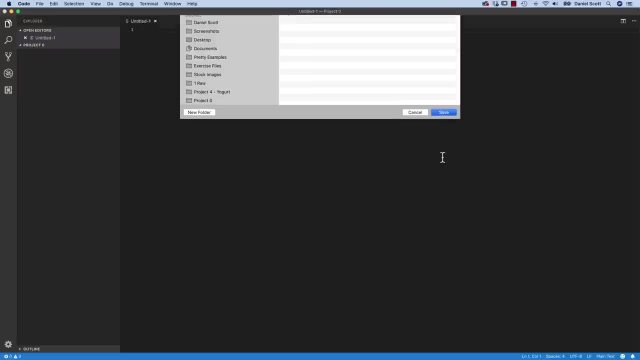 It's going into Project Zero. This one's going to be called HelloWorldhtml. Don't give it any spaces. one word and it has to be html. Let's click Save And just in here in our Editor, let's type HelloWorld. 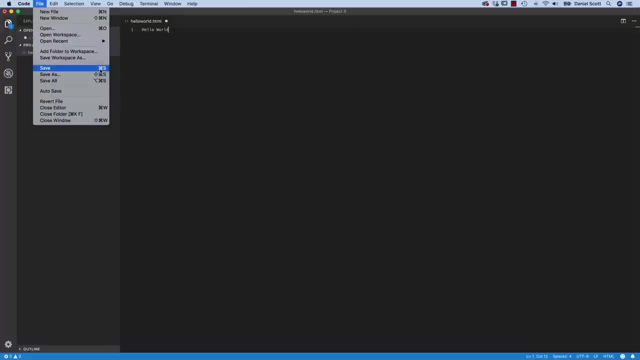 Let's go to File Save. I'm going to stop showing you the long way. So on my Mac it's Command S, on a PC it's Control S. I'm just going to say Save from now on. Now we need to work out how to preview this thing. 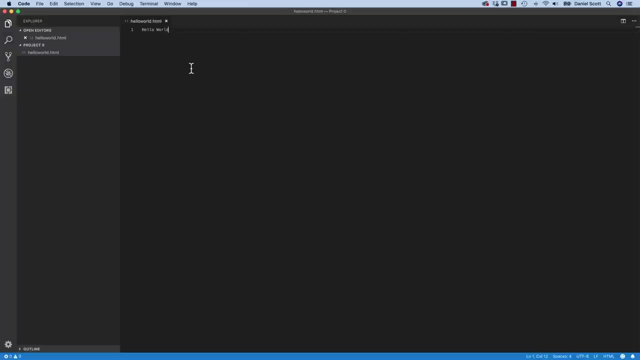 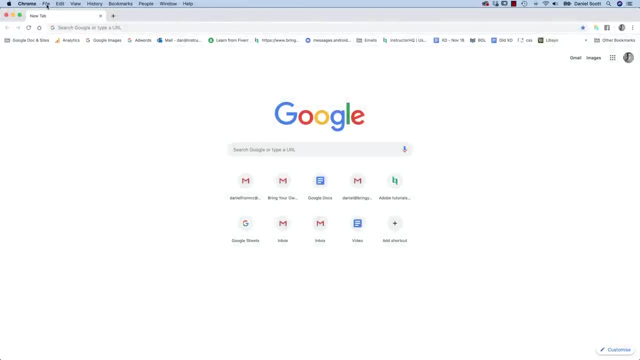 because we've made it. you've made a website, a tiny one, But how do we check it? We need to use that Google Chrome. So go in, open Google Chrome. So I've opened Google Chrome and we're going to go to File. 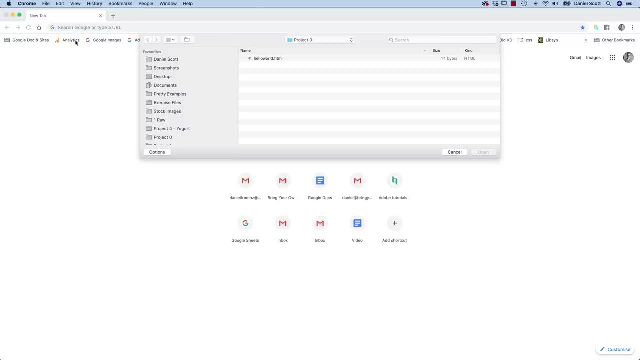 I'm going to go to Open File and then we're going to find our Project Zero. So on my Desktop, there it is there, Project Zero. inside of there, Hello World. before you click Open, remember this moment: If you've made a website before, it's not as exciting. 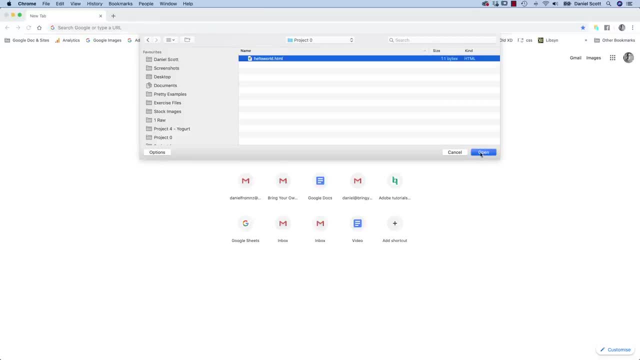 if this is your very first, get ready for this moment. It's a moment of glory. ready, That's it. That's your Hello World website. But look around, remember this moment. This is the first thing you've ever made. 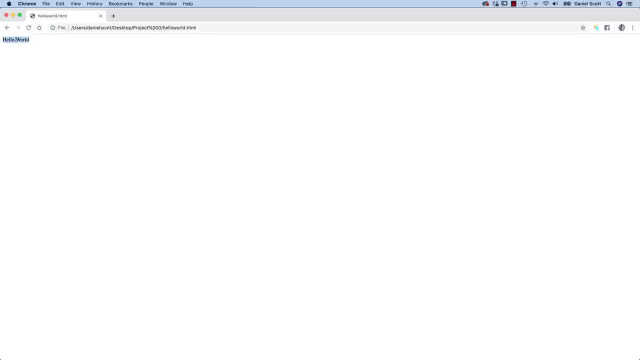 I remember when I made my first website. it was a little bit more exciting than Hello World. Yours will be too, And I'll show you the website that I made, my very first one a little while later. I think maybe if I show it to you here, you might turn the course off. 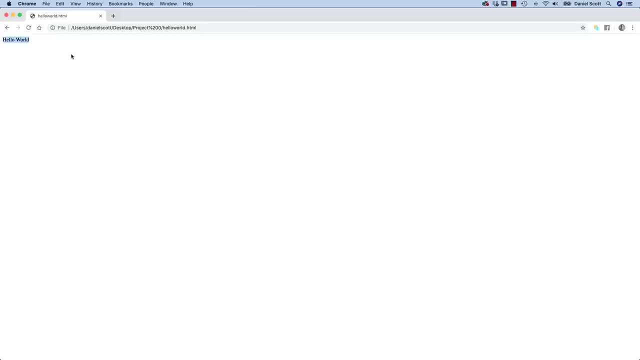 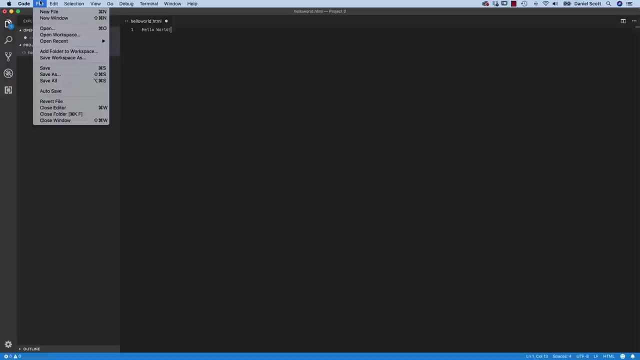 Anyway, it was bad, but it was 20 years ago. So let's recap the process Back into VS Code And in here we're going to put an exclamation mark, Then hit File Save. I promise not to show you the wrong way I did. 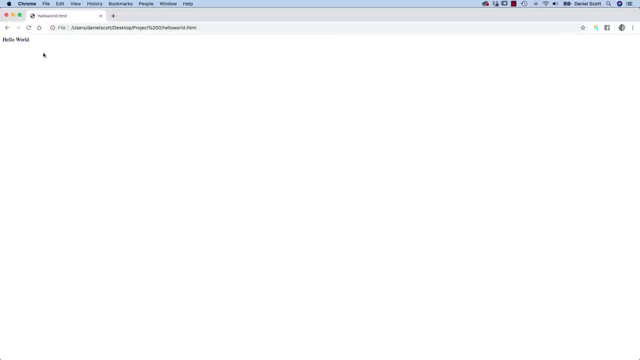 Then I go back to Google Chrome and it hasn't updated. So whenever you make a save or make a change in VS Code, hit this little refresh button or reload button. If you can't see it up there, it'll be somewhere. 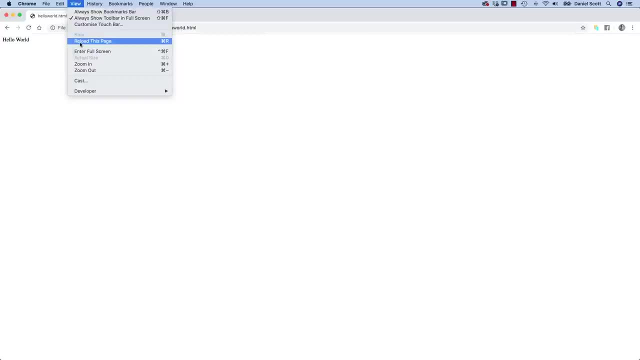 Where is reload? I don't even know the wrong way for reload. there it is there. So View Reload and there he is there- Exclamation mark. So that's the process. Do the coding in VS Code. Check your website in Chrome to make sure it's working. okay, it's not broken. 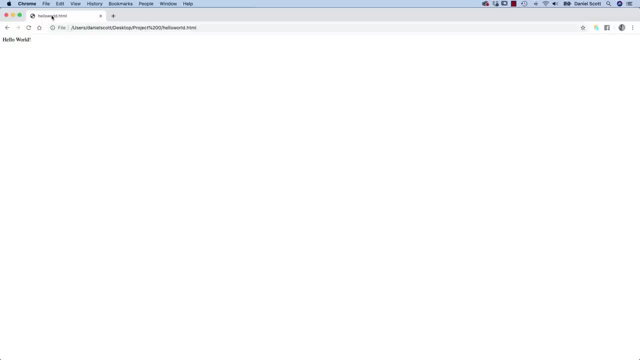 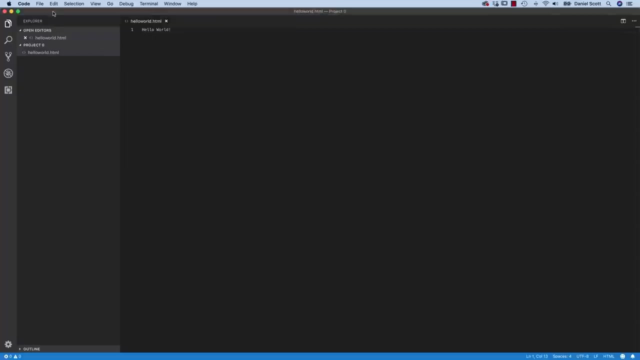 You do a little dance because you made a website. If yours broke during this process, it's a bad start, but it's okay. What probably happens is you forget to add the html If that happens, and you've just got something called Hello World, not html. 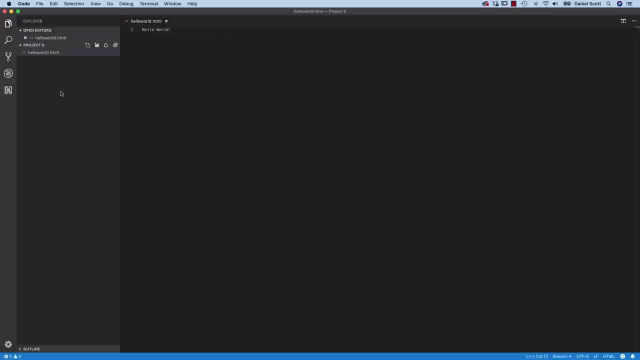 this will happen to you. you're like, of course I did. I followed you Dan Later on in this course. if you're new, that will happen to you, So all you do is over here in either one of them. 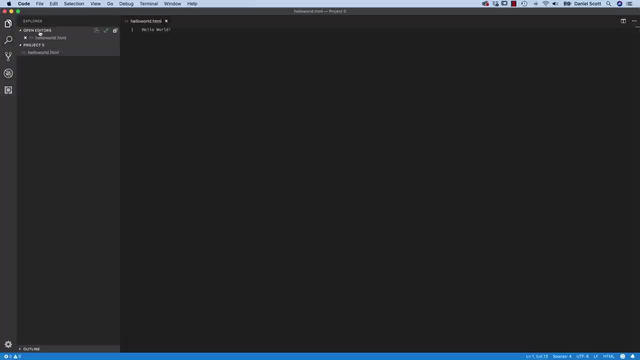 this can be a little confusing. this Explorer- This tells you all the pages you have open over here. This tells you every possible file in your folder. Now, the trouble with that is that you've only got one in each, So they just repeat each other anyway. 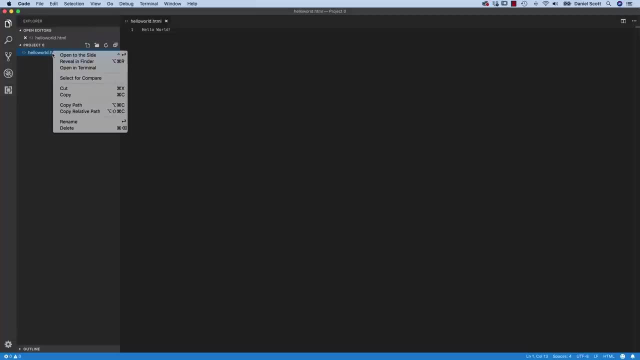 You can double click it over here. No, you can right click it and go to the one that says Rename and just say: actually, if it's missing html or you spelt it wrong, you can just type it in, hit return. then go and test that file in Chrome. 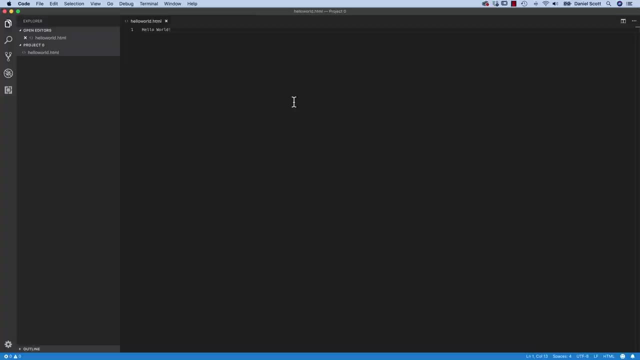 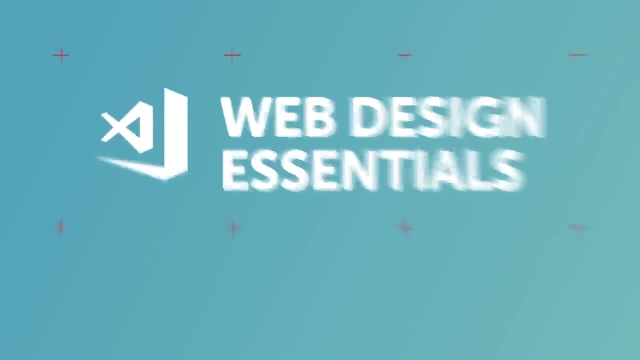 You should be fine. All right, that's not really web design. it's the start. Let's get on to the next video, where we actually start doing some proper HTML and some proper CSS. Hi there, this video is all about learning. 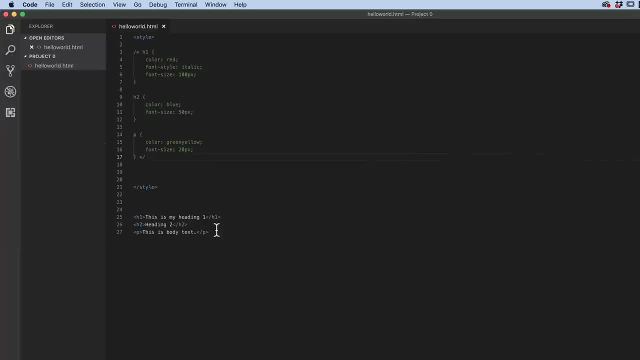 the absolute fundamentals of what HTML is versus what CSS is. You can skip this if you've got a basic understanding. We're going to do some real simple stuff here. We're going to add some HTML tags. it will look like that. 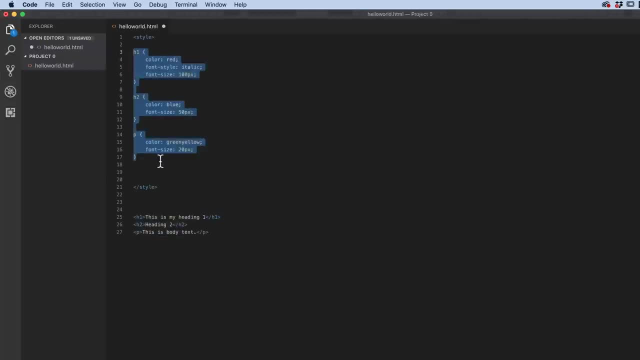 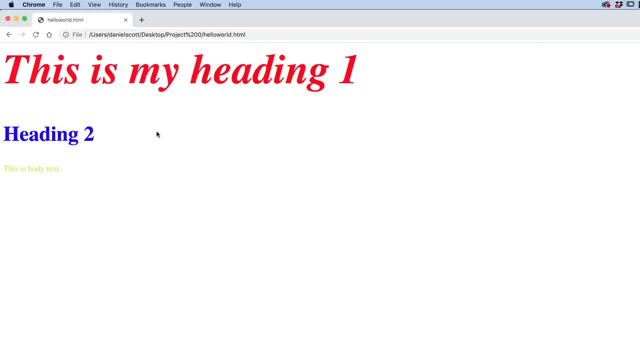 And then we'll style them using CSS And it will look like: here we go. that Better, A little worse, But you get the idea We're going to do HTML and then make it look pretty using CSS. Let's jump into the video and learn out how. 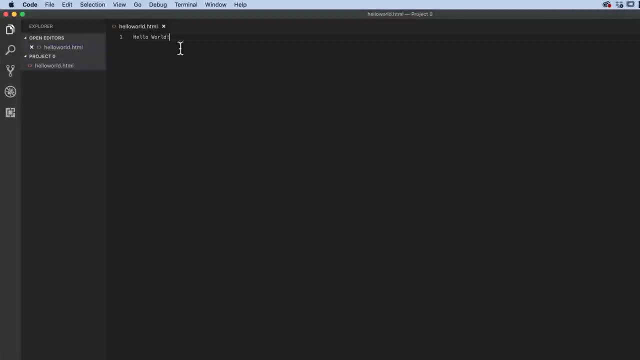 To get started, we're going to type our HTML first. So this word hello world is not HTML, it's just some plain old text we typed in, delete that. So when we write HTML we need to follow some syntax. 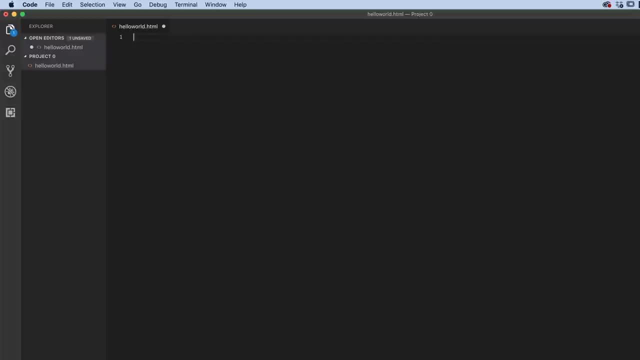 So we're going to put in something called a heading, And in this case a heading 1, the most important heading on our website, And in HTML it uses the abbreviation of H1.. Now we can't just type H1, we need to wrap it up in angle brackets. 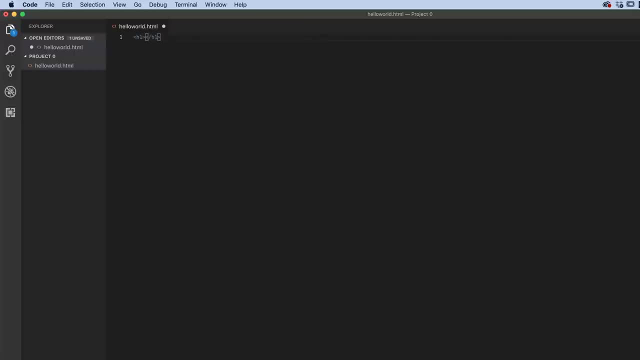 So open angle brackets- H1, and then close angle brackets. So you can see it there. it did a couple of things We typed in our H1, we put the brackets either side And you'll notice that VS Code automatically put in this extra closing tag. 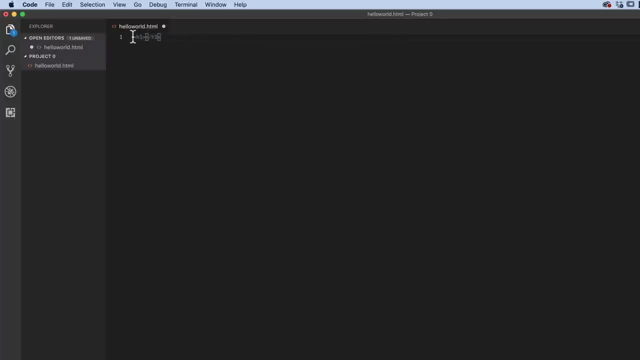 So that's how HTML works. it's a wrapper tag. It's a tag that goes around the beginning and the end and everything in the middle. This is my heading, Heading 1, even So, as long as there's H1 on one side, on the other side. 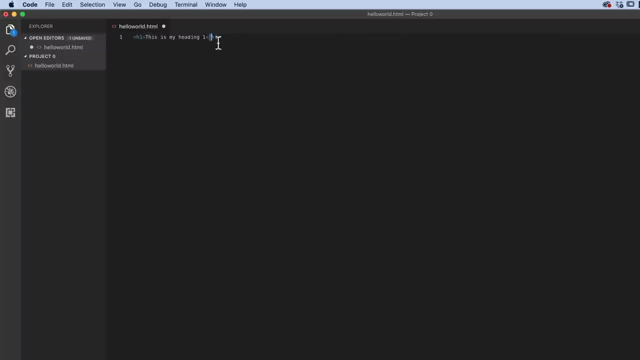 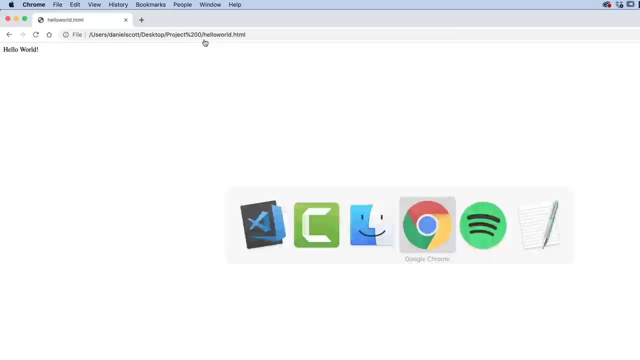 they're wrapped in angle brackets. The closing, you'll notice, has this forward slash And that tells the browser that this is my heading. Let's save it. let's check it in Google Chrome And you can see there refresh. 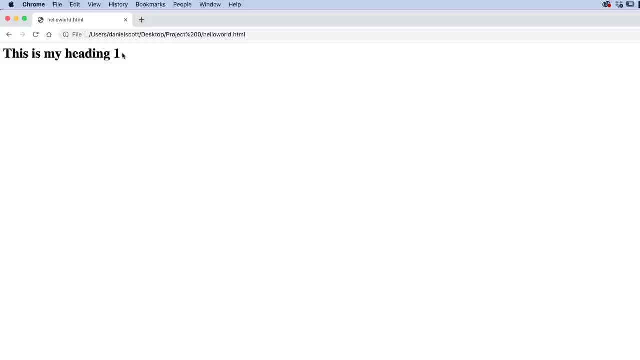 I've got my heading 1, it's big, it's bold, it is Times New Roman, it's black. That is a default setting for a heading 1.. Let's add a couple of other HTML tags. So in here we're going to return in. 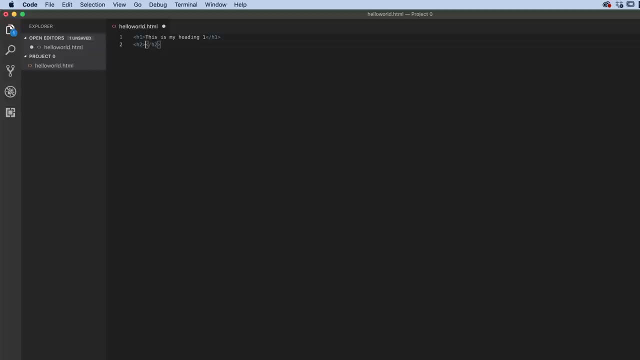 I'm going to type: angle brackets H2, close them. You'll see it puts in the extra syntax. If it doesn't, for whatever reason, you can just type it in. So I'm going to start typing. oh, it really wants to help out. thanks, VS Code. 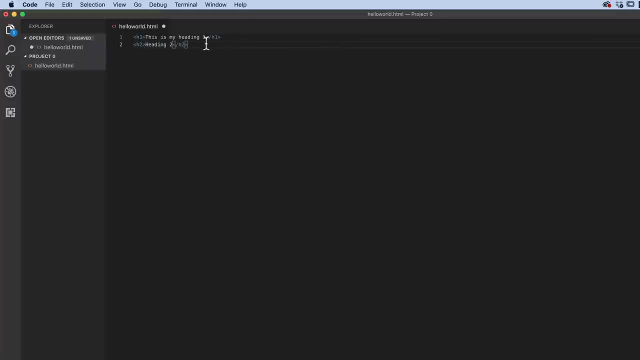 This let's just write heading 2.. So those are a couple of real basic HTML tags. Another really common one is a P tag, So angle brackets, P close it off, And this is like body tag, Body text. often you'll have a lot. 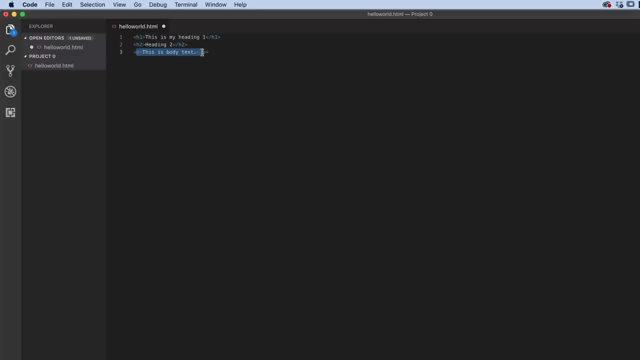 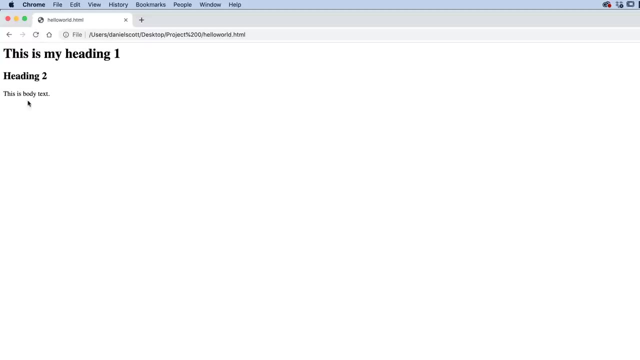 you'll have probably just one, each one, on your page, but you'll have lots of different paragraph text because it's the body text. Let's save it. check it in our browser: You can see. these are the default stylings for those three tags. 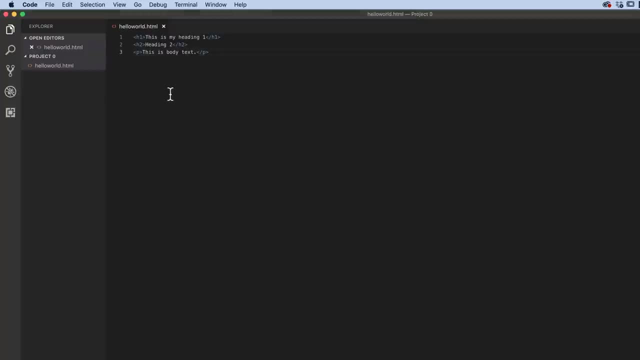 To override the styling. that's where CSS comes in. So what we need to do is our HTML is kind of like things on the page and our CSS is the styling of those things in the page. To make this work, let's put a couple of returns at the top here. 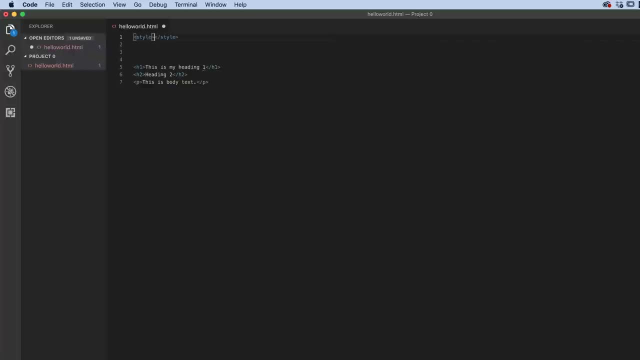 and type a tag called style, Close it off, and again it puts in the closing tag. And what I just did there is: I put in a few returns. Returns don't mean anything in code. You can have a million of them. 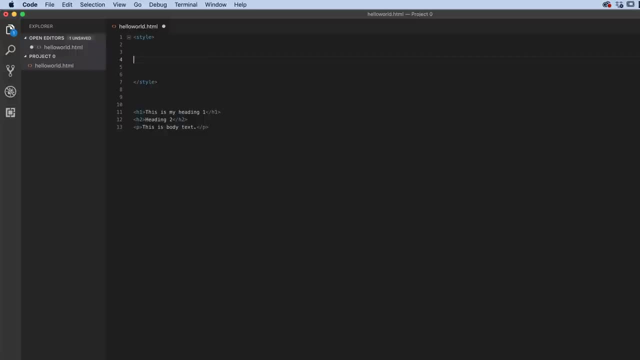 It won't display on the page. I just use a lot of returns when I'm styling things just to give some sort of visual breaking up of different parts, rather than trying to cram them all together, Because what you'll notice down here is if I delete this. 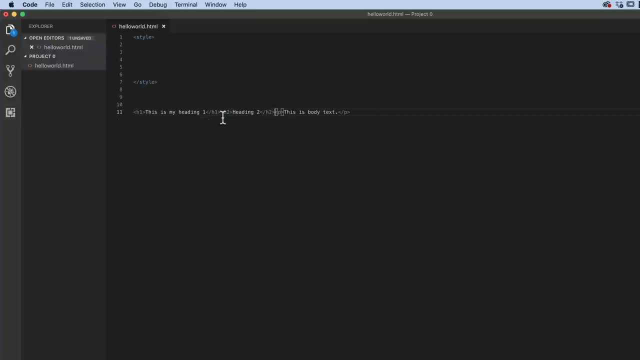 I'm just bringing it up so they're all on the same line. If I save it, you'll notice back here in Chrome. it's exactly the same, So it doesn't matter whether you put returns in here or not, except that it looks hard to work on. 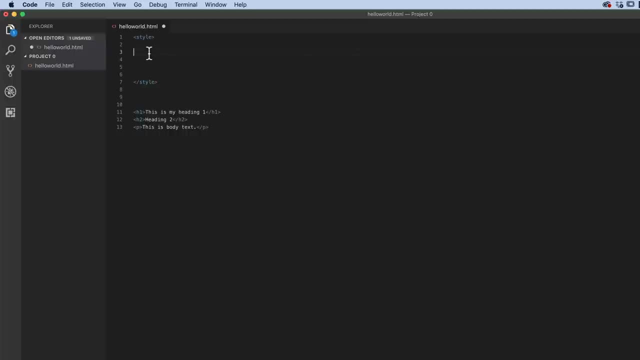 So in this style tag, this is where our CSS is going to go, And CSS has a different type of syntax. Whereas HTML had an opening, closing angle, brackets and a forward slash, there the CSS. you do things like this. you say: 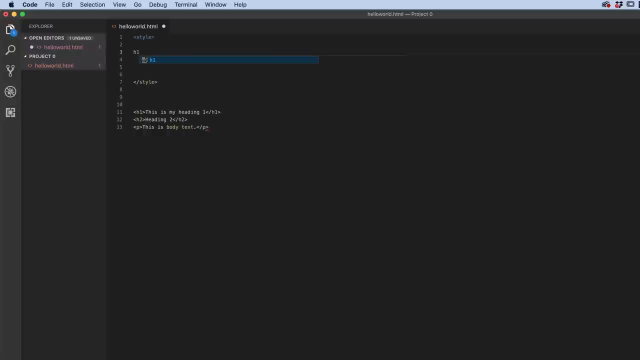 I want the H1, this is called the selector. I'm selecting the H1. Then you put it in a space and then put in the curly brackets rather than the angle brackets. I'm going to put a return in my curly brackets just to separate it out. 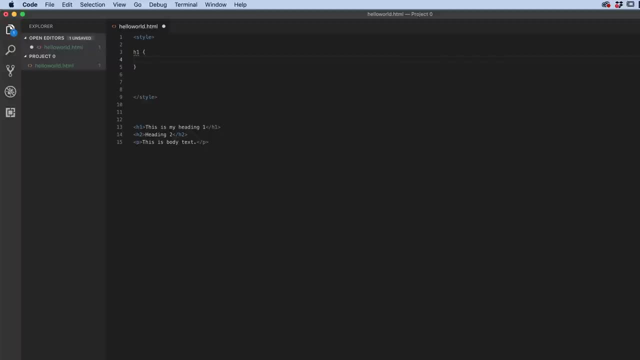 Not for any good reason other than it looks a little bit more easier to communicate to you. And in here I'm going to do some H1 styling And we'll start with color. We've got to spell it the American way. 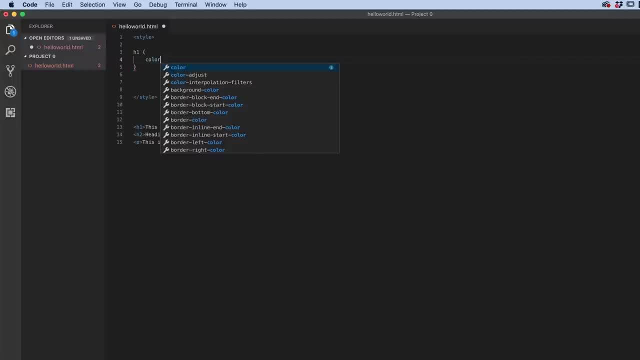 Color. and after this, this is the property. so selector, I'm selecting the H1.. I want to add the property color to it. it needs to end with a colon And then you pick a color. there's lots of default ones in there. 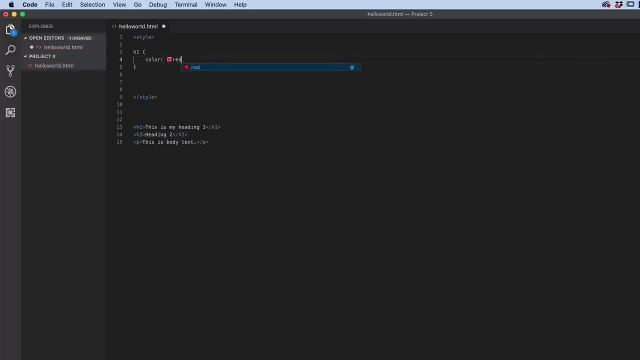 I'm just going to put a space in and type red And at the end of CSS you have to have a semi-colon, So curly braces, colon, semi-colon. That is the syntax pretty much for all of CSS. pretty simple. 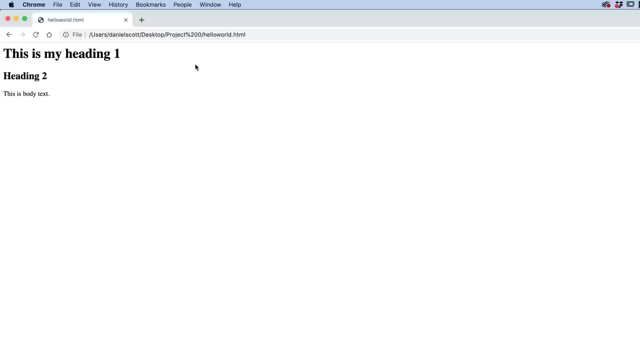 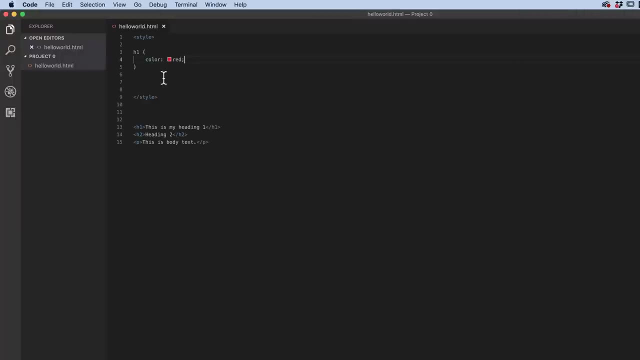 Save it and let's see if it works. Jump into the browser and refresh and look at that H1 is styled Now. I know this is not a huge amount we're doing here, but I'm excited. I'm excited for you. 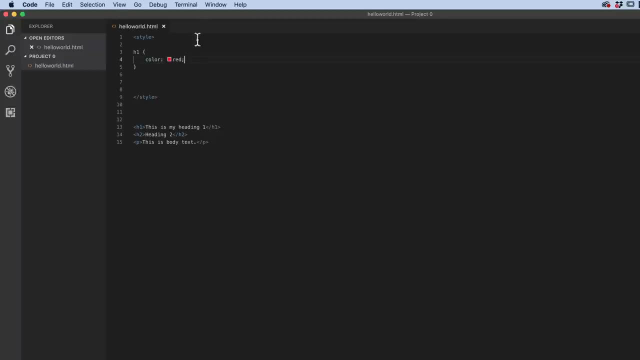 I remember learning this stuff and it was a revelation. So let's do something else. I'm going to put a return in here. So, if you want, we're going to group CSS. We want to do a few things to the H1.. 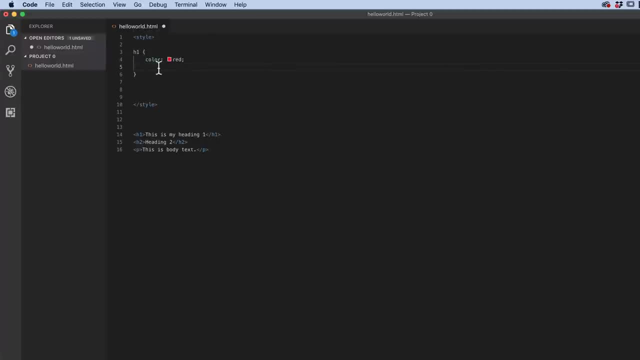 So, as long as it's within these curly braces, we can type in something like font. I'm going to put in font style. You can see VS Code really wants to help you kind of suggest things You're like size style. 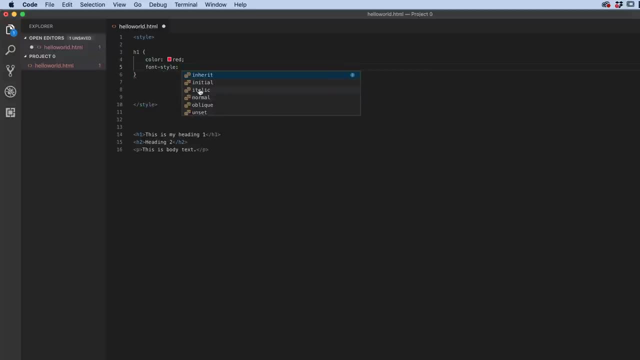 Display. I'm going to use style. I'm using my mouse now instead of typing it in. That's just one of the little helpful things you can do with VS Code, Or you can use your arrow keys on your keyboard. Can you see that little blue line moving around? 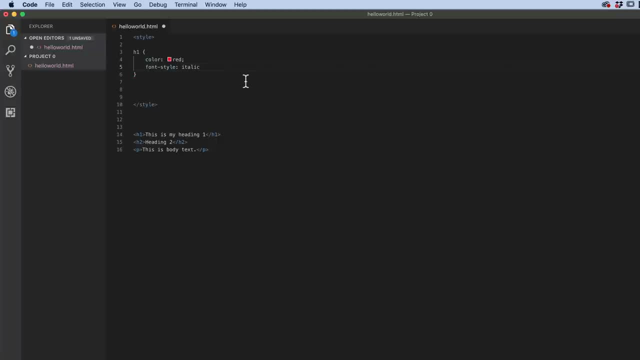 I can go to there and hit return on my keyboard. We've got almost all of it, So we've got our property. there's the colon. We've got our actual value, which is italics, And what goes at the end. 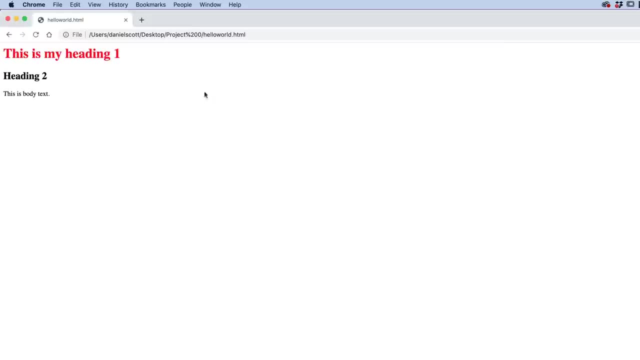 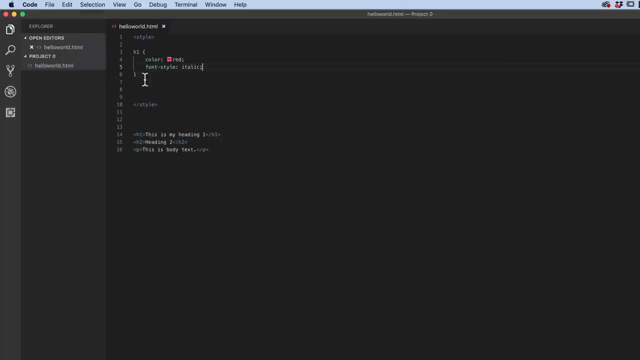 You got it semi-colon. Let's hit save. let's see what it does. Let's hit refresh. Oh, it's italics and it's red and it's an H1, brilliant. So I'm going to set a class exercise now. 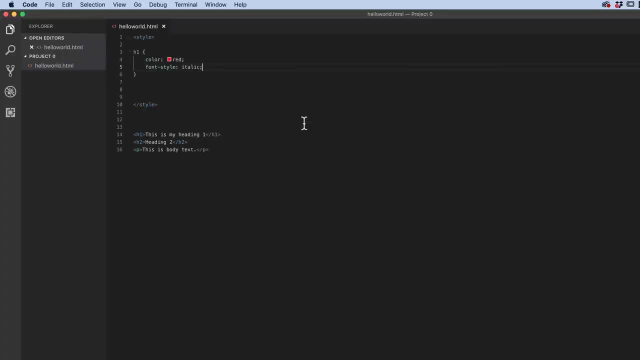 I want you to change this H1 to be a font size of 100 pixels or PX. I'd like you to pause it right now. go hit the button And I want you to see if you can do that Font size at 100 pixels. give it a go. 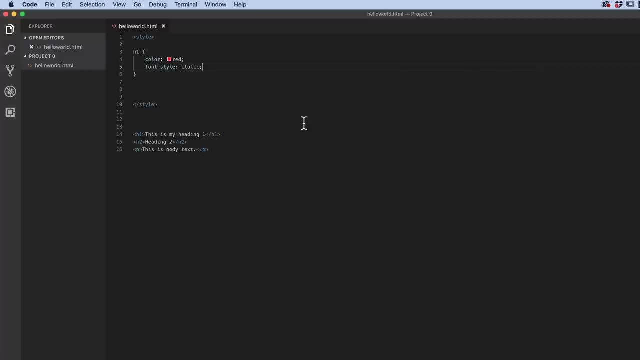 I'll give you a hand in a second pause. go. You may or may not have paused. You may or may not have made it work. Let's see if you followed me. So font Size, here we go, got a colon. 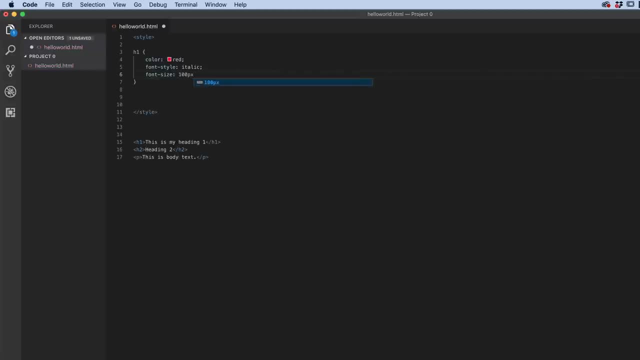 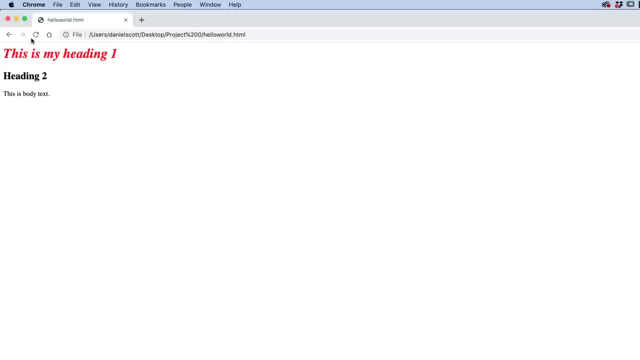 Then put in 100.. And what people often forget is you need the PX. We use pixels when we're dealing with fonts at the moment. What goes at the end Semi-colon? Save it back into here: refresh. Look at that giant H1.. 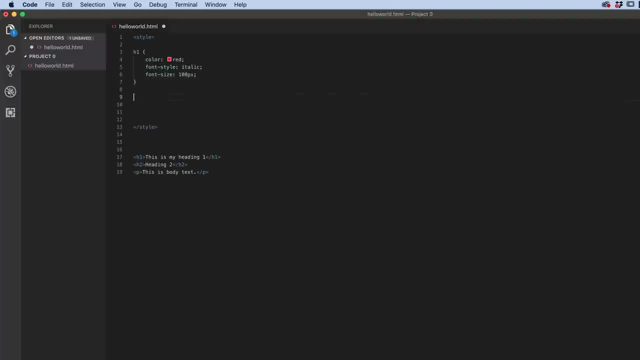 Let's style the H2 together And then I'll set another little exercise. So H1, now I put a couple of returns in here. Curly braces: You can kind of separate them up using these kind of the selector, then the curly brackets. 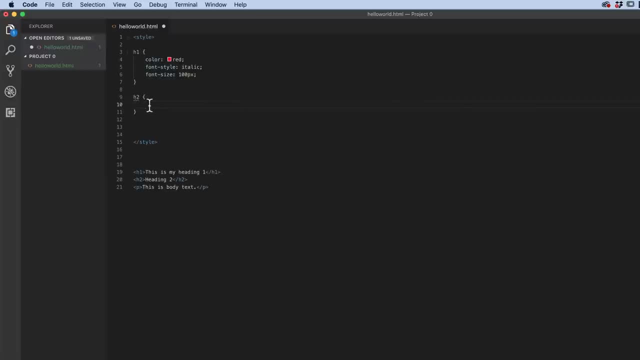 And everything goes in the middle that you want to do to that particular selector. So in this case, we're going to do a color of, we'll do color blue semi-colon And we'll do a font size. font size of 50 pixels. 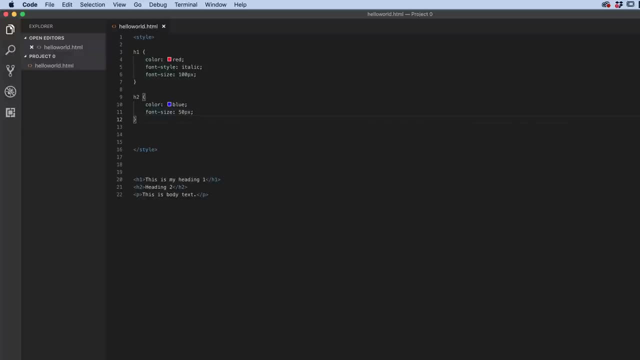 So give that a go now, And I'm going to set a verbal exercise. I want you to try and do the P tag all by yourself. I want you to make it green and I'd like to have a font size of 20 pixels. 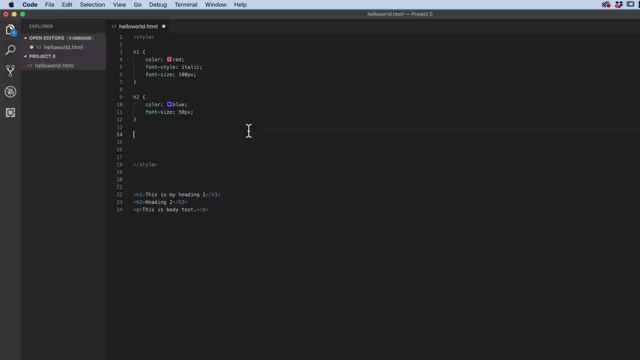 Give it a pause now see how you go and pause. All right, how did that go? I hope you did well, let's follow it together. P tag curly braces. color of green: There's a few different greens. 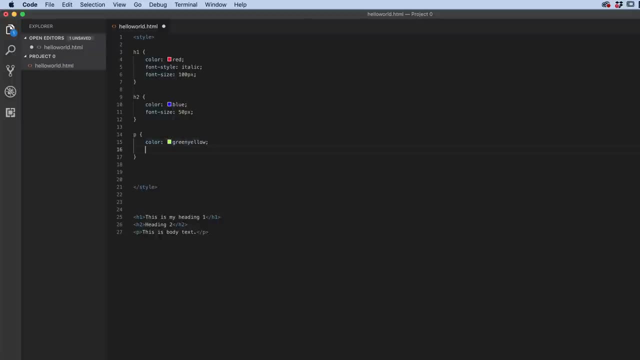 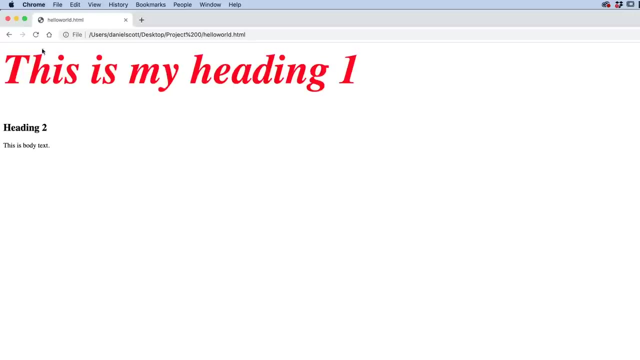 Yellow, green, green, yellow- that's my one Semi-colon and we're going to put in a font size of 20 pixels Semi-colon. save back into here. refresh. Look at all that good stuff. 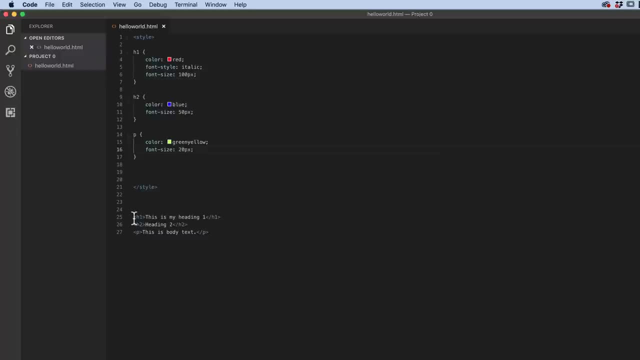 So that's just an introduction to what HTML is and what the syntax looks like. These are these guys down here And the styling of them. We talk about selectors. I use the kind of nerdy words here so that it becomes a bit more natural for you. 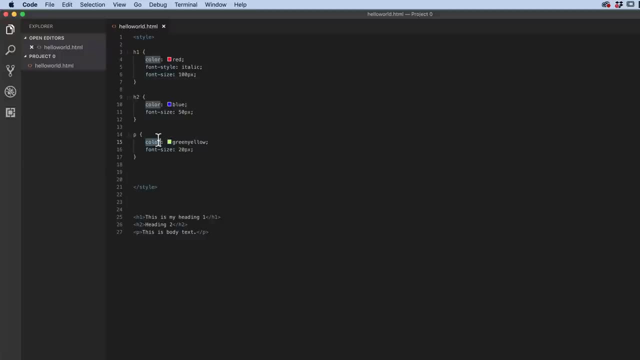 So the selector, this is the attribute. No, that's the property and that's the value of that property. And that's the basics of websites. We're just going to expand on that. We'll build some boxes to put this stuff in. 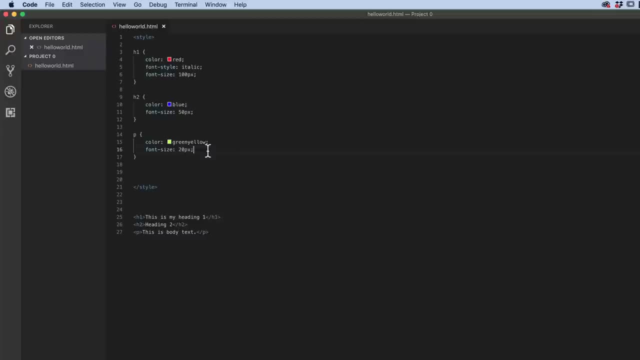 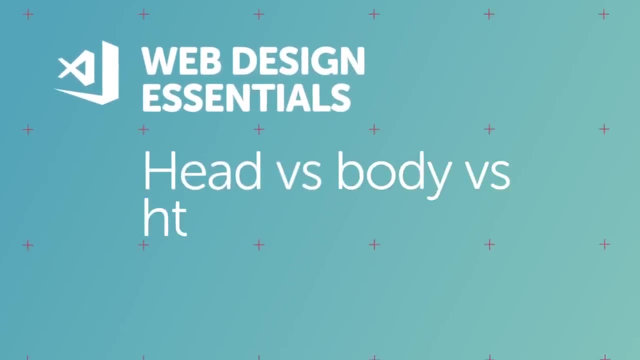 We'll start doing some interactive bits and pieces. But yeah, that's the fundamentals of HTML and CSS. Let's jump into the next video. It is time to make an actual, proper website. The moment, we've put in some HTML tags and some basic CSS. 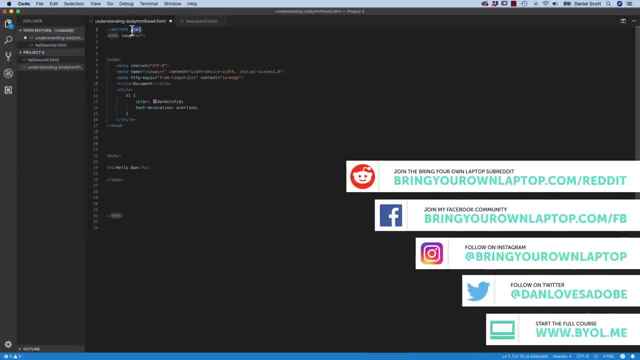 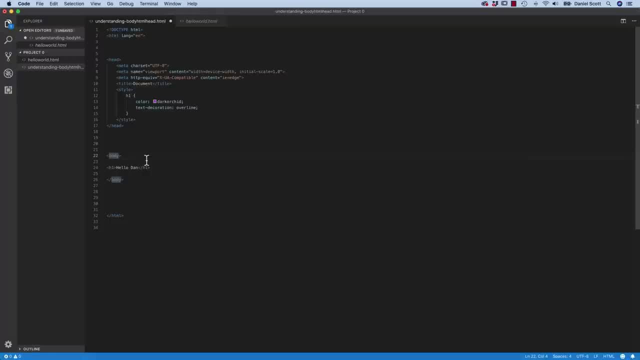 But that's not all we need. We need some other bits and pieces, like the doc type, The head tag, the body tag. So in this video we'll work out how to add those quickly and what they all do. Let's jump in. 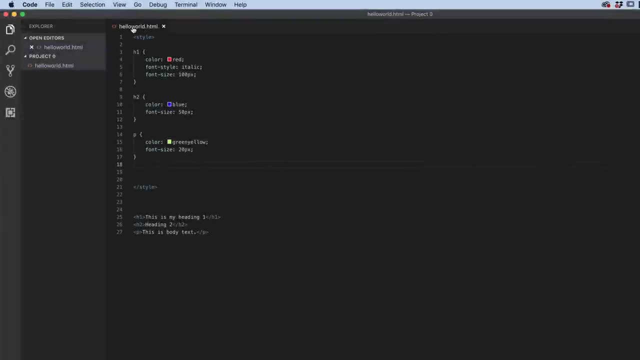 First thing is: is that this page that we've made this Hello World HTML? it's got the basics in it, but it's missing a chunk of elements to make it an official web page. So let's close it down and look at those. 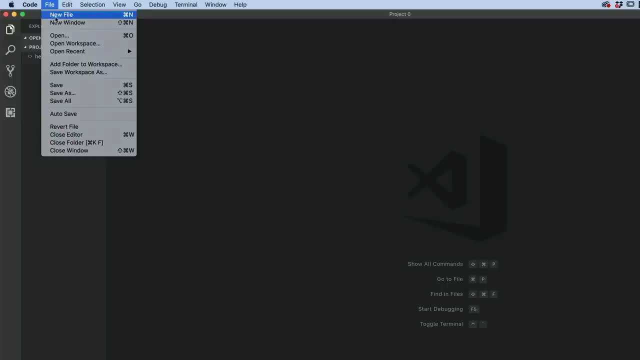 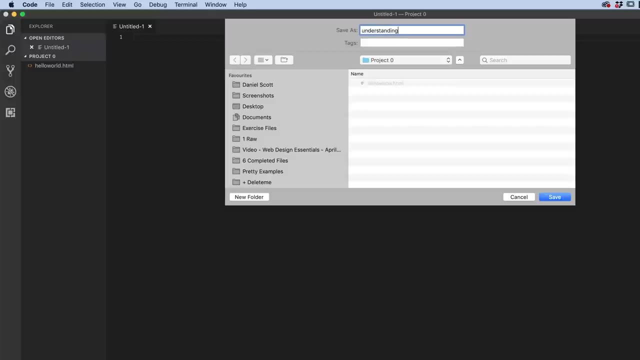 Close it down. let's make a new page, so File New. Let's save it. This one's going to be called Understanding. Let's put in a hyphen and let's put in body HTML and head. 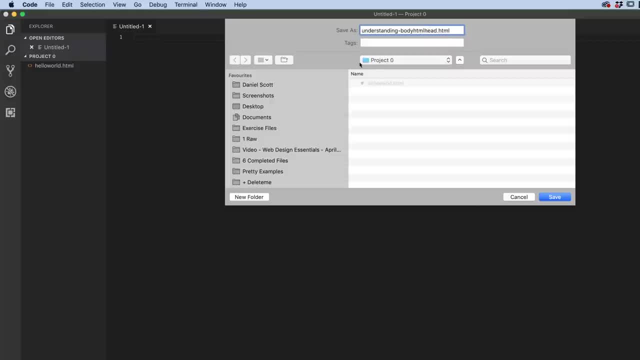 Make sure at the end you add HTML: html At the end, otherwise it doesn't know what you're doing. The other thing to notice at this point is that you can't use spaces, or you shouldn't use spaces. You need to use hyphens or underscores, it doesn't matter which. 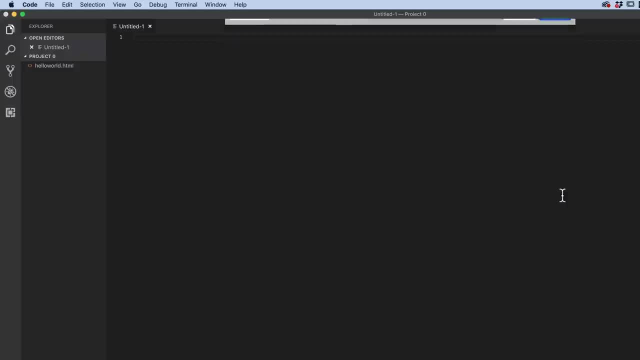 I use hyphens and let's hit save When you are naming things, try not to use things like dollar signs or ampersands or any kind of. just use numbers and letters To make this an official web page. 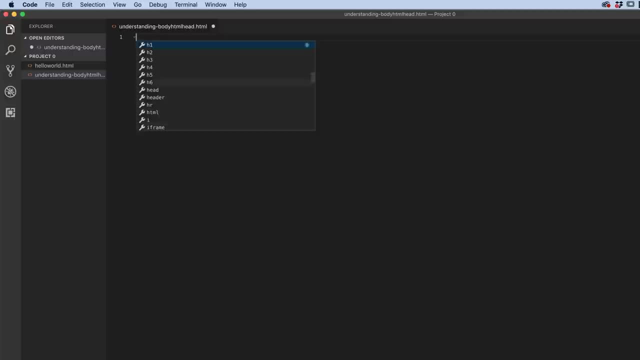 it needs a couple of things. It needs to know that we're dealing with an HTML page, so it's something called the Doctype, So it's a Doctype of HTML. Then we need to establish that it is an HTML document that is set in the language of English. 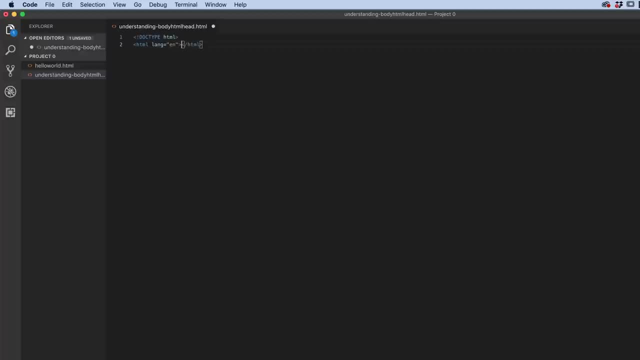 Close that off, And there is probably another five or six lines that we need to add to make this thing official. So we don't type that out. There is an easy shortcut because it's such a consistent, repeatable thing that everyone needs to do. 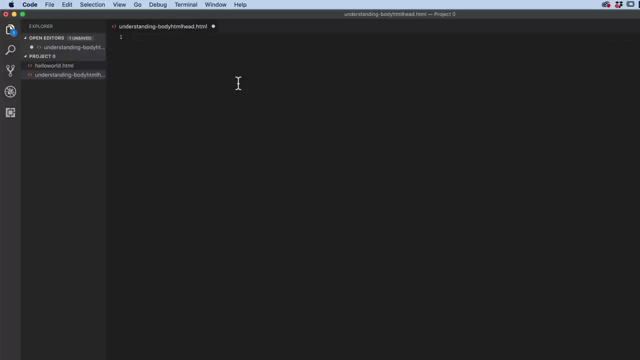 VS Code uses something called Emmet. Don't worry that Emmet's the word, but it's a little bit of code hinting that really helps you go fast. So instead of typing all the things we need out to make an official web page, 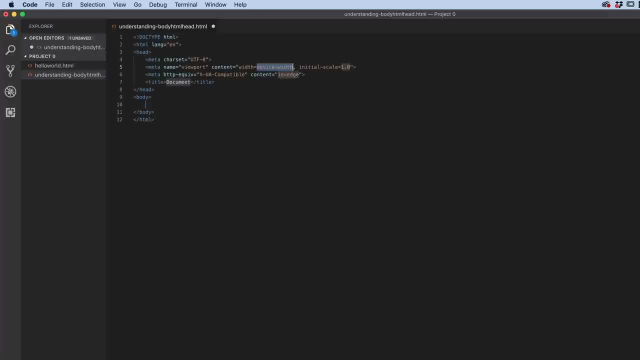 we type an exclamation mark and we hit return on our keyboard. Cool, that's all the official stuff. we need to make this a legitimate HTML page. There's our Doctype. there's the English language. it has something called the head and the body. 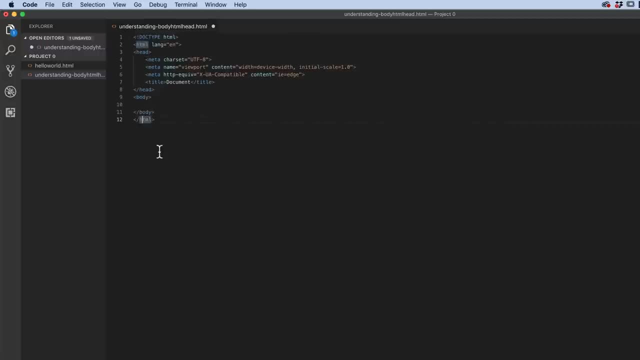 and then it's all wrapped up in this HTML tag. Now, what are all these things? So the Doctype just tells us that it's HTML. This one here. if you see, if I click in here HTML, you'll see there's a corresponding wrapper at the end here. 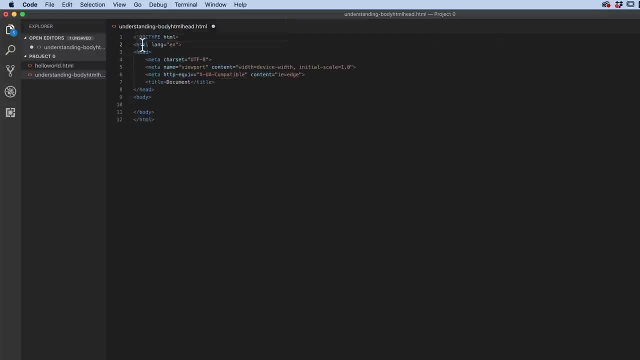 And all of the website is inside that HTML tag, Like we had the H1 earlier. remember we had H1. and there was a beginning and a closing and everything inside inside was the H1. It's the same with all of the HTML tags. 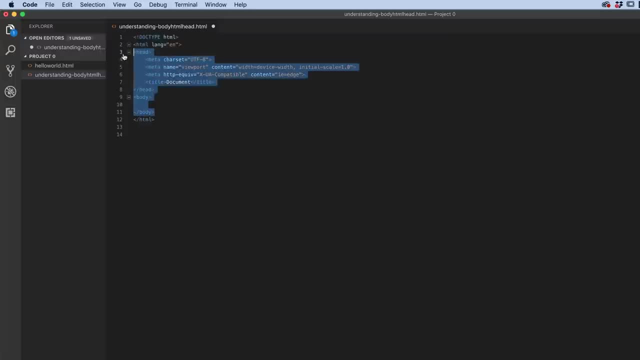 This one just says: all of this is HTML. thank you very much. Not a very exciting HTML tag. you're not going to deal with it much at all. These other two tags inside of here you will. There's the head, there's the body. 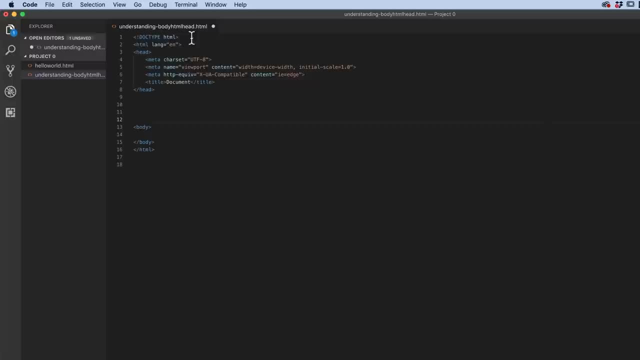 So the head tag. I'm going to put a couple of returns in- Remember, returns don't mean anything- just so that we can segment them when we're learning. So the head has an opening and a closing and everything inside of here. 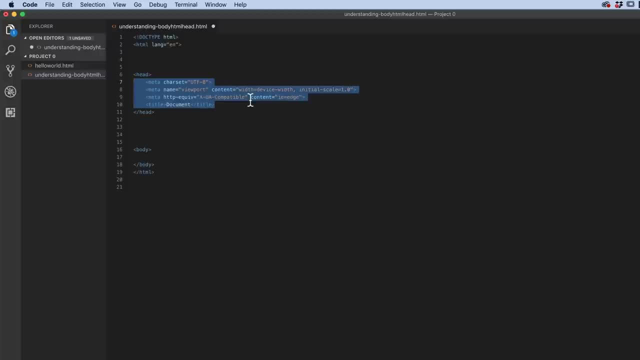 is stuff that the browser needs to work. So Chrome needs that. It needs this stuff, but the user doesn't see it. So if we save this File Save, we jump out to Chrome. We'll go to File. we'll go to Open File. 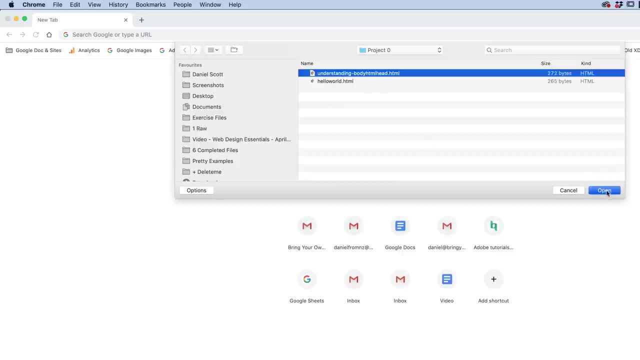 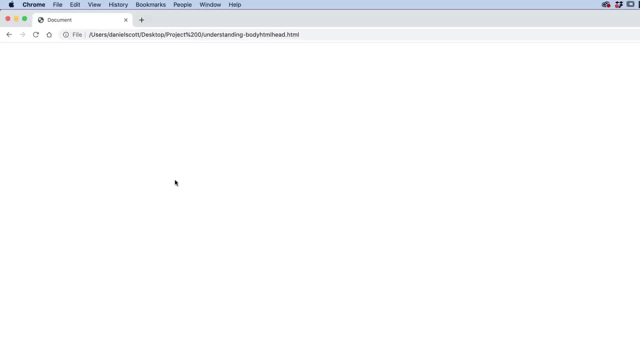 And let's find this new one. Understanding Body HTML Head, You'll notice that there's nothing on the page. So this is the body. there's a white square down the bottom. that's the body. The head is stuff that the browser absorbs but doesn't show you. 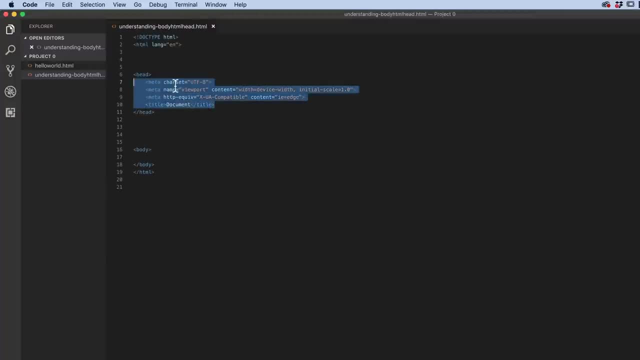 You can see there's lots of stuff that just doesn't show. I'm going to deal with all of this sort of stuff later on, but the basics here. this one here, the character set, it's just telling it we're using kind of a Latin keyboard. 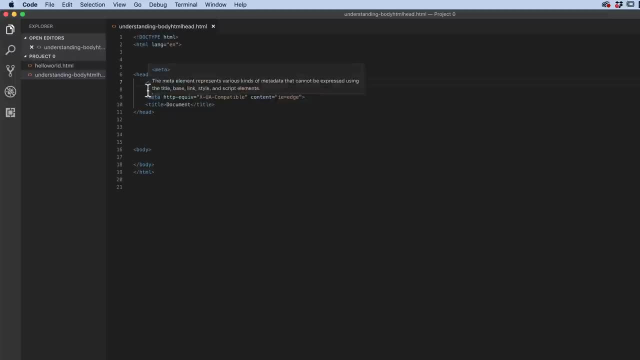 A, B, C, 1,, 2,, 3.. And we'll talk about these things later on. Responsive design needs this. There's some problems with Microsoft Edge that it needs to be compatible with things. The document title we'll do in the very next video. 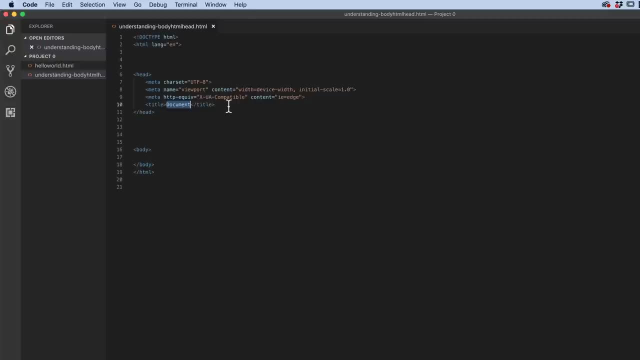 but it's all stuff that the browser needs, that we don't really need to, that the user, our audience, doesn't need to see. What the audience needs to see is everything in the body, So I put a couple of returns in here. loads too many returns, Dan. 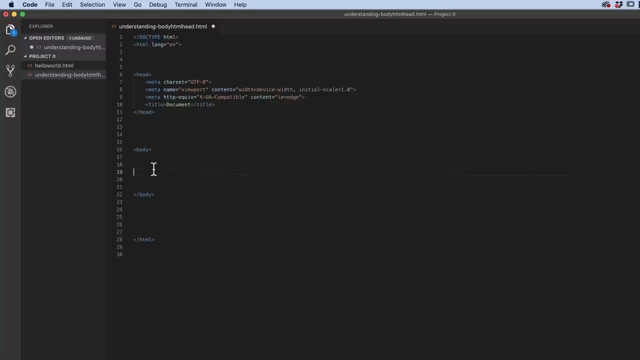 But in the body, this is where we add stuff, So let's add an H1.. So we're going to type in angle brackets H1,, close it off, And in here is hello, Dan, or your name. We're going to save it. 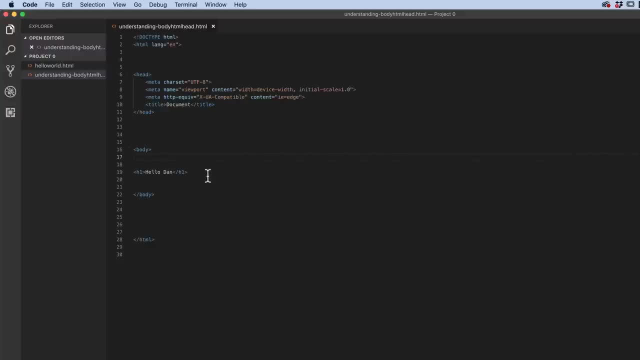 So everything in the head browser doesn't see Everything in the body actually gets seen by the user. So let's have a look in our browser, Let's refresh there. it is there, Cool, So HTML Everything's inside of there. 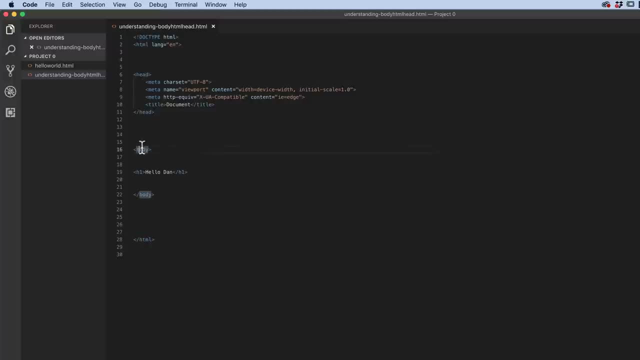 Head stuff that the browser needs to work. Body is the stuff that the user sees. Those are our three main tags. Now let's do a couple of things. Let's look at the head tag. So remember, we want to style this H1.. 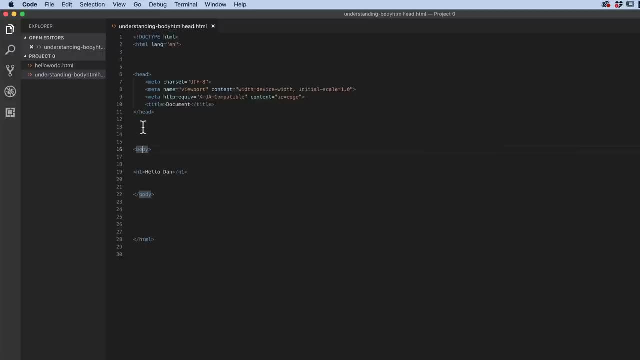 Where does the style go? We don't put it in the body, We don't put it in between the head and the body, It goes inside the head. So after the title put in a return, Then we can put it in our style. 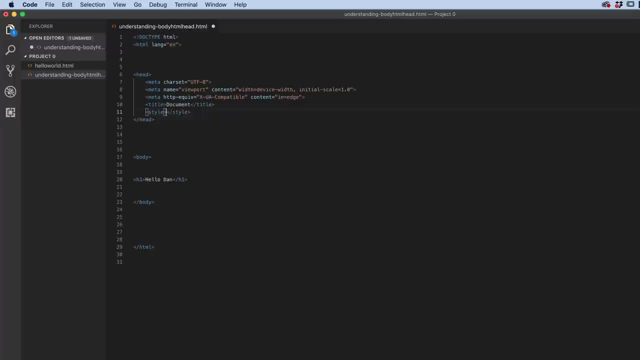 So remember, open square brackets, close it off And return between the two. Everything in between these two tags is the CSS, And the CSS can go in the head. We don't really want this code appearing on the page. We want it just to affect the stuff that's in the body. 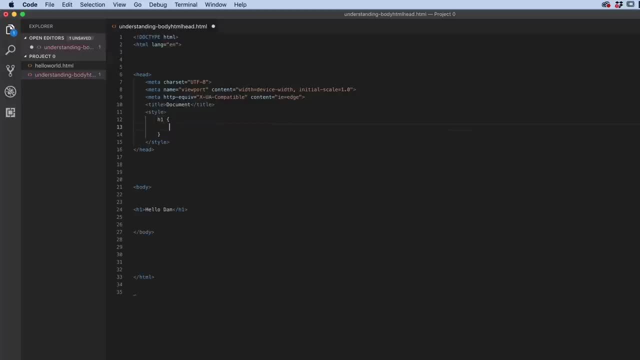 So we say, remember our syntax: H1, curly braces. And we say we'll make it the color of random color from this list: Dark Orchard. there we go. What goes at the end, Semicolon, Save it. let's have a little look in the browser. 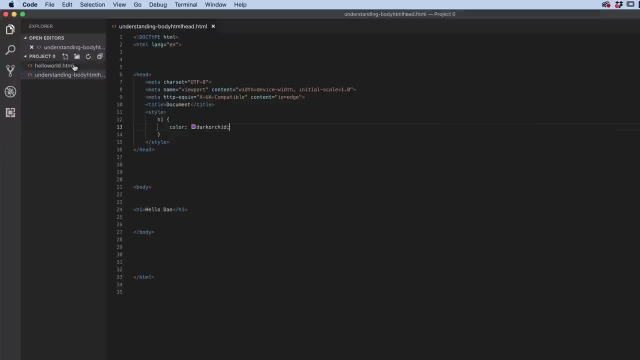 Browser refresh. Awesome Dark Orchard, Orchard, Orchard, Orchard, So head stuff that goes on the page. I've said this 20 times now, but you get the idea. Things like this can go in the head, But the thing people see are in the body. 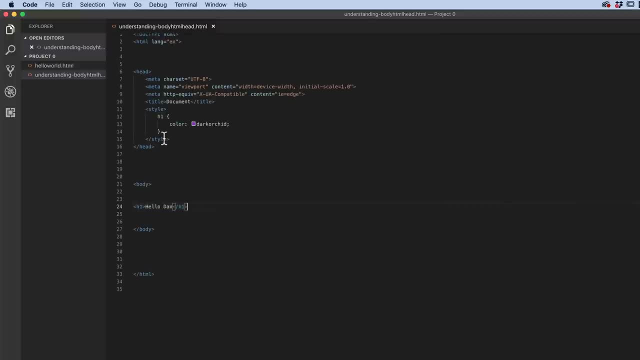 Now a couple of things I want to explain before we move on. is: I'm jumping between these two and you're like: how did he do that? So on a Mac you can hold down the Command key and hit Tab and these little things open up. 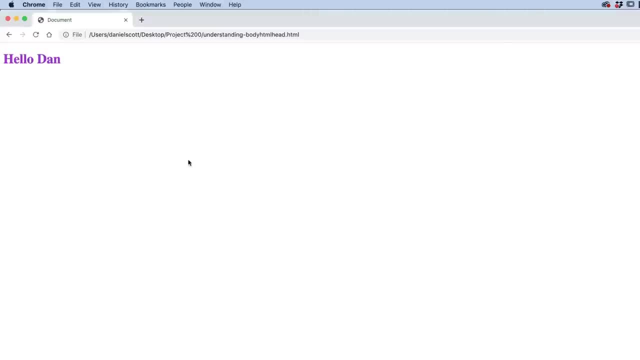 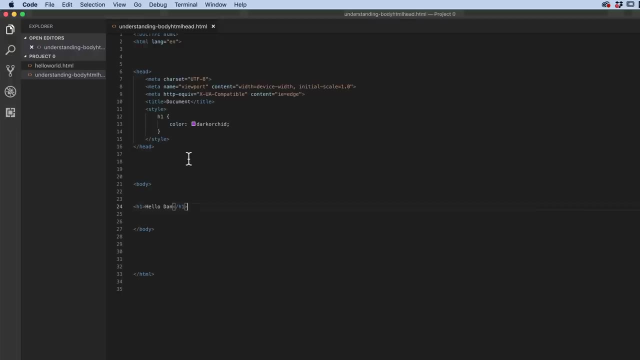 And you can keep hitting Tab to move through them. On a PC it's Control Tab, And you can flip between them too by just tapping them. So Control Tab, Control Tab. You don't have to do that. 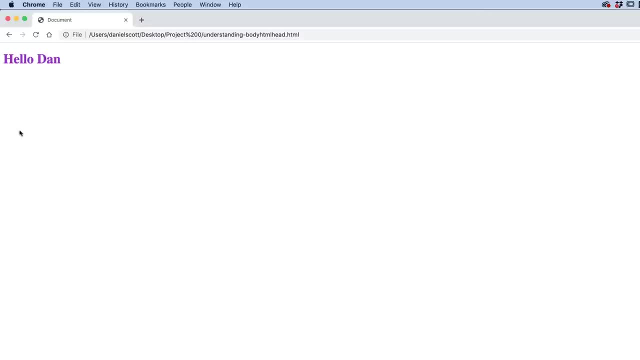 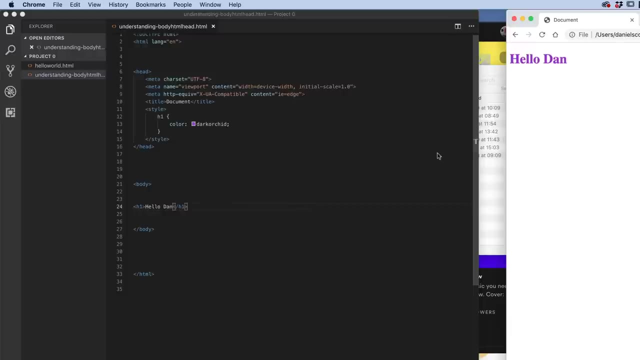 What you might do is just have it over here, Do some window resizing So you can kind of see one on one side, one on the other, And it's a lot easier to work that way up to you. And another thing I want to do: 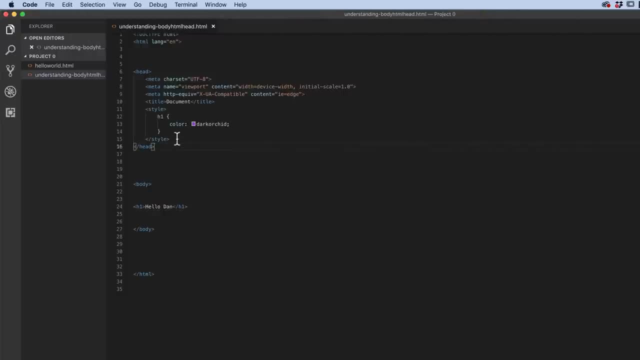 before we move on, I'm going to totally wreck, that is that I don't want you, at this point, to go back. how am I going to remember all of these things? Because let's say that I want to make this. Hello, Dan, underlined. 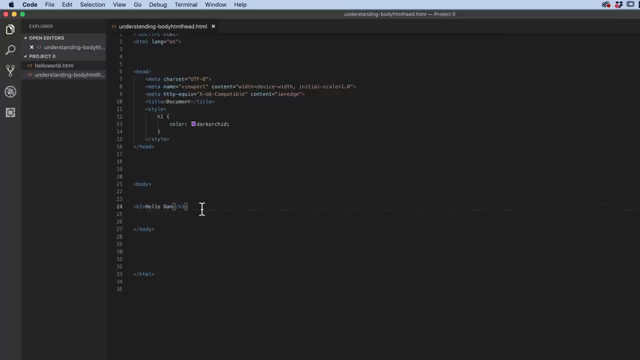 The cool thing about the Internet, and especially HTML, is there's a load of resources, So I want to make this underlined. What is it So? do I go in here and just start typing? underline Doesn't seem to work. 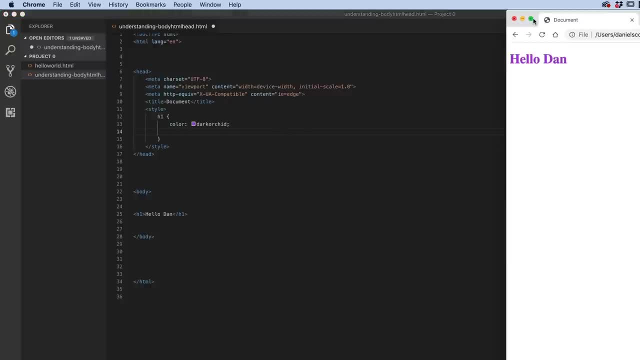 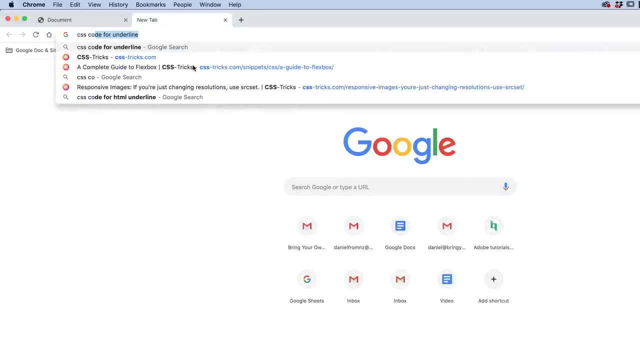 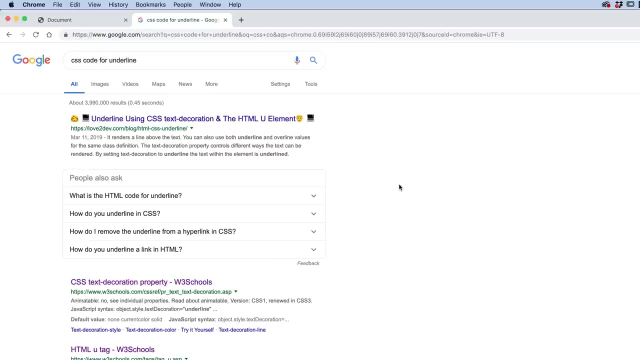 So let's say, I go to Chrome, Open that up again. I'm going to make a new search box. I'm going to say HTML or CSS code for underline, And we're going to do this throughout the course, because I'm not here to teach you every single bit of syntax. 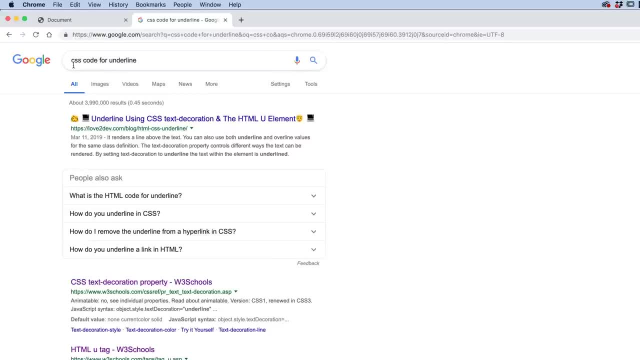 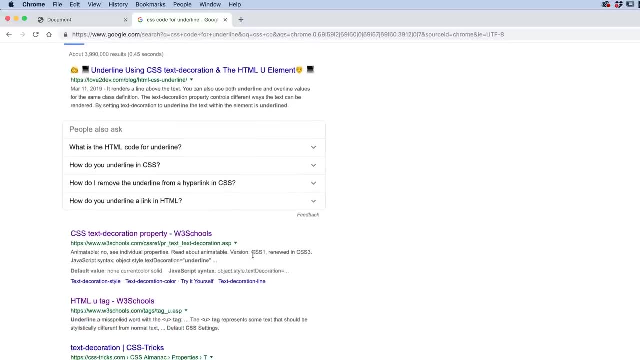 I want you. I'm teaching you to fish, So let's have a look. So I've asked for the code for underline. There's going to be kind of three main places that you'll use in your like that most web designers use. 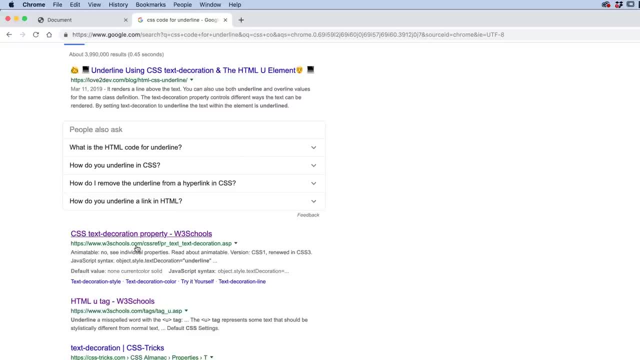 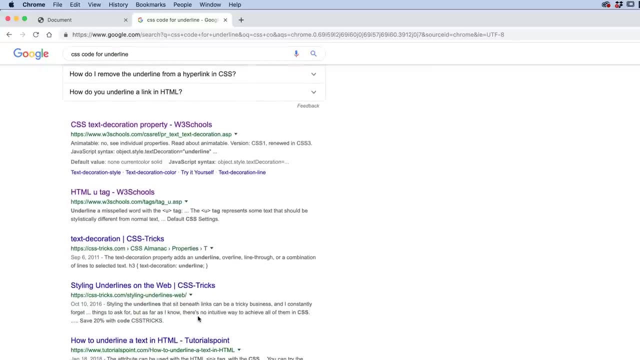 There's something called w3schoolscom. that's a really good resource- CSS Tricks. that is an amazing website by Chris Coyier. And there's another one that appears quite often and it is. it's not appearing in that list, but it's called Stack Overflow. 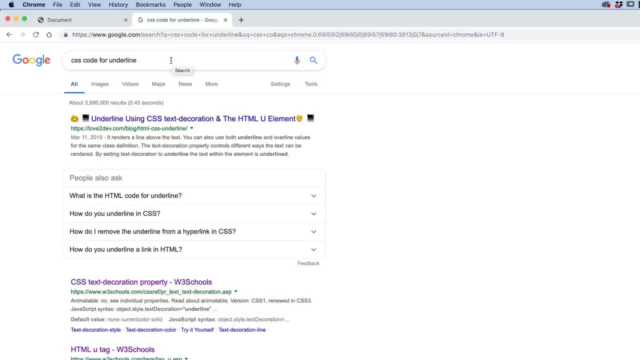 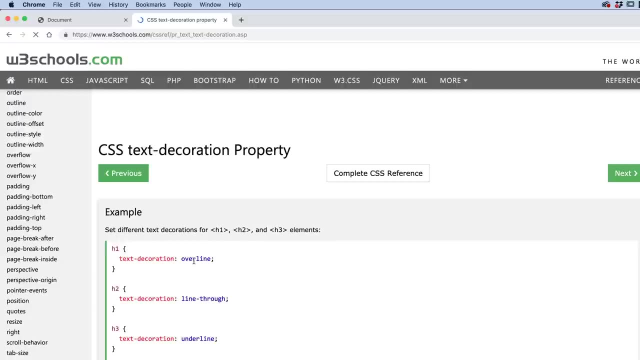 Those are your three main ones to write down and say those are the go-to places. so let's have a look. CSS Text Decoration you can see here using an H1.. there's an overline. it's not what I want underline. 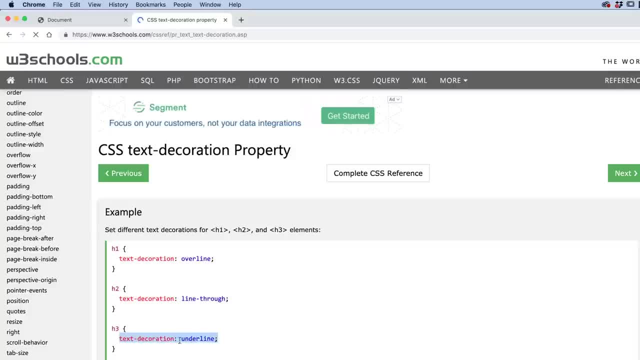 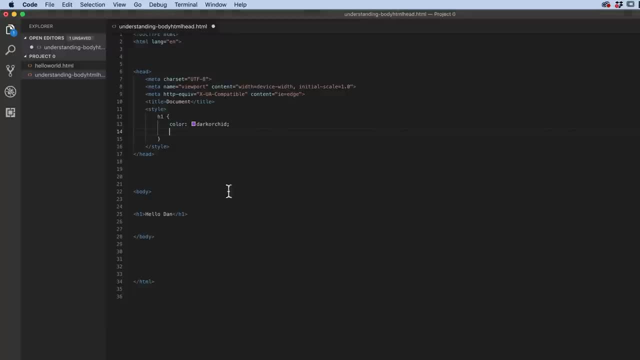 So, instead of kind of remembering them, you can either copy this, just copying it with my keyboard, Command C or on a Mac, or Control C on a PC, and go back into VS Code and I'm just going to paste it in. 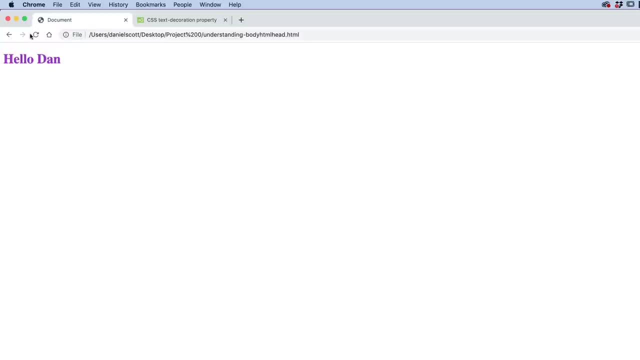 Save it and then jump to our browser, preview it, and it's underlined. So there's going to be a lot of that. If you're like man, do I need to write all this down? There's lots of times where you're just like: 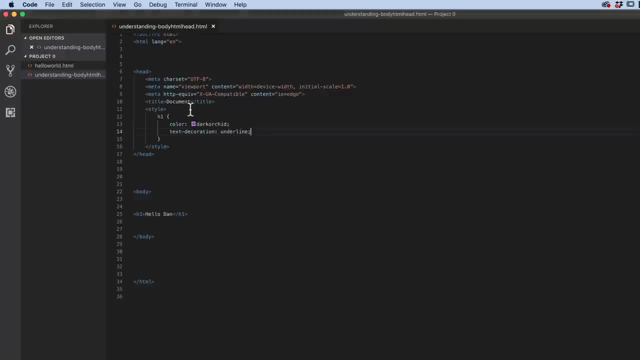 I can't remember what the syntax is so you can go and find it, Because Text Decoration is a weird way of discussing underline. But after a while you will learn some stuff that you're doing quite regularly: Text Decoration, Overline. 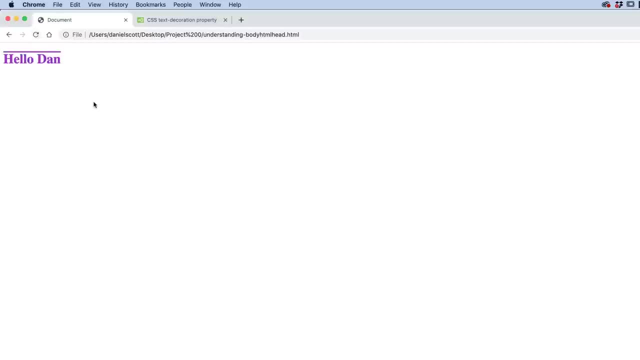 Never used that one in my life. Refresh, look at that, you can do it. All right, that's going to be it for this video. Let's jump into the next one. we start talking about the Meta Title that we've been ignoring. 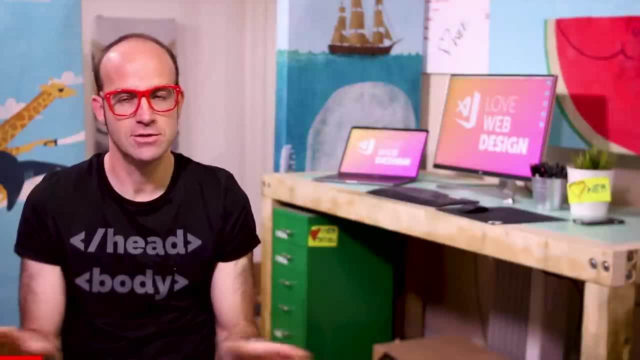 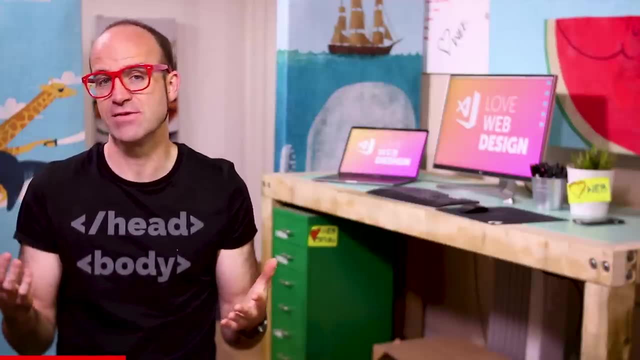 Hi there, I hope you're enjoying the video. Now. there is loads more to come, but if you like this course, there's a link in the description, because there's about like another 90 videos that I've got, that kind of follow on from where this course finishes. 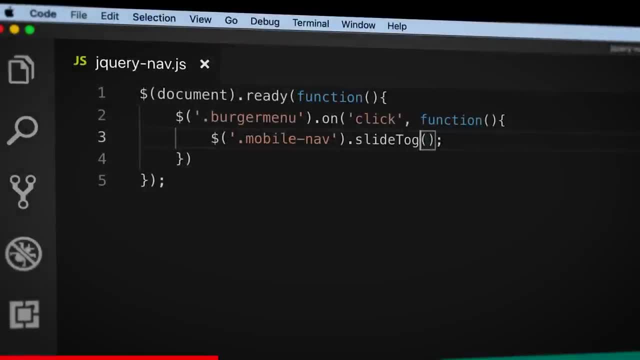 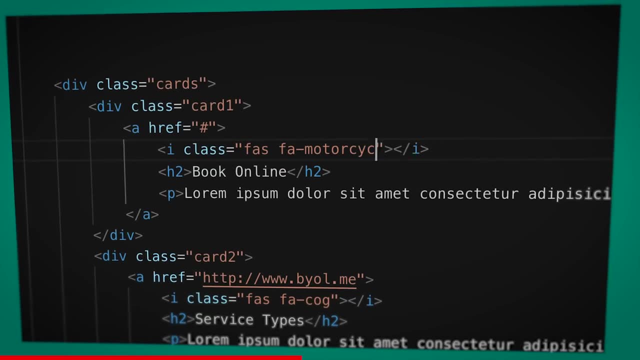 We'll cover in that extra course all the fun stuff like how to create your very own burger menu from scratch using some basic JavaScript and jQuery. You'll learn how to work with responsive images and icons, and probably one too many gradients. You'll learn how to create forms. 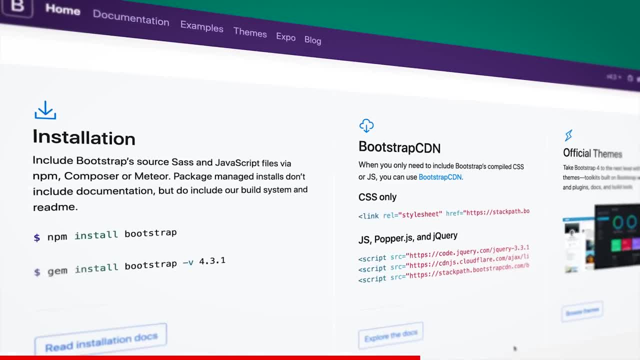 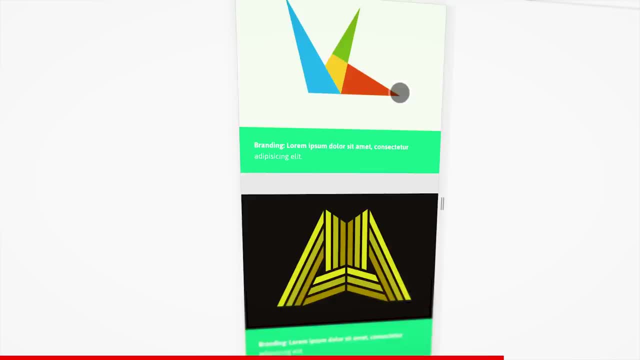 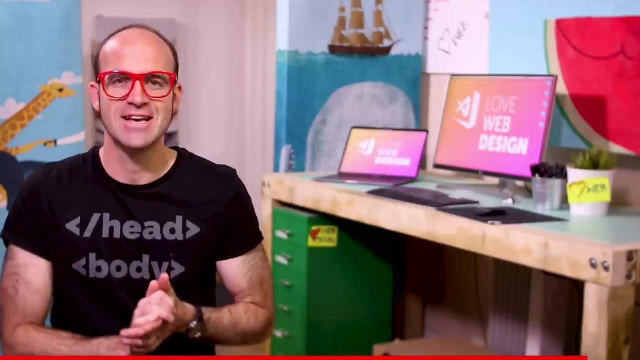 and how to choose great fonts for your website. You'll learn how to work with Bootstrap 4.. We'll create this bicycle repair shop, This responsive portfolio site And this Bootstrap website for my prototype yoghurt company, Yum. All right, if that sounds like you. 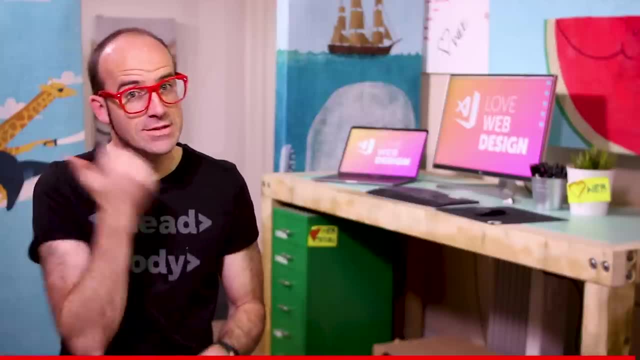 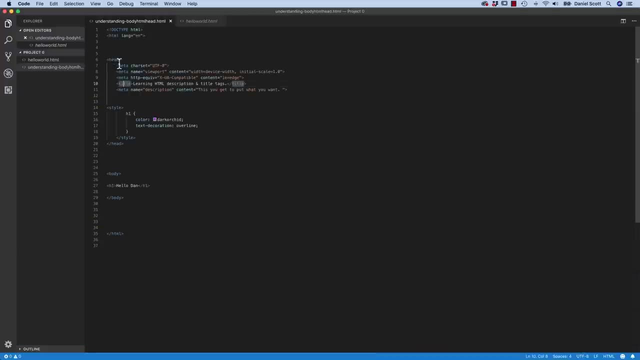 check out the link in the description, But for now, let's continue on with the course. Hey there, this video. we're going to learn what the title is in your head tag and we're going to look at what a description is. 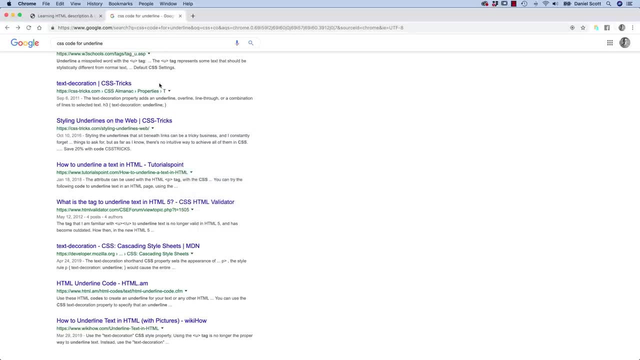 The very short version is in Google search results. that is the title, that is the description. We need to add it to every page. Let's jump in now. show you how to add it, what the pros and cons, what you should do, what you shouldn't do. 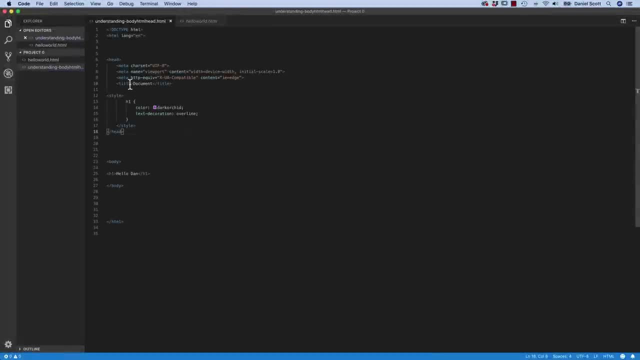 Let's get started, All right, so let's start with the title tag. So this gets added to the top of every page in the head. I've got it added there automatically by VS Code. So what is it? It is a way to describe what's on the page. 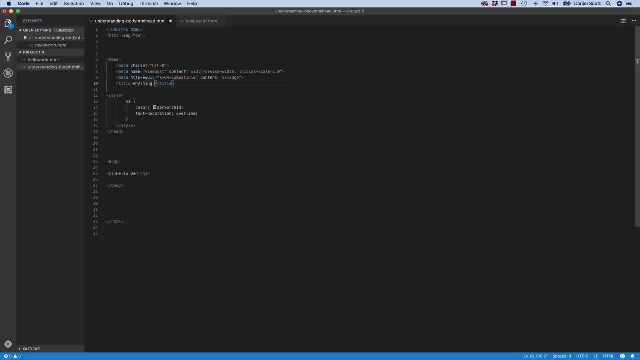 So this word document here is just a placeholder. You can type anything in here. You'll notice that it's not really code language. You can write, and you can write brackets and all sorts of things. It could be anything you want to write in here, but you don't want it to just be anything. 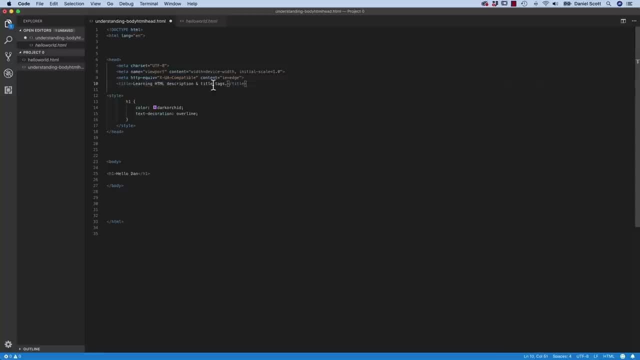 Let's say this is one I've kind of thought that really describes this page. It's learning HTML, description and title tags. That's going to really describe the page I'm trying to build here. Now, if I save it and I go out to Chrome, let's see where it appears. 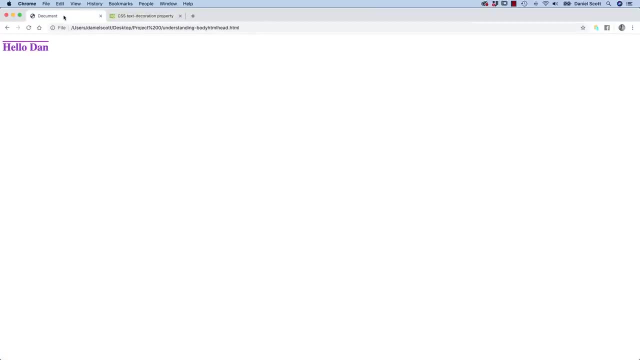 So, Chrome, there's the document that I'm working on. You can see the word document there that was from earlier on, before we replaced it. If we hit refresh, you can see. that's where it kind of ends up. that's your title tag. it ends up in the tab. 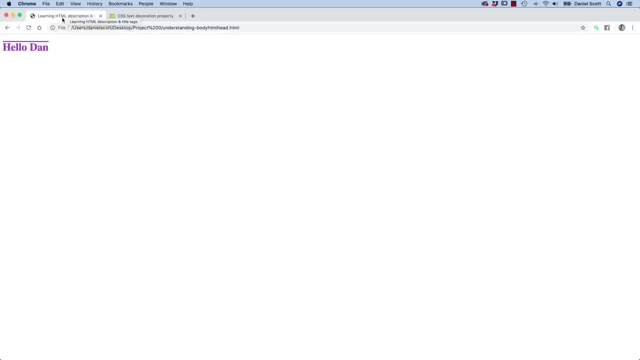 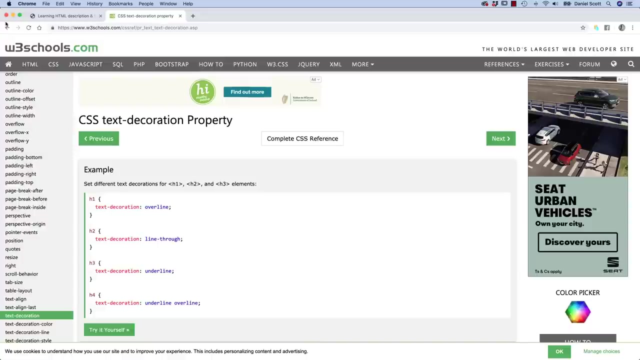 But that's not that exciting. What's really important is where that gets used by Google in its search results. So remember we did this search earlier on for underlining in HTML. We did that search. See these chunks of blue text here. 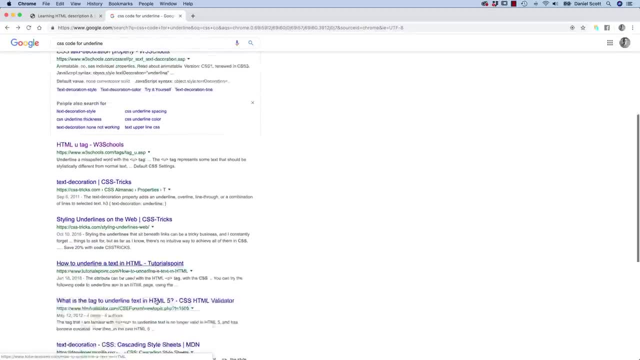 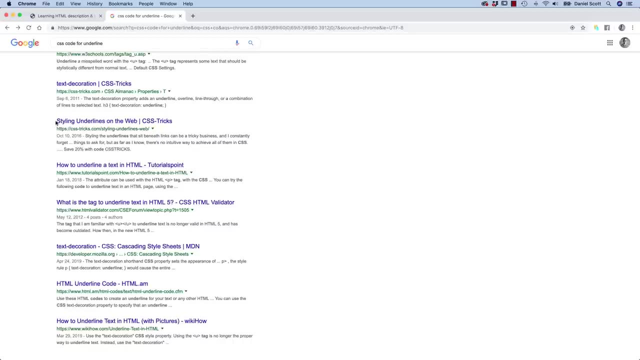 These chunks of blue text are the title tags. So whatever you write in there will appear in this little list. So you can imagine if you left it as document. first of all, the word document. Google's just not going to list your page. 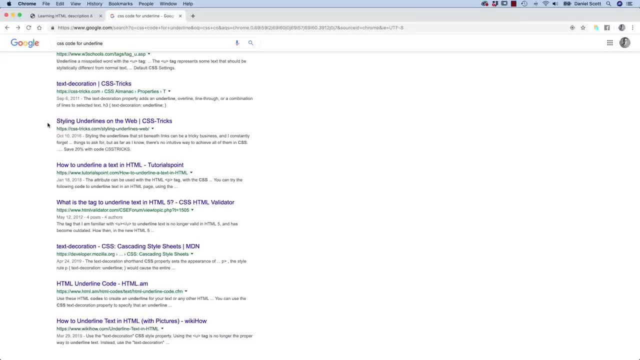 because it's too vague and there's probably a million pages online with the heading document, So you need to make it unique for every page, which is a bit of a pain. So if you've got 20 pages on your website, 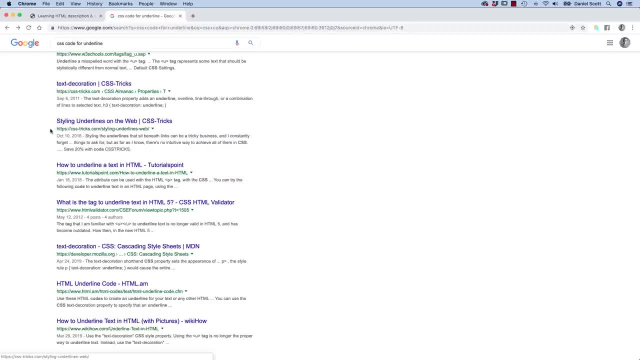 you need 20 different title tags for each page And it needs to really describe what's in that page. It's about 50 characters. you can see some of them get a little bit longer, some of them are shorter, but be really concise and exact about what's in the page. 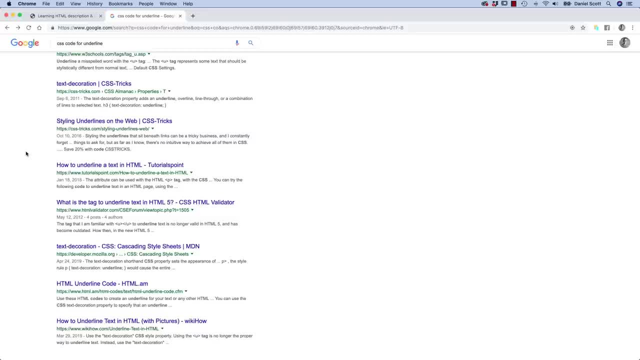 Don't call it like home page. If it was me for my site- mine is called Web Design Tutorials by Daniel Scott- It would be a good home page title tag for me. So that's the title tag, The other tag you should add, and it's not there by default. 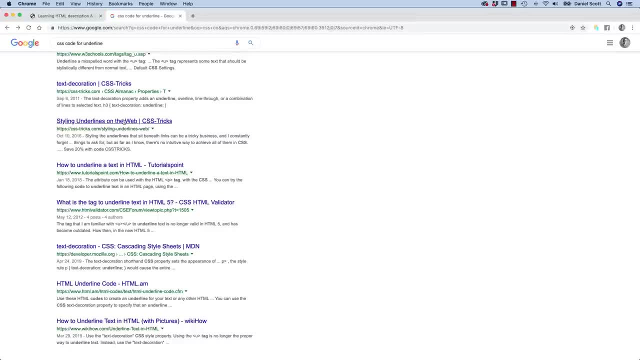 and very common. just underneath is adding the description. So what is the description? before we make it, It's this chunk That there is the title, that there is just your website address, This thing here you have control over. You can tell Google what to put in this description. 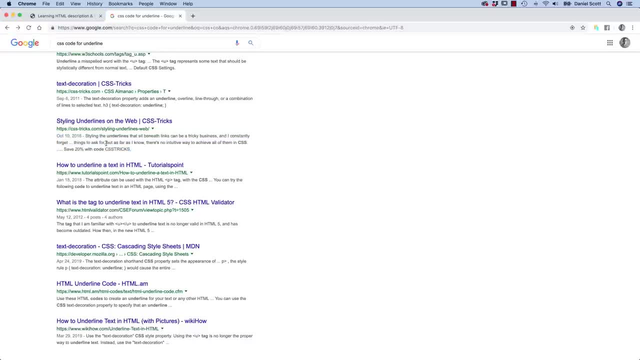 Sometimes it ignores it, but most of the time it won't. it'll list it here, And this is a bit more marketing than it is like this one here. be really concise, really good keywords that really describe what you're doing. 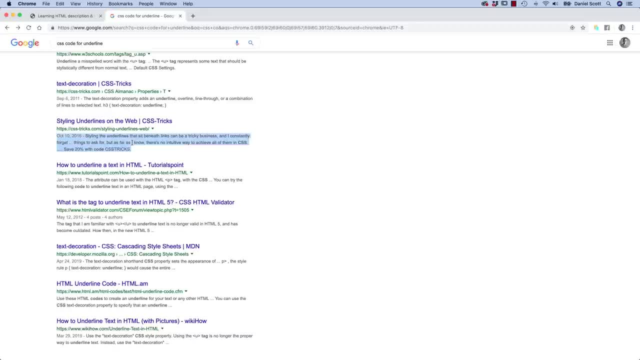 Down here is kind of like we all know it. when we're doing a result, we search, we check that to make sure you're kind of in the right ballpark. then you use this just to confirm that you're. you get more into the details. 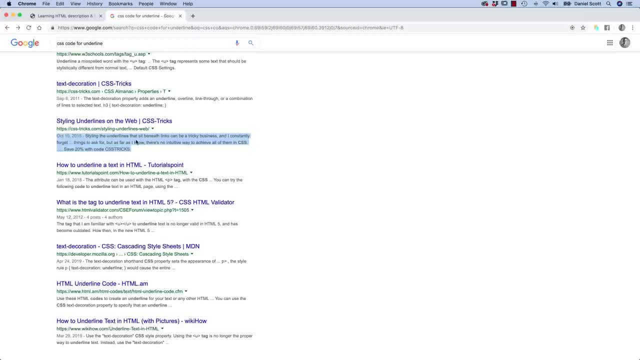 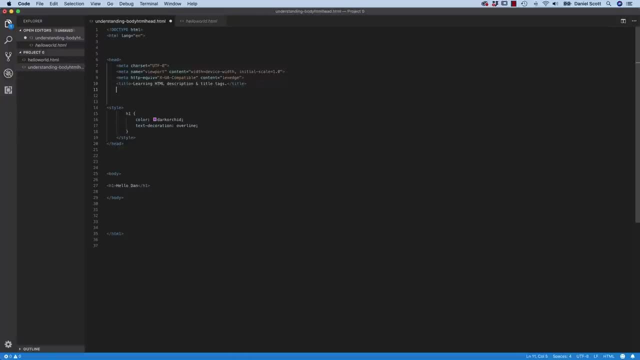 and just kind of just checking you're in the right sort of zone. This is where more it's more marketing than it is, say, coding. So down in here let's add the meta description, So by default it's not in there. 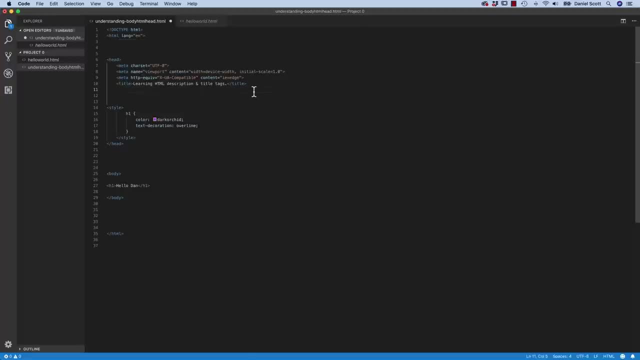 because you can't survive without a title, but you can survive without a description. But in my opinion you should definitely add it. This is where it's kind of some ugly syntax, but you type it up once with me now, and later on you can just come back and copy and paste this one. 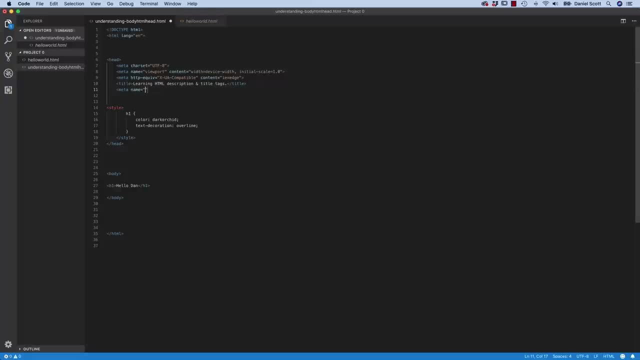 So it's called a meta name and you need to add all that syntax. I'm just using the shortcuts that appear via VS Code, but you need name equals and you need the quote marks and inside of here this one's called description. 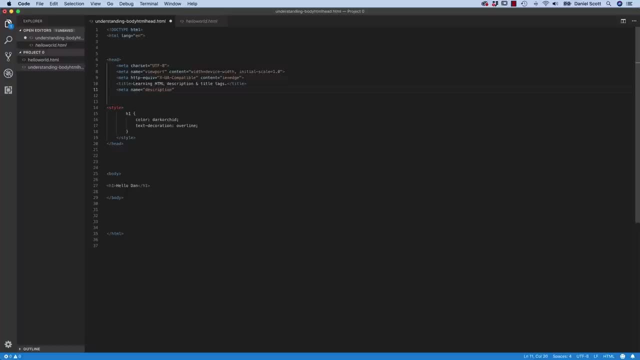 It needs to be spelled exactly like that and we need. so the name is description and the content is going to be what you want that description to be. So this is where you get to put so in here. you want about 100, between 120 characters. 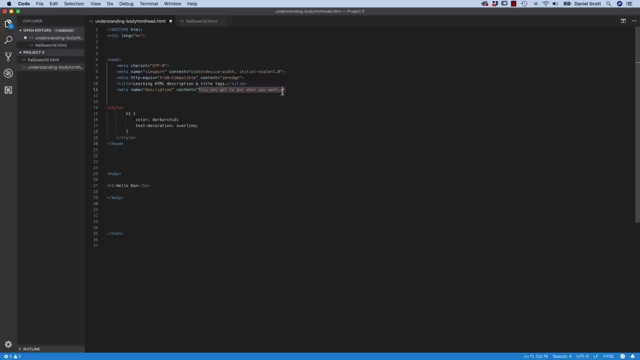 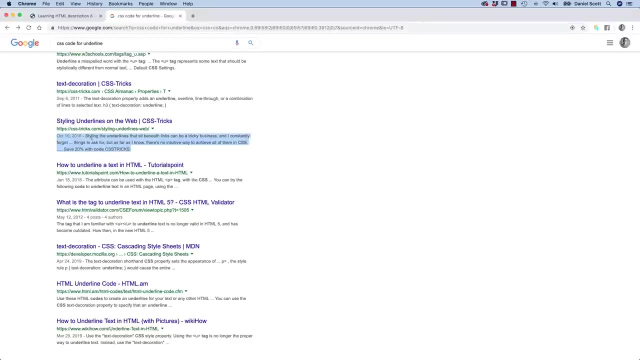 or 150 characters. so 120 is what generally will appear in mobile results and 150 on desktop. So you can see here: this one here got given quite a big chunk, whereas this one got cut off quite small. this one's got a really small meta description. 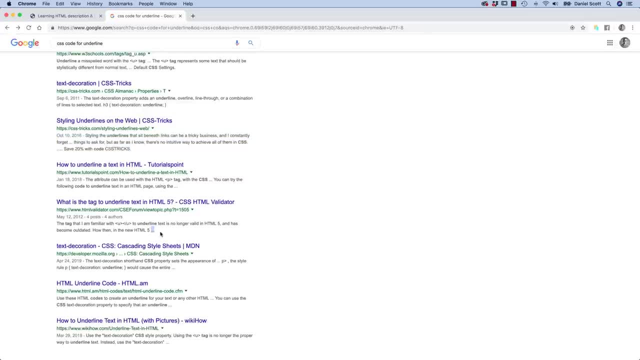 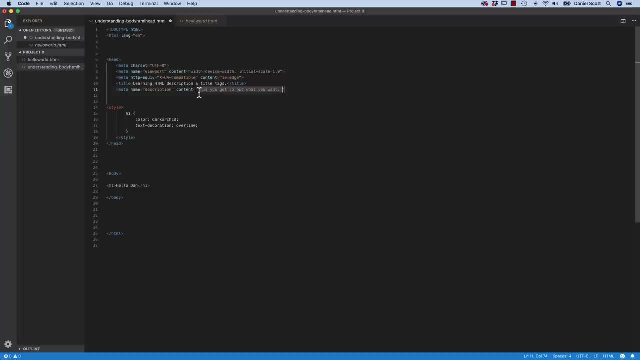 Sometimes as well. doesn't matter how long you make it, Google will cut it off. So make sure all your good stuff is at the beginning of that paragraph. Just make it one, and make it about 120-ish characters. Now, the one thing, for this is kind of brings up a good point. 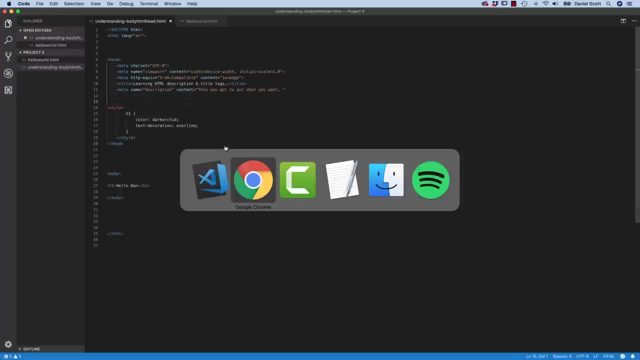 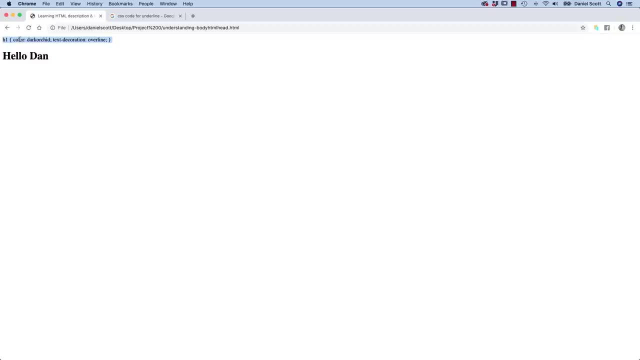 Can you see this guy's gone red. If I save this and let's view the page, let's refresh it. it's gone a bit crazy. it's like that was in the head tag. why is it displaying down here in the body? 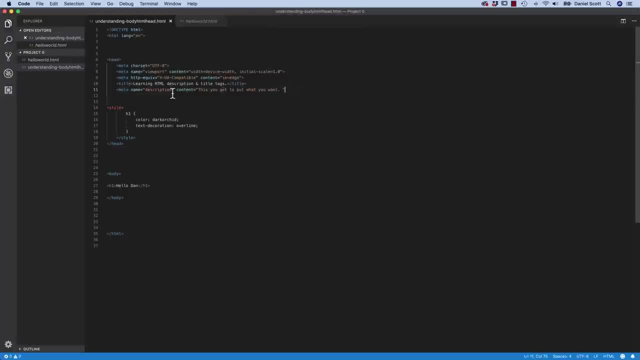 It's because we forgot to close out this meta description tag. So I say we, me. It has an opening there and can you see? all of them have this closing angle brackets. So at the end here, closing angle brackets, you'll see the red disappears. 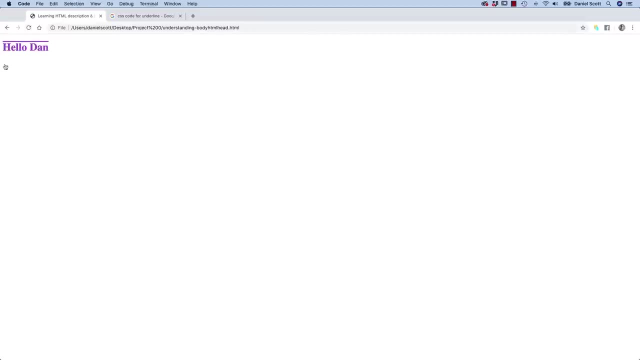 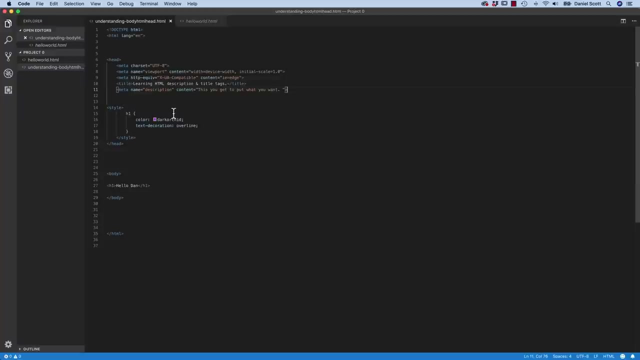 and back here, refresh, it's back to normal. So if you ever have red stuff- bad And often you'll notice the difference- when you get into previewing in Chrome, It'll kind of show you. everything will go haywire. 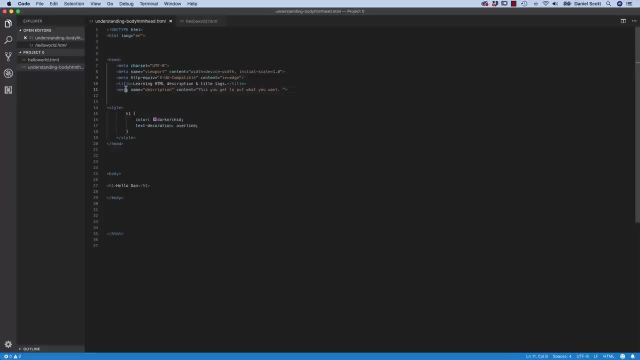 That is the meta title, meta description. Copy and paste that into a notepad so you've got it handy for when you're doing it next time, so you don't have to type it out every time. Really essential to pages. let's get on to the next video. 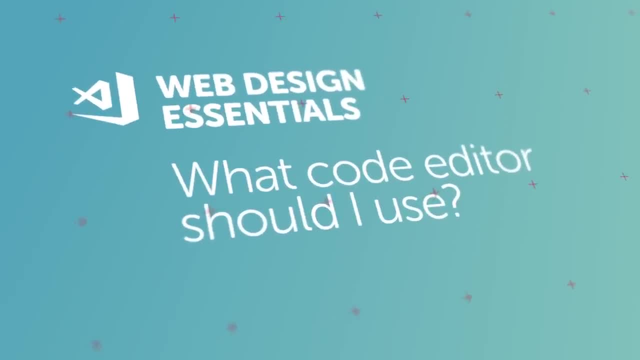 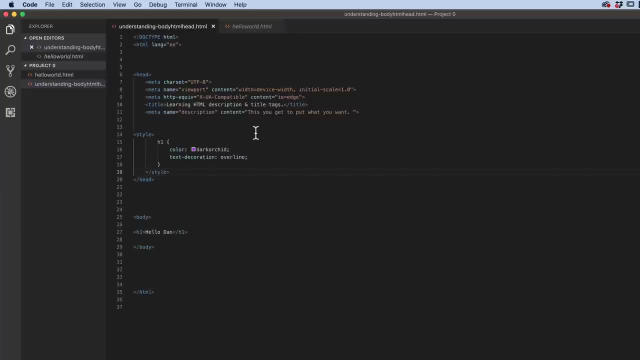 Let's talk code editors. We've been using VS Code so far and we're going to continue for this course. Why? Because it's the most popular And mainly because it's the most fashionable. There are some quirks to it that make it awesome. 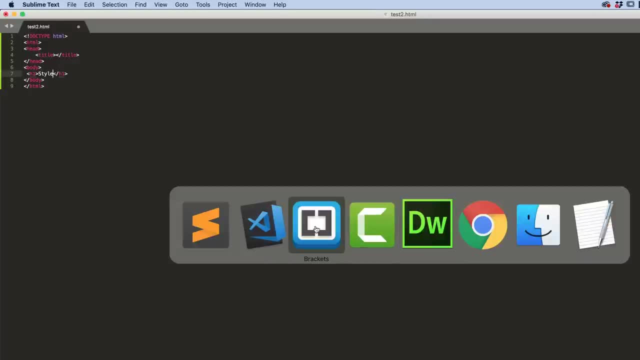 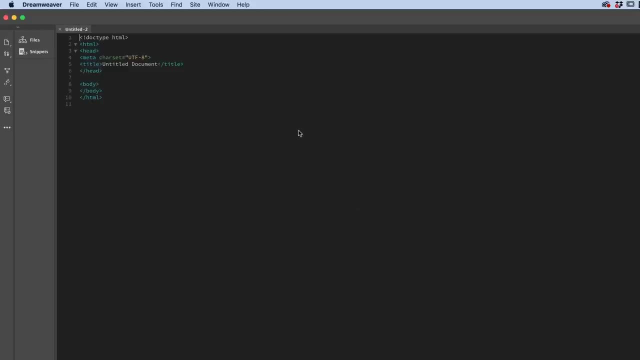 but there are people out there that argue that Sublime Text is the best, or Brackets is, or Dreamweaver is, or Atom or Notepad++. there's lots of different editors. Let's jump into this video and just give you a quick run through a few of them. 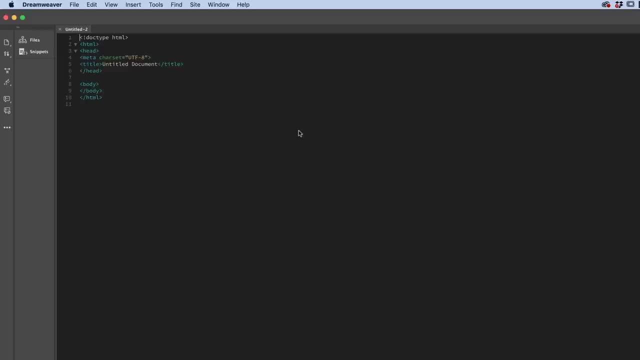 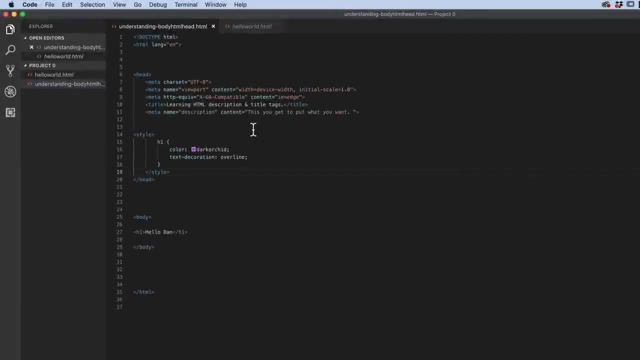 just to kind of show you what you should look for and what's important. All right, let's get in there. So we've been using Visual Studio Code for our text editor. Now we could have done this course in any of the editing programs. 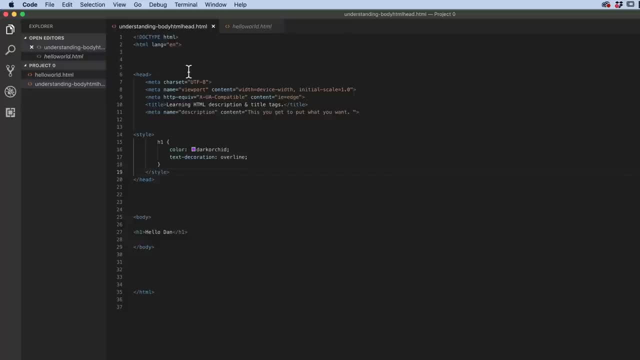 Now we're only using VS Code in this case because VS Code is the most popular. So in my previous courses I've used Dreamweaver because I often spend my life in the Adobe world. But I guess what I wanted to show you real quick was: 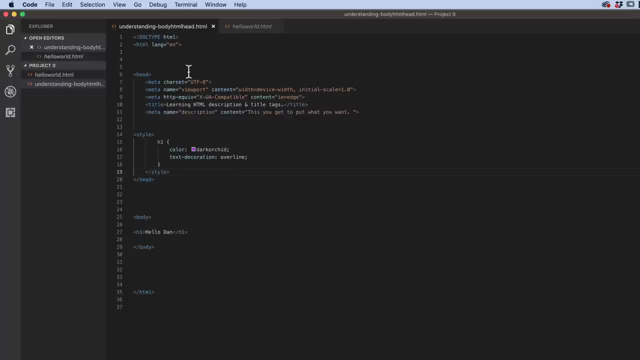 first of all, how these editors are really helpful, but often can be very- what do you call it? fashionable. So if I had done this course a year ago or two years ago, it probably would have been in this one called Sublime Text. 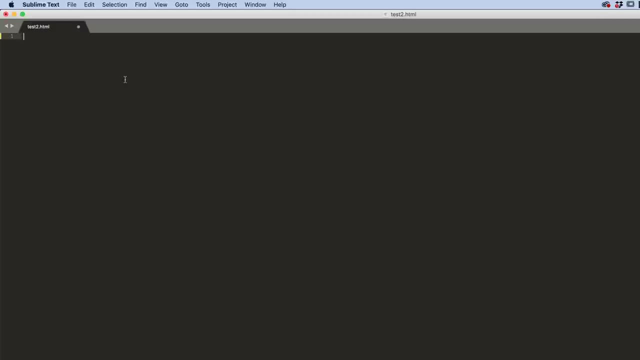 because it was the most popular then, And before that there was things like Komodo, and before that there was Notepad++. There's lots of different editors, but we all end up in the same place doing the same thing. People get used to some of the quirks to them. 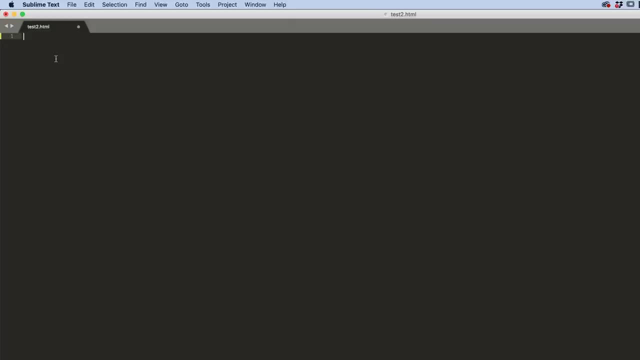 so I've downloaded and installed Sublime Text just to show you. if you're getting started in Sublime, it's a lot cleaner. And if I want to put in all my kind of document stuff for HTML, in this case, instead of exclamation mark and tab, it's HTML and hit tab. 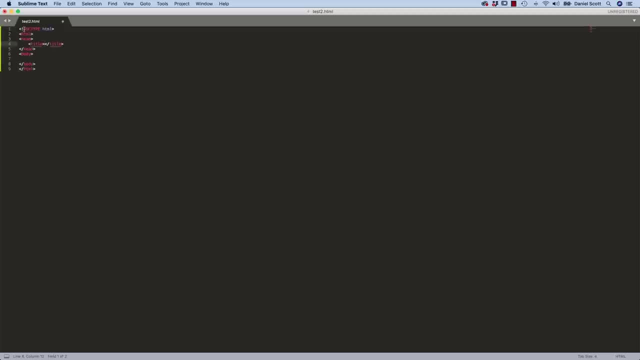 You can see we get to a very similar place. It doesn't have as much in the document type, just the real basics, But we end up with the same place, right? We go down here, we type H1, and we start typing. 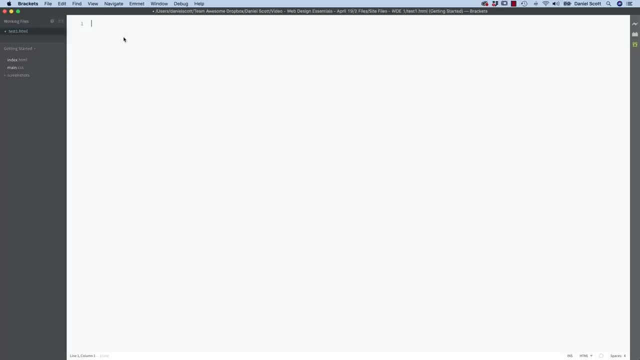 Same with. let's look at brackets. Brackets is another popular one. Exclamation mark tab works the same as it did in VS Code. They don't have all the bits and pieces that we want in VS Code. They decide on a real kind of minimum option. 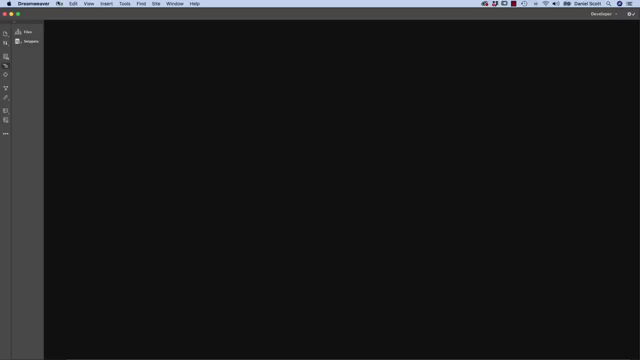 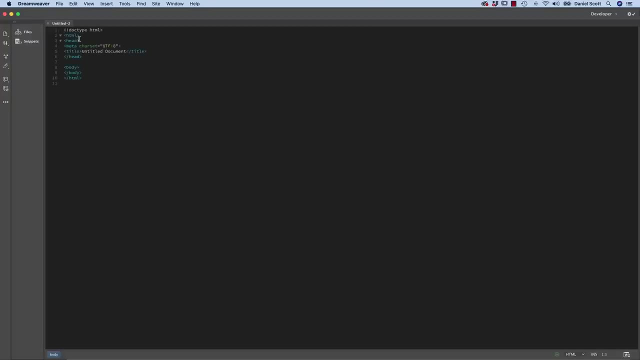 Dreamweaver as well. great code editor. If we go to File New, they do it automatically. If you say you want an HTML page, you say HTML5, click Create. You can see. it puts in all the bits and pieces you need to get started. 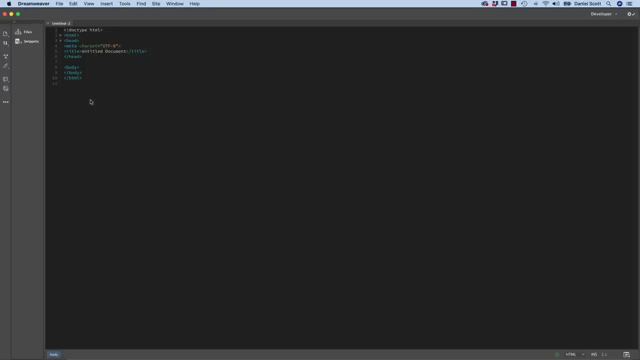 The reason I show you this is if you're looking for work after this or you start working with different developers and they're using different editors. there's not really. they have their own perks and quirks, but we are creating the same thing. 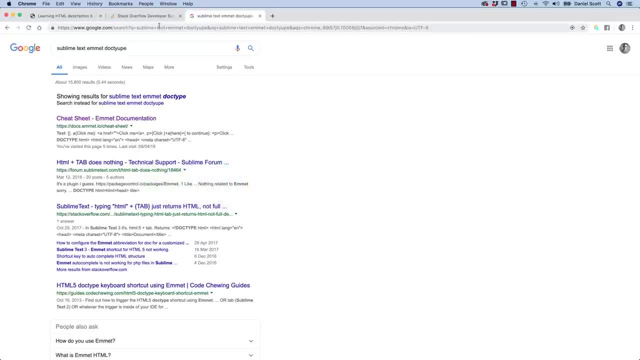 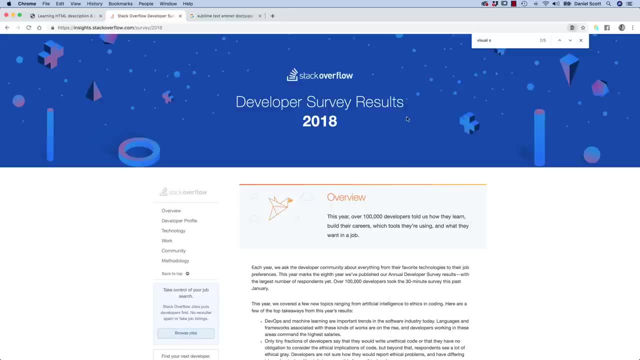 The way I do it like. when I was designing this course, I was trying to work out which one to use Stack Overflow. I mentioned that earlier. They do a developer survey at the end of the year, so it's 2019 now. 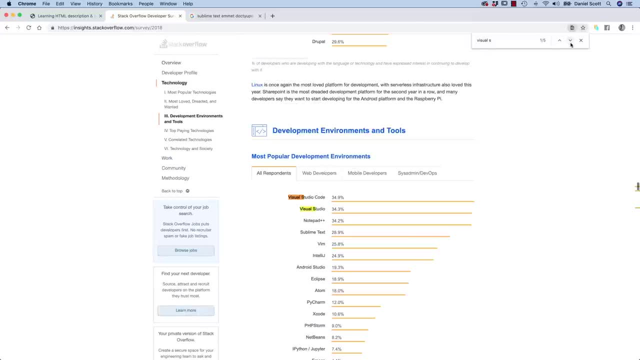 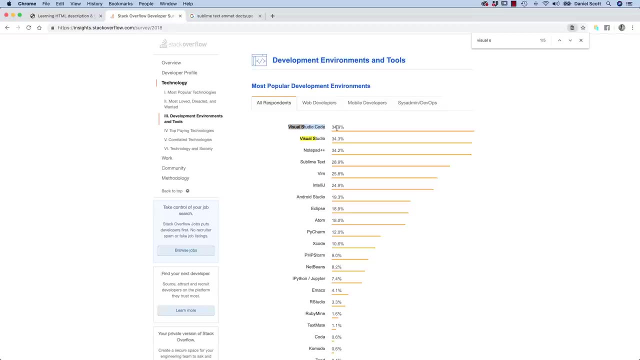 and this is last year's survey and I just kind of went through and you can see down here, way down the page, the results back for Visual Studio Code is by far the most popular. You can see, Visual Studio is the big version of this. 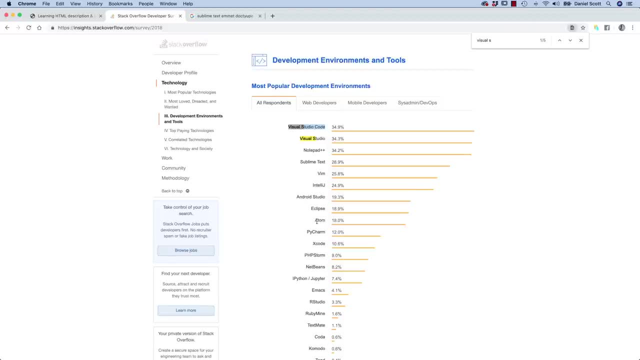 Notepad++ Sublime Text Atom. I thought was a lot higher. There's just people love their own editors but, unlike something like Photoshop where there's only kind of one product and one or two competing, there's a lot of different code editors. 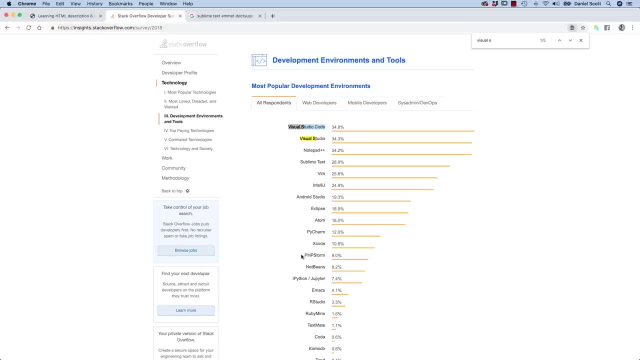 Some of them quite general, like the one we're using, some of them a lot more specific for, let's say, PHP or Xcode. But anyway, I thought a little short video explaining different editors, in case you want to move to something else. 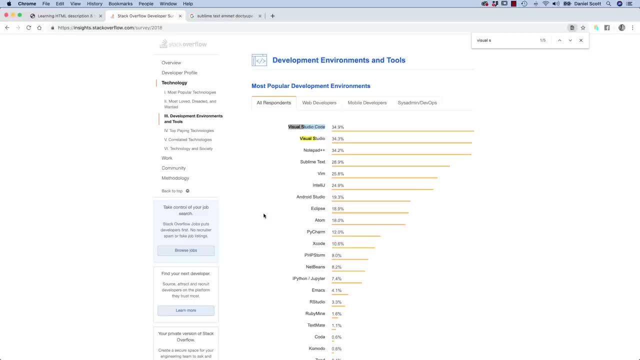 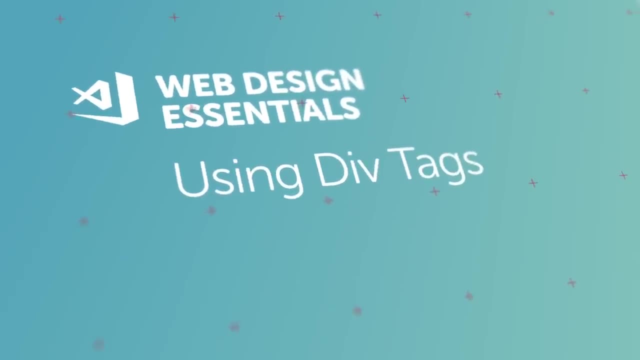 or expected to use something else. you can use what you learn in this course in a different editor. All right, let's go on to the next video. Hi there, this video we're going to build a yellow box and then a pink box. we'll try to, at least. 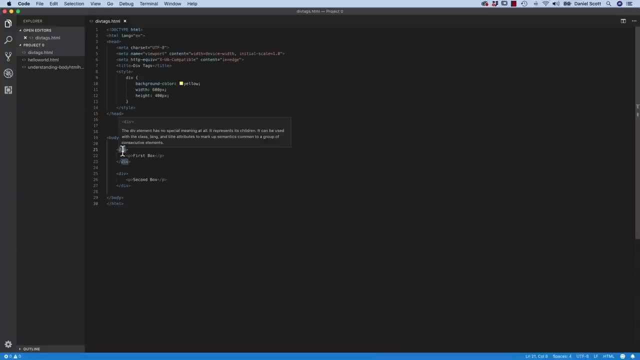 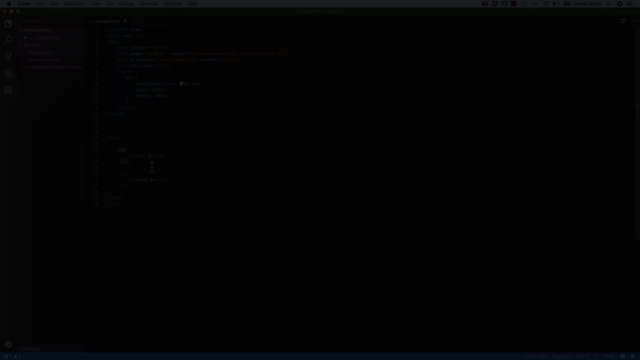 We're going to learn to do it using something called a div tag. It's a division of space and it gives us the kind of boxes that we get to put our website inside of. All right, let's jump in and learn it. 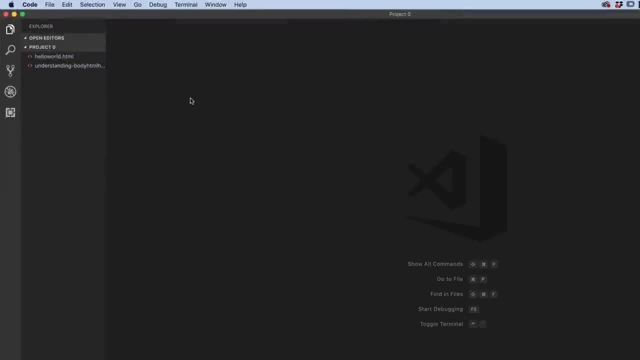 To get started, let's close down the other documents we've been working on. We're not going to use those again, We're going to create a new one, just to kind of separate everything and all our different bits of learning. So File, New File, let's save it. 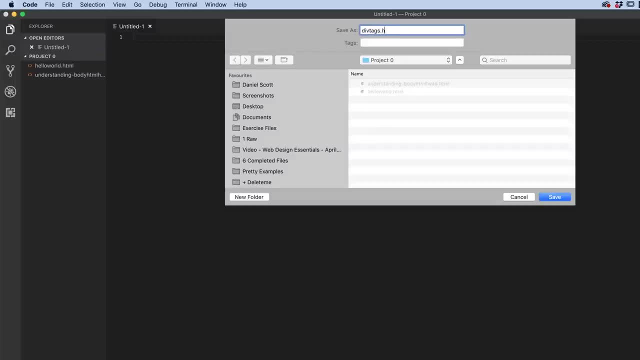 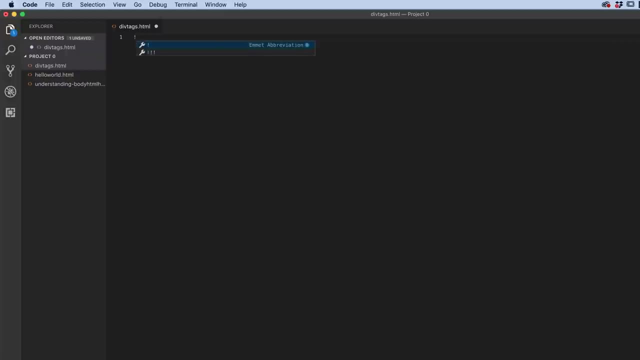 Let's call this one divtagshtml. don't forget the HTML. And we're going to add all of that head tag. goodness, by putting exclamation mark, hitting return Puts all that junk in. we make sure we update the title. div tags. 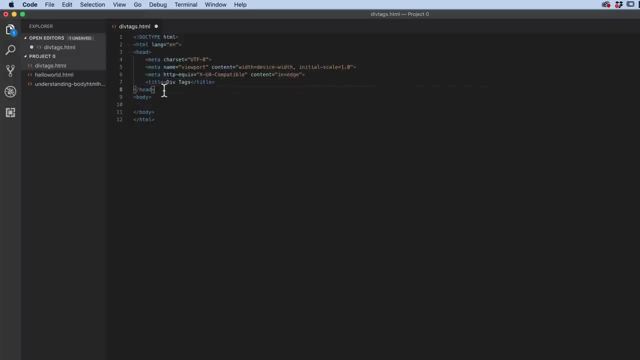 We put in the description, but we're not at the moment because it's kind of like a throwaway project just to learn what division or the div tag is. So the div tag goes on the body because I want people to see it. 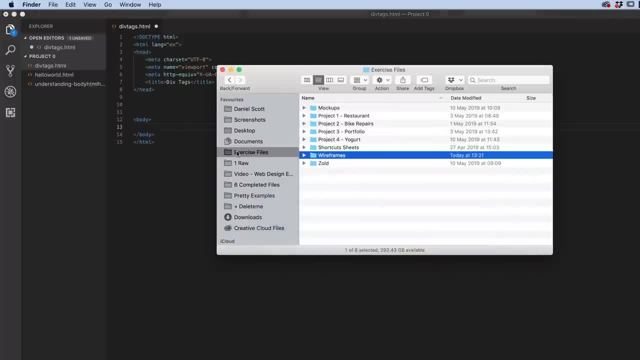 Now, what do we want it to look like? In your exercise files, there's a folder called wireframes And this one here called html-div-1, I'm going to open that. For no reason. we just, I don't know. I drew it out in my notebook. 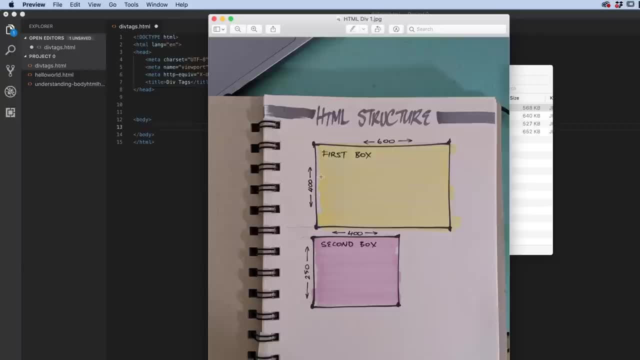 so I figured I'd show it to you. This is what I do when I'm wireframing. It's not a particularly good or exciting wireframe, right? We want a yellow box and we want a kind of a pinky box underneath. 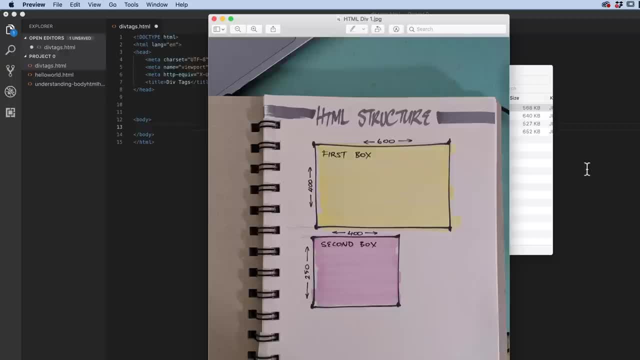 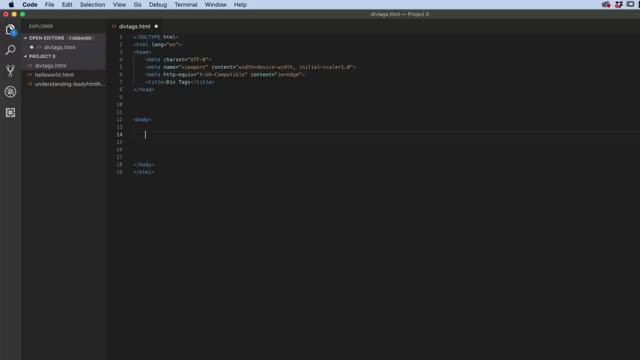 So first box, second box- that's what we're going to make. So to add it, we add a tag called div. So I'm going to make some space in here in my body. I'm going to tab across for no good reason. 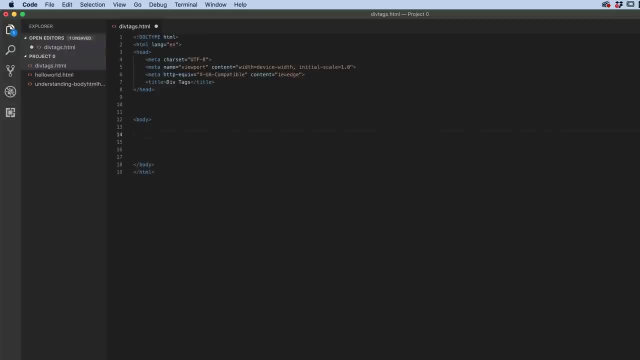 Other than it looks nice, we're going to put in a div tag. So div tag starts with the angle brackets, Div close angle brackets, and it's very clever and puts in our closing of that tag And everything inside. of this is going to be my square. 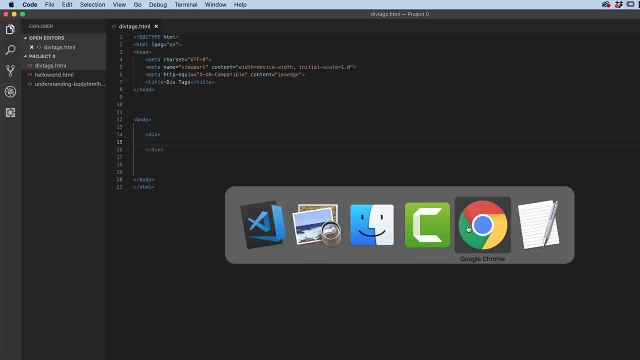 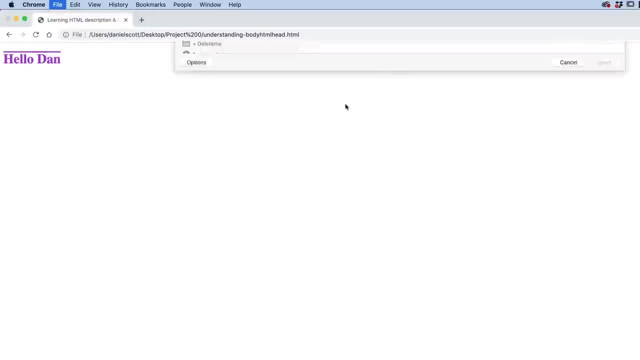 Let's preview what we've made so far. so let's save it. Go to Google Chrome. let's go to File. let's go to Open. Where is it? Open File? There's my new div tag. click Open. I've got the title, but there's nothing appearing on the page. 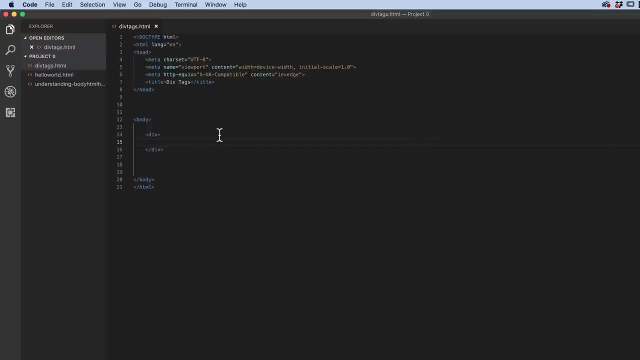 So a div tag without any CSS is invisible. It's there but we haven't styled it. So what we need to do is tell it to do some stuff, Like be yellow and give it a size. So we do that with our CSS. we'll do it in the head tag. 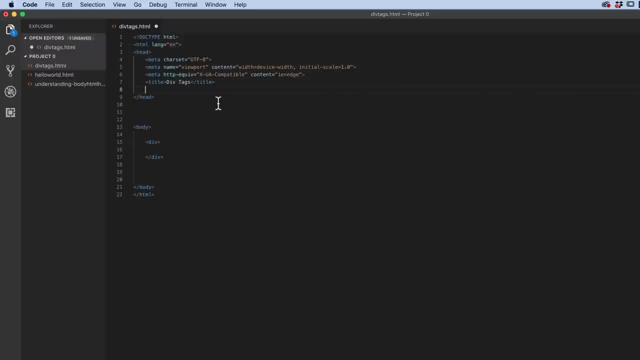 Remember. before the head closes, I'm going to type in: do you remember what goes up the top here? You remember style, Style And close it off. put a return in. I'm going to put all my styles in here. 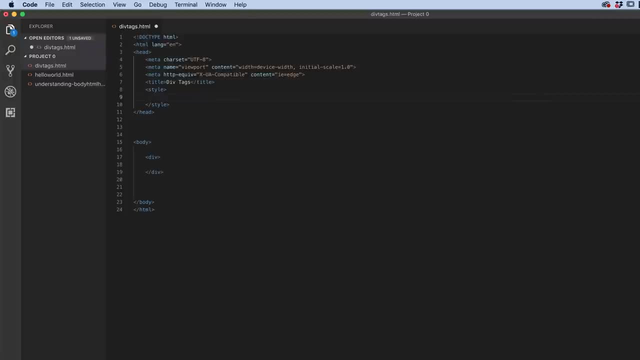 I'm going to tab in, just because it looks nice, I'm just using my tab key And what we'll do. so we need to style the div. Remember we had H1 before, So we're going to style this div and what goes next. 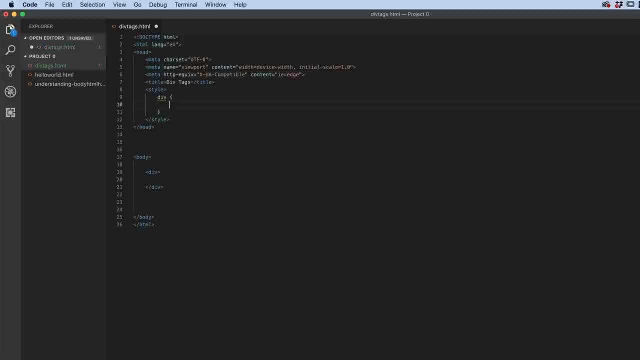 Curly braces, perfect. Then let's style it, let's give it a color. Now, when you're styling text, it's always just referred to as color. When you're trying to do a background color, you have to go to the full background. 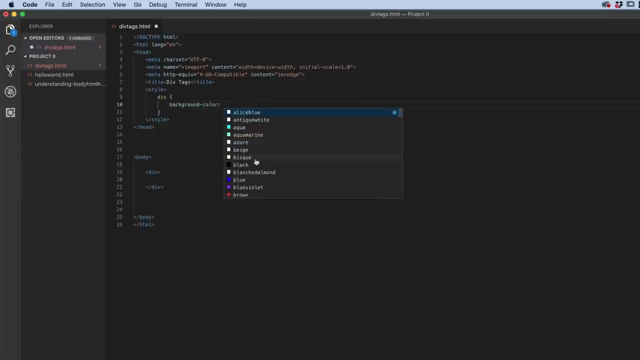 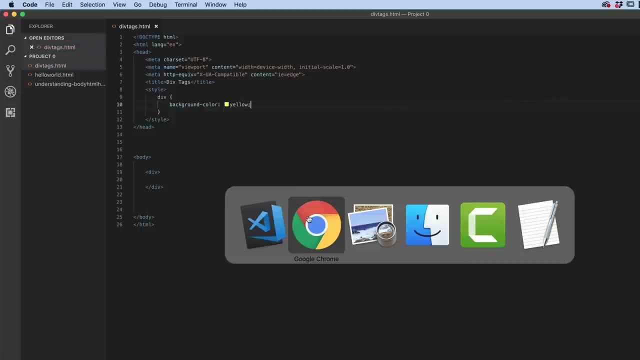 There it is. there you can see background color, What color we're going to use. I'm going to put in yellow: Remember what goes at the end: semicolon: save it. Let's preview it in the browser and nothing appears, because at the moment, this div tag is yellow. 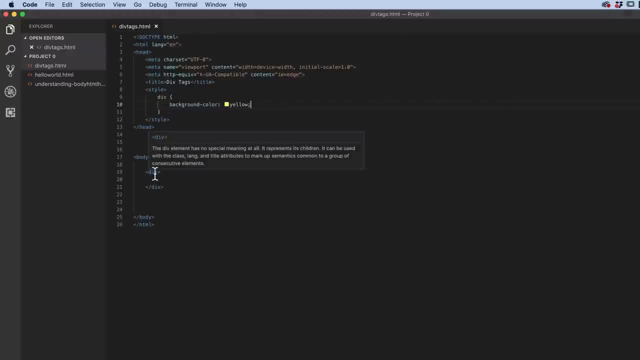 but it has no dimensions. It either needs a height or it needs some stuff in it. So inside this div I'm going to tab across stuff in it. If I do that, save it. go back to my browser now. 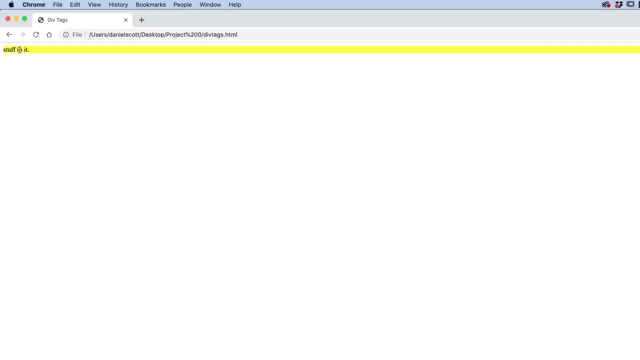 At least now with some text there. it kind of forces that div tag open a little smidgey bit so I can see it Now. it doesn't know how big it is, it's just showing me enough to squeeze the text in. 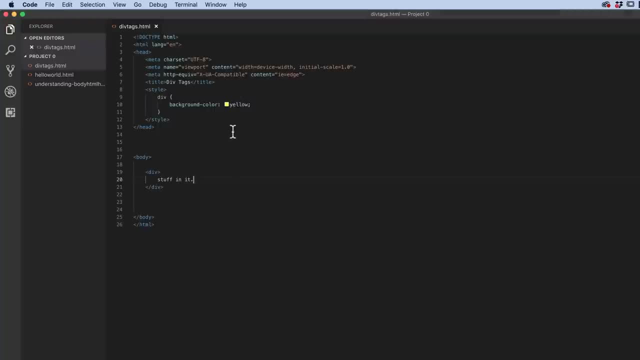 and it's kind of spilling across. So let's give it a height and a width And in here let's just put in a P tag rather than just plain old text. So we're going to put in some body text, maybe a paragraph for P. 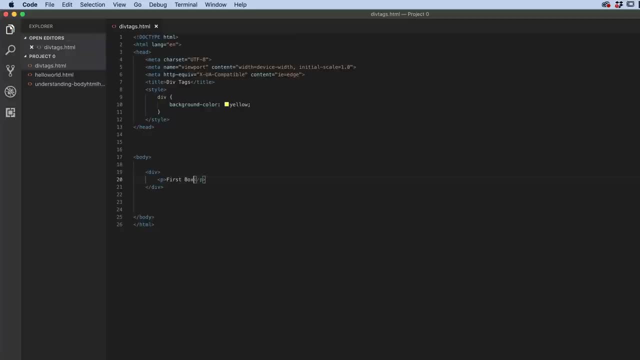 And let's just put in first box, Save it and let's style it So up here the div tag is yellow. I'm going to put a return afterwards and let's give it a width and a height. So width I'm going to give it. 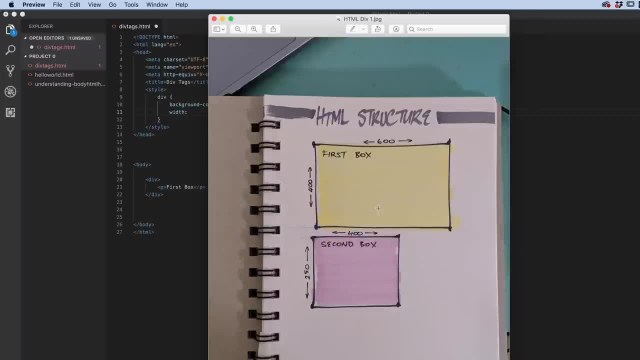 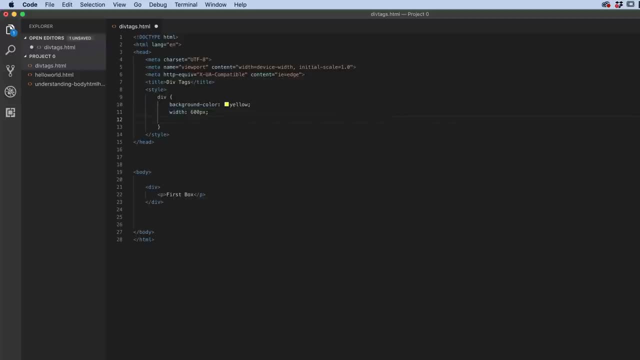 what did our little style sheet say? 600 by 400.. So we're going to go 600 pixels for the width, Remember it has to have PX and you have to have the semi-colon and the height the same. it was 400, right. 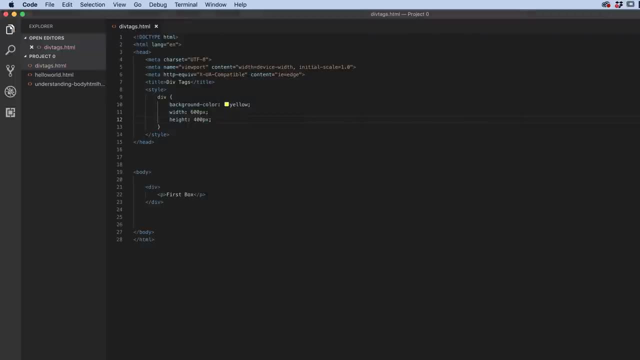 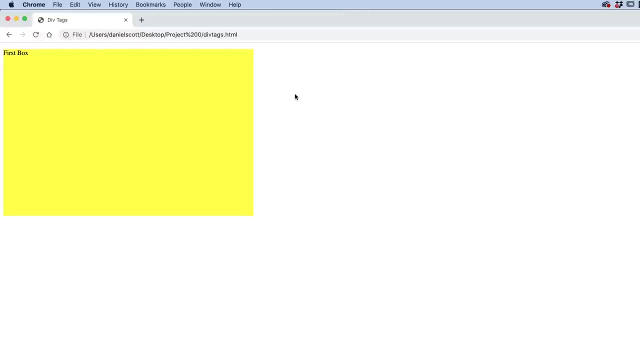 400, I wrote it down. come on, Now we've saved this. let's jump into my Google Chrome. Hit refresh. Hey, hey, so that is my structure. That could be your navigation, pretty big navigation, but it could be the middle of your website or your footer. 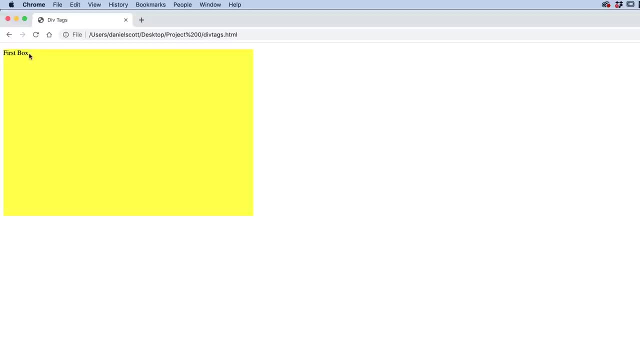 It's a nice big cube that we can start putting things like H1s or P tags in Cool huh. So a lot of your- basically your site's, made up of structural bits, these div tags and text elements and images that go into it and videos. 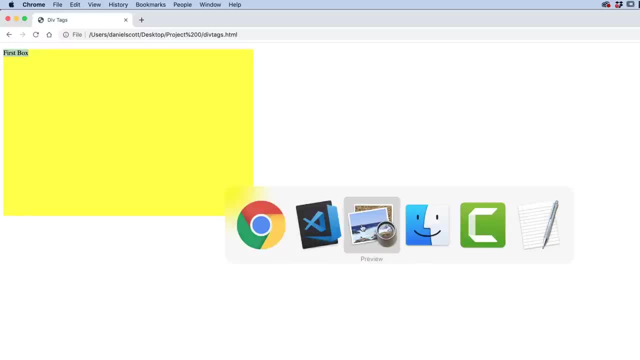 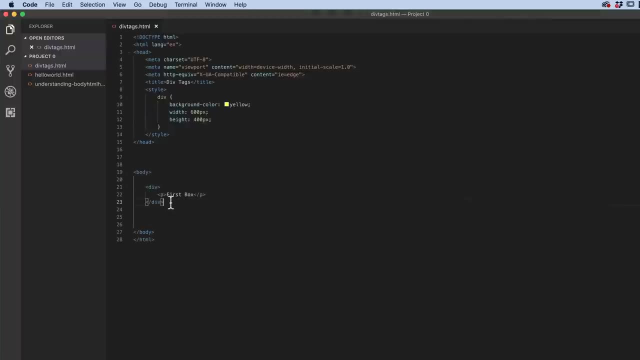 But the div tags are the structure. Now, what we want to do is we want to put in this second box down the bottom here. So in VS Code I'm going to go down here, make a second div. Let's just copy the first one. that would save some time. 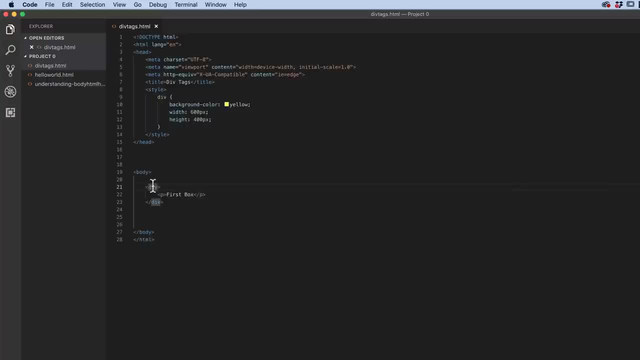 Copy. when you do your copying, make sure you grab the opening and the close. It's easy to know where the closing is if you click on. it Kind of highlights it here. just have your cursor flashing in Like the head. here there is the closing. 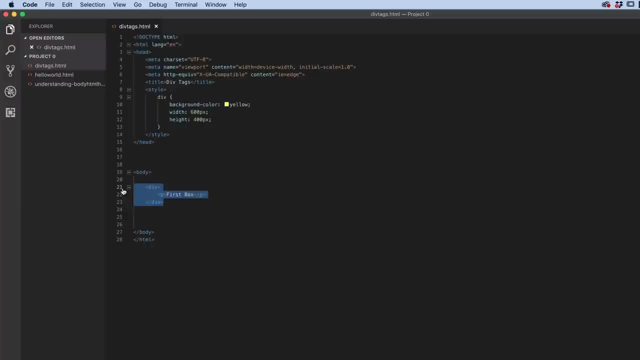 So I've got to make sure I grab all of that, Copy it. so I'm just using Edit Copy. I'm going to paste it in. The tabbing is a bit weird, and because I'm a bit OCD about this, I'm going to make it all look nice. 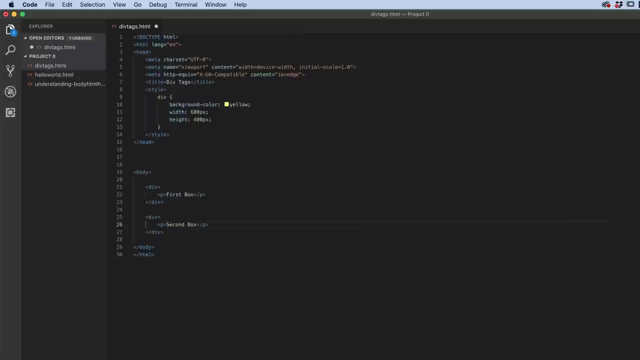 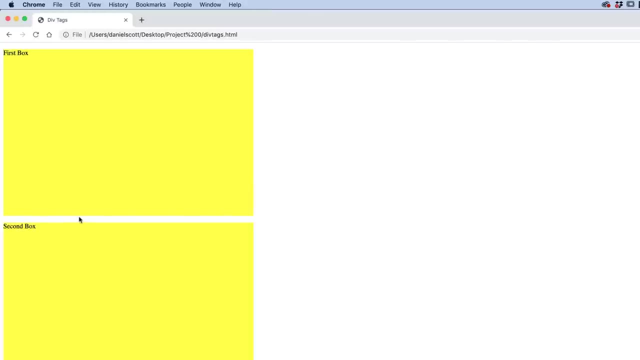 So first box and second box. second box: Save it, let's preview it in a browser Preview. we've got a second box, hey, And the last thing we want to do is we want to make it a color. 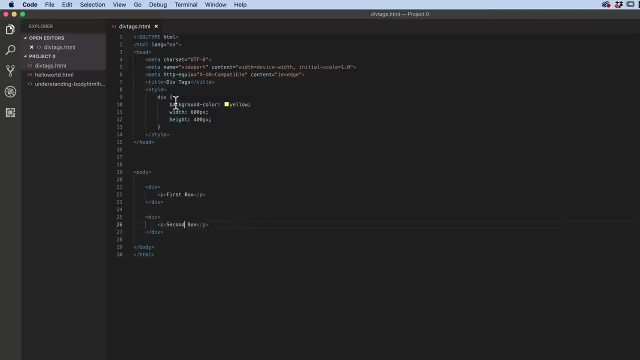 We want to make it this pink. So in VS Code we're going to go up here, and this is where we run into our first problem. We're styling this thing called Tag, an HTML tag, this div. The problem with it is that. 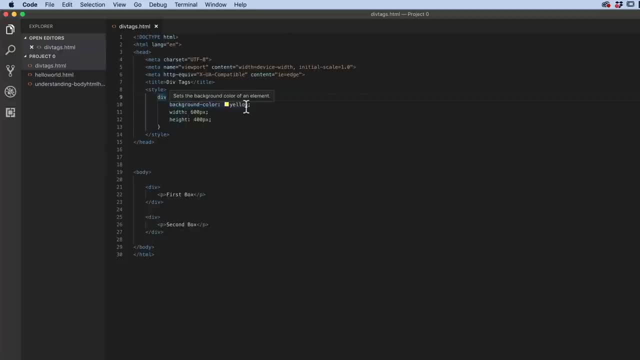 this div appears twice, but we can only color it once, So we're going to learn in the next video what something called a CSS Class is, And it allows us to individually attack this first box rather than the second box and style them differently. 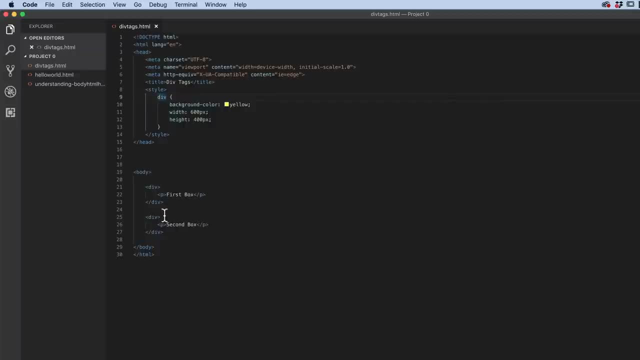 But for the moment we've put in our div tag. it's awesome. Now we need two different kinds of div tags that have different sizes and different colors, And we'll learn how to do that with a CSS Class in the very next video. 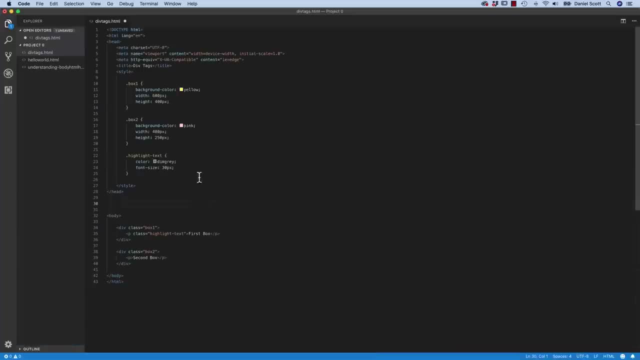 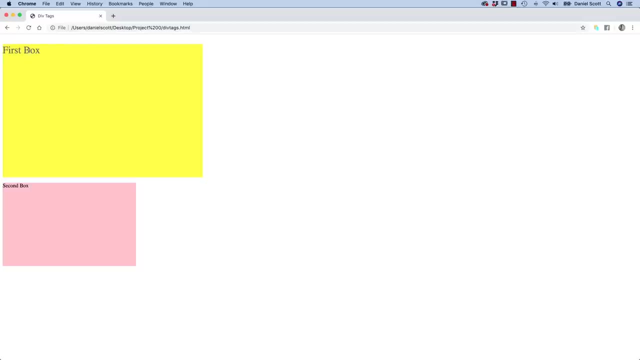 Hi there. this video is all about a Class Selector. It's going to allow us to do this where we style the yellow box differently from the pink box. We'll do the same thing with this P tag. We'll make one P tag different from the other one. 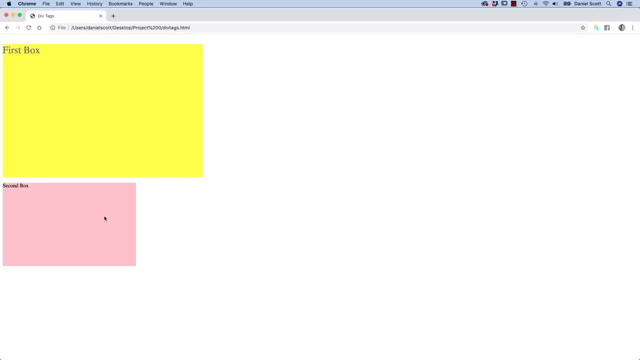 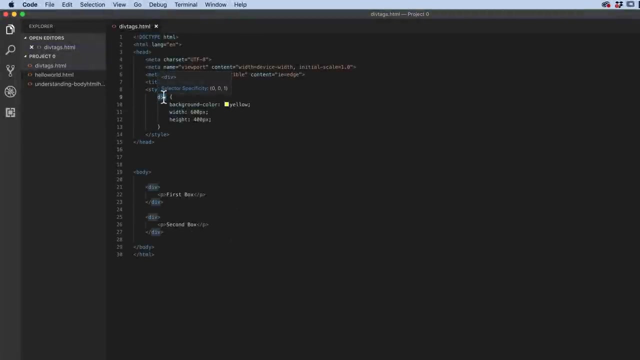 That is the job of a CSS Class Selector. Let's jump in now and learn how to make it work. So here's our CSS. this thing here is called a Type Selector, So it's selecting all the div types. The problem is it's quite generic. 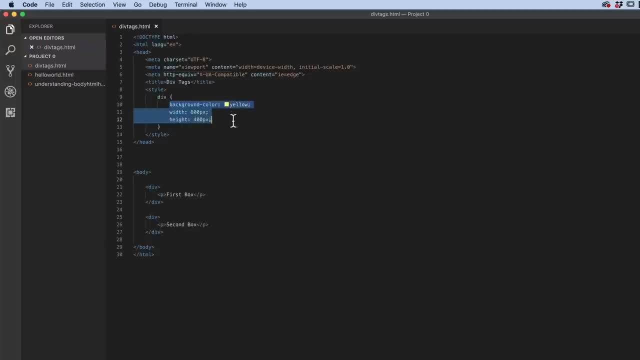 It goes. every type that happens to be a div do this stuff to it, And that's why we have a Class Selector. So what we want to do is let's bin all of this, Put my returns back in my tab in. 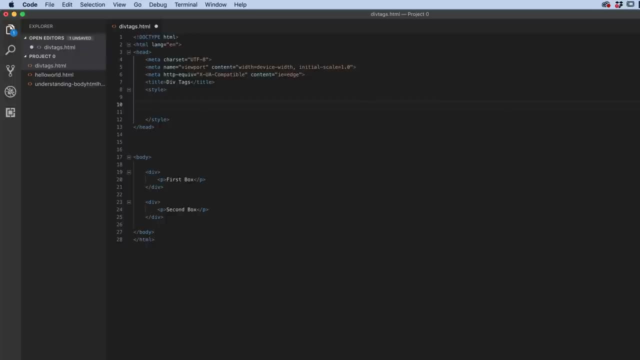 So instead of deciding all divs on every page are the same thing, let's create what's called a Class Selector. So all it means is I get to be unique. I get to say I'm going to create a class, To know it's a class and not like that Type Selector we just did. 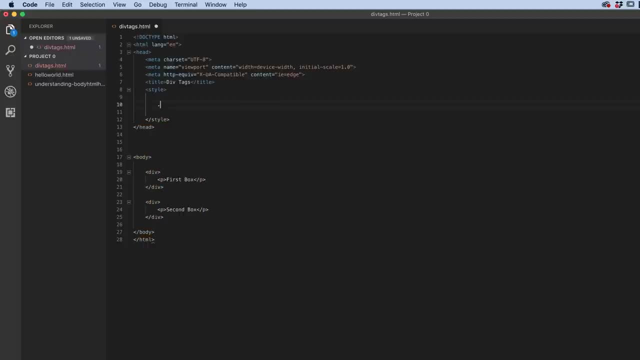 you put a full stop in the front of it in your CSS. That says: I'm a class. what kind of class? I'm going to give it a name? you can call it anything you like. We're going to call it Box 1.. 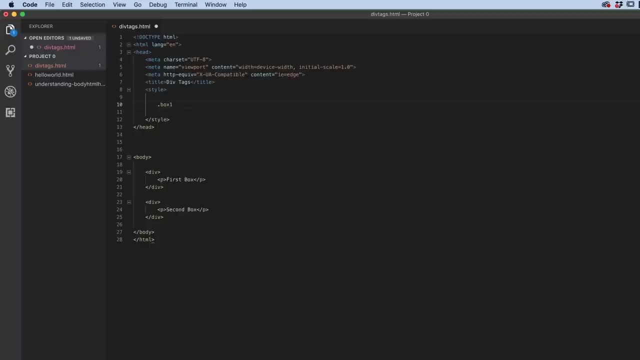 Okay. Okay Then, like the rest of the CSS we've been doing, it's the same. So curly braces return, and then we style it So that little full stop at the beginning means I'm a class. What are we going to do to that class? 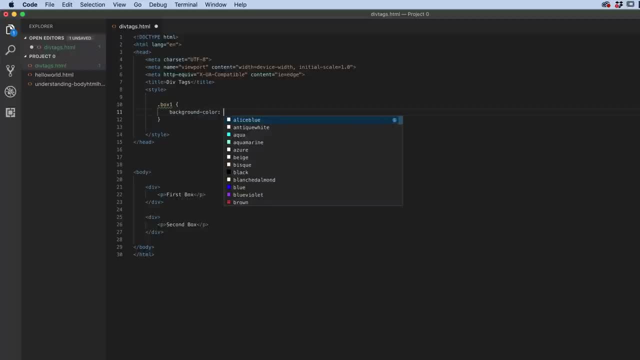 We're going to say it's a background color, Background color of yellow Semicolon. we're going to have a width and height With 600px by a height of 400px. Cool, so we've got Box 1.. 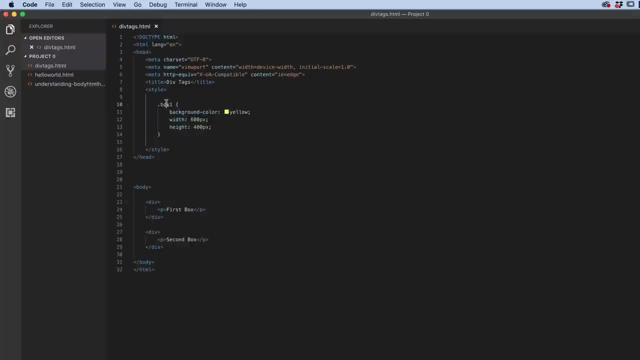 Now there's no way of kind of connecting these two yet. So it says, hey, Box 1, be yellow. But down here it's like I don't know what you're applying it to. So what you do is you leave the div. 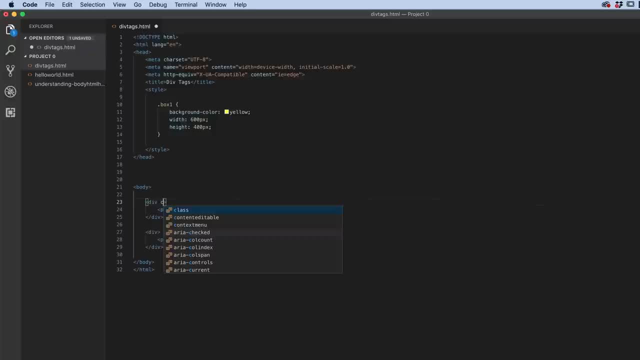 and what you do is afterwards put a space and type in the word class. You can see VS Code really wants to help out. If you're typing it out, make sure you put in the equals and the quotation marks. So we have a div class and what we want to do is apply Box 1.. 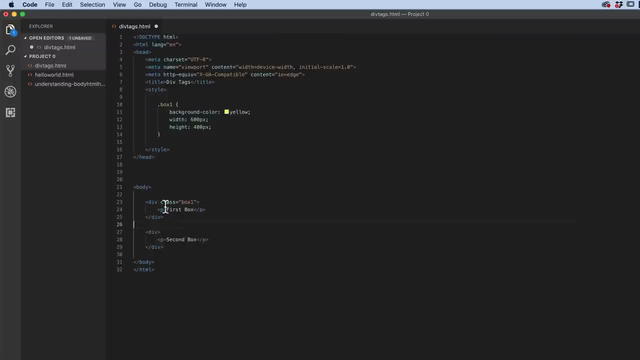 So now that is attached, The differences are just to make sure that when you're styling it up here in your CSS, you have to use the full stop to say: I'm a class Down here. you have to be a bit more long-winded. 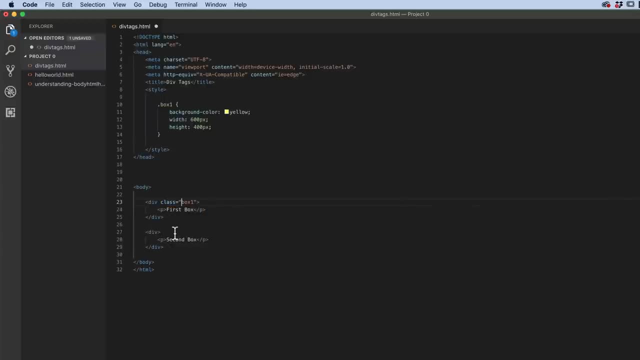 So you say class equals and you don't put that dot in there. That won't work. So class long version, short version. Now, hopefully, if we save and we go test it in a browser, we reset and the first box now knows it's yellow. 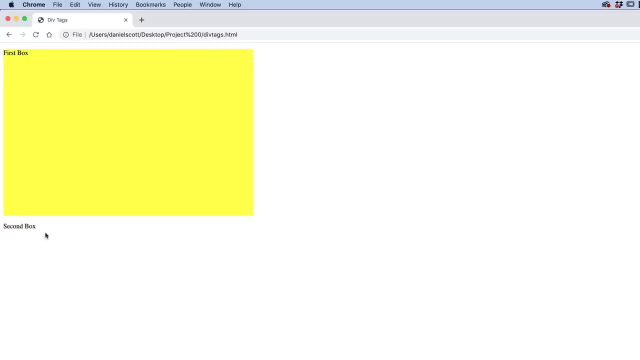 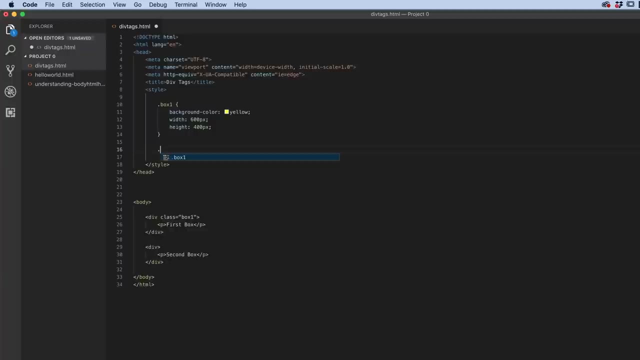 and it knows that it's 600px, 400px. this box down here has no idea what it needs to be, So let's tell it It's the same before let's make a second class. You ready? So dot box 2.. 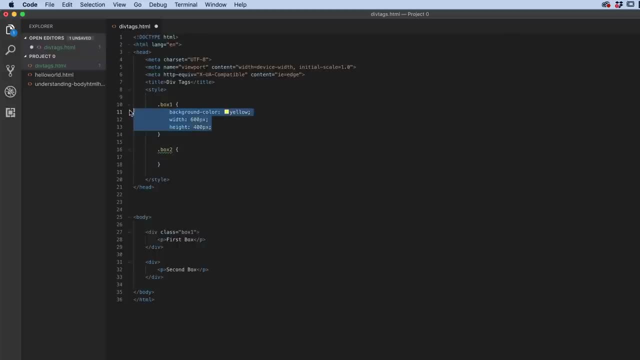 Put in curly braces and we'll tell it. we'll steal all this Because I'm lazy. But we want this one to not be yellow. we want it to be that pink color. That's not a color, it's to be pink. 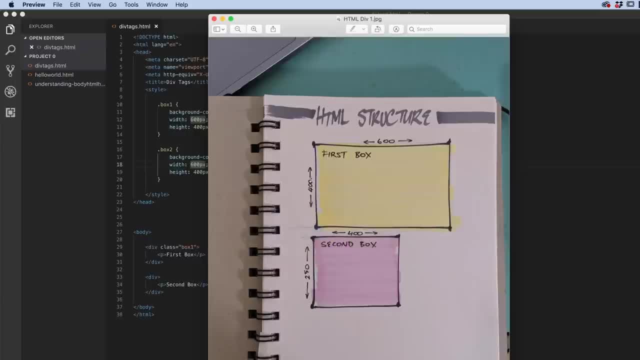 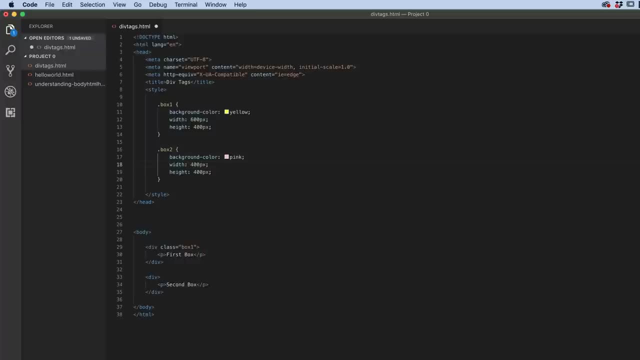 Save it. it's the wrong size and weight or size and height, 400 by 250.. So I just made up these sizes. you can type anything you like: 400 by 250, save it. and now it's not going to work. 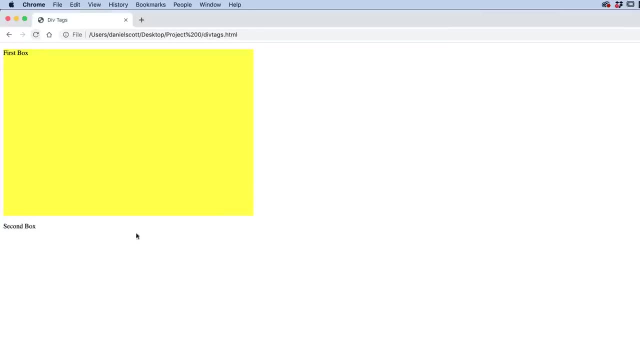 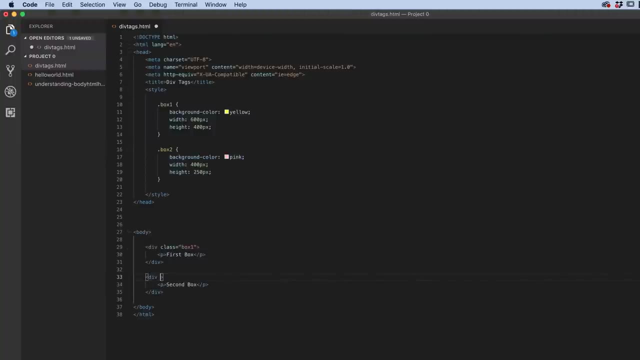 Why is it not going to work? Let's check, refresh, just to confirm it's not working. It's because we haven't applied it to it, So we've styled it. now we need to apply it down here. So, after the word div, type in class. 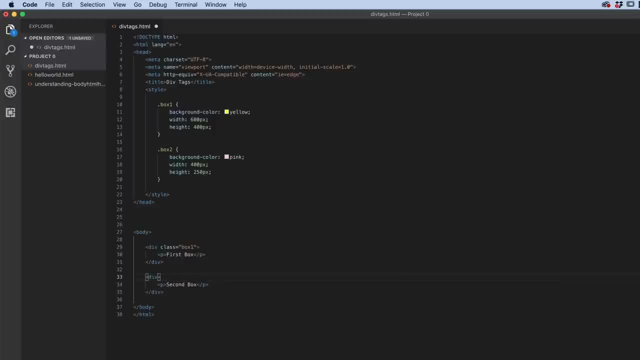 And you can see there the way I work. I'm going to work a little bit more shorthand as we work through. You can start writing all the syntax if you like, but you'll notice that I space hit C. that's all I've done. 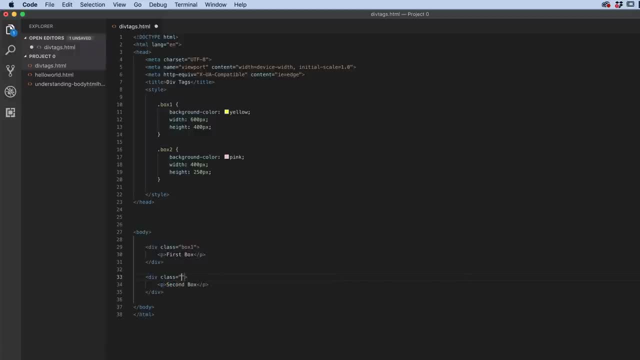 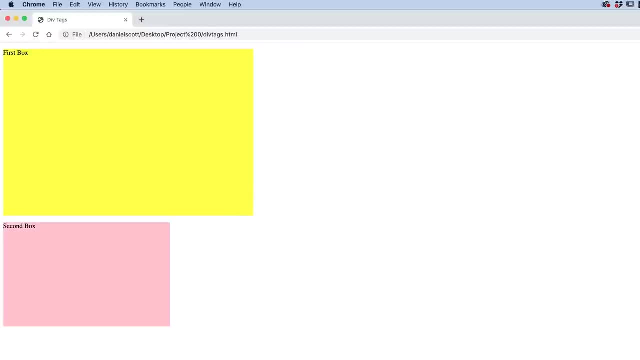 And I'm just going to hit return on my keyboard or the Enter key And it fills in all that lovely syntax. I type in box 2, hit save, Now hopefully refresh. There you go. we've got a first box and a second box. 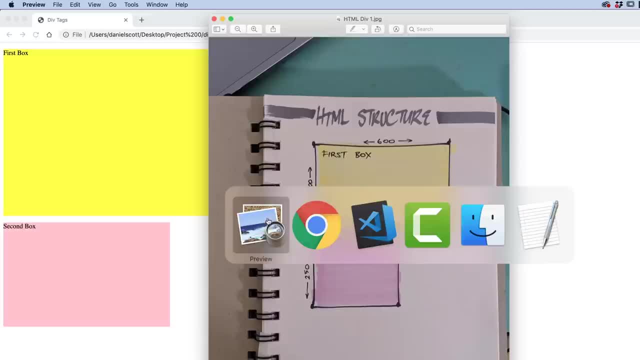 and it vaguely resembles this. So we learned what a Type Selector was. You don't need to remember that name. but a Class Selector for CSS is something we're going to do a zillion of in this class and it's a way of individually. 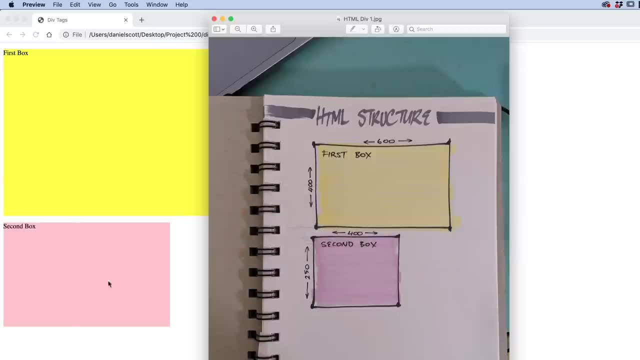 targeting this. So, instead of box 1, this might be header And this might be navigation and this might be main content. And we get to style them, color them and size them. Let's go a little bit further and add a little bit of styling to it. 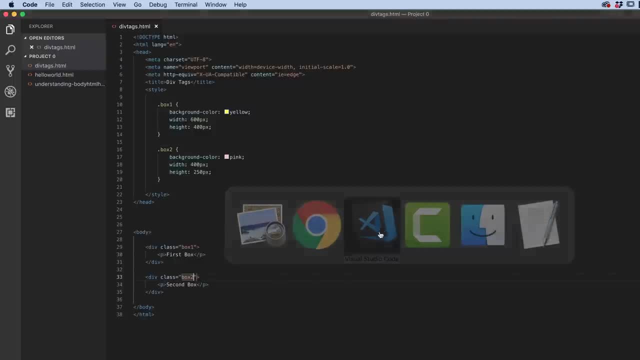 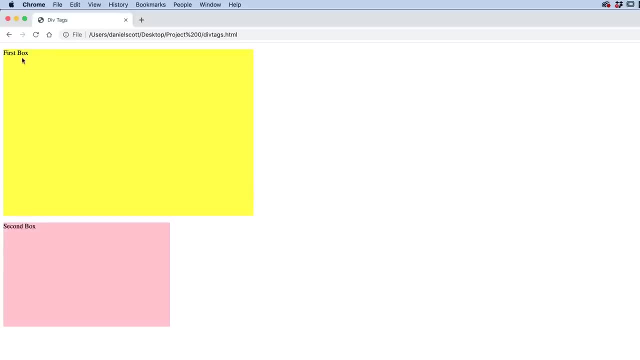 and look at a Class Selector, but in a different kind of context. So back in VS Code here I've got two P tags and they look exactly the same in the browser. Let's say, I want to make this one a different color and a different size. 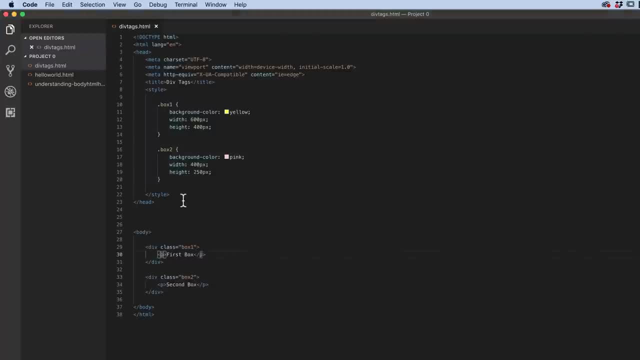 So, instead of styling the P tag like we did earlier, remember we made all the H1s, but the problem is, is that's every H1 on every page, Whereas this one? I just want this little unique guy in the first box to do something. 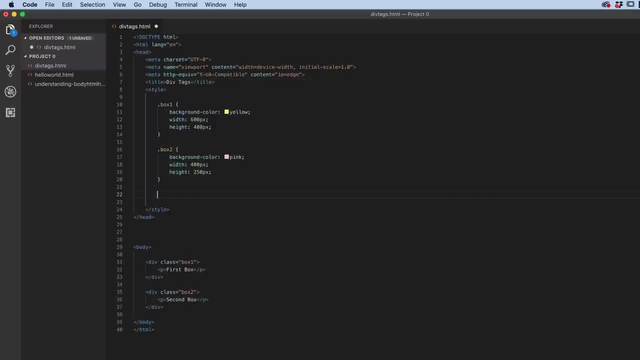 So up here underneath box 1, or box 2.. I'm going to put in another class- remember it has a full stop- And I'm going to call this one my highlight Highlight. that's highlight, Highlight text. 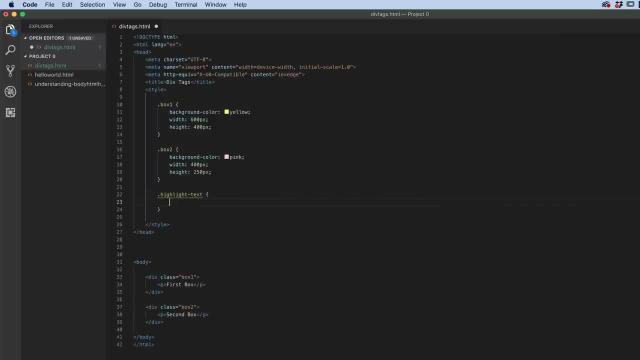 You have to put a space in, then you have to put in your curly braces, Your curly braces next to your P key, And then we're going to say: I'd like you to be a color, remember background color for the background color. 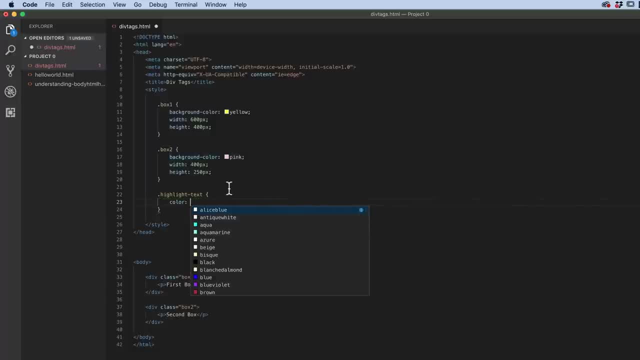 Just regular old color. if you want to style text And let's say I want to make this, what are the crazy colors we've got in here? I'm going to make this dim gray. They spell it both ways. look at that. 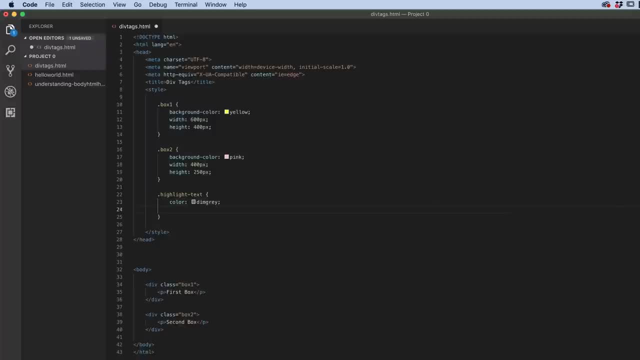 All right, let's put in our semi-colon And let's make the font size so font size, Just something really big, so we can kind of just easily see it. So I've saved it. now I need to apply it. 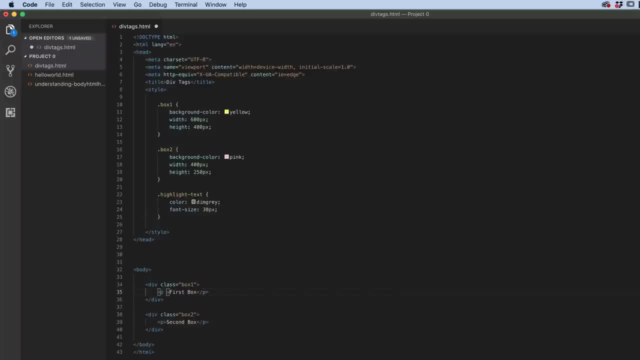 And it's the same thing. I can say U. there's a P tag, but also a class of dot, not dot. it was a test. I failed my own test. Highlight text. Let's save it. let's check it. 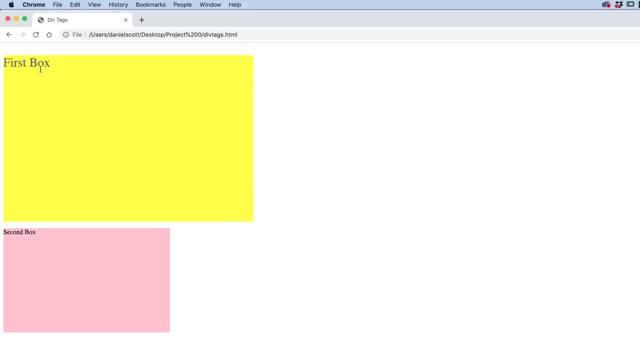 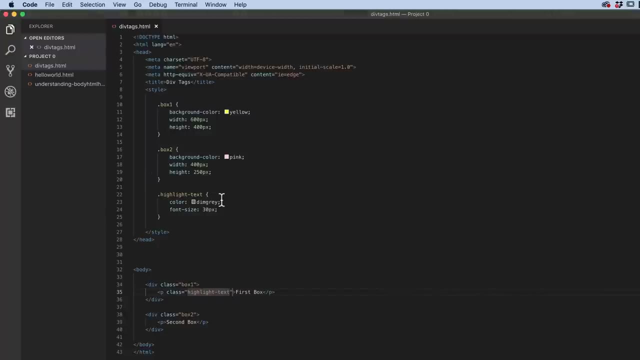 Refresh. hey, it is bigger and it's the gray. So you style the type selectors to do kind of big general broad strokes. Then you do little specific things using classes. You apply them to individual little bits and pieces. you can use it twice. 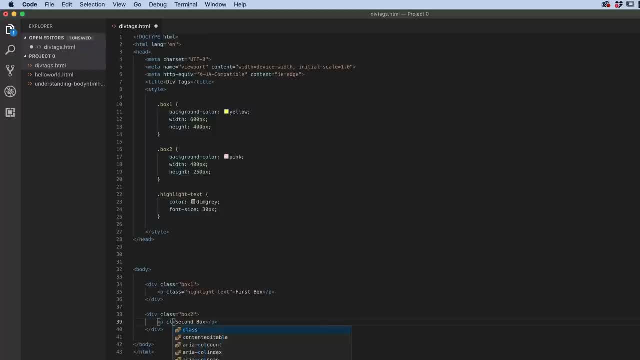 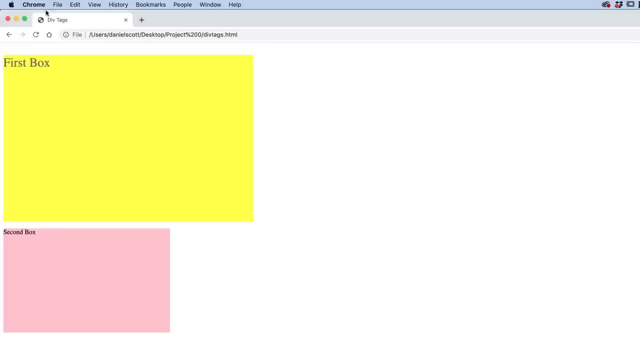 There's no reason why we can't say: you, my friend, also have a class of highlight, Highlight text And it will apply to both of them. hopefully It didn't. you're like. you see why? I have no idea why. 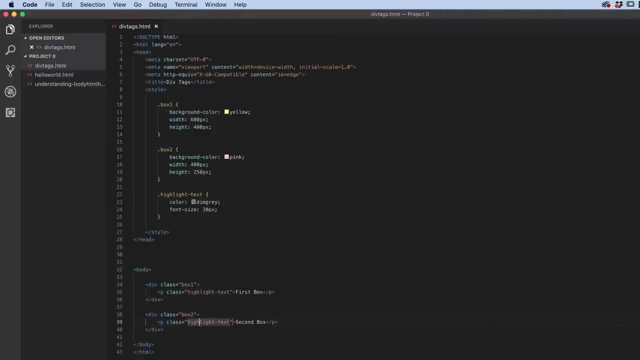 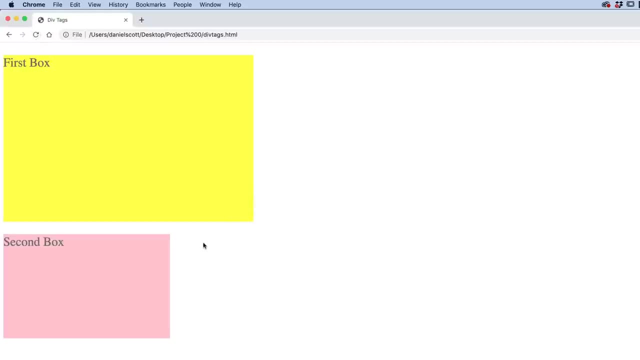 Because Now I pretend like I put that in there on purpose. but that is always my problem. You might not be as grammatically challenged as I am, but I find it very hard to type this stuff in, So like when I'm not doing tutorials. 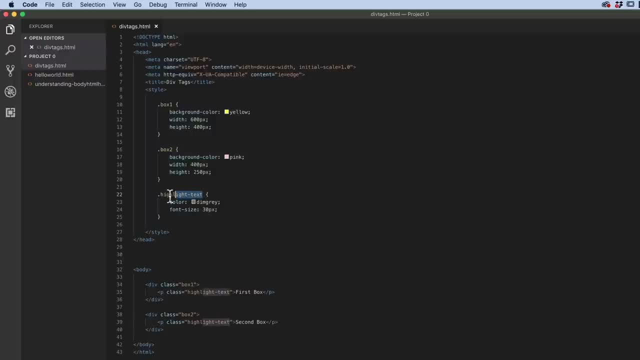 and trying to impress you with my typing speed. I copy and paste everything. Copy and paste. It is painfully slow, but it gets around my problem of typing the wrong word in and then trying to fix it, not working out what it was. 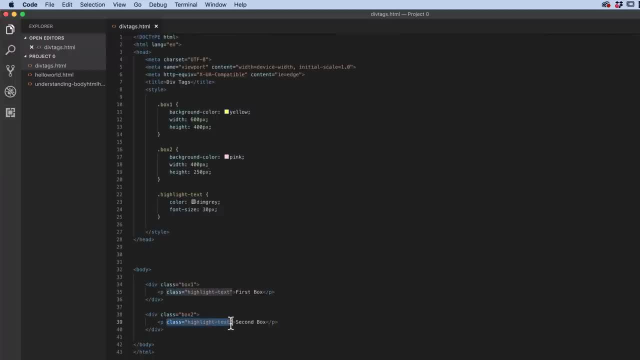 it's just because of typos. Let's delete this and I'll show you some other tricks for kind of just making sure, yeah, you can keep up or fix any errors. So the easiest way is to compare against the file that I'm making. 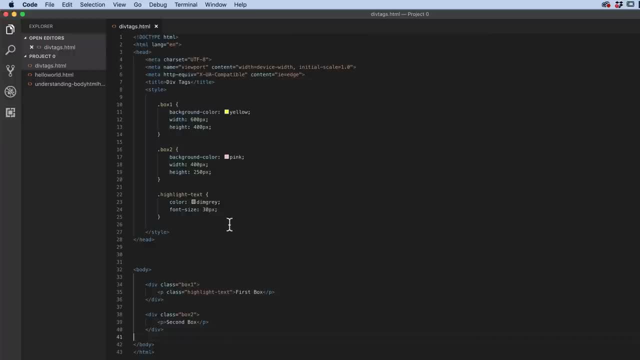 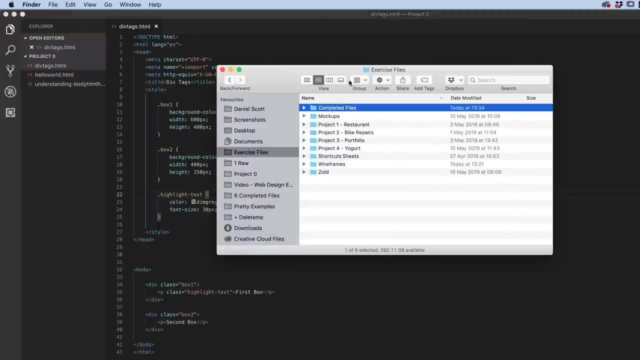 So say it looks like you've done the same thing but it's not actually working for some reason, is in your exercise files that you've downloaded? you will find in that folder there's something called the completed files, And in here I've zipped up. that was the fifth video that I made. 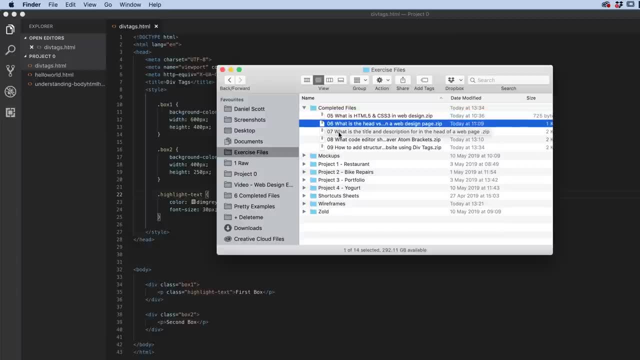 this is the sixth video, so if you're watching this video, it's probably what are you up to. I think video 10, you will find I haven't finished this video yet, so you'll find a folder in here called O10.. 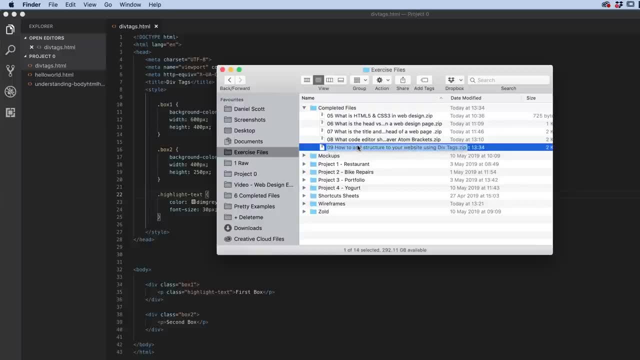 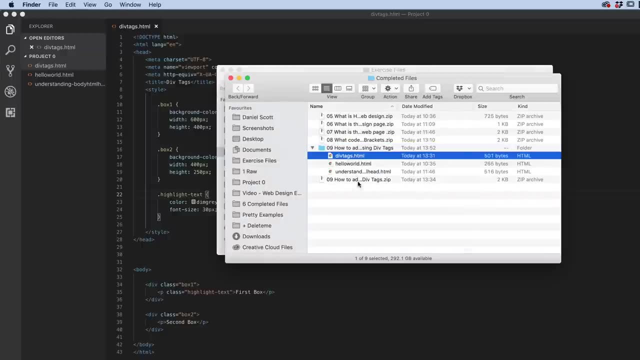 No, it won't be O10,, it'll be 10.. You can open that up and open up, so let's just do one. I double clicked it, opened it up and there's the stuff we're working on. 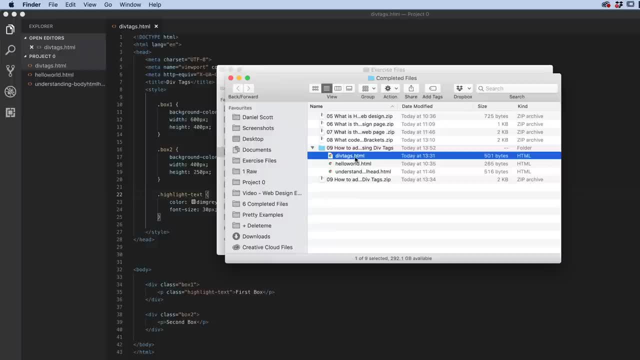 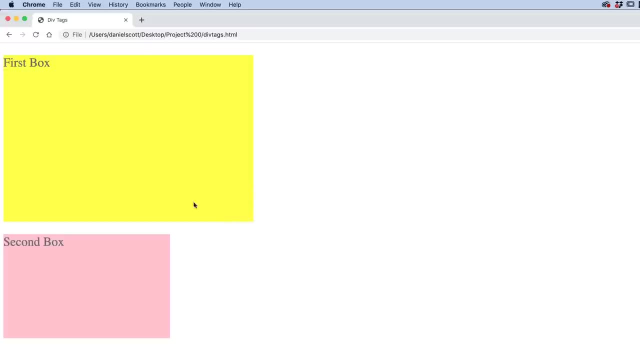 And you can just open this in VS Code. So go to File Open and compare yours versus mine, And I'll do that throughout the course. That's one of the ways you can check your code. The other things to note or, I guess, to check: 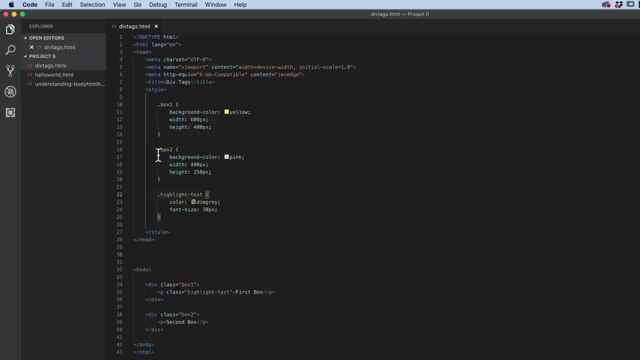 and these are the things that I find my students run into when I'm teaching live classes- is people forget the full stop to identify a class, Or they start adding the class dot down here, which you're not meant to One. that always catches people out. 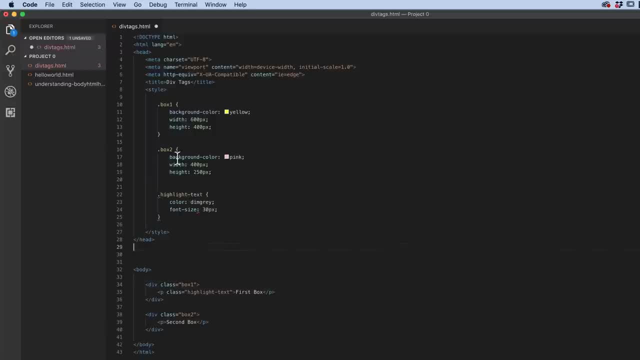 is they'll accidentally delete one of these with the curly braces, And because that one opens and then doesn't close, it kind of freaks out a bit, doesn't it? You can see it's changed the highlighting color a little bit. 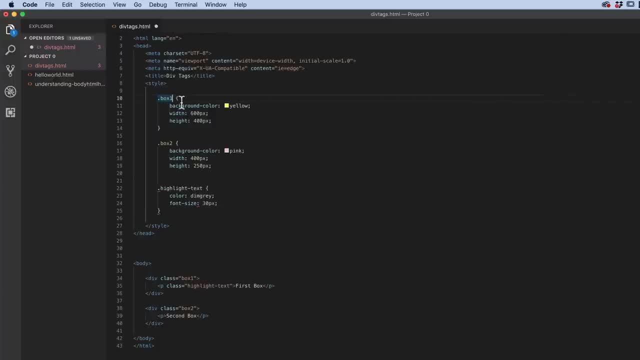 but it's just kind of missing So often. you can go through, click on this, find your, click on that first bracket and you can see it's highlighted- the closing one. If I click on this one, it won't click on it. 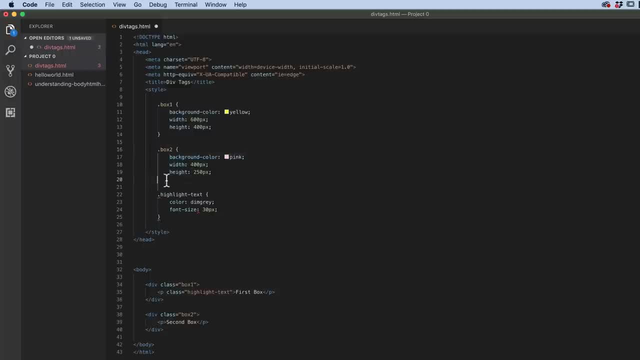 because it doesn't know where the ending is, So it won't highlight its buddy. Let's put his buddy back in there he is Now. if you click on them, they kind of just connect to each other. There we go The other things: are people forgetting to put colons in and semi-colons in? 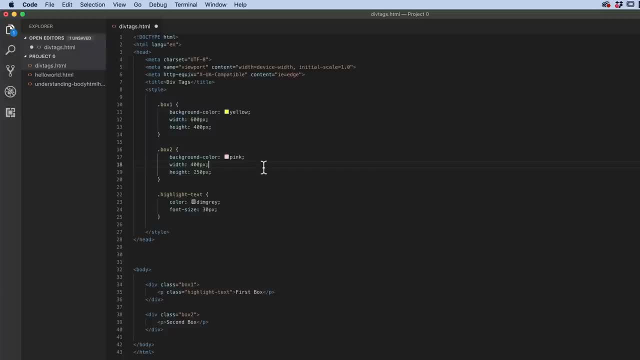 Just basic syntax problems, Basic spelling mistakes, like I do all the time. We'll do a bit more error checking. later on We'll install some plugins for VS Code to help us with that syntax errors. but for the moment those are the basic ones and that'll be it for this video. 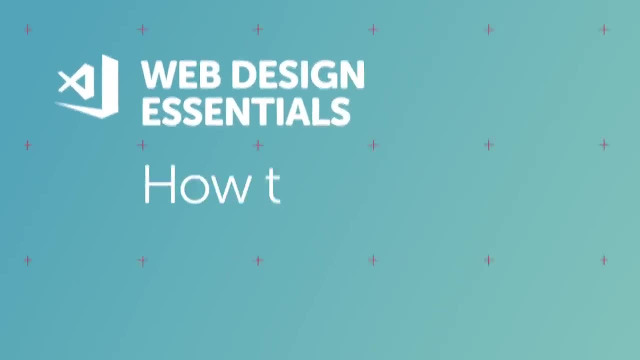 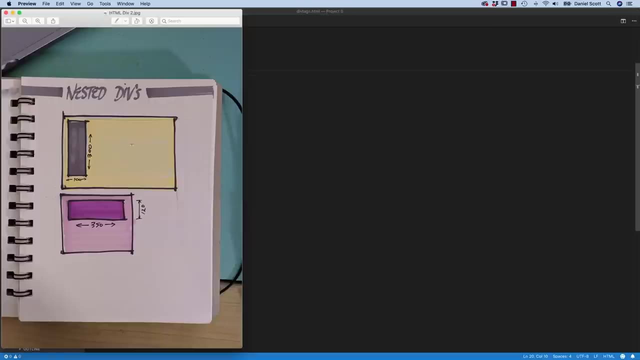 Let's get on to the next one. Hi there. in this video we're going to talk about nesting div tags. All it means is we're going to end up doing this where we have our original yellow and pink box and we put other boxes inside of it. 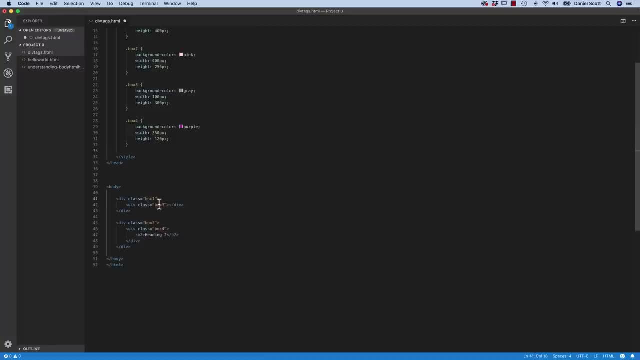 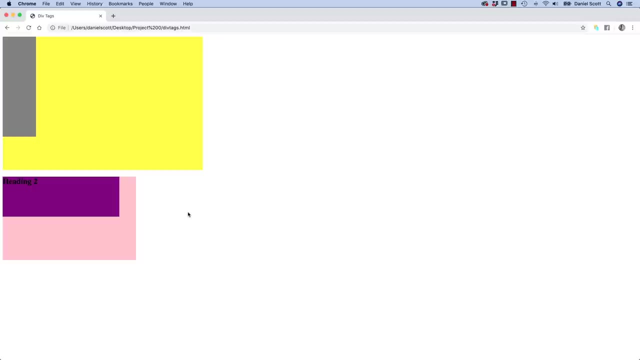 It's called nesting. it's not that fancy. You can see here boxes inside of boxes. they end up looking like this: in the end, We're going to put text inside of boxes which are inside of boxes. Yeah, let's do that now. 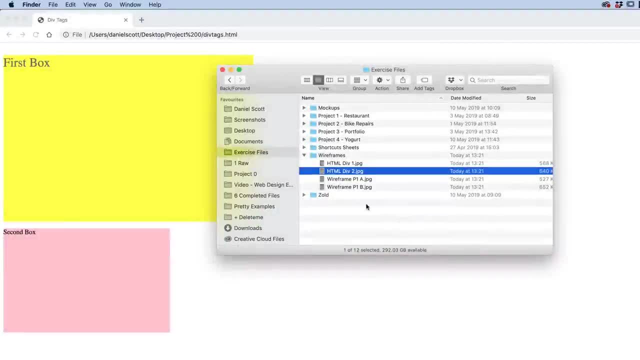 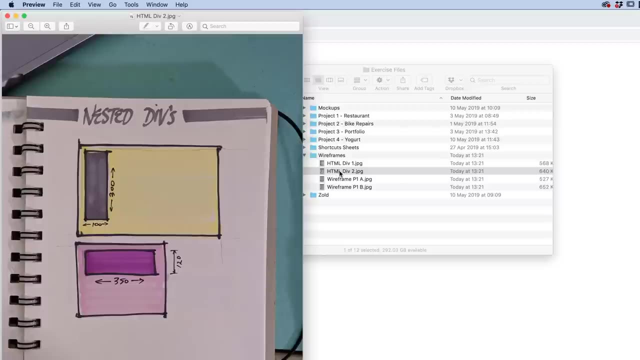 I'll show you in VS Code. let's go All right. what we're doing is in your wire frames folder in your exercise files. we're looking to make this one here, HTML, Div 2, so same boxes. We'll use the same thing we've created so far. 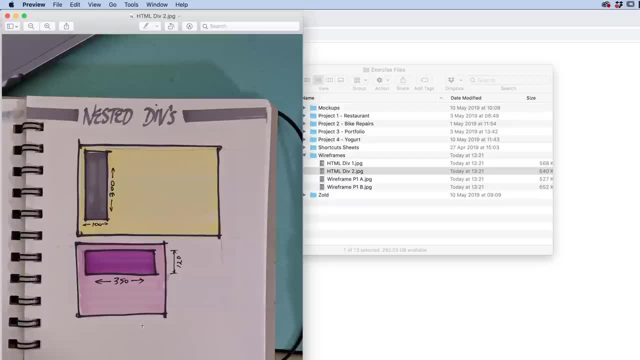 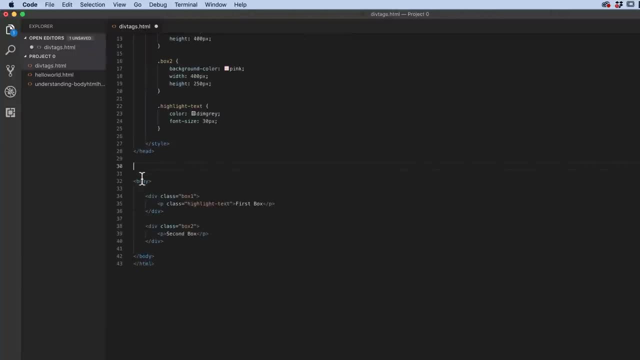 and we're going to put two boxes inside, a gray box and a purple box. Those are the heights. let's work out how to do it. So in VS Code, we're going to do what's called nesting, Just means we're going to put divs inside of divs. 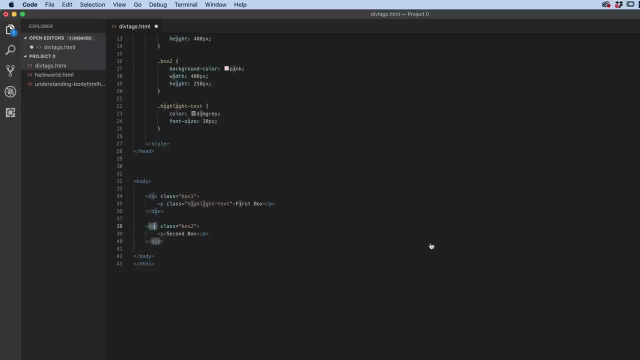 So we have one div here and a second div here. Let's work on that first one, which is going to be our gray 100 by 300.. So where does it go? Depends on where you want it, I guess. 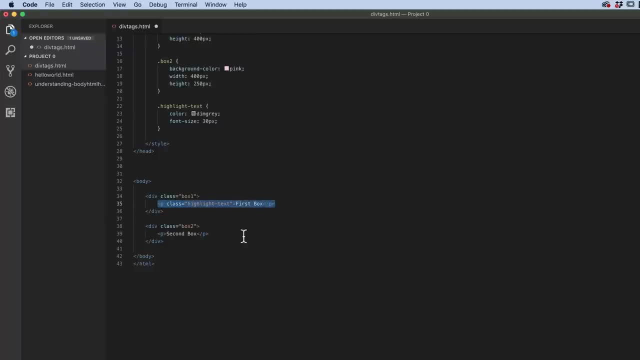 We've got this text in here. we don't really want anymore. That was just. I guess I put that P text in there to show you how we could highlight and just so the box will have some content in it. Let's delete that for the moment, just to make it nice and clean and clear. 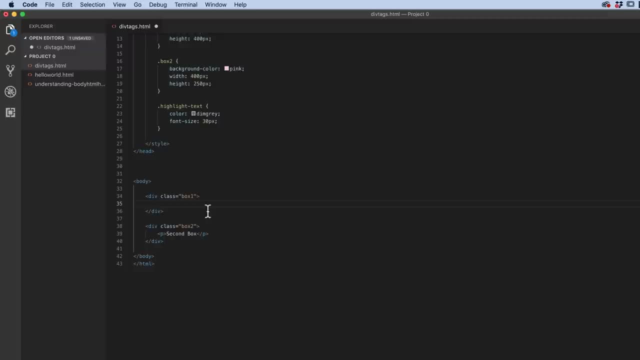 So what we're going to do is put a div set just where that P tag was. So if we go angle brackets div- Now we're not going to make a div, then create a class up here, then come back and name it. we're going to do it all in one go. 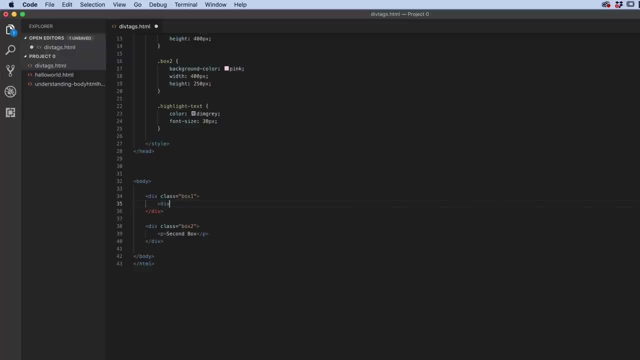 So instead of just closing it off here now, I'm going to undo that I'm going to put in class before I finish it. Then I'm going to call this one call, box 3.. Then I'm going to close it off, just to save some time. 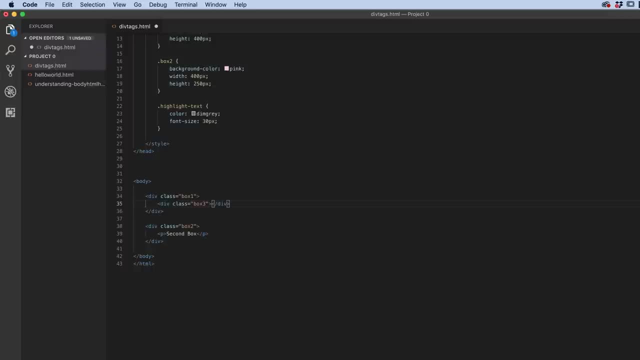 rather than coming back and doing it later, I'm going to put: should I put anything in it? No, I'm just going to leave it empty. But remember, this is where it would go inside of that div. Let's leave it empty. 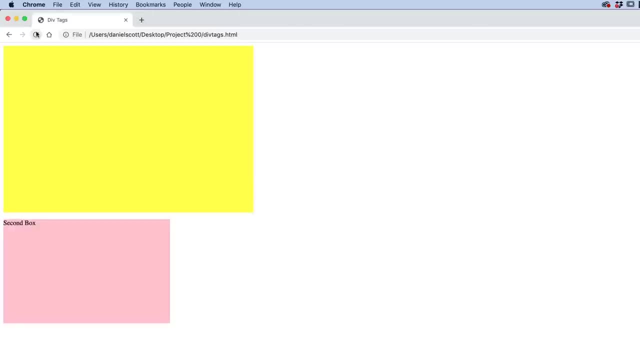 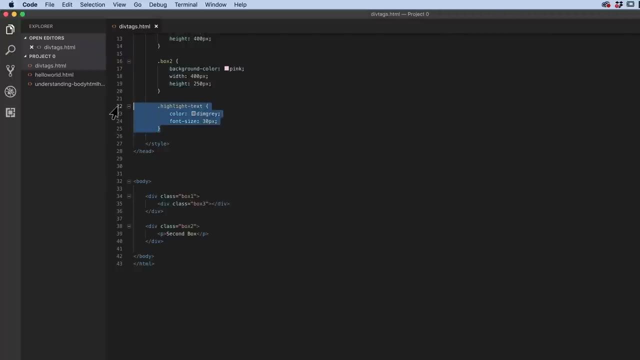 Let's save it and it's not going to appear yet. Refresh. the text is gone and the div tag is in there, but I can't see it, So we need to style it. We do not need this anymore because I got rid of it. 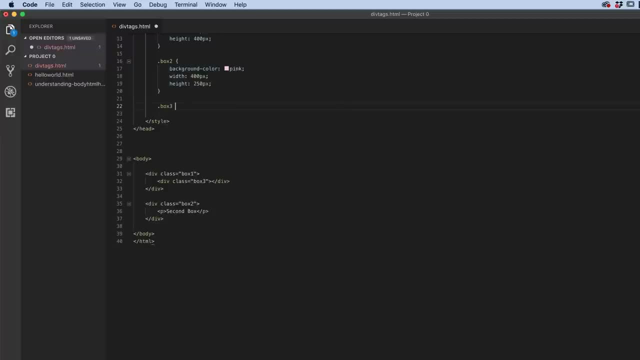 I'm going to call this one dot. remember box 3. Curly braces, and we're going to steal all of that And we're going to pick gray, which is spelled both ways. Wow, I get caught up with that every time. 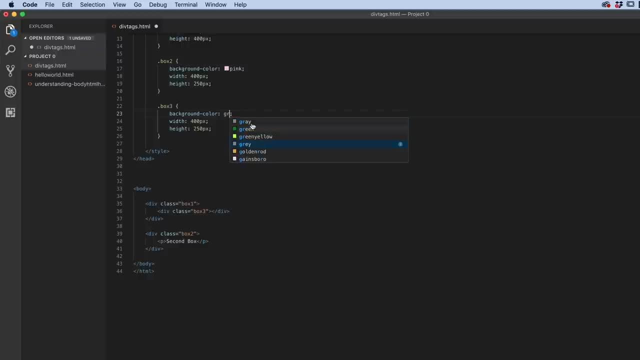 Gray. look, Gray and gray. I don't know why. I find that amazing. It's the same gray just spelled the different ways, And this one was a width of 100, and a height of 300.. There we go. 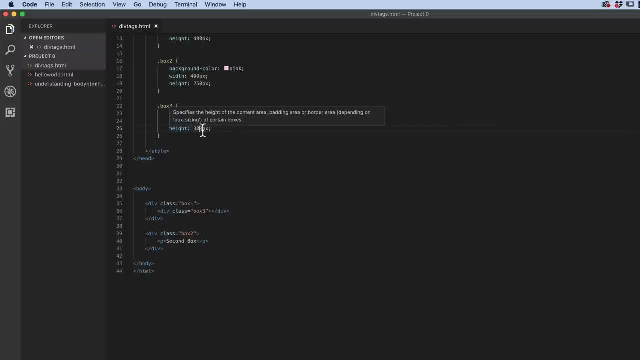 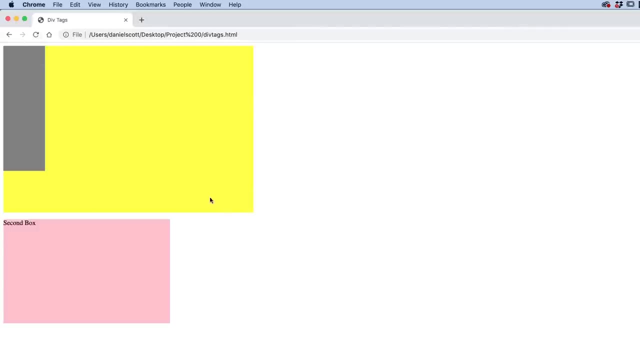 Or 3000, that's not going to work. Let's save it and let's check it out. Let's see if we made it work. Refresh, look at that So often when you're making a website you'll make kind of like an overall website background. 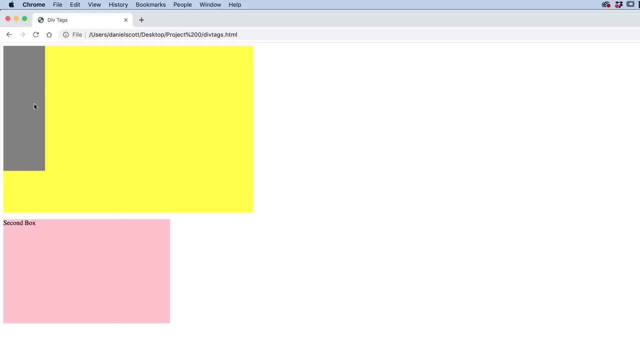 a big container and inside of that container you'll nest lots of different div tags, Like the header and the navigation and the images and the carousel and all those things That's nesting. Let's do it with the second box. 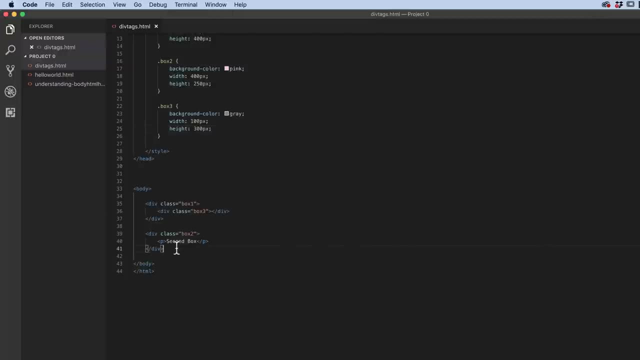 And I just want to show you a couple of things, Like: if you don't get it in the right spot, so let's delete that P tag from here. That's where it should go, but let's say we do it just outside of here. 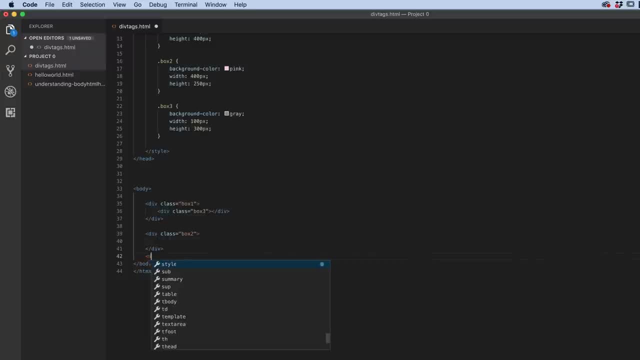 So let's go. angle brackets- div space class return. This one's going to be called box 4.. Close it off with the angle bracket, hit save At the top. here I'm going to copy and paste the whole thing: real lazy. 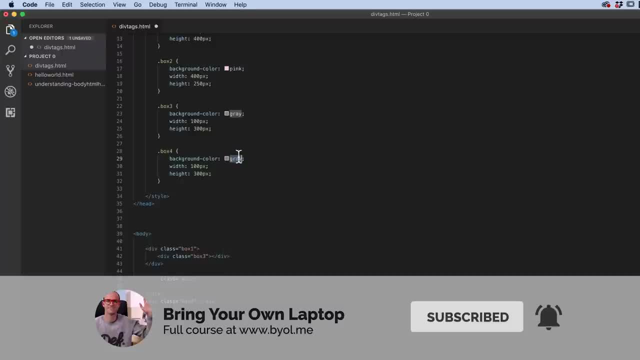 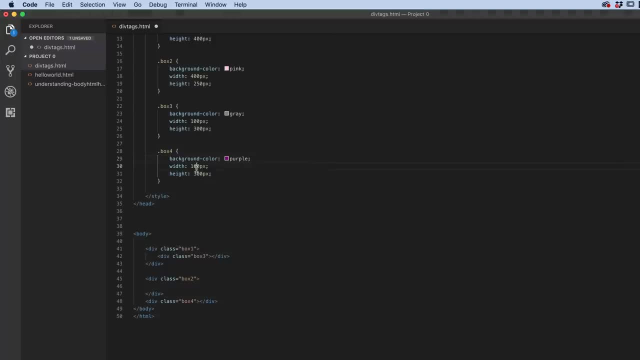 Box 4, this one was purple. Was it purple? Yeah, purple Purple, and it was 120 by 350.. Wow, it's actually 350 by 120. Height of 120.. Let's give it a look and preview in the browser. 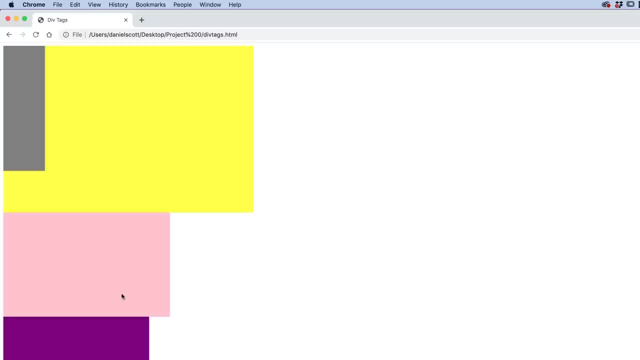 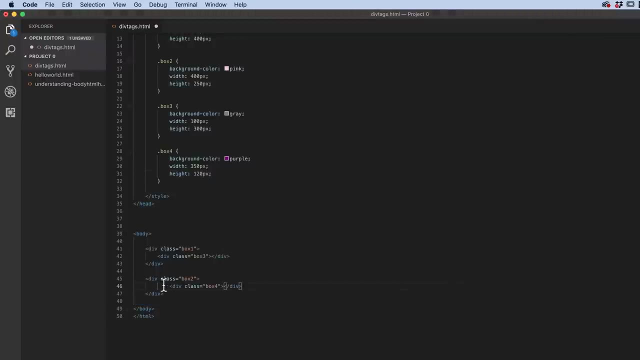 Awesome. Well, not awesome, It's in the wrong place. So if you get it in the wrong place, it's really simple in the code to go: Actually you cut and you paste. I'm going to line it up so it looks nice and all aligned. 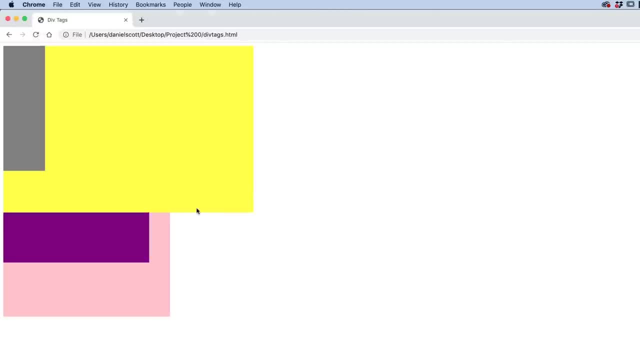 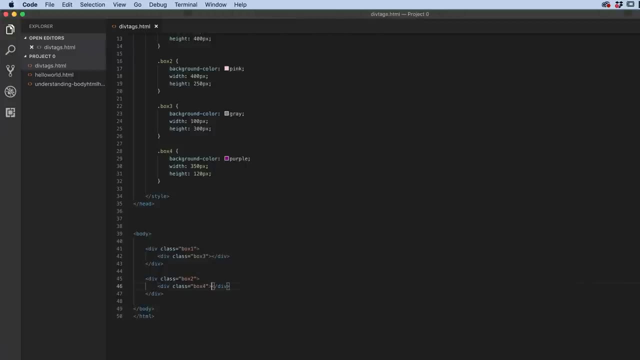 Hit save and now refresh. it should be in there. awesome. Now if I want say an H2 inside of that purple text, So here I could just put it here. There's nothing wrong with typing H2, closing it off and typing it in here. 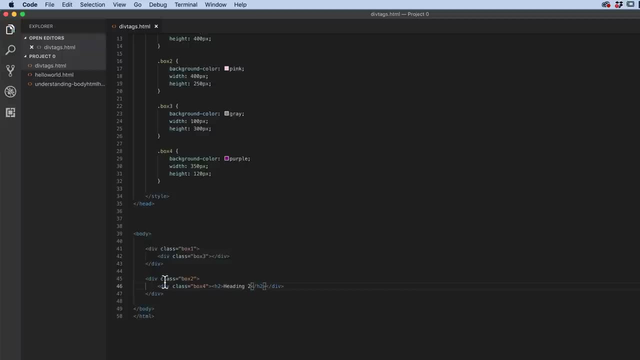 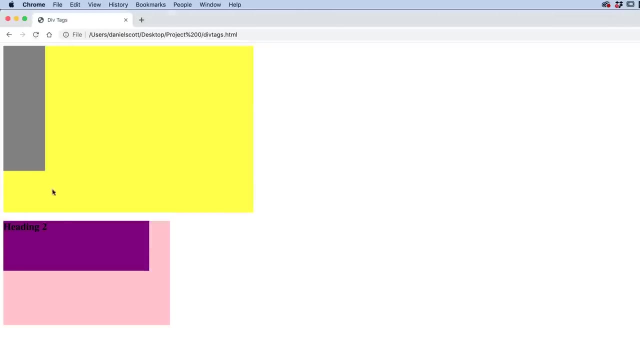 Hitting 2, and that's perfectly grammatically and syntactically. I doubt that's a word correct, so let's give it a preview. It's in there what ends up people doing What I like to do to make everything look nice. 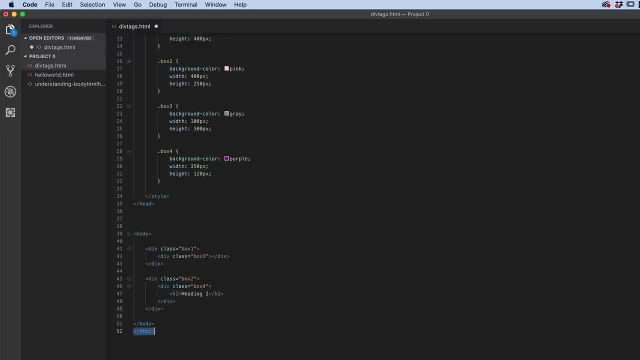 is put returns in between all of this to really expose the nesting. So I know that there's a body tag. inside of that is a box 1, inside of that is a box 3. You can kind of see the indentation, same with this box 2.. 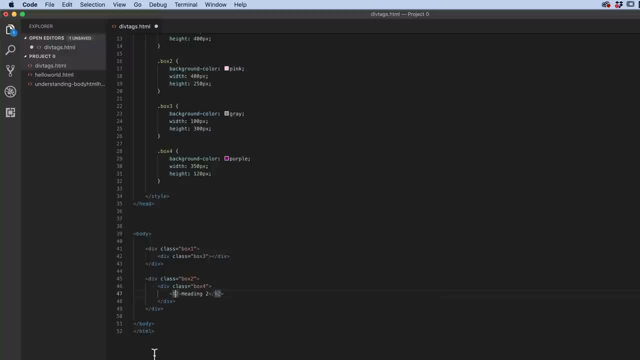 And inside of that is box 4, and inside of box 4 is H2,. does that make sense? All right, so we're getting the hang of this div tag, division of space thing and putting boxes inside of boxes. Let's get on to the next video, where we set our class project. 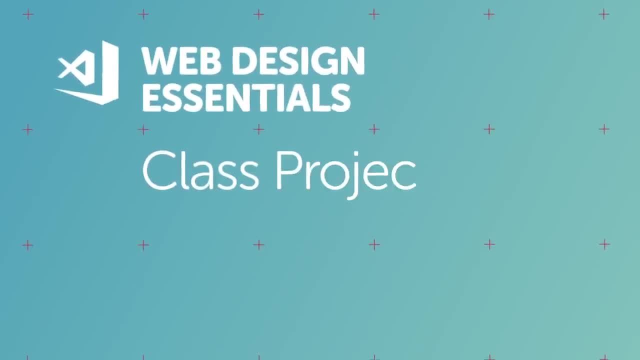 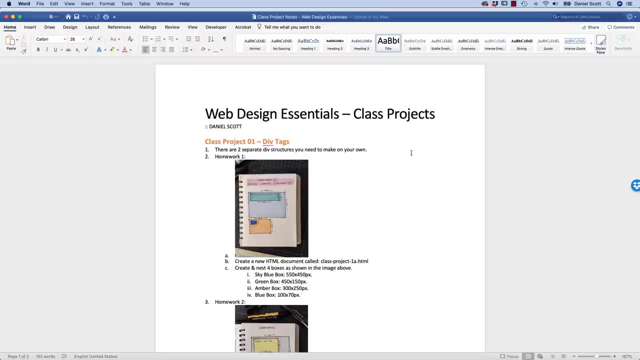 Homework time. Did he say homework in the last video? I did but think of it more as like an awesome way of getting your skills better. So I'll set projects throughout the course. You'll find the details of them. I'll make a little video like this to explain it. 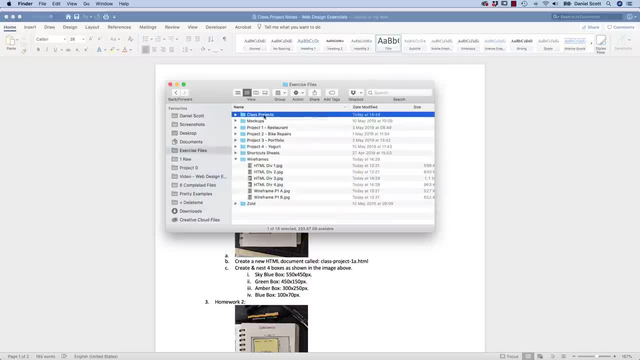 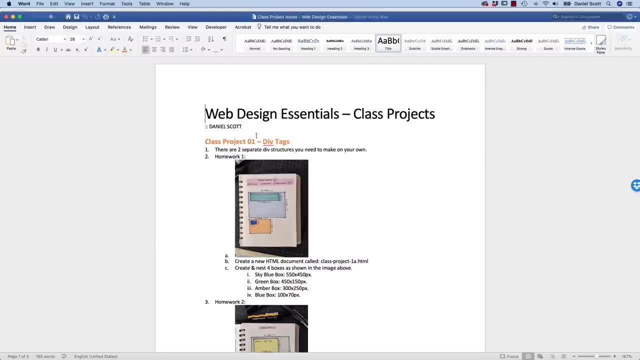 But also in your exercise files. there'll be a folder called Class Projects. There'll be a Word document in there and that's what it looks like. We're up to Class Project 01.. So we're going to work through what you need to do. 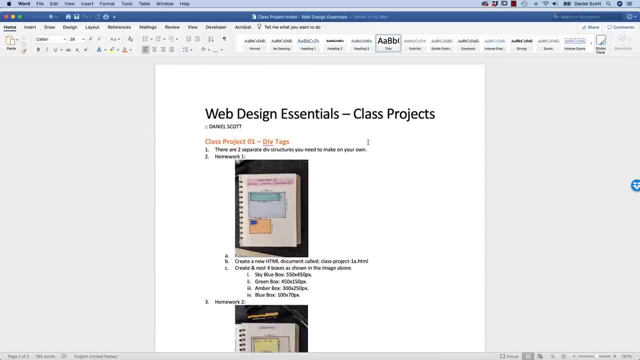 and I'll keep adding to this as we go through the course. If you don't have Microsoft Word, you can open this document and lots of other programs. If you get really stuck, try Google Docs. You can use that to open a Word doc. 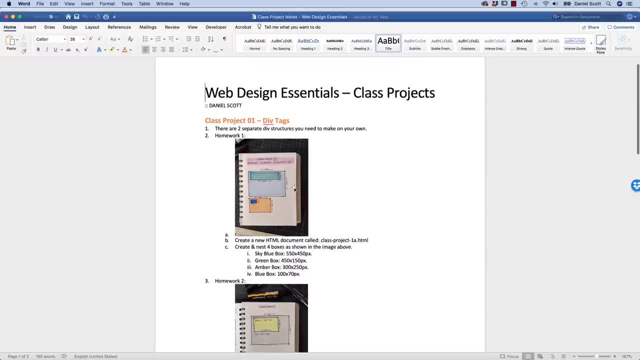 Anyway. so what do you have to do? You have to create two separate websites. So what I do is, in VS Code, close down everything and make a new document. So you're going to make a new one. The first one's going to be called Class Project 1A. 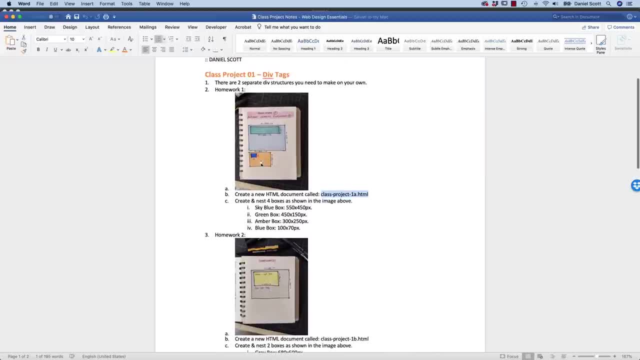 There's two parts to this, 1A and 1B. So the first one is this: I want you to make this. I've given you a bit of the details, so the name of it. These are the boxes and you can kind of see in this visual here. 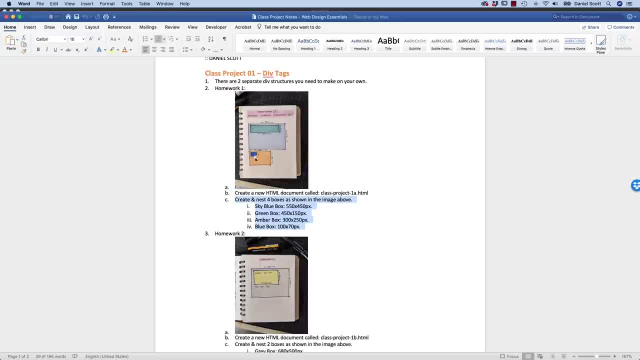 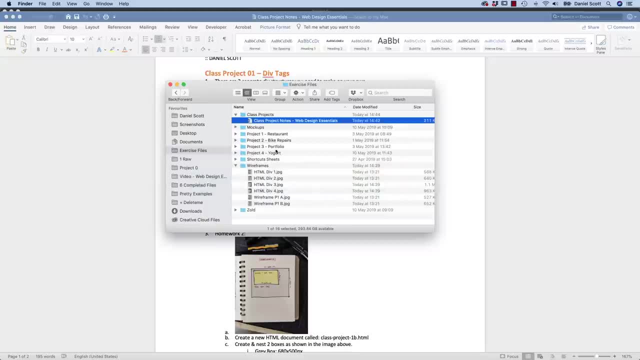 the nesting I want you to do. Green box is inside the blue box, etc. The sizes are down here because my handwriting is not great. There are larger versions of this. You can either make it bigger here in Word or in your exercise files. I'll put a copy of them in wire frames. 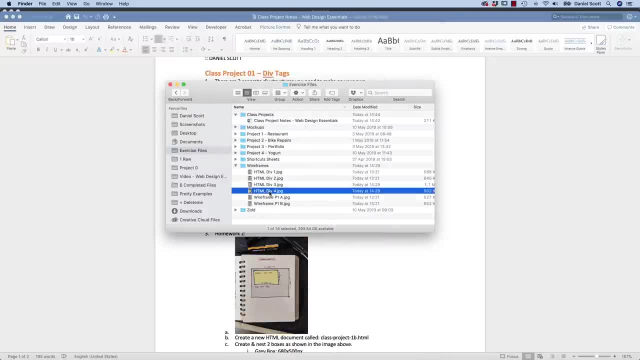 and it is div 3, there. it is there and div 4.. So those are the two things. you're going to be making This one's pretty easy. we've done it before. This one's a bit of a curve ball. 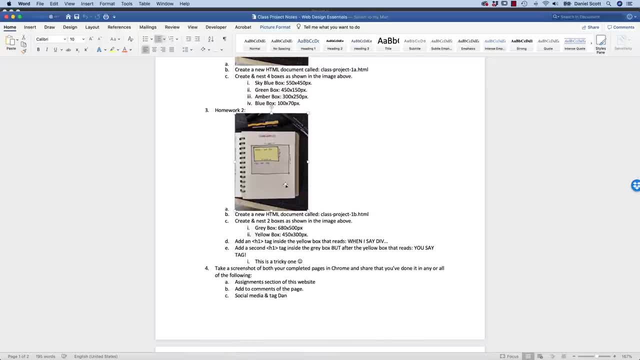 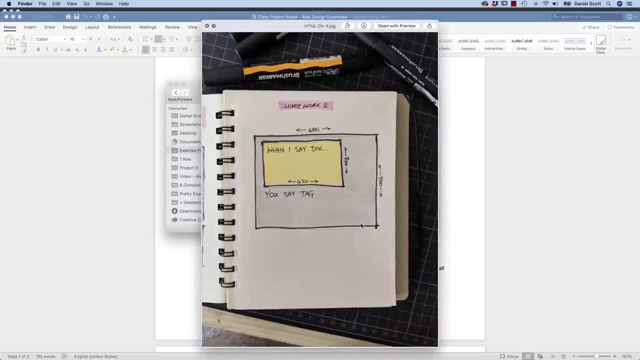 because I want you thinking about div tags and how they work. So this one. let's look at the second one. The difference is we've got two boxes inside of each other. That's easy: yellow box, gray box. But then I want you to put it. 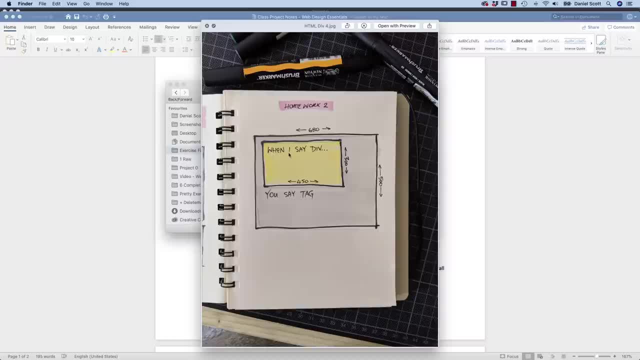 in two H1s- there's one inside this yellow box- And put some text in it. doesn't have to be what I've written here, but some text in this one and then some another H1 out here. How do you get it out there? 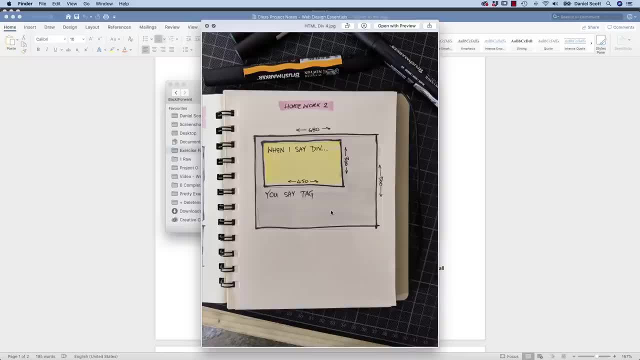 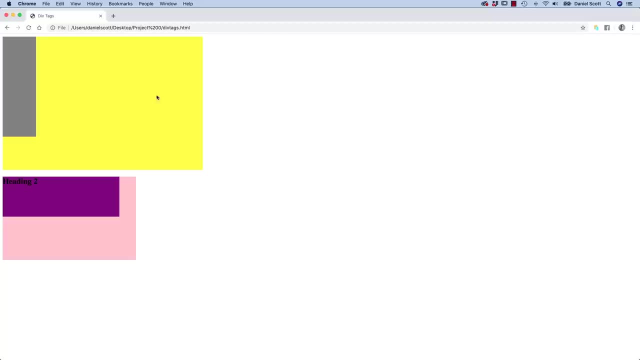 So it's kind of like it's outside the yellow box but inside the gray box. So I want you to play around with that. Once you've done it, say you build it all in Visual Studio Code, I want you to preview it in Chrome and take a screenshot. 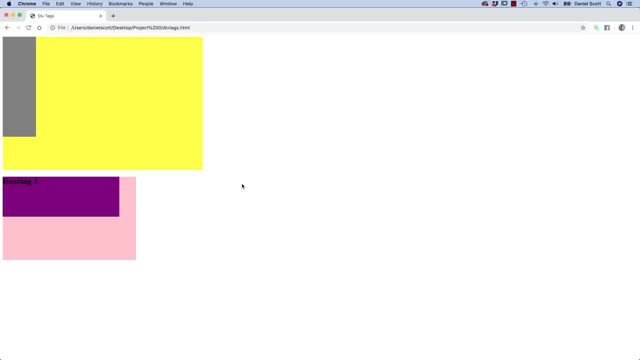 Now on a Mac, you hold down Command Shift 4. And you can drag a box around it: click, hold and drag, And that gives you a screenshot. you should put it on your desktop. You can see mine down here. 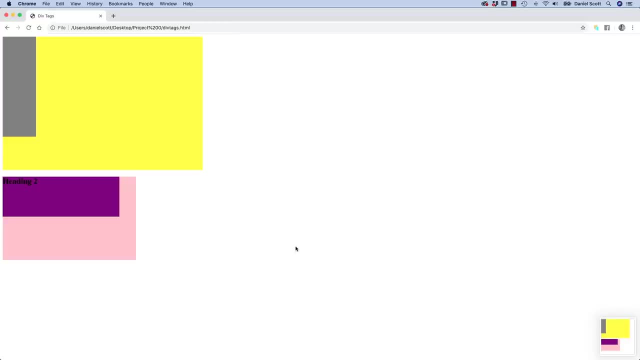 And I want you to share that with me. On a PC it's different. You've got a Print Screen button on your keyboard. You might have to double check that how to do it on your version of Windows. It's different on lots of different versions of Microsoft Windows. 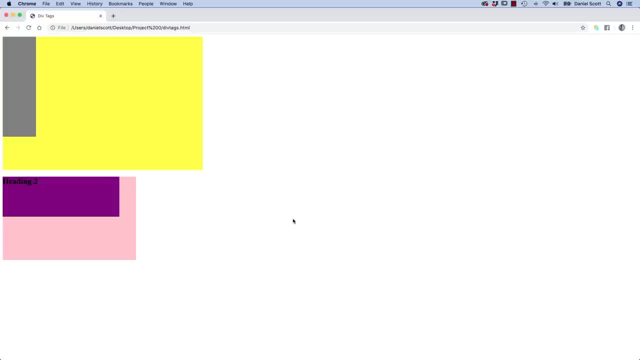 and I'm not up to date with them all. So just check out how you do a screenshot. I think it's just Print Screen on your keyboard and then you can paste it, But the reason is I want you to share it for me. 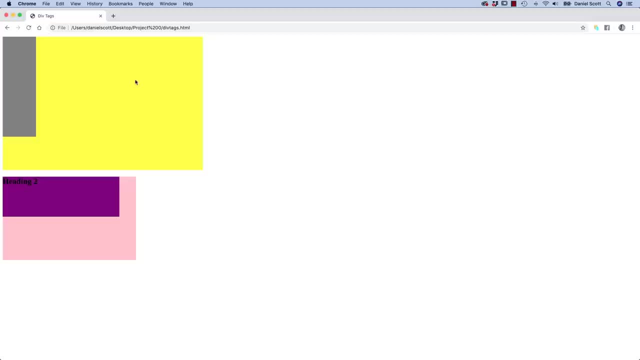 because I want to hold you accountable to these things. I want you to prove to me you've done it. All you need to do is share it in the comments here. just say, look, I did it, And if you run into any problems, drop it in the comments. 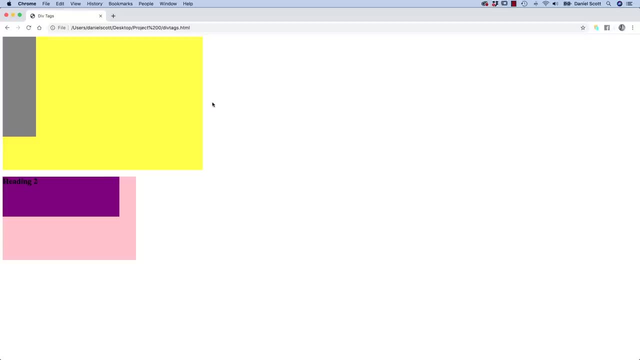 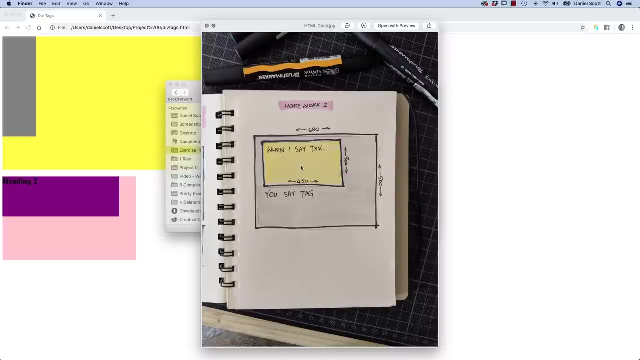 And what I'd like to do, because we're at a reasonably simple stage. if you do run into a problem and you're like I can't make this one work, post your questions in the comments and ask for help And for the people that are doing this course that do do it successfully. 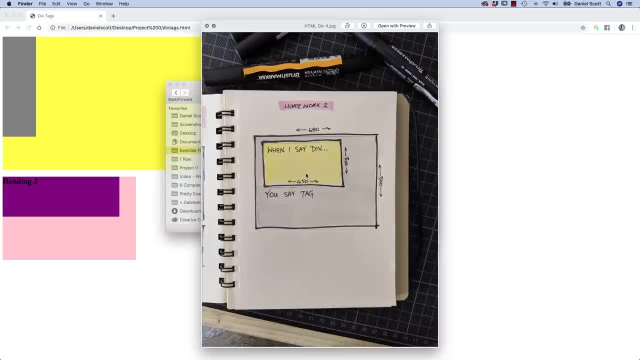 I want to kind of instill a bit of helping everybody else out. So if you're in there and you're posting yours and you did it and you're like, yeah, I did it, Go in there, and if somebody has a problem, 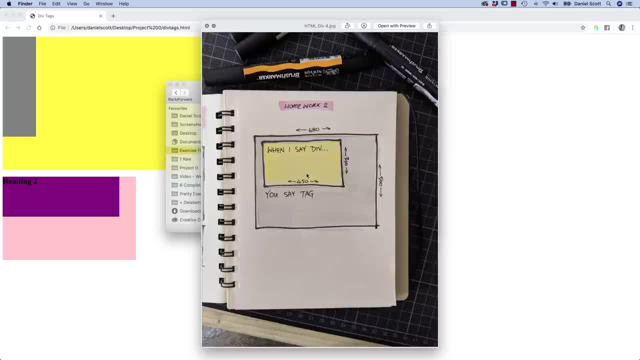 and they're like: oh, mine's not working because of this X, Y and Z. you can help them. just explain what you did to make it work. Get this bit of text outside of this tag. I want to kind of instill this in the group. 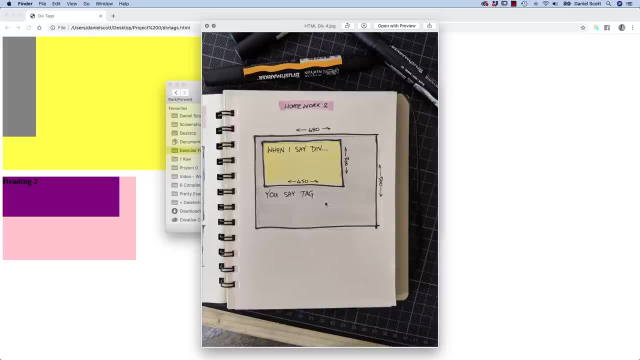 so that we're not just all relying on me to kind of go in and start working on everybody's code. I'd like you kind of to help other people so that you learn it better. You get what I mean, right. So where do you post these things? 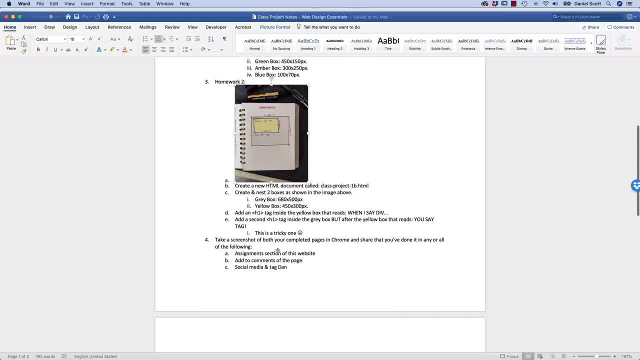 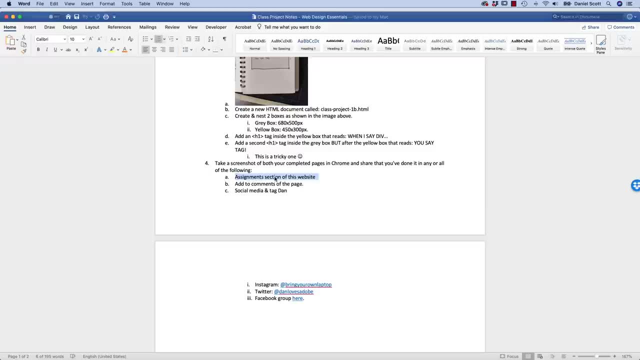 So you've taken two screenshots and your Microsoft Doc explains it. It says: depending on which website you're viewing this on, you might have an Assignments section. there might be a place to actually put it or there might just be a place in the comments. 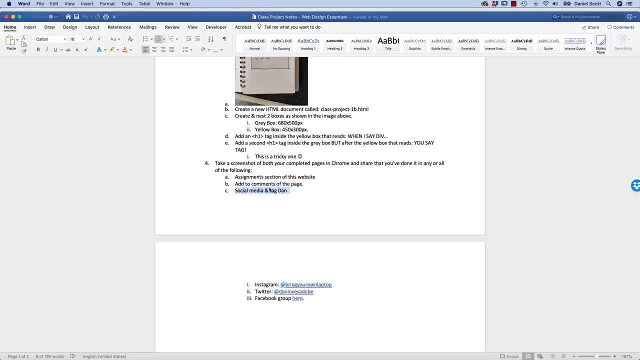 So just stick it in the comments. Also, like this, this or this, or do them all Social media, so stick it on Instagram, tag me. Twitter, tag me. Facebook group here: tag me, Just so I can see that you've done it. 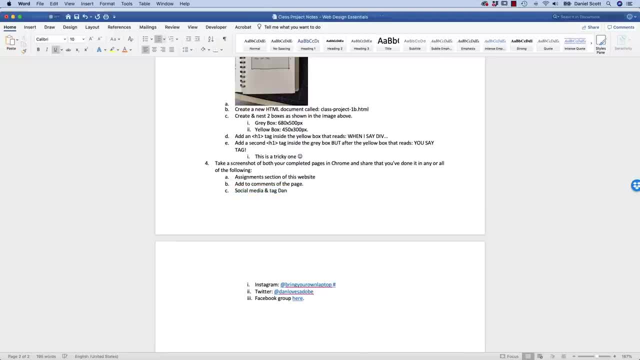 And what you should do on all of these is add a hashtag. I thought about this earlier. add a hashtag when you are So, tag me and add the hashtag BYOweb, Just so that I can group them all together in all of them. 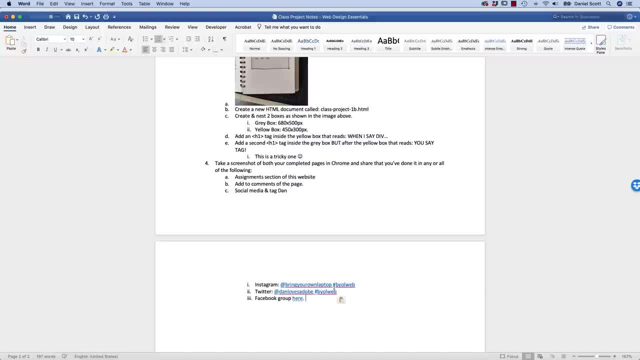 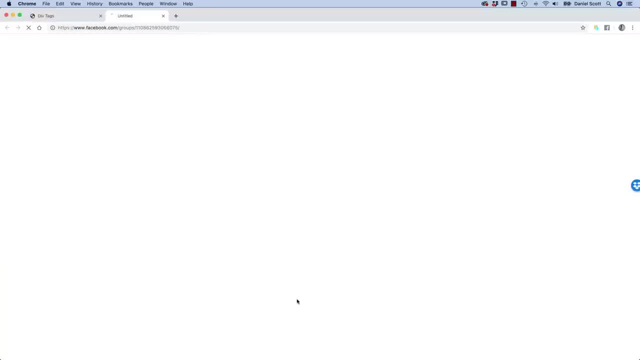 So that when I'm reviewing it I can look at web stuff different from my other courses. So Instagram, Twitter are good places to post visual stuff, And in Facebook there's a group here It's got a terrible name, so I've added a link. 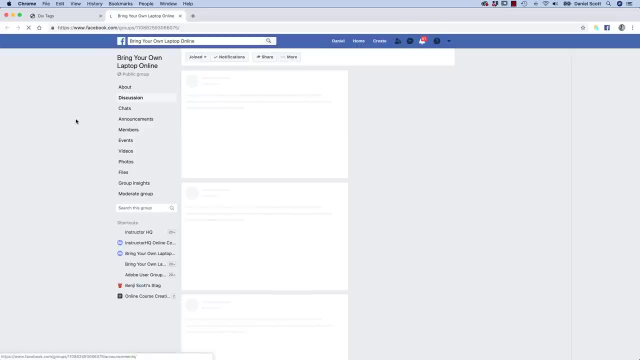 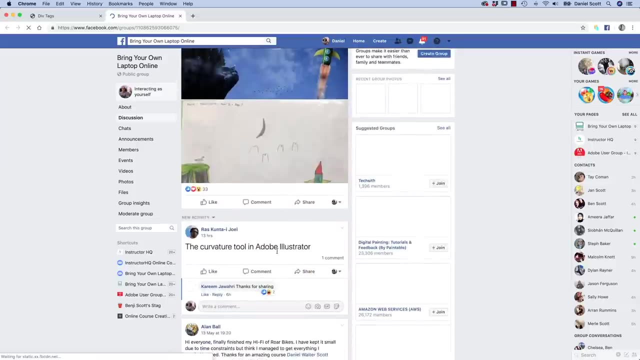 It's called the. what's it called? The Bring Your Own Laptop Online group, And it's a group- hello me- where we share lots of. at the moment there's not a lot of web stuff, a lot of UI stuff, a lot of Illustrator. 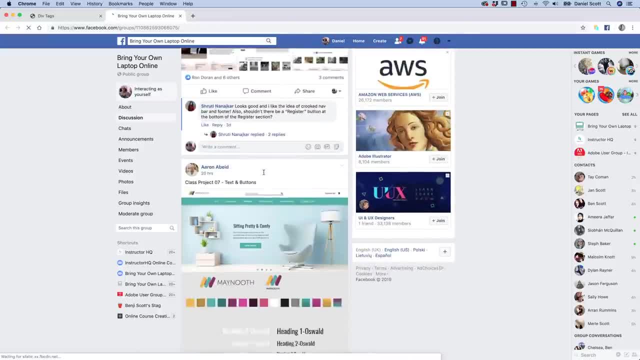 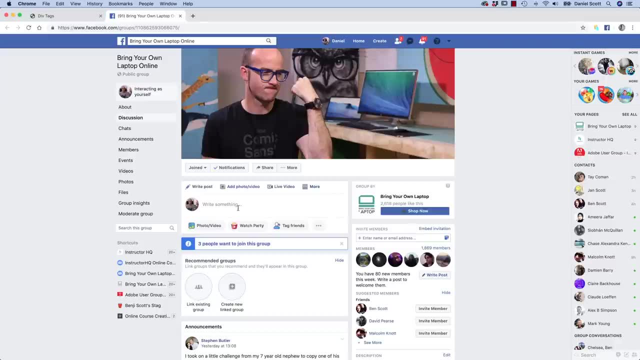 Photoshop, InDesign, a bit of UX UI and now we're going to introduce the web stuff with this course. So post it in here, add that hashtag and say yes, I did it, Or it's broken, and hopefully somebody will jump in and help you. 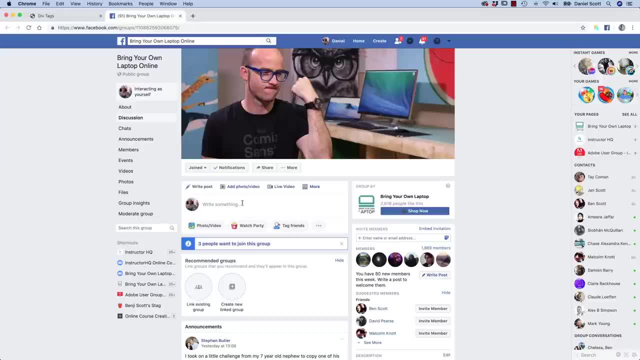 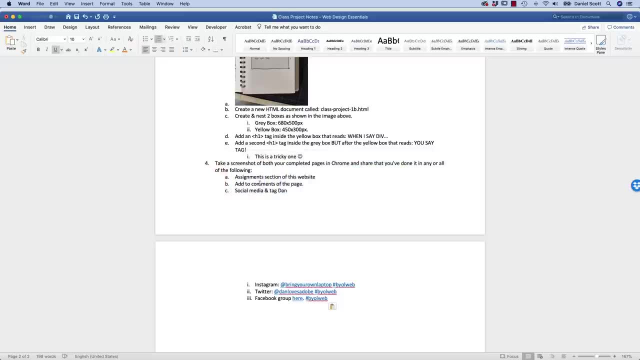 I'll try my best to get it. I'll try my best to get in there as well and help out. That is your homework. don't think of it as homework. Think of it as getting more awesome at web design. Is that it? That's it. 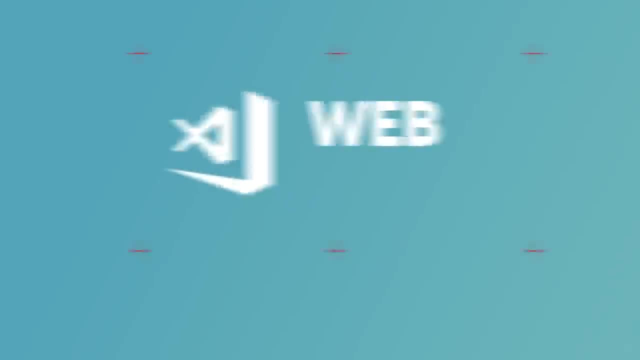 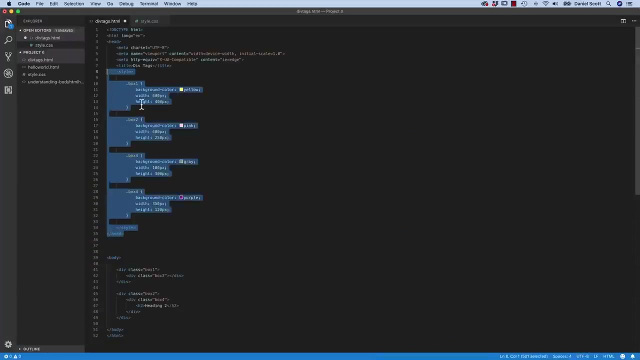 Class project over. I will see you in the next video. Hi there. this video is all about separating our style sheet by taking it all out of the HTML. We'll put it up here in the head and we're going to remove it. 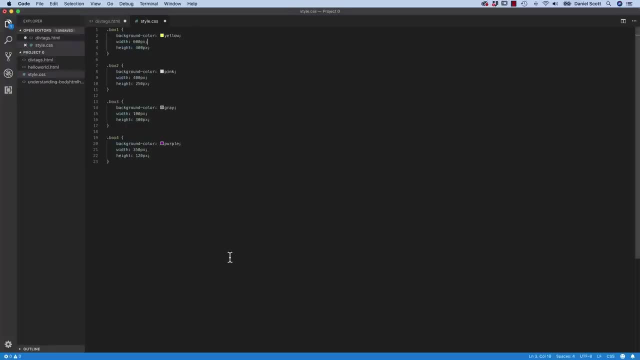 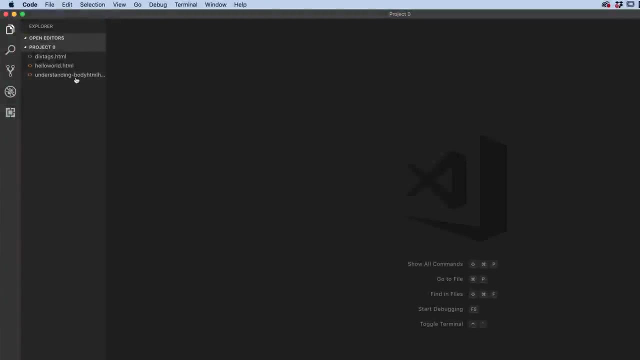 and put it in its own document and connect the two. It's pretty simple. Let's jump in and do it. All right, It's pretty simple to create a separate or external CSS style sheet We're going to work with. 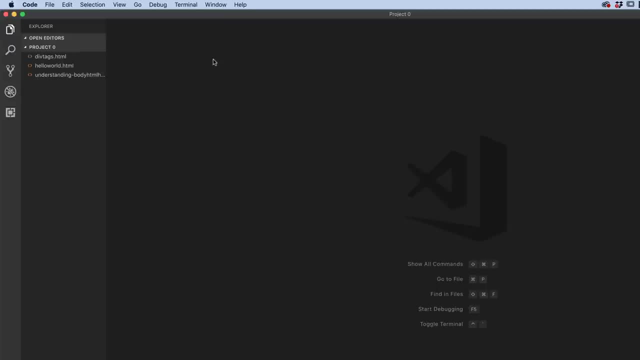 close down anything you've got open from previous part of the course. So it's nice and open or empty. If you can't see this, click on that first little tab here. If you can't see anything in here, go to File Open and find Project 0.. 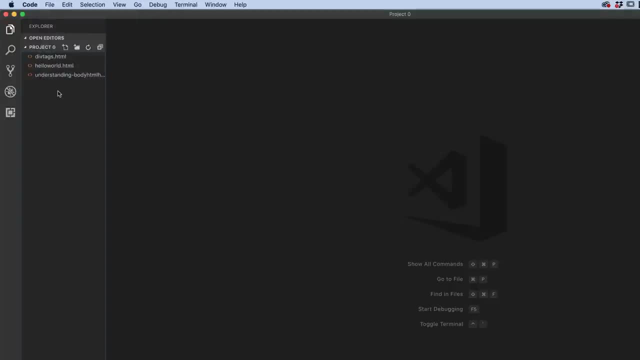 It's a folder that we made and click Open. You should see all the files. So we're going to work on the div tagshtml. It doesn't really matter which one. Okay, So we've got this one here. What we've been doing is we've been half-cheating. 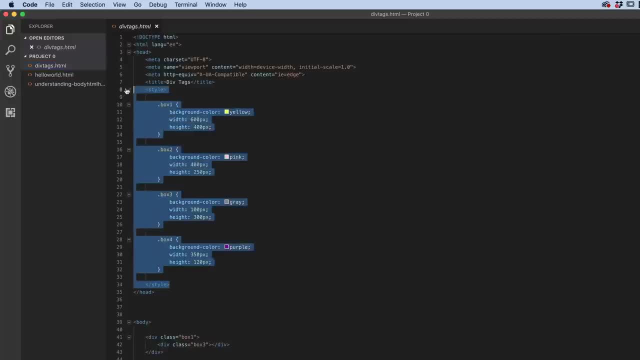 It's not even cheating. We've got the style, all the CSS, in the header of the HTML And that works. there's nothing wrong with it, except it's a bit painful. if we have 20 pages, Say we have 2000 pages. 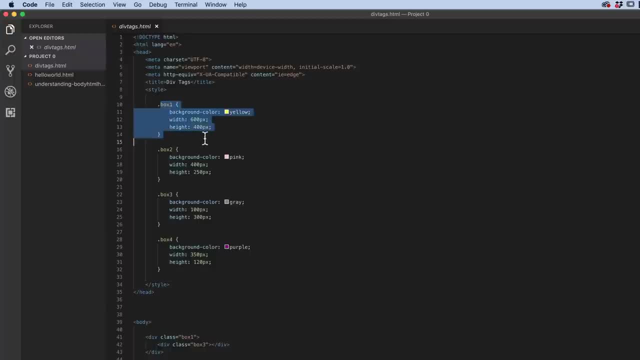 Each page has a Box 1. We'd have to write Box 1 on all of our separate 2000 pages And if we wanted to change it, you just wouldn't. If the client comes back and said can you make it readier? 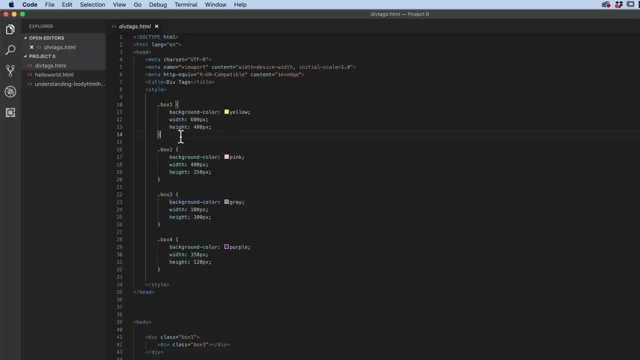 You're like: no, I've got 2000 pages that I need to open and go and change. So what we want to do is put it in a separate sheet and our 2000 pages can reference that one CSS sheet. 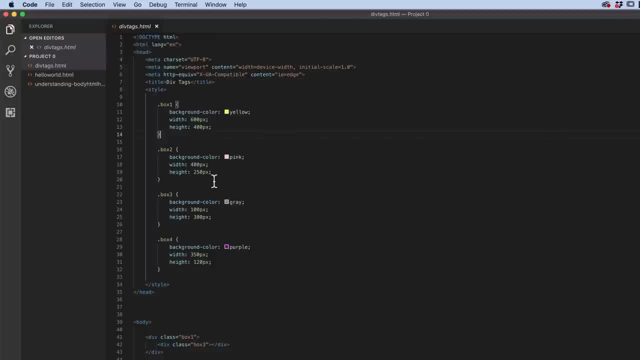 So we can change it once on the CSS sheet and the HTML. all go looking for that one sheet and we'll update all nicely in one go. It's hard to explain, let's just actually do it. So, first of all, what we need is our CSS document. 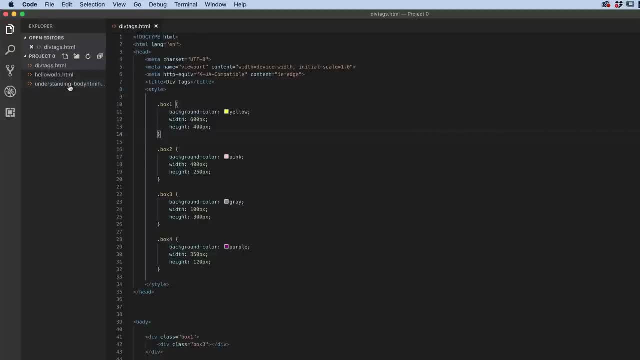 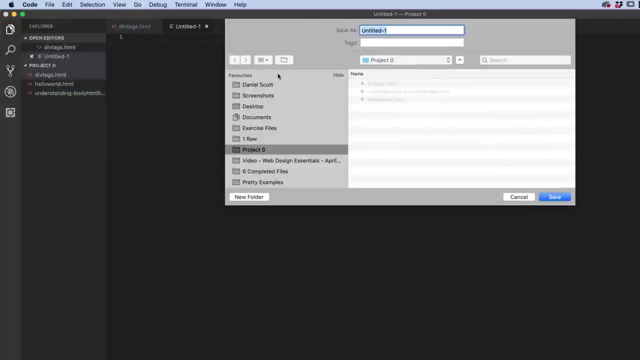 So let's go to File, let's go to Save. No, not Save. Let's go to File, go to New File, Let's save it now. The difference here is: we can call it anything we like, as long as there's no spaces. 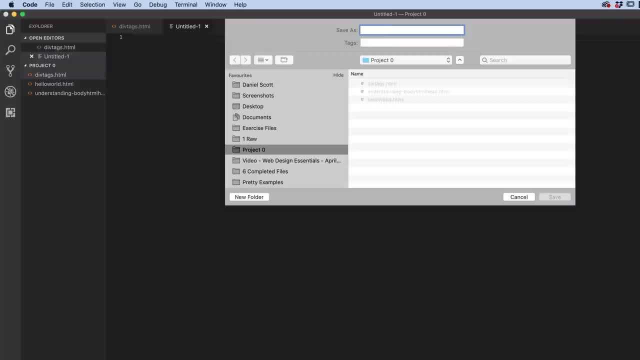 So we're going to call our style, but we could call a style styles plural, and what else does it get called? What else? I'm just trying to think of other generic names. You can call it anything, I can't think of any of them. 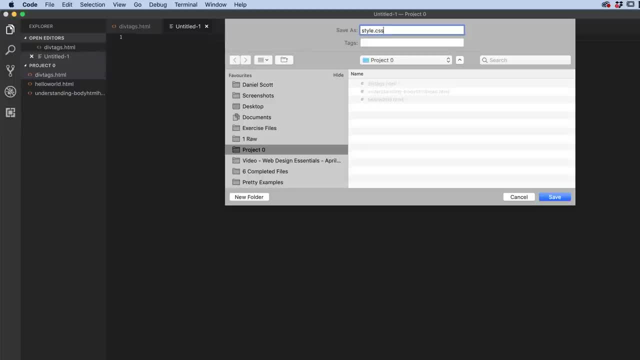 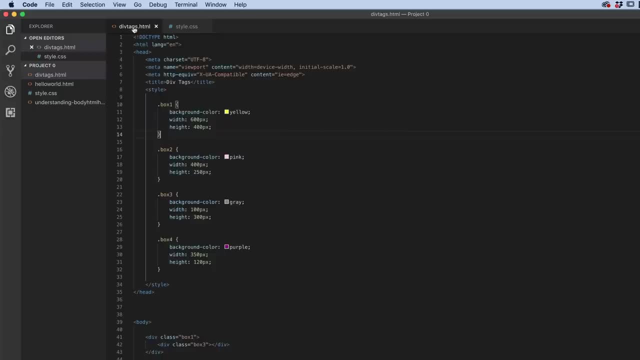 We'll call it style Style and it's going to be css. Let's click Save. Basically, what we want to do is copy and paste the style from this document to this document. So we've got two tabs open. So, from this document, what do we need? 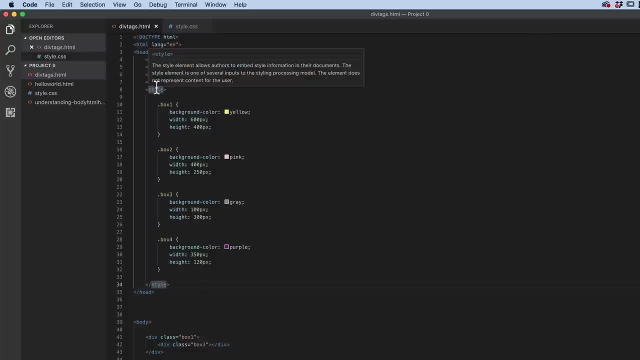 We don't need this style tag. This style tag is in here just to tell the browser: hey, this is not HTML Inside the style tag. everything in here is CSS, So let's grab everything. And when you're copying and pasting stuff, 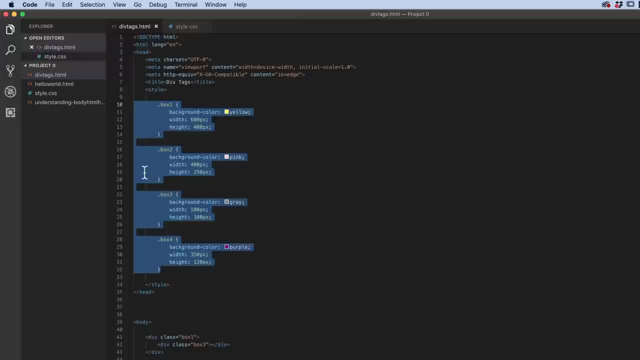 happens to me all the time. as always, forget the closing brackets. Make sure you grab all of them and let's go to Edit, We'll go to Cut and we don't need the style tag now. It was just there to tell it was CSS. 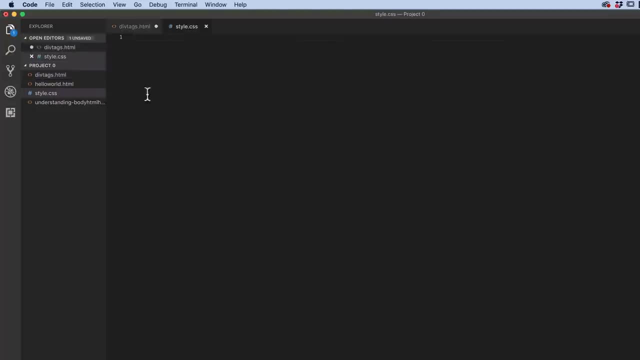 It's a lot cleaner. first of all, And here in stylecss, just go to Edit Paste. That's all you need to do in a style sheet. Is you just like we've learned before? it's just in a separate sheet. 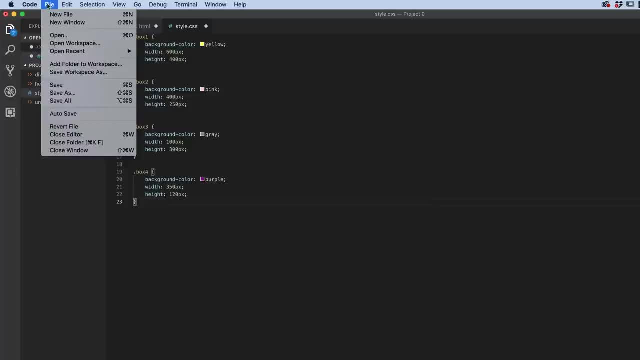 Now it's not going to work, let's test it. We're going to learn a new function as well: File Save All. Why that's useful is that because we'll be doing changes to the HTML and the CSS And they're separate documents, right. 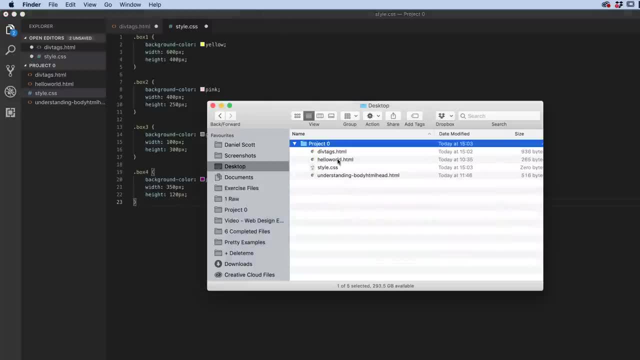 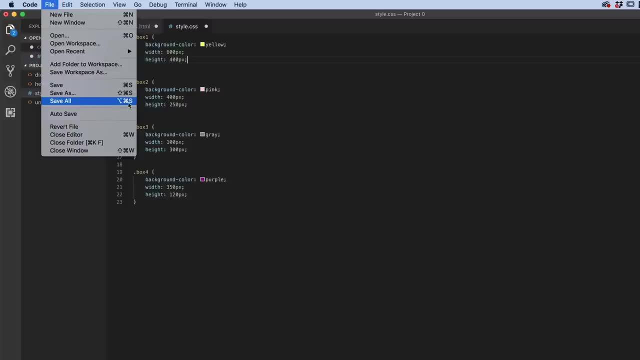 Let's have a look on my Desktop in Project Zero There's DivTags and there's stylecss. These two guys are separate so it's easier just to go Save All. I learned the shortcut on my Mac. it's Command Shift 3.. 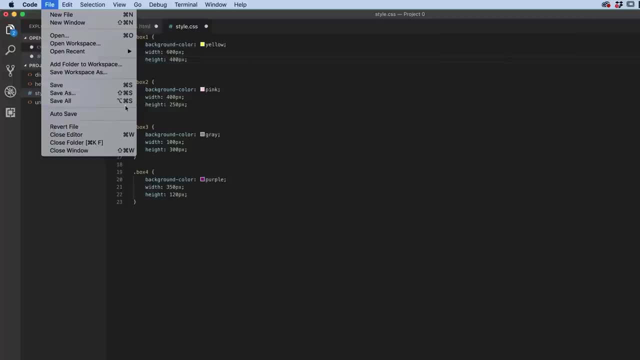 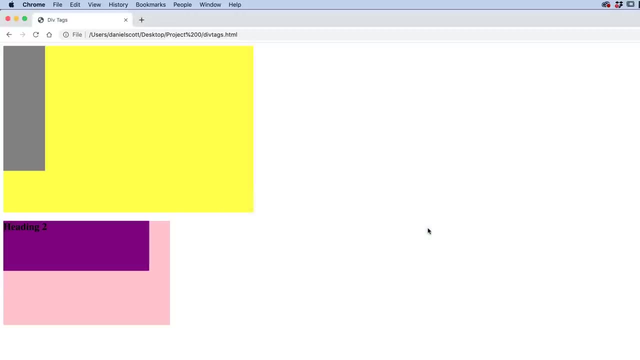 What is it on a PC? If you're looking at a PC, go to File. it should have it right there. I'm guessing it's Ctrl Alt S, So let's save it all and let's check it in a browser. 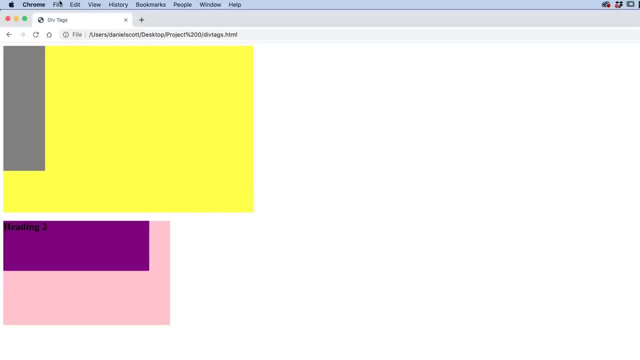 So back in here, Enter Chrome. I've already got DivTags open. You might have to go to File and where is it Open File? I'm going to refresh it and it's going to go all bad. So we've moved all the styling. they're there. 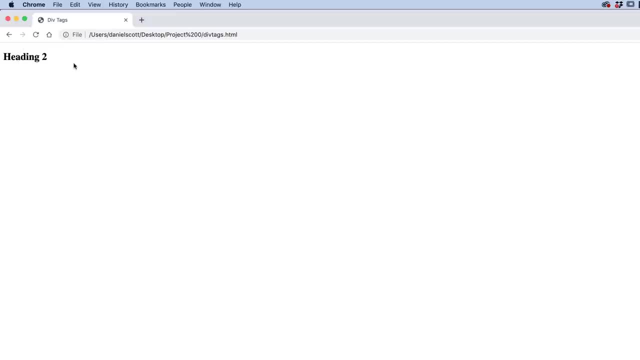 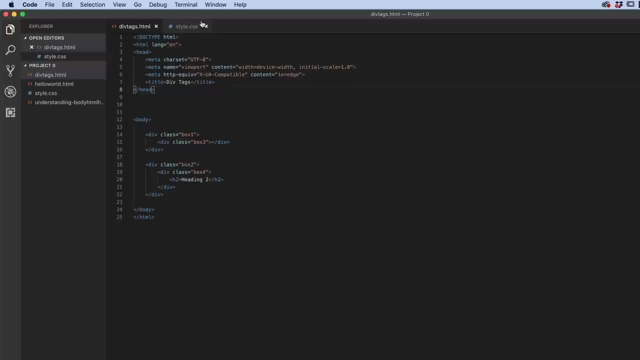 The DivTags are there, but they're all collapsed because we've got no height for them anymore. So what we need to do, the second part is we've copied all of it from there to there, but this HTML document doesn't know this guy exists yet. 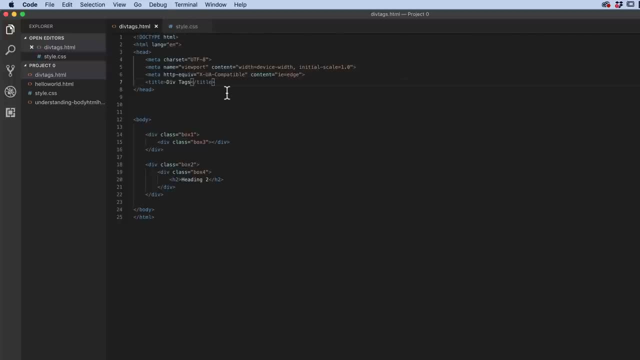 It doesn't automatically go and find it, so we need to tell it. So let's do that. so underneath the title, let's push Return. Now the long way is bracket link and we're going to have it. relative to the style sheet. 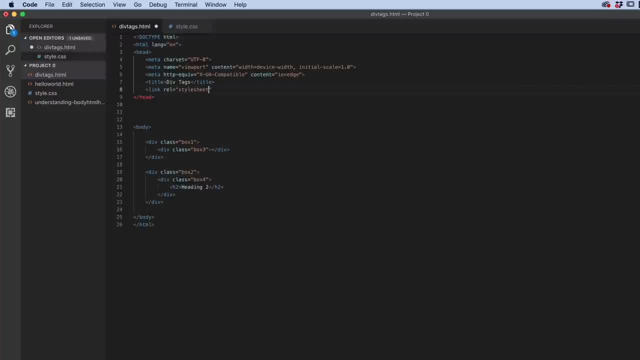 Style sheet. you can tell I never type this in And you've got to do or you got to reference it and you type in the style. So what do we call ours? We call ours Styles- plural, I can't remember. 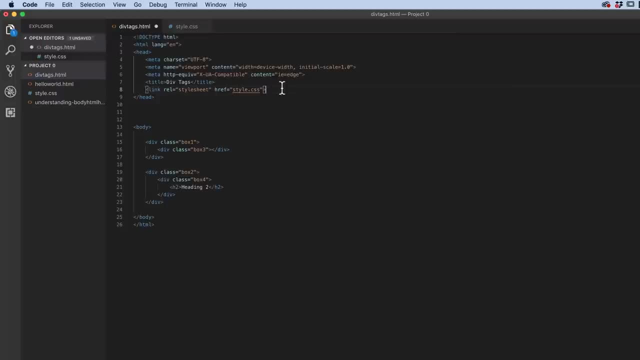 You got to make sure it closes off and you're like man, I'm not going to remember that And you don't have to, so the long way is the bad way. Let's close it and we'll use VS Code to help us out. 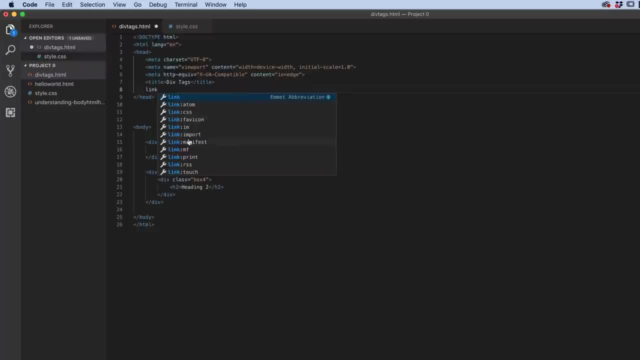 So we can type Link and then just kind of scroll down here and click on this one, because you can link different things. You can link to a favorite icon, you can link to JavaScript, we're linking to CSS and it puts in all that stuff for us. 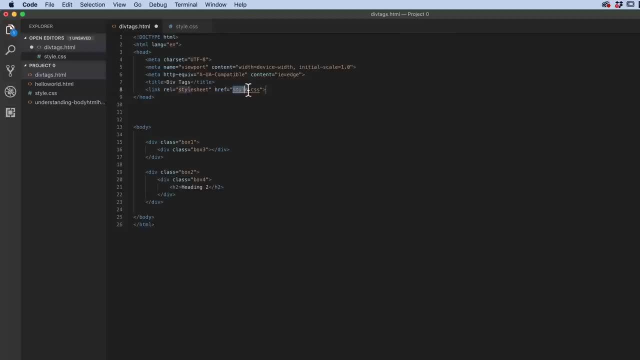 It even puts the name in there. so that is not. that did not automatically go and figure out what I called it. that's just the default thing in there. So if you've called your Styles, you're going to have to go through. 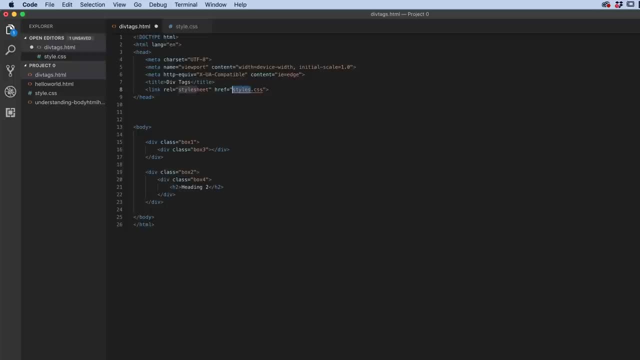 and add the S there If you called it. I can't think of another name, but let's call it. you called it Theme. you'll have to go and change it Because it puts Style in there just automatically. So it's probably a good habit just to call it Style. 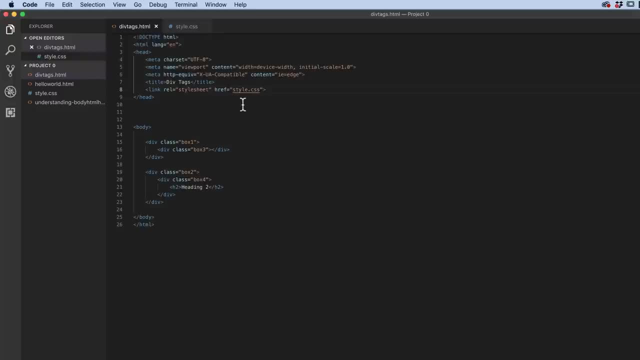 Let's hit save. let's do save all Shortcut time. let's check it in the browser. now, There we go, refresh, it all works. You're like that's a lot of work, why don't we just leave it? 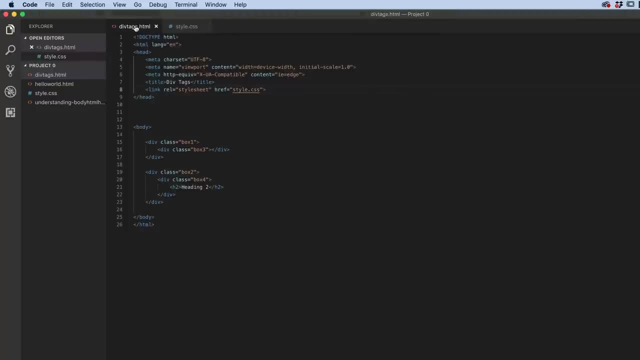 You can tell, the main reason is that all the HTML documents now that I create will link to this one Style Sheet And when I make a change in here it'll flow through an entire ginormous website easily, because they all look for that file. 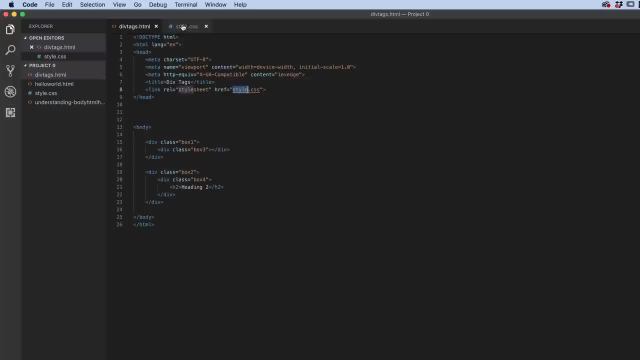 It also keeps it nice and clean, so we can keep our HTML separate from our CSS, And it means that this is kind of nice and tidy. and then this is nice and tidy. You can see how CSS without all the HTML is a really clean looking language. love it. 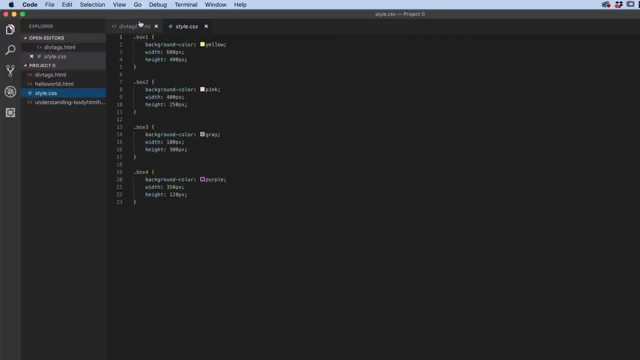 Before we move on, I just want to show you- close that down- And a couple of little things to do with CSS in a Style Sheet. If you hover above, let's say so. it's telling me that's an element. If I hover above this one, can you see? it just tells me. 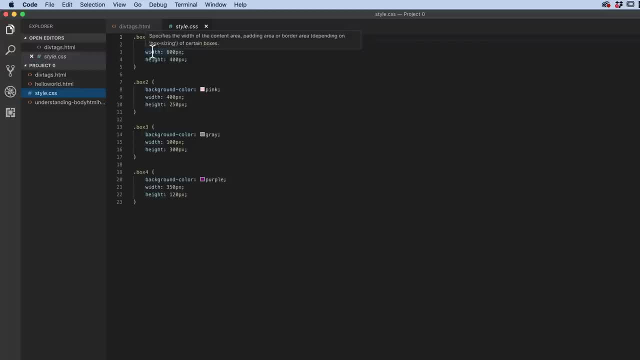 it's the background color of the element. This one here specifies the width, So you can hover above these things if you're unsure what they do. or you open up somebody else's website and you're like: what does that thing do? 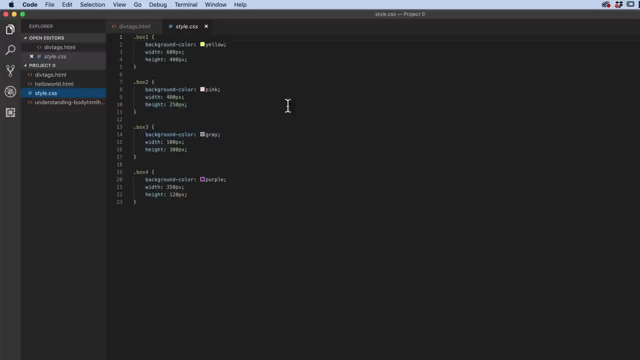 It can give you a brief explanation within VS Code And also something that's built into CSS but not HTML by default is if you have errors, say I delete. with the opening bracket by accident you'll see down here there's like a: hey, you've got an error. 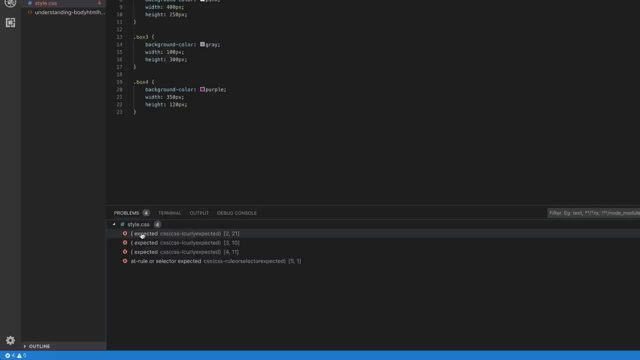 If I click on it it says that in your CSS sheet there's an unexpected error. The problem is that that's not that helpful. I've never found these errors to actually be helpful. I can kind of decode it because I broke it. 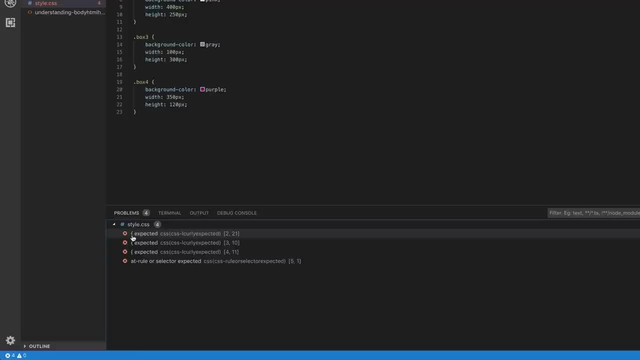 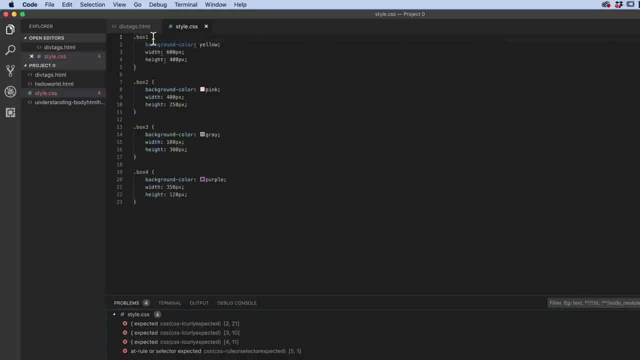 So it says it's expecting a curly brace at the beginning. there And you can see there's lots of errors. there's four of them. You're like there's only one. It's because there's like this trickle of errors So that one breaks, so it can't understand the rest of it. 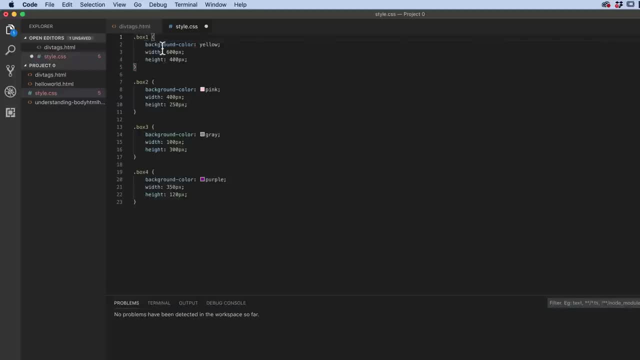 But if I put it back in, go to Brace, don't need the second one, All the problems gone. We don't have that functionality built in to VS Code for HTML at the moment. If earlier on you were like, hey, it didn't go red like yours did, 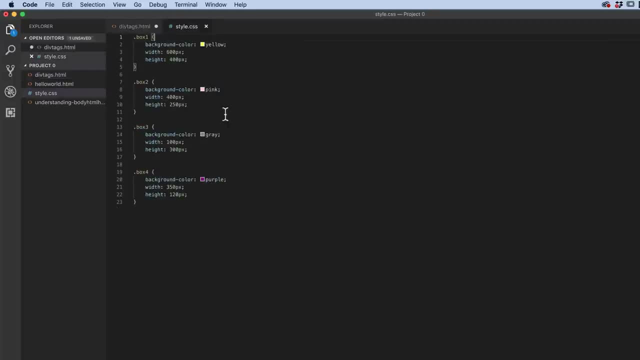 it's an option that we're going to add a little bit later on when we start looking at extensions, But we need to do that a little bit later in the course. Now, if you do see errors, it's probably your brackets, your colon or your semicolon. 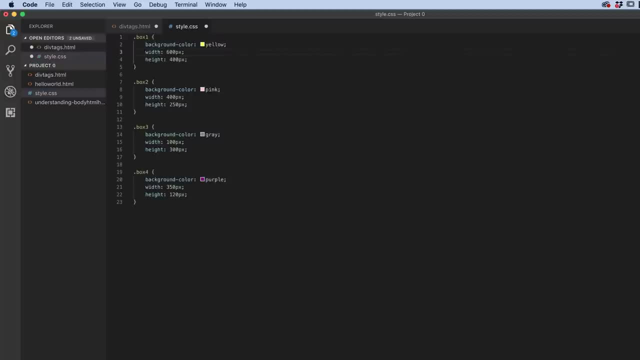 They're missing. Do that. it breaks it. Put it in, unbreak it. So I get a lot of students kind of like: hey, mine's not working in classes and in videos And it's normally always just a syntax error, normally. 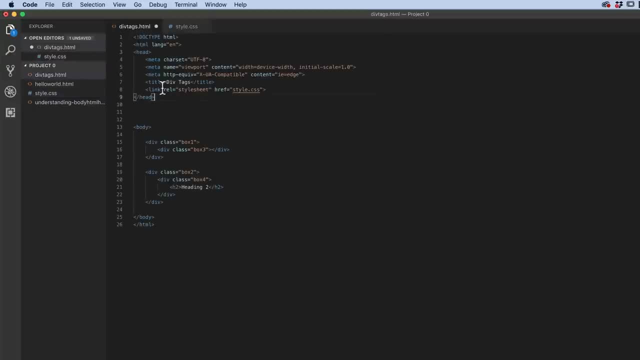 The other thing people always forget to do is that they forget to connect it in their HTML. They make it and they separate it all out, and then they forget to come back, double back and connect it up And they'll use. it'll be just something like this: 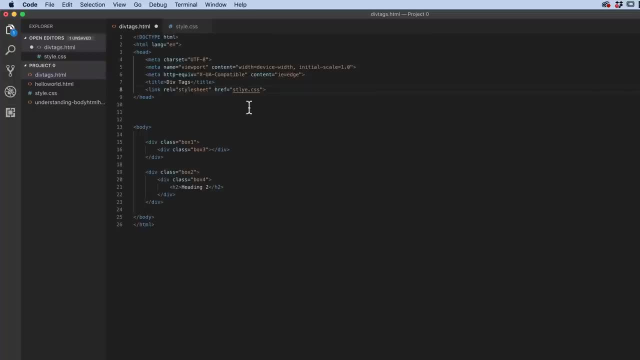 There's people, loads of people like me who are like it's not working And I can see very clearly it's a spelling mistake. So maybe some copying and pasting just to make sure the syntax is all spelt right. 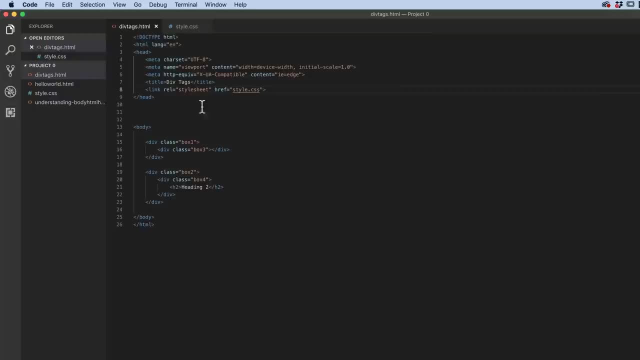 Now I'm going to set a little project now. It's not going to be a separate class project, because there's no point sending it to me, because it's going to look exactly the same. So what I'd like you to do is: 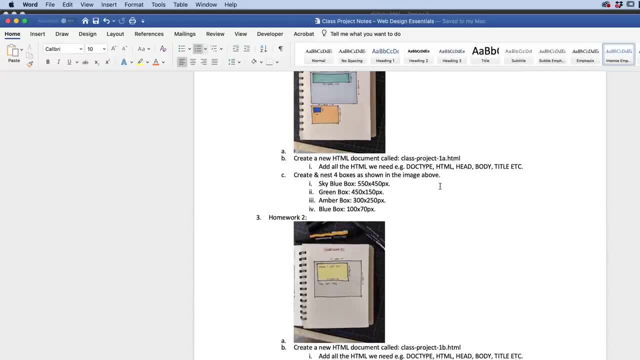 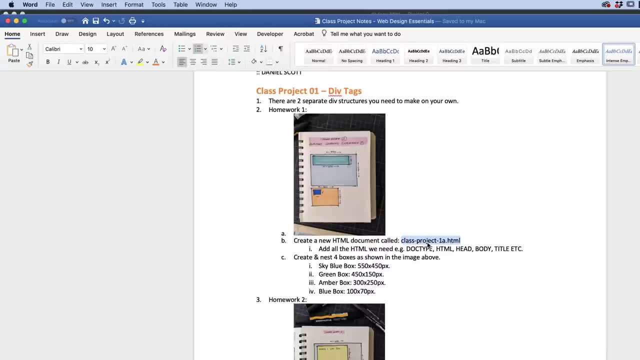 you created two documents in the previous tutorial, previous homework. If you didn't do it, go back and do them. But you've got these two HTML documents. I'd like you to separate them out and have separate style sheets for both of these. 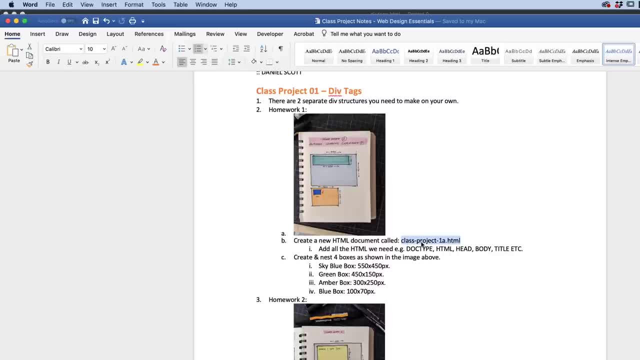 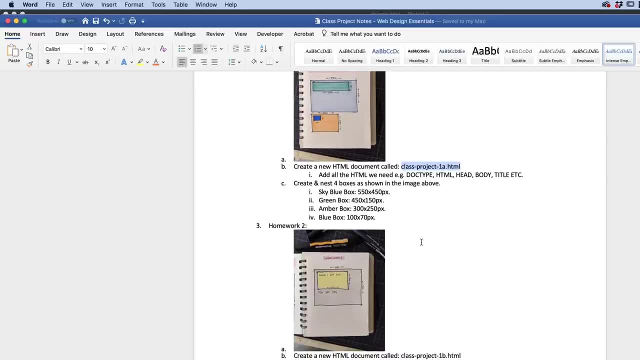 Now, when you are separating them out, one can be called styles, but because they're going into the same folder, you can't have two of them called styles. So I have two separate style sheets, just to go through the motions of copying it out. 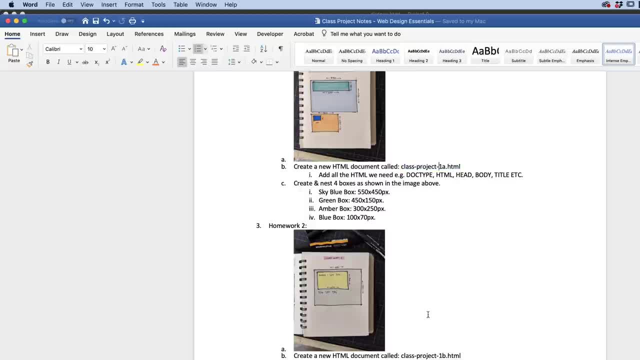 and making sure you get it right. So maybe call this one style1.css and call this one style2.css and see if you can make it work. That is it for separate style sheets. I will see you in the next video. 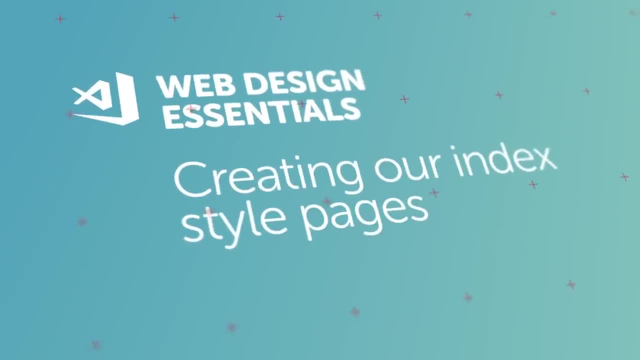 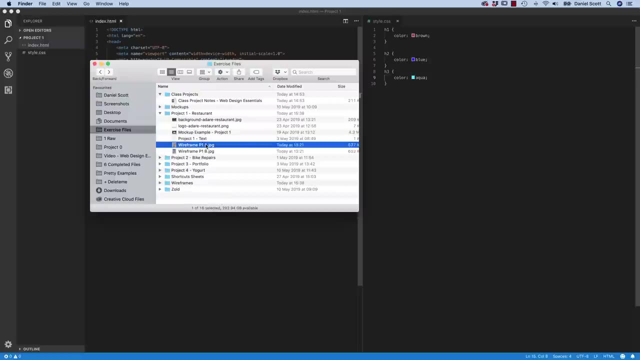 We're on to project number one, So project zero is finished. That was our getting used to things and just learning the basics. Now we're going to actually start making some stuff, So we're going to build a structure. That's our project. one structure. 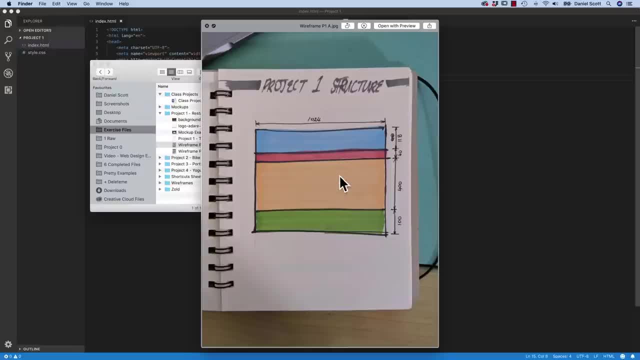 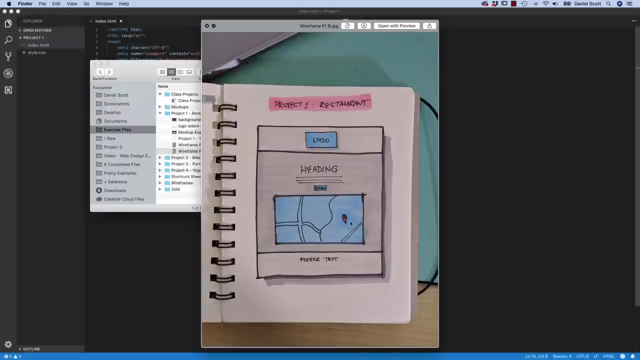 I've written it at the top there. We're going to make some basic kind of div tag structure to it. Then we'll add some details to it. These are my wire frames. We'll add a logo and some headings and some buttons and some maps and cool stuff. 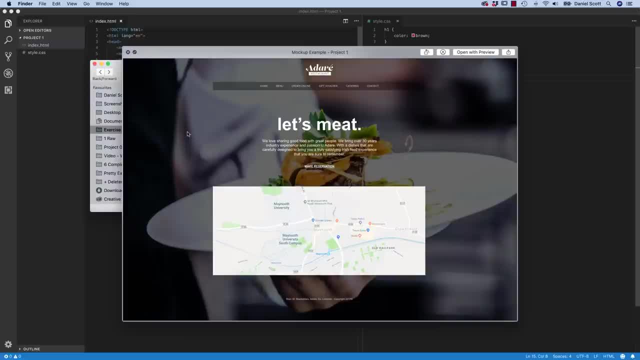 Eventually, hopefully, it'll look like this. This will be our final kind of looking thing. I know exactly it'll look exactly like that because I've already made it. But first of all in this video we need to work out how to create an indexhtml page. 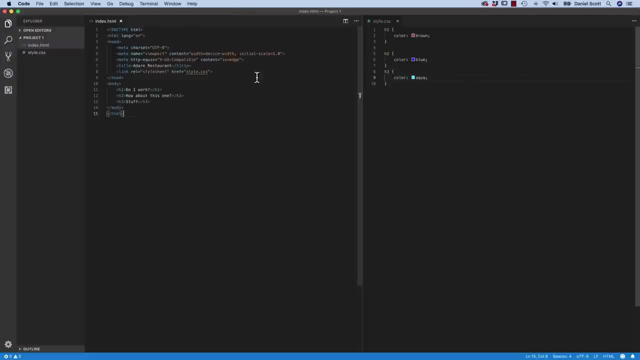 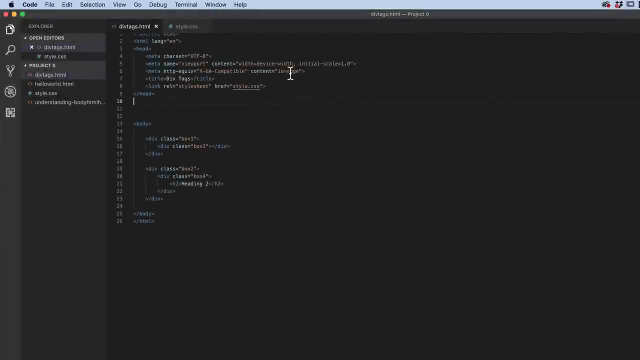 and how to connect our CSS together. We'll also show you how to kind of separate the documents like this: side by side. All right, you ready Project one about to begin. Okay, so it's time for our new site. 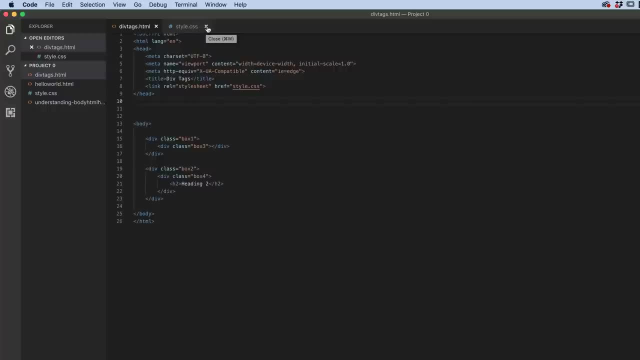 So let's clean things up and get our new site started. So let's close down everything in VS Code. it's got nothing open And we've been working in a folder called project zero. We're up to project one. Zero was like a throwaway. 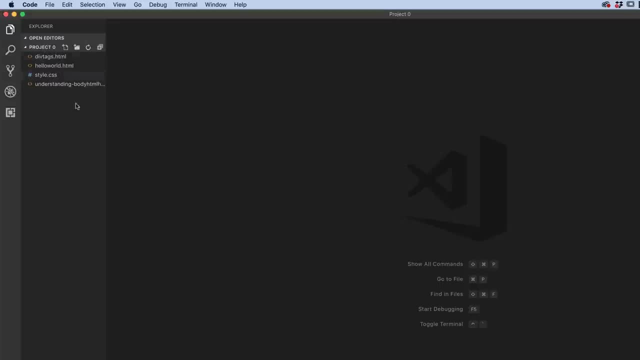 project. so those are things that we just use to test understand what a few of the basic things we've had to learn so far. So what we need to do is create a new local folder. So we call it the local folder because it's on your computer, not on the Internet. 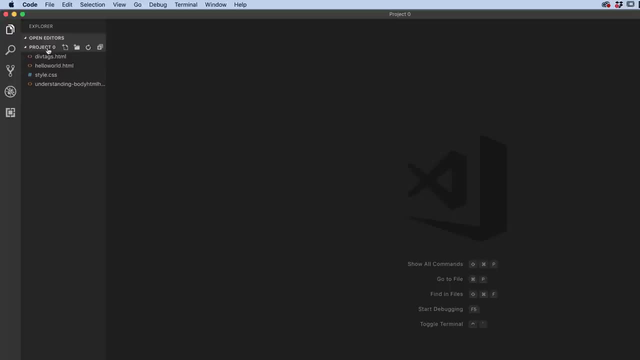 So it's local- local to you at least- So we need to create a new folder and create our HTML And CSS, give them names and link them together. So, first up, let's go to File and we're going to create a new folder. 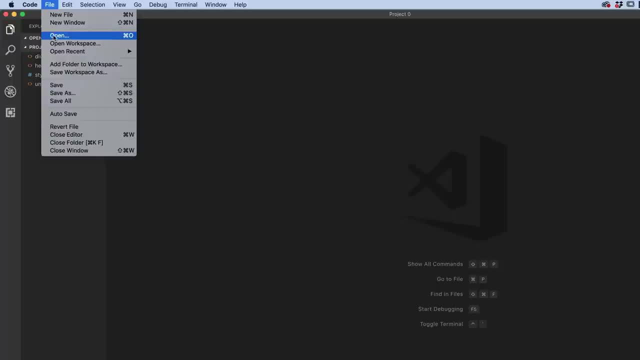 Now, it doesn't matter if you find it a little bit difficult to go, because we're going to open a folder and then create a new folder. It's kind of weird. you can do it through your operating system. So if you're on Windows it's different, but on a Mac it's in Finder. 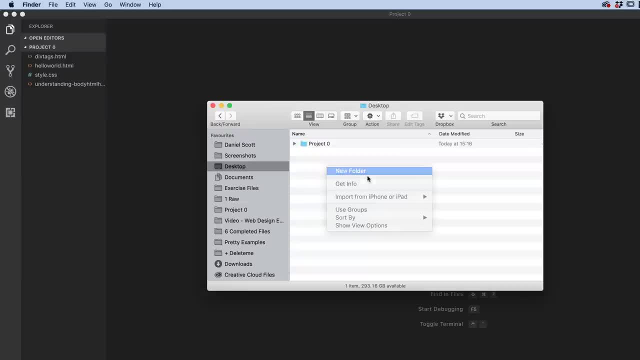 Go to your Desktop and in here I can right click and say New Folder. It doesn't really matter how you get this new folder, but we need a project one. If you're on a PC, it's very similar. Open up your My Documents, find your Desktop. 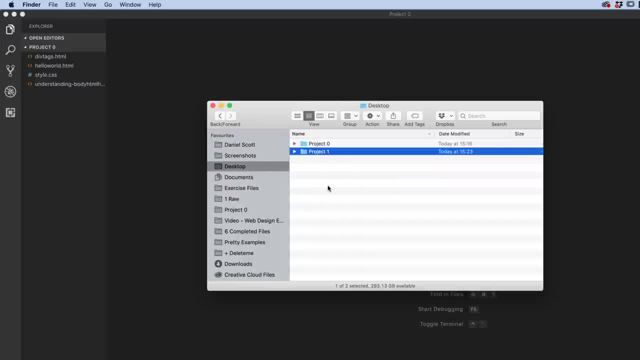 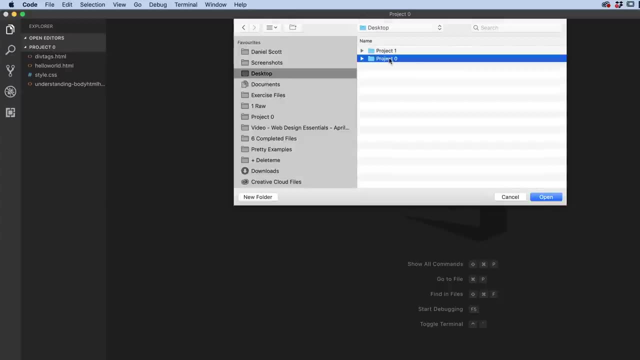 and right click make a new folder. So either way, we want to have a new folder. I'm going to open it. On my Desktop there's my new folder, Project 1. Click Open. Nothing really happens, it just kind of flashes. 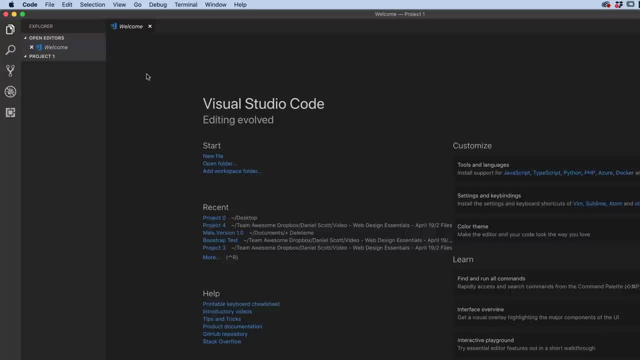 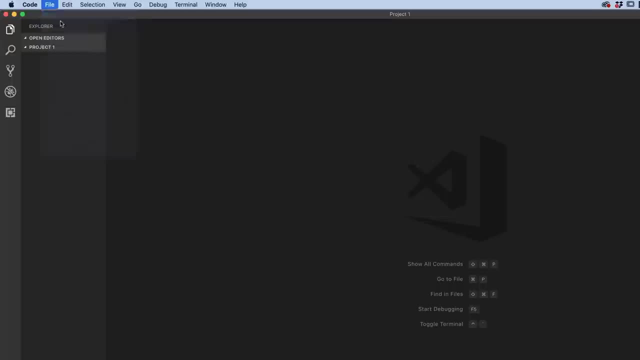 and you get the welcome screen back again. I remember when I first started using VS Code and I was like, oh man, it's confusing, so get rid of that. Let's make a new document File, New File. We're going to create two of them. 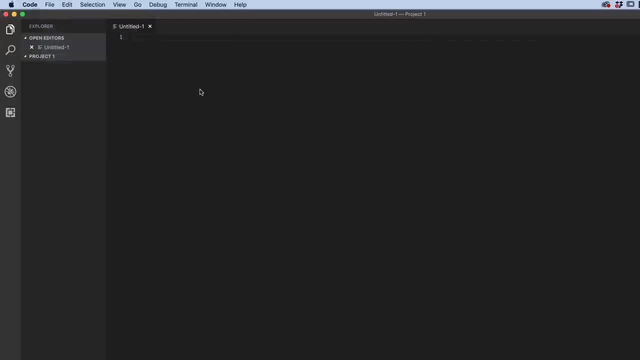 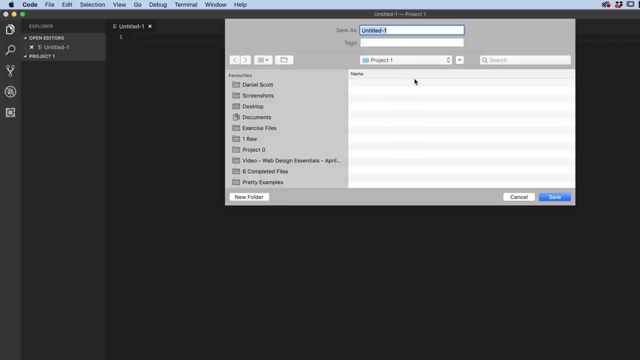 We'll create our HTML. so File, Save Now this HTML document. we've given it random names so far, like divtagshtml or hello-worldhtml. Now, for a website, you need at least one page, or at least one page. 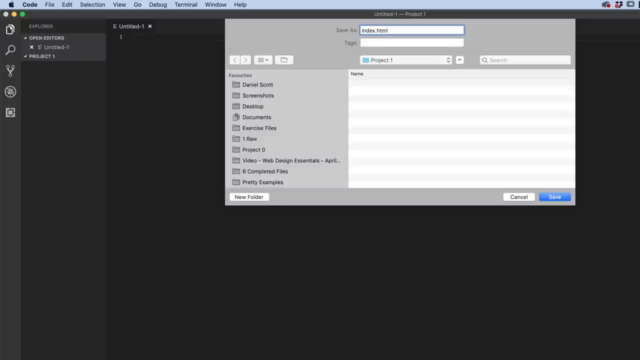 You need your home page to be called this exact thing, So it needs to be called indexhtml. If you called it homepagehtml, put it up on the Internet and the browser would go to your site, dansawesomewebsitecom. 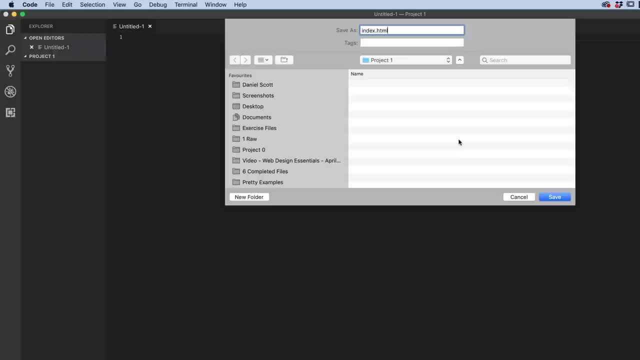 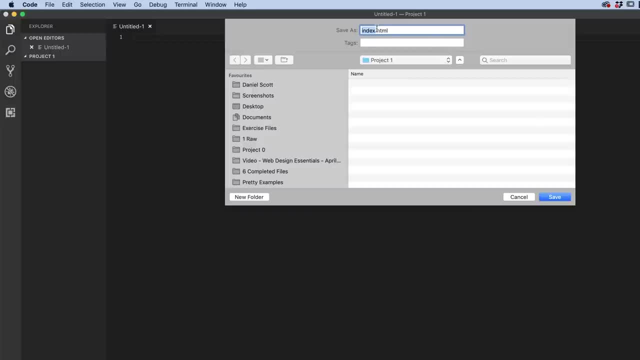 So you need at least one page called indexhtml. Use lower case rather than uppercase, No spaces has to be exactly that, And the browser goes and looks for this page as its initial first page. So call it index, click it, save it. 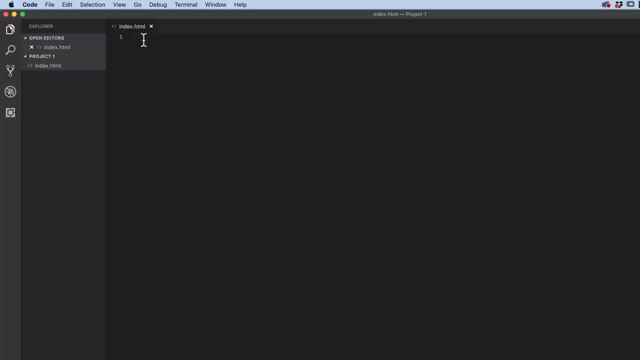 Let's add some basic HTML, all of our metadata, So remember exclamation mark return. Let's give it a title. This one here is called the Adair Restaurant Restaurant. I can't spell restaurant. is that close? There's no spell check in here. 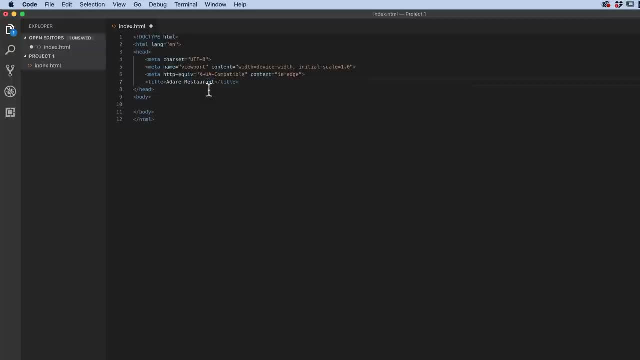 And I'm cheating as well. I'm looking at my notes. like I've written it in there- I don't even know if that's spelled right anyway. So Adair Restaurant is going to be my title and we need to create and connect a CSS sheet. 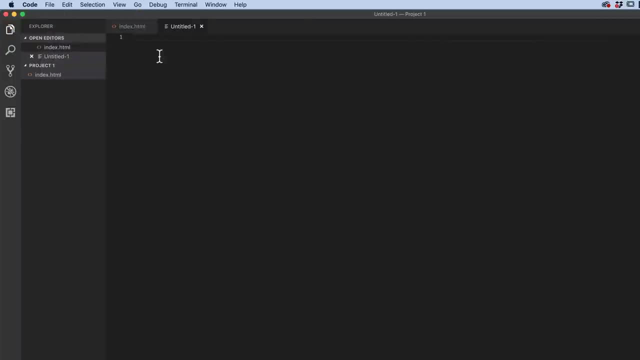 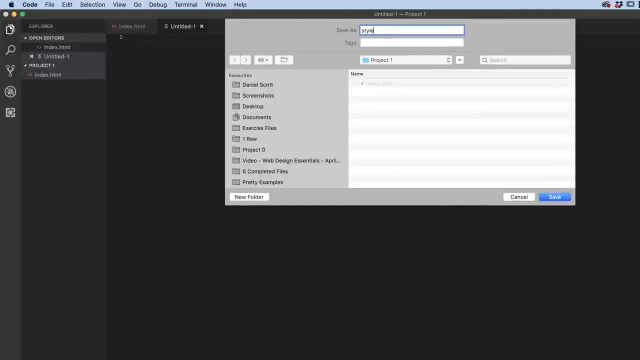 So let's do that by going to File New And let's go to File Save. We can give it any name we like. I was thinking about it before in between videos I was like there was style, what is? 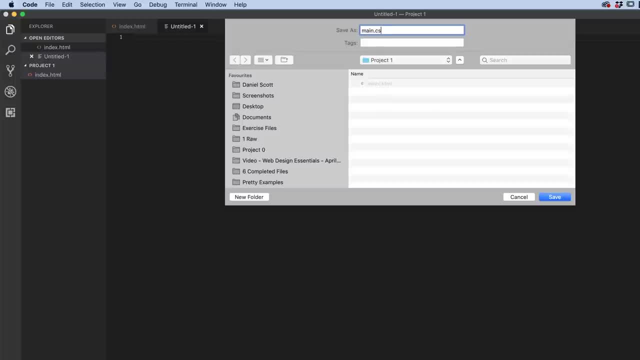 I used to call it main, all the time maincss. It doesn't matter what you call it. The only problem is if you call it style and you're a web developer or designer and you're making loads of websites, you're going to have lots of files on your desktop called style. 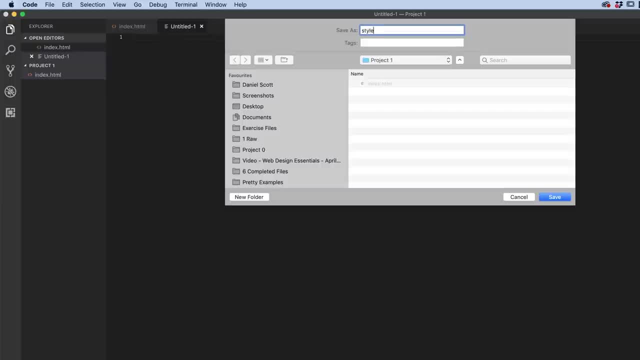 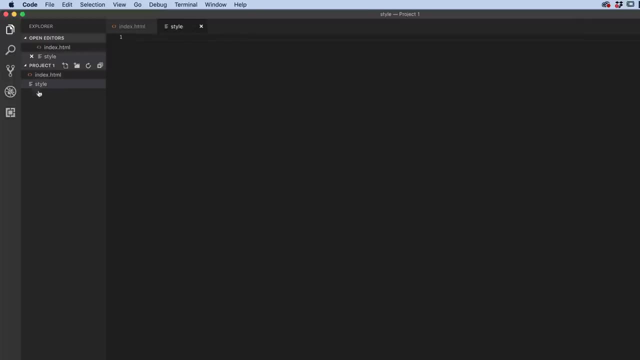 So it makes it a little bit hard to find the one you want, but not that hard. let's just call it style. Remember css. if you forget, like I do all the time, hit style. It doesn't work, but over here you can right click it, rename it. 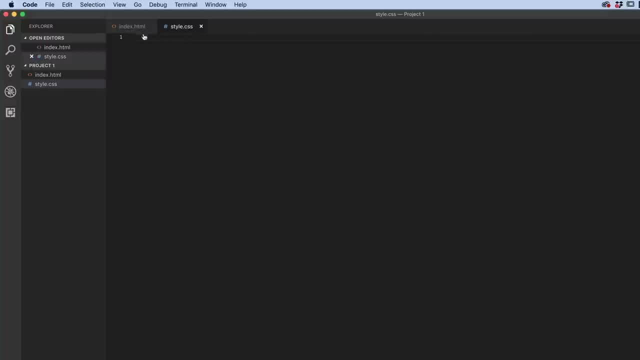 And just put a css afterwards so it knows. Now we're going to connect the two. so back to HTML, And just under here under Title, we're going to put Link And we click on CSS and it gets the right name. 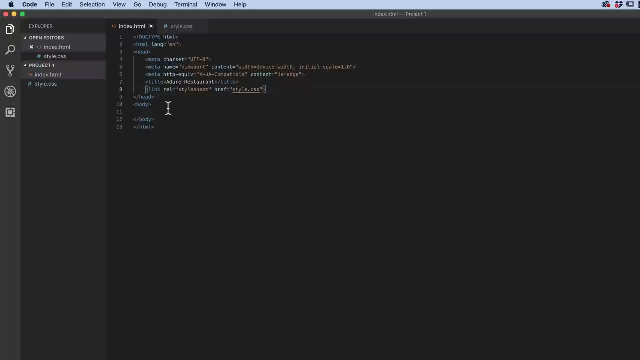 because I gave it the right name. I'm going to hit save and that should work. Let's test. it works. Let's just put in the body here. let's put in an H1.. Now I'm going to show you a slightly different way of working. 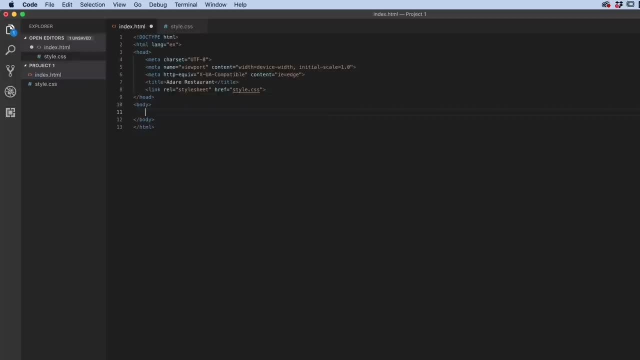 We're going to add shortcuts as we go around. If you're like man, I'm not ready for shortcuts, just type in the long way, angle brackets: H1.. close. it already does a little shortcut there, but I'll show you a shorter shortcut. 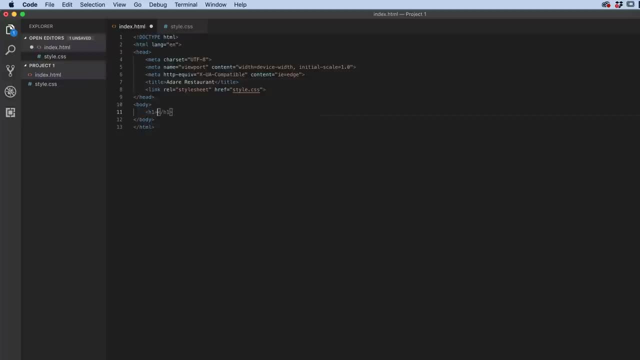 So I'm just going to type H1, and hit return. You can see there I don't even have to put the angle brackets in the front. So I'm going to do that probably for the rest of the course, Only because I do it out of habit and you might be wondering why, but anyway, 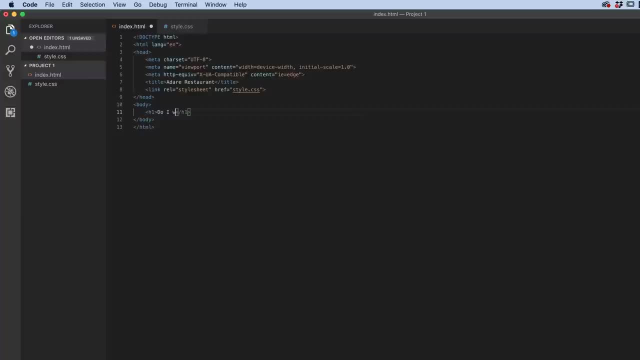 Let's call this one. Do I Work Save? let's go to our Styles. Let's add a style for H1.. H1, curly braces. We'll make it just change the color, is it not columns Color? and we're going to call it. we're going to give this one brown. 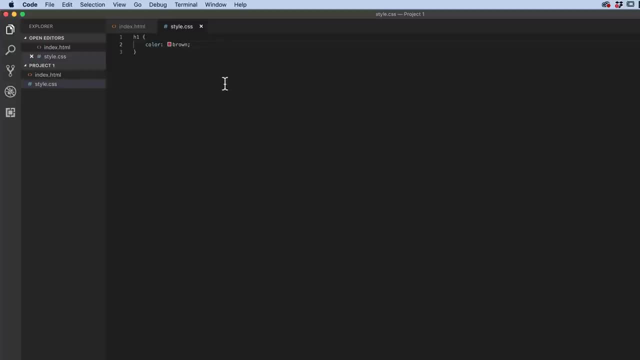 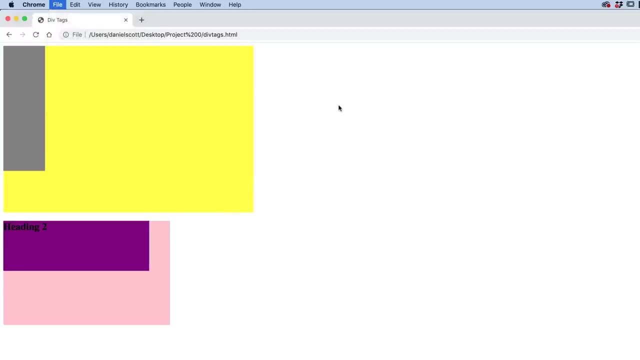 It's got our semi-colon in. we're going to save it and let's go test it in a browser. So that's our old page that we're working on. I'm going to go to Open File. let's go and find it. 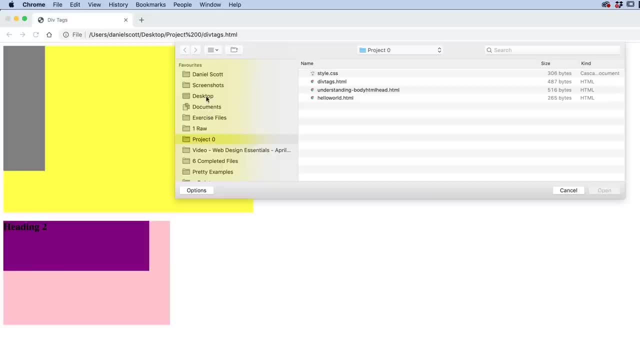 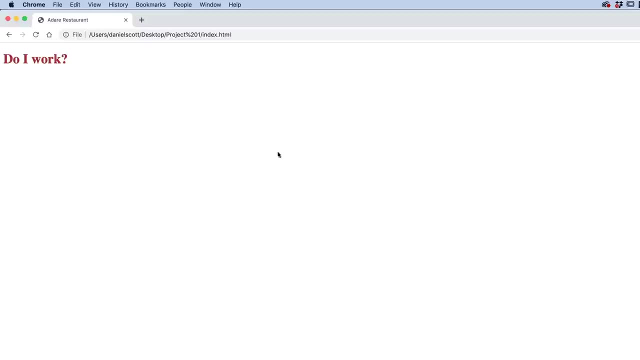 So we're looking not for Project Zero. now Go to my Desktop or your Desktop: Project 1.. And there's my indexhtml. Hey, there's my H1, and he's brown. Now a couple of other things I want to show you in VS Code. 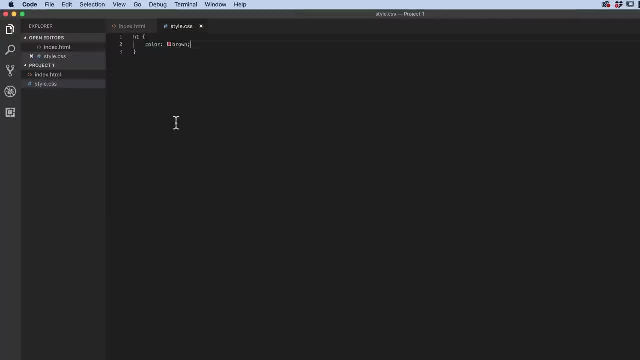 is this thing, the Explorer. It's cool once you've used it for a while, but at the beginning you're like it's a little bit confusing. So there's two sections to it, right? I'm going to have these little chevrons here to kind of tidy it all up. 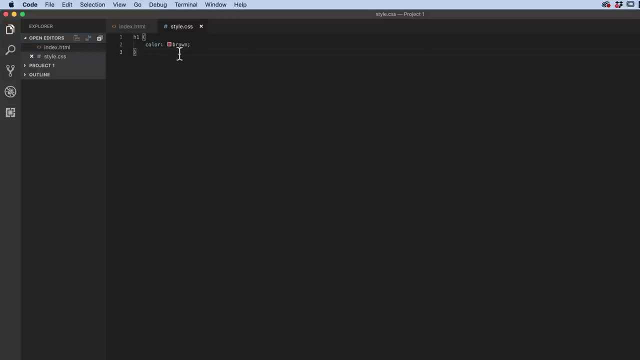 So Open Editors? I never have Open. It just shows me when it means Open Editors, that's an editor, that's an editor. It's showing me that I've got these two documents open. I don't find that useful because I can see there. 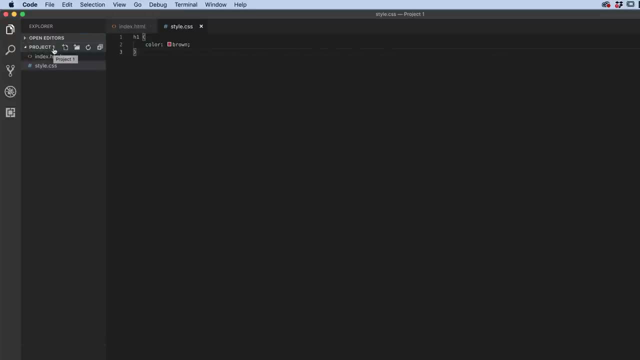 Project, though, is really helpful. That'll be the name of your website, So we've called it Project 1,, but if you're working on this website, you might call it Adair Website, And that will be the name there. And in here there's all the different pages you have. 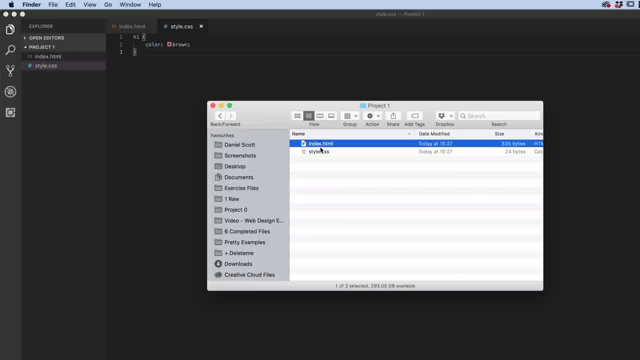 So in here, if you end up in Project 1 creating a bunch of other pages, let's say we call this one, Contact Us. We make a bunch of other pages, let's make one more. I'm just kind of cheating, right. 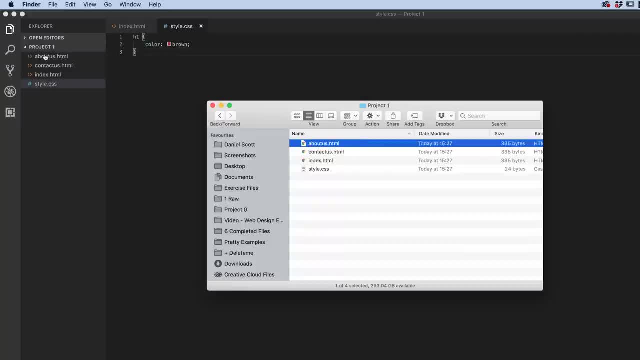 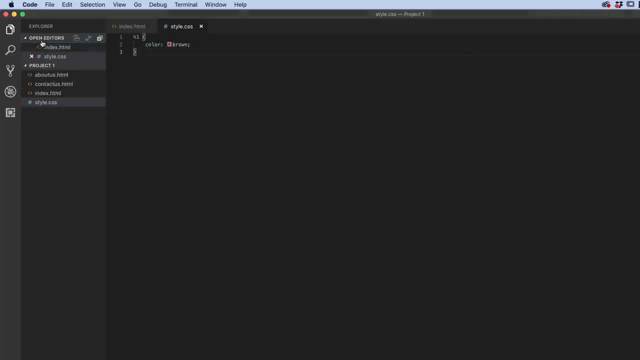 You'll notice that. can you see in here. It's adding it to that project. it's going okay. I've looked in that folder and I'm seeing everything in there And Open Editors is just showing me the two that I have open. 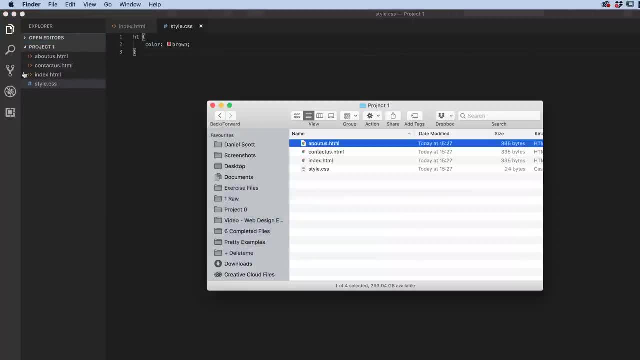 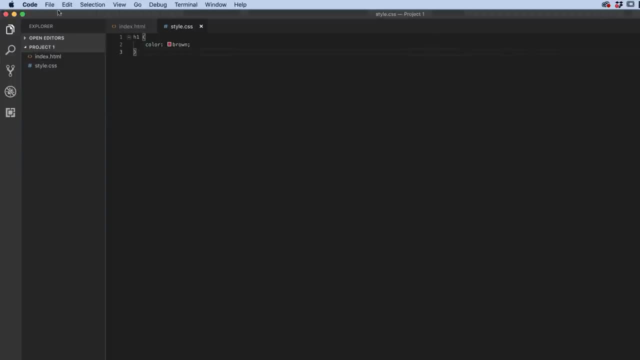 Not sure if that's useful for you. I found it quite difficult getting my head around that weird little explorer there. I'm going to pin these guys. they're not anything, You'll see it updates. So instead of going File Open, you can just double click these. 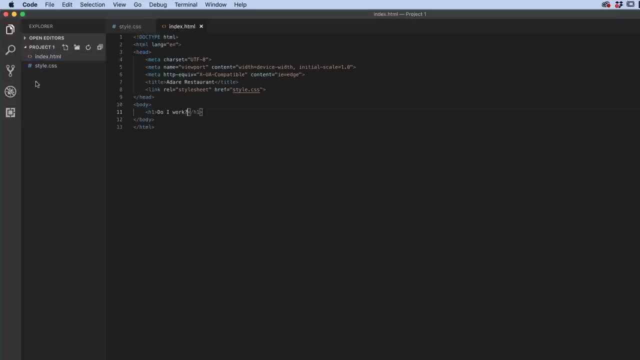 and it will open them up if they're not already open, Look at that. The other thing I want to do is I've got Index and Style and I'm going to toggle between the two, and you spend forever toggling between the two. 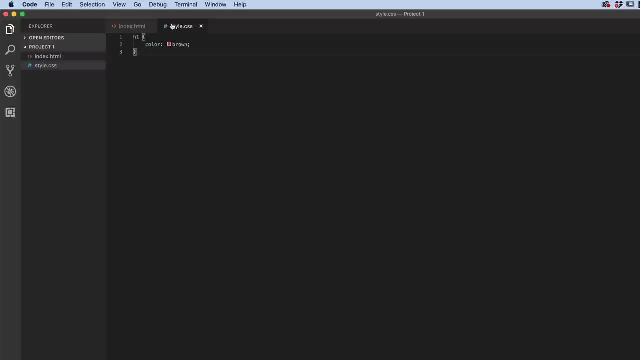 I'm going to show you a little trick- Not too many tricks- earlier on. we're going to get trickier as we go, but this one is just. it's good for teaching and handy for what we're doing. If you click and hold the tab at the top. 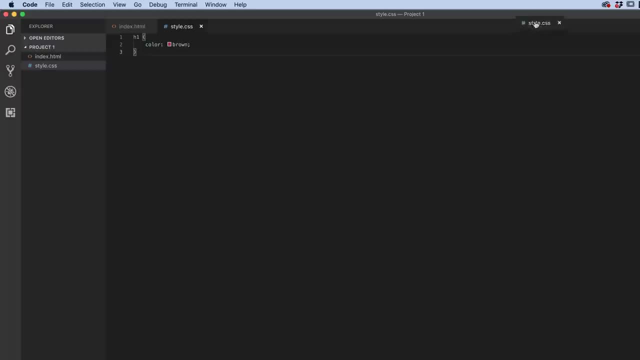 so I'm going to grab the word Style: hold it, hold it, hold it, start dragging it around. You can see these boxes appear. it's a bit weird. You're like: is it that one? is it that one? 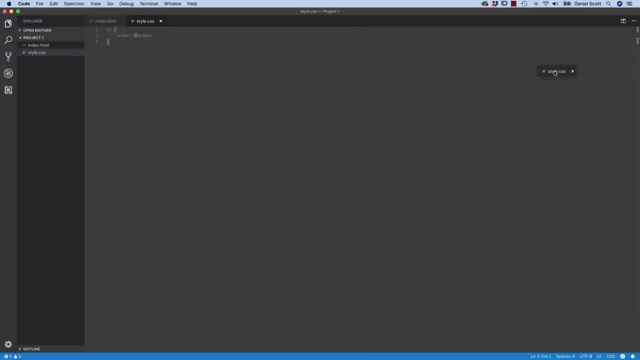 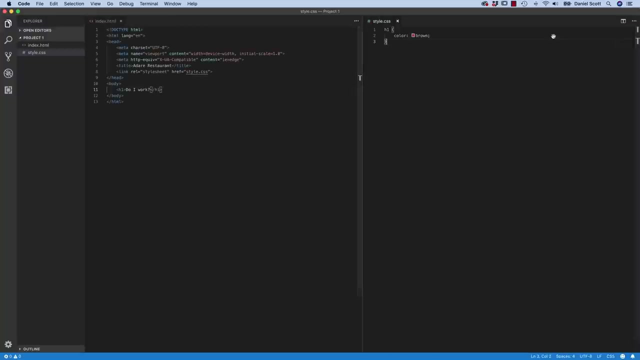 Move it around vaguely over here, not too high, not too low about there. You can kind of see it's taking up half. it's got about like that gray, it's got half of it. There we go. So the cool thing about it now is I can see my Index and my Style. 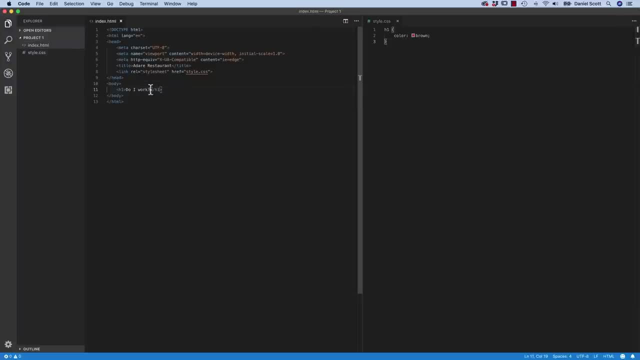 and I don't have to toggle between the two, So I can go over here and say: actually, I'm going to change this, I'm going to add an H1, H2, H2 tab. What about this? And over here you can see, look, I don't have to leave. 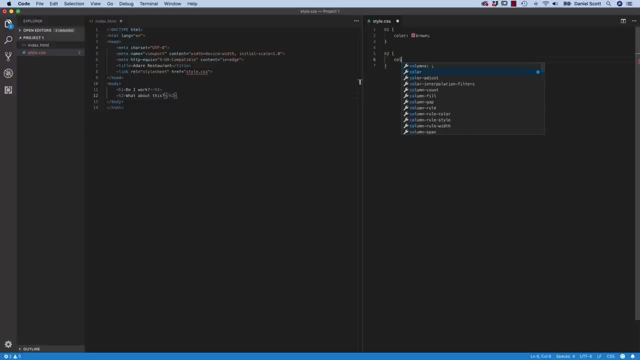 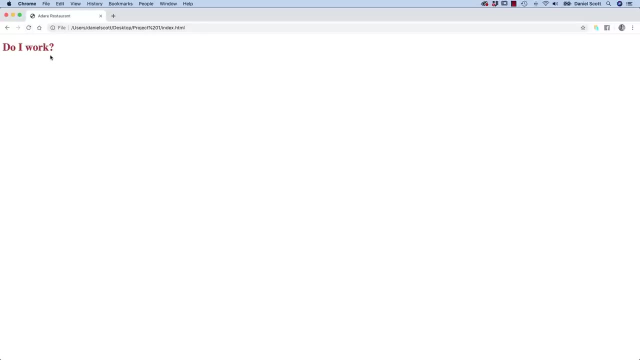 or toggle between two tabs, And I'll make this one a color of red. And now, in Browser Refresh, It's not working at all. why is it not working? You've noticed, you're like aha, I can't see it. 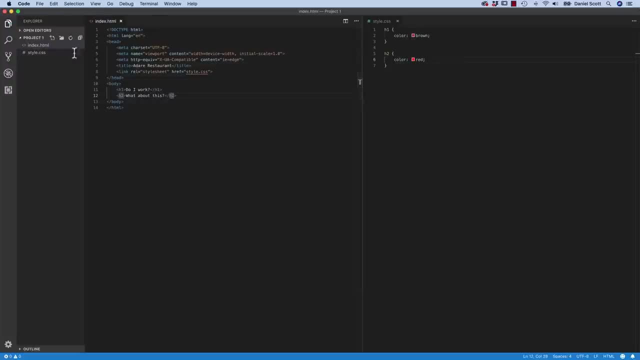 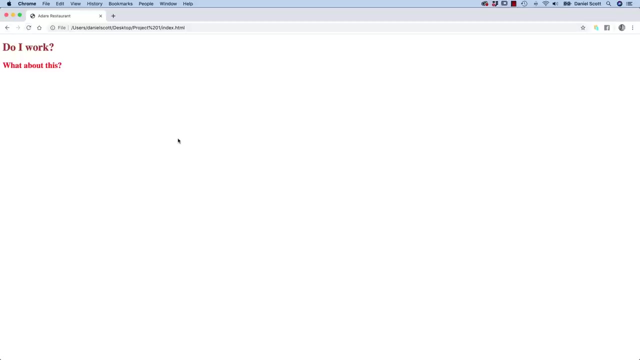 Red. do I work Save? I didn't do Save All. There you go. You know how I said before. I ran into problems: File Save All because I saved this side but not this side. I'll pretend like I did that on purpose, but I didn't. 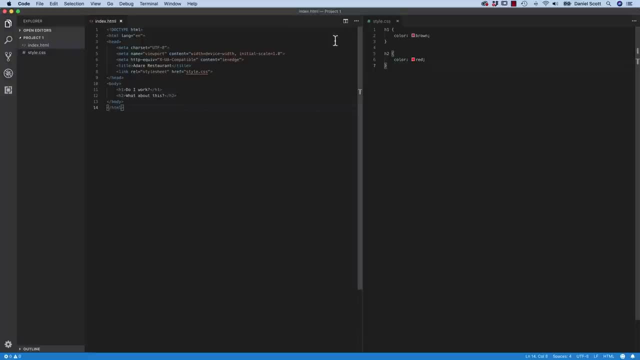 So that's a nice little helper thing to work through. If you want to get rid of that, you can click on this little icon here. You cannot, it just splits it again. Close, Close, All Close Saved. I don't know which button to click there. 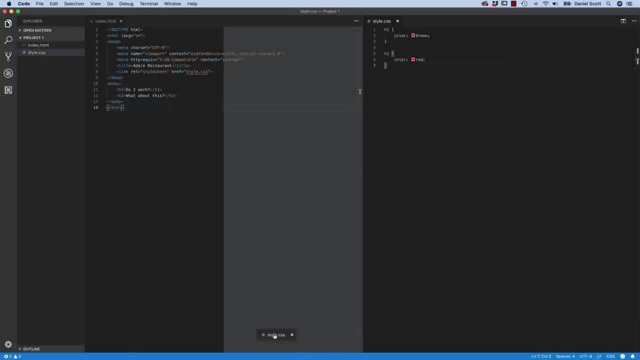 You can drag it to be down here as well. Where is it? There you go, so it can be underneath. Last little thing I want to show you is that you spend your life going from HTML, putting stuff in and then styling it in the CSS. 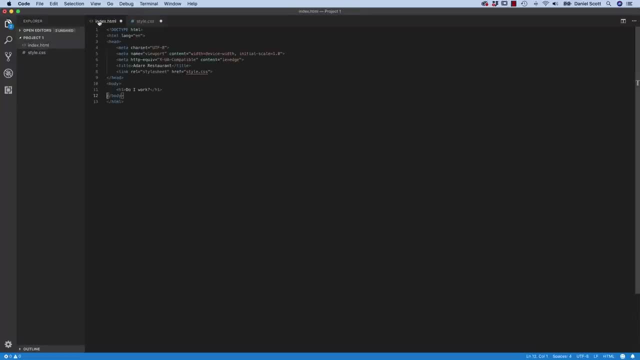 So a nice way to kind of just split these up is you can be on any of these and click on this little icon in the far right here. Give it a click and it will separate them up. It does a weird thing, I find, that button, although it looks amazing. 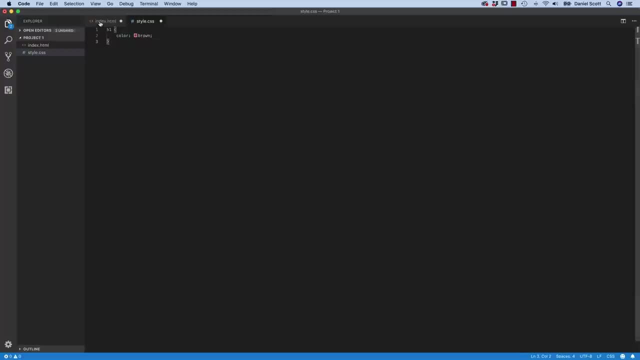 I find the easier way to do it is actually just to drag it. So I've got these two. so, stylecss, If you click, hold and drag the name there, just drag it over here you can kind of see it makes this big gray box that appears. 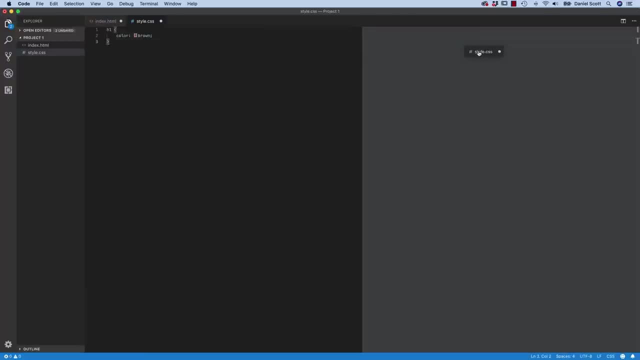 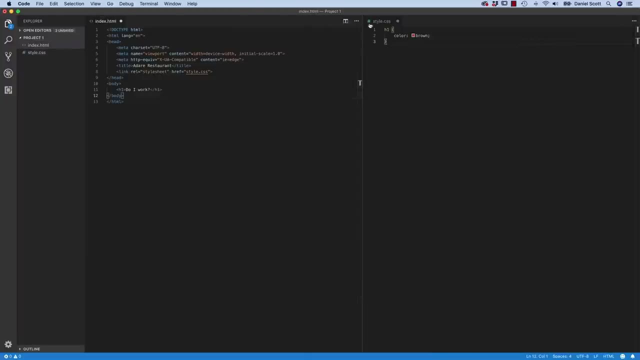 and it's a little bit random in terms of where it ends up, But what we're looking for is vaguely in the top right here, because we want that half you can see. so HTML on that side, CSS on that side. You can close it down. if you don't like that, I'll save it. 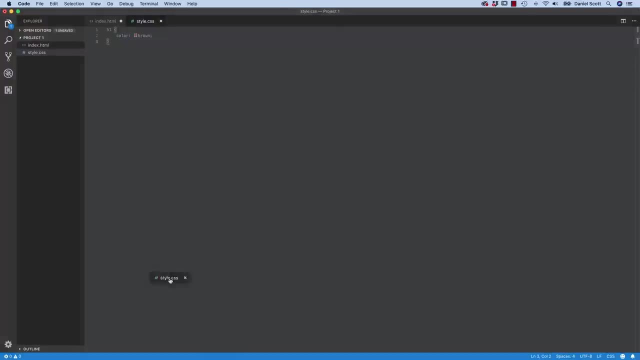 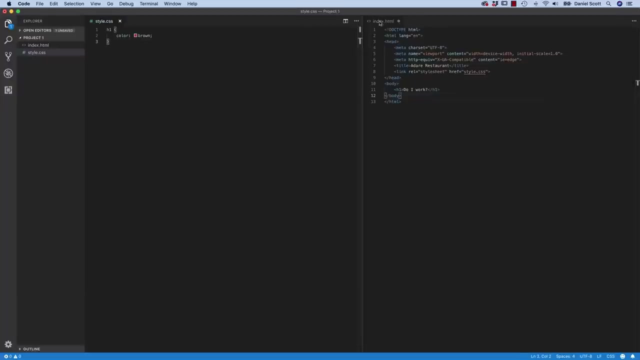 Open it up. so it's two separate tabs, but I'm going to drag it. You can have it down here as well, depending on your laptop. So I find my screen works really well, for I just mixed them up. You can, man, I find that hard. 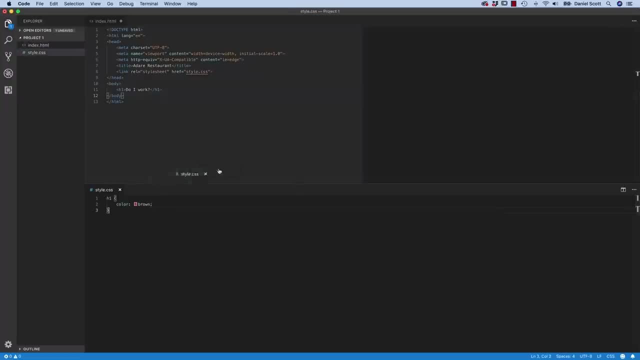 You can put HTML above CSS. I never do it that way. I always have it over here. There we go side by side up to you. So now I can go into here and say: actually I want an H2 tab. 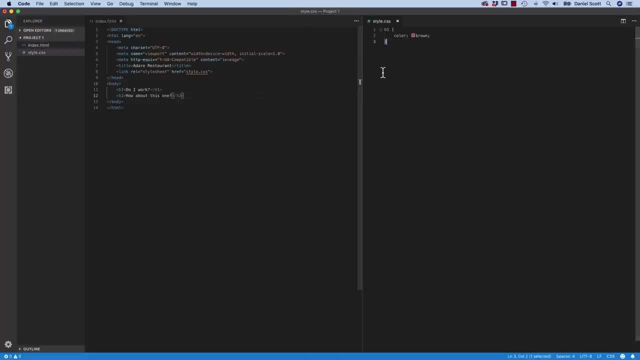 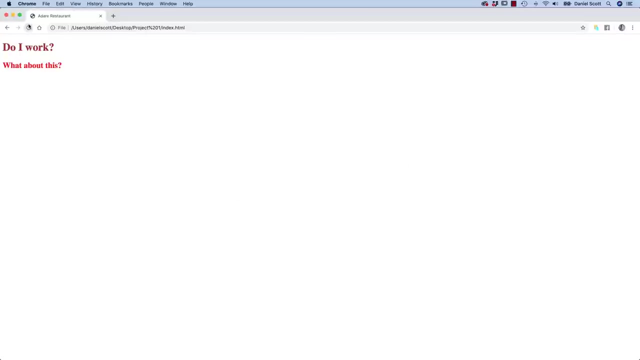 How about this one? Then over here I can type in: leave my bracket there. I can type in H2, you can see it's handy Color: blue: Save. check in the browser Browser. check blue nice. 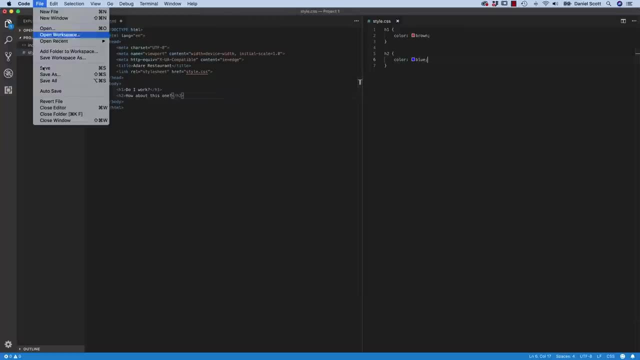 One thing you need to do as well is you need to go File, Save All. I find I accidentally hit save. my cursor is flashing over here, So if I hit, watch this, if I add an H3.. H3, and stuff. 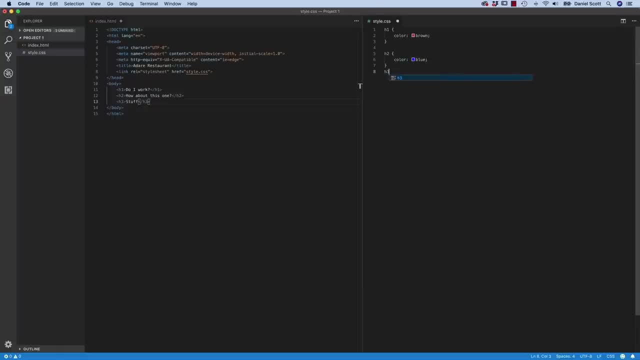 And over here I start working and I add style my H3.. Color again: whatever. I save it and I'm like refresh, refresh, refresh. I've saved it. But because I've only saved the CSS, it didn't save my H3. 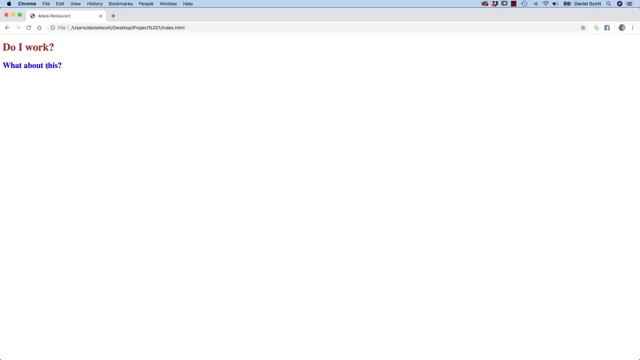 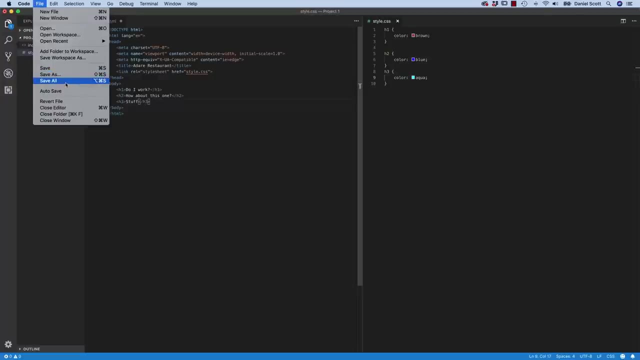 So I can spend ages trying to fix this problem. I'm like what is wrong with the code And I spend ages trying to fix a problem that doesn't exist. It's just me being silly and not going save all as the shortcut. 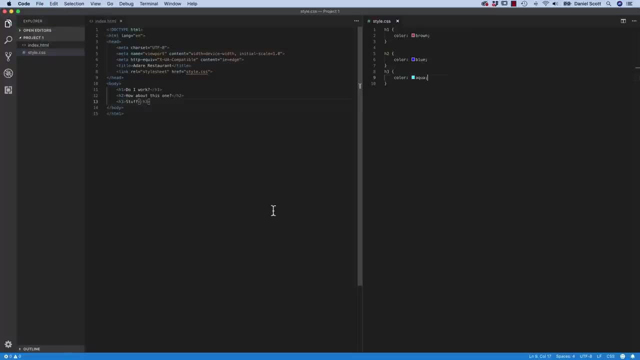 So if you're in a habit of Command S or Control S, you need to learn the Command Alt S as your default save. Or on a PC, it is Control Alt S to save all. Now let's have a look refresh. 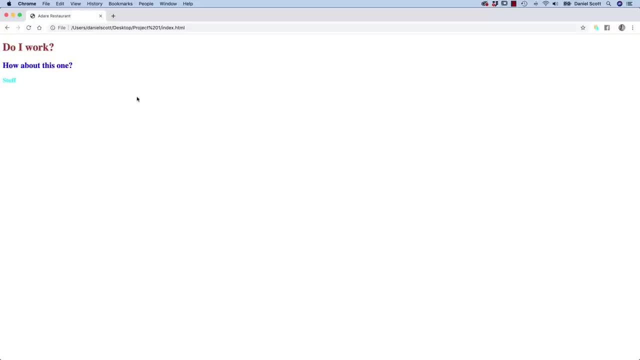 Easy, let's get into the next video. Actually, no, I'm going home for the day. I've been recording all day and it is time for a break. And tomorrow you'll hear either a more excited Dan, depending on how well his baby sleeps. 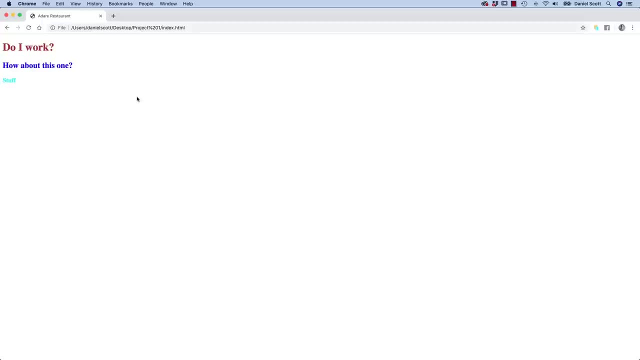 or a less excited Dan, depending on how much coffee I've had in between videos, But for you it won't matter, because I'll be right here in a second with the next video where we start looking at plugins in VS Code. 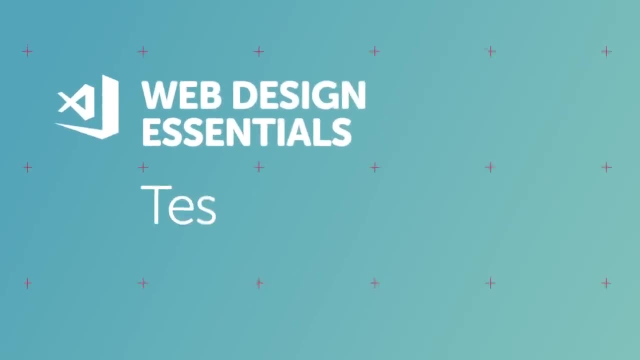 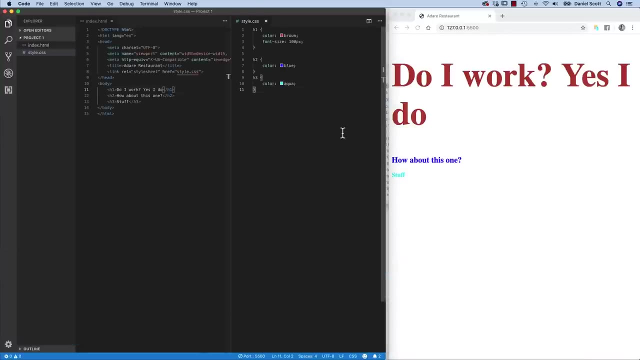 I will see you then. Hey there, this video is going to do dual purpose. It's going to show us how to install what's called an extension in VS Code, And that extension is going to show us how to do live updates in our browser. 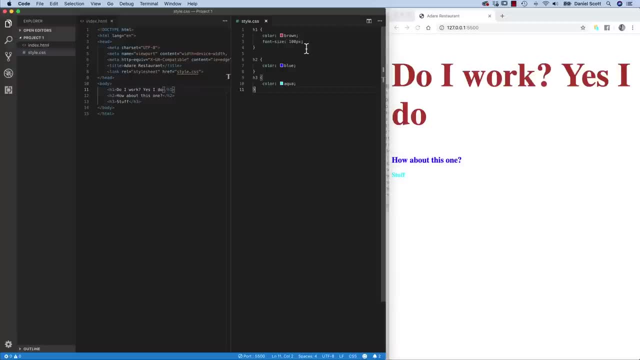 rather than going and hitting refresh every time. So I've installed the extension. I'm going to change the color here to green. It's going to be green-yellow and watch it change over here when I hit save. I'm not hitting refresh ready, just updates, naturally. 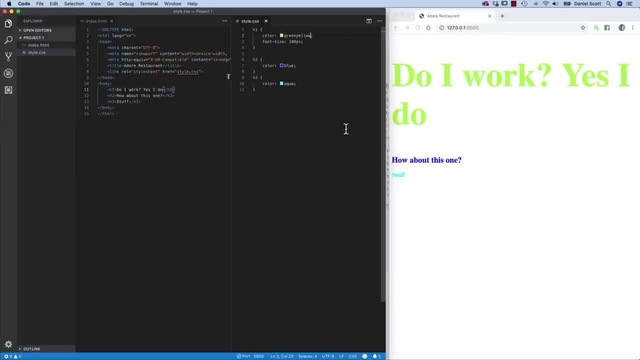 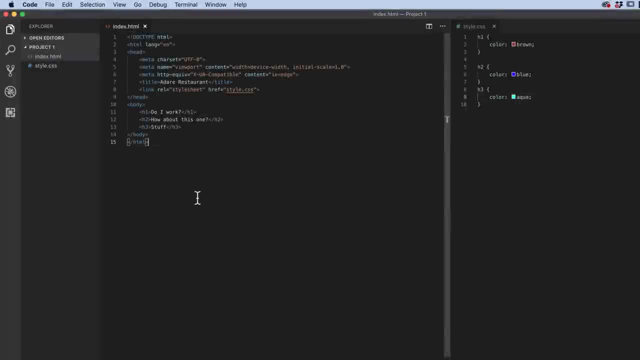 I'll show you how I use this, how I set up my workspace, my physical space, with my desktop and my laptop, and we'll learn all about extensions in VS Code. All right to get started. open up any file. I've got our indexhtml open. you can have anything open. 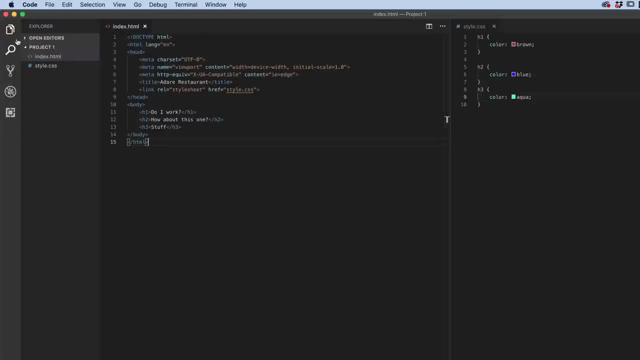 And we're going to go to the Extensions tab over here. So there's a bunch of icons. this is the last one, Or at least this one- with the square, with the square- I don't know how to describe that. one click on that. 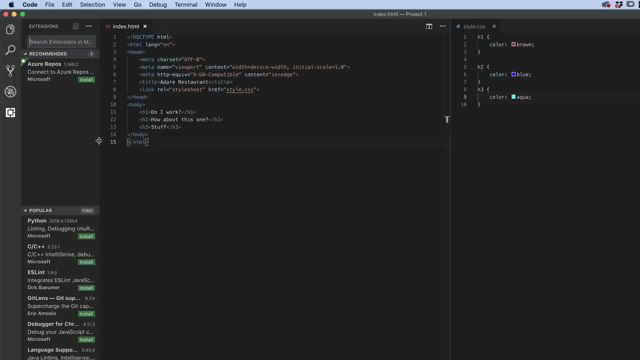 And the other thing that you might- it might- look different to mine slightly because of the width of it. So see this, see my cursor. when I get close to this edge here, I can click, hold, drag it out and eventually, if I drag it big enough, 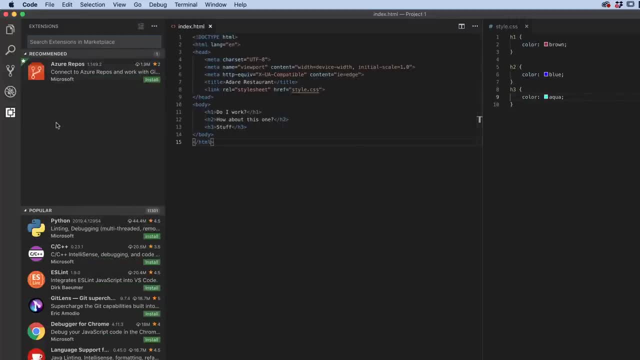 let's just drag it big enough so we can see the icons. it might be a bit big for you, but it'll make it easier for us to work out which extension we're actually looking at. So let's do a search at the top here. 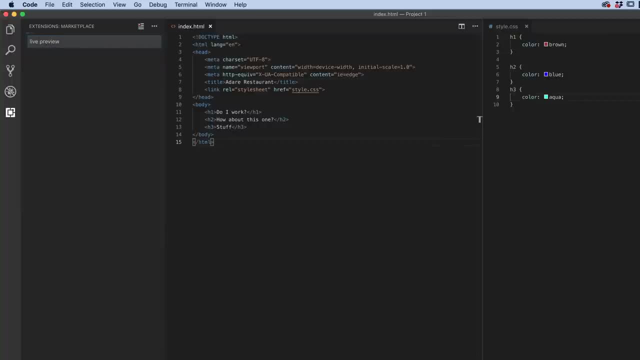 So I'm going to put in Live Preview. Let's pretend I know exactly what we're going to install, but let's pretend you don't. You're like, I want to do live previewing of my HTML, So you do a kind of a search in here. 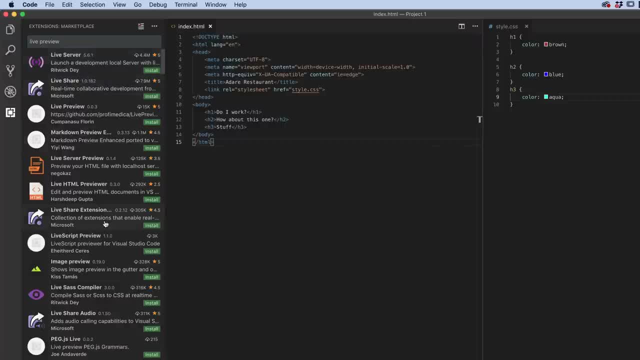 and you might have to keep typing a few different things to get the extension you want. Now, the one we're going to use is this one here, called Live Server. Now, this is, I guess, to be clear how extensions are made. 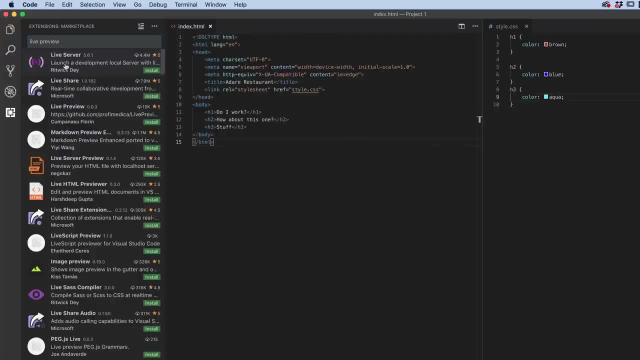 So, Microsoft, amazing people made VS Code and shared that free with us. You're like, thank you, Microsoft. What they also did is said: hey, rest of worlds, we will allow other people to build extensions for the software. We won't do it- not Microsoft, but we'll let other people do it. 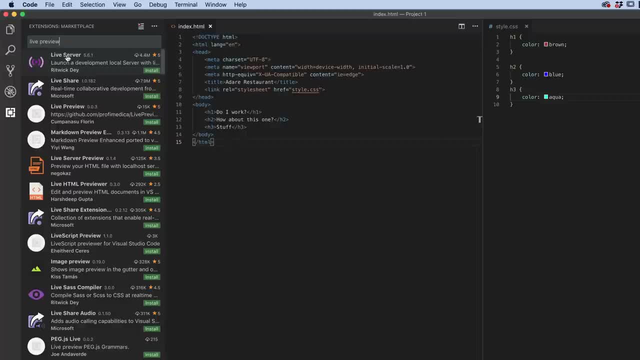 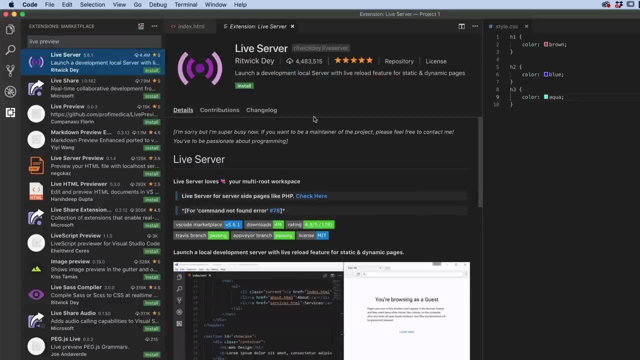 So that's a big thing to remember. we're using a live server and it feels like it's part of the product, but it's not. If I click on it, it is something made by Ritwik Day, And one day he decided I'm going to build this plug-in. 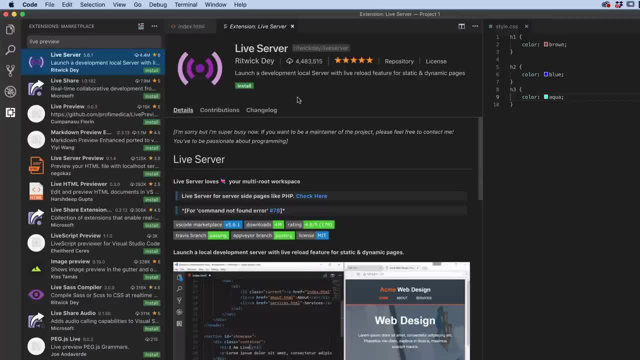 to help me use VS Code because it's not built in by default. So he did it. he made it and other people started downloading it. Now the trouble is that there might be a better live server out there. There might be another person who've made one. 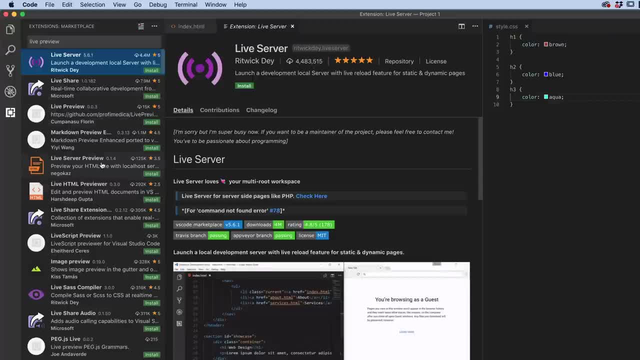 and it might here Live Server Preview. That looks pretty good, but it's got lower stars- 3.5.. This one here: it's got 5 stars and it's got a zillion downloads. That's how I judge it. so when I'm looking for an extension, 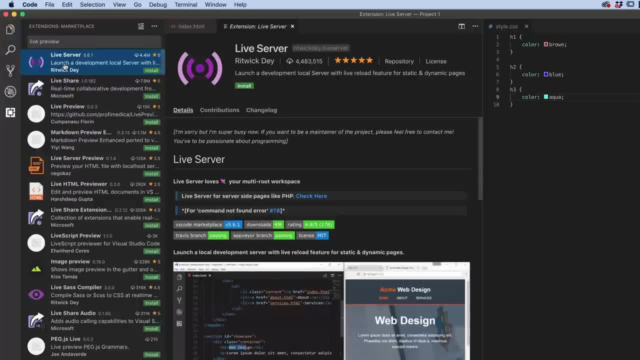 to solve my solution. solve my solution, solve my problem. I type it in and then I go through and say: how many times has it been downloaded versus how many stars it's got, And then it's like X Factor. I kind of just compare them all. 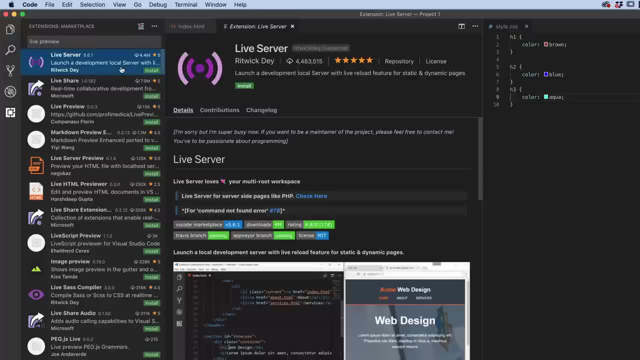 and see who's got the most stars, who's got the most downloads, and then I just pick that one. I guess I want to show you that because you might be watching this in the distant future and it might be Live. Server is not that good now. 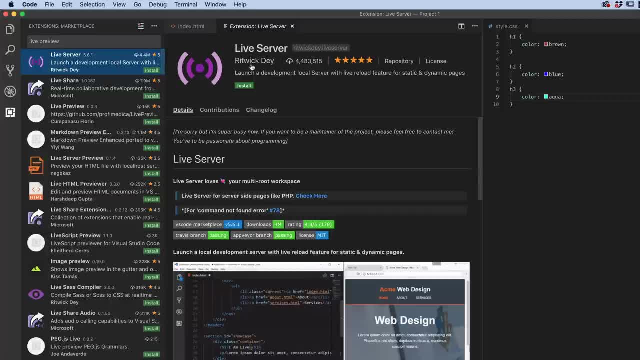 It's got like 2 stars because Rutwig Day got hit by a bus and nobody's been looking after this application. So you have to make your own choices here about which one you might use, and these will change over time. We're going to use this one, and I'll show you how to install it. 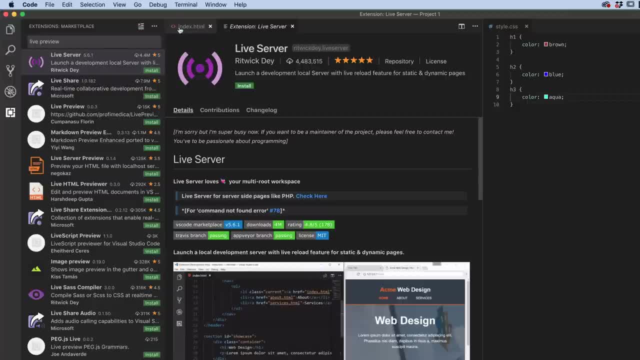 It's pretty easy. click on it- it should appear over here- and another little tab. this is my website. it isn't gone. This is an extension. tells me a little bit about it and I generally read through it to make sure. 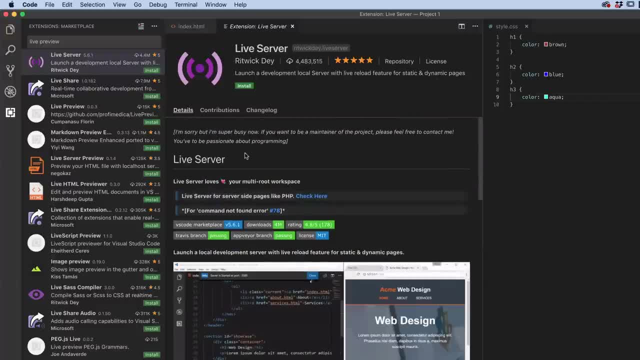 it kind of does what I need it to do And it tells you how to install it and I'm sorry I'm busy now if you want to maintain the project, See, this is a good one. there's a note in here from Rutwig saying: 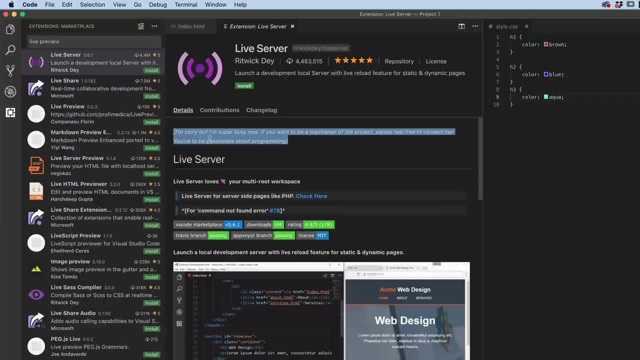 I'm not going to support this product, this extension, anymore. I know it works perfectly because I was using it today, but there's going to be a time where it's probably not going to work and the stars will drop off and he says: sorry, I'm busy. 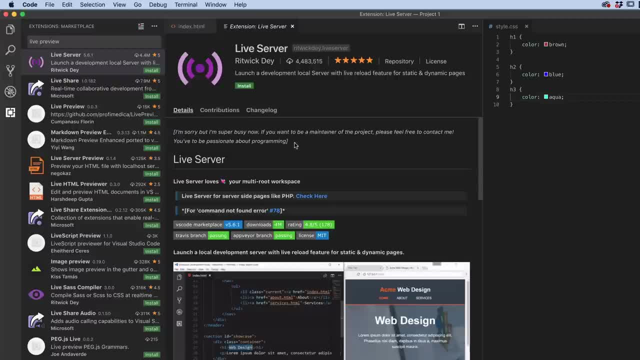 does anybody else want to look after it? And that is true of lots of programs now. a lot of software XD is doing it. they're allowing extensions to be added rather than the software makers. they just do the core and they let other people make all the interesting extras. 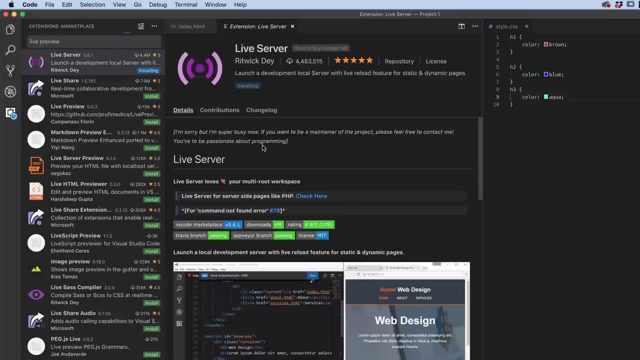 So to install it, it's easy: click the Install button. Come on, Dan should have done it at the beginning. You can kind of see it over here. that's your only visual cue that it's doing something, until it says Installed, and you can uninstall it if you don't like it. 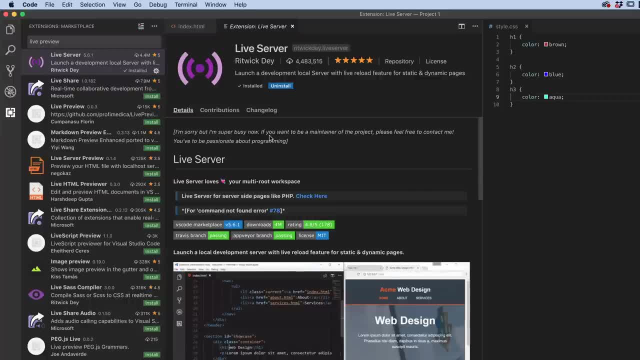 You can run through a couple of them, turn them on and off. Now for this particular one, I don't think we need to restart VS Code, but a lot of them will. They'll say it somewhere in here and if it's not working, that's a pretty good way to do it. 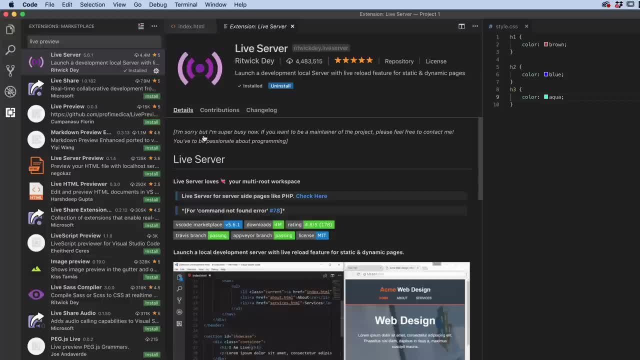 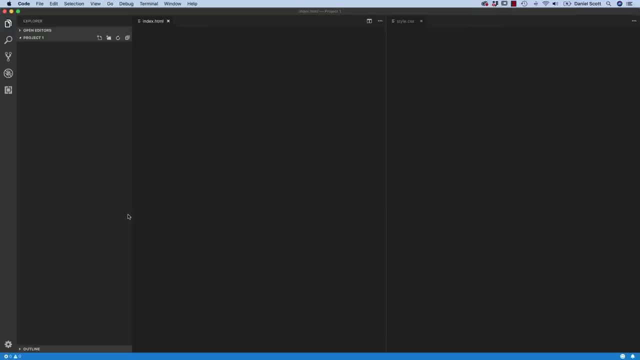 So if it's not working, let's just do it anyway. So let's go to Code Quit Visual Studio Code and now I'm going to reopen it and it's probably going to work How this particular plugin works if you read the documentation. 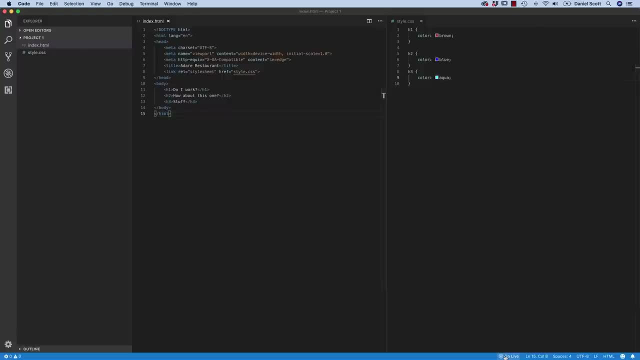 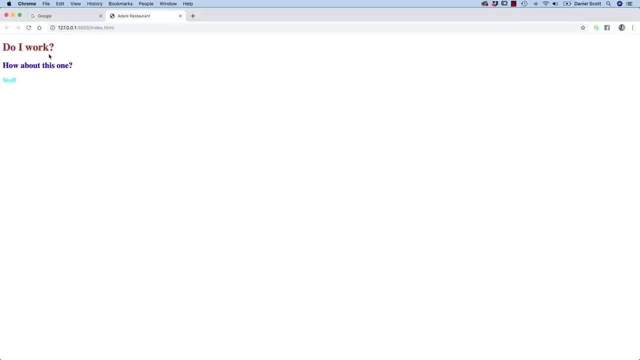 basically, it says: have a document open and click this button down here. So click on Go Live. it launches Google Chrome and it doesn't look much different than we were before, Except this one is it'll update live. We'll show you what I mean by making it a bit smaller. 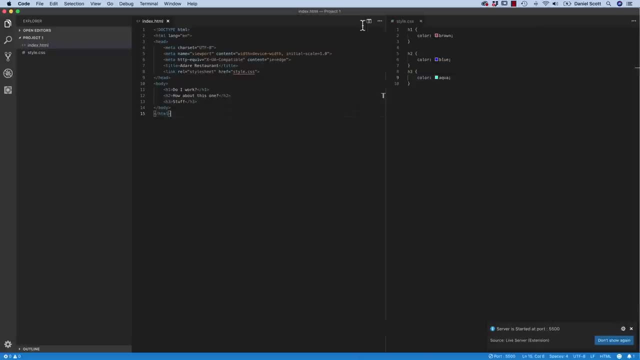 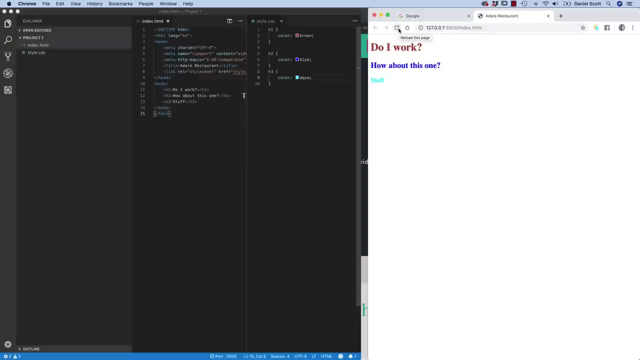 I'm going to push it over here, Move this over here, just so you can see it. So, basically, it stops you hitting the Refresh button And you might be like I don't mind hitting the Refresh button, Then don't install this plugin, we don't need it. 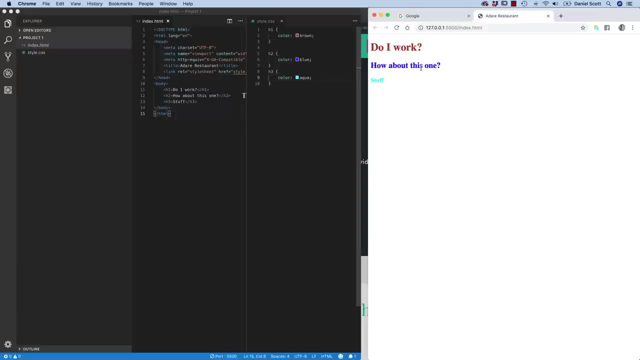 It's just handy. I like it. but if you're like man, that's just too much work and too much hassle. just yeah, you can just do it by hitting Refresh. But I guess what I want to do. 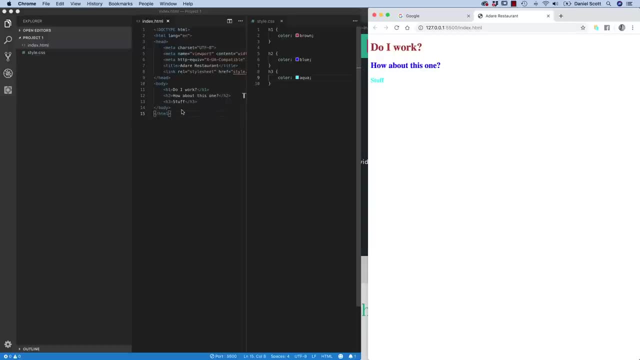 is mainly in this video: show you how to install other extensions. We'll do another one in the next video, but yeah, So what ends up happening? So watch this before I had to hit Refresh. now do I work? Yes, I do. 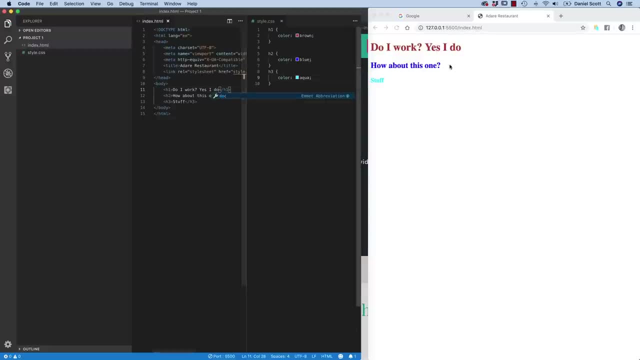 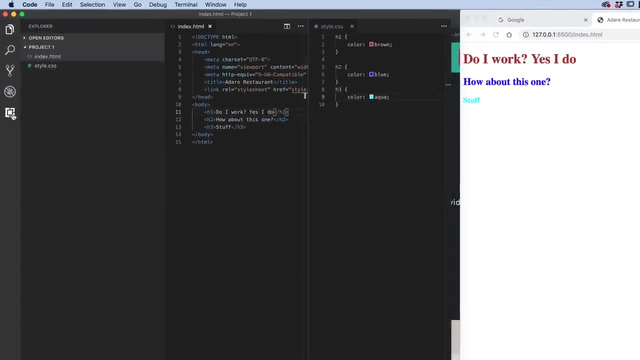 Now I hit Save. can you see it? just I saved over this side. it just automatically refreshes. So I'll show you in a second how I use this. but let's just quickly recap. Find extension type in what you want to do. 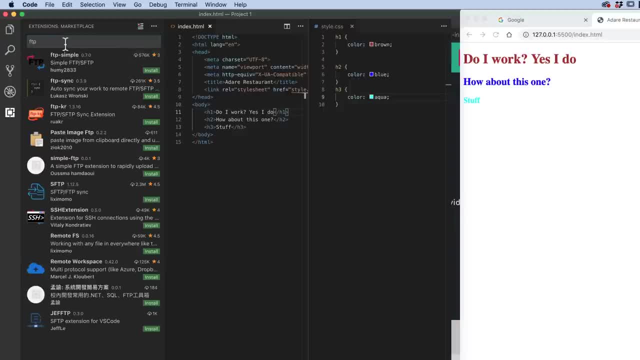 We're going to use FTP later on and we're going to use some code hinting, Find it, go through and say they've got about, not about the same. this one's got twice as many, but these both got really bad reviews. 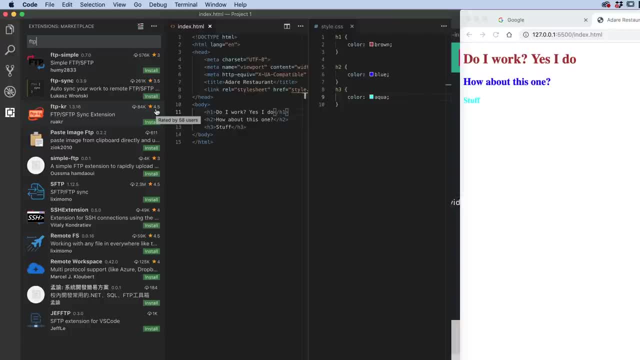 So this one's got less but it's got higher stars, So you kind of make a decision based on stars versus downloads. This one looks good, that's the one we're going to use And because it's got 2.3 million downloads. 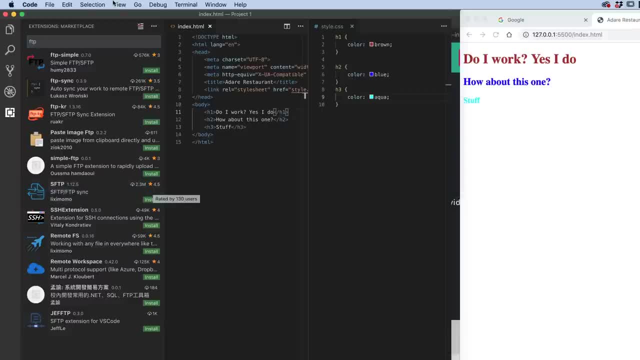 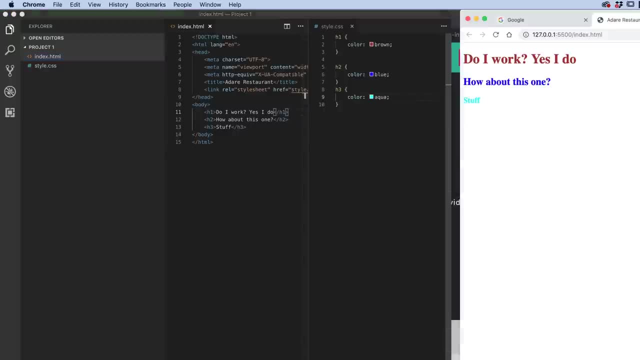 it'll be different when you look at it with a high star rating And you can close the extensions by clicking back on to your Explorer. So we're going to preview here, and what I've been doing is either having it side-by-side, like this: 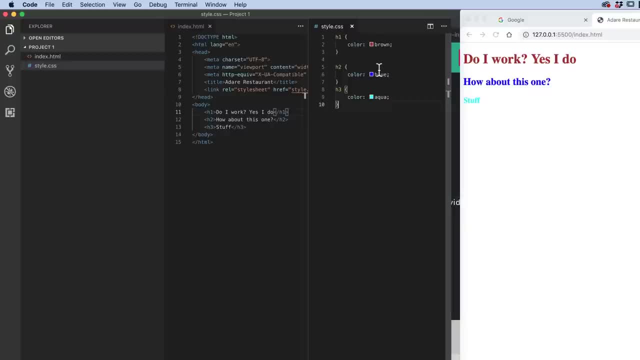 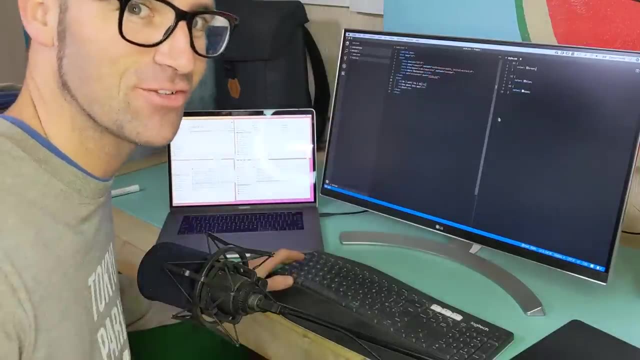 which is going to work for my really big screen. I'll show you how I normally work, though I'm going to jump out to my cell phone now and I'll show you. Hi, everyone, it's me, real me, not just the computer screen, me. 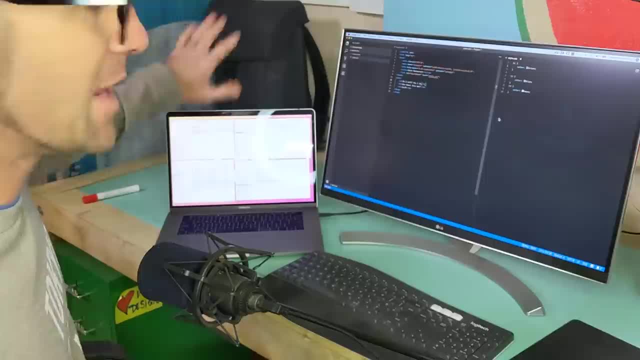 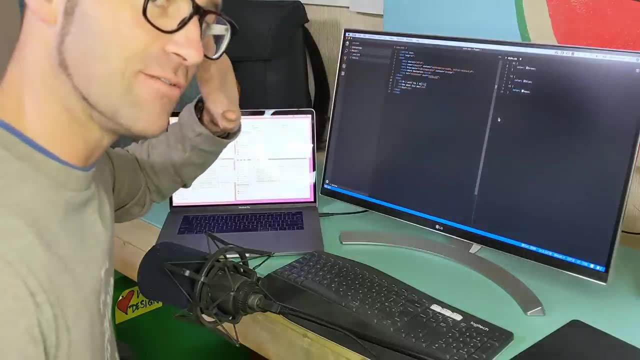 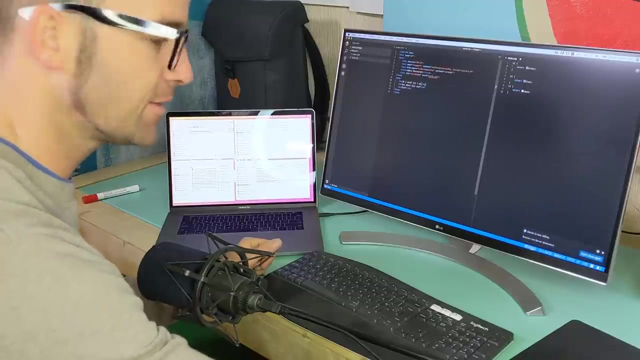 I want to show you how I kind of work. So laptop, big screen, I plug them in so they're connected, And when I'm working on the big screen here I have that. using VE, VSCode and VSCode, I'll launch the cool live server thing. 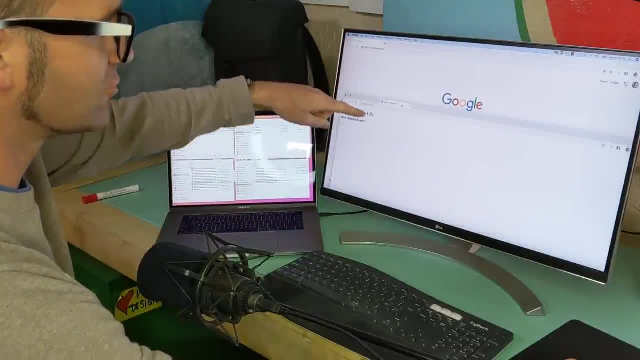 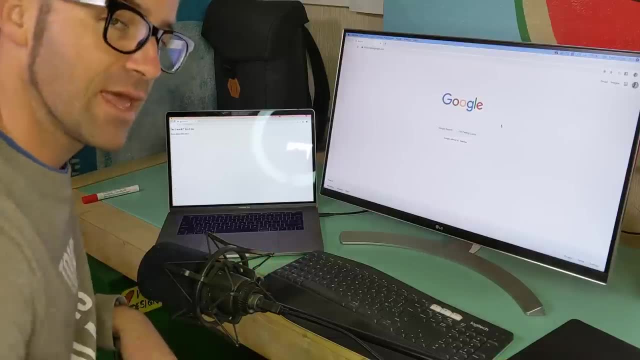 So I'll launch it. it goes big. What I do is I just click hold and I drag it And I drag it to over this screen And I leave it on there all the time, And that's how I kind of do my editing. 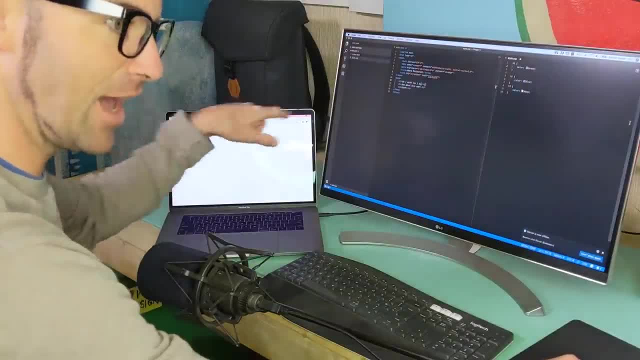 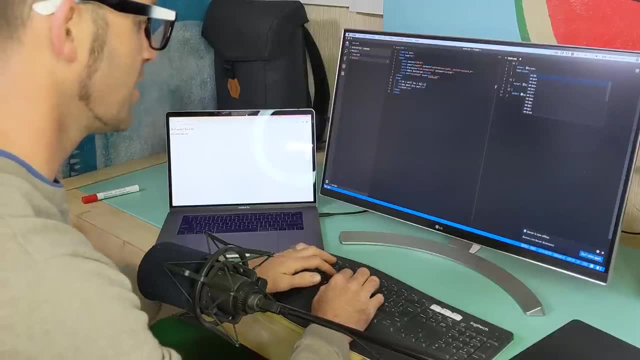 So over here in VSCode I'll try and do something so you can see a change live. So, H1, I'm going to go set font size. Font size is going to be like 400 pixels, massive. Hit, save and watch it. update over there, you ready. 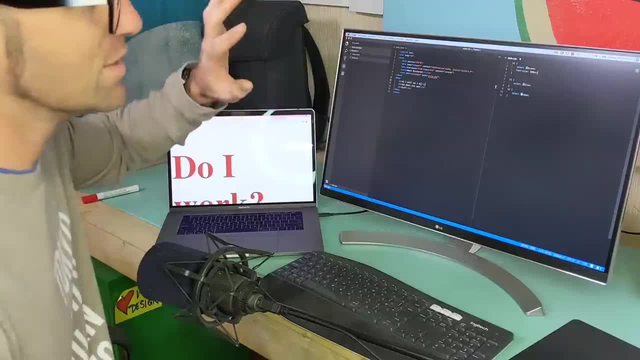 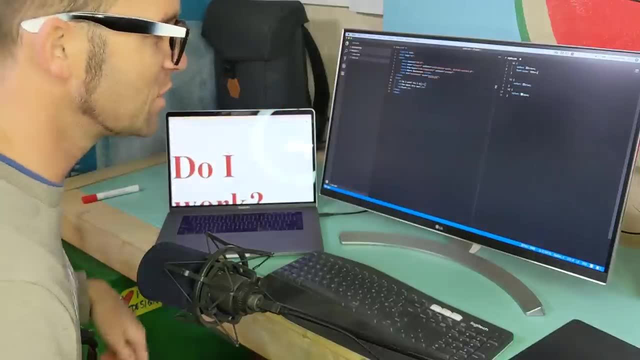 Did it update? It updated, yay. So I'm always hacking away over here and watching it to make sure the results are good over here So I don't have to kind of toggle between screens or switch between them. You're going to have an extra problem while you're learning. 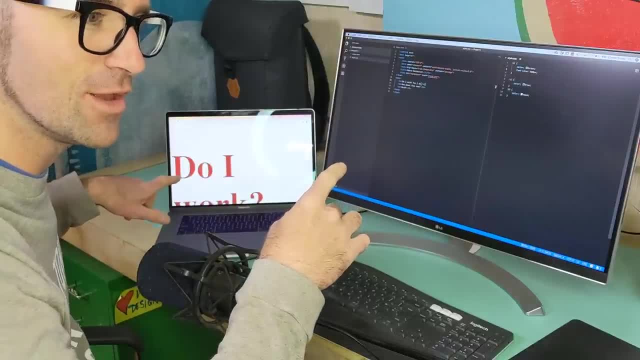 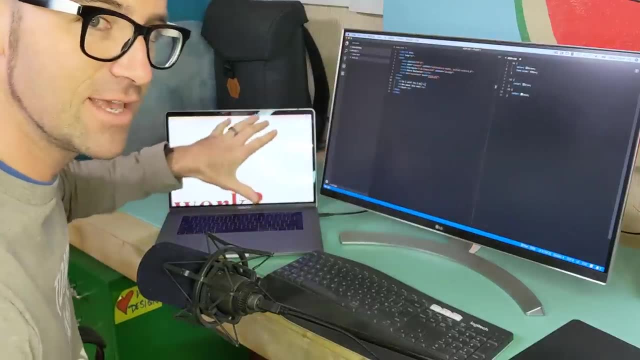 because you're going to try and do this, but you also need to watch the video that I'm making, So maybe some people use an iPad down here to watch the video on and then do these things here. You might have a tiny laptop that you're working on. 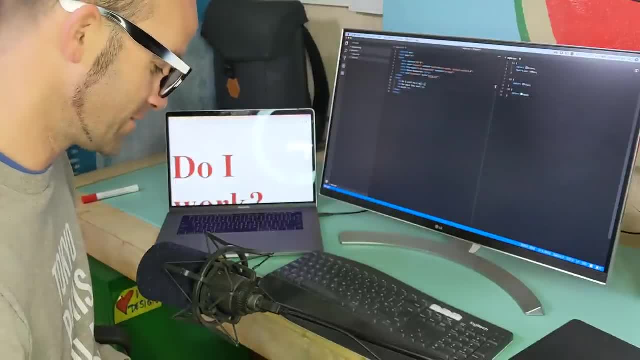 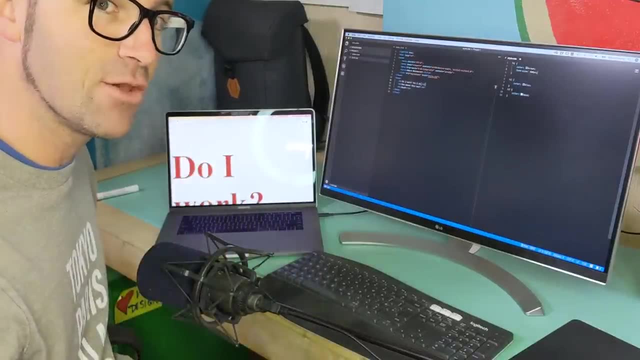 and that's just going to be fun. You have to toggle between all three videos, But that's it. extensions. make sure you check the star rating versus how many times it's been downloaded and make your own choice. The live server at the moment is pretty good. 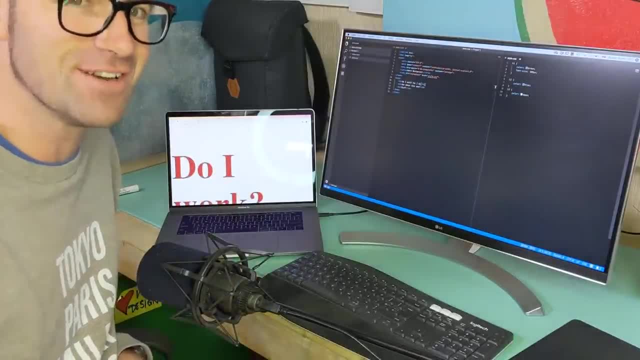 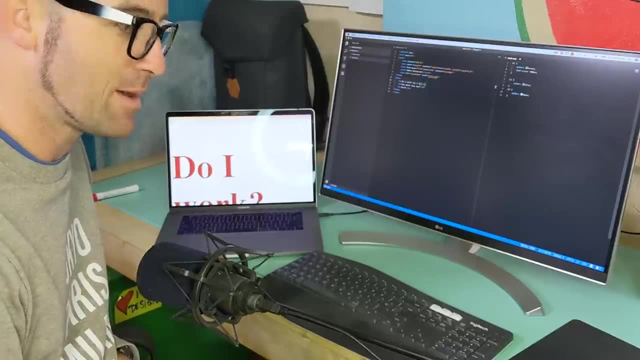 but it might not be in a year because nobody's looking after it. And that is it. We've installed our extension live server's ahead. It's helpful. I'm babbling. It's hard when you're on live camera. 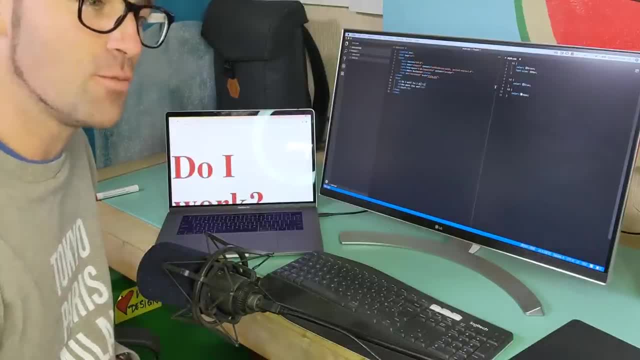 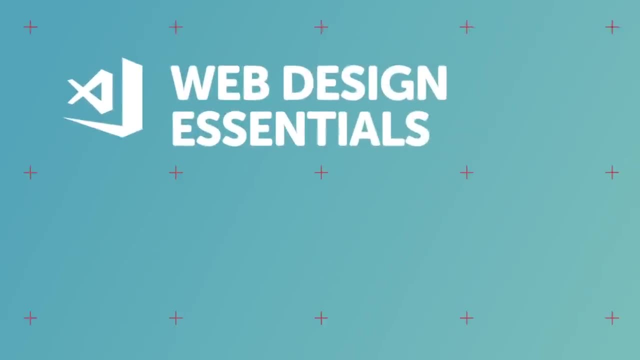 It's easy when you can edit. when you're doing screencast, I sound a lot more sensible, More rambling. I'll see you in the next video. Bye, Hey, there, wouldn't it be nice if you made a typo? 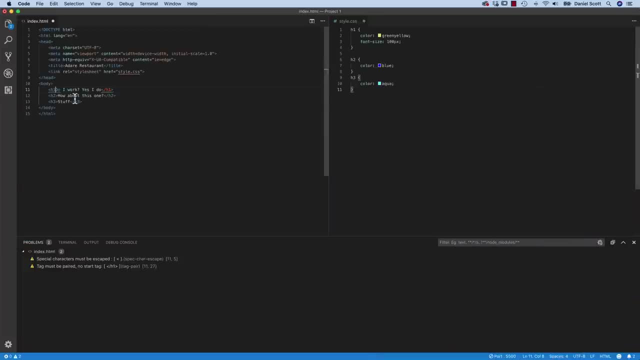 or you forgot to do something or left the brackets off, that there was actually errors that appeared and told you which line they were on and how to fix them. There is such a thing. it's not installed by default, it's an extension. 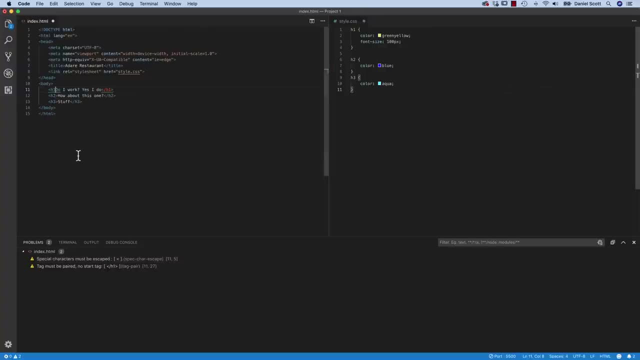 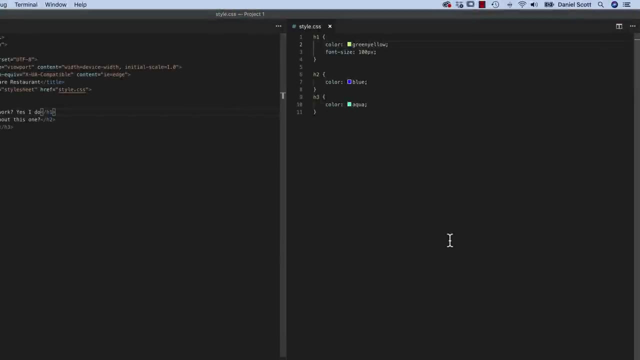 I'm going to show you how to work with that, plus other ways of checking your code and asking for help. Let's get going By default. you've got error checking in CSS for some reason, but not in HTML. You might have noticed that already. 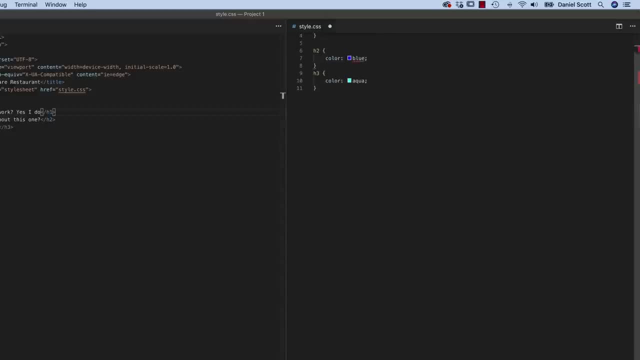 So when I do something wrong in here and I forget to put a colon in, or yeah, put a colon in, kind of like some weird things come up and it says it doesn't know, it's not expecting things and how to quick fix. 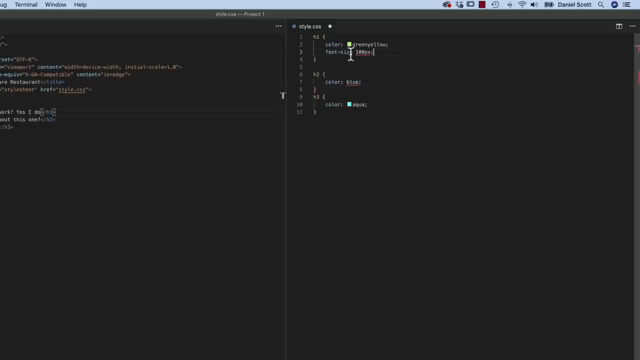 These never seem to work. None of the quick fixes work. it's going to be down to you to fix. You're just going to have to go through and say: where does the problem start? The problem starts here, so something just before. that is wrong. 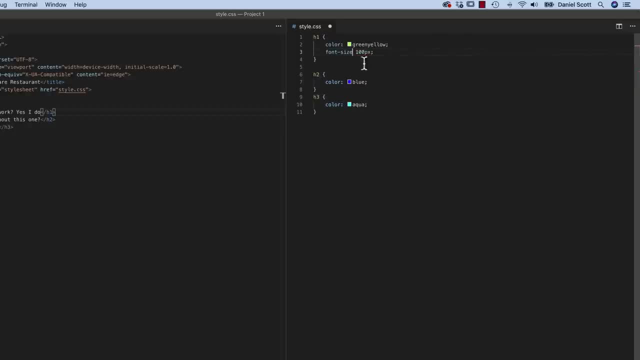 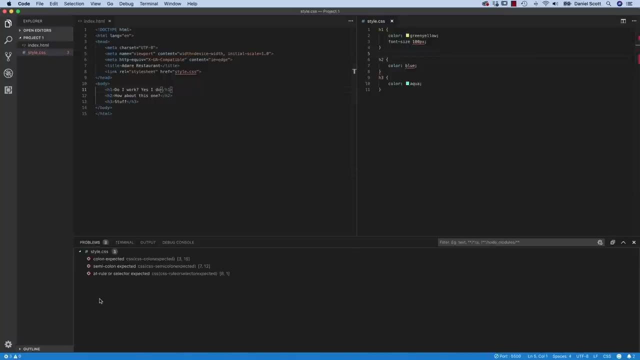 But that's helpful just to know, kind of where it starts. Actually this is deleted as well. I'll show you where else it starts Down here. can you see there's like a little errors right down the bottom left here. I click on this and it says colon expected. 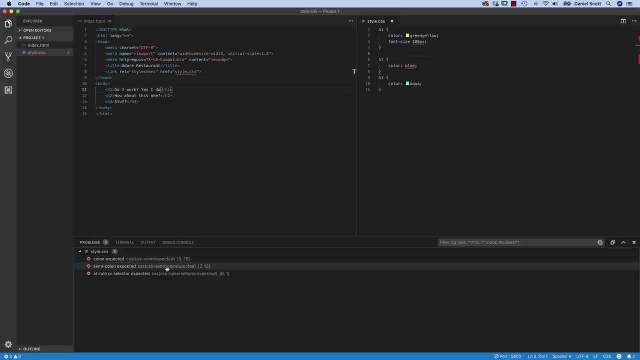 That's actually helpful. it's expecting a colon, didn't get one, So on line 3.. and it's affecting down line 15 as well. is that what it's saying? But line oh, no, character 15.. 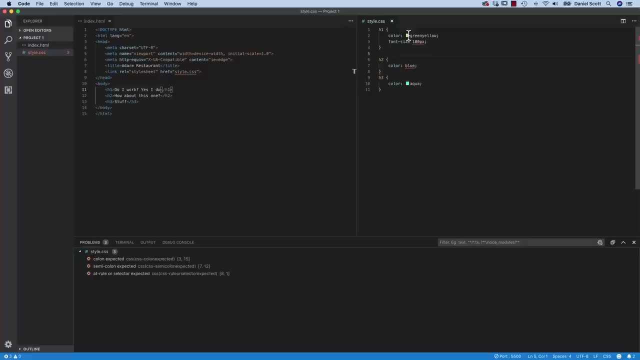 So line 3, there it is there. Now, when you have a really big CSS sheet, it becomes more useful when there's like on line 1,000.. So on line 3 there's a problem, and all the rest of these don't worry about until you fix the first one. 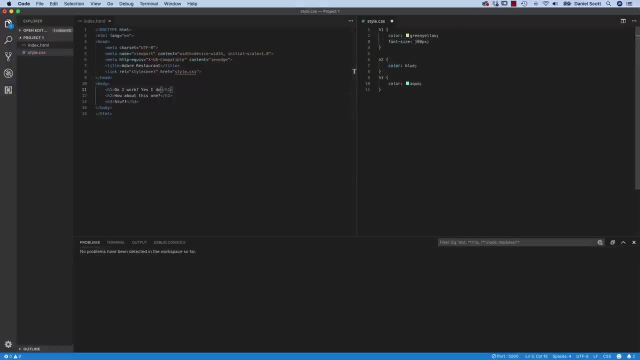 because if you fix the first one, they will all go away. There's a cascade of errors that are fixed by the first one. Now, this doesn't work in HTML by default, So if I put something in here that's not meant to be in there, 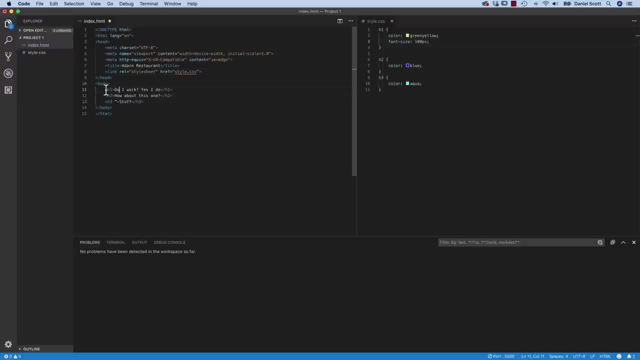 and the thing doesn't know what to do. it doesn't tell me there's nothing to do. If I miss the beginning tag- and I do parts of that- it's gone red. but there's no kind of like problem error. I'm not even sure if it goes red by default. 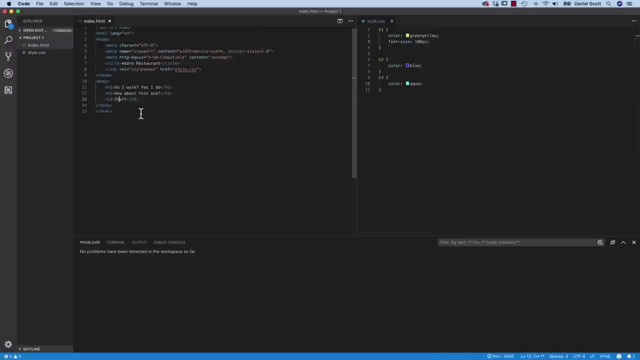 I'm pretty sure that's because of the plug-in I installed earlier on, So let's turn on this error checking. We're going to do the exact same thing as before, So it's the same as installing an extension. click on this icon here. 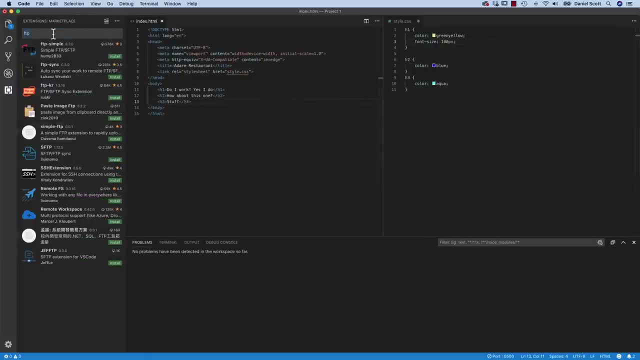 And I'm going to make it bigger so you can see And this top here and delete what's there And I'm going to say I'd like HTML and error. So this is where it gets a little bit hard. 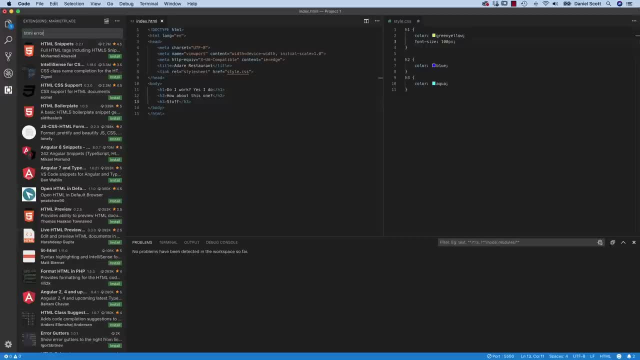 because you're like what do I call it? And there is no good rule. you've just got to start typing and seeing what results appear. you might do some Google searches In terms of error checking. sometimes it's called hinting. 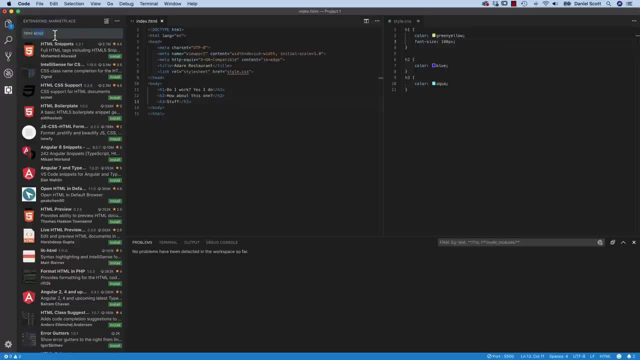 or linting. with an L L-I-N-T You can lint things, and I searched around trying to find one, and the one that I use is called HTML Hint. But even then it's really hard to find in this list. 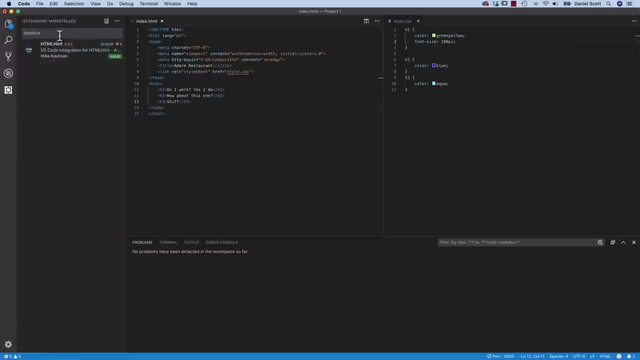 I did some Google searches and I found the one I want. It's actually just one word HTML Hint, so you've got no chance of finding it. So know that this extension search bar is okay to get started and try and find things, but just jump out to Google. 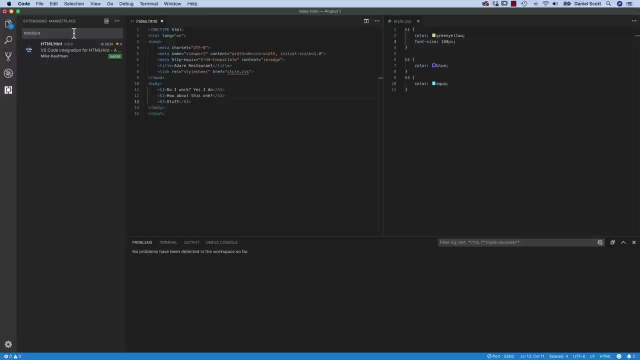 and figure out and just ask the question: what is a good plug-in for this thing that I'm trying to do? You can see here it's a really popular one. four stars works for me And it's got half a million downloads. 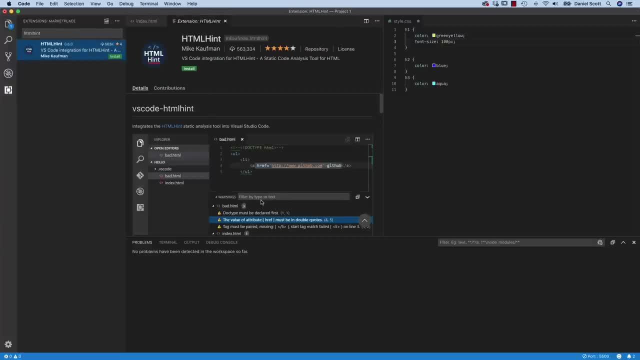 Click on it, have a look. You read through what it does and how it works and I'm going to click Install. I'm going to wait and it works. This one doesn't say restart, does it? No, some of them say restart. a lot of them don't anymore. they used to. 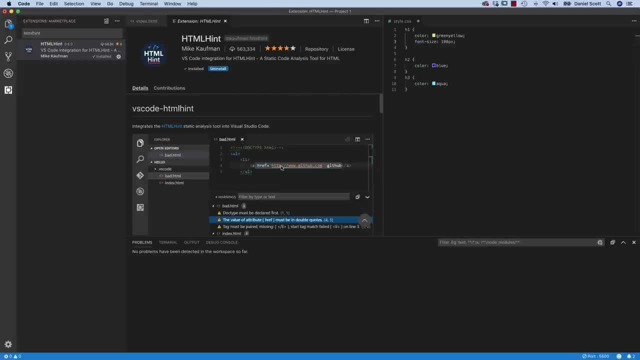 But if it's not working you can turn it off and restart it. So let's make it work. So let's close down this little tab. It was just showing me like a little preview to the product. Let's get it all reset. let's go back to our Explorer. 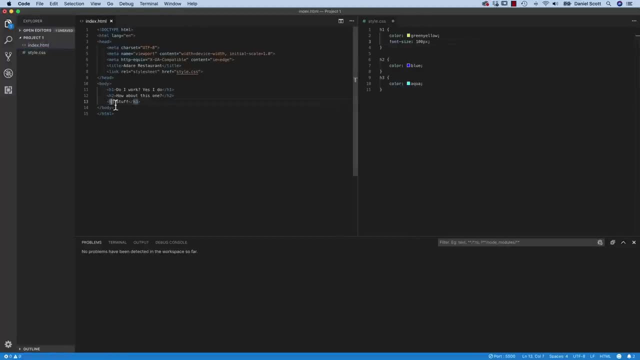 and let's make this a bit smaller. And now, if I do some errors, put in some random codes where they shouldn't be, Look a little green thing and it tells me there's a special character in the wrong place. 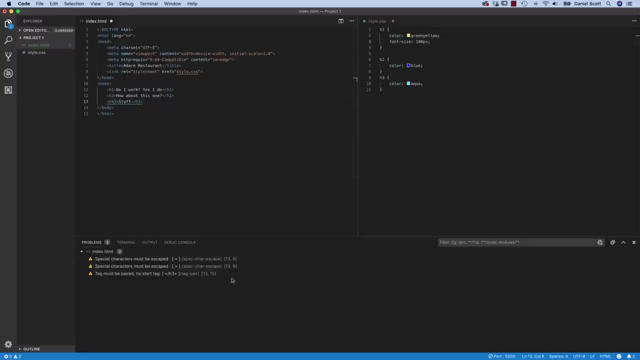 It doesn't really tell me much again, but at least I know where the error is. It's on line 13,. I can go find it. So in terms of error checking, that's a good place to get started. Turn on the extension. I'm going to close it down. 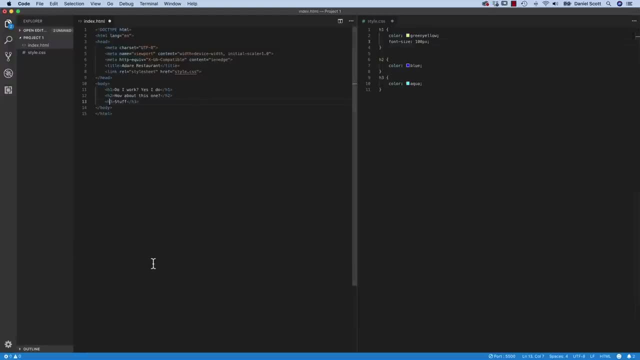 for the moment and just keep an eye on this If you're like it's not working, And before you email me and say hey, it's not working, check your errors down here. you might be able to self-diagnose. 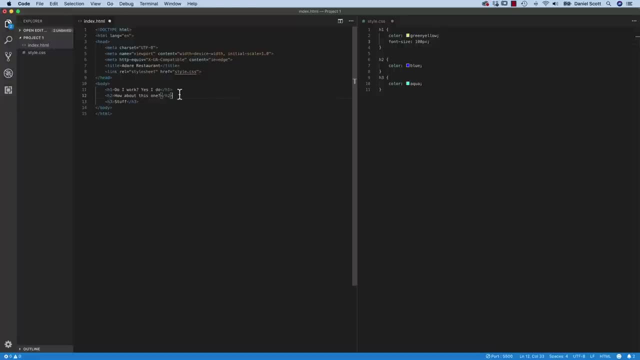 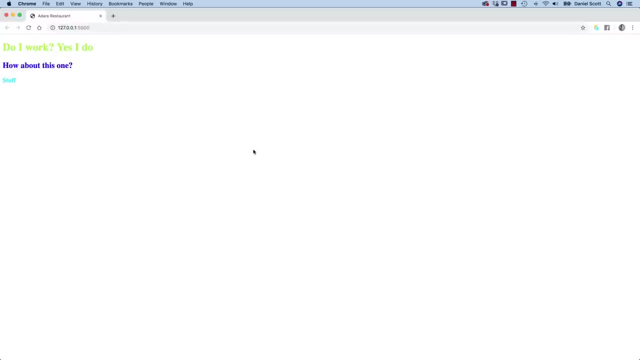 Now another thing to do before you reach out, to see if there's a problem, because sometimes it's not actually a problem. You might do something in here and change the code and check it in your browser and the browser's not showing it and you're like something's wrong. 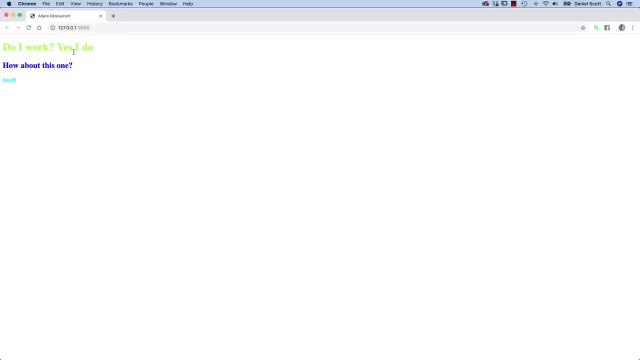 Sometimes probably one out of every 50 times. for me, it's not actually broken. Your code's perfect in here. the browser where you've been previewing is just holding on to old data. It can do something called caching, and it caches your previous version of your website. 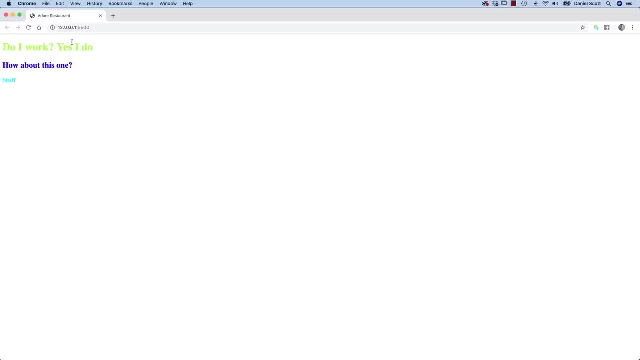 so when you're saying update, it's going, I'll use this other cached version of your website to be fast and smart. And you're like: no, no, no, don't be fast and smart, I want you to reload it every time. 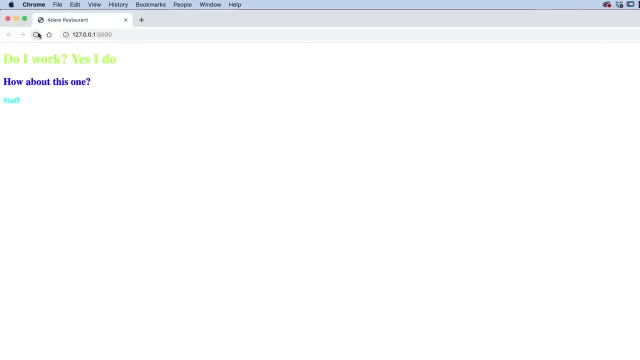 The way to make it do that refresh can work, but there's a real, definite way of making it work. You're making it reload because sometimes refresh still like if you've downloaded images here- often the browser goes well if it's the same name of the same image. 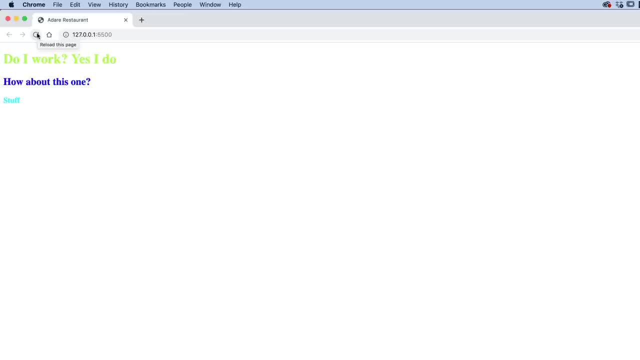 I will not update it because it's the same image with the same name, But you've, you know, you've physically changed the image, So sometimes things don't update, even though they should, talking too long. Show them how to do it, Dan. 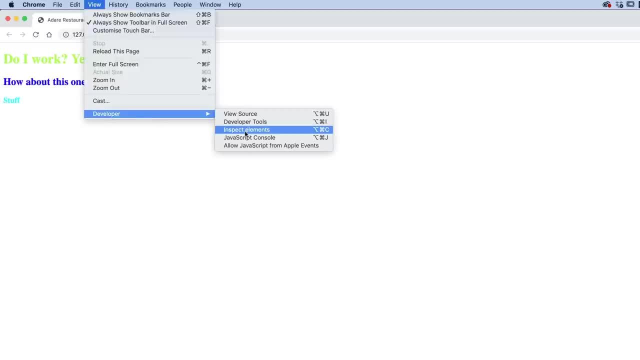 It's under View and turn on this scary set of tools. So View Developer and click on Developer Tools. Click on that and this opens up the panel down at the bottom. Yours won't look like mine. I can't remember what it looks like by default. 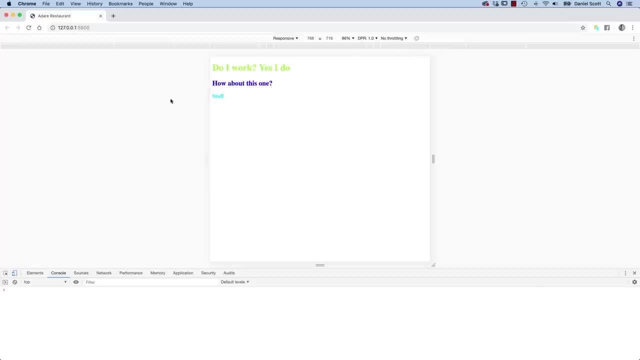 I'm going to turn that off. Oh, I can't remember. But let's talk about the main thing. So don't worry about what appears here. What you want to do is the option. so now, when you hit Reload, you can right click it. 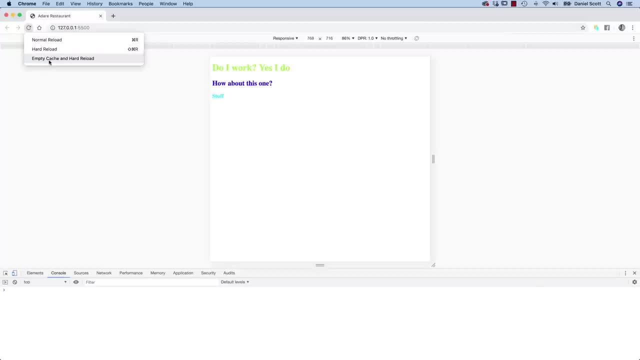 and it gives you these two new options that weren't there before. So now you're like looking under the hood. using the Chrome Developer Tools, You have this option: Empty Cache and Heart Reload. That's the. you forget everything you know about my website. 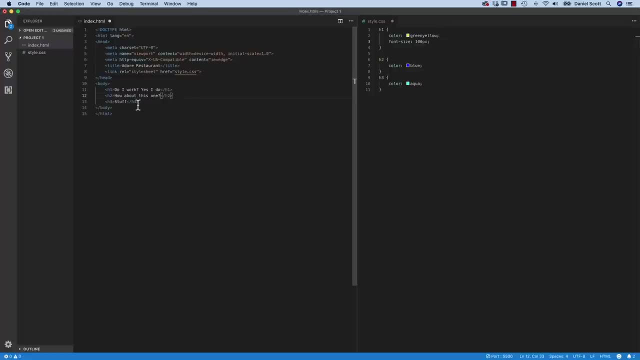 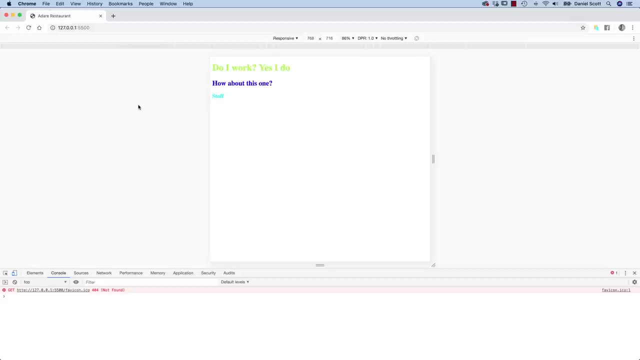 and reload it exactly the way I'm displaying it here in VS Code, And that can sometimes you know if I'm doing problems. I'm like sure it should be right. why is it not working? Everything's perfect. I go in there, check that, do it and sometimes it fixes it. 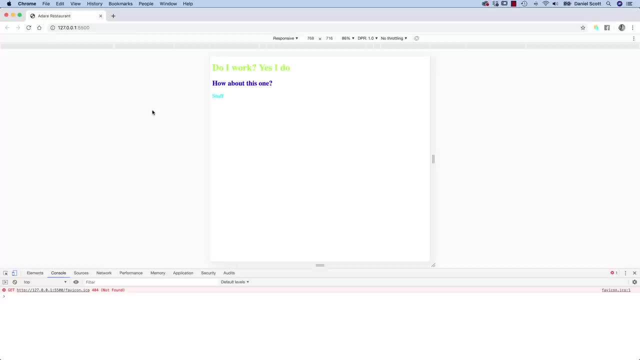 You're like phew, You know, instead of spending time trying to reach out and figure out how it's broken. it's not actually broken, Just the browser didn't update. All right, What else can you do Now? you can totally ask questions of this course. 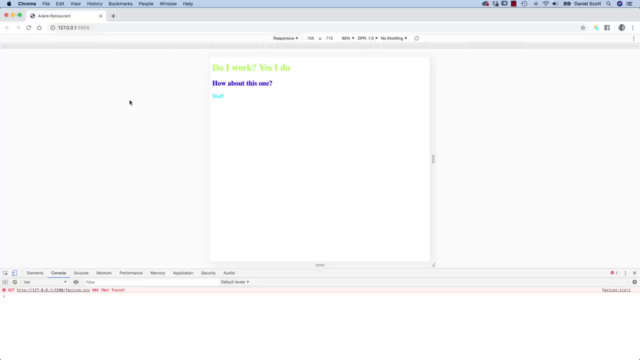 Like there's comments. use the Comments section. use social media like you'll see all the social media in the class exercise files. Reach out that way, But often, like it's just me. for this course it's a new course. 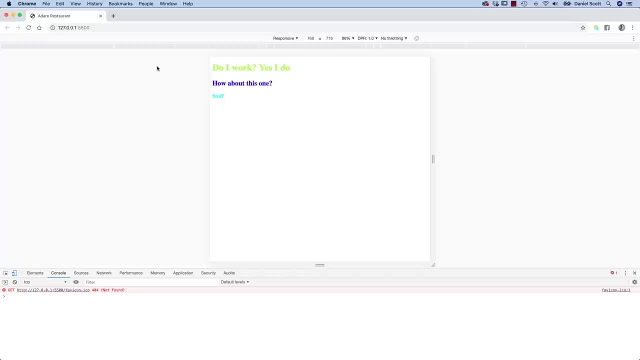 You know I try my best to answer questions. Sometimes I get a bit backlogged, or it's the weekend or I'm on holiday. So definitely use that as an option. But you'll also find Google searches. I know it's a lame thing to say go and search on Google. 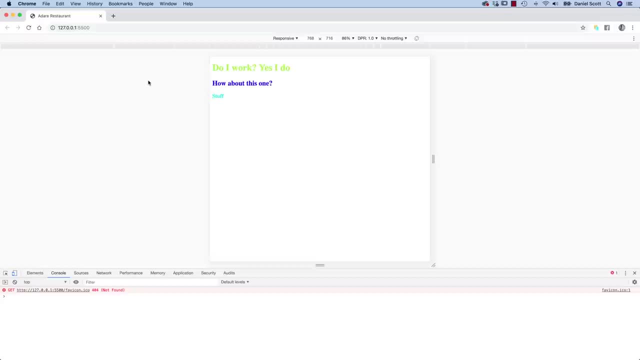 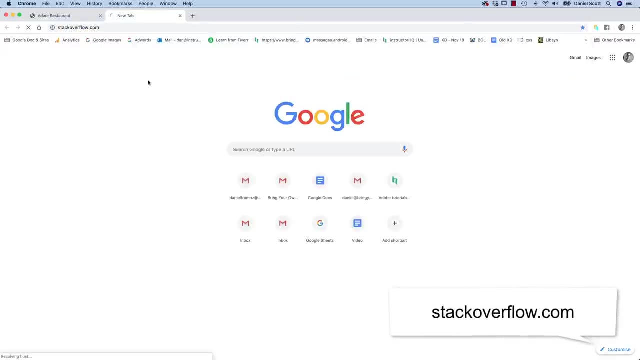 but what you'll find is there's a couple of main places, actually one main place. it's called Stack Overflow. Stack Overflow will appear in lots of your search results, but searching in this site, it's just amazing. I listened to a podcast. the guy started this. 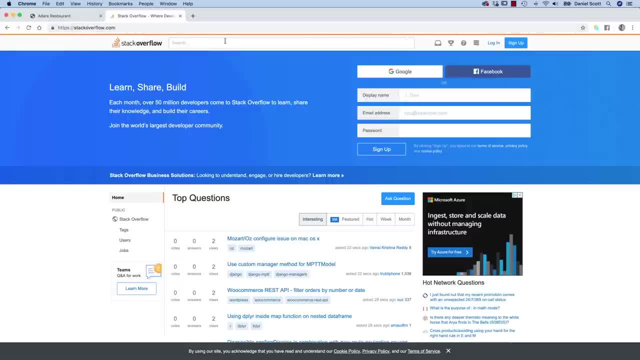 Like it's for designers and developers, anything web. Ask a question in here. you will find lots and lots of really useful answers, and they're curated answers from other users. What you'll probably find is: you don't actually have to ask a question. you can log in and sign up and ask a question. 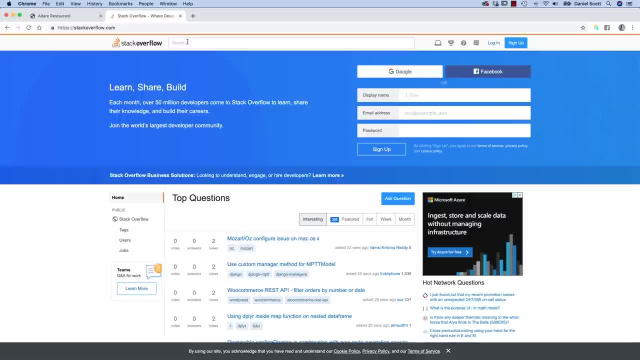 but you'll find it's probably already been asked, Especially at kind of our level here where we're just getting started. So Stack Overflow is an amazing site to get and you get a response straight away. I guess what I'm saying. 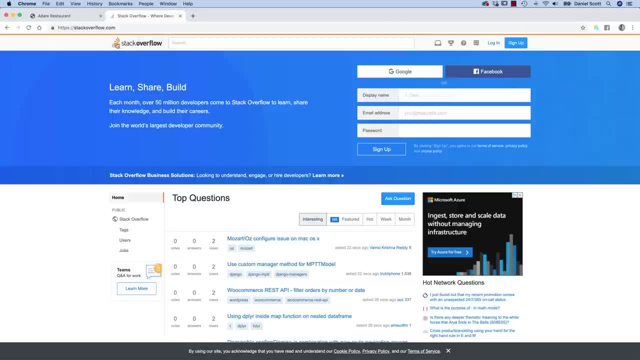 If you're still having problems, drop me a line. All the different ways that this site gets viewed, that this video course gets viewed: Use the comments or the Ask a Question button, And often to kind of fix your problem, I need to see the code. 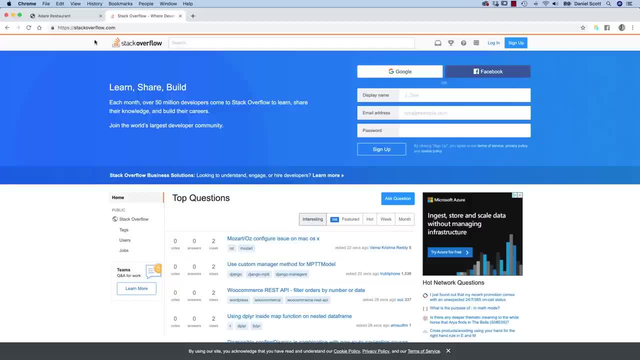 So zip it up, So compress it into like a little folder and send that along, you know, like a link, maybe using Dropbox. So I need the files. you'll have to work out a way that works for you. Sometimes you send it as a system to sending things. 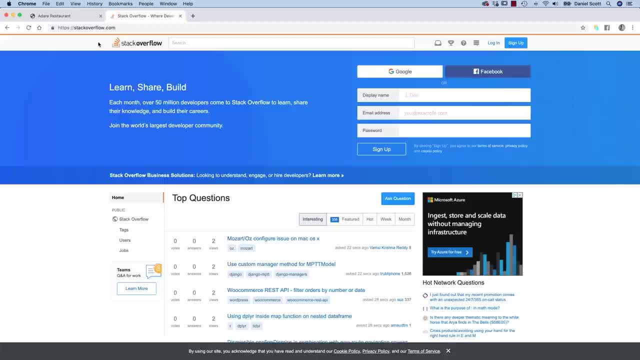 Dropbox is a really good one Because obviously screenshots are really hard to kind of. I can kind of see what's going on, but it's a little bit hard to edit your code, Otherwise I got to start retyping the whole thing. 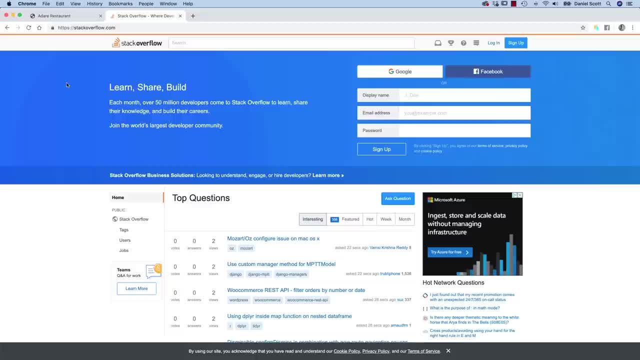 and try and work out what went wrong. Now my only thing is, if you're asking questions, say you post a question, have a look through the other comments and see your questions and see if there's one that you can answer. 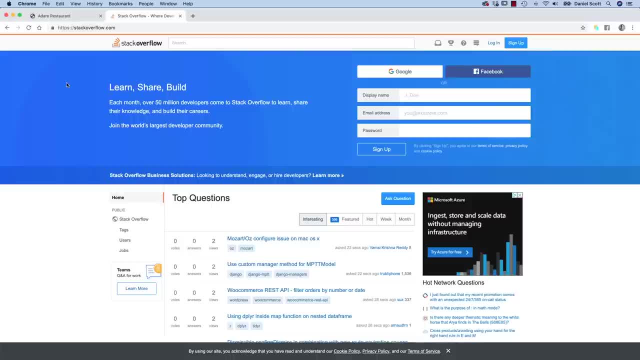 Say you're finding this not easy, but you've got that concept. you're like man, div tags, got it locked in And you see a question, somebody asking about div tags. I'd love to try and start that sort of momentum. 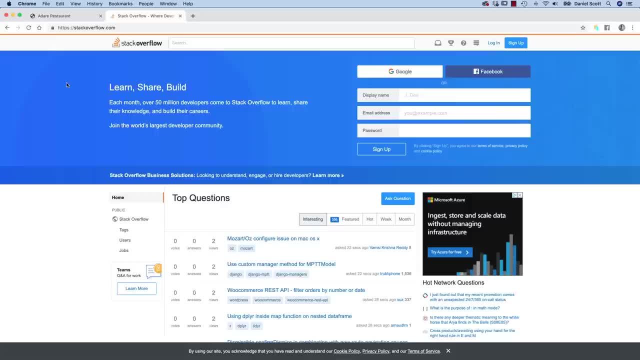 where, if you're asking a question, you have to answer somebody else's as well, or at least give your best opinion, or try and do it so that we can, I guess, get answers quickly, And for you you'll find it super valuable. 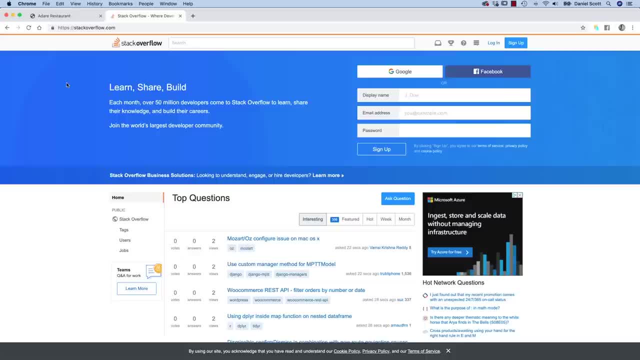 if you are able to answer somebody else's questions, It's pretty amazing. Something like being able to articulate that to someone else really drives it home in your own mind about that topic, And plus, if I'm on holiday sipping pina coladas. 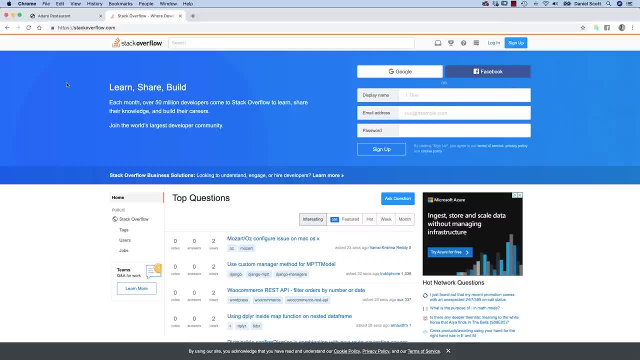 somebody needs to help. but don't worry, I've got a baby and a five-year-old. there's no pina coladas in my near future. So, to recap, do your own error checking using the HTML hint that we just installed in Visual Studio Code. 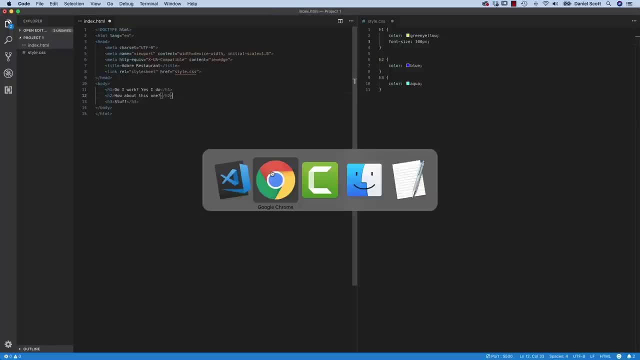 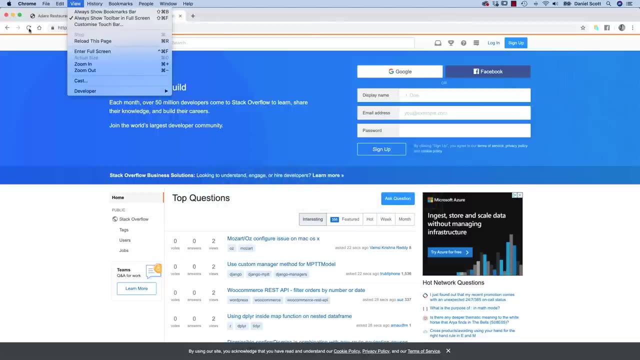 Check that it's not actually a problem by refreshing your browser. but remember you've got to do that by going into View and going into Developer and Inspect Tools or Developer Tools, and then right-clicking the refresh button. Stack Skills is an amazing place. try it with me as well. 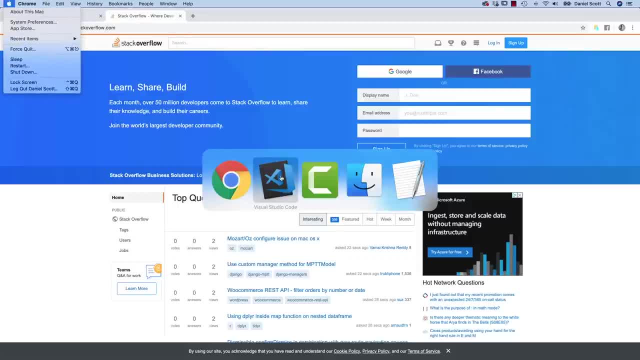 We're using the comments or hit me up on social media. One last thing before we go is there might be a say. it happens a bit like I'll go into my extension and I'll be like, great, this one works. 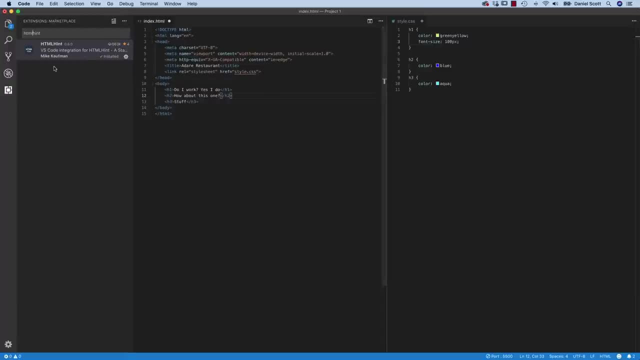 It looks like it works, I install it and I just can't make it work or it's broken. So sometimes you need to uninstall extensions. So to do that, click on this little weird Clear Extension Inputs. So with that cleared, your search disappears. 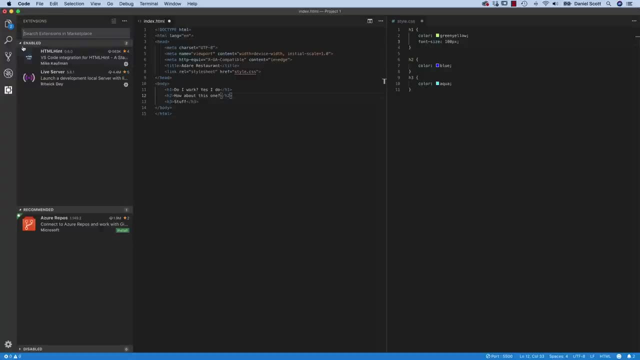 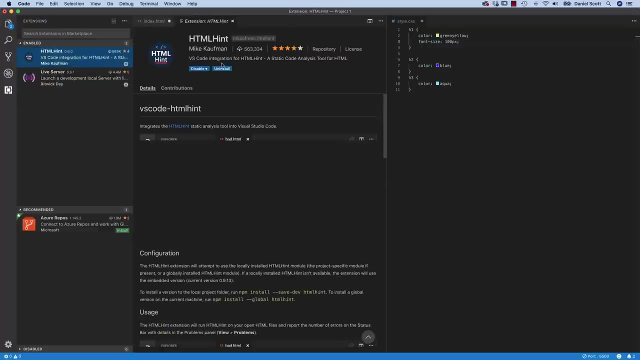 and it tells you things like the ones. well, it tells you exactly what's enabled, What's recommended. I never find that useful, but over here it tells me the ones I've enabled, So I can click on them and say, actually, HTML hint doesn't work. 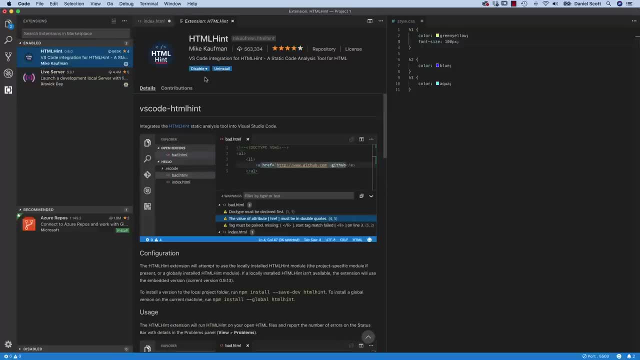 I'm going to uninstall it and try a different one. You can disable it temporarily. Say that you're like: actually, is it working? Is it breaking something else? Let's just disable it and then test something and then enable it again to see if that thing goes away. 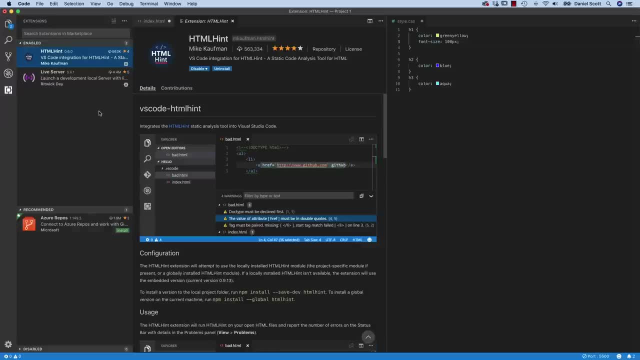 I've never had to do that. Often the star rating kind of fixes that or at least guarantees a half decent plug-in or extension, And that's it. that is HTML checking. It's on by default for your CSS. Let's move on now and actually start building the structure. 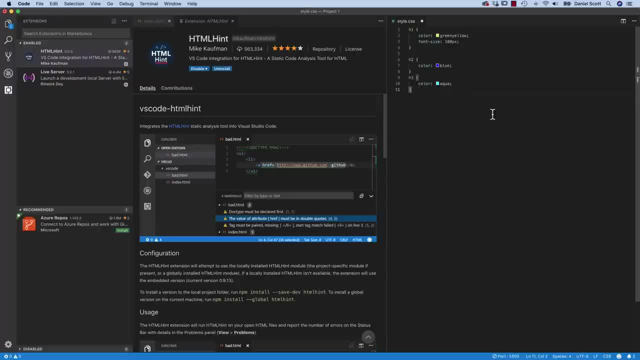 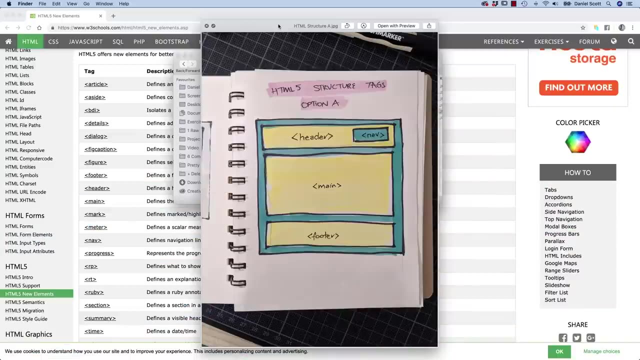 for our Project 1, the restaurant. I'll see you in the next video. Hey there, this video is all about learning what the HTML5 structure tags are. They are things like header and main and footer and nav. 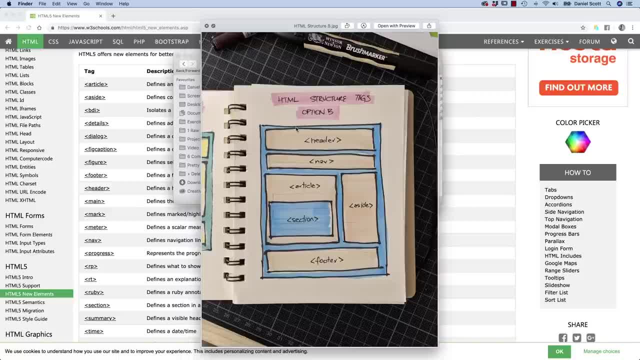 And you can kind of see. they're pretty simple. They're just containers that we put stuff in, exactly like a div, except we give them special names because they do special things. They're pretty easy to do. Let's jump in now. learn what they are. 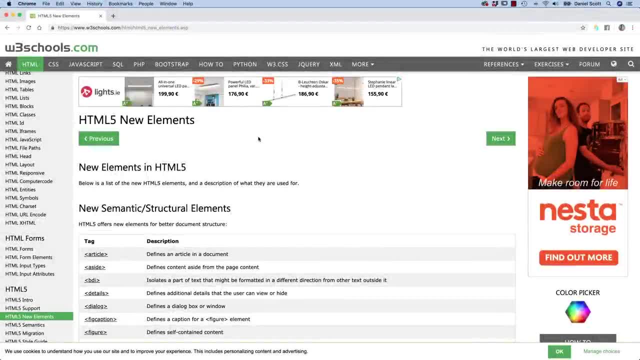 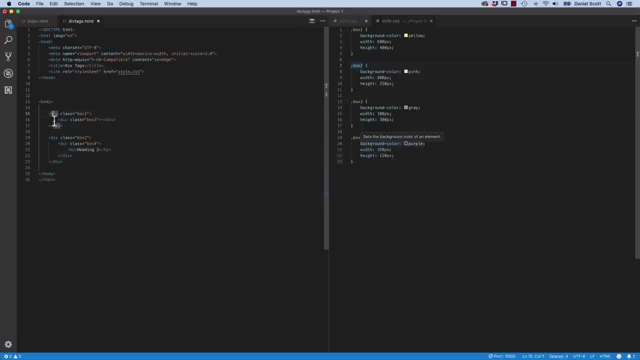 All right. so what are these HTML5 structural elements? Basically HTML4, what we used to do is what we've done up until now. We just make a div tag, remember a division of space. it's kind of a box. 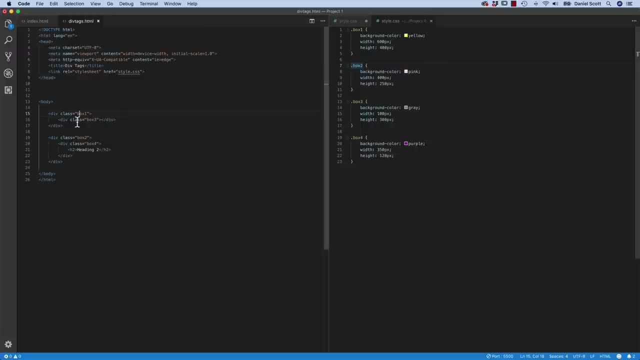 and we'd give it a class name and then style it over here on our CSS and that works fine. We'd have a box at the top for our heading and a box for our navigation, a box for the main parts, a box for the footer. 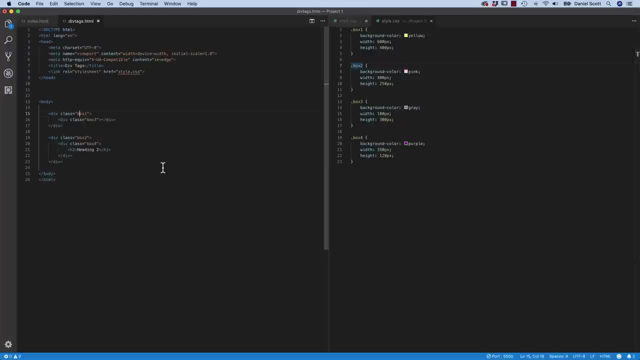 and we just create all these divs with all these names over here. So what they decided in HTML5 is like: hey, we're reusing these things. wouldn't it be nice to have an actual tag? instead of writing div equals blah, blah, blah, you just write nav. 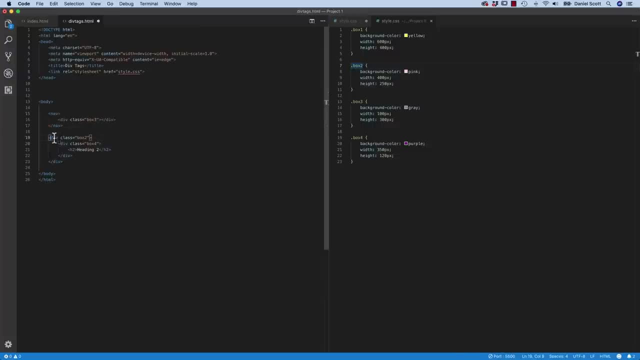 And at the end we're going to close the nav. Same with this one here. maybe this is the main part of our content. We'll just call it main Over here. call it main, Spell it right And over here style the word main. 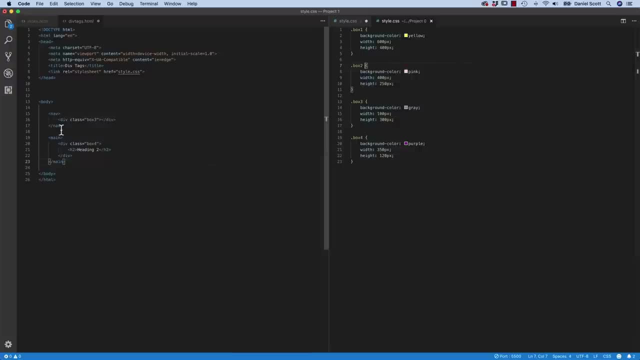 So that's what it is. They're just replacing some commonly used div tags with some pre-existing names. Now, other than that, there's not a lot of difference between divs and these kind of predefined names. They're just ready to go. 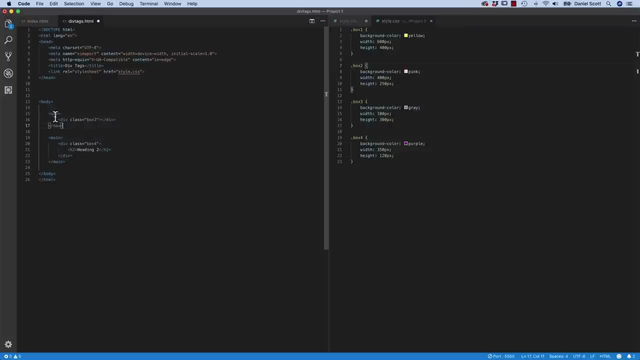 There must be some accessibility options for like screen readers that might use these types of tags. I'll have to do a bit more research in that It's never come up in my work, So I'm going to undo this because I'm wrecking this document. 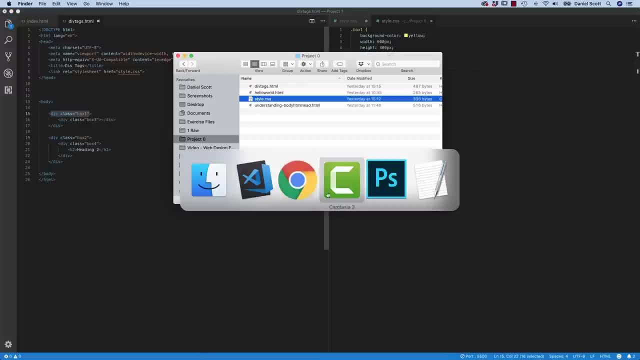 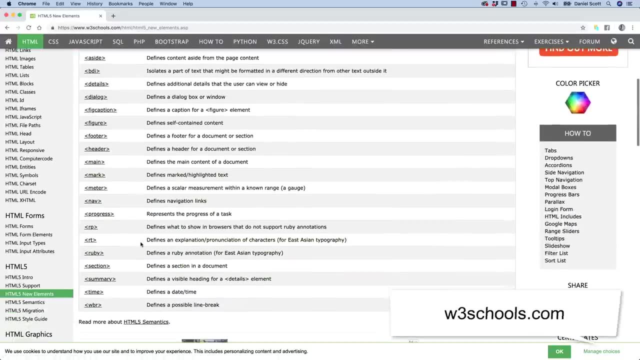 So what are these tags? There are some main ones. they're all kind of suggestions. So I'm at w3schoolscom and here's a bunch of the kind of new structural tags And there's basically just a couple of them that get used. 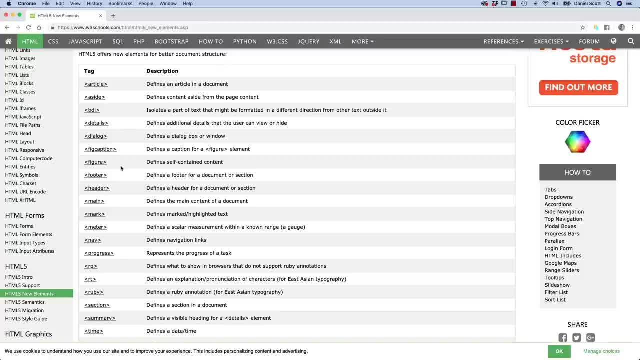 You should, if you're going to be like the best HTML5 implementer in the world- go through and research them all and use them all perfectly. What you'll find is that most people pick the good ones and there's a lot of confusion about some of where you should use some of these. 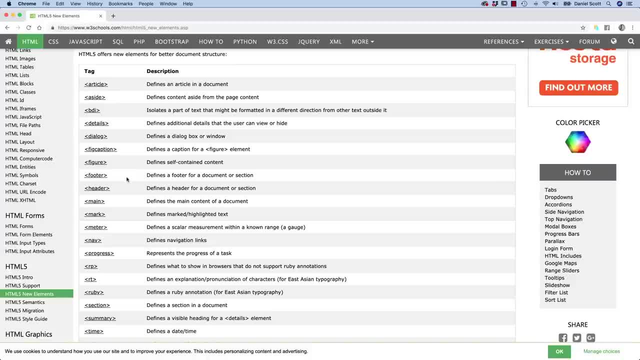 And because they're like pros and cons. well, the pros aren't huge for adding them, other than it's just a bit clearer. people don't use them. So I guess I want to be honest about that so that we're not. 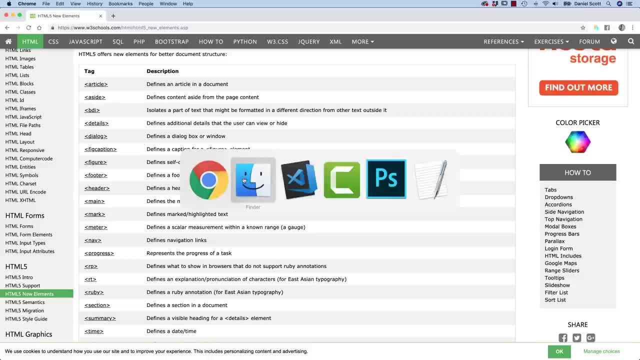 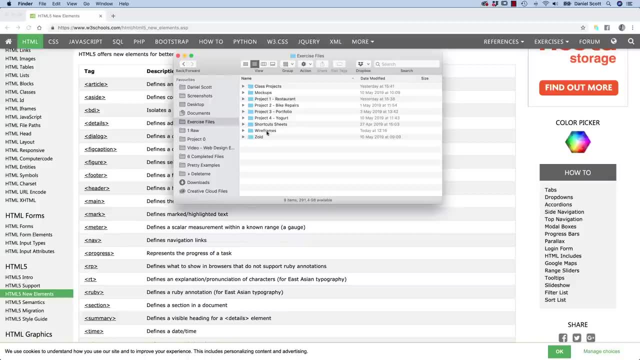 so I'm not telling you. you have to use these tags. Now. I made a little handy exercise file, a little drawing. Why am I drawing these? I don't know. I could use Illustrator, I don't know. I feel like it's proper if I go into wireframes. 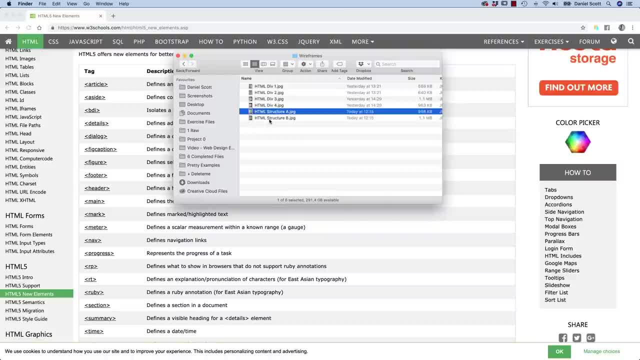 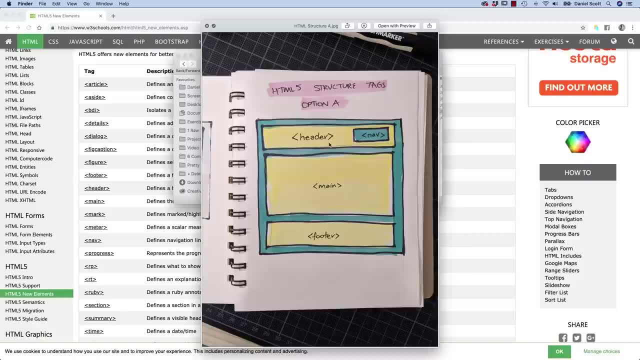 if you go into wireframes in your exercise file. I've made these two, So there's HTML Structure A and B And I'll show you two really common kind of uses of them. So instead of printing div header, we're just going to use the header tag, the nav. 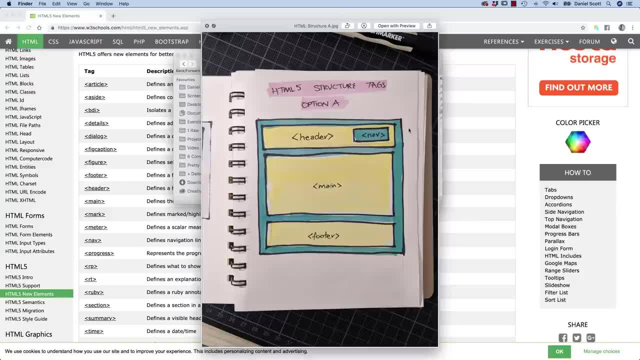 This is what I normally do. I throw in a website. this outside box, the kind of green one, doesn't have a name. they should have just put one in called container, that everybody uses in web design, but they didn't. 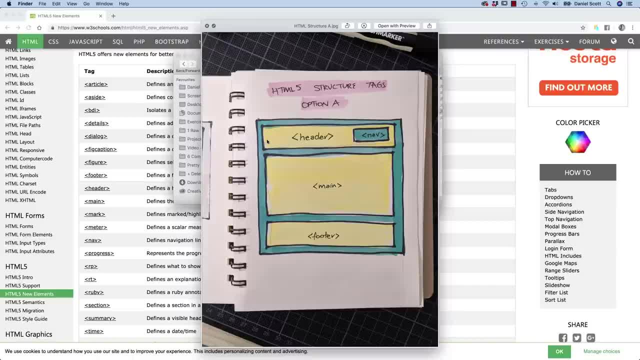 So there's no name for this outside one. we have to give it a div name. But inside of here I often put my header. inside of that header I put my logo over here. There's no specific HTML tag for logo. 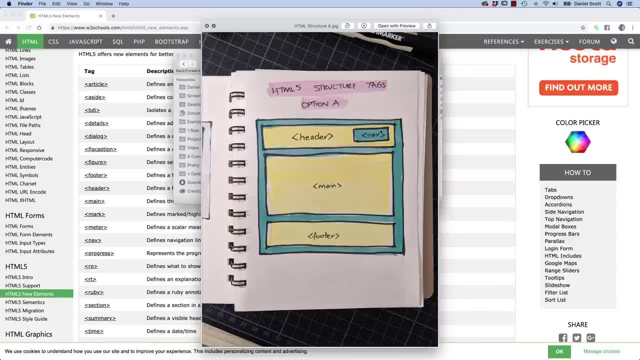 so you'll put that in as a separate element. but there is a nav, So I put the nav in there. often in the top right There's a big section in the middle. I call it the main. Well, I call it the main. it's actually a predefined 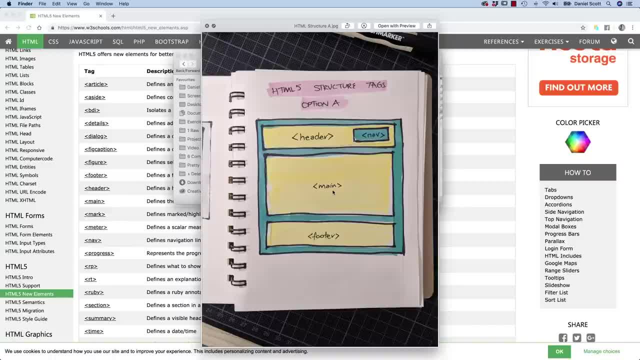 you can kind of see it over here. it's actually a predefined HTML5 tag. The way I think about main is that that one doesn't get used very often. I'm like, why wouldn't you Such a good explanation of what this area is? but anyway, 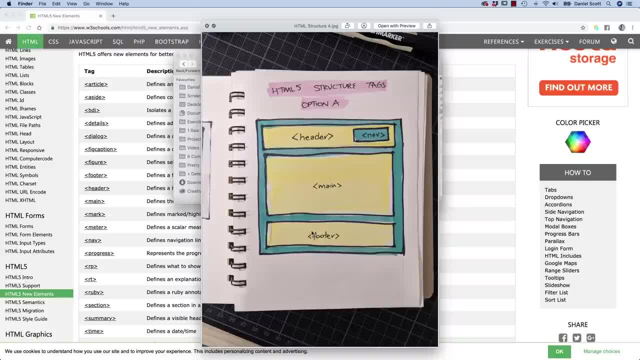 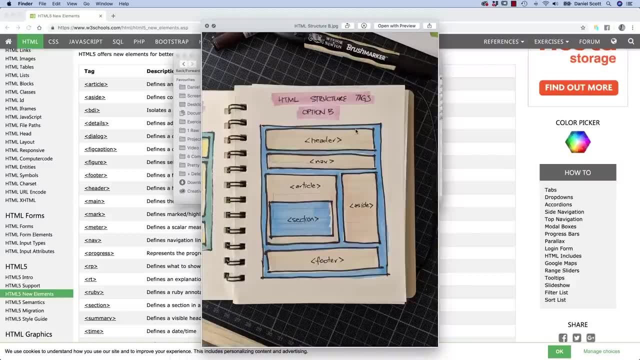 And footer is a really easy, really easy one. so that's what I do. I want to show you another way of working that I see a lot of other sites done. I guess I don't want you to all follow me perfectly, because there's different ways of doing it. 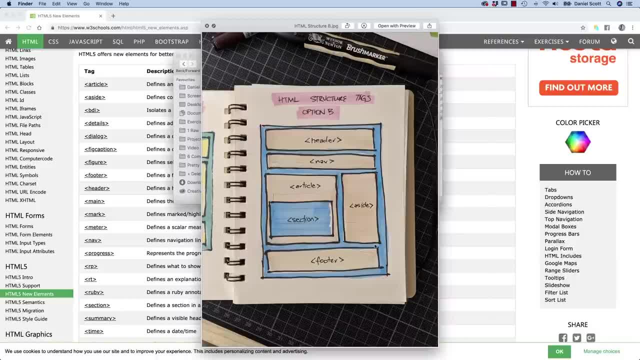 So again, the big blue thing around the outside is doesn't have a specific name. we'll give it a name in a second- but header. So I wanted to show you this one as well, because the nav doesn't have to be inside the header to work. 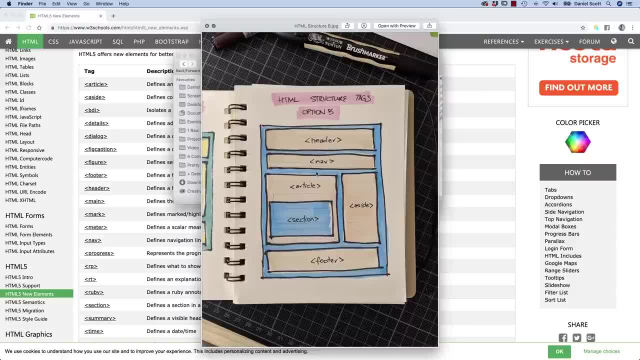 You could have the header. they could have your logo and some graphics. I don't know what's going up there, but you can have your navigation separately. Your navigation could be down the side, though nobody does that anymore. Then you've got your footer. we've already talked about. 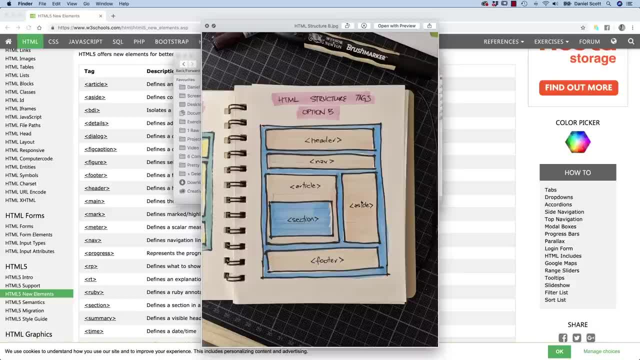 You've got these three. these are common enough. And aside is pretty easy. If you've got a web design where you've got a sidebar or something- often it's like related articles or latest Twitter feeds- you can have this. you can put it inside a div tag called aside. 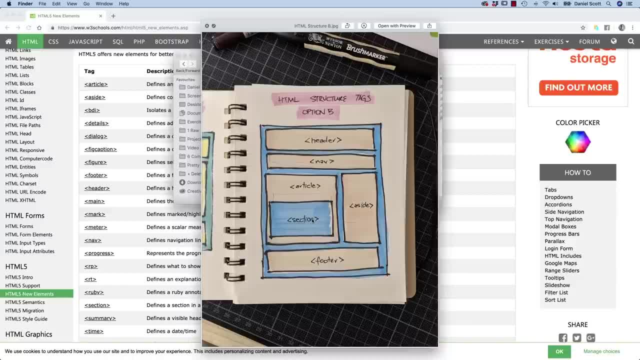 That's clear. great, These two are the ones that are real confusing. So this is how I interpret how it was set out. So you have an article and it's unique to that page. it might be a blog post, it might be you're writing about a topic. 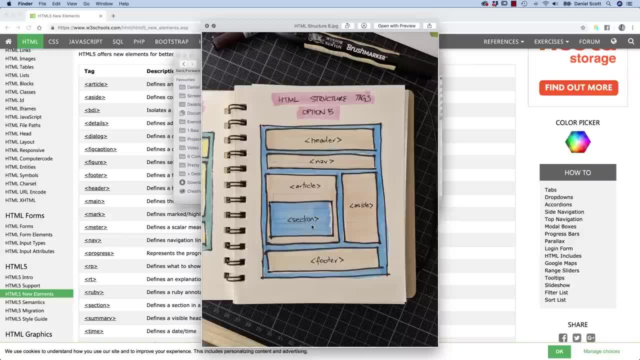 and then within that article you have sections. You might have a main kind of article but you might have some bullet points or like little FAQs or kind of pull quotey extra bits. You might have 10 sections or two sections. 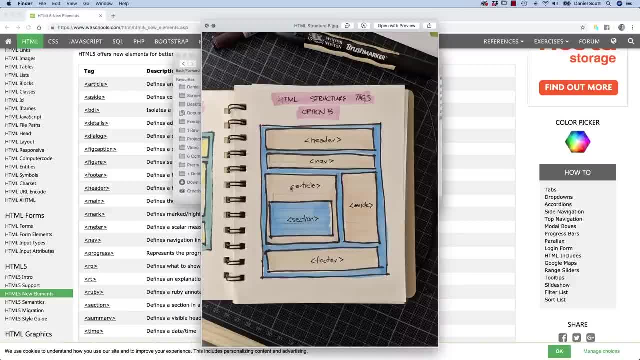 but you have a main article. There is arguments on sites where that can be completely the other way around. You have a section and you have articles within the section and you have multiple articles on it. on the page The documentation is not super clear. 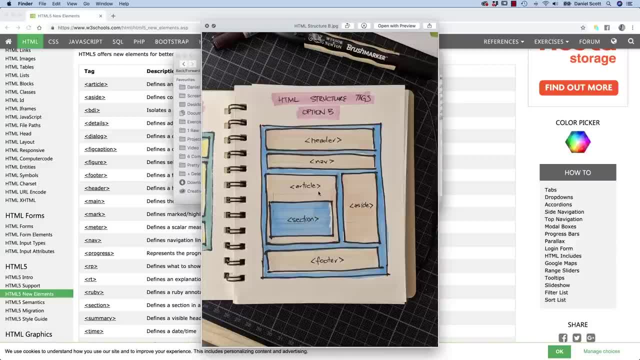 and I guess I wanted to share the unclearness, because you might get to one website where they're being very deliberate about using articles and then sections within the articles, and then you get to another site and they've implemented this article section thing completely different. 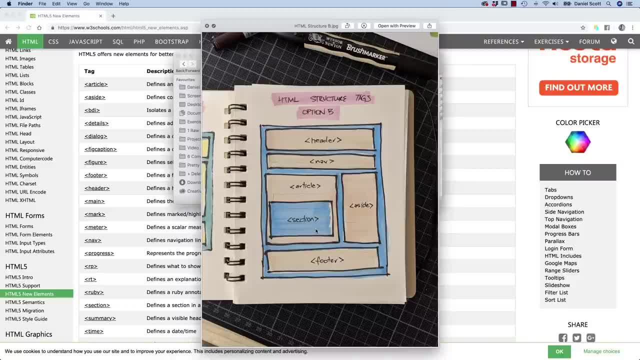 and you'll be like huh. So if that happens, if you get to the huh moment, it's not you, it's the internet. Clear, clear, clear, clear. weird, But a lot of people don't use main. that's why I didn't include it here. 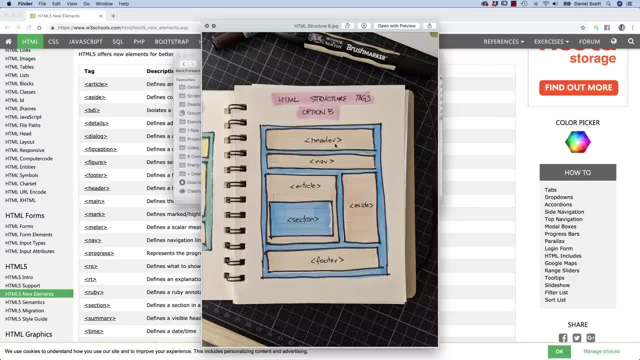 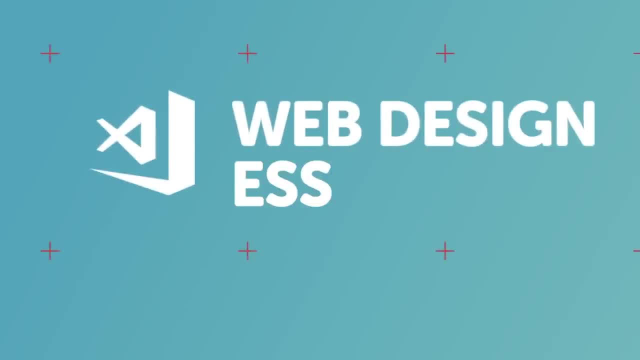 So we've learned what these kind of tags are: just replacements for divs with special names. We are going to go and start building our actual project structure in the next video. see you in a sec. Let's start actually making the website. 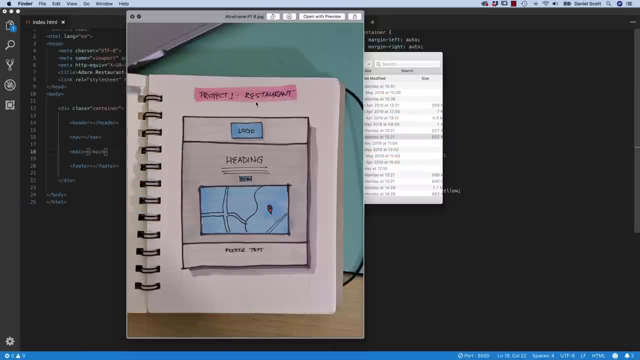 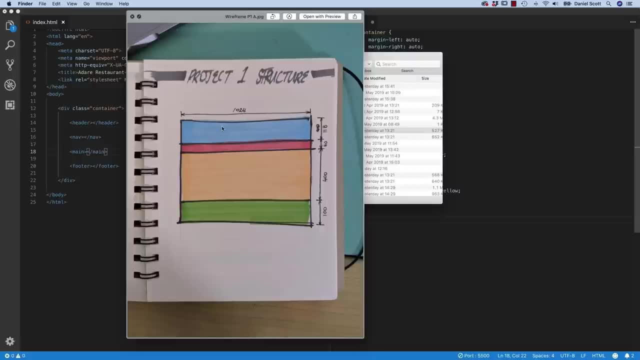 So our first project is going to be this restaurant. So we're going to put in the structure for it- the header, the main and the nav- And it's going to look something like this. It's going to be the kind of main structure that we're building in this video. 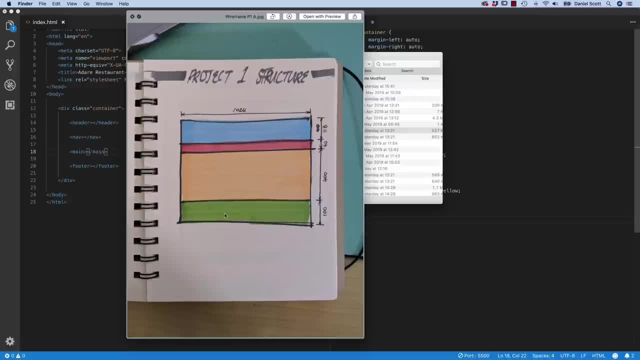 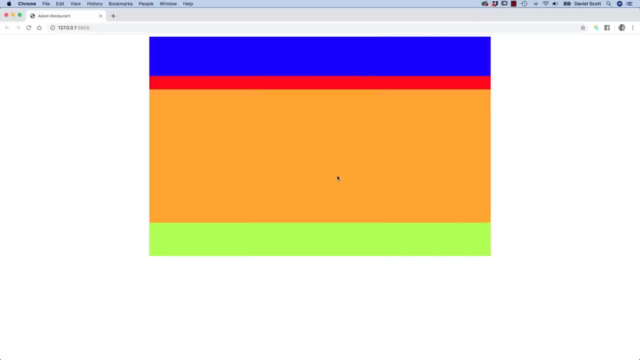 So header, nav, main footer- easy, Let's make it, and that's what it looks like, and we'll center it as well. That's the job of this video. Let's start coding. All right, depending on how well you've been following along. 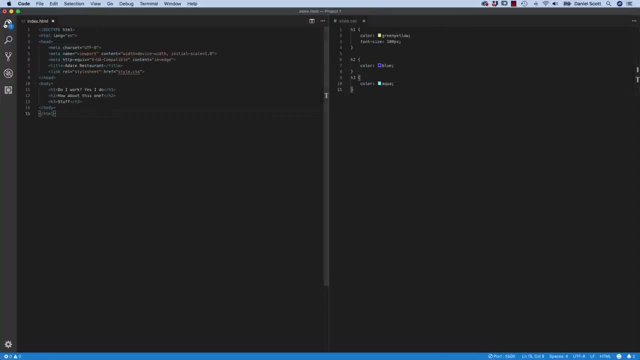 I'm going to close down everything in here, except for I'm going to open up my Explorer. I'm in Project 1. and I've got Index and Style open, So make sure those are open. Now in the Style CSS, let's delete all the code we've got so far. 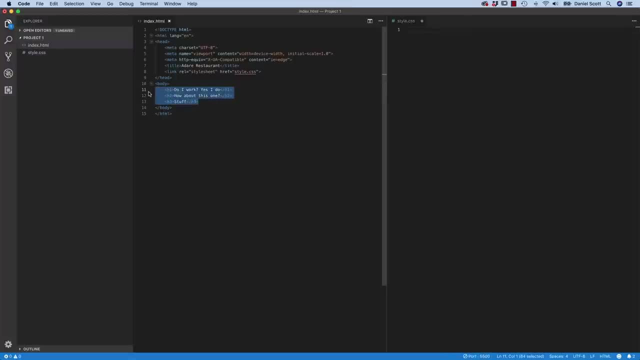 and clean it out, And same in here. let's get rid of all of the body, So that's nice and clean. Put a few returns in, because we're crazy and we need lots of space. Make sure that your Style Sheet is linked and the title. 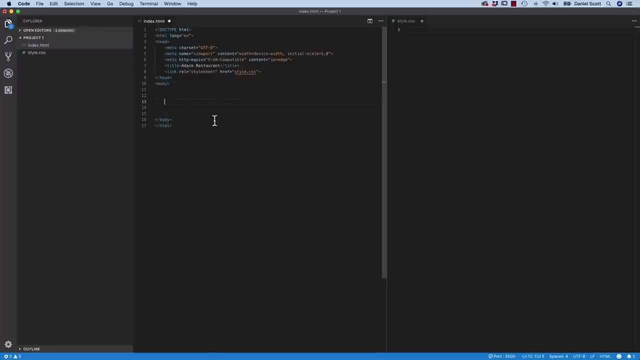 You've got a title, any kind of title. What I also want to do before I move on is I'm going to close down the Explorer. I keep meaning to do it in every video, but let's do it now. Let's go to View. 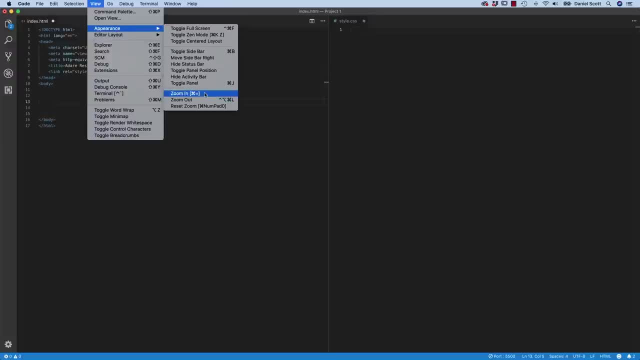 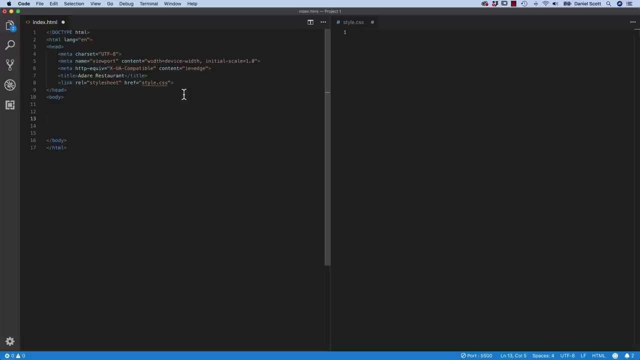 Now I'm probably just going to do this. We're going to go to View Appearance and see Zoom In. You'll see if you want to do it in a sec. watch. See all the text got a bit bigger. It's probably to help- mainly to help the editor- from zooming around. 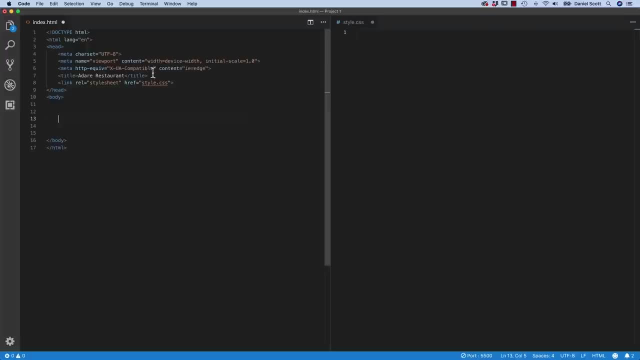 You're probably getting dizzy as well, going side to side checking CSS and HTML. So I made the text a bit bigger. You might be the same. you might be like I wear glasses and I need to make this stuff bigger. 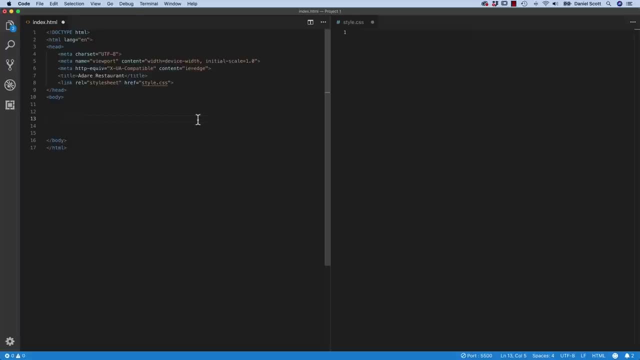 So View Appearance and you can Zoom In. So you're reset, we're ready to go. What did you get in the frame of mind? Let's say we've woken up, we've got to our desk, we've got our coffee. 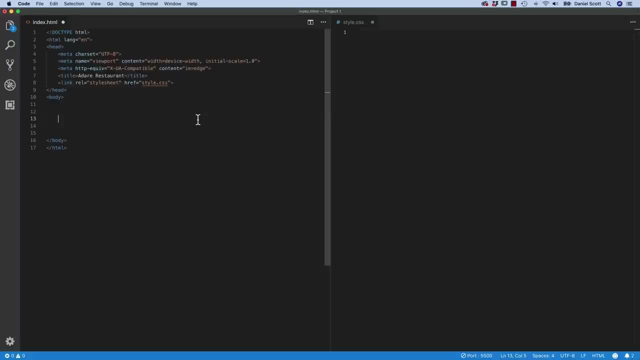 and we're like: okay, we need to make a website for this Adair Restaurant Company. We've created our local folder, which is called Project 1.. and we've created two files: index and CSS. We've added our title and that's all we've done. 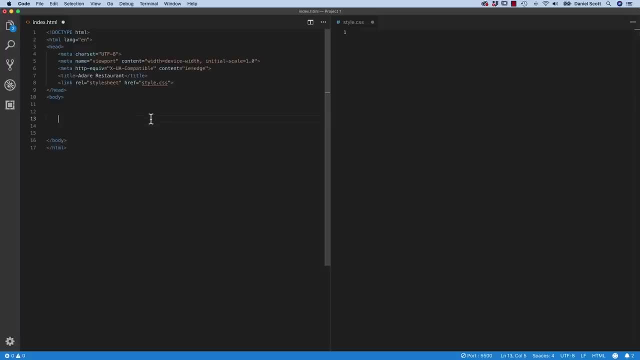 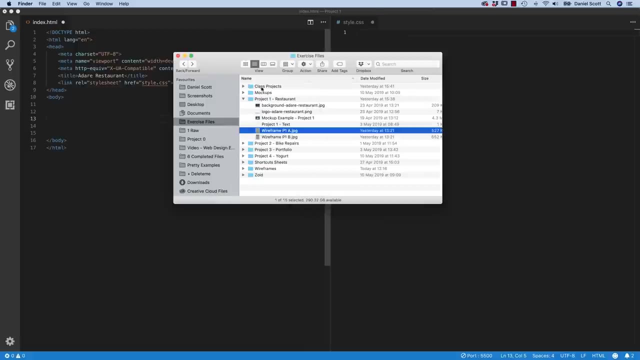 Actually, we've connected the stylecss, so you're ready. Next thing I want to do is start adding my HTML5 structure tags. Now we're going to work off a diagram that I've hand-drawn for you. It is in Project 1, on your exercise files. 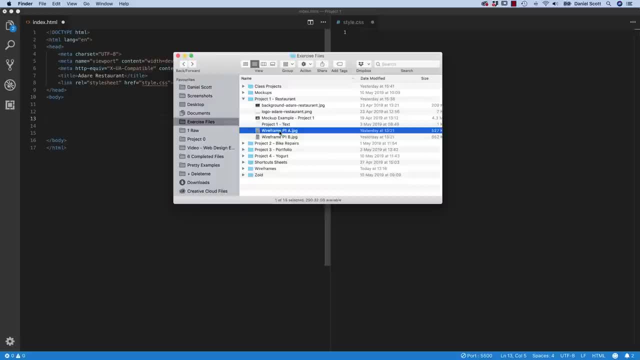 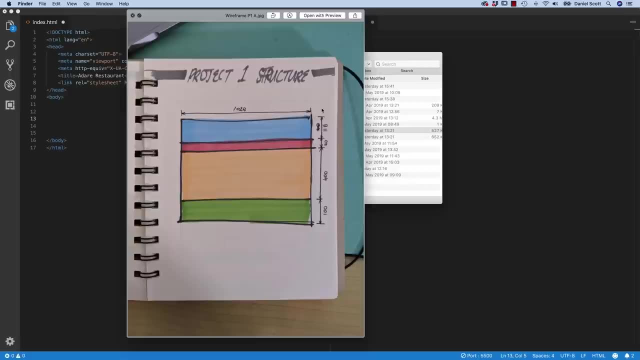 and it's called this one wireframe P1A. So if you want to have that open on your other screen, like I am, I'm going to put it over there Just to kind of work out the sizes and the colors and stuff. 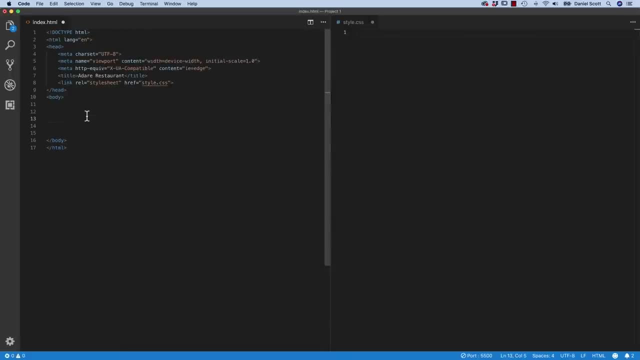 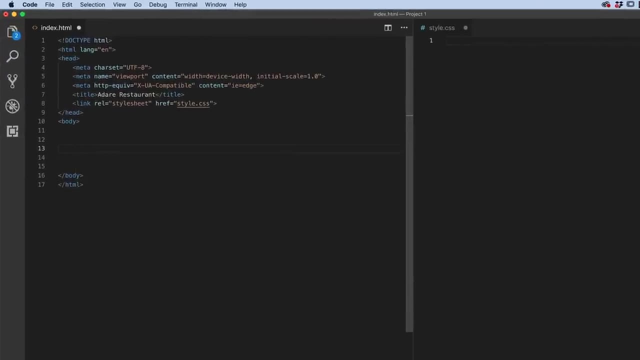 You don't need it. I drew it anyway. So we're going to need our first one, and the first one is header. So instead of writing div equals header, we're going to just write. actually, we don't even need the angle brackets anymore. 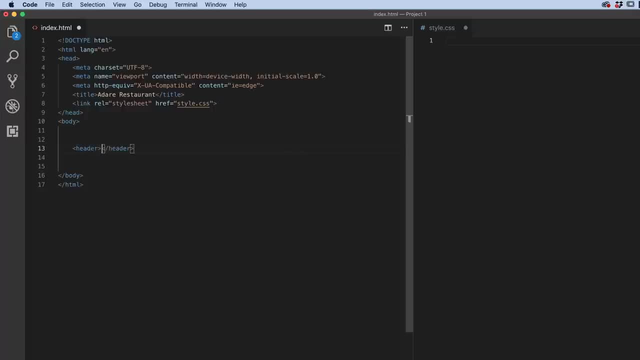 remember. we're using new tricks, so we're going to type header There. it is there, Put a return in. so there's a bit of space, because I like space between the tags. Now we're going to style it Over here in my CSS. the difference between what we're doing now. 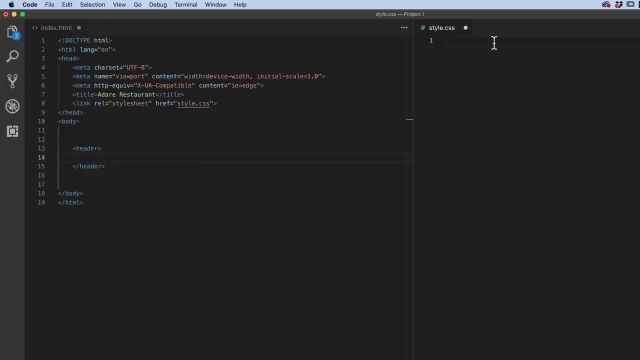 and what we did before is we put. when we write a class, we have to put what's the thing that goes into the front. It's that period or full stop. then we write header. But this isn't a class. you know it's a class. 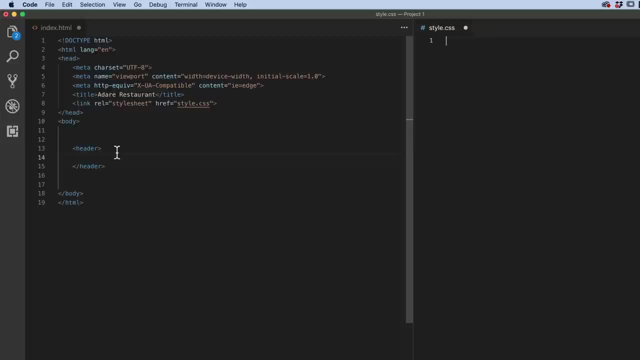 because remember we write over here: div equals class. it's very clear. When it's not a class, it's just a plain old tag. there's no class in front of it. we don't have to put that period. So you only put that dot if it's a class. 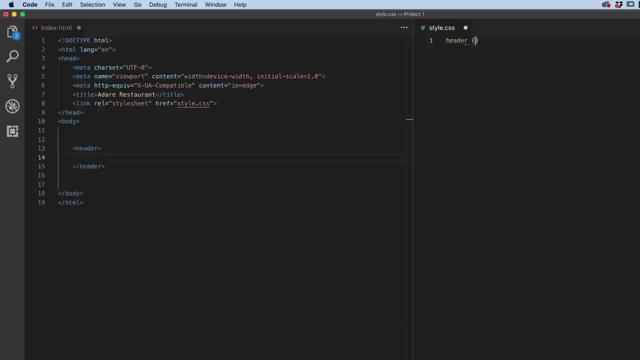 This one we don't have to header awesome. Then we put in our curly braces and we're going to style it. Now, like before, we're going to kind of open ours out to be a clear box, but often you wouldn't give it a background color. 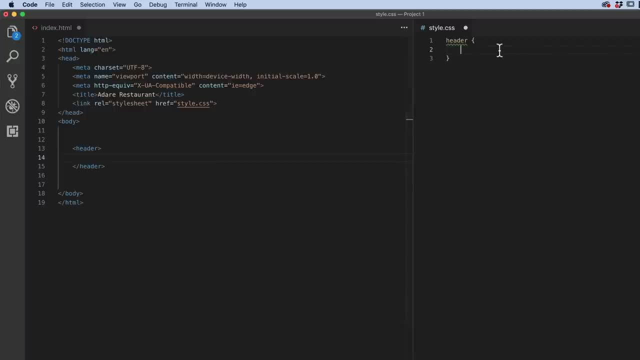 and a height, like we are in that kind of diagram that I showed you, because you let the logo and all the text kind of fill the gap. But we'll put the structure in first, then we'll delete things like the height and the background color. 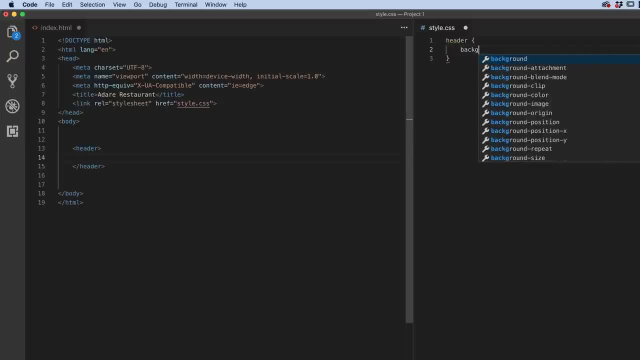 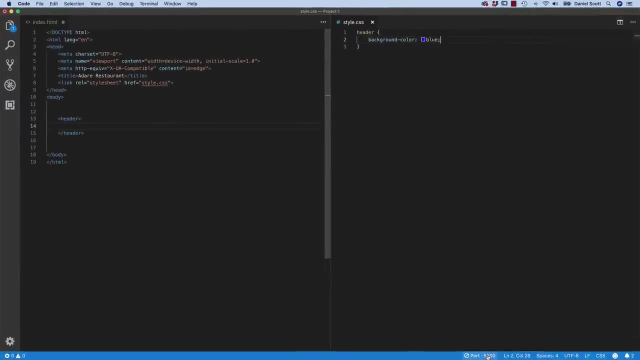 So first up header you, my friend, get a background hyphen color. there you are. We're going to use blue for this one, we're going to hit save And we're going to go and launch our cool little live preview thing. 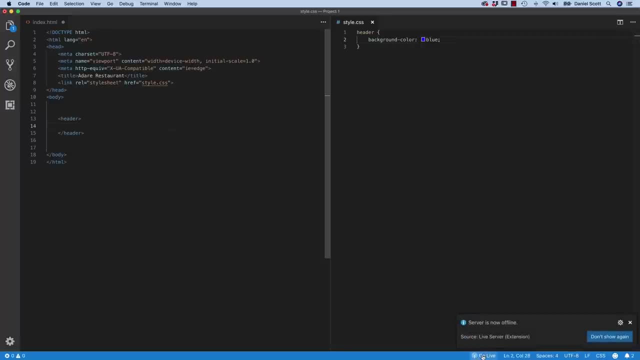 Actually mine's still going from last time. Go live, Start it back up. There it is there, And great blue background. Why can't we see it? Because it has no height, So we either put content in it, which you'd normally do. 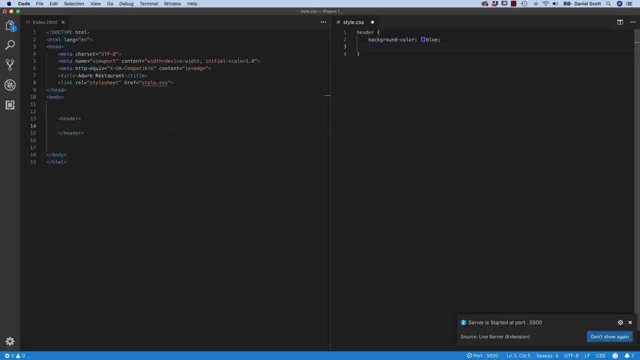 but because we're not doing content, we're kind of separating this all out into separate videos so that we can get our kind of knowledge going first. So we're going to have a height of 118 pixels. Just that's what I decided. for no good reason. 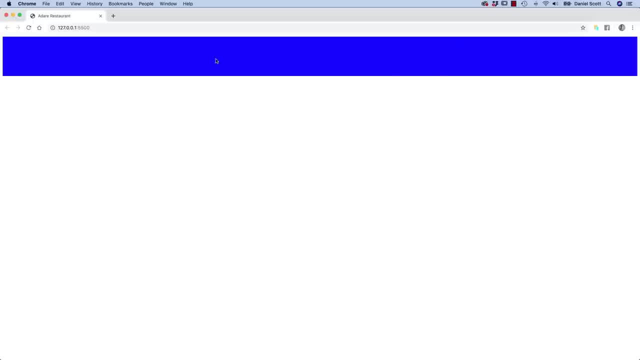 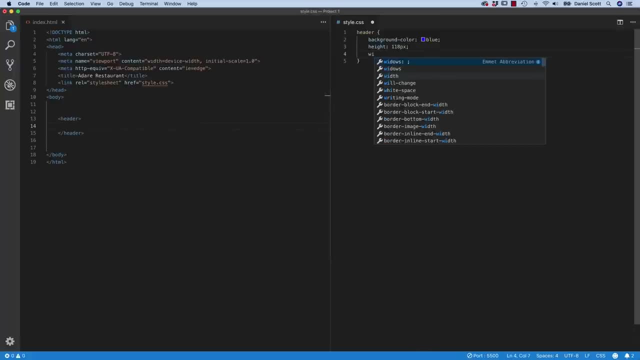 Now let's go and preview. there we go. Now. I like to give it a width, because stretching all the way across it might be what you want, but for the moment we want it to be nice Physical width. So how wide should you make your website? 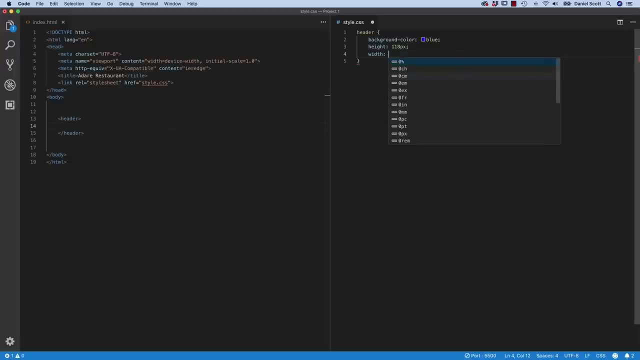 So this part of our course, we'll give it a physical width. So we'll say: you need to be a certain width. Later on we'll get it to adapt or respond. So when we get into a section about responsive design, 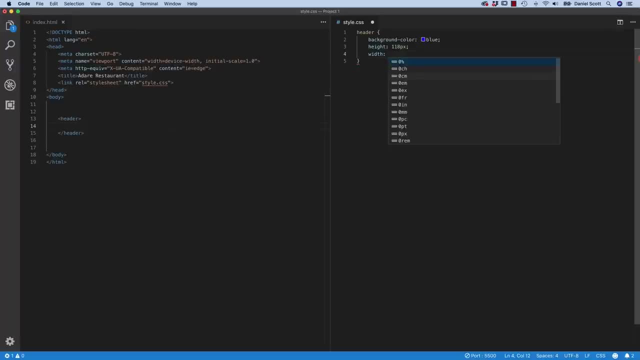 we'll get it to respond to different sizes, But at the moment we're just going to target like a standard laptop size And basically your width can be anything. It's up to you what you think the width should be. But you're new so you need some sort of guidance. 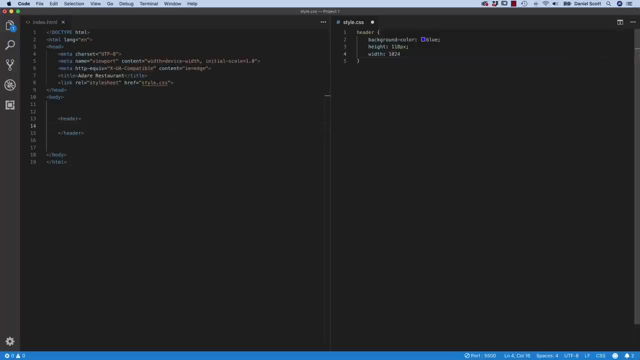 So often, I'll make mine 1024 pixels wide. That is a really kind of common generic web width. It fits on like laptops by default are about 1300 across, So 1300.. So as long as it's less than that. 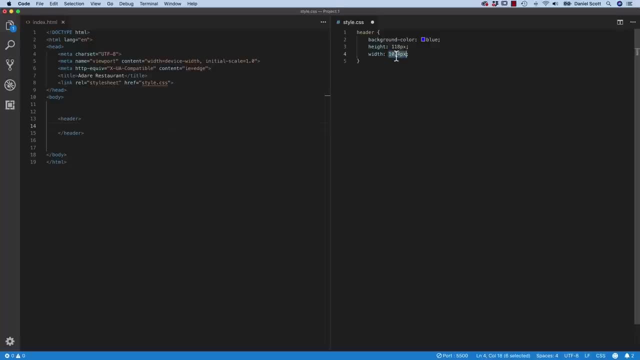 it will fit on most screens. Other really common sizes are 960.. It gets used quite a bit because it's- we'll look at this later on- but it's easily divisible by 12. Which doesn't make any sense now, but it will later on. 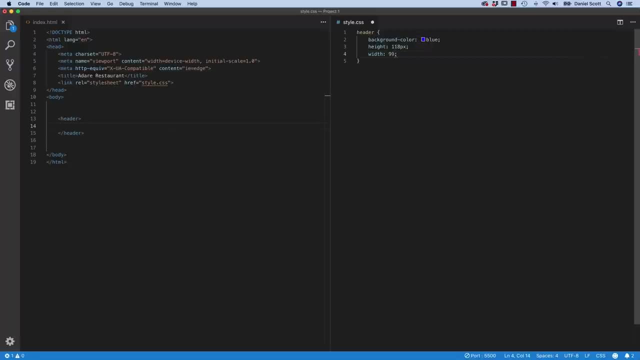 It's the columns that we're going to use later on. Bootstrap, which we'll look at later on as well, uses 992.. It's a framework that we'll look at, But don't worry too much, It can be Mesh Keyboard. 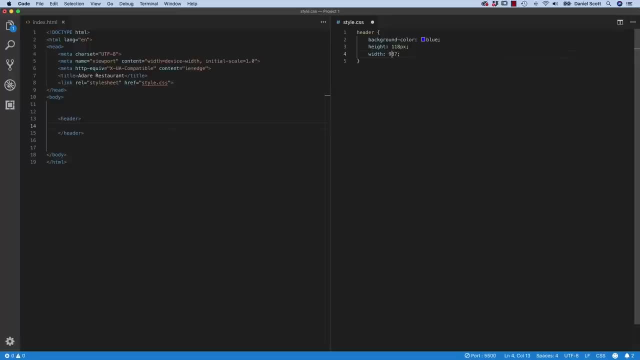 It's going to be a pretty small website, that one, But if I made it 8., 9,, 8,, 7,, nobody would care. it wouldn't break the browser As long as it's smaller than a laptop screen. we're going to use 1024.. 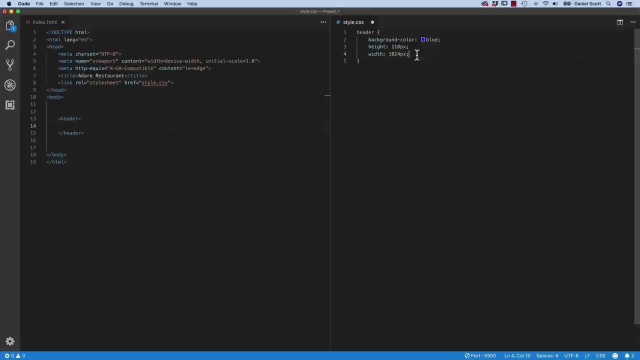 The other thing is you've got to say 1024.. If you're at a web design group meeting and you start talking about 1024.. they're going to know that you are a newbie. You've got to say 1024.. 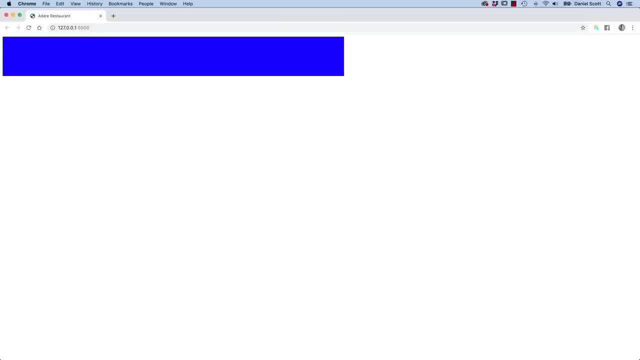 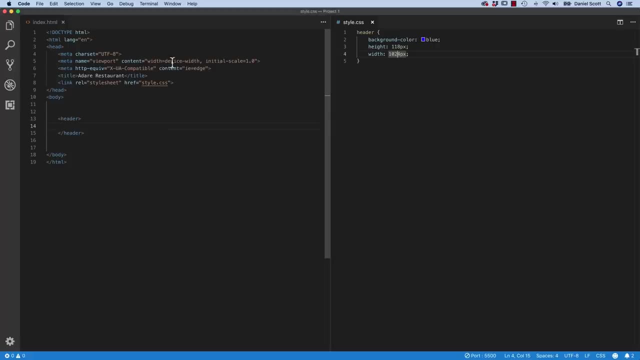 Let's save it and let's check it out. Browser cool 1024, fits on my giant screen, But it will fit on smaller screens. it's got a height and it's background blue. And the main important thing is we used header instead of naming it a div. 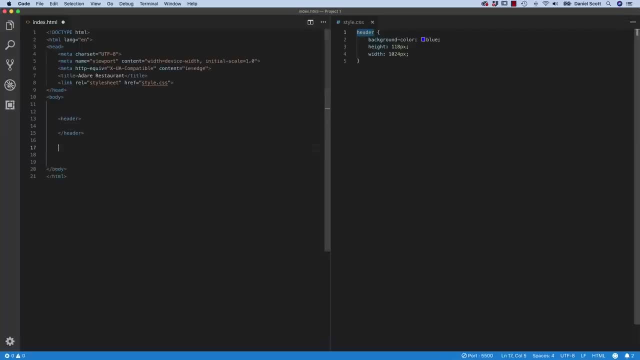 giving it a class and styling it over here. So the next one: a couple of spaces. I'm going to type in nav. So nav hit return space. there we go. I'm going to do the same over here. 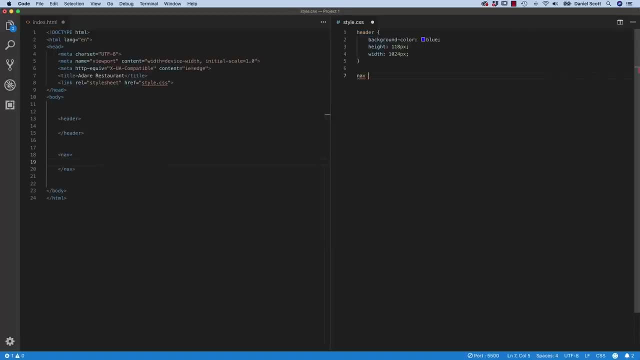 Remember leaving that curly brace there. I'm going to type in: nav doesn't need a full stop in front of it, And we're going to add a background color. we're going to cheat Because it's already typed up the top there. 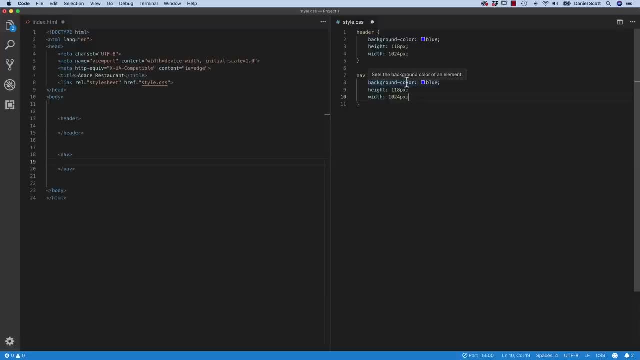 Background colors you'll get used to. That's a really long one to type to get the right suggestion. I hate that one. It's just a long group of characters anyway, So let's check our diagram. Where is my little diagram? 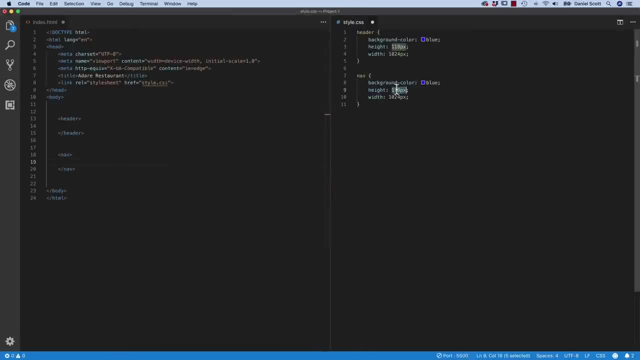 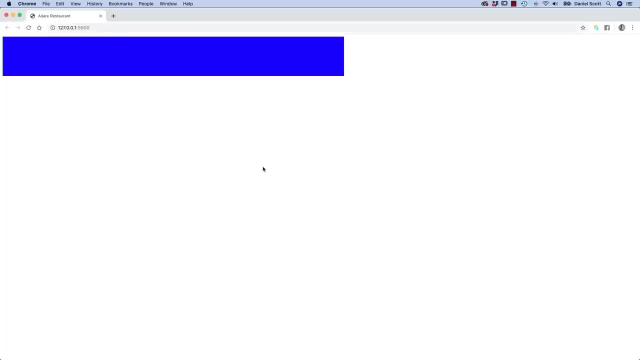 He's going to be 40 high. we'll use the same width, but we'll use the height of 40. Now, this happens quite a bit. I do it and I forget to put the PX back in What happens in the browser? Let's just check. didn't appear. 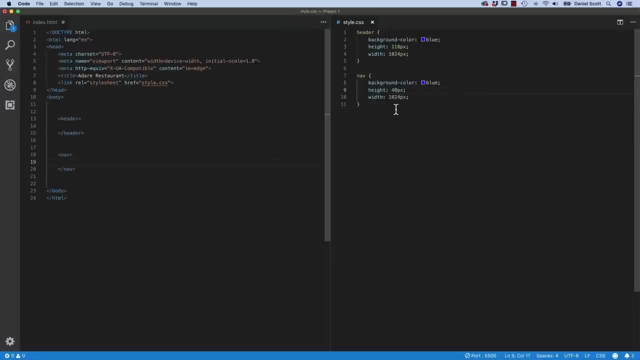 Save Still didn't appear. why You can see it? It's because it's blue. Come on, Dan. it's meant to be red. It was there the whole time. Still not there? Come on browser. So it's meant to do automatically updating. why is it not? 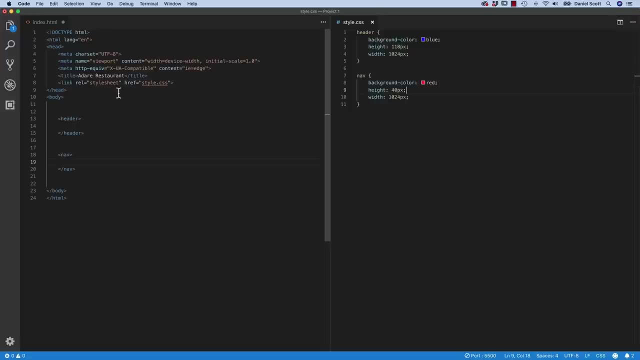 Oh, you know why? It's because I didn't save this site. I'm hitting Command S. it's Control S on a PC, So I'm hitting save, but I'm only in this document, Out of the habit this morning of hitting Command Alt S. 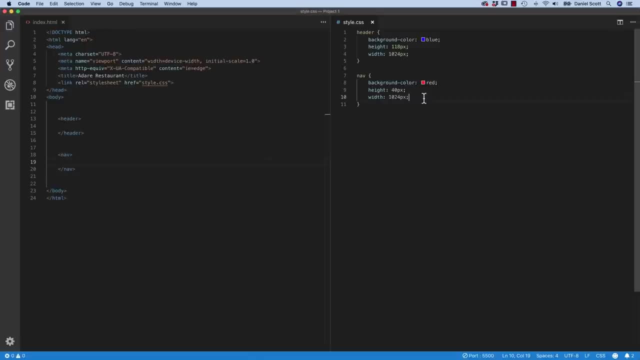 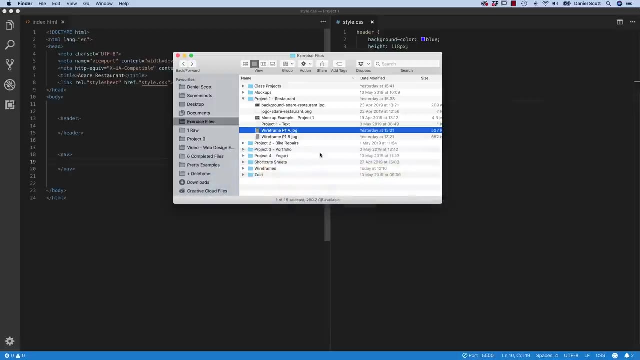 which saves both sides. then it appears- I pretend lesson that I'm teaching you, but really I just messed up. So there's a nav. what else we got to do? We've got this section here which is going to be my main. 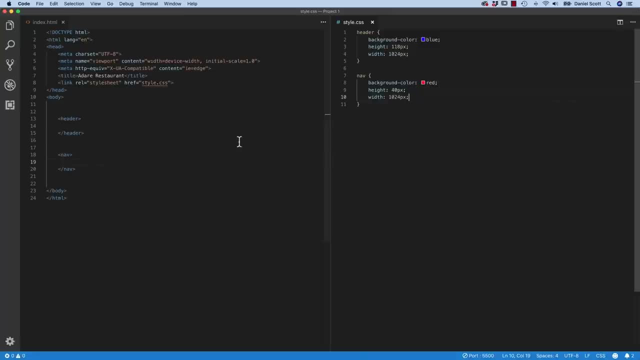 and this is going to be my footer: 400, 100, check it out. So over here I'm going to bulk them in, So I'm going to put in. no, I'm going to put in main Return. put some spaces between them so you can see. 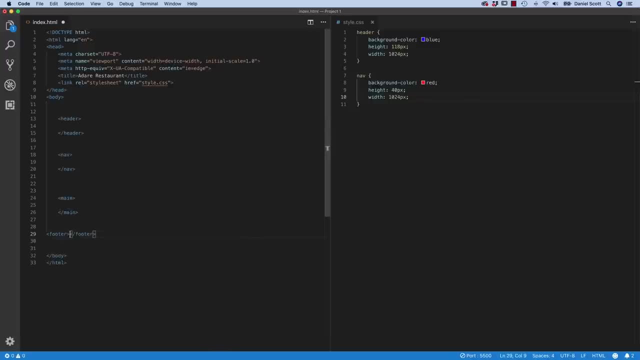 And down the bottom here we're going to put in footer. Now notice that I was kind of messing around with my cursor, so it's all kind of. I just put my cursor in front of it, hit Tab, so it all lines up. 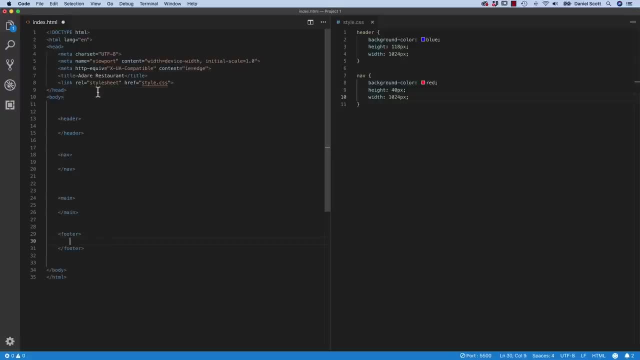 You don't have to do that And I'll put a return in it to look like all the rest of them. So there's my sections over here. I'm going to cheat paste that in that in. This one's going to be main, this one's going to be footer. 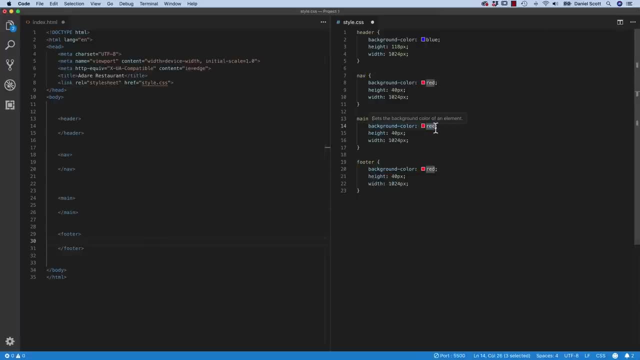 So we're doing lots of things one at a time, but often when you're working you're going to start kind of doing this a little bit more bulk kind of doing things. So orange, it doesn't have to be the colors. 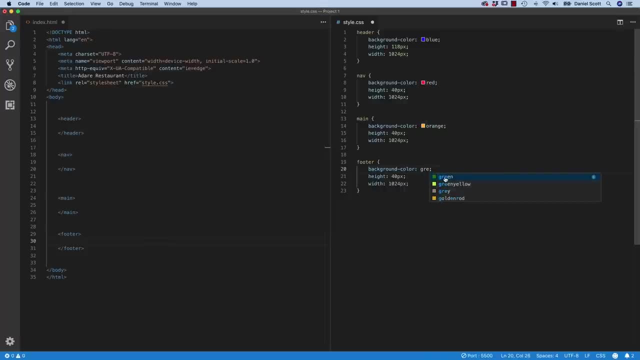 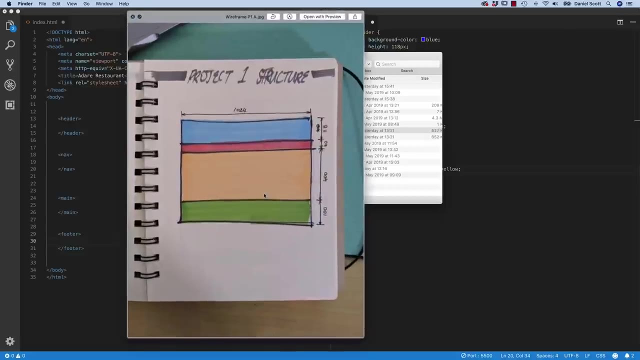 Like there's some random colors in here. we'll look at kind of more code-based colors later on, but I'm just using the ones that are pre-filled in. It was 400 and 100, I can't remember 400 and 100, it is. 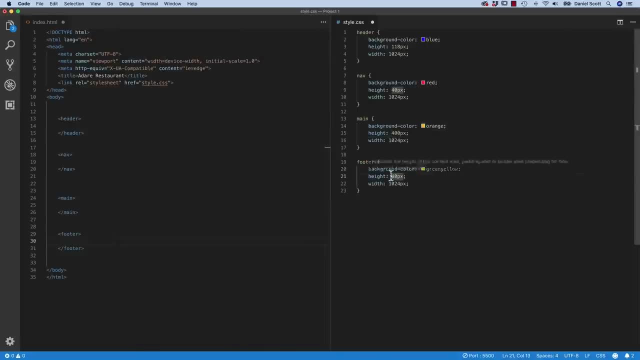 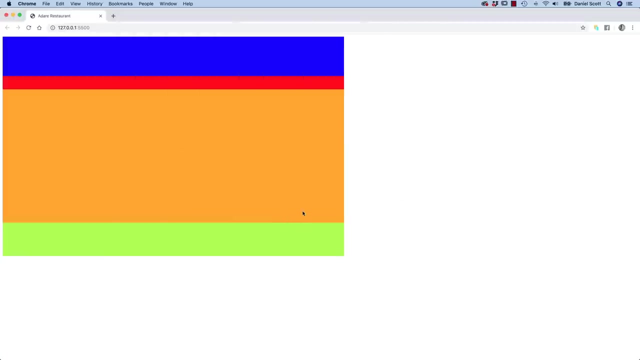 So height 400, and this is 100.. Get in the right spot, Dan, Save all and then go to your browser and there we go. It's the kind of core structure Now, the big thing you're like. I want it centered. 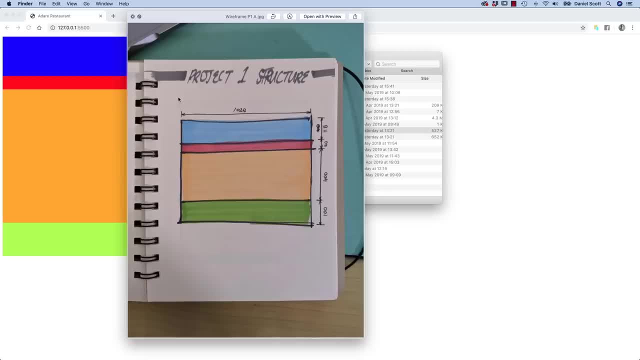 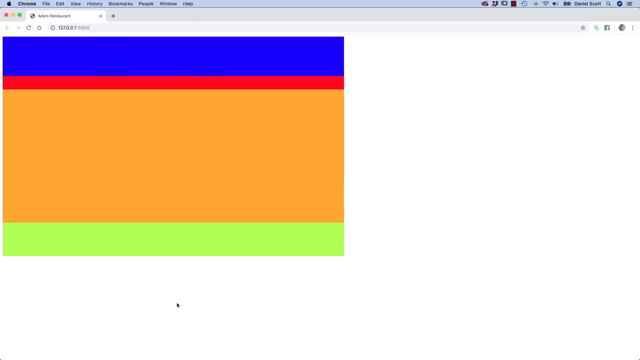 Why isn't he centering it? Let's do that one next. So what we can do is we could try and center every single one of these boxes and that would work, but what's really common is to wrap it all up in a div. 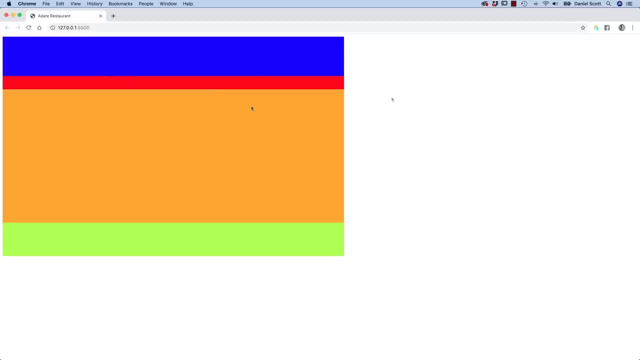 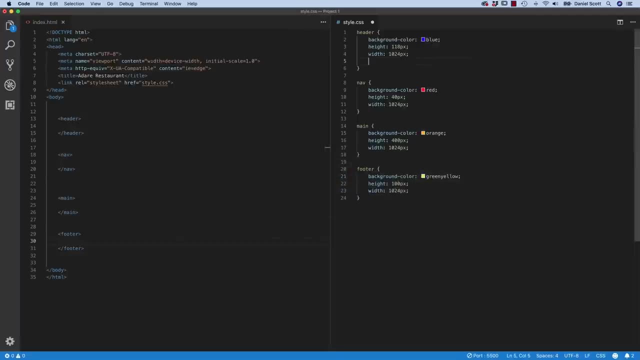 or in a container and make that centered so that these guys come along. Actually it's easier just to show you. So in VS Code we are going to go in here and say the header, So to center something. it's kind of weird. 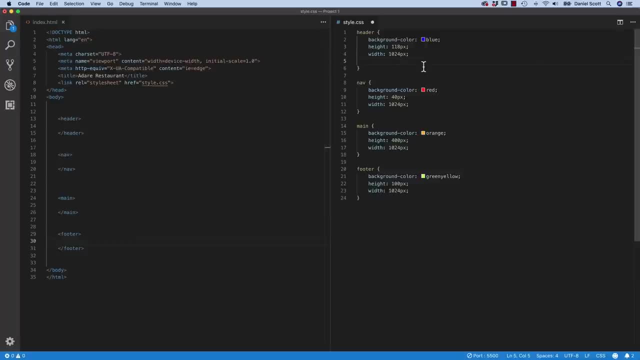 To center kind of a structural element like this, and there's no like make me centered. So it's kind of weird, It's kind of a trick. it's the way it gets done anyway. So there is so you can put in a margin. 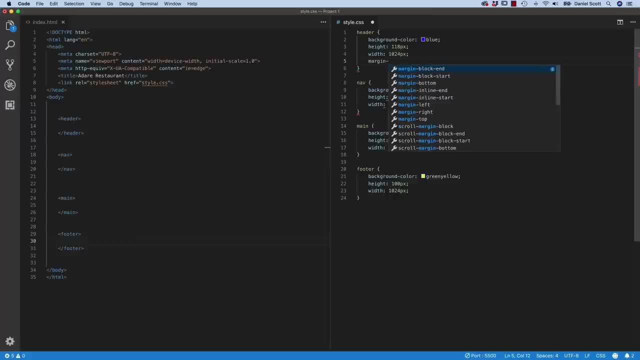 which is the space around the outside. but you can put a margin on the left. I'm going to click on that one- And instead of putting in an actual measurement, you can just type in auto make sure semi-colon goes at the end. 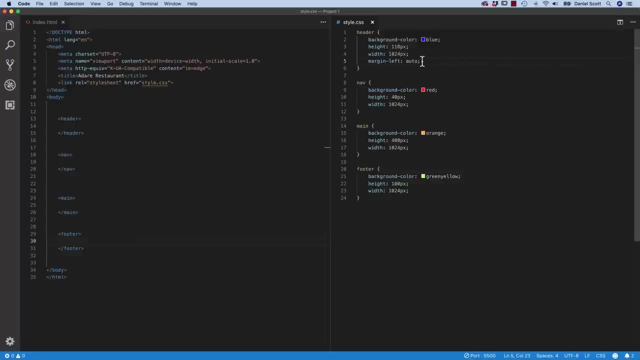 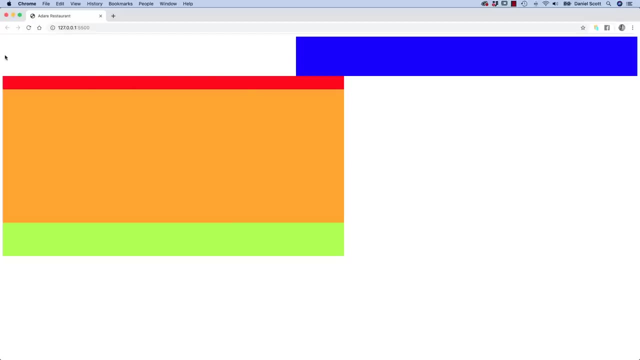 So syntax has to be like that. I'm going to hit save. What that does is: let's have a little look at the website. Can you see? I've done it to the header because the margin is automatic. it tries to be automatically as much as it can be. 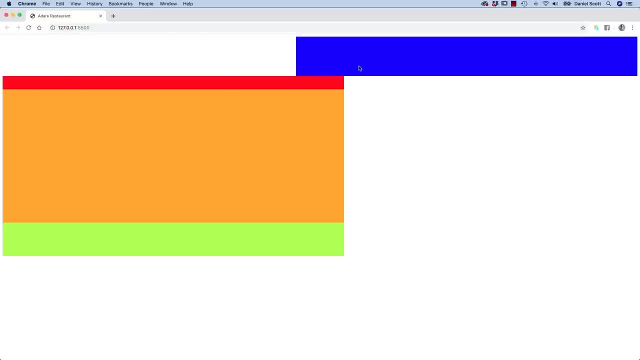 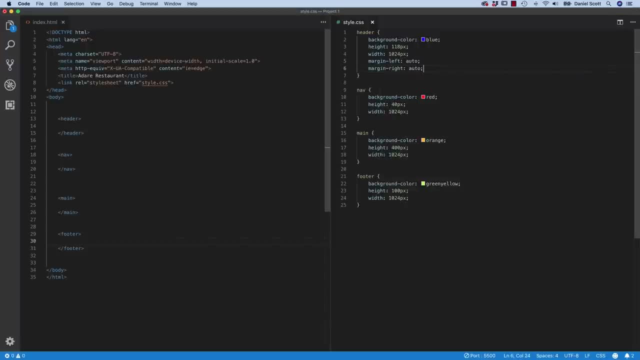 And so it just says, well, I can be as big, I can be massive, so it goes massive. To counteract that, you say I want a margin on the right. So the exact same thing and they battle it out. 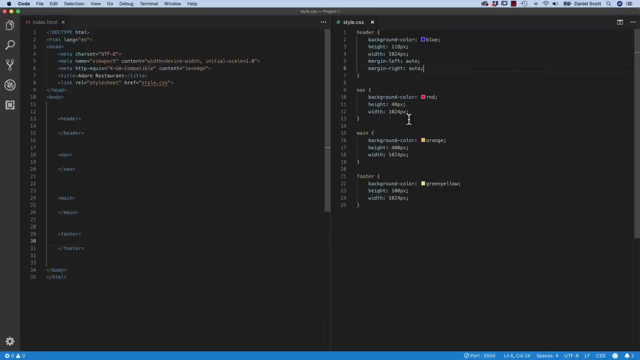 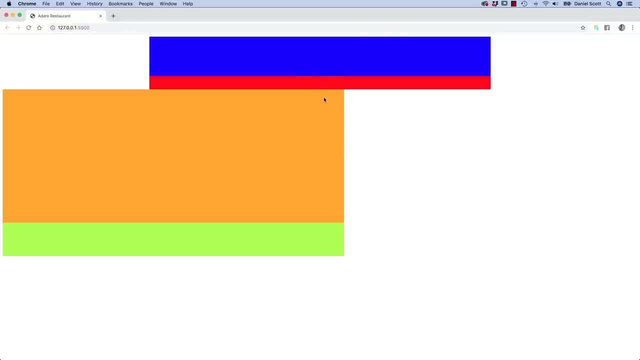 and somehow, magically, they end up in the middle. So that's how you center things. So we could do it for this and we could do it for this one as well. You could slowly work your way through it and there wouldn't be any technically problem with that. 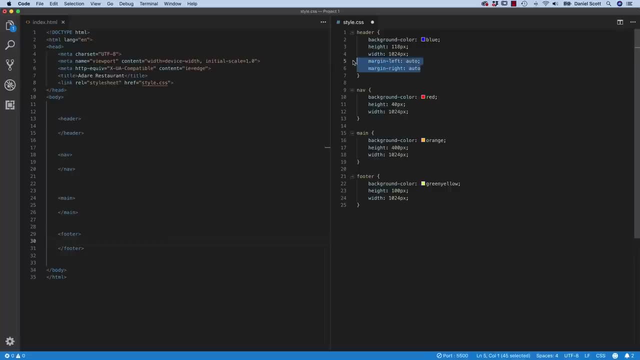 except it just be a bit weird. So I'm going to grab all of this, get rid of it, Save it, so we're back to here And I'm going to put all of that stuff into a container. Now there is no container like predefined tags. 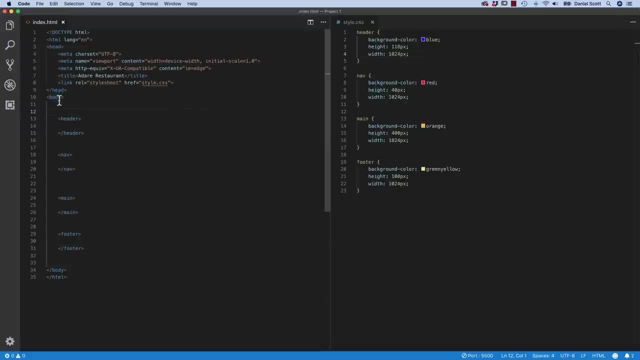 We have to use our old school div tag, So at the top here. so I want it to be before the header and I want it to close just after the footer. So here I'm going to tab out once and I'm going to say: 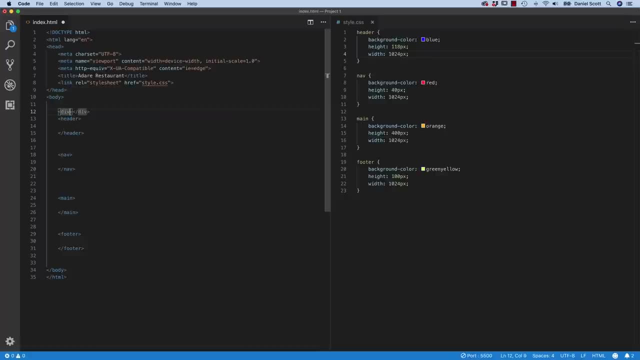 I would like a div with a class of container. Now I'm calling it container. you could call it binomial Banana, you can call it anything you like. Some people call it. nobody calls it banana. just in case People call it a wrapper, it might be box. 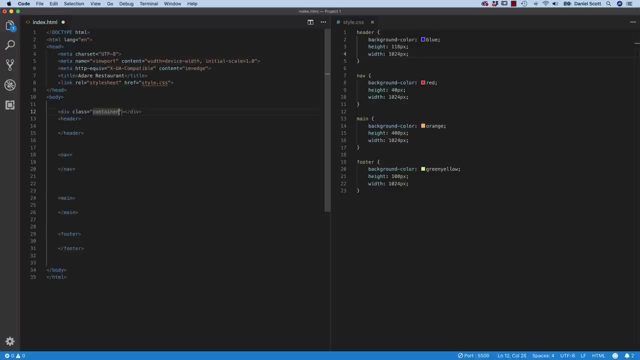 We're going to call it container, for that'd be a really common one, this container. So I've styled that. the problem is it opens here and closes just here, so it opens and closes straight away. I need the ending of this. 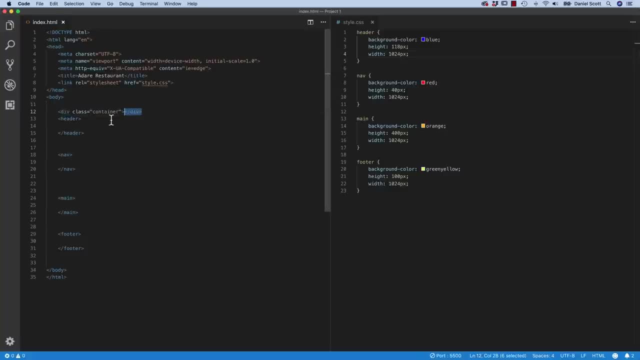 We did this kind of playing with our div tag box thing earlier on. That's the reason we did it. it's because I need this. I need to cut it, Grab all the little bits and pieces and after Footer finishes, I'm going to paste it in. 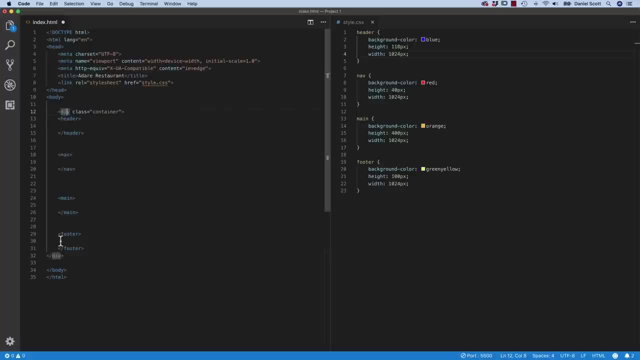 So now, if I click on this top one here, it opens there, closes there, so they're all wrapped up. Let's tidy it up, because it's looking a bit weird. We're going to do this. I've selected all of this. 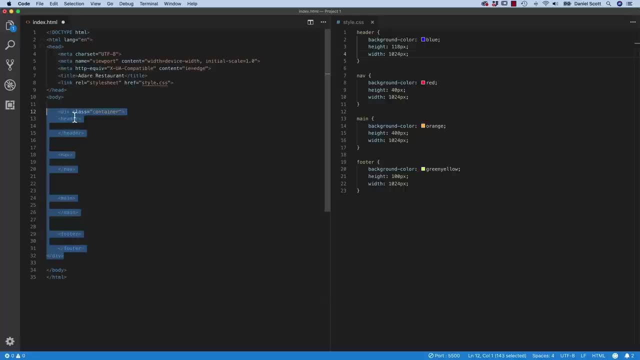 There's a sneaky shortcut to tidying it all up rather than tabbing it all yourself. Just right click it and go to this one that says Format Selection. It just kind of indents everything nicely. The other thing I might do to kind of make this seem a bit nicer is: 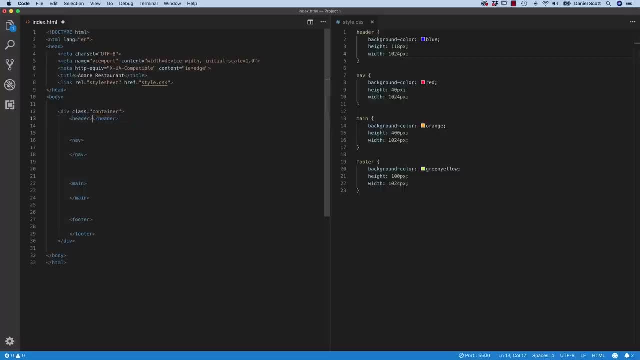 I know I put Returns in. I'm getting rid of them. I'm trying to clear this up so it looks nice for you. Editor, can you speed this up a little bit? I'll see you guys in a sec. All right, you're back. 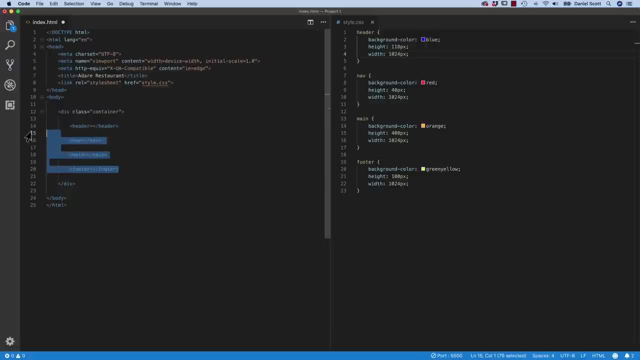 Now you might go. that looked painful and it is, but it's kind of how I work. I liked everything to try and be as nice as I can, and especially doing tutorials, because it's nice for you to be clear about where everything is and what it does. 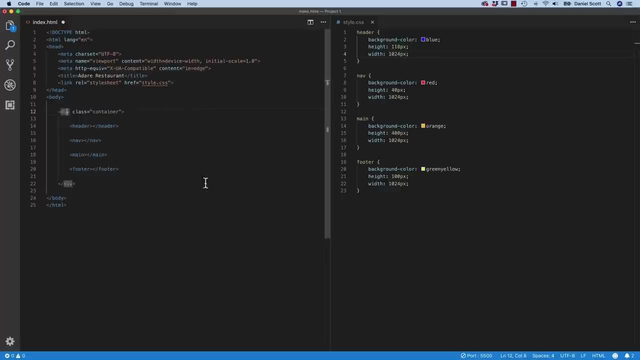 So it's nice and clear now that that's inside of a container, right, Because it's indented. So all we need to do down here is we need to say style the container And you're like he's doing it wrong. 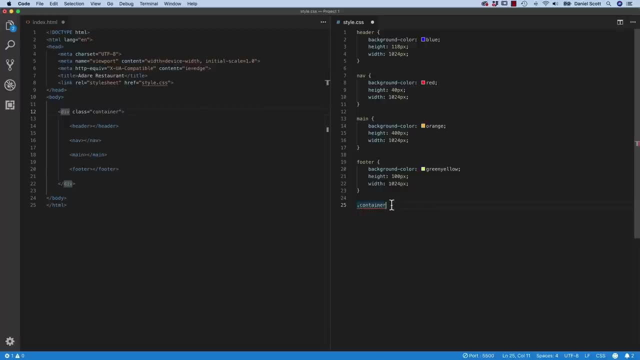 You're like: definitely, That was an actual test that I set up, So you have to, if you're signing a class, remember the period goes in front, And then we can say: and we paste that we don't. So I've got to do it again. 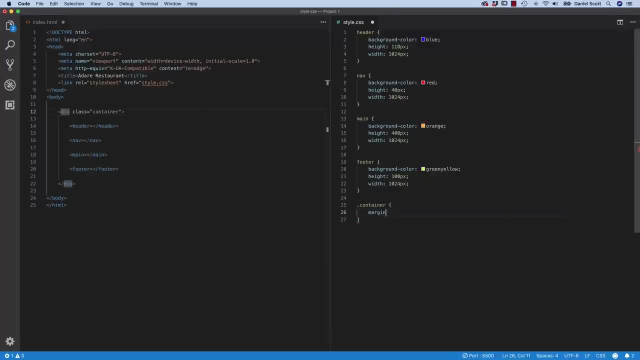 So margin, we'll do margin-left, We're going to make it auto semicolon, same thing, margin-right, Auto semicolon, save it. And because all of these fellas are inside of the container, they should not work. 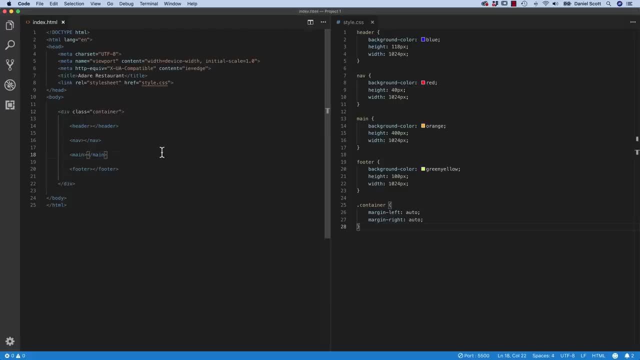 Save all, not a test. Why is it not working? Div class container: right, left. there are no errors down here. I've saved it all. what's going wrong? I know what it is, So I've added a width, because I'm doing this a bit backwards. 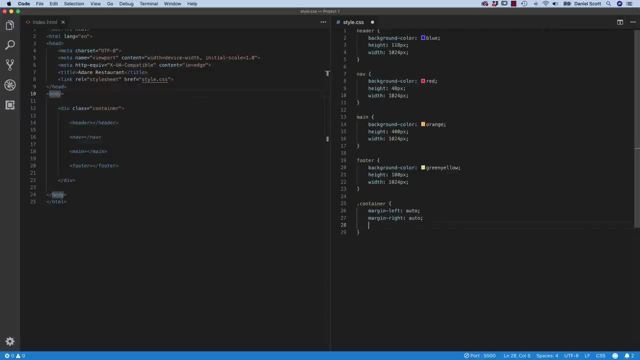 I added the width to these internal guys. The container needs a width. We need to swap them. So you need a width, not windows widows. We need a width more flustered, a width of 10, 24.. 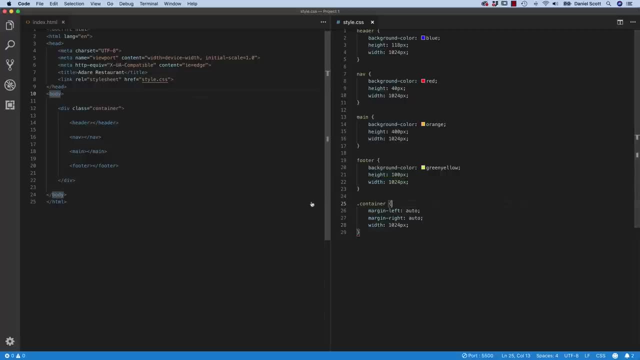 And these guys can come off. Well, actually they can stay on watch. let's have a look. So the container now is width, so now the margins know to push out from the sides there. So we could leave these here, but because by nature, div tags will try and stretch to fill the space provided. 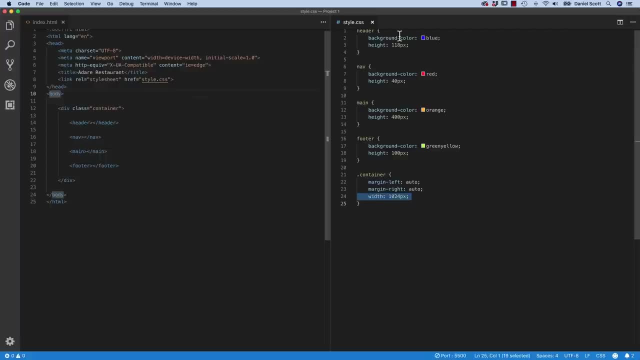 and we've said the space provided is container. these guys don't need to be told twice. There they go. looks exactly the same. Now, in terms of the flow here, I want the container to be at the top, just because later on when I come back into here, 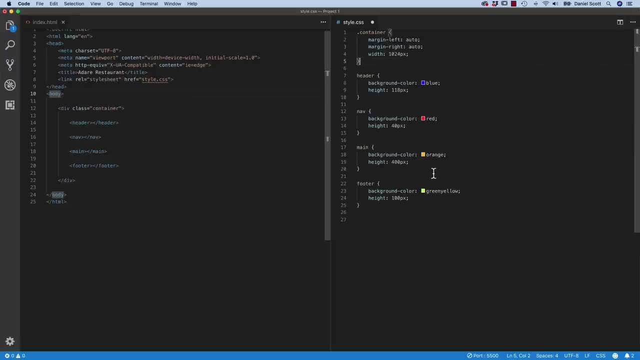 I'm looking for kind of when the CSS sheet gets quite long. I'm like, all right, the stuff at the top are the most kind of overriding things, So container and then header. these are, I guess, lower in the picking order in terms of the structure for the site. 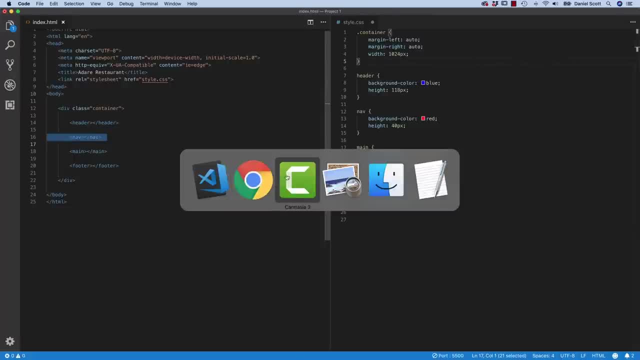 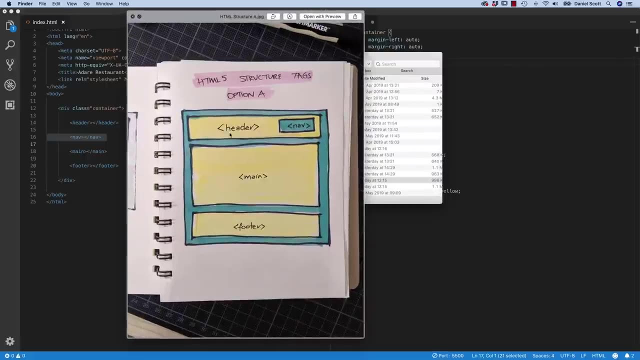 All right, so that's applying the HTML tags. now. In a previous- where is it This one here? I showed you in wire frames I made this one called Structure A and I put the nav inside the header. So we'll do that one first. 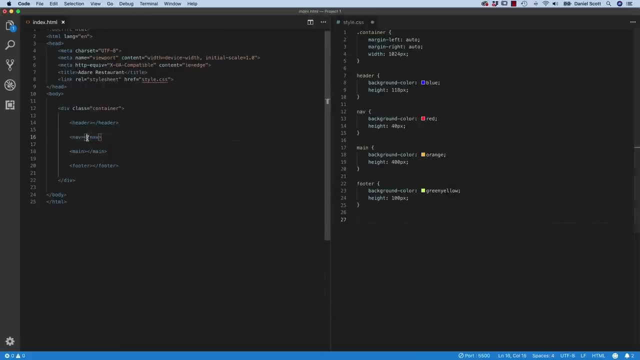 That would just mean cutting that out Wrong side, Grab this, cutting it out and putting the header inside of this one. So that would be a way of structuring that kind of design. Let's say the other design didn't use main, they used section instead. 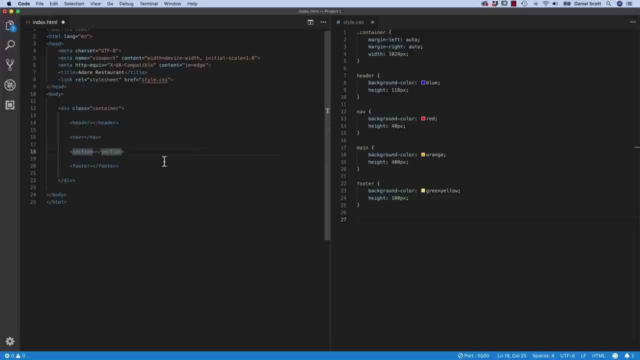 Or so section open and close. they'd use that and style section over here, But nothing would really change. I'm using main because that's just the way that I like to do it And I get confused by sections and articles. 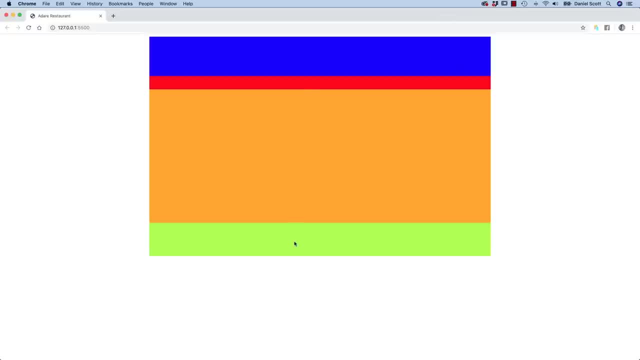 All right, buddies, we've got our kind of basic structure for our site, with some ugly colors. Let's start adding extra things, because we've only done simple text and boxes. We'll start adding proper background colors and we'll start adding images and text. 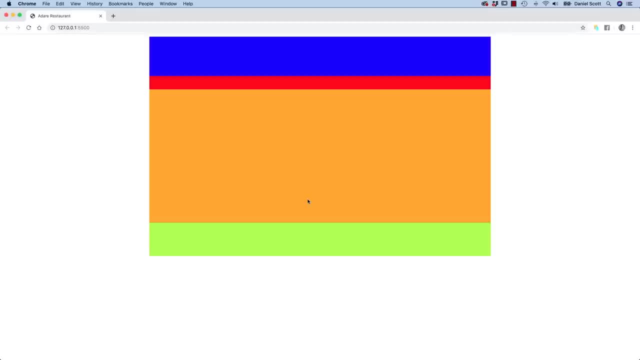 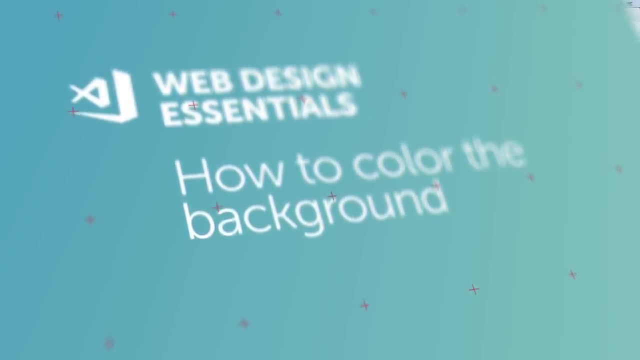 and all sorts of stuff in the upcoming videos. I will see you in a little bit, after lunch. Hi there, in this video we're going to go from this plain old white background to to this toxic green color. Basically, I'm going to show you how to color the background. 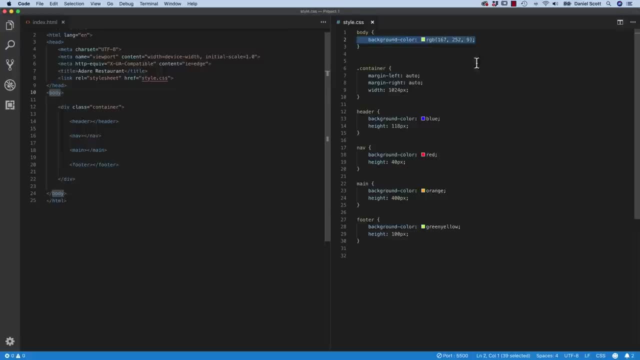 using your HTML body tag. And then I go off on a bit of a tangent to discuss RGB colors and hexadecimal colors and how to use this little color slider picker thing. It's all ahead of you in this next class, All right. so now we need to color this background part here. 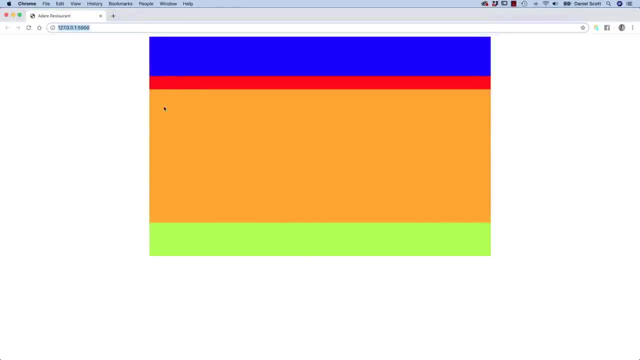 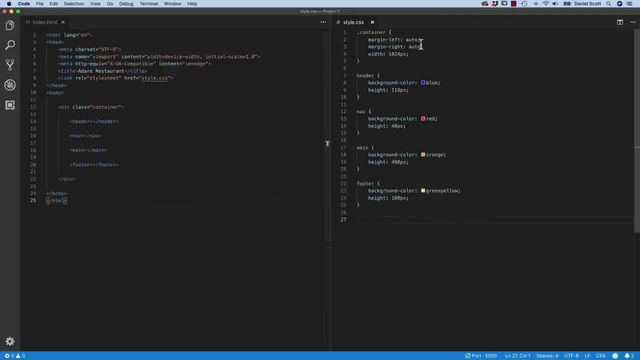 So this white we can't color just the container, because the container is just sitting here in the middle. So we need another way. imagine if there was a tag that wrapped around everything on our page. Look at that body tag, it's already there. 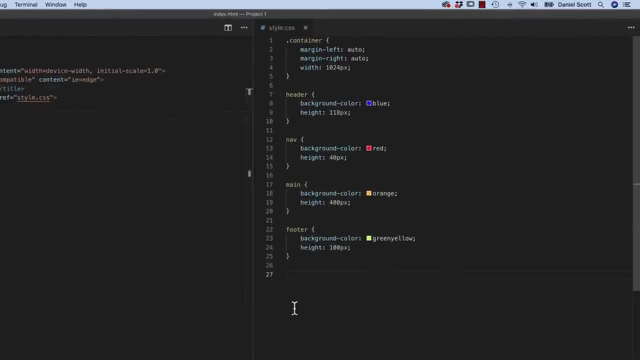 And this is the tag that you style to change the complete background color. Now we could put the body down the end here, but it's really common to have it at the top. So body remember, it doesn't need a period or a full stop in front of it. 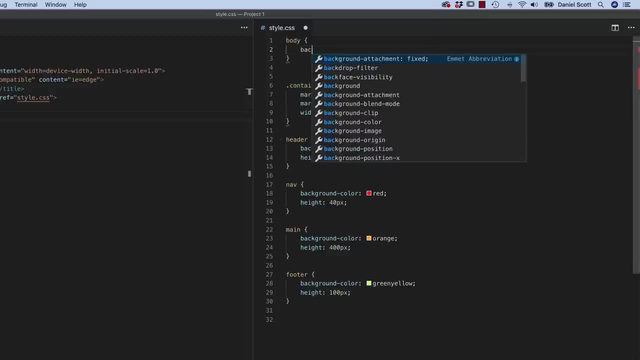 Just type body and we're going to add our background. We've used this loads of times now: Background color. There it is. Now we're going to pick one of these random colors for the moment, Coral. Let's check out what coral is. 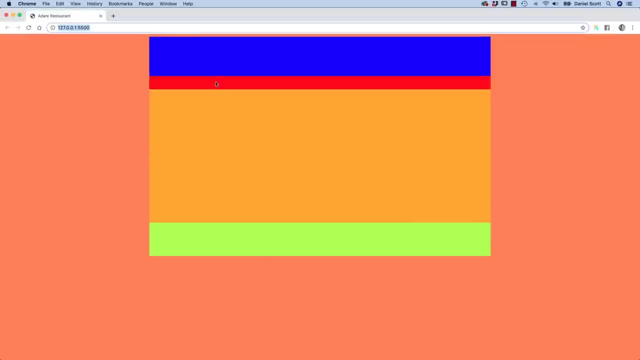 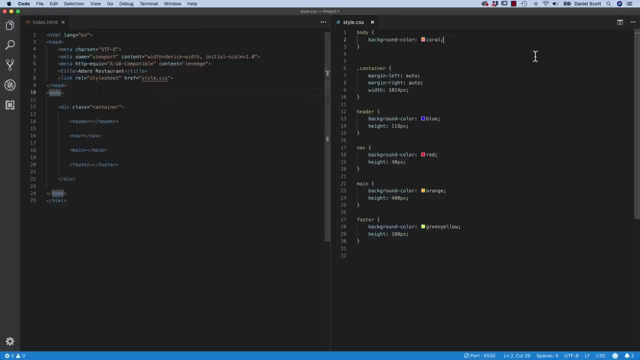 And it's, yeah, kind of like it, kind of do. It's not working with these colors, but that is how to change your background color. We'll do background images later on in the course, But for the moment I want to focus a little bit on color. 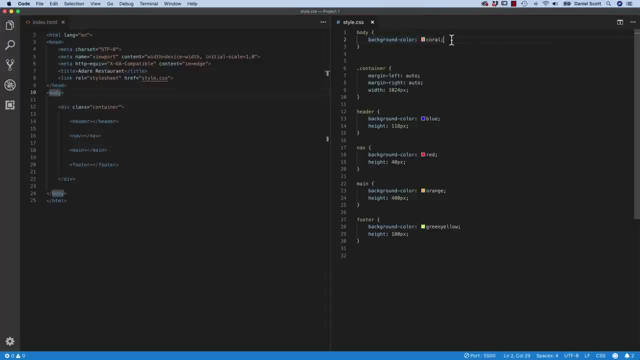 because, using coral and red and Indian red and ruby red, there's lots of different kind of naming. I don't know who's in charge of naming those colors, but hey, that's what they are. Often what we want to do is just hover above it with your mouse. 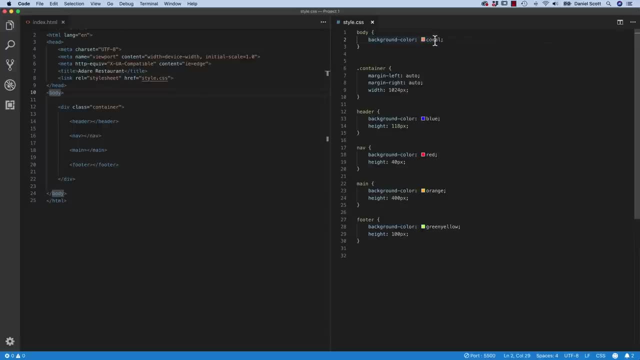 I'm not doing anything. I'm not clicking on it, I'm just hovering above it. It's kind of weird in VS Code. Sometimes it turns on. you're like sometimes you just can't make it turn on, even though you really want to. 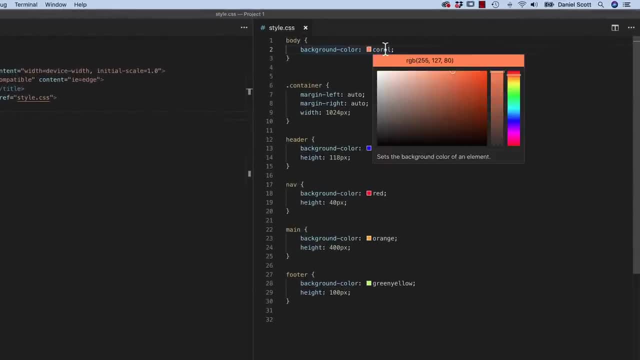 So just hover above it, See it won't turn on. Now it will, And then down here we can do a couple of things. This kind of far right slider is the hue, So drag it to get it roughly in the zone. 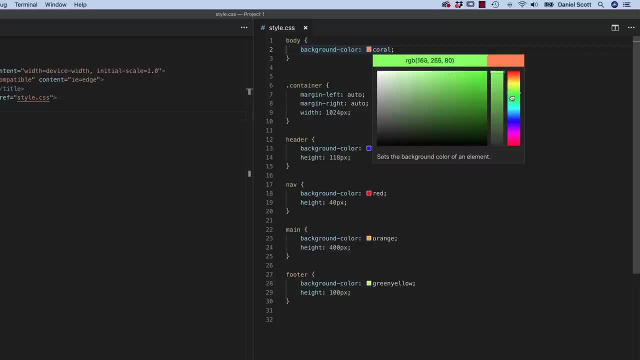 So say we want to change this to, let's say, bright green, just because. So we get it in the bright green range and we go: do you want a bit more yellow, Yellowy green or a bit more of a bluey green? 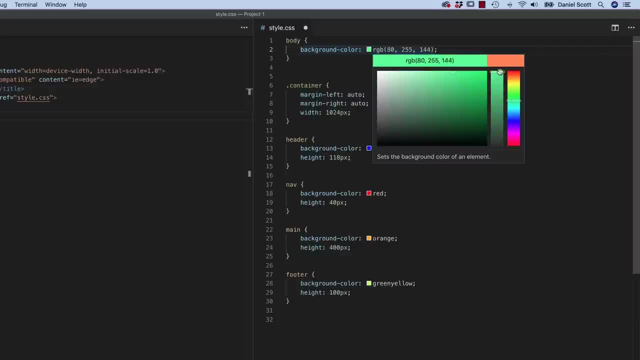 Let's go with the bluey green. Then over here is the opacity. so how see-through it is For a background color. you can't really have see-throughness or opacity because there's nothing to see through to. But later on that will be useful. 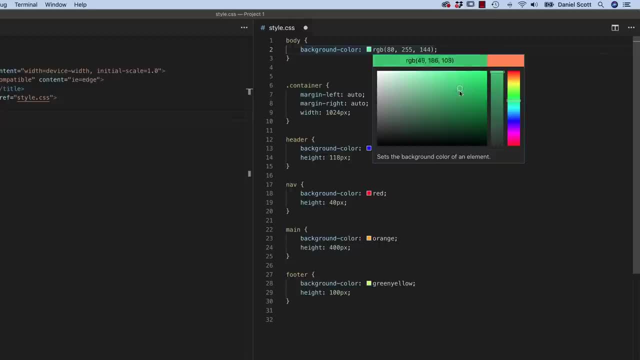 And in here it's wherever this dot ends up. So you click, hold it and move it around. So if I go up here, it doesn't matter what the hue is. I'm going to have white, which is RGB, 255 across all of them. 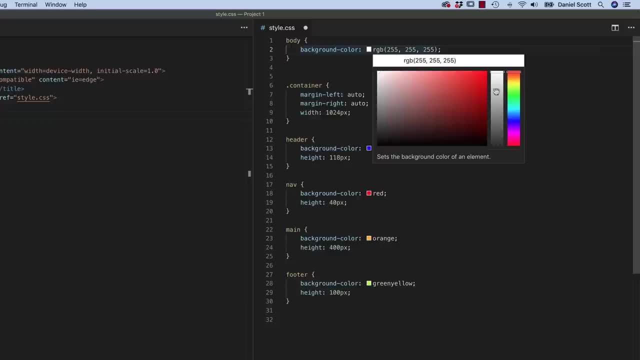 So what I want to do is get back into it by hovering above it And going back into here, grabbing the green, getting the kind of bluey green and then clicking in here. I'm just kind of getting it to where I feel it should look nice. 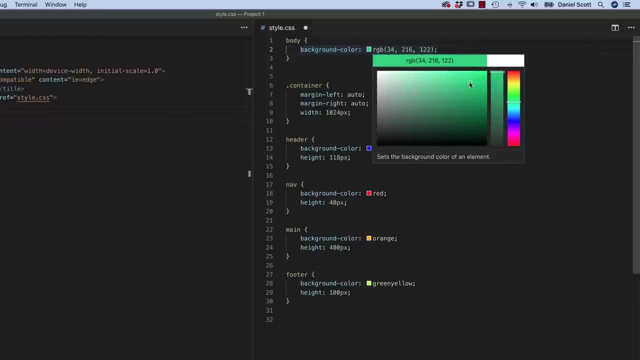 And that's what I want to do. I'm picking a random color for the moment. Now you just click off in the background or move your mouse away, You'll notice the colors change from being RGB- Sorry, from a name- to this red, green and blue mixture. 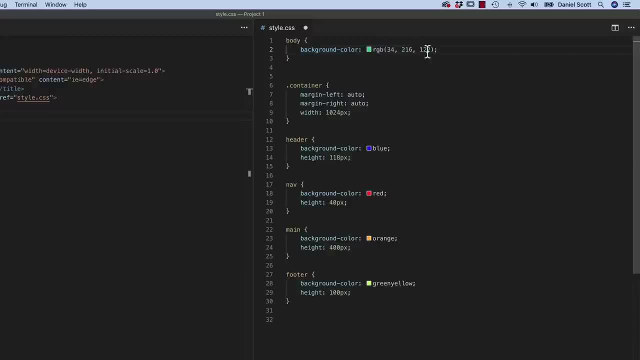 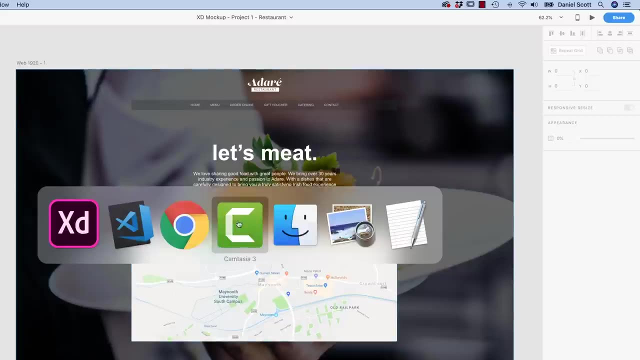 And those red mixed with green, mixed with blue makes that kind of crazy green color. Let's save it and let's test it in the browser. That's the wrong place. There it is. this is my green. Another way to do colors is to use hexadecimal colors. 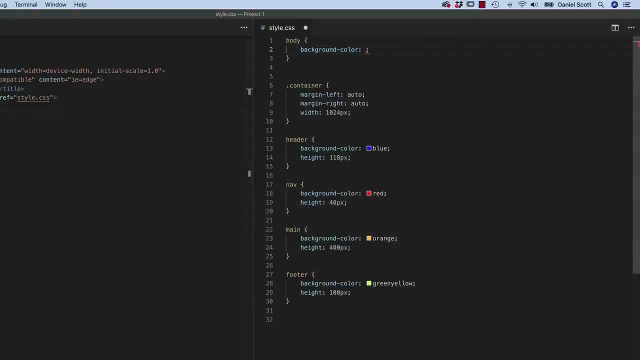 So I'm going to delete all of that Now. this is for the people that know already. So let's say that you do know what a hexadecimal number is. It starts with a hash, and often people will use three or six-digit code. I'm just going to fake one. 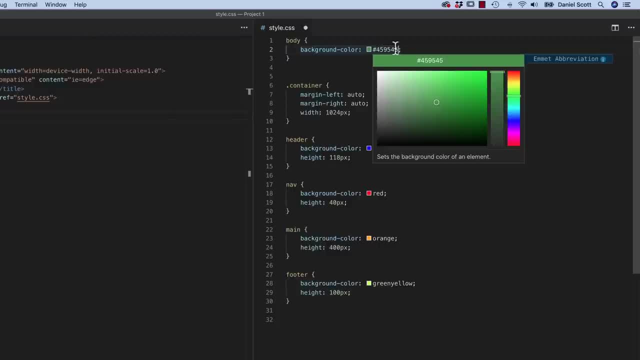 So it turns out, if I hit those keys randomly on my keyboard, I get a green. So it's either three or six digits, mainly six digits. And where do we get these colors from? They're actually made up of red, green and blue. 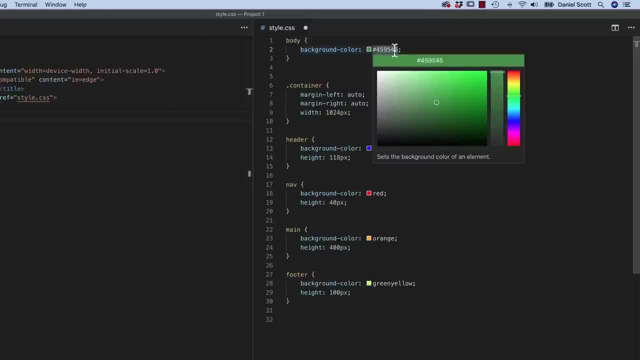 So the first two digits are red. second two digits are green. Last two digits are blue. you don't need to know that. Let's say that you're working with brand guidelines, So you're working for a corporate client. They might give you this hexadecimal number or the RGB number. 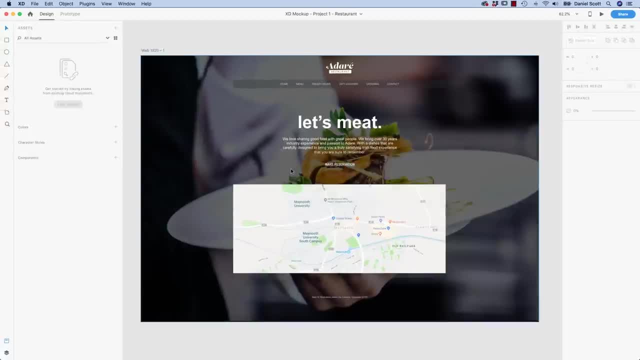 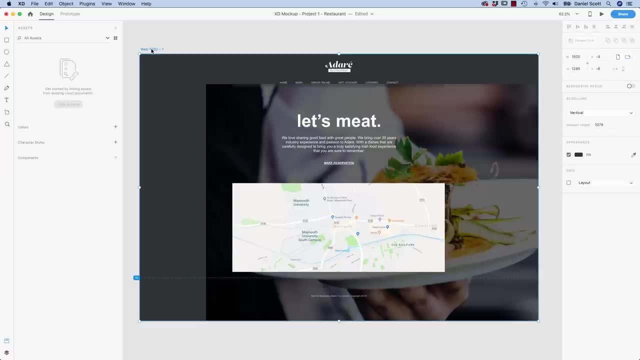 You can type in whichever works for you. For me, I'm working from this mock-up here in XD. We'll look at XD later on, but this color in the background I've clicked on my name up here. don't worry if you've never used XD. 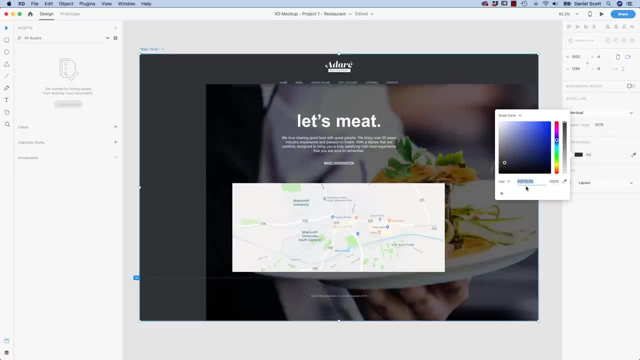 We'll talk about it later on in the course. I click on this and you can see. it gives me my hexadecimal number, Or it could go RGB. I could type those in All these different kinds of web creation like design products. 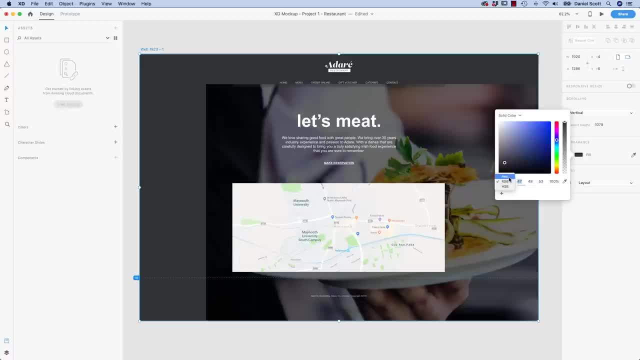 like you could use Photoshop or Illustrator or XD or Sketch To design your website, but you build it in VS Code And then just figure out what color code you want to use. That's the code I want. I'm going to copy it. 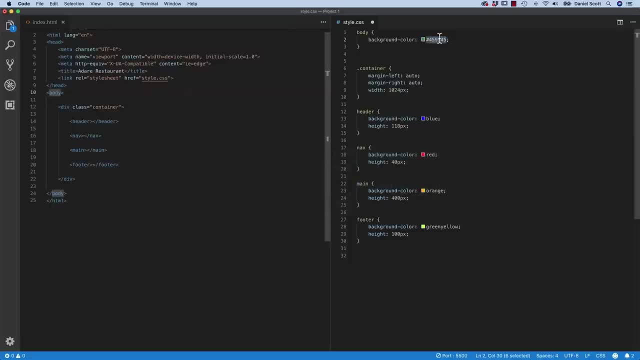 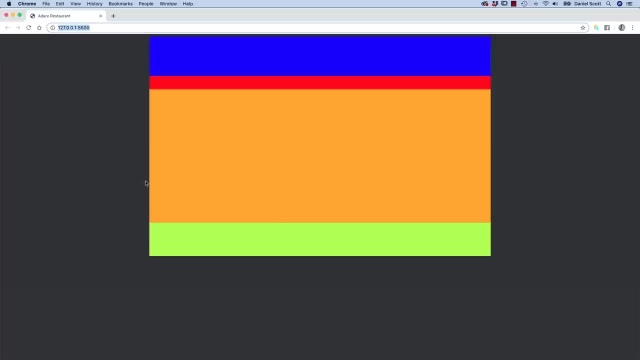 I'm going to go into VS Code and that, my friend, is the kind of dark gray that I want Save it Browser. that's the dark gray. The first bit was easy. we talked about adding the body tag and then I went on a little bit too long about colors. 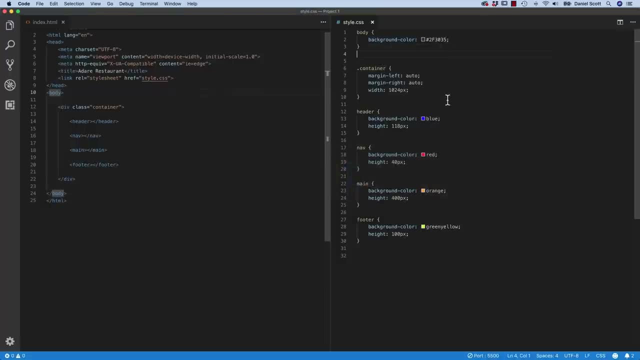 Felt like it was the time to do it, but maybe it's for later. We'll cover it again Then as we go through, if that felt a bit fast. I'm back for lunch. I've had a coffee. I'm racing through stuff. 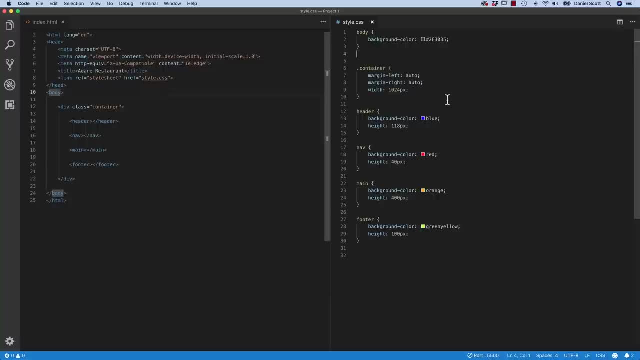 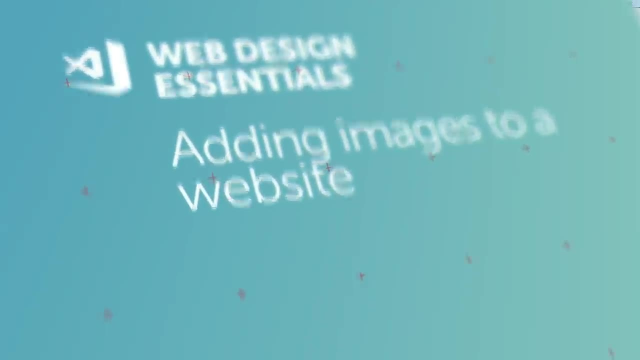 Slow down there, take breaths, And I will see you in the next video wherever you're taking a breath. All right, this video is all about adding images to your HTML. It's pretty easy. let's jump in now and learn how to do it. 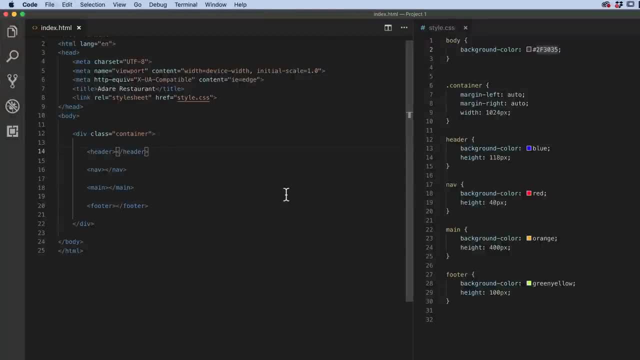 All right to add our image. we're going to put it inside the header, So click in. in between the header angle brackets, put a return in, And we're going to use IMG. That's the kind of shortened version of the tag that describes an image. 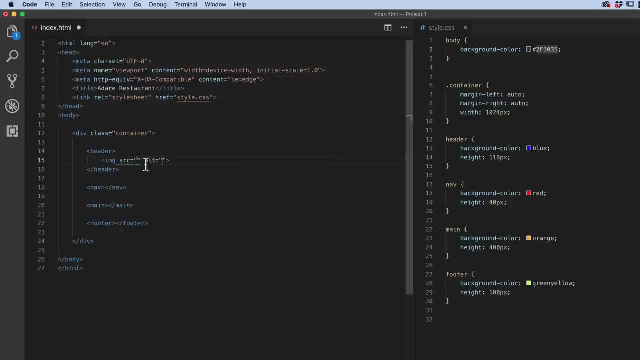 And hit return and it puts in all the junk we need. So the image source, just where it is, And it's nowhere at the moment, so we need to put it in a place inside of our local folder. so let's do that first. 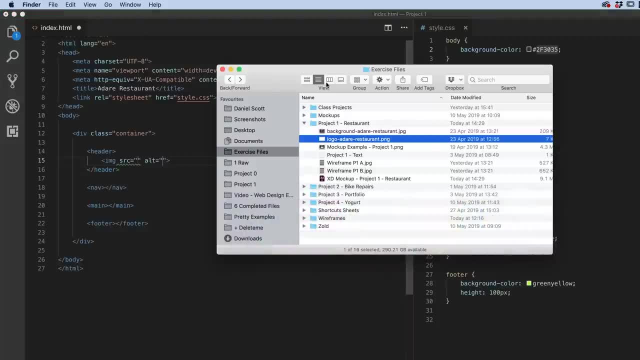 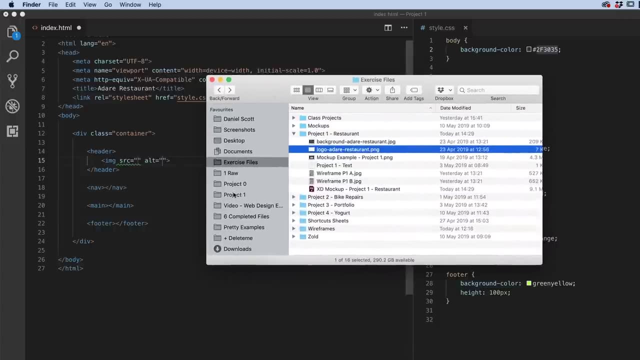 So what we're going to do is we're going to jump out to our Finder. So on a Mac it's called a Finder. in your PC it's called a Window. So find your My Documents Panel, get this up And on your Desktop inside of your Project One. 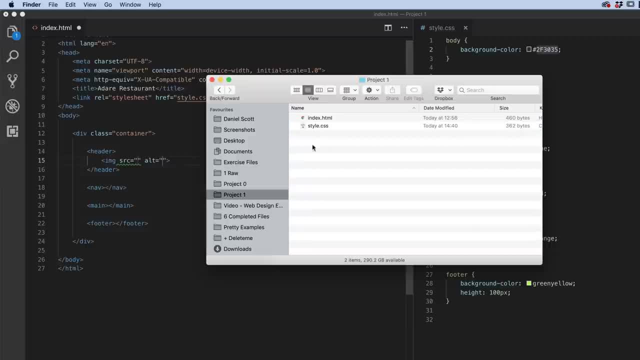 we've got Index and Style but we need to put our image in here And it's really common not to just dump it sitting kind of in with these guys. You put them in a group in its own little folder called Images. 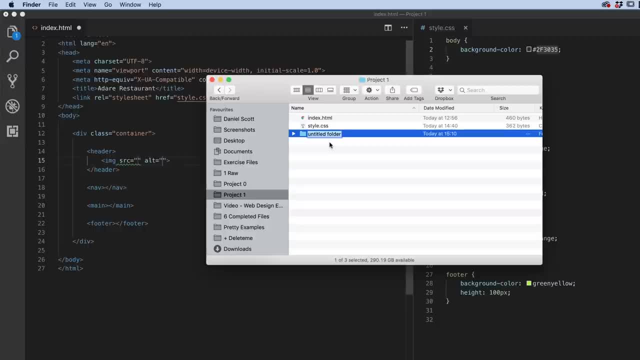 So we're going to right click, I'm going to make a new folder. That's basically the same on Mac or PC And you either call it IMG or Images. I call it Images, Half the world calls it IMG and the other half of the world calls it Images. 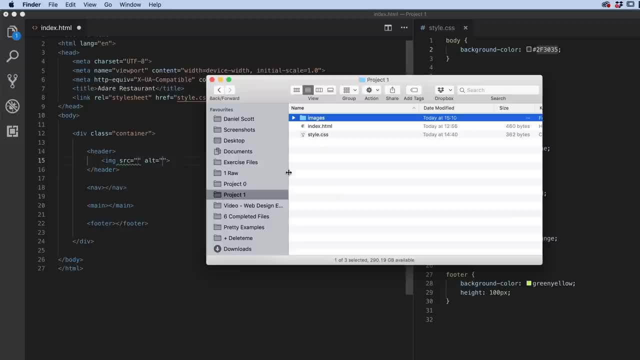 I call it Images. it's not good or bad, but you have to take sides. So we've got a folder. We've got a folder in there called Images. there's nothing in it, So let's go into our Exercise Files. 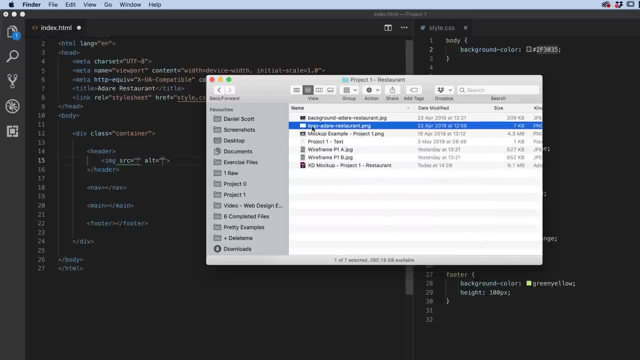 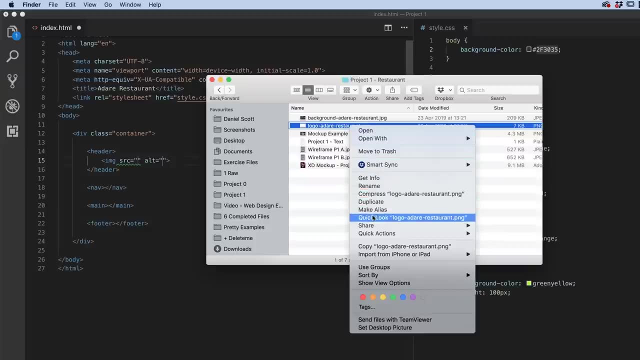 Let's go to Project One And inside of here there's a PNG called Logo Adair Restaurant. I'm going to right click it, I'm going to copy it. Where is copy? I use shortcuts, you can tell. Can I copy? There you go, copy. 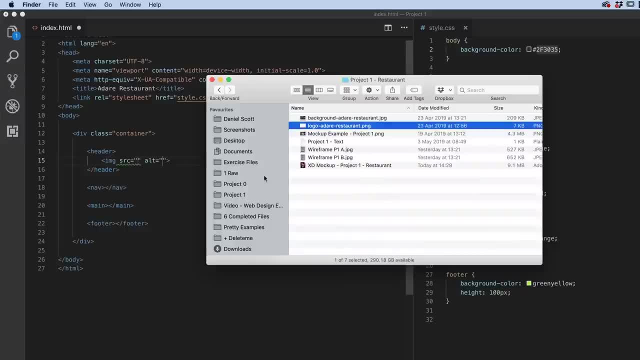 Or Command C or Control C on a PC. Let's go back to our Desktop and paste it in Desktop Project One Images, Right click, Paste Item and there it is. So it hasn't really done much, so I guess it brings up a really good point. 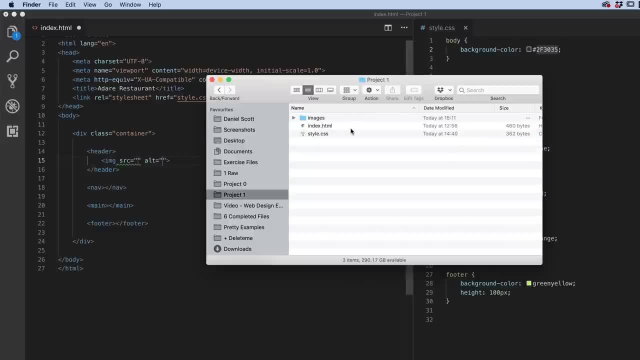 Everything in this website needs to be in this folder called Project One. Remember, it doesn't have to be called Project One, but everything has to be inside of here. It's called the root of the website, So it needs to know that this is home base. 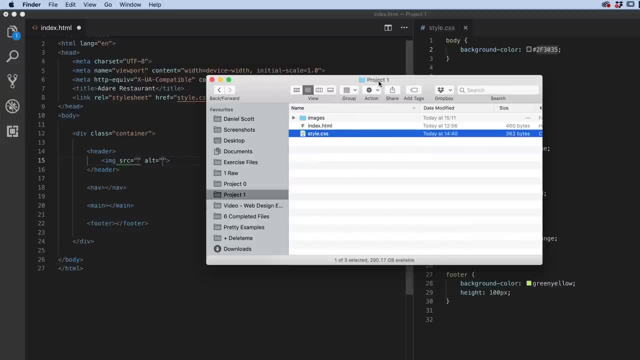 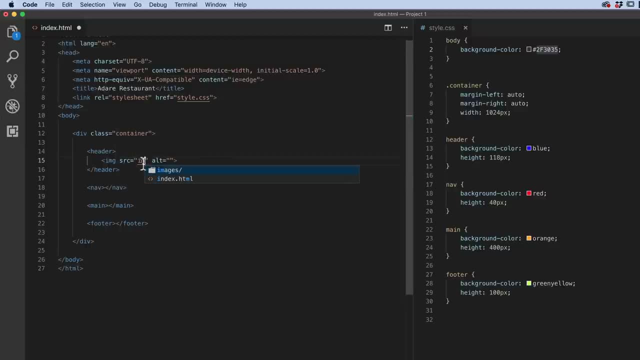 and it doesn't need to know. the rest of your computer exists, It just needs to know this little folder. it's its own little world. So under Image Source. so I just type in IM: Type it. I just started typing IM. 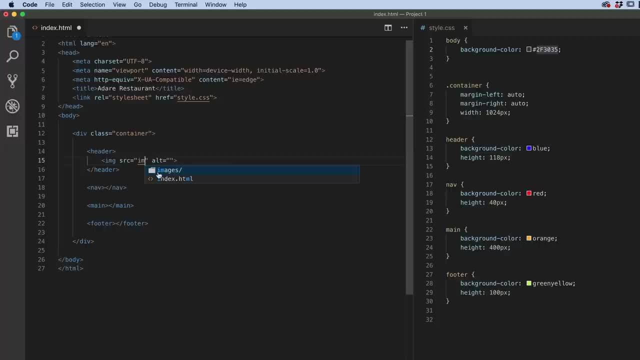 You can see it goes. hey, I've looked into your root folder and I've seen this folder called Images. Would you like to use that And you're like I would? If it doesn't appear, it's probably broken. 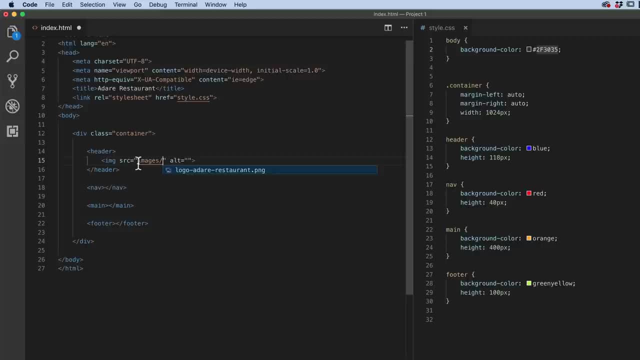 and you need to go and make sure that Images folder is in the right place. But if it's still not working, just type it in IMG and then you need a forward slash to say: I'm inside that folder And what's inside that folder. There's only one thing. it's pretty clever. 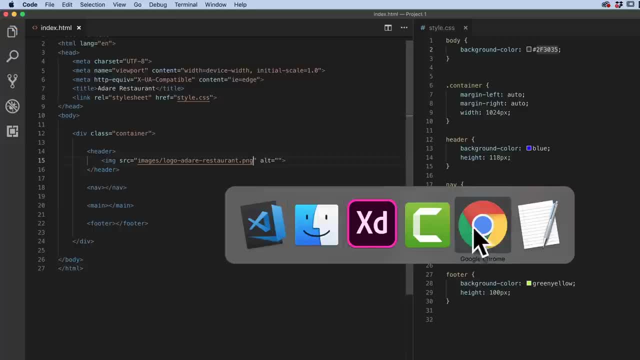 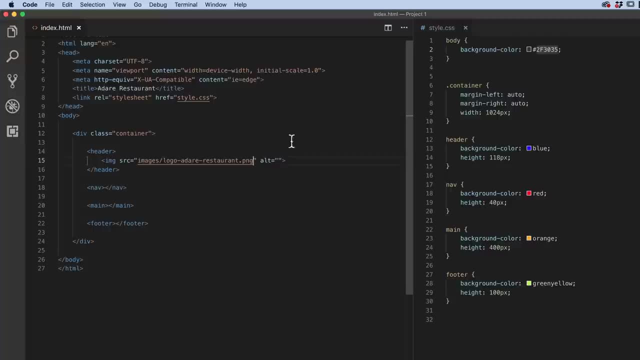 Now let's save it, save all and let's preview in a browser. There it is. it's left aligned. We're going to move it into the middle, but that's how you add an image pretty easy. The Alt Text is super important when you're adding images. 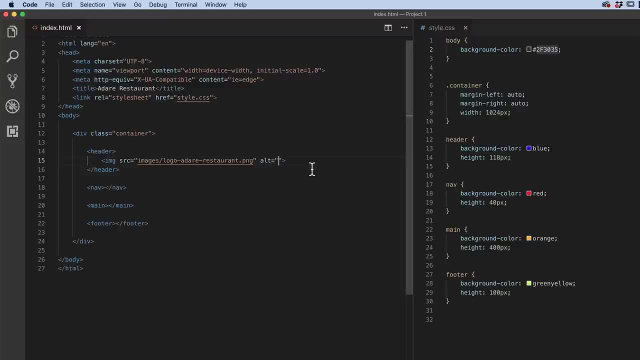 Basically, Alt Text is short for Alternative and it just means: if this image didn't load, what text would best describe this image? And this is going to be the logo for Adair Restaurant. Is that what we call it? It is Adair Restaurant. 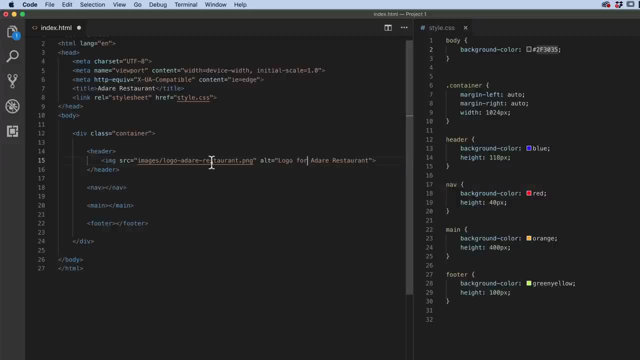 Can I spell restaurant? It's close, So that describes that image And why we do it is for a couple of reasons. The visually impaired will have a screen reader that will read them the website. So obviously, if you can't see the logo, you need to be described what it is. 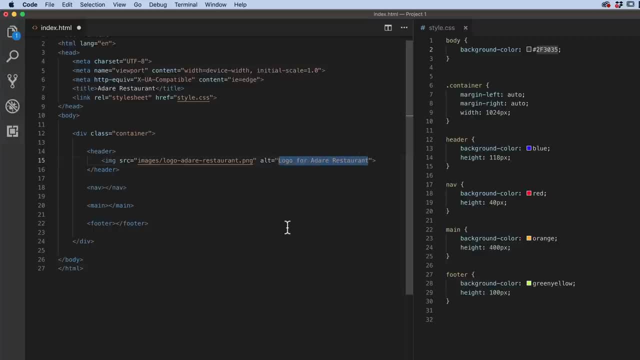 So it needs to be a very good descriptor for people getting read out your website. The other thing is that Google uses it to help kind of work out what your site's about. So if you just put logo, that's fine, but you might as well put in for Adair Restaurant. 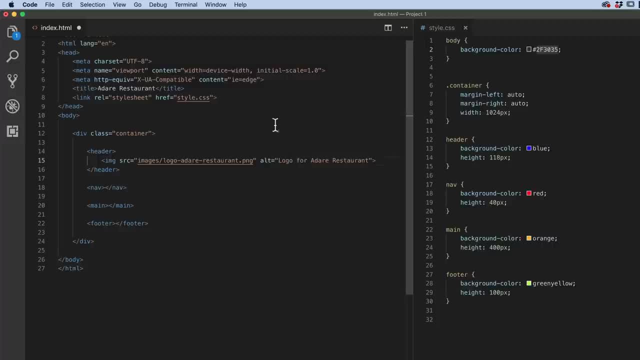 because if somebody's searching for Adair Restaurants and your website is very clearly for Adair Restaurants, it helps your rankings. So make sure Alt Text is really clear what it is, but also is very specific to your kind of target. In our case, we want people looking for restaurants. 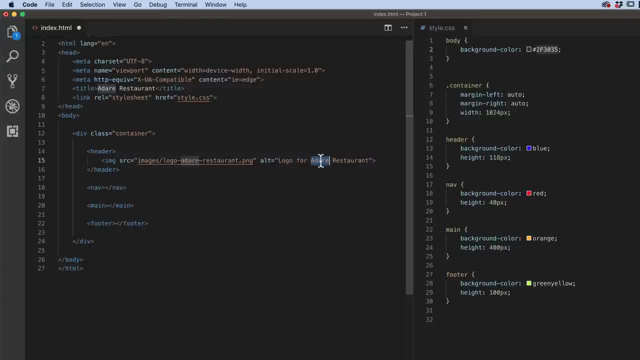 in this town called Adair, where I'm moving to in a couple of weeks. can't wait, Anyway, that's going to be it for this video. We've put in an image. We'll do how to create images out of programs later on in the course. 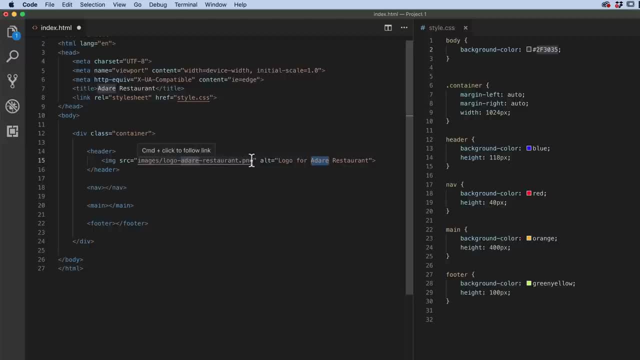 We'll separate that out. we'll do Photoshop, Illustrator and XD. how to make images. The one thing, all you need to know if you are creating them now is that they shouldn't have any spaces. If I have a space there, or at least in the file that I've made- 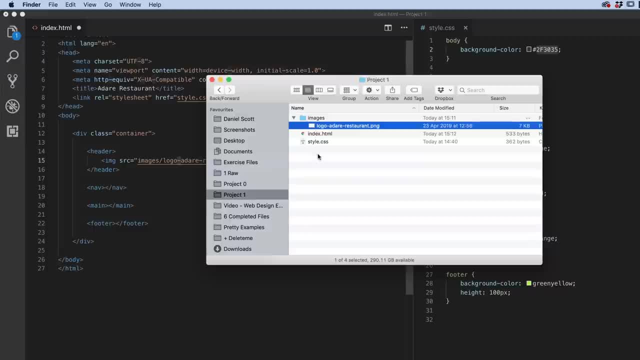 in my images folder that shouldn't have any spaces. Same rules as naming. these Should have underscores or hyphens, or it doesn't matter if it has no spaces. So just make sure, no spaces. Now the next video. let's go. 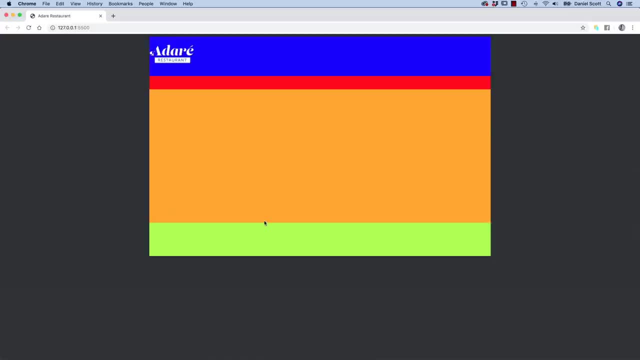 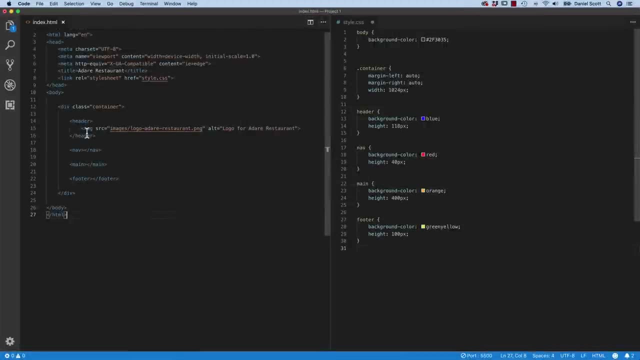 Hi there, in this video we're going to take our image- that's default, sliding to the left, and change it to into the middle. Yay, it's easy, let's jump in and do it. All right, so we want to center this image inside the header. 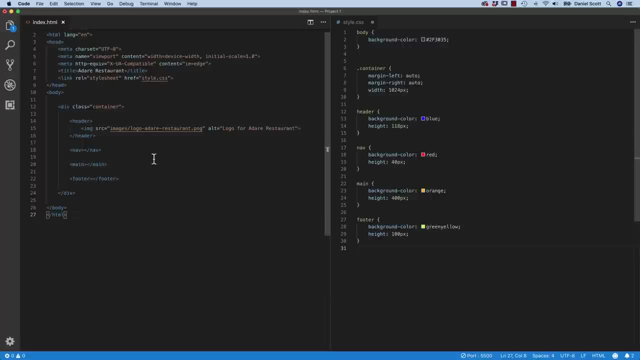 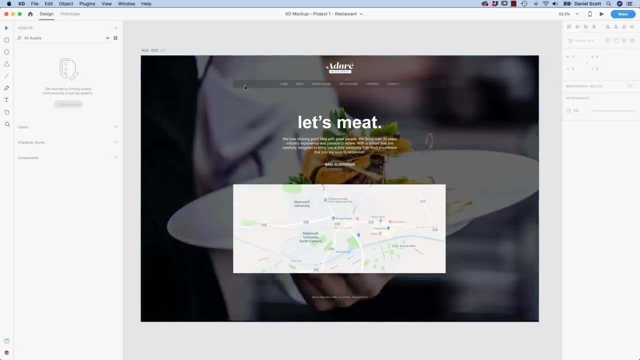 And the easiest way to do it in this case is the header. let's have a look at our design. We would center everything that's inside of it, Because that's the only thing in this header. There's nothing in this. the navigation is outside of that header box. 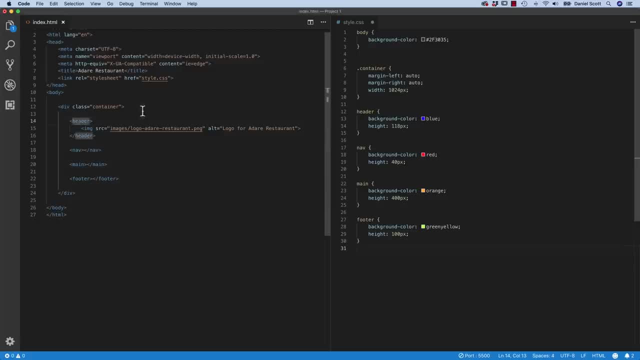 So it's just an image, so it's nice and easy. So let's find the header style over here And let's align it to the center and we'll use Text Align. you're like: why are you using Text Align Center? 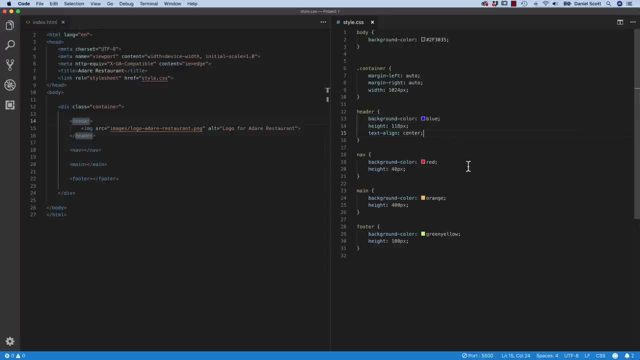 That's just the way it is. Text Align Center works really good for horizontally. horizontal- I get this wrong all the time- horizontal vertical- you know what I mean in the middle. that way, Text Align Center works really well. 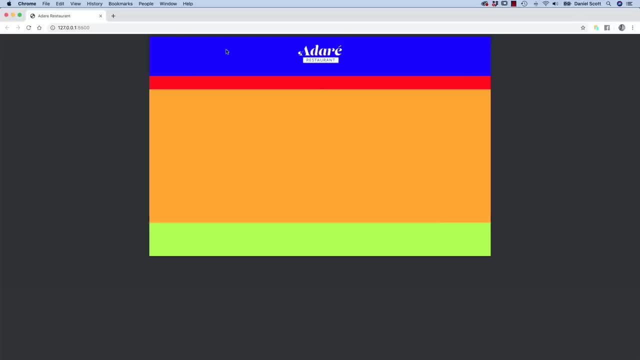 Let's test it. let's preview in a browser And inside of my header, everything is Text Align Center. That is how to get our little image in the middle. And yeah, let's move on to start working with some of the text in this document. 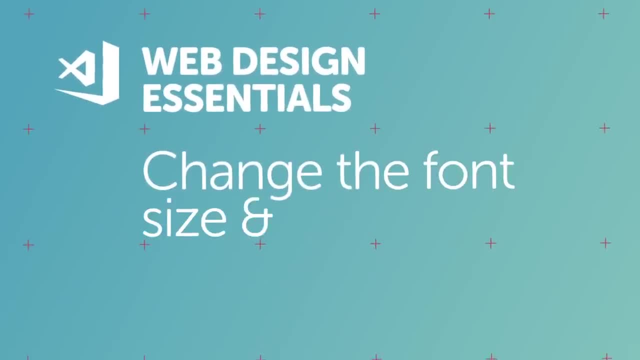 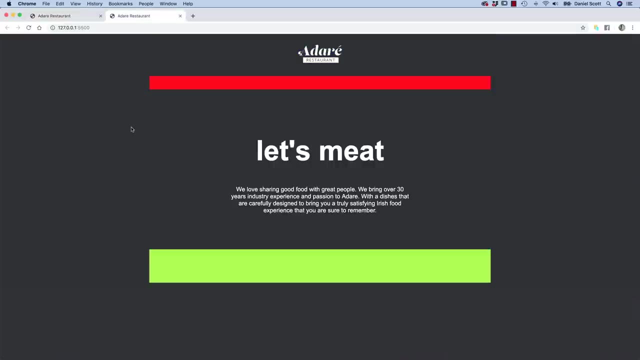 Next video, please. Hello there, fellow web designers. This video we're going to go from this to this: Removing some backgrounds, adding some text, styling the text, looking at font families. We're going to look at padding from the outsides and the top. 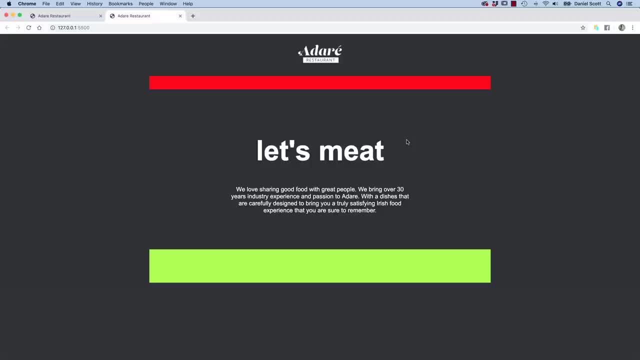 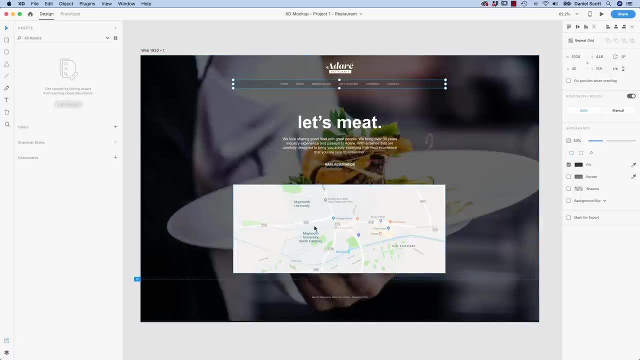 We're going to look at the difference between padding and margin Loads to do in this video. let's jump in and get started, All right? so we want to put in our text And get it kind of looking like this: So there's an H1, and then there's a P tag. 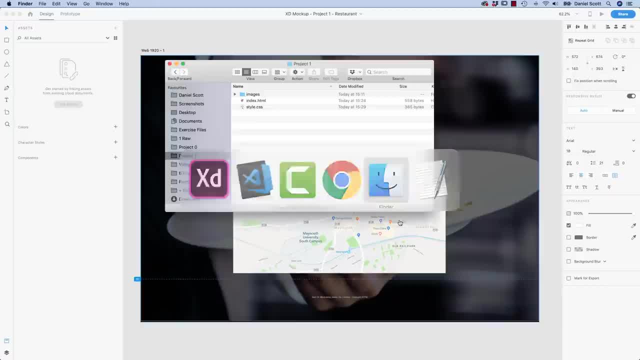 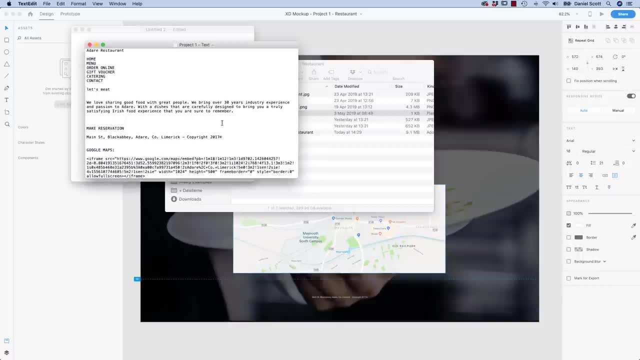 So let's grab the copy. I've put it in your exercise files. So find your exercise files and in Project 1.. there's one called Project 1 Text. Open that up in something and yeah, got some stuff in here. 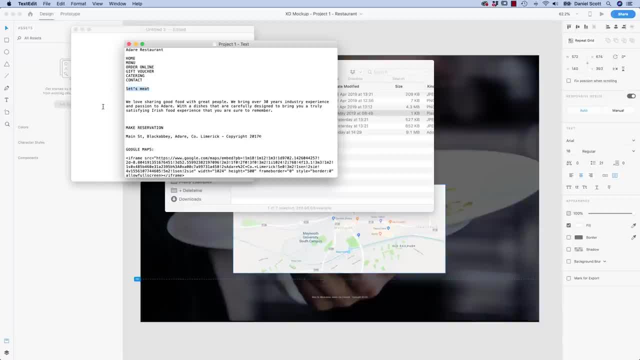 So what we want is: let's meet and let's bring in that. first It's all lowercase, just for looks. You can add the uppercase if you like, and then we'll bring that in a sec. So let's jump in to VS Code. where do we want it? 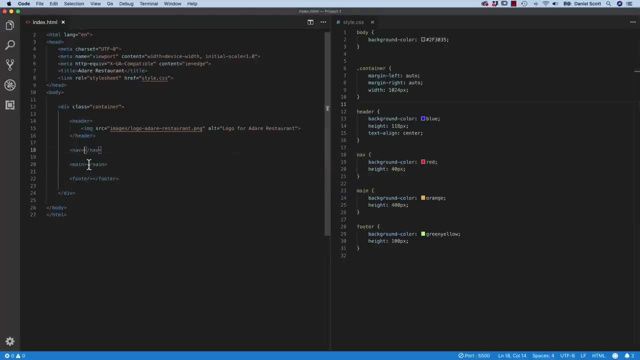 I want it to be: we're skipping the nav. You'd be like, hey, let's do the nav, We'll do the easy bits first and we'll move into. we're building on our skills. let's say So: H1, Tab, we'll return and paste in that text. 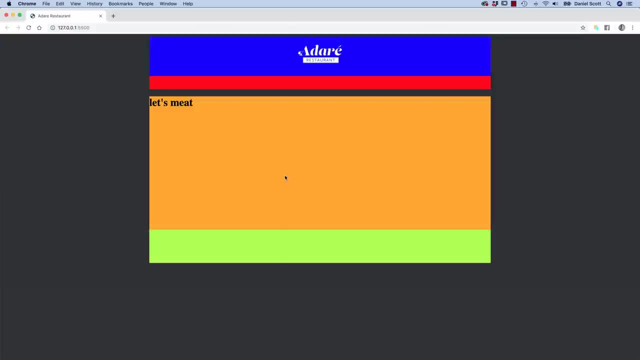 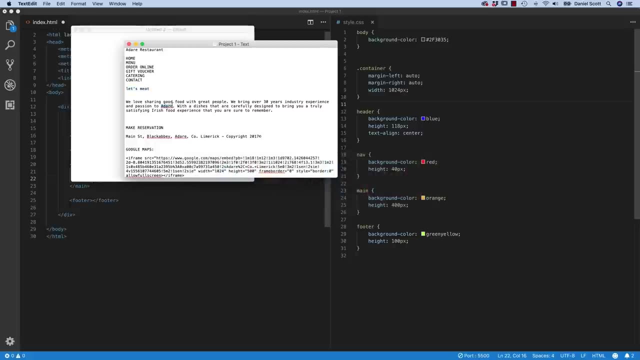 Save. let's have a little look in the browser. There it is. let's meet, Let's add the P tag- P tag- and let's grab the text, copy paste it in. Now. this brings up a good point. 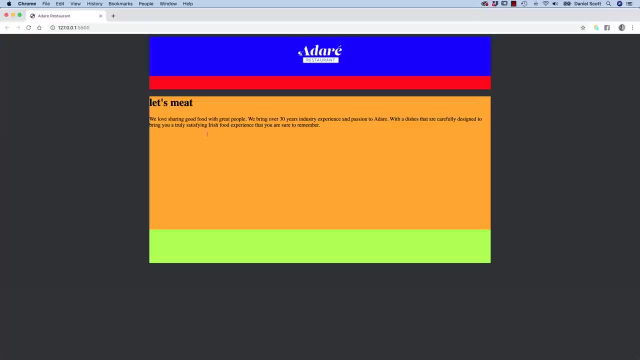 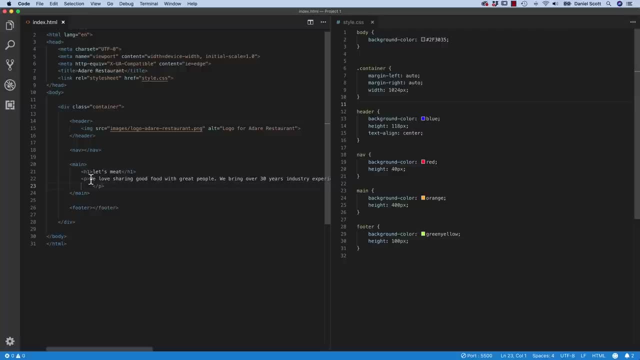 So let's save it in preview, make sure it works. Where are we There? you go, it's in there. Now, in Code view, this can, whether you like it or not, and I'll show you something that I do. 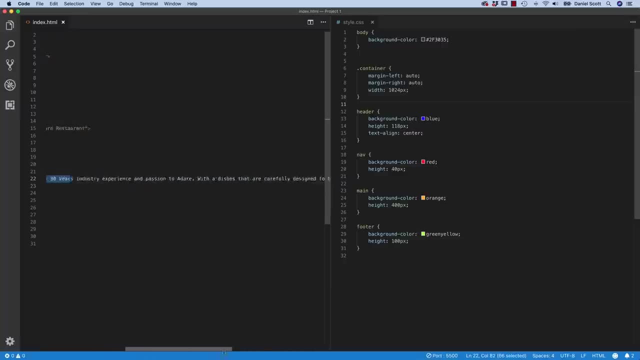 So the text kind of goes off and see on the bottom, here There's lots of text, so you have to kind of scroll across. It's up to you whether you want to leave it like that, because I feel like this is, there's pros and cons for both. 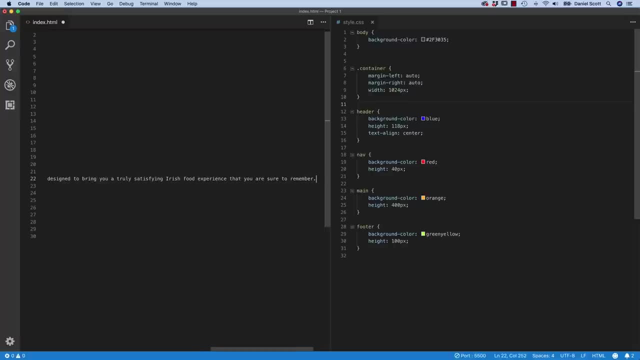 I'm going to delete that. so the P tag, Come on delete. I'm hitting my delete key because there you go, it's all on one line. There you go. nice, like the H1, it's a P tag, all on one line. 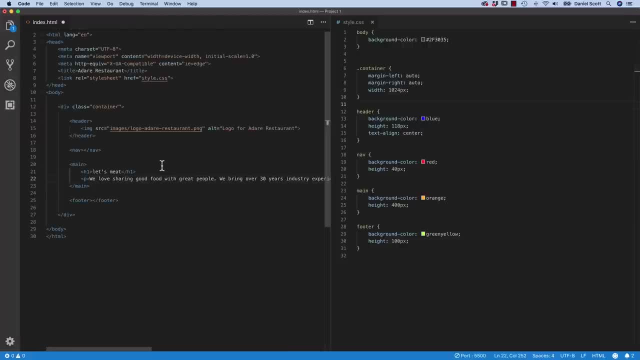 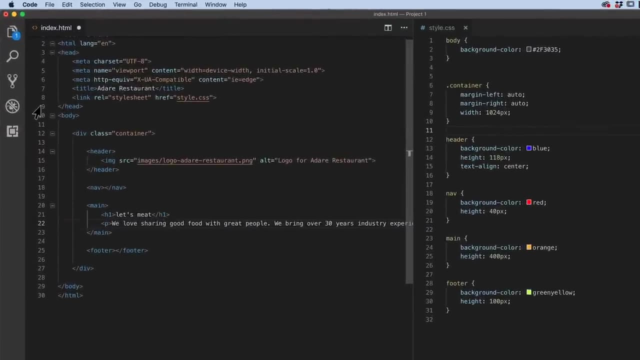 You might like that. A lot of people, and me included, I flip and flop, so I'll show you both. I want that to wrap around. One thing I want you to notice is that every new line starts with a new number, and that makes it quite clear. 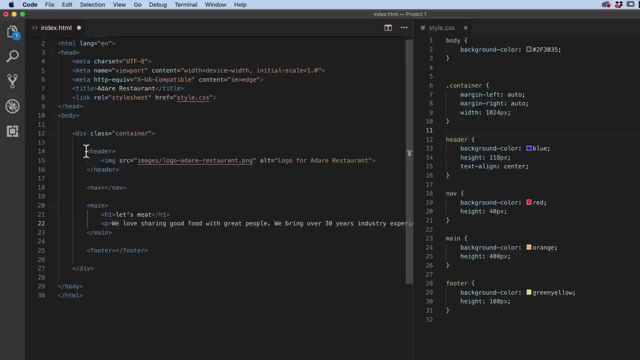 So on line 22,. even though it's quite long, it's all on line 22.. But if I go to view and I do this one here, toggle Word Wrap, can you see it opens up a gap in the numbering. 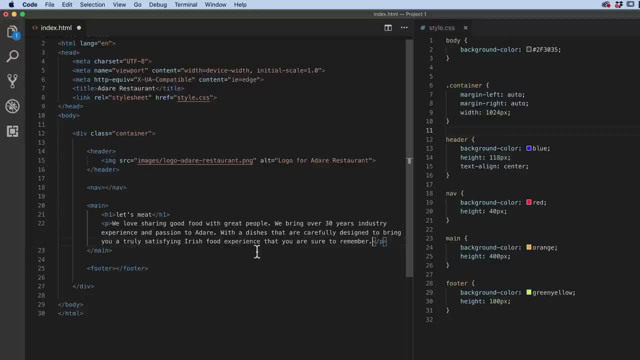 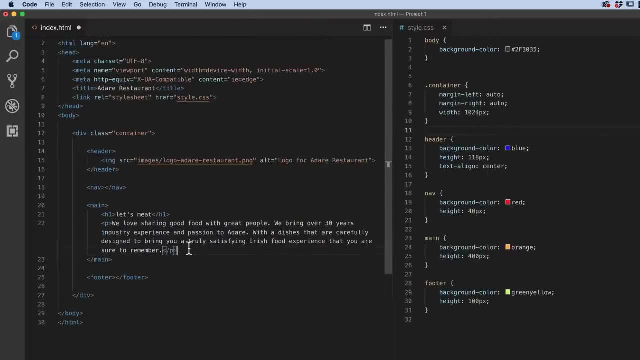 because that's technically still that next line, but it's just kind of wrapping it around because it depends on how wide the spacing is. Do you know what I mean? So it's up to you. I'm going to wrap mine, but you might not like that. 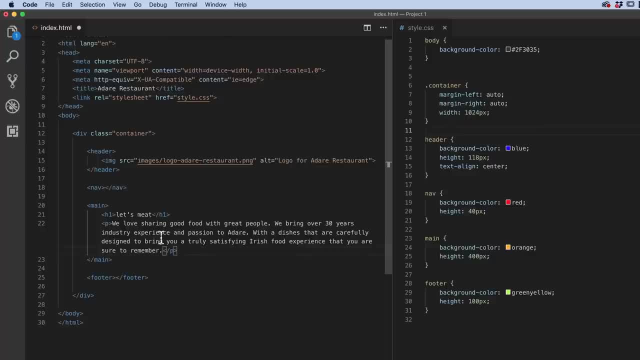 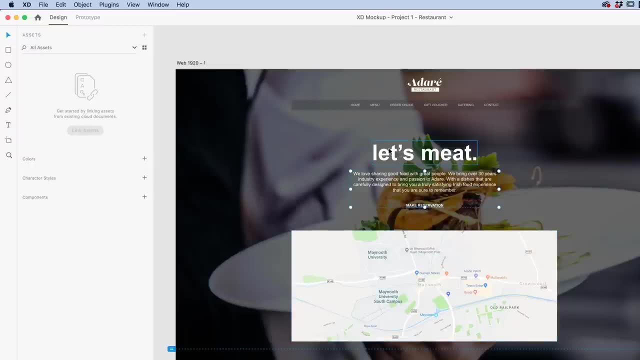 It's easier to turn it off by clicking that exact same button. So now we need to style both of these guys and then add some padding, because that one's bold and it's white and it's not Times New Roman. We're using Arial in this case. 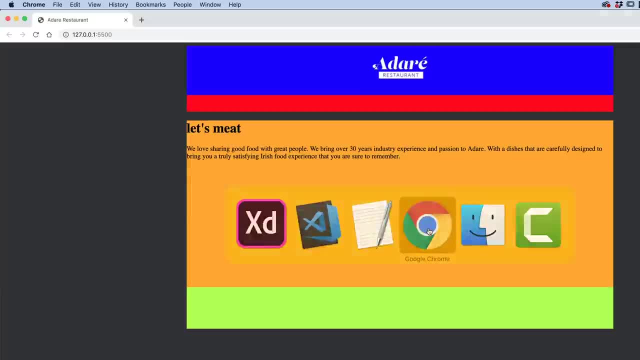 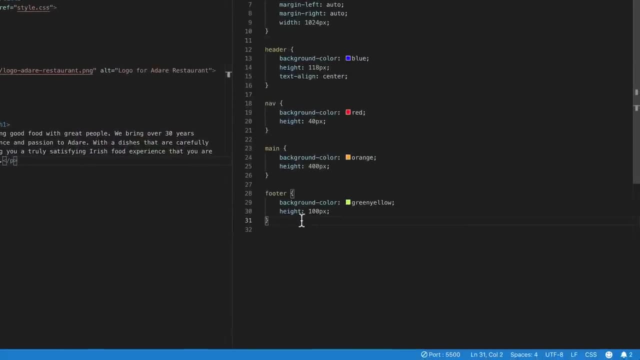 And you can see there's some padding in from the edges, whereas at the moment you see it's running all the way along. Plus we need to center it. So let's do all of those things. So over here in my CSS H1, I'm going to put in curly braces. 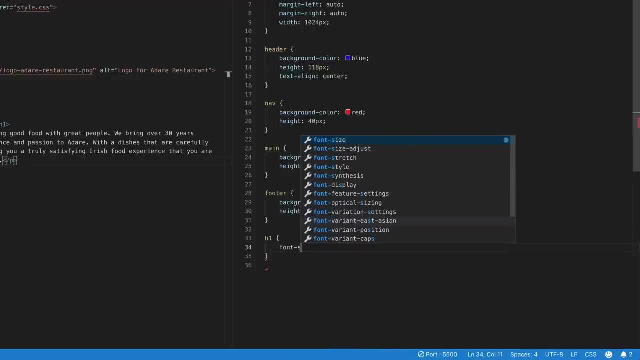 and we're going to do. we'll start with font size When you're building it. you're going to spend a lot more time going. is it 40, or maybe 60?? And just testing, because I've made this class for you guys already. 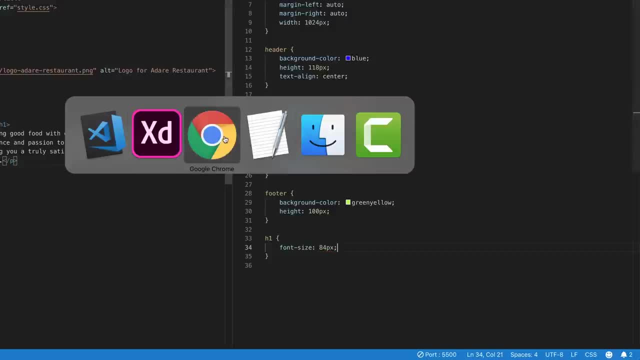 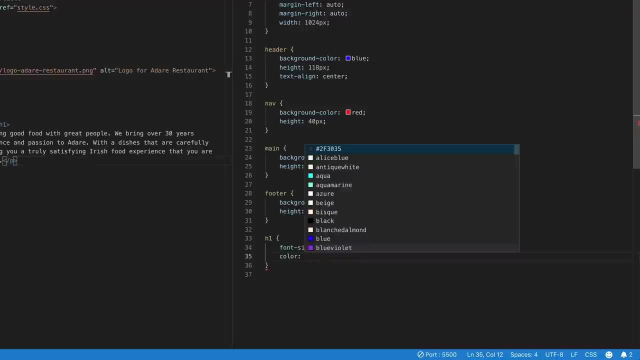 I already know it's 84 exactly. So let's test in the browser. You'll get into the habit, and then out of the habit of just trying to do all of the styling, You'll go in here and you go. okay, now it needs the color of white. 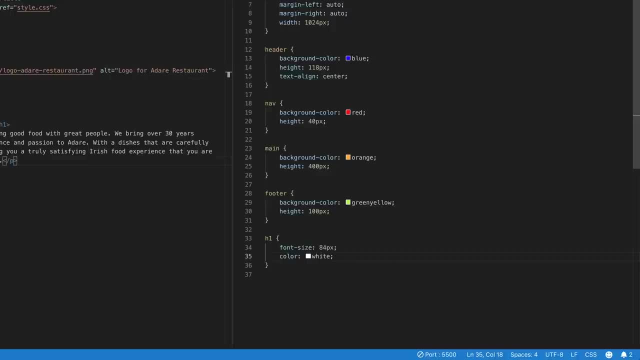 And then you do the next thing, and then the next thing without checking, And then you'll check and something will be totally wrong and you'll have no idea what part of your code you actually broke. So my advice, especially at the beginning, is to do one thing: go check it. 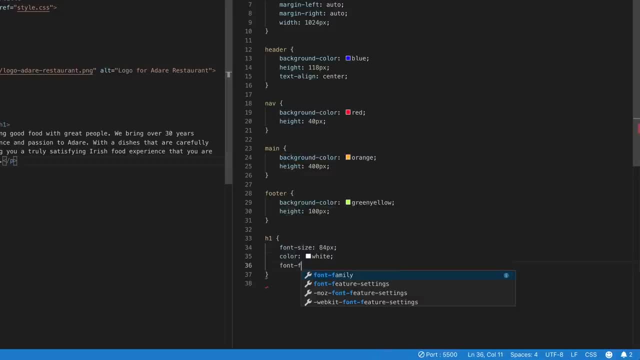 then come back in here and do another thing. In this case, kind of a big problem with this that we haven't done yet is the font family. So think of it as changing the font or the type from these default ones. 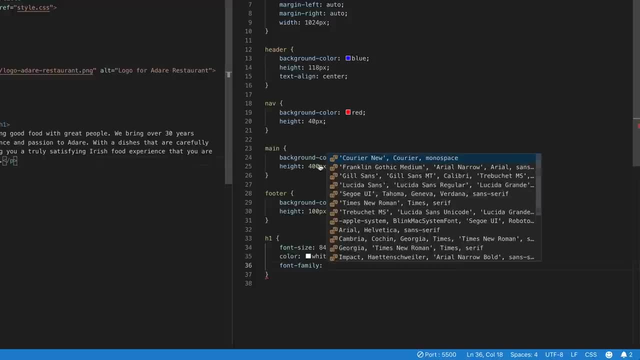 We're going to use the default ones. for the moment there's not very many, But we'll look at expanding that as we go through. So what I'm going to use is with Arial, I'm going from Times New Roman to Arial. Helvetica, Sans, Serif. 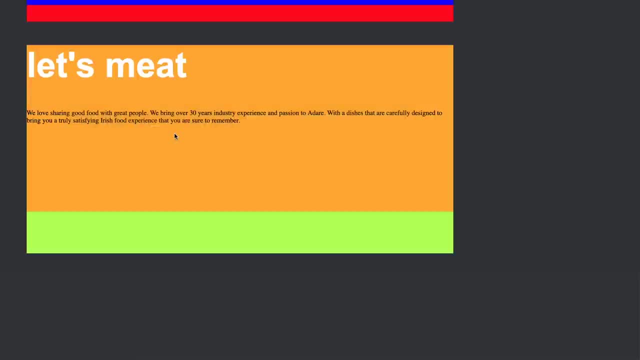 Let's hit semi-colon, let's save it, let's preview it. So, instead of it being Times New Roman, let me turn that off. I'll show you how I do that in a second. So Times New Roman with all the little feet. 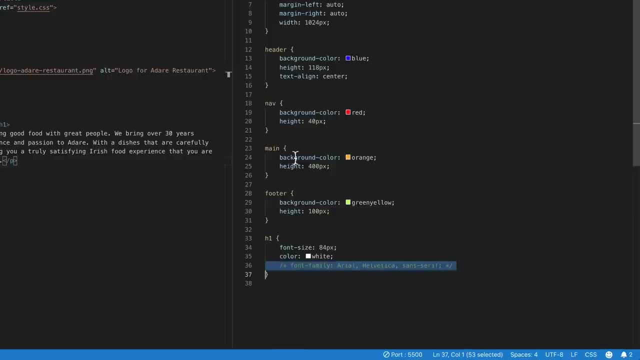 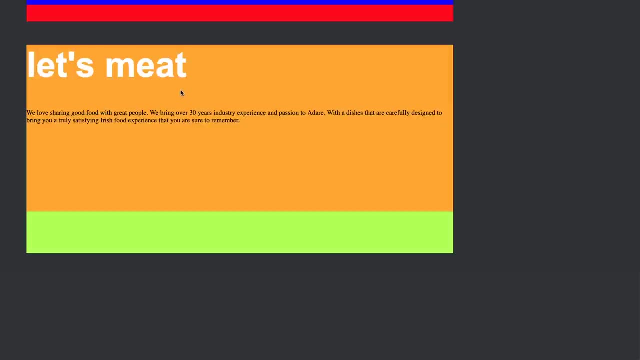 This is called a Serif font, So it has the little bits that hang out the side And if I change it to Arial, see no little feet. It's a Sans Serif, so without the feet, Did a couple of things there. 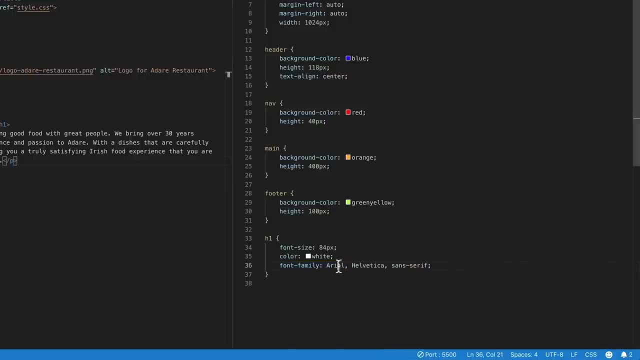 One was we'll do commenting in a second. this one. This is kind of weird. why is there three fonts? Say, you want Helvetica. Now what we're doing here is we're using what's called a default font. So what's happening is: you're not like putting Arial into this website. 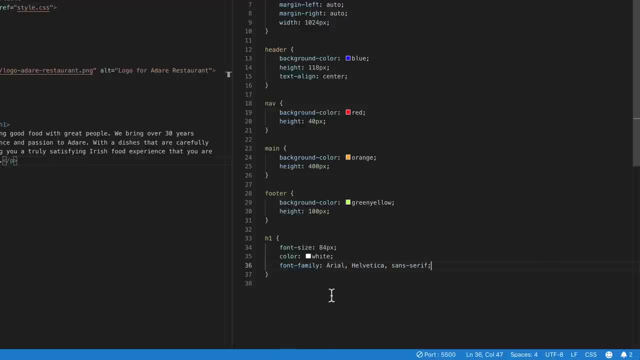 What's happening is, let's say, I built this site and our friend Bob Bob loads your website. What happens is his browser goes in and checks his system. So it checks Bob's computer to see if he has Arial and loads it. 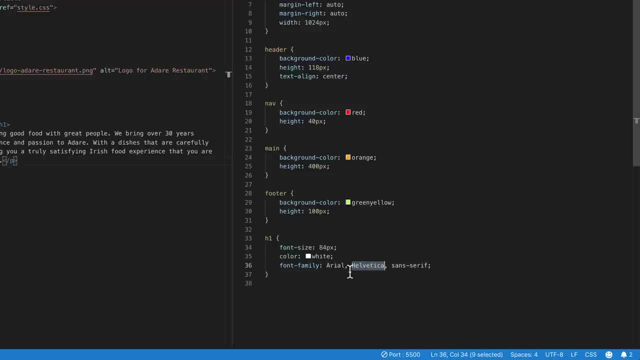 If he doesn't have Arial, it'll check for Helvetica, And if it can't find Helvetica, it'll look for this. Every computer has at least Sans Serif. It's like the default font for the core of the machine. So that's what you're suggesting. 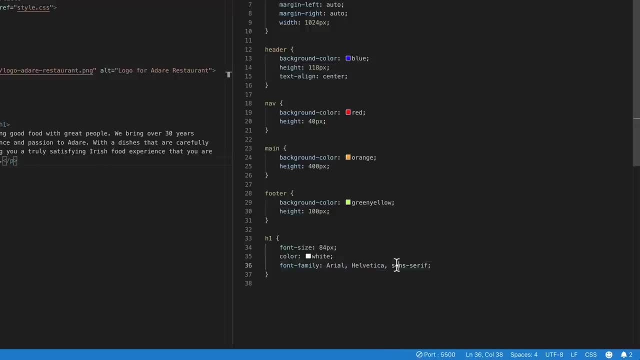 I suggest Arial, but if you don't have it, I suggest Helvetica. If you don't have it, I suggest Sans Serif. That's why, when you see some of these longer ones, we picked Arial, because it's easy. But let's delete all that type family colon, family space, hit, return. 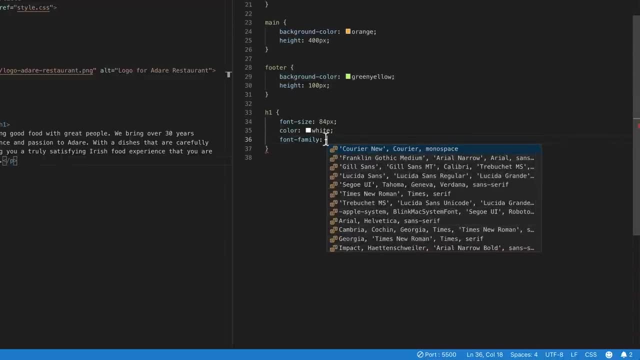 Now yours might not have done that. I guess I skipped over that as well. Let's go back. so when I'm typing in family, instead of hitting the colon, I click on this because it gives me all these cool suggestions. So looking at these guys, can you see? Gil Sans, Gil Sans, MT. 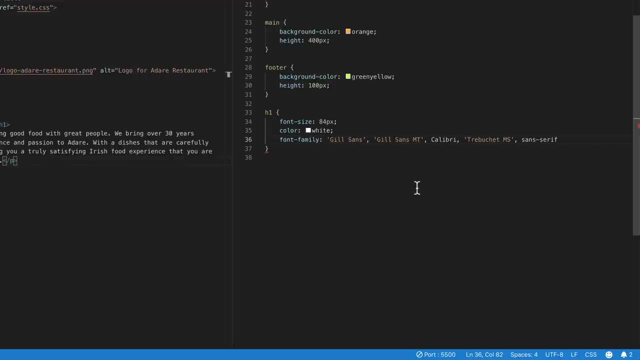 Calibri Trebuchet. there's lots in that list there, right? So it's saying: check Bob's computer for Gil Sans. If he doesn't have it, have Gil Sans MT. If he doesn't have that put in Calibri. 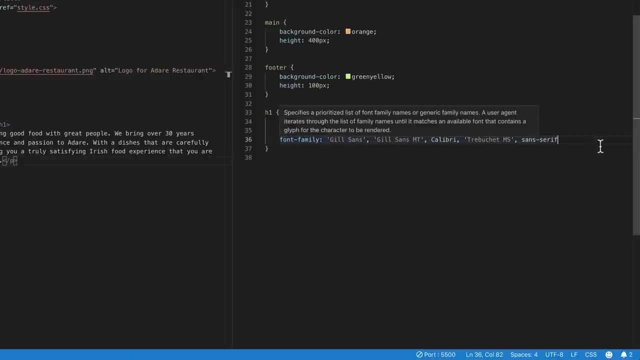 If he doesn't have that Trebuchet. If he doesn't have that, I give up and use the default font size, Sans Serif. You'll notice that some of these are white and some of them aren't. Some of them have these little marks around them, some of them don't. 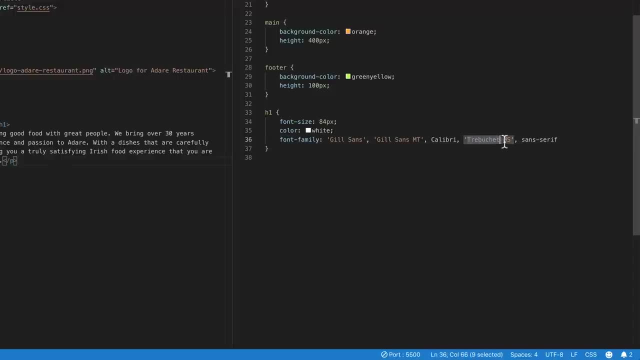 Single words don't need them. Words or fonts that have two like a space in between need these apostrophes? I'm going with apostrophes, little ticky things, So I'm going to go back to Arial, Because you could write in here, say you're a designer. 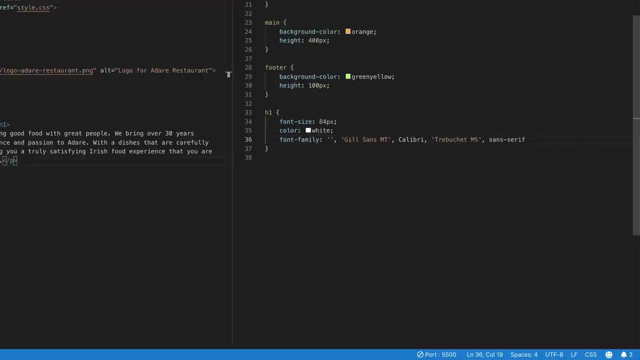 and you're like man, I would love some. I was going to say Lust. it's a font I was using today Out of context. it's not a. you get what I mean. Let's pick a more less suggestive font. 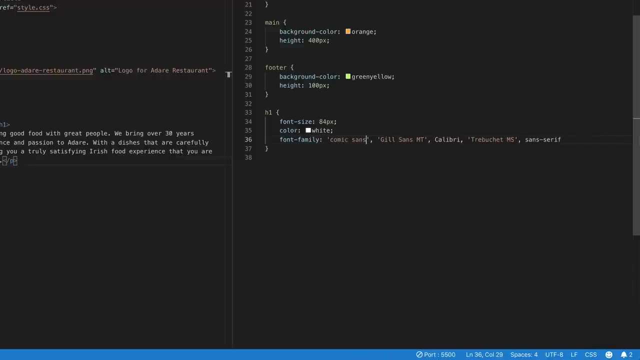 What have we got? Comic Sans. You're a Comic Sans lover, You could type that in there and it will probably load on most computers, Because most computers have Comic Sans. But if it doesn't, it'll have Gill Sans and then Calibri. 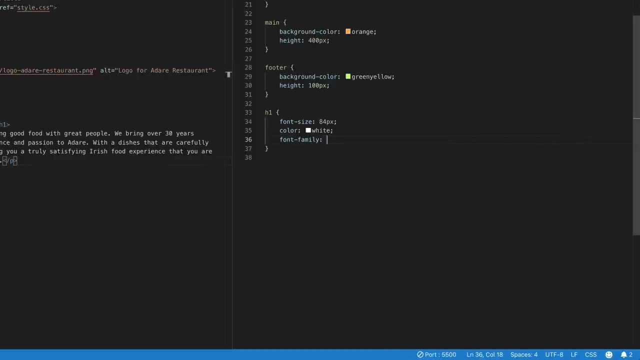 You get what I mean now, right? So I'm going to get rid of all of that and start typing in Arial. Make sure the semicolon goes at the end, And that's what it's going to do. The other thing: I snuck in there and I didn't mean to. 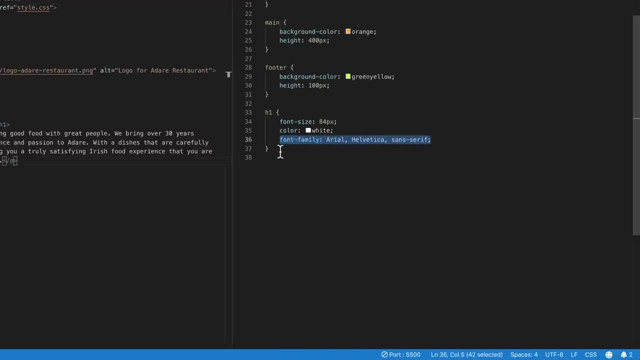 I feel like this will be later in the course, but I've kind of opened that box. Is that? I highlighted this and I wanted to turn it all off because at the moment it's working. it's Arial, So if I want to disable this, I can do a sneaky trick. 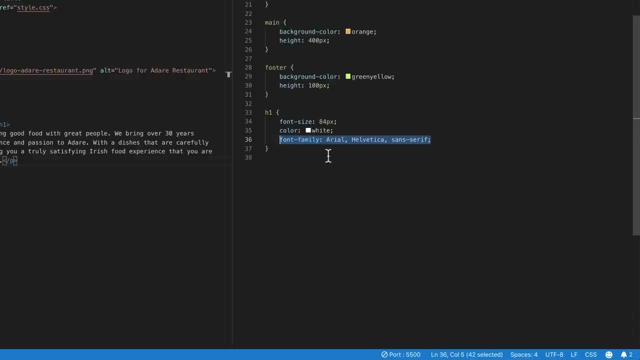 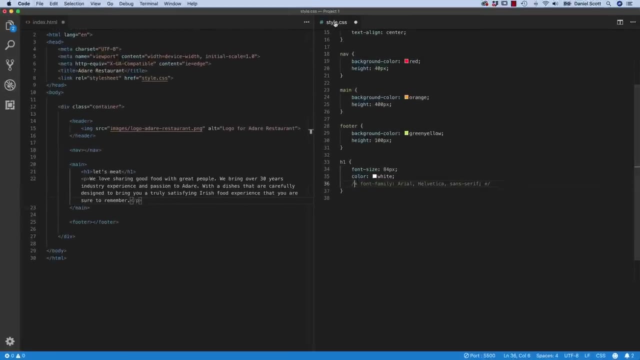 Rather than deleting it and then saving it and then checking it, you can kind of disable it momentarily And basically you need this syntax. You need to put a forward slash in front of it. This is for CSS only. You need to put a forward slash, then you need to put your asterisk. 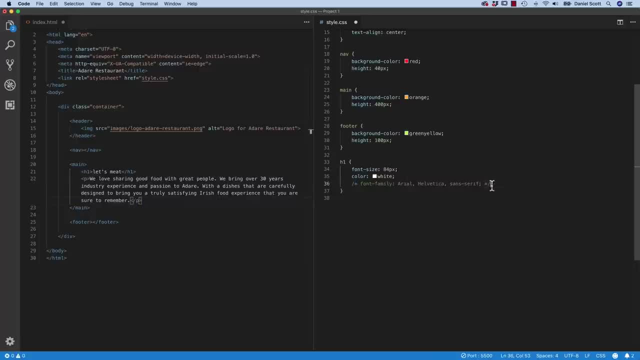 which is tied up with your 8, number 8 key on your keyboard And kind of the reverse of that at the end. So if you, if you put that around anything, so forward slash, apostrophe and at the end of it, apostrophe. 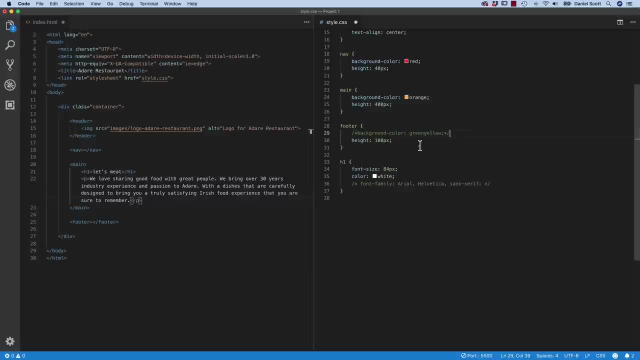 that's not apostrophe. that is your asterisk, sorry, Asterisk. forward slash. Can you see? as long as it's inside of that little group of characters, it will turn it off. Goes green and the browser doesn't know it exists anymore. 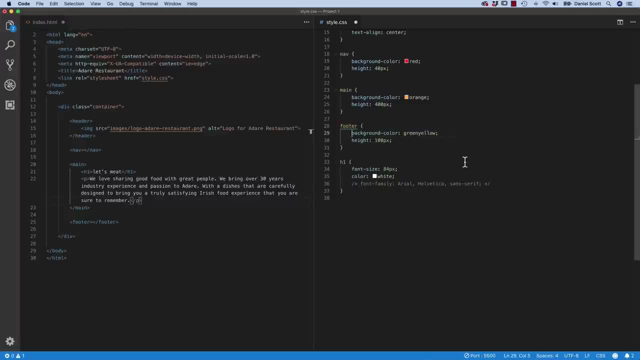 And it's just a handy trick. But you would have also noticed that I did it super quick. There's a shortcut, So it's a bit early for these shortcuts, but we're already there. So what we do is we highlight the bit we want to turn off. 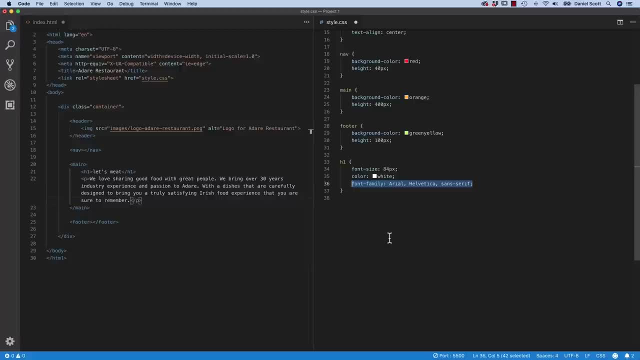 and we hold down the Command key on a Mac or the Control key on a PC and hit the forward slash button On my keyboard. it's down the bottom right of my keyboard. Yours might be somewhere else. Basically, you're looking for this key. 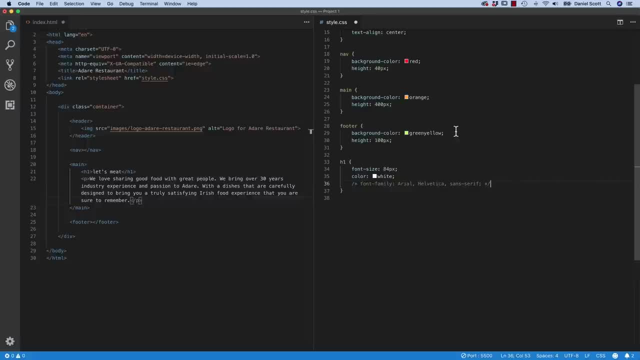 So hold the Command key and click it and it will automatically do it. It's really handy. Highlight it, Command forward slash or Control forward slash- All right, So let's move on and do the P tag. So P this one here. 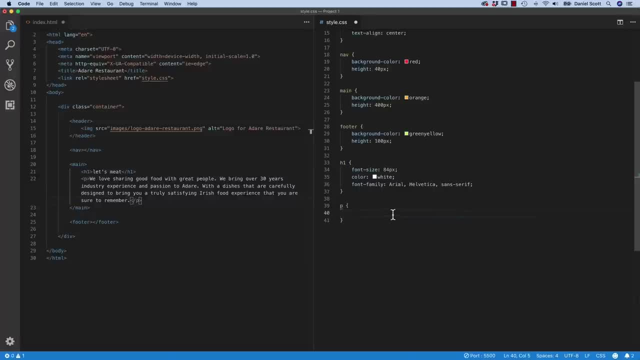 What do we do with this one? We did font size. I want all of this. My lazy brain says, just copy it. But the size is going to be different. We want the size to be 18 pixels And we'll leave the color and the font. 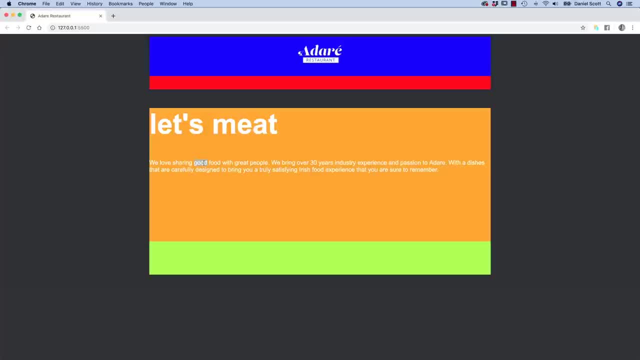 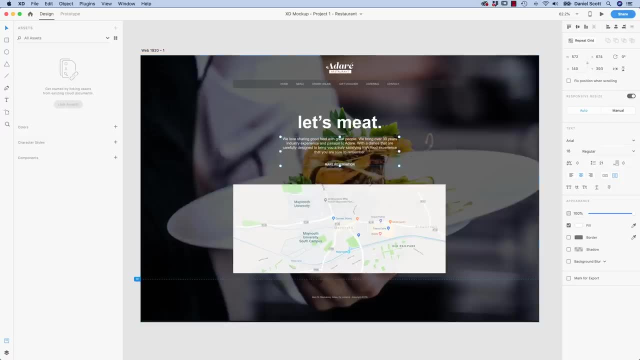 Let's check it. So there's now 18 pixels, it is Arial and it is white. Now the next thing I want to show you is we could now go through and say: because we want it centered right To match this, we want it all in the middle. 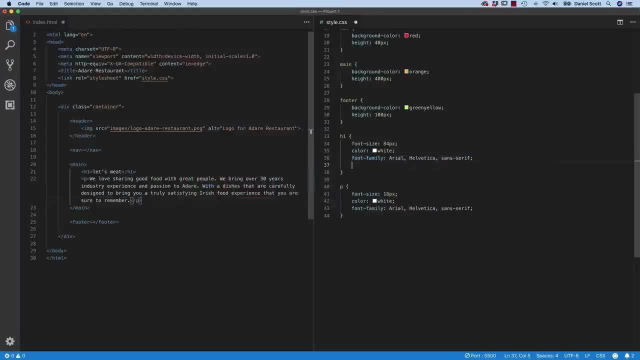 So what I could do, so I can go into my VS Code and I could say we did this one and this one makes a lot more sense. Text Align Center: perfect, We've done it for the H1, and it's done. 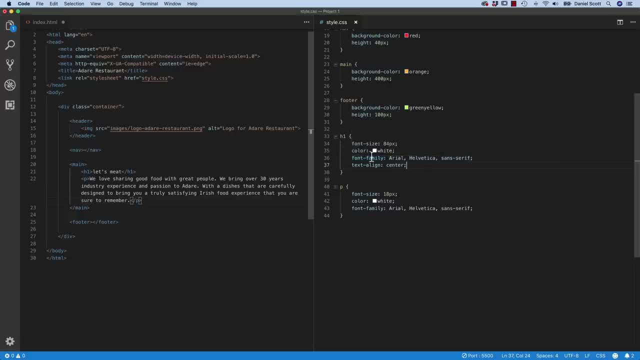 But it's not done for this bottom one, so it's not centered. So what we'll do to be- because it's all about being economical with your code- Do it once rather than doing it like 10 times. So the same thing. 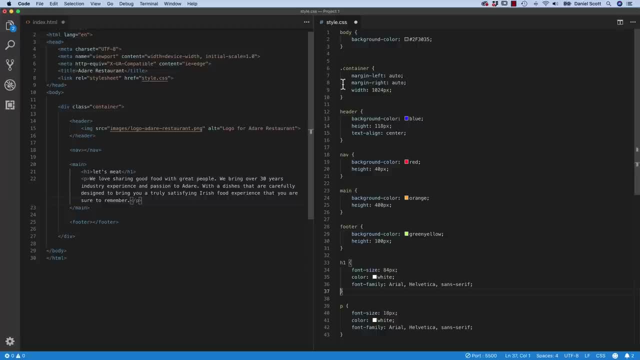 remember earlier on, we did the container, we did Auto Left and Right on the thing that wraps everything up. We'll do the same thing for this. So what wraps all of this up? It's that main tag. So where is it Main? 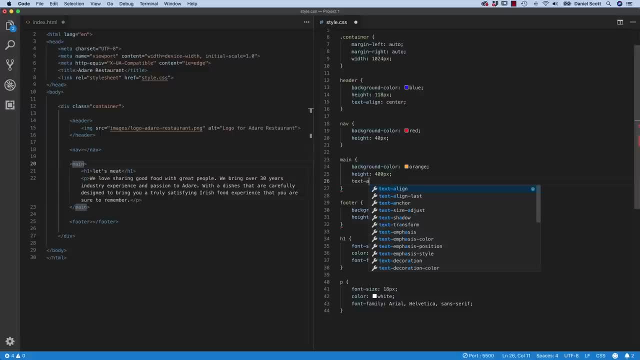 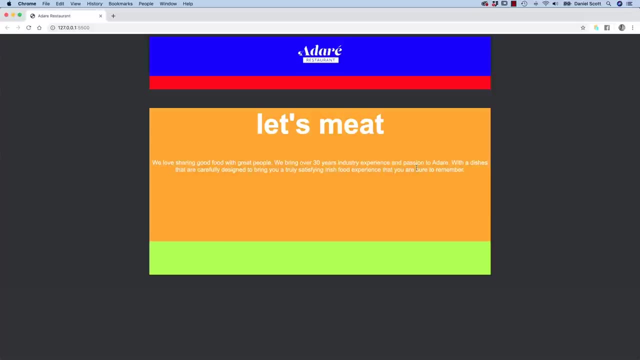 So if I do the same thing for there, I say: you, my friend, everything inside of you, be Text Align Center, It'll do the same thing. it doesn't really matter, but we're looking for like style points. as a front-end designer, 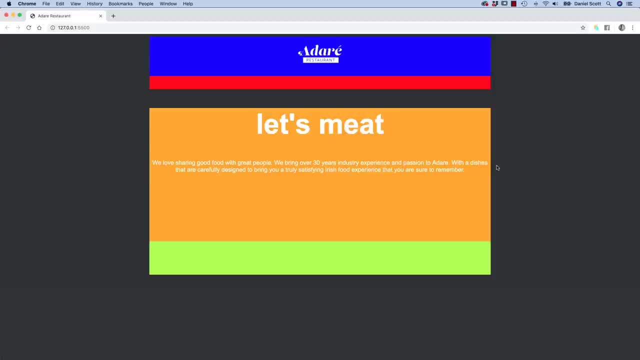 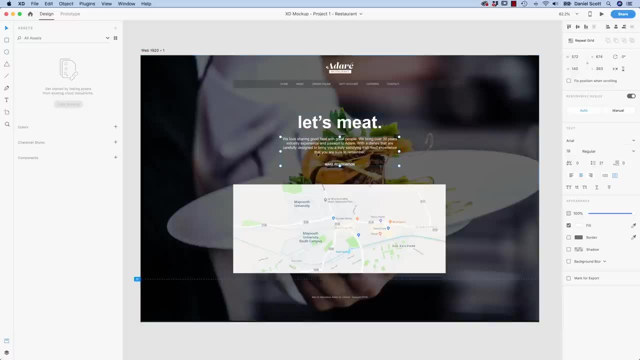 That's working. that's centered. that's centered. Let's work with the padding, Because I want a big chunk at the top and a big chunk on the sides. Now we could do it to the specific type again, but we'll do it to the container. 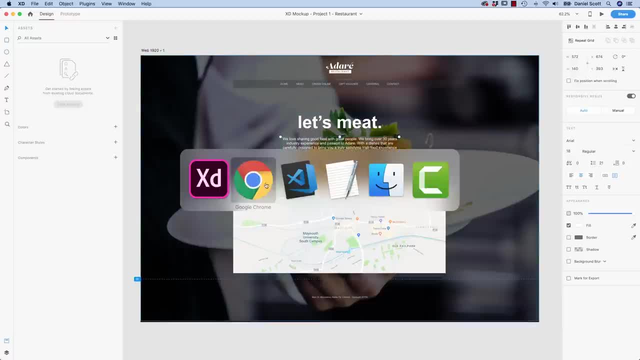 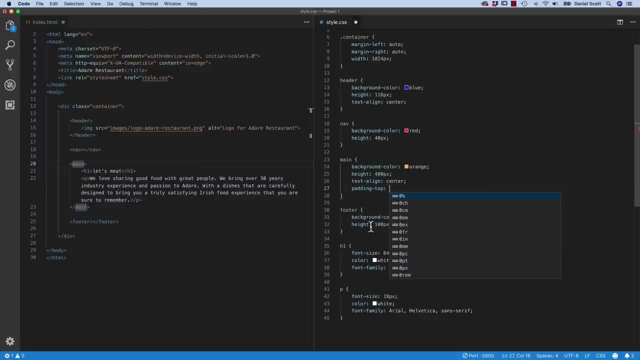 So we'll use, we'll add some margin to that main tag, So we'll do Main, we'll do Padding and we're going to use Padding to the top, What I want it to be. I've already worked this out: 80 pixels. 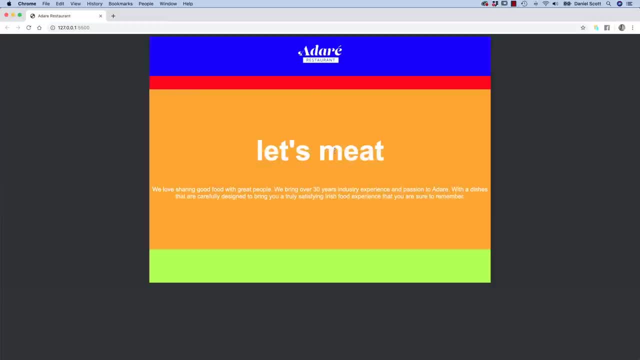 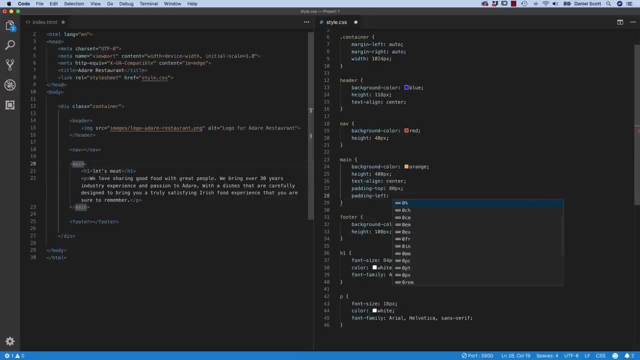 And let's check it. Awesome. so there's 80 pixels padding at the top. Let's do it for the left and right. So Padding left, In this case it is 240, 240, even pixels, And make sure it's semi-colon at the end. 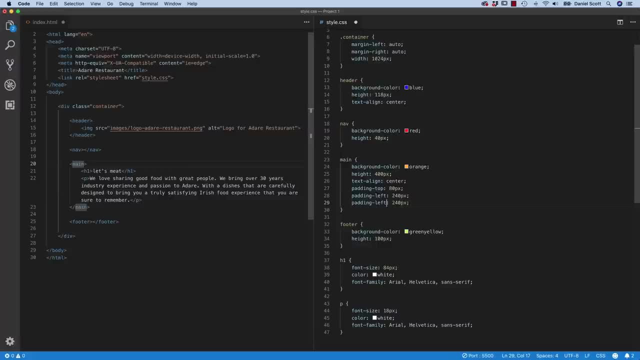 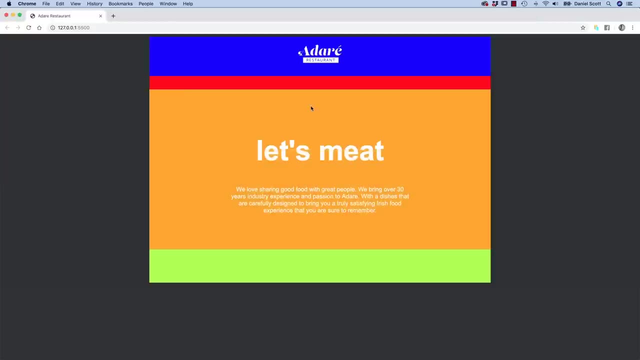 And do the same for right. Let's give it a test, see if we've broken it. No padding at the top, padding on the sides- nice. Now, throughout this course we're going to be looking. there's kind of two ways of putting spaces in. 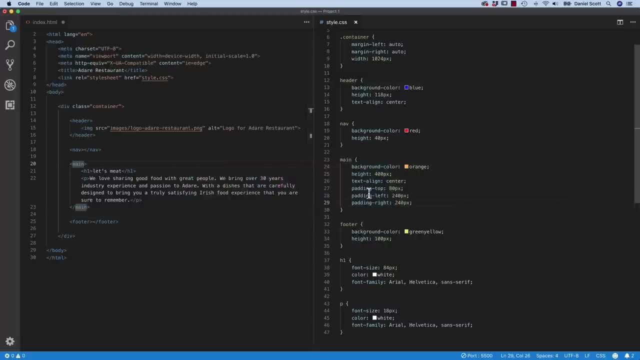 There's padding and margin, And this is a really good, I guess, way to show it the difference between the two. So what we'll do now is Main, we've done padding, Let's do the difference. So instead of Padding Top, we'll do Margin Top. 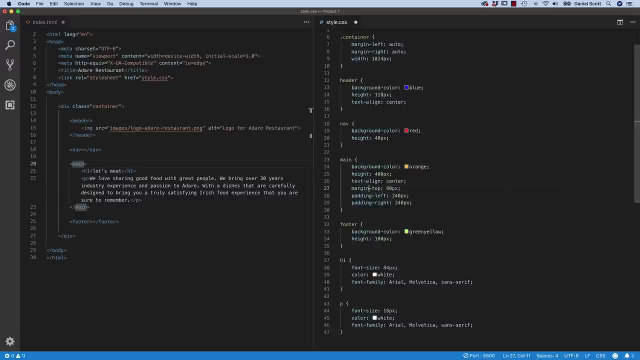 Because it can get confusing, like which one do I use? And sometimes it doesn't matter. So let's show at the moment, because it makes it really clear. So I've done Margin Top instead of Padding Top. Look what happens. 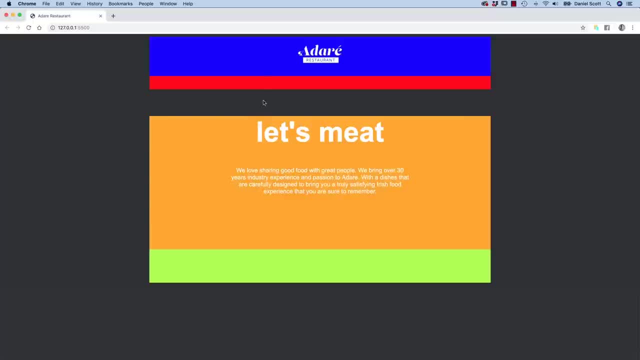 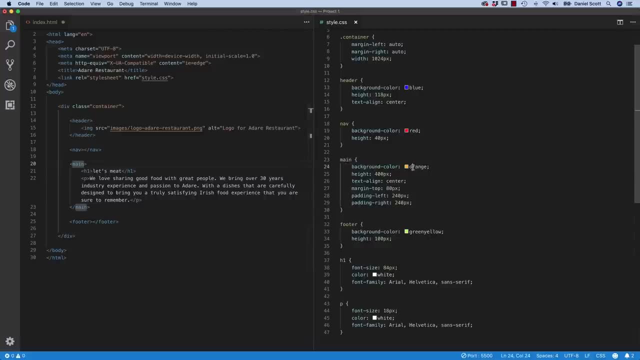 It works. the text is just as far down from that red box as it was for Padding, except Margin is the outside of this box Because we said Main B Orange, Margin Top pushes it away from the top of the box. 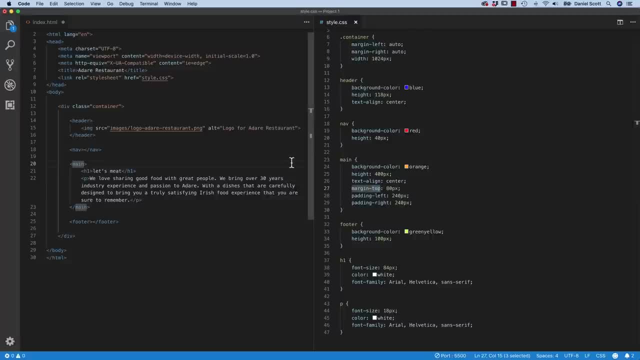 The whole orangeness comes down, Whereas Padding is the inside of the box, the internal parts, So the text will end up at the same place. but Padding is the inside of the box, So the orange. do you get what I mean? 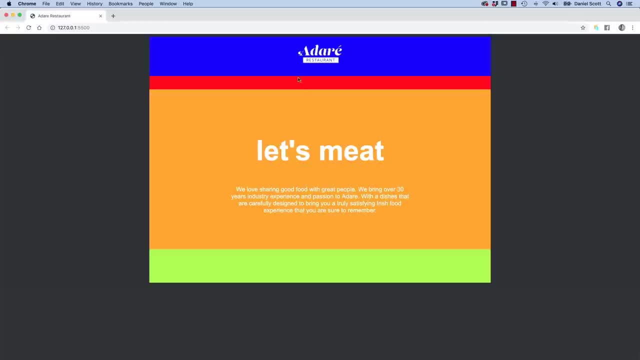 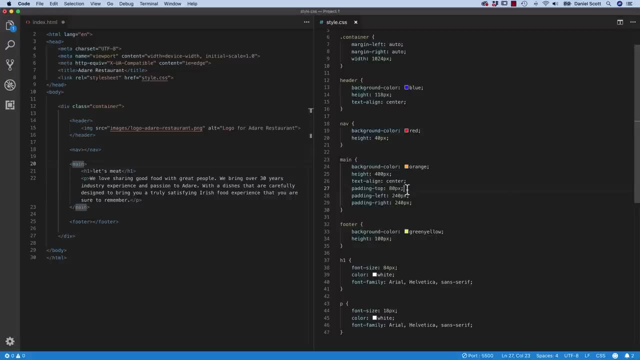 Let's have a look. So text: same place, But the box reaches to the outside Margin pushes the box down. so let's add a little bit more. Let's add Margin Top and Padding Top to hopefully clarify it. 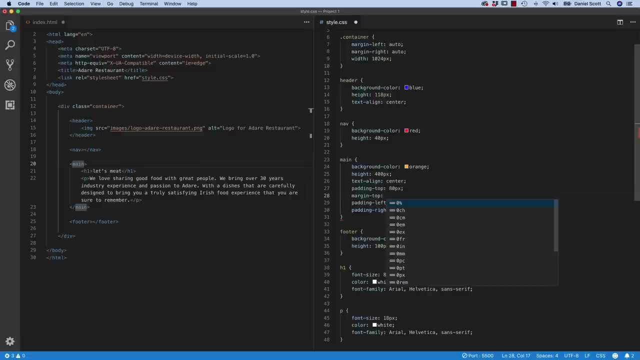 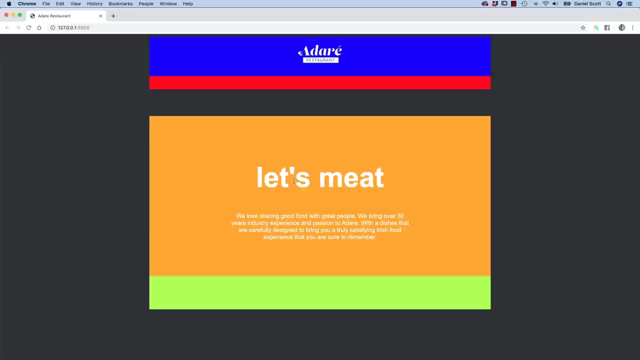 I feel like I've almost explained this right. We'll do this a few times, so let's do another 80 pixels to hopefully solidify this idea. Can you see? there is 80 pixels there on the margin. then there's another 80 pixels here just afterwards for this. 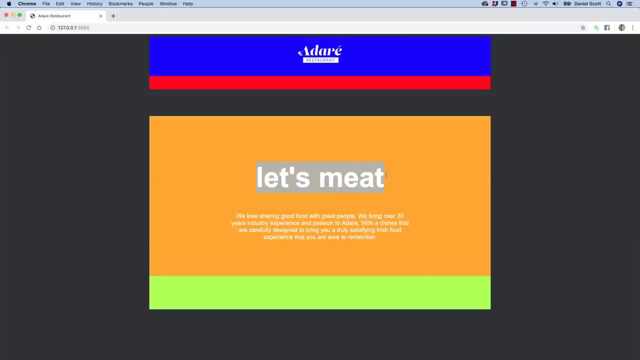 There's a little bit more here, because this font here has a little bit on it by default. So there's probably Padding on the top of this H1, by default, which will turn off later. but do you get what I mean? 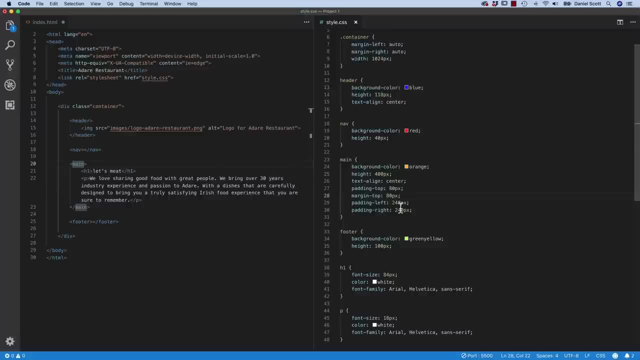 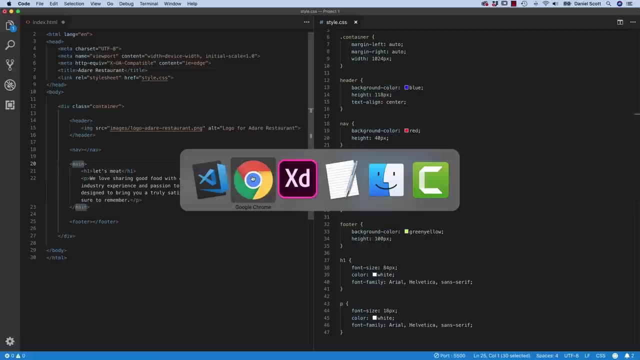 Margin on the outside, Padding on the inside. And then I also said: sometimes it doesn't matter, And it doesn't matter when you get rid of this background color, because we only use this background color right Just to kind of identify these boxes. 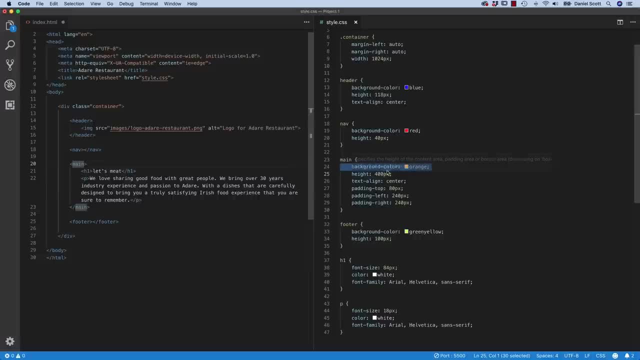 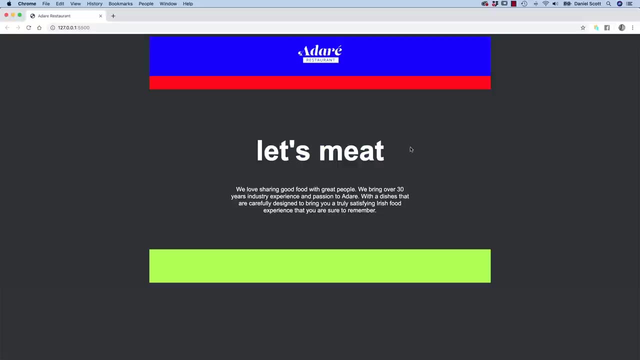 I don't want a big orange box or a blue box, So what we'll do is: in your margin, let's delete this, good bye, Save it. have a look, that's what I want. And now if I added margin or padding, 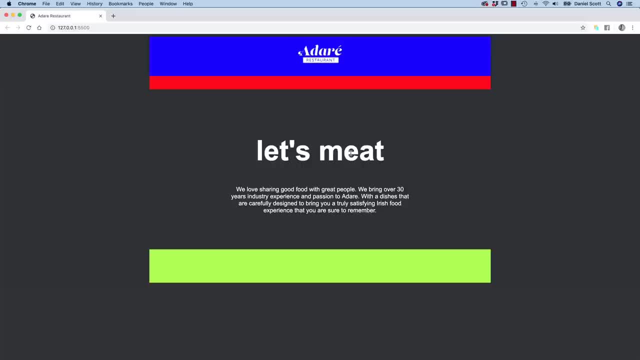 you can see, it wouldn't make a lick of difference, because the text would end up in the same spot and because there's no background color. you get what I mean. Dan, you've said it 10 times now. all right, we got it. 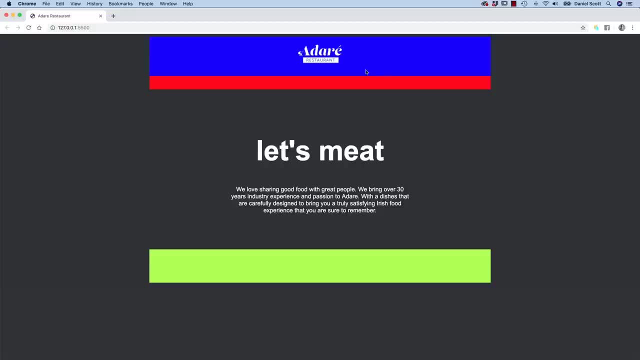 If you haven't, we'll do it again later on. While we're here, we'll get rid of the logo background. So where is it header? the background color blue. delete it. There we go, All right, last thing before I go. when I teach this thing live. 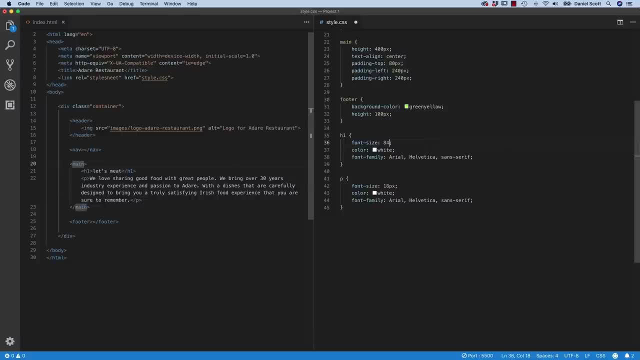 there's always one in the class. you might be that person. People forget to put the PX in, Save it, and you're like, hey, it's not working. I'm changing in the numbers and I'm making it up and down. 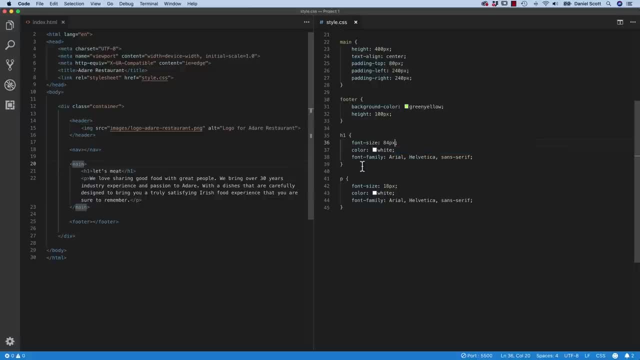 and it's not working. it's just because you forgot the PX, because it's not something natural, all right. So there we go. don't forget that. All right, that is it for this video. I'll see you in a second, in the next one. 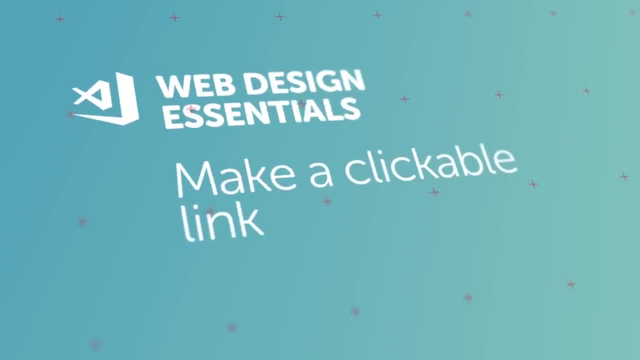 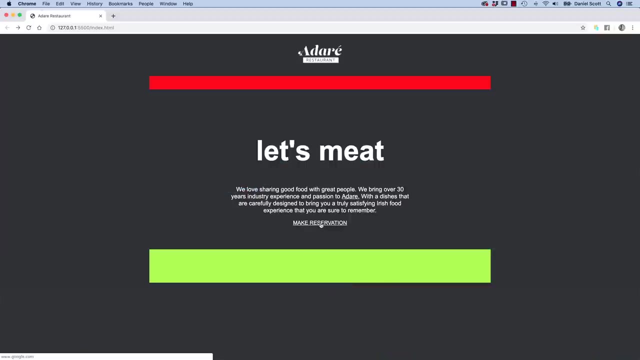 Good afternoon. it is time to talk about hyperlinks. Sometimes they're called hrefs or A-Tags. they are clickable links Like this. make a reservation, we're going to add it and when I click it in this case, it's going to open up a new tab. 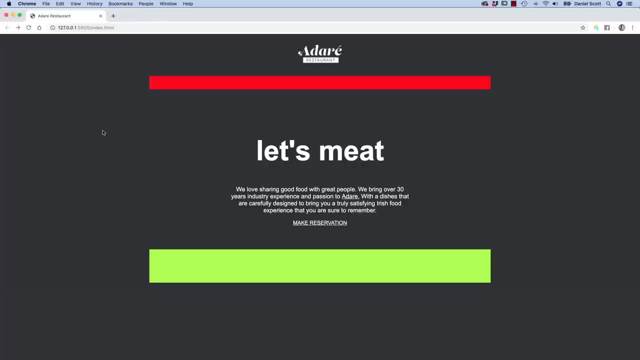 It's going to go to Google because I haven't got a good place for it to go to. But that's what we're going to do. We're going to do one both by itself and in line with the text at the top here. 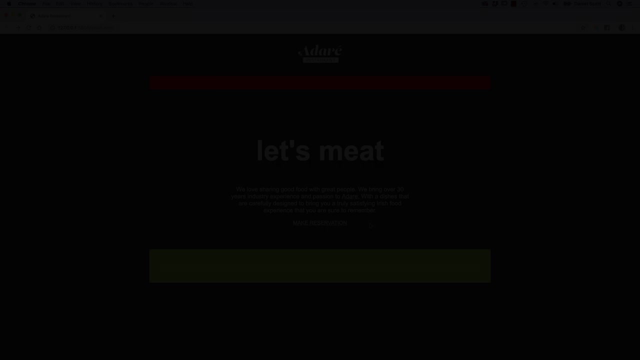 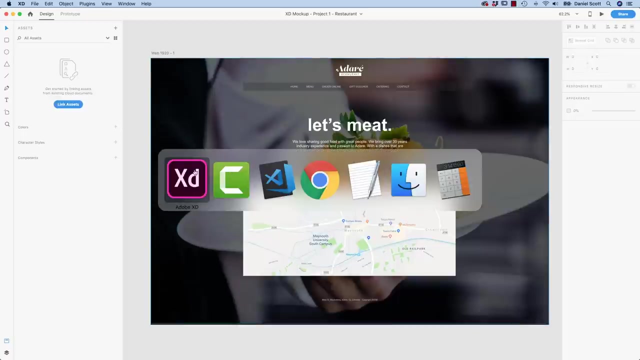 Let's jump in and work out the ways of the hyperlink. All right, to add our link. it's going to be this fellow here called make reservation. It's called a hyperlink, so let's add it to VS Code. It's actually referred to as an href. 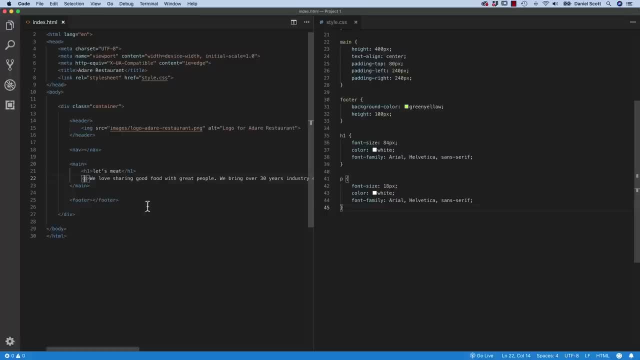 So where do we want it? I want it after my P tag And you'll notice my wrapping's turned off. It turns off every time you close the program down. So in between videos I was going to go home and then I was like, no, I'll do one more video tonight before I head home. 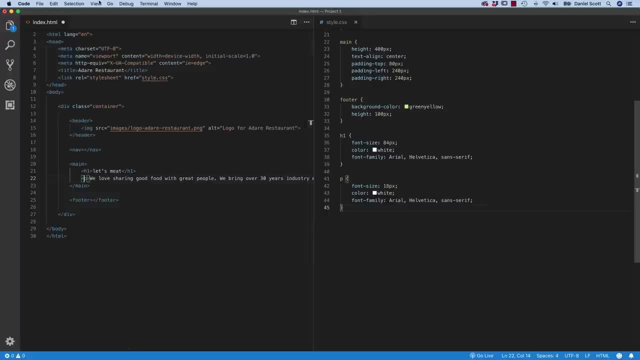 So I close down VS Code, open it back up and wrapping's gone. And it's, I guess, a good thing to show that it's got a pretty easy shortcut, if you can be bothered remembering it. So I'm going to put mine just under the P tag here. 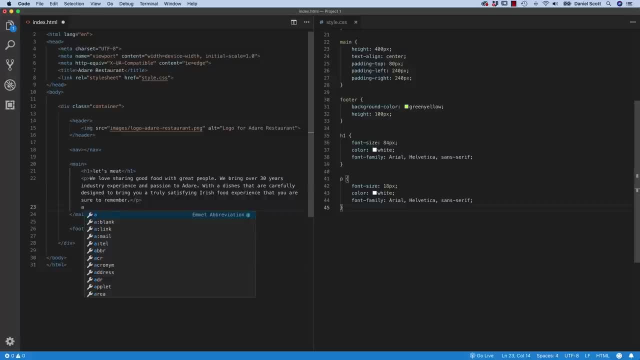 And what is it? It's an A tag, So if I type in A and hit return, it puts in all the stuff we need. So it needs a hreference And in between, the quote marks, like most of the things in here. 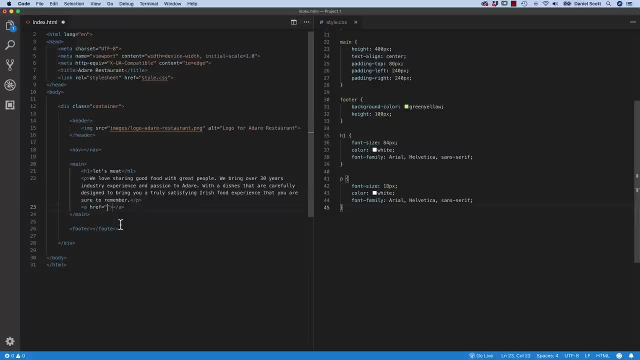 is where we put the link. we want it to go, So in this case we'll get it to go to. I'm going to use something in Yelp, So I'll pause it here and I'll be back in a second with a link. 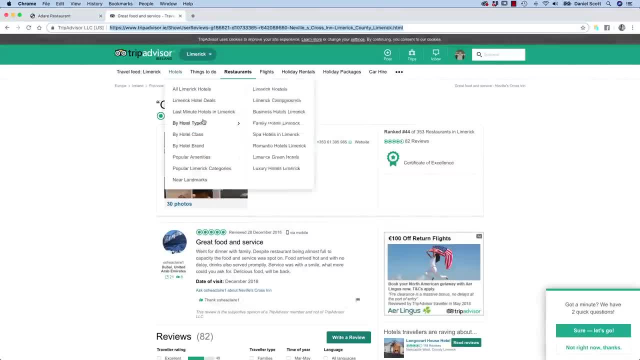 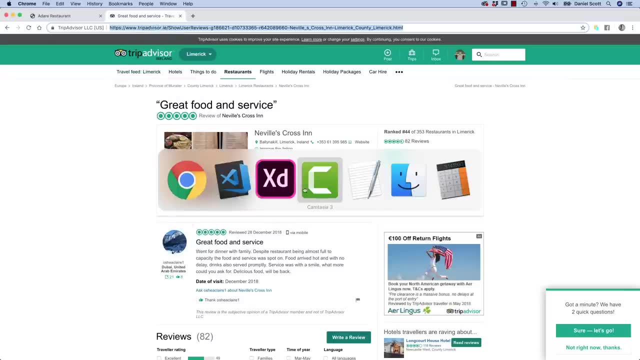 All right, I'm back just with a random restaurant I found in a deer Random. I went there once I really liked the food- Neville's Cross Anyway- so I've grabbed a link for us to go to. so we're going to go back into Visual Studio Code. 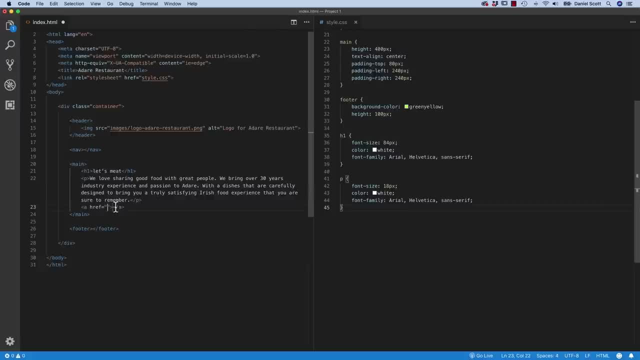 So when somebody clicks this button it's going to go where You could type in http//. we should have just done that www. You need all the junk. it's best to have all the junk, So http//www and the URL. 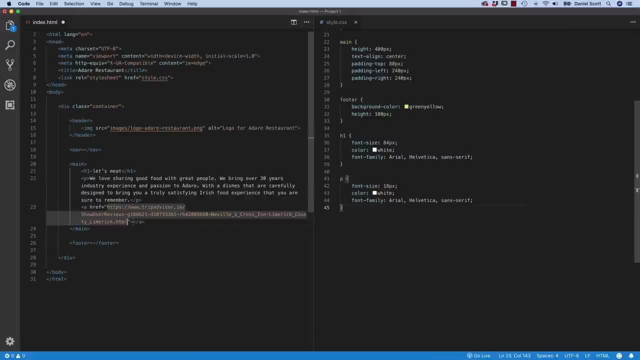 That's where this button's going to go, Because I went to all that hassle and found a link. I'm going to type it in, even though it's really big Now, at the moment it's not going to really do anything. 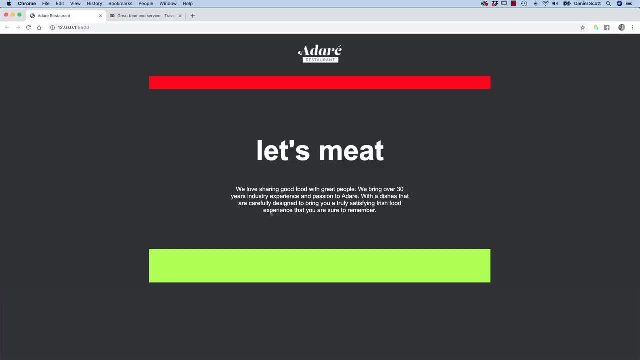 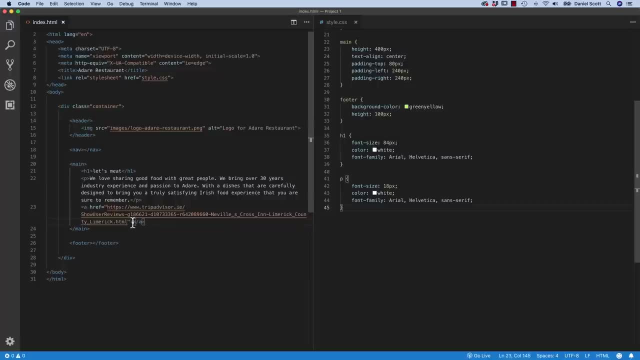 So I'm going to save it Preview. let's have a look. So it doesn't work. it needs some text and the text goes in this A tag. So there's an opening and you can see the two little curly braces. 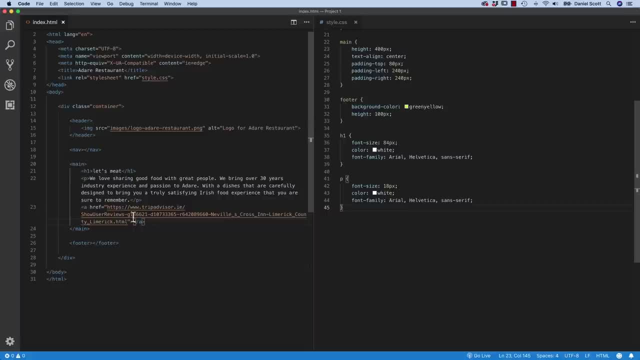 Like between the two H1 tags. we're going to go between these A tags And we're going to have Make Reservation. that'll work. So I just typed in it can be anything, just text, like the P tag. 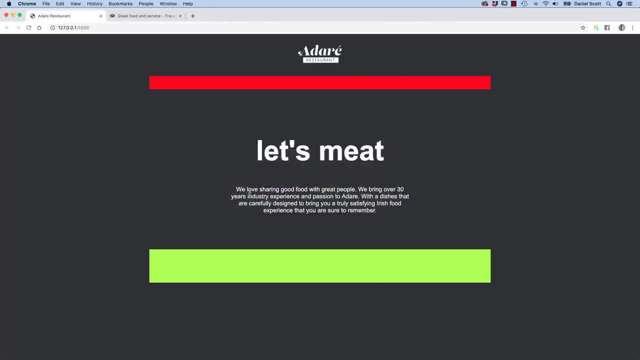 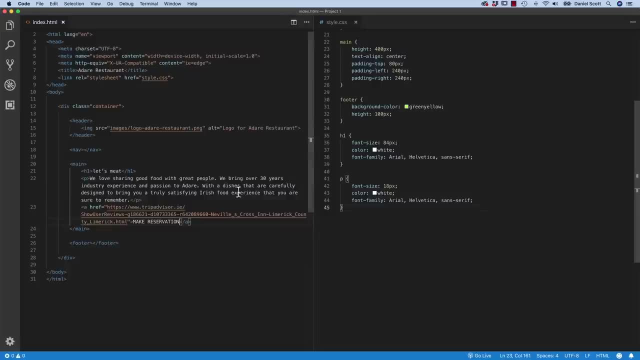 But because you wrapped that up in this HREF, HREF tag: nothing happens. Hit save now nothing happens. This brings up a good point. Remember: I said I closed down VS Code, So I closed down VS Code, but I didn't close down this Preview window. 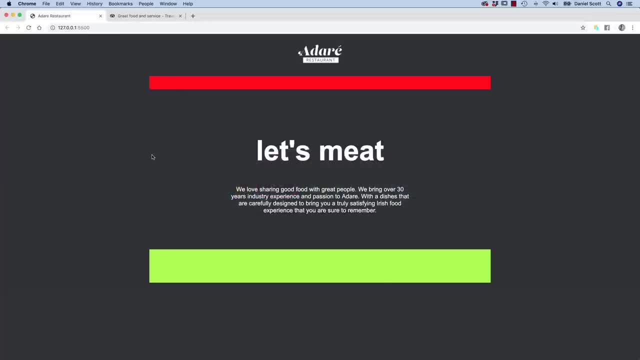 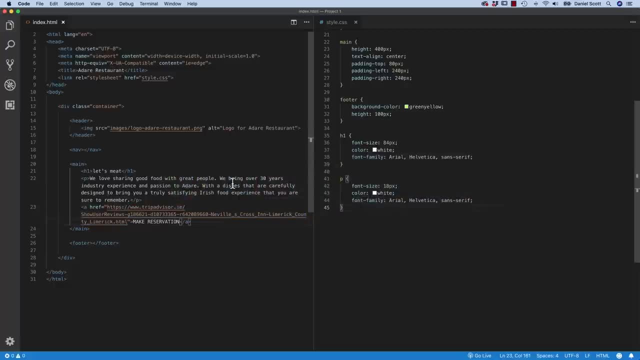 Remember the what's it called Live Server. So this brings up a good point. I just assumed it was still connected. I know it doesn't, but I forget. So I closed down Visual Studio Code, opened it back up and that connection broke between those two. 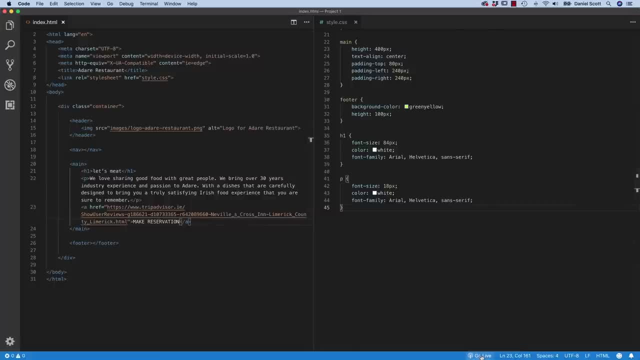 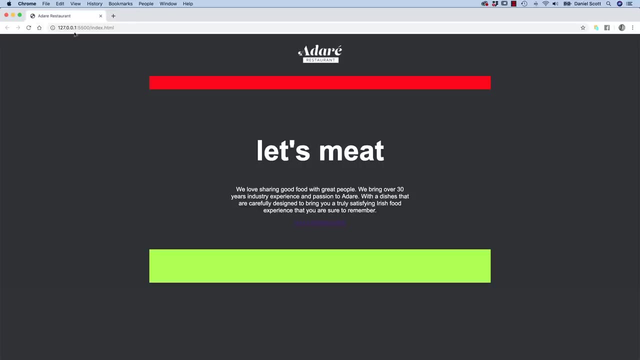 I'll leave this in the video because it's a good point. So what I'm going to do is go live again. It's going to start up a new page. There's my old one that's no longer connected. I'm going to close it down. there's my Trip Advisor. 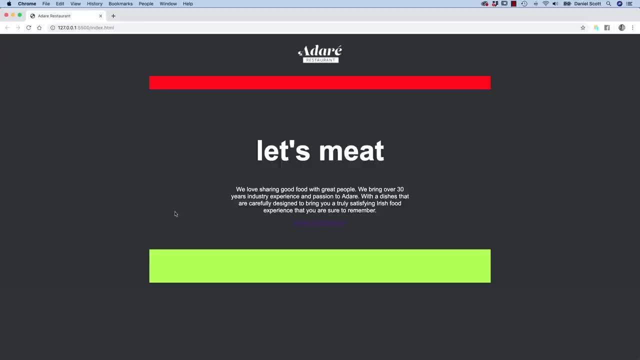 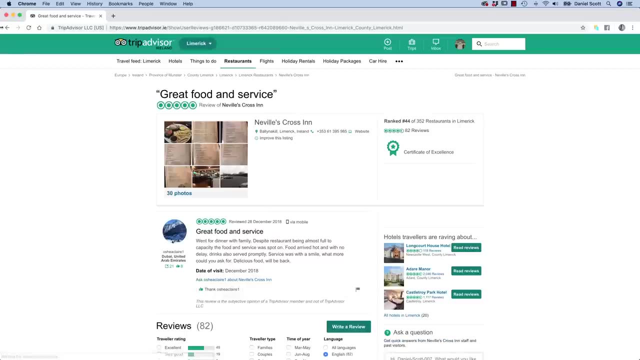 And now it's connected. there it is. Now it could be blue- mine's purple, because I've been to that link before- But give it a click, it loads it up and there's that lovely Trip Advisor. So that is how to add a URL. 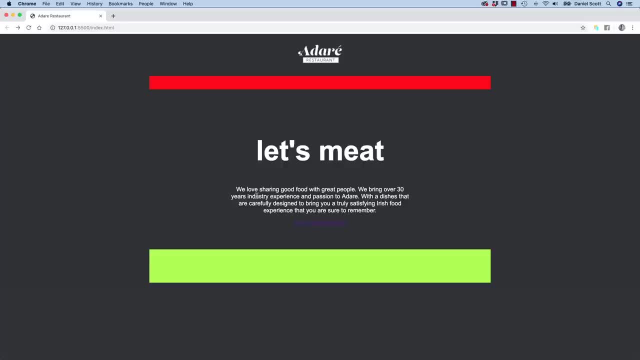 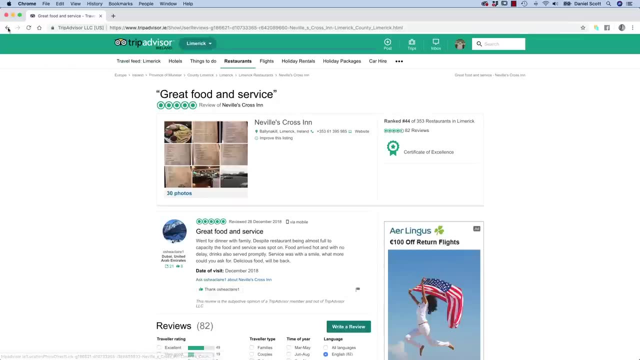 We'll do some styling in a second as well. One thing you might want to do, though, is, when you click on it at the moment, it clicks on it and it's actually going to, it's replacing that page with this, So you can't really go back easily. 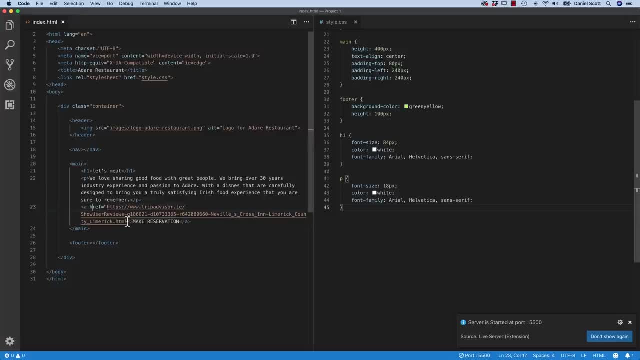 So what you do is there's an option in your Ahrefs. What we might do is get rid of that whole. I feel like it's made it look ugly. I'm all about making it look nice for you, So let's just put in Google. 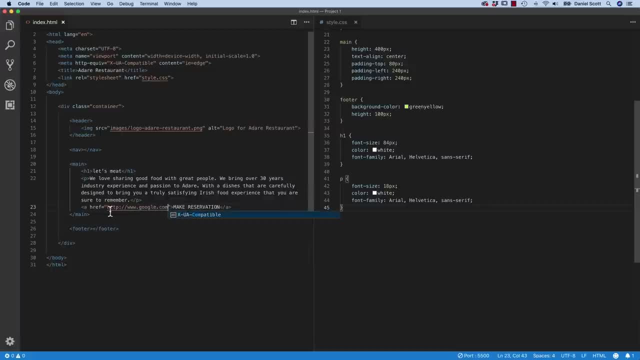 Googlecom. So all you need to do is after the Ahrefs. so A tag is the thing we're using. Ahrefs is just a page, It's just a part of it. So after this, we're going to add something called. 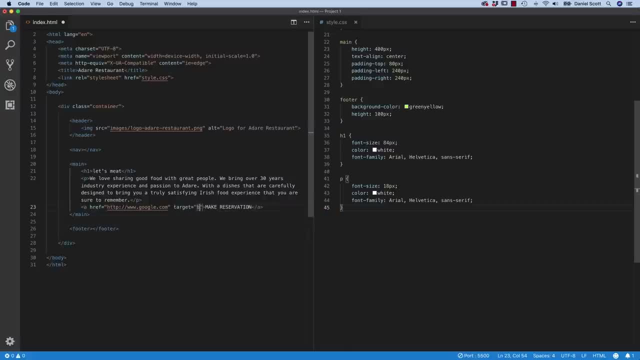 target equals blank. Actually, I think it needs to be underscore blank. I need to double check that. let's give it a preview, Trying to guess here. remember, Save it all, preview it in a browser And let's give it a click and it does work. 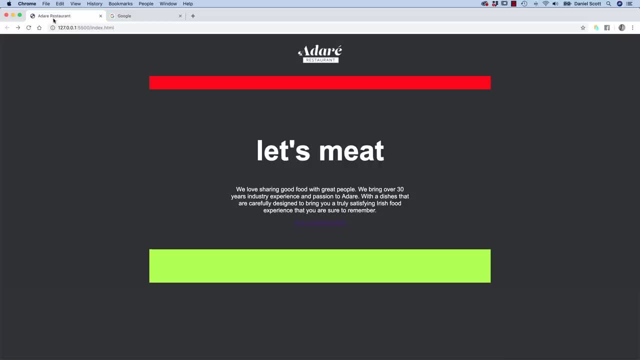 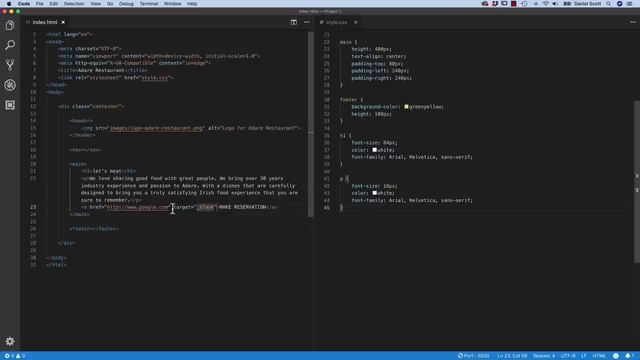 So if you add that underscore blank, can you see what it did? It left that tab there and launched this link in its own tab. Sometimes it's its own window. you can't really control that. But if you just add target blank it can do that. 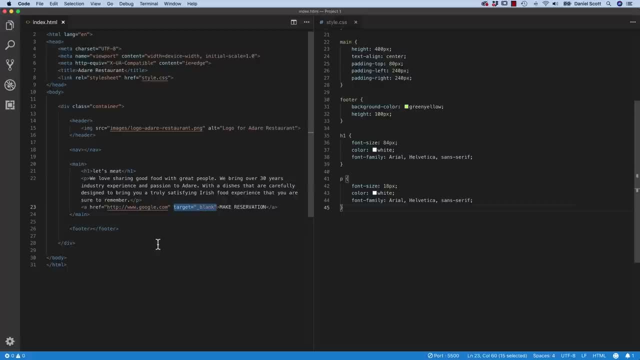 In this case it's not what I want, but it's going to be something that I'll tie into this video so you can come back to it. I'll leave it in there. The other thing to note is that when you are doing URLs, 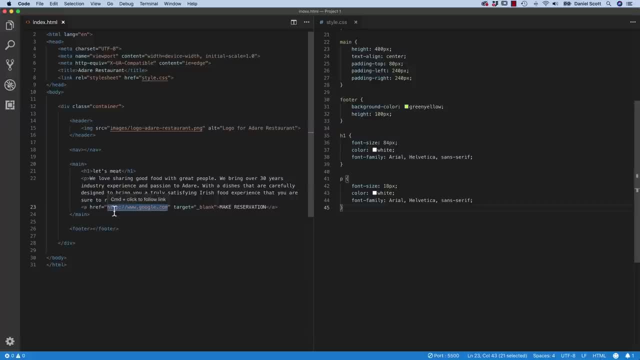 let's say, this wants to go to another page on this website. Often you don't know what that is yet. You're like: is it going to be the About Us page, html? but you don't have that yet. So what people tend to do as developers is you put in a hash. 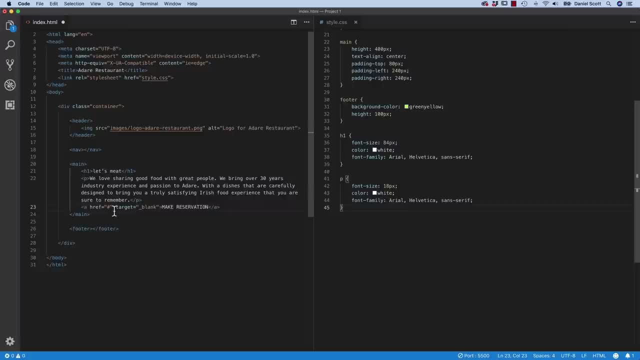 Up near the 3 key, The pound symbol, hash, whatever you want to call it. What that does is that's a really good placeholder. It's kind of clear that that's a placeholder And if you leave it blank, often what can happen is it can throw an error. 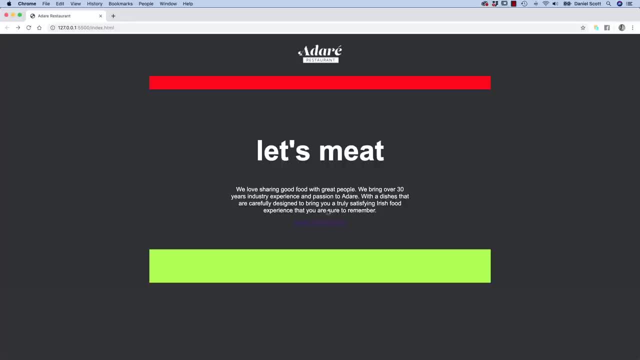 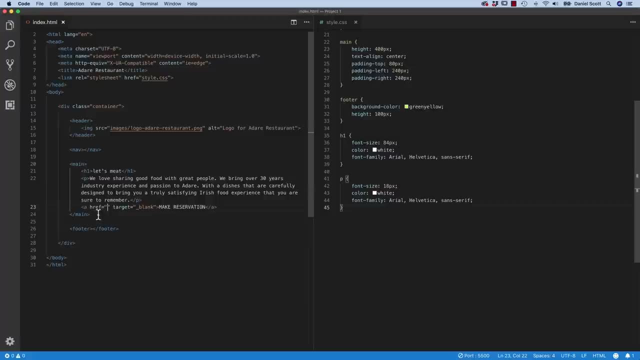 So if you leave it, I'm not sure if Chrome does an error anymore, let's check. Just kind of launches it in its own window. that's fine, It's working all right. But some browsers freak out if there's no link in there. so you put in hash. 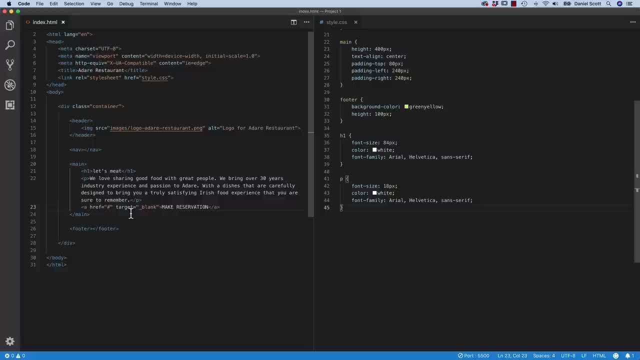 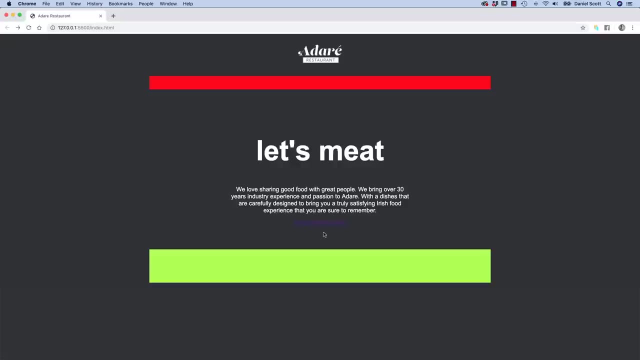 I show you that because that's really common to have. You might get a template website from someone else and they've left hashes in there and you're like: what are those? They're just placeholders so that when the button's clicked it doesn't throw an error. 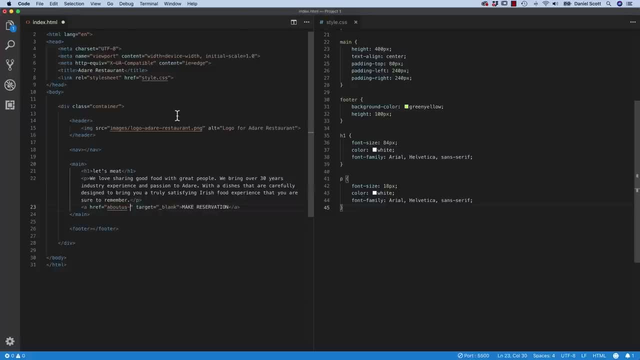 So we'll leave hash in there. Now let's go back to Google. Now let's style this. I want you to pause right now and do a little pop quiz. How would I style this? Just think it through, you don't actually have to do it. 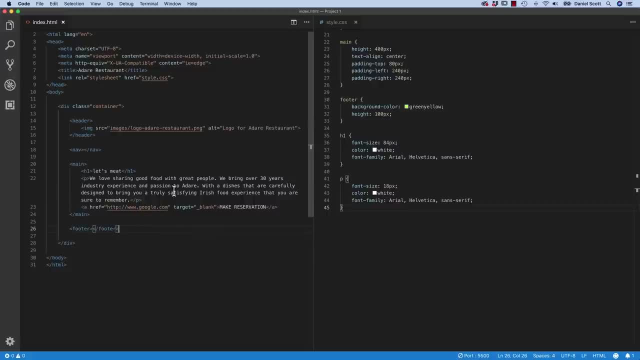 You could do it. that'd be cool, But I want you to see if you can style this thing. The first thing I want you to do is make it white, because it's purple at the moment. sometimes it's blue, but if it hasn't been clicked yet, I want you to do that. 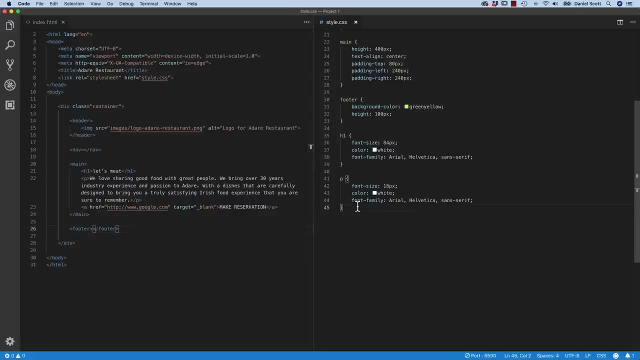 Did you have a think? Don't worry, it's early for thinking Or late in the afternoon for me. So it's the A tag. So A over here I'm going to say color please is going to be white. 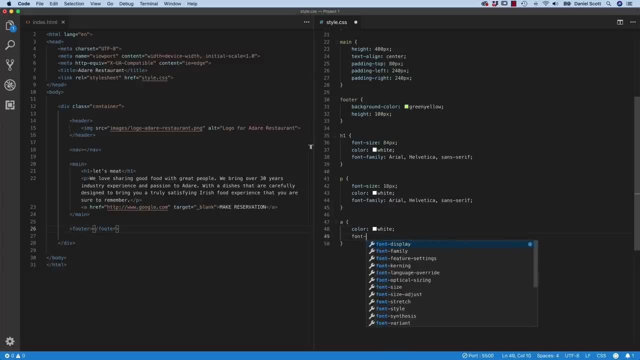 Now it's going to change the color of it And also we'll say I want the font family to be the same as the rest of it. So I'm going to type in all that. You can see now that I'm not going as slow as I did in the beginning of the class. 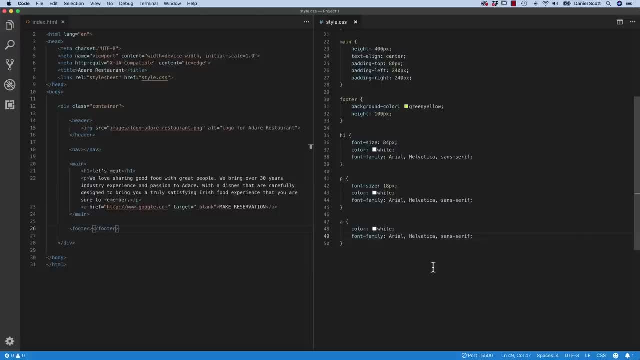 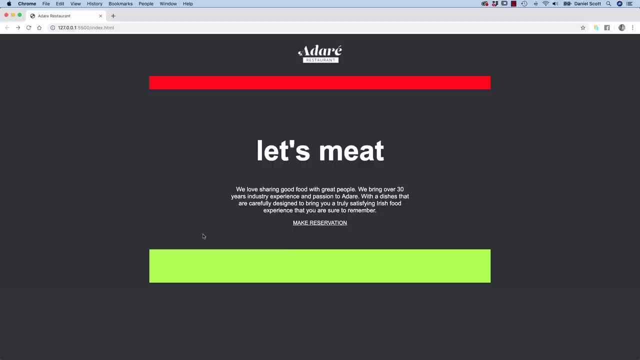 you can actually add code quite fast using all those helpful little hints. If I'm going a little fast, sorry, But we've done that a few times now Let's have a look. it's the right color, it's the right font. 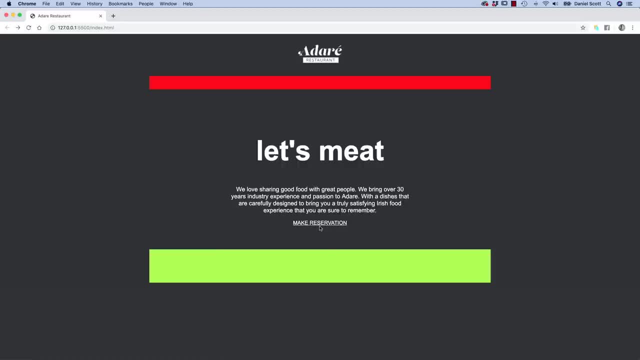 And we're going to leave the underline because I want it here, because I feel like sometimes if it's not very clearly a clickable button, you need to leave the underline. But let's say it's not and you want to get rid of it. 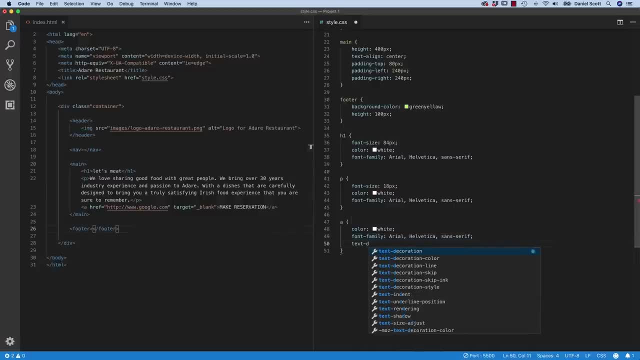 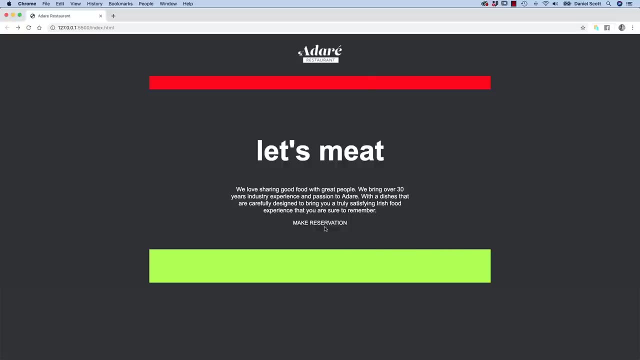 It's a weird thing. it's called Text Decoration. Kind of makes sense, but it's also kind of weird. And you want to set it to None, So Text Decoration: None. we'll get rid of the underline there. I want the underline. I'll leave this in the code here for you. 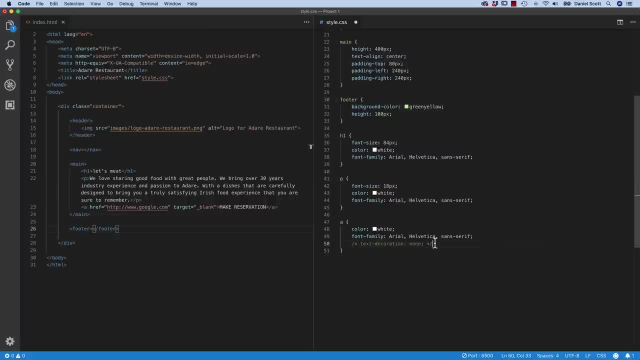 So I'll just comment it out. I'm going to do that a little bit more in this course, so that things that I've shown you will be in the saved completed files, even though I don't want to use them myself. Now. the other thing to know about this hyperlink: 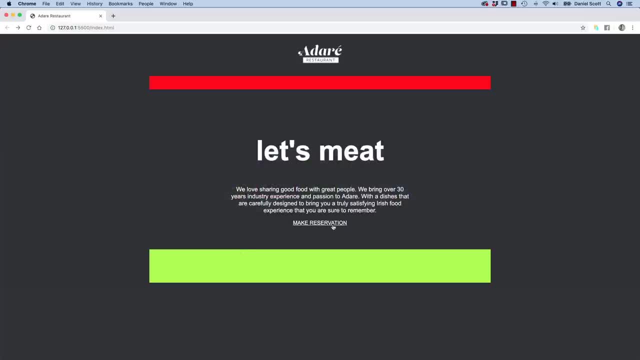 we did it as its own kind of like separate tag, So it's ended up kind of hanging down the bottom here. Let's say: you want to make this word like the word Satisfying a link. Let's use the word Adair. 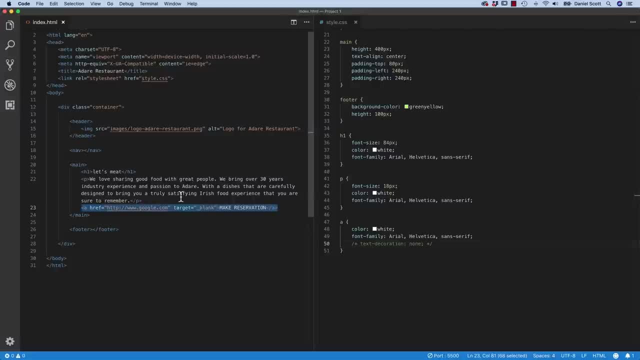 So people can click on it and it goes to a map of Adair. So where's Adair? So I'm just going to put some spaces, just clear a hole. I don't want there to be spaces, but I want to make it clear for you. 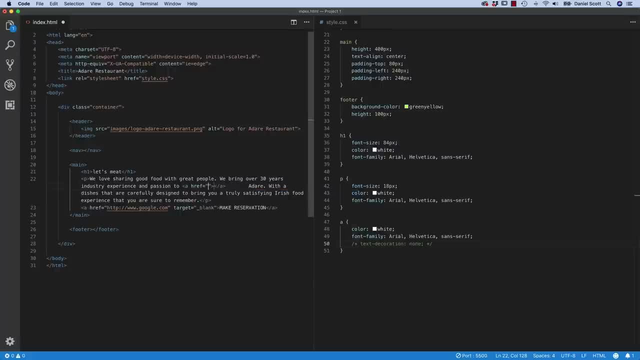 We do the same thing: A tag, Just an A, and that return puts it in there. Where's it going to go to? I don't know yet. it's going to go to Hash And inside the brackets here, what I want to appear. 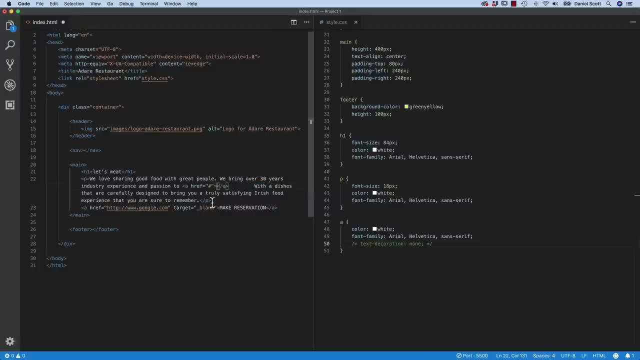 I'm going to grab this. come here, Adair. It's going to go inside of there. Let's save it. let's check it. You can see it's underlined. It's been told what to do in terms of the A tag. 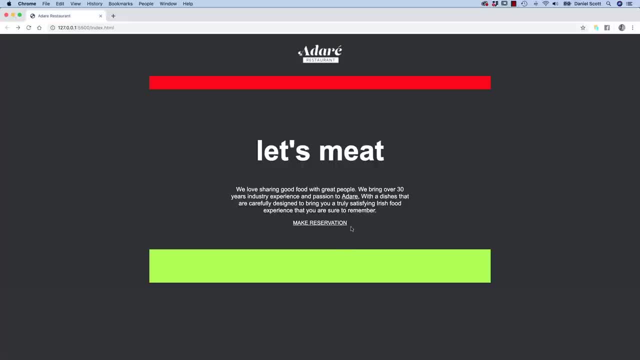 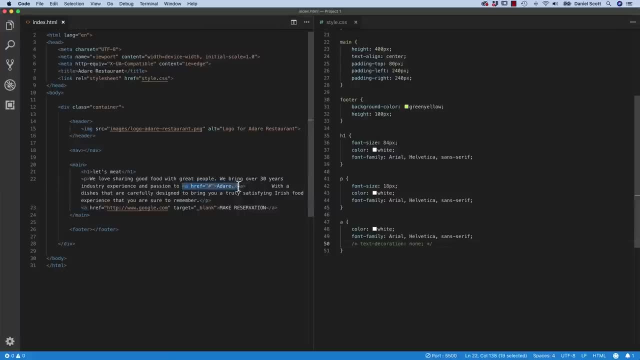 So the A tag still refers to both this one and this one And it's adding the underline and it's in the text. So this one is called Inline. This is an Inline href or an A tag or a hyperlink. 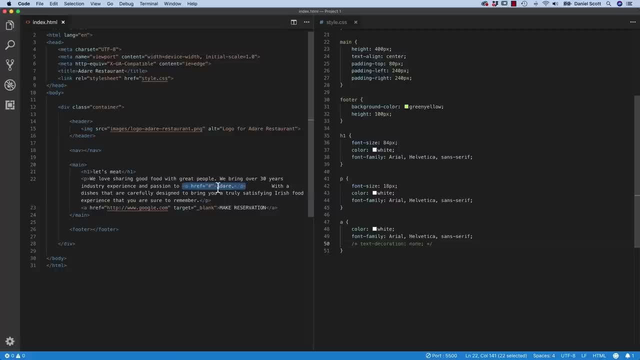 Loads of names for the same thing. A? what does A stand for? I think it's Active Link. We should check. But because it's placed in the flow of this P tag, it will just flow along This because it's placed by itself outside of the P tag. 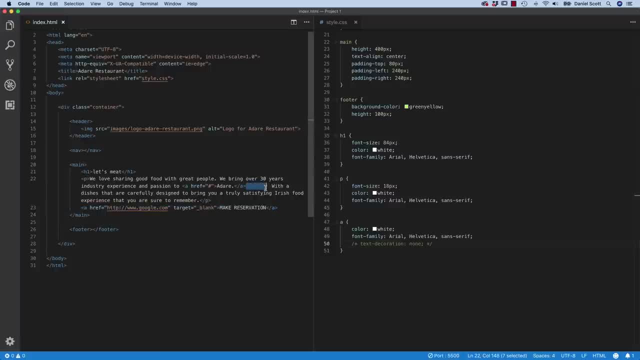 it hangs out by itself, so you don't have to actually do anything. You'll notice, see all those spaces. It didn't change anything, You see, I just added in there to make it look tidy. But I'll put it back in. 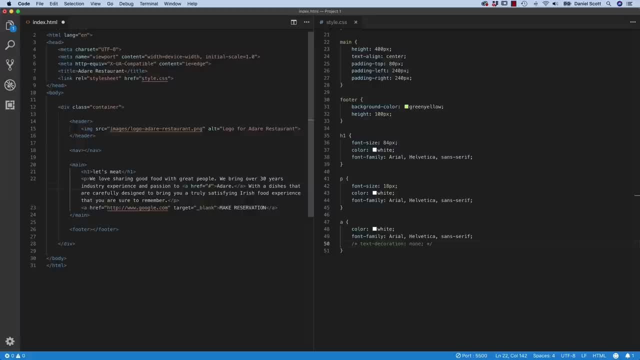 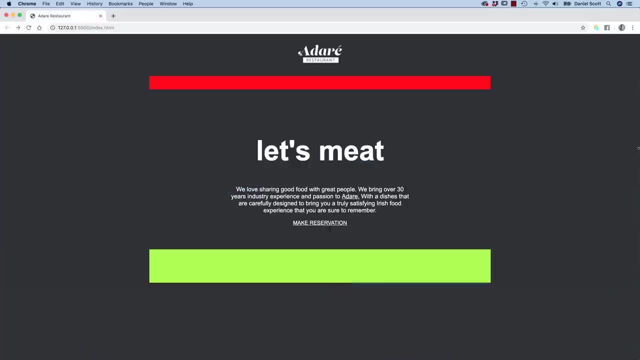 All right, that is the crash course on hyperlinks. Let's get into the next video. Hi everyone, it's time to replace our boring gray background with our exciting background image. It's cool. it's kind of stretchy, fits in there. covers all the background. 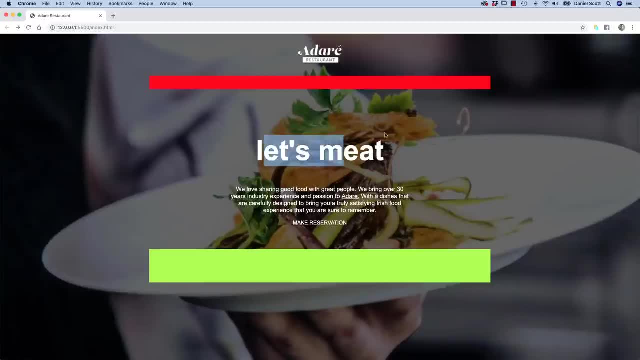 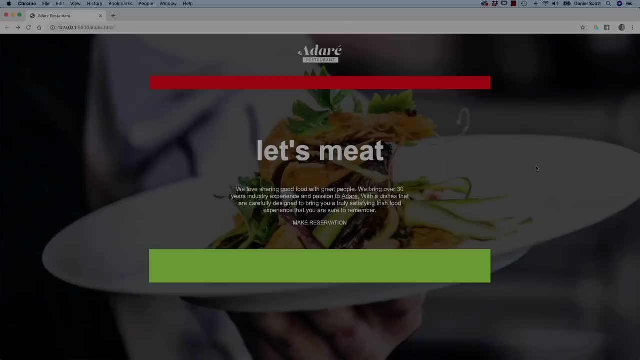 Looks neat. not sure what we're eating, but it kind of looks tasty. The irony is I'm a vegetarian, but meat looks so good, especially in these kind of photographs. Anyway, let's get in and work out how to do the background. 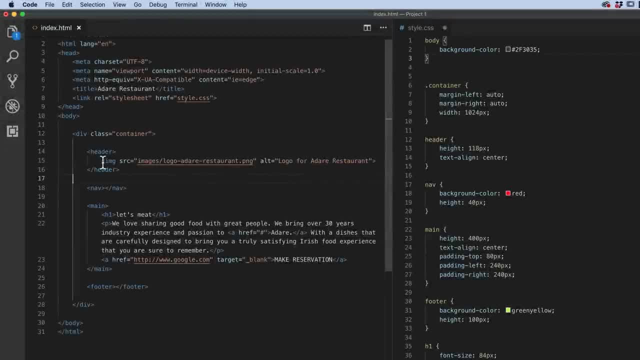 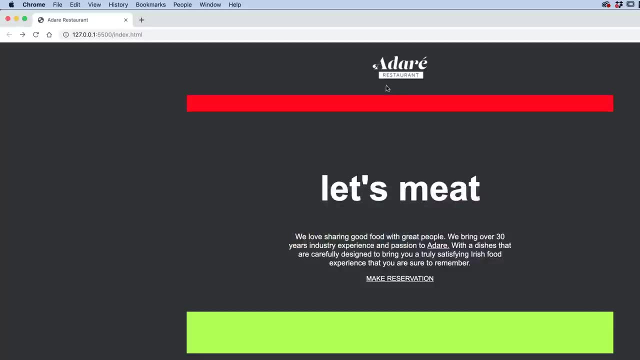 All right to add our background image. it's a little bit strange. The previous video, or one of the previous videos- we added our image, We added it to the HTML and it appeared at the top of our document here and it's great. 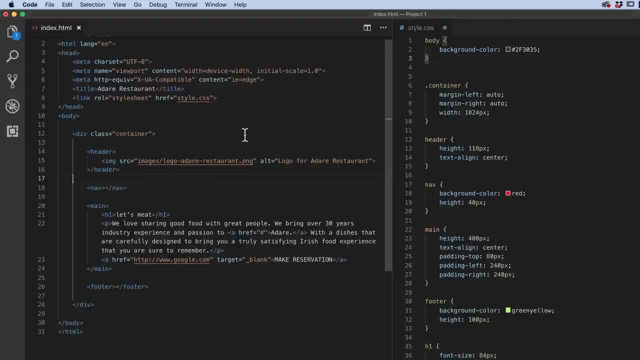 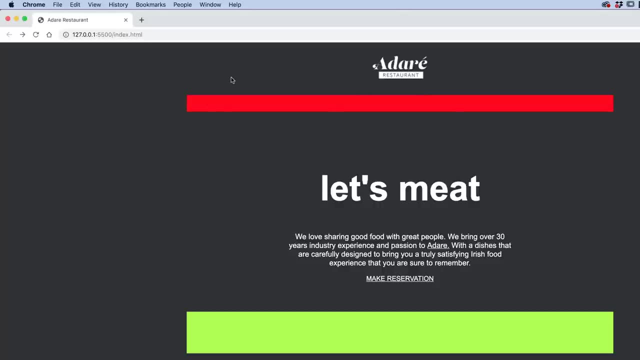 The only trouble with adding it to your HTML is that you can't have things over the top, or at least not very easily. So we want it in the kind of background and we want it to be more of an effect rather than something you can interact with. 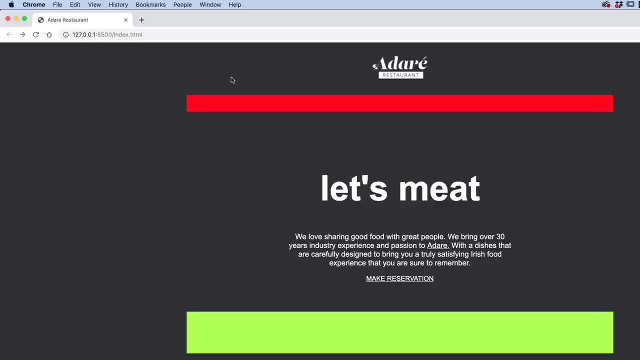 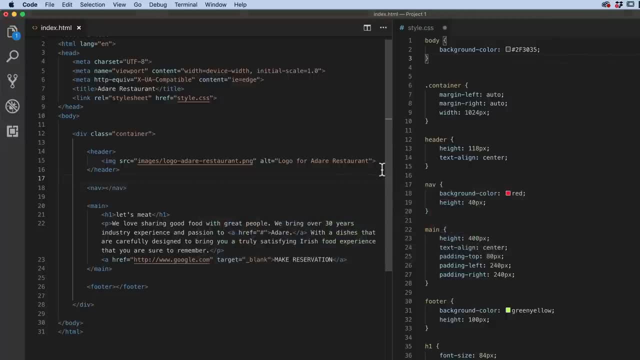 Just kind of hiding at the back, so it's more like a style. let's say: So we add it in the CSS styles, So we do it here in our stylescss and we add it to. which one should we add it to? 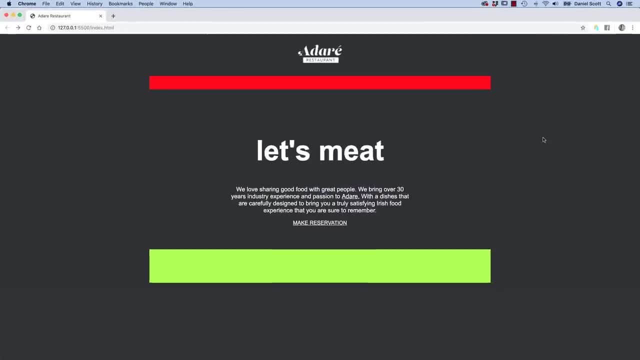 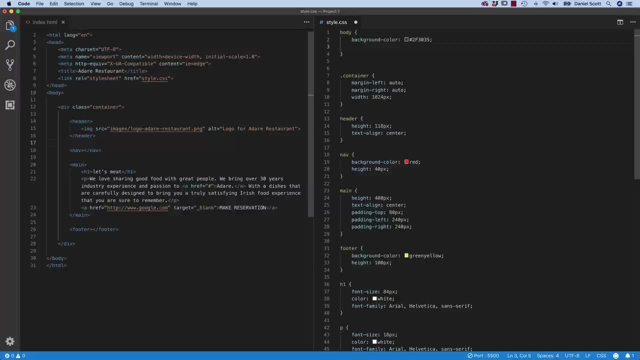 Remember our tag that covers the whole background that we made gray. It's the same tag. So the body tag here we made gray. We can leave gray there. I leave the background color there normally because sometimes it takes a little while. 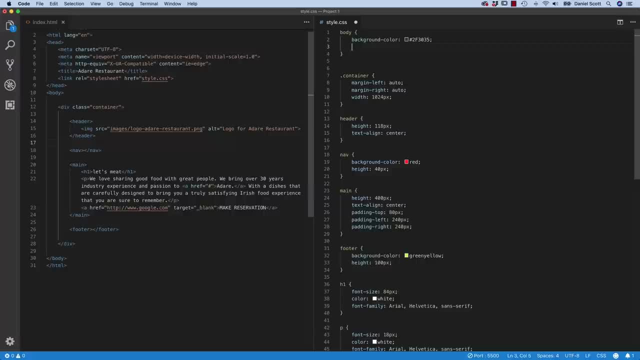 for the image to load. So at least there's something in the background until it loads. And the way to do it. it's well named: It's called background-image. The one thing that isn't very clear is what to do next. 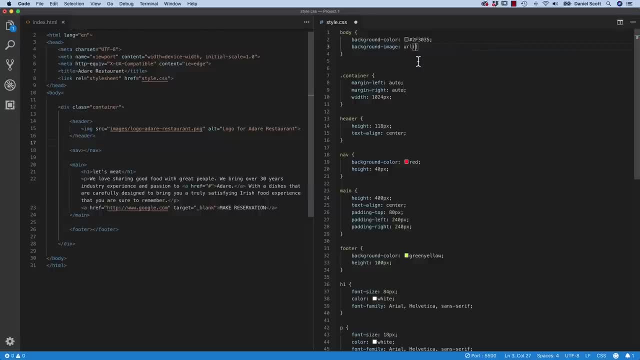 And it's URL. It's one of those options in there. So URL, so background image, URL inside of that bracket- sorry, the brackets you type where it goes, So it's going to be in images: forward slash. 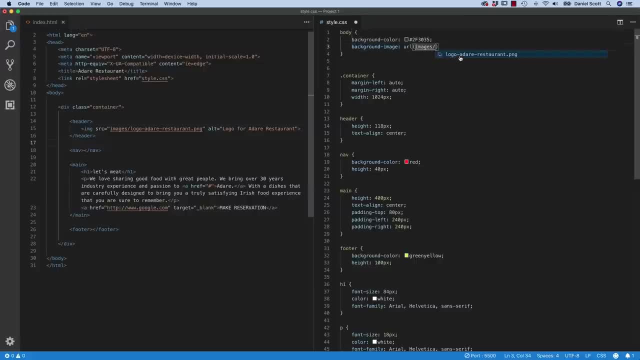 And as soon as you add the forward slash and the CSS says, hey, do you mean this image, the logo, And you're like, no, not that logo. I want another image that I've used for the background, So I've saved it for you. it's in your exercise files. 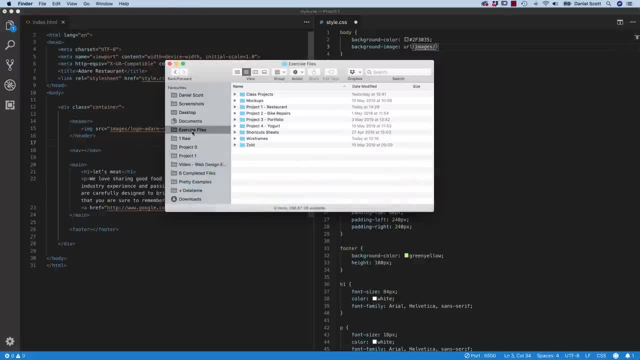 So you need to come out to your Finder, find your exercise files, find Project 1.. There's one in here called background. I'm going to copy it. I'm using Command C on a Mac, Control C on a PC Desktop. you're going to paste it into this images folder. 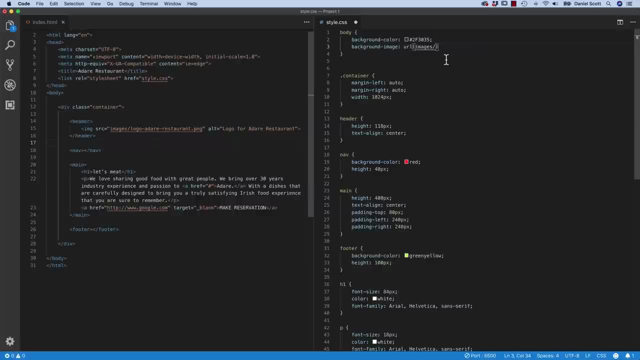 along with the logo. Now, hopefully I can delete the forward slash. there you go, Type it back in and it says: do you mean this guy? You're like I do, that's the guy. All good, Let's put in our semi-colon, hit save and let's see if it worked. 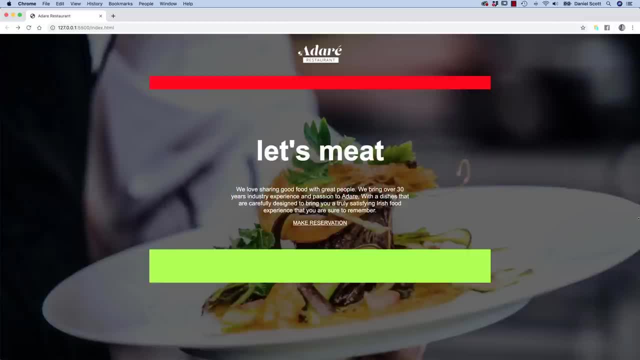 And that might be enough. you might be like: done, move on. But if you're like me and you see the moment kind of doesn't do exactly what I want, you might like it, But at the moment I want it to kind of move. 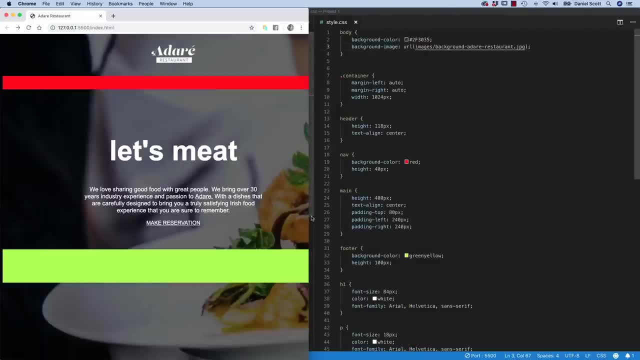 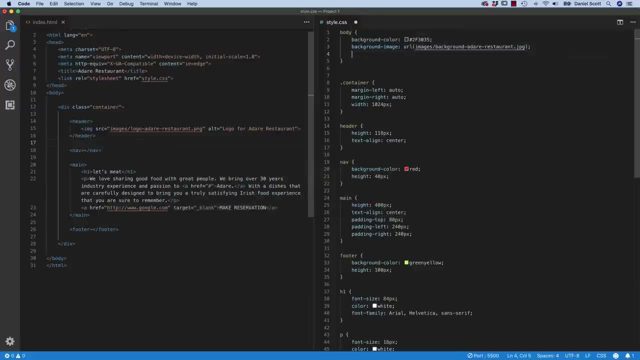 So if somebody's looking on a smaller screen that the image is still kind of centered, There's a really nice, easy CSS class that we can use. Well, not a class attribute, So it is called background. another good one. 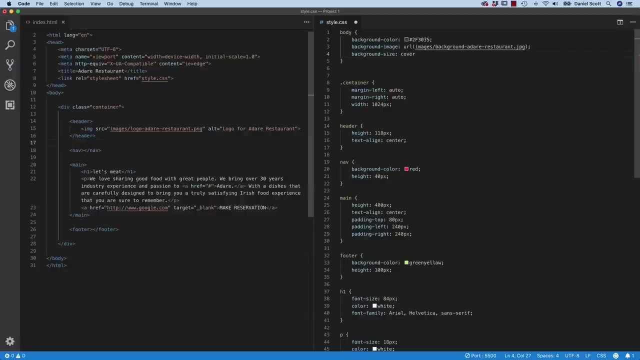 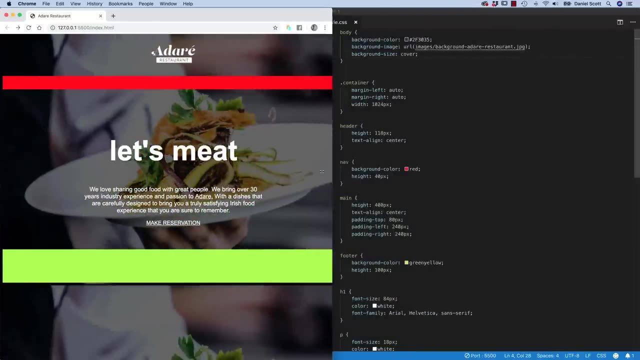 Background size and there's this one in here called cover. So background size cover will allow us to do that. Let's give it a go: resize nice. Now see down the bottom, there it repeats, because the ratio of this thing is a bit weird. 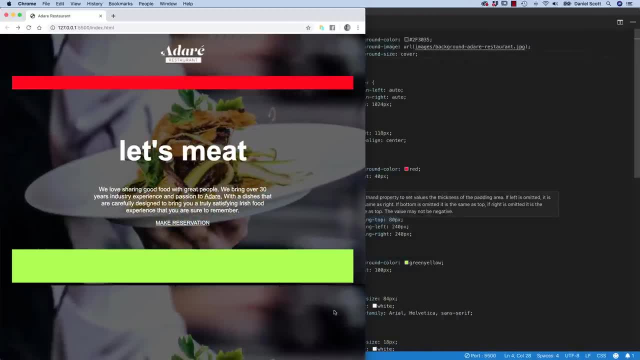 The image that we've got doesn't quite fit in there, so it has to do something, and at the moment it's repeating it. So let's have a look at getting rid of the repeat. It's going to be half our problem fixed. 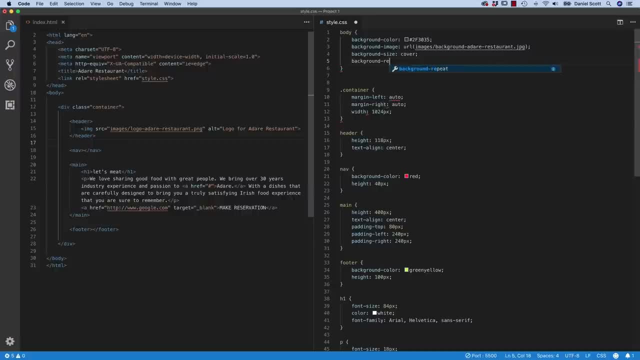 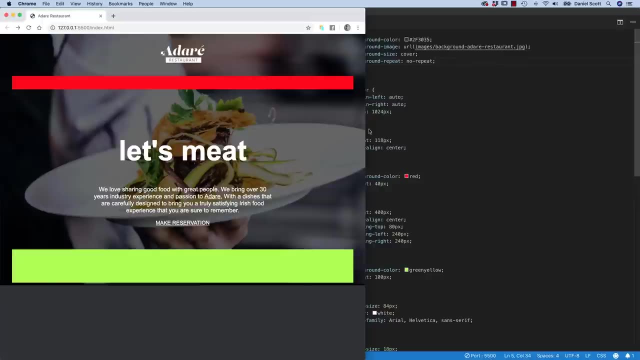 So we say background repeat, So background repeat. I'd like to set it to no repeat, please. Awesome, let's give it a go. and it's gone. There's great boxes there. You've got to decide how much that annoys you. 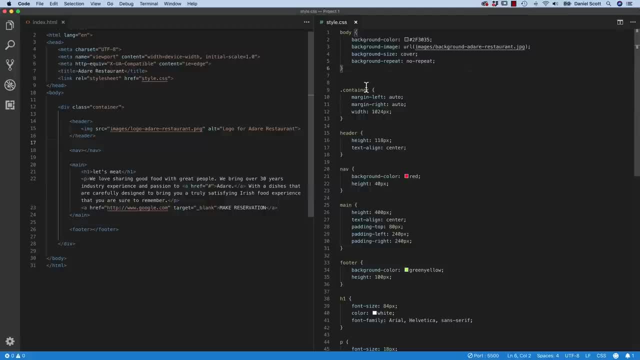 Because the next thing we need to do is a little bit kind of strange. So, to make this work, what you do is the body is the tag we've been working with, right, But there is an overarching tag over everything called HTML. 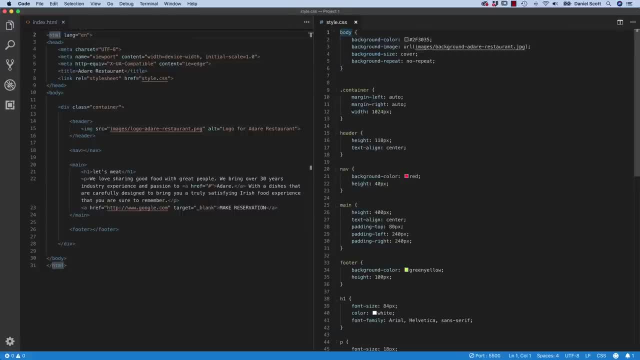 And to make that go away you've got to put in another tag just above it and say I'd like the HTML tag to have a height of 100.. or a height of 100%, And that fixes that. I'm not even sure why, but that's what we do. 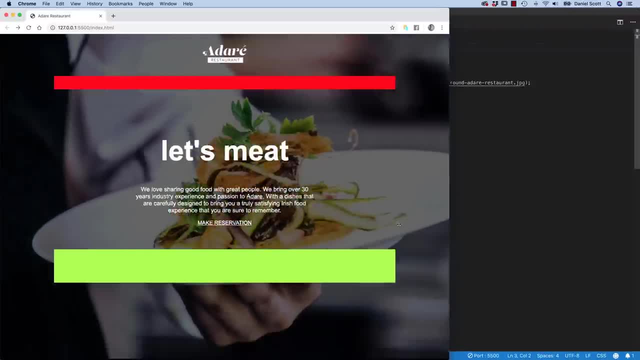 It depends, like I said. sometimes in web design I can explain it to you and sometimes I can't. So there you go, it's covering, it fits, it's nice. And one more thing, if you're getting picky, 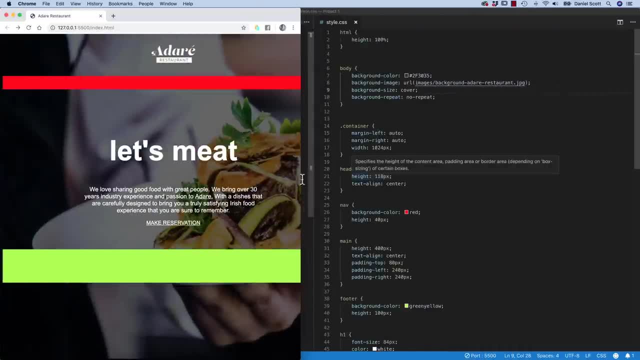 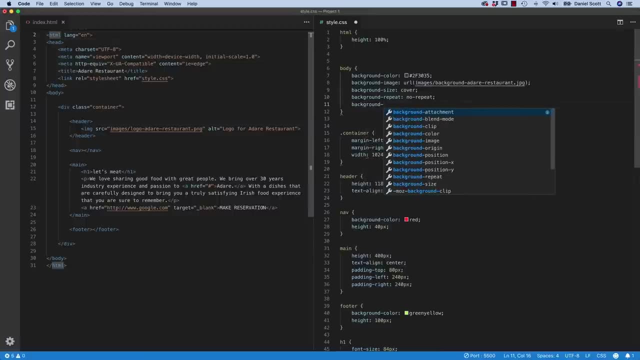 is that it's kind of centered and stays in there, but it's not quite centered. you're like: why aren't you quite centered? You can mess around with the background. what is it called Background align? I spelled it all right. 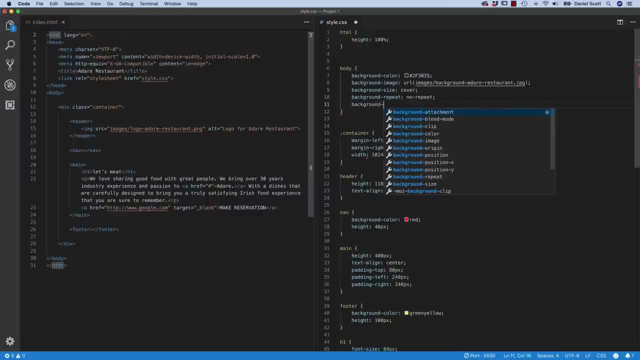 Background alignment. no, it's background, man, I can't remember position, that's it. So background position and we type in center semi-colon and that should fix that. So now, instead of it'll go from the center. 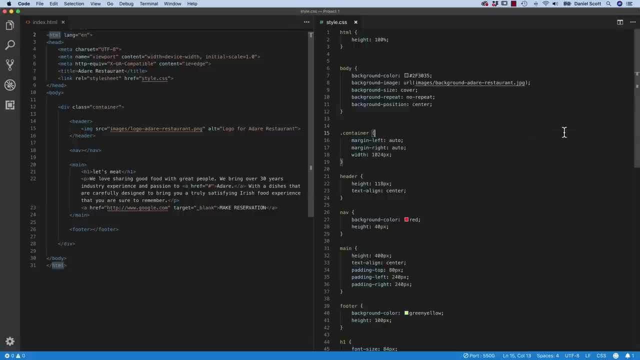 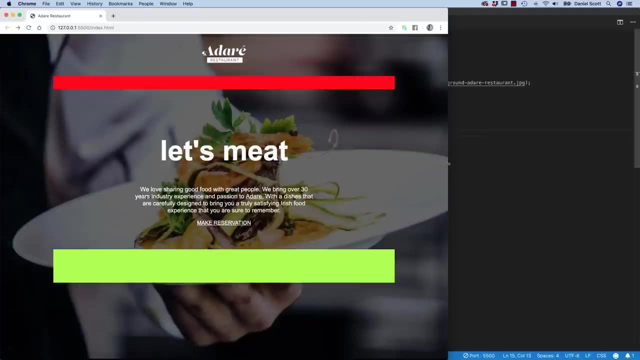 rather than kind of left and right. Yeah, I like it. Now, one thing: if you are following along on a really small screen, you're like I can't even make it. do it. that, Dan, It's true, I just thought of that. then I'm like: 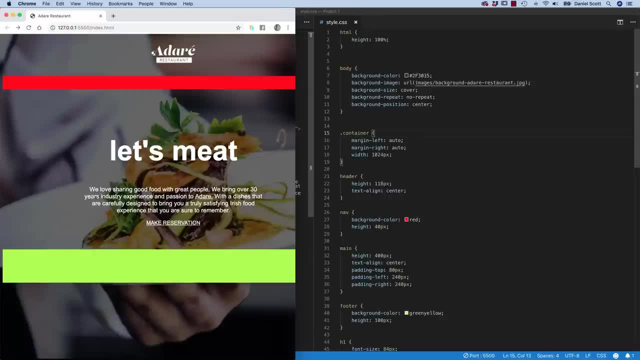 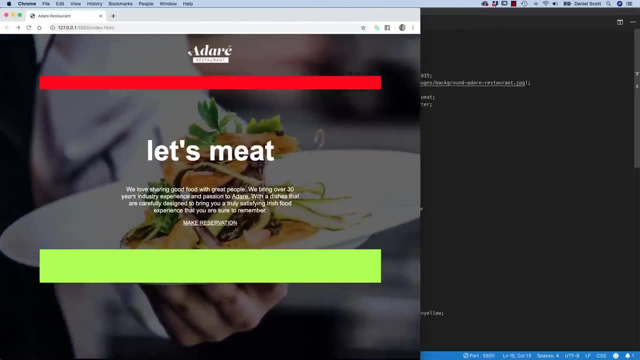 if you have a really small screen, it's going to be very hard to drag it out, big enough to make it do all the kind of resizing bits. So that's something to know, I guess. what you're doing then for like 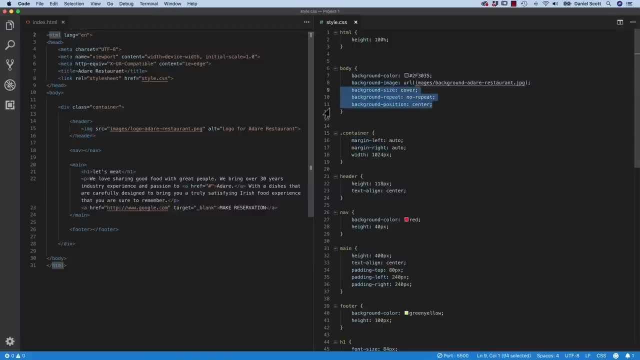 you probably can get away with pretty much all of that gone. The trouble will be is when somebody like me with a giant screen opens it up and goes: hey, it's not looking nice. So if you are working on a really small laptop, 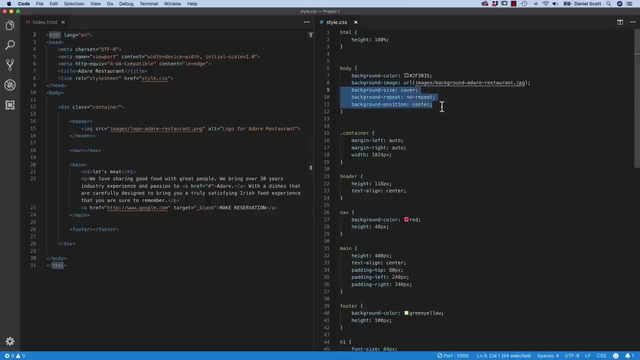 and you're like I can't even test this stuff and later on in the course I'm going to show you how to fake being a really big screen. But yeah, just thought I'd add that there, just in case you're like can't make that work. 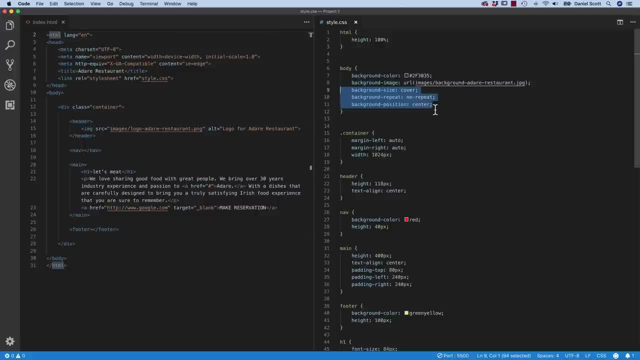 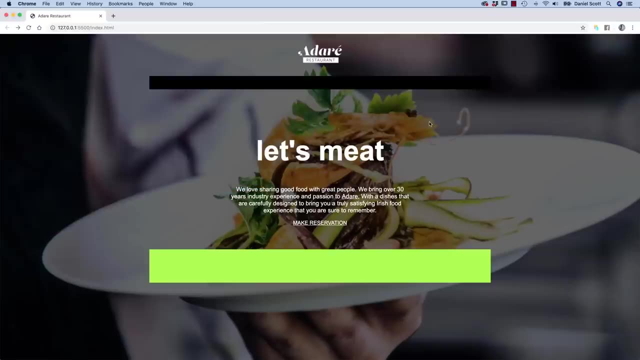 But it is potentially necessary. All right background images done and dusted. Hi everybody, we're going to look at making things see-through, Normally referred to in code as alpha- transparency, opaqueness. You get what I mean. we're going to go from this to this. 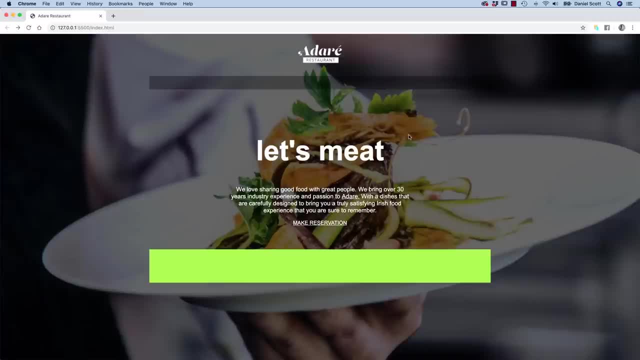 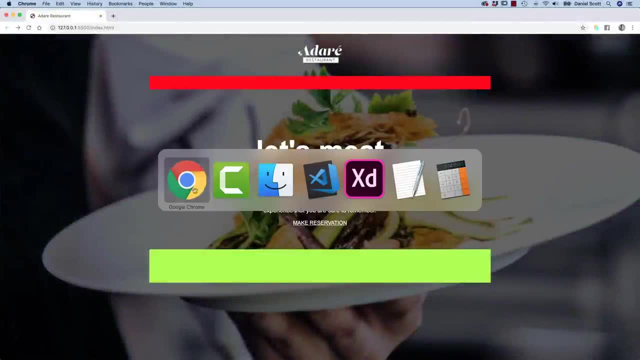 where it's a little bit see-through or a lot see-through. I'm going to show you now how to do it in CSS. All right, to do the transparency, we're going to do it to this nav. Currently it is red. let's first change it to a color. we'll change it to black. 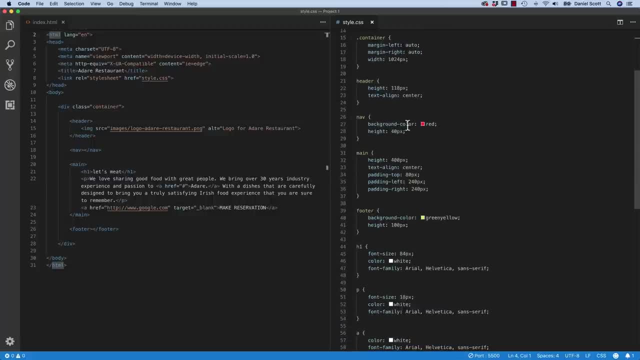 And so let's go to VS Code. let's find our nav. There he is there. color we're going to type in black. We didn't really need to do that first, but make sure you save it all. Preview it. there it is, it's black. 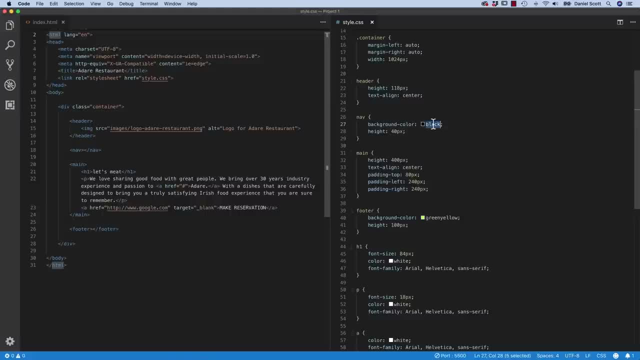 Now we want to make it a little bit transparent. I kind of mentioned this earlier on, but if you highlight the word black or just click in here, it's a little bit hard to get this thing activated. I find Man, here we go. 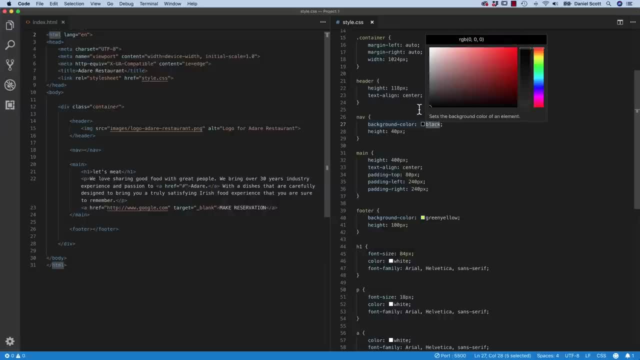 Eventually you can get this thing going. Now it doesn't really matter. you can make it black in here on the fly And what ends up happening is, if you pick a solid color, you get three options: Red, green and blue. 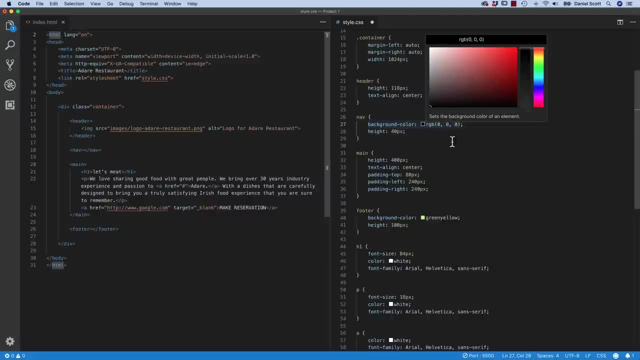 At the moment. if they're all set to 0, that means you get black. You set them all to 255, you get them all and it creates a white color That has nothing to do with what I'm going to say. 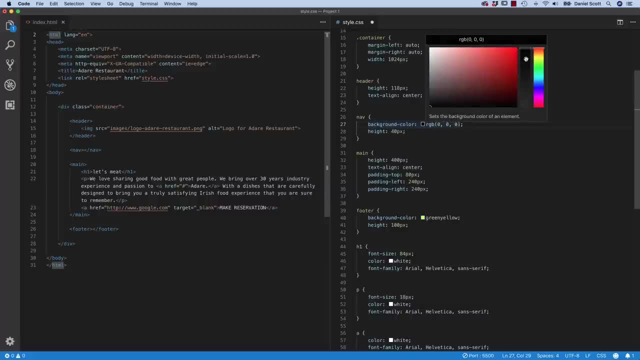 except that you can add a fourth dimension. So over here, if I drag the slider down to say I'm kind of looking up here that one, there see 0, 0, 0.. and there's this new extra added option. 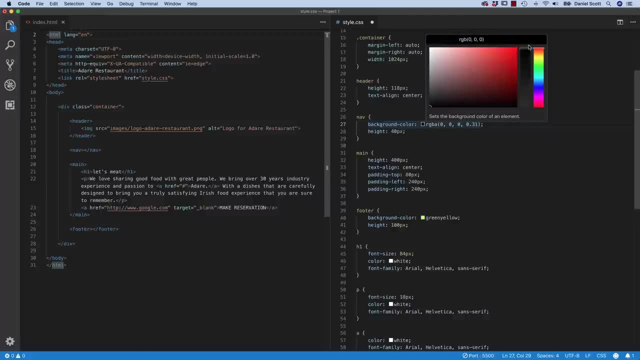 And think of them as percentages. If I go higher, look when I'm at solid 1, it disappears. but if I come down 0.975, it's like 97%, That's 50% see through, And getting right down here it's like 10% opaque. 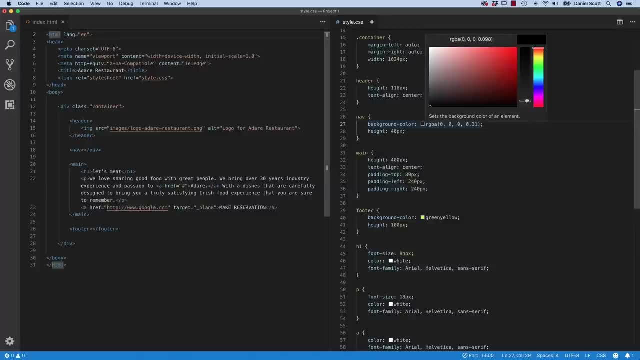 10% opaque is a better explanation. So 10% color in it, 50% of color, 90% means it's almost completely black. again, If I explain that, okay, you drag it up and down, you'll work it out. 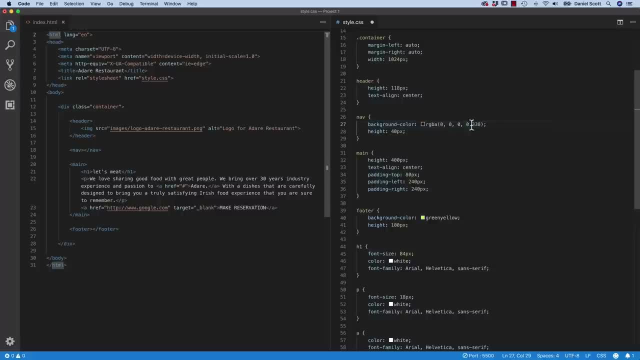 So I'm going to have mine about 30%-ish And you'll see, there it is there. So 0.3 means it is 33% black. They're not very. let's save it, let's test it. 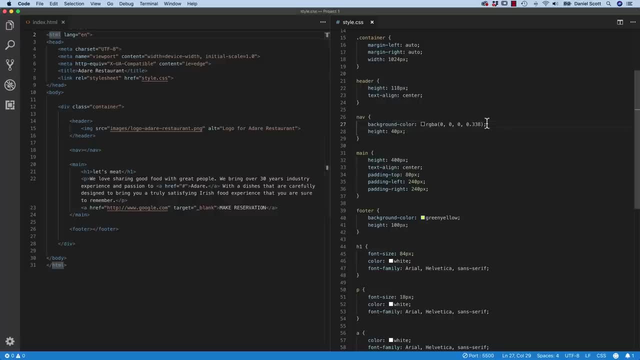 And so look there you go. Now, if you're old school web design and you're using those hexadecimal numbers, remember the hash. We did them earlier on: hash, hash. oh, come on, don't do hash. And I picked some random colors. 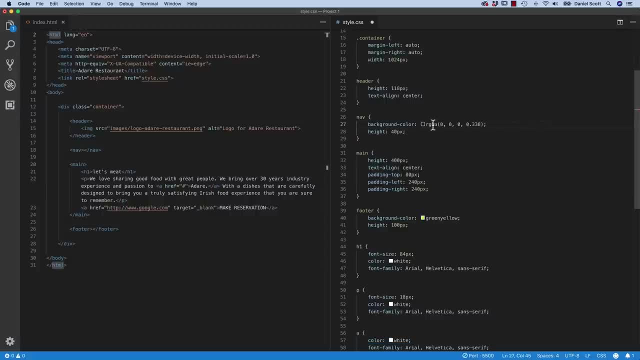 You can't do alpha transparency with that. You have to use this thing called RGBA, which is red, green, blue, and alpha, which is the see-through-y bit. All right, that is how to make something see-through. Now we've done it for the background color here in our nav. 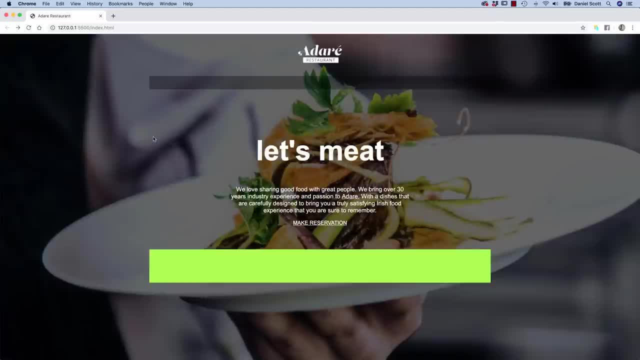 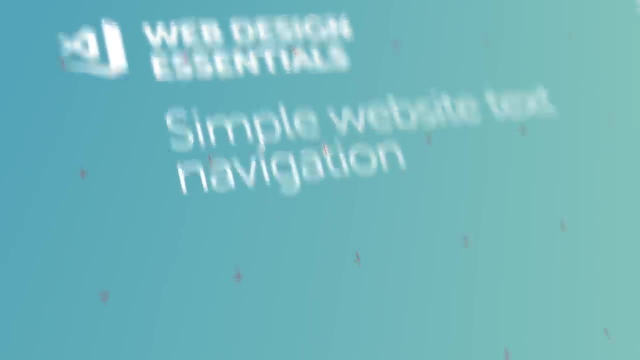 But you could do it with type. You can make any color that you've applied to things Slightly opaque or lots opaque. All right, that is it. I'll see you in the next video. Hi there. in this video we're going to make this simple text navigation. 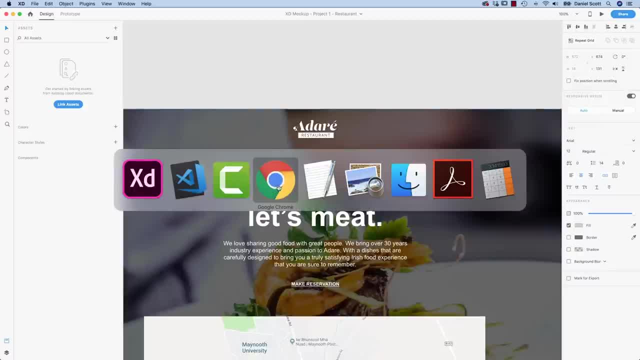 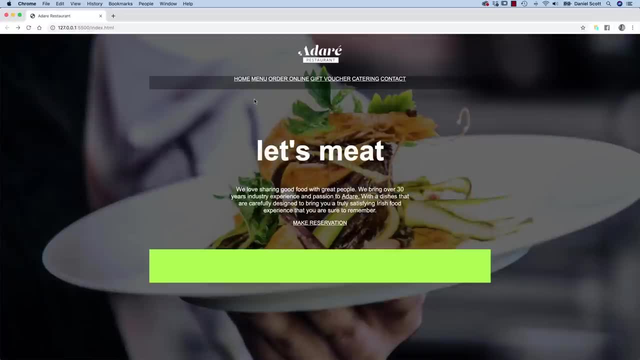 So we're actually going to build. that's the mock-up. We're actually going to build. we're going to get this far in this video anyway, So it's just kind of lumped to the top here. The alignment's not perfect yet, but it's in there. it's all linking. 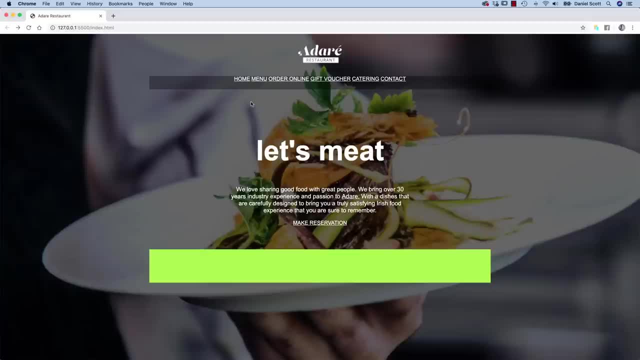 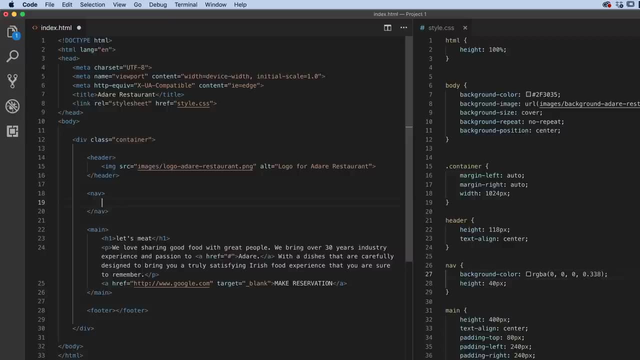 And we're going to learn some sweet new shortcuts along the way. So let's get going First up. let's put in our links. So in here, inside of our nav, I'm going to put a return in And I want to put in: how many options do we have? 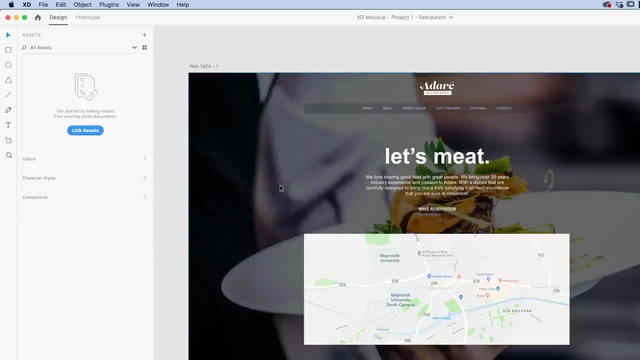 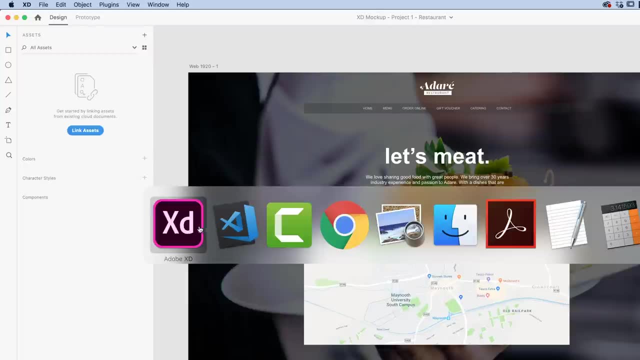 We have 1,, 2,, 3,, 4,, 5, 6.. So I want 6 A tags. This one's got a pretty simple menu. We're going to build probably 4 in this entire course. Simple text one. we'll make buttons in the next project. 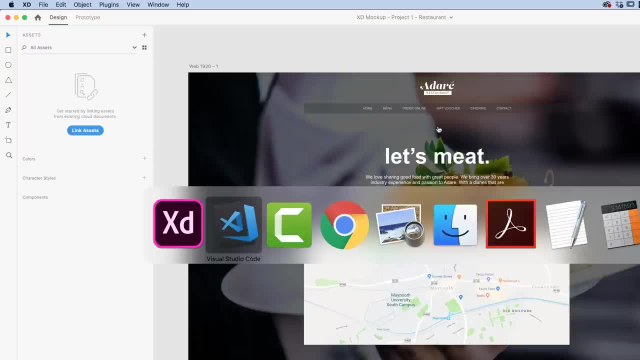 and then we'll do drop down and cool jQuery burger menus from mobile. We'll get fancier and fancier as we go along, but a nice simple one to start with. So what I want to do is add my 6 links. 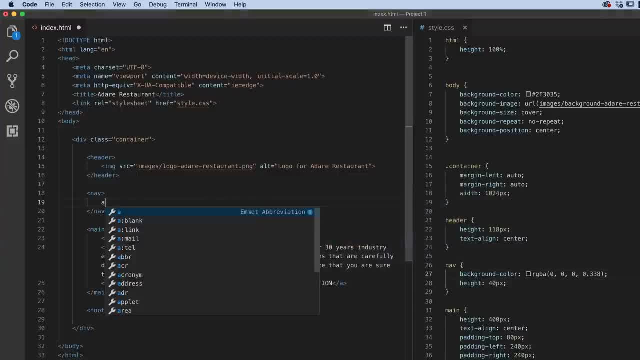 So in Visual Studio Code I want to type in A tag return. We're going to put in hash so it doesn't go anywhere And the first one is home. Now we can do that 6 times and that's totally fine. 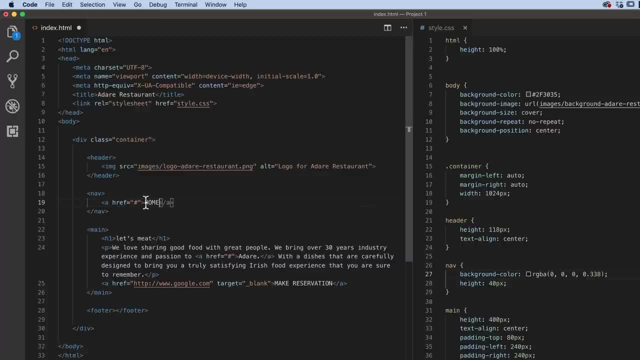 You can copy and paste it and change the text. I'm going to let you in on a little shortcut. I'll try and introduce little shortcuts as we move through. They're just fun and they're good and they're useful. 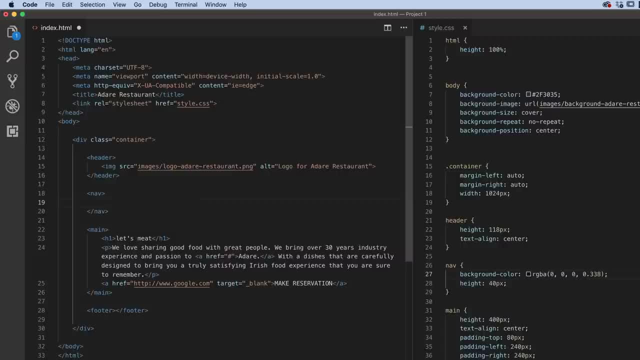 and I use them, so I know they're good. So what we can do in VS Code is we can do: say, I want an A tag, lower case A, But I want 3 of them. we can use the times 6 of them. 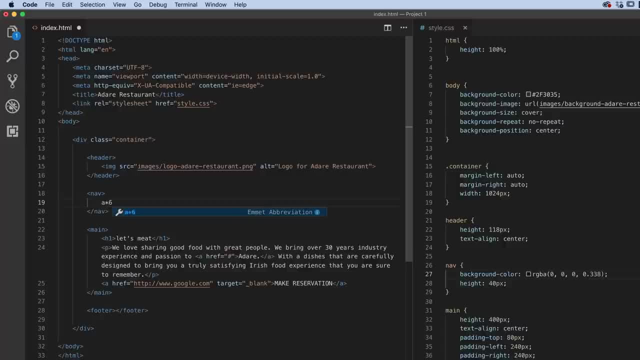 So times in this is the asterisk key, So it's underneath, often combined with the number 8.. So hold down Shift and click 8.. So A asterisk 6.. means I want these. I want 6 of them. hit return. 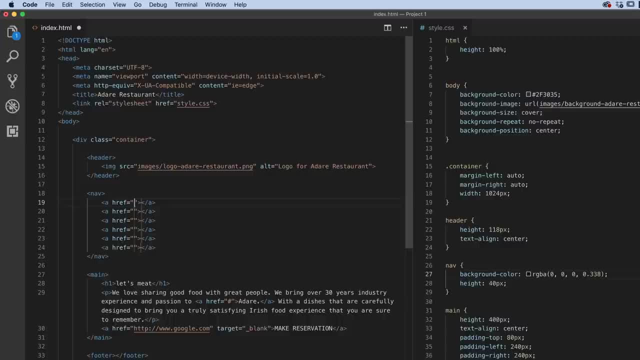 Look at that, cool huh. You're a web designer and you're hardcore and you're coding. I don't know coding fast. cool huh. So what I want to do is I want to put a hash in all of these. 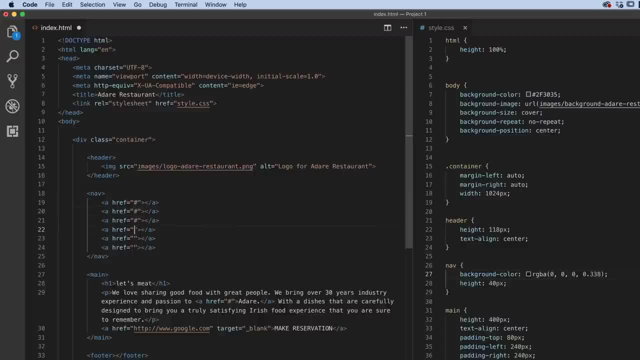 You're like imagine if there's a shortcut to do all of that. There is. that's a bit of a slow process, So a lot of the time you end up working on these kind of like multiple groups doing multiple things all the same. 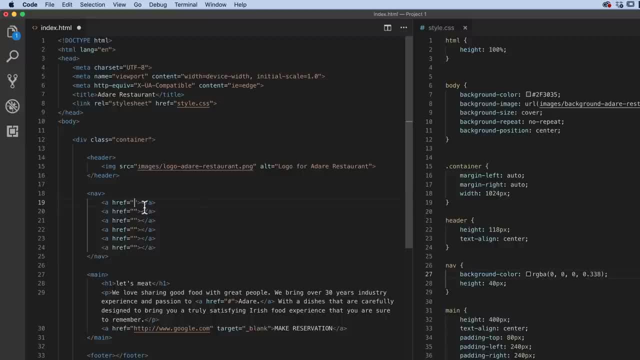 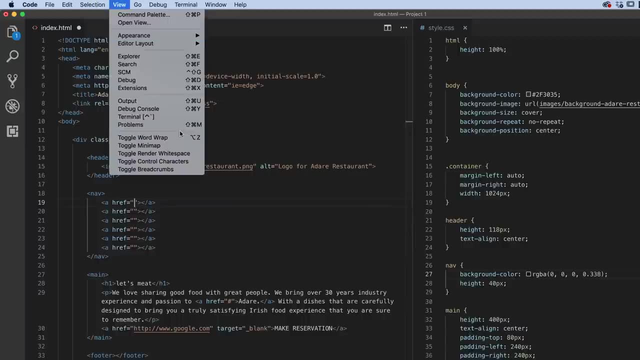 So what we can do is we'll do one more, one more shortcut, And you can just obviously type them in. but if you on a Mac, it's under this one here That's the shortcut you're looking for. So it's under View. no, it's under Selection. 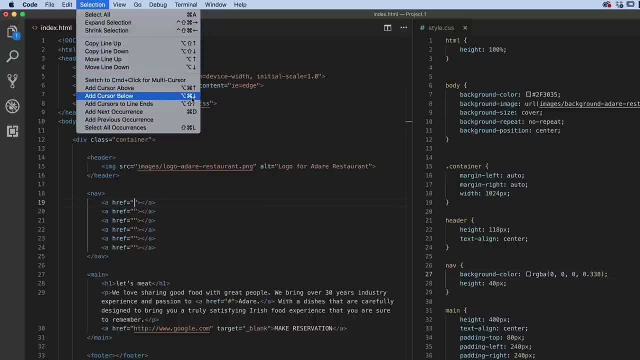 And it's this one here. Add Cursor Below. On a Mac it's Option Command. so Alt, yeah, Option Command. and the down arrow, So the cursors, you know the up, down, left, right. 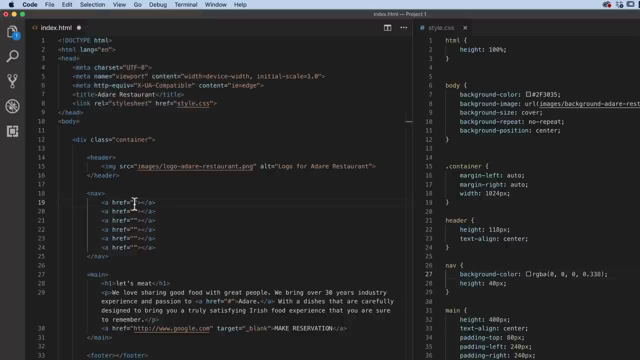 On a PC it's Control Alt down arrow. So here we're on Facebook and I'm flashing, so make sure your cursor is flashing there. On my Mac I'm going to hold Command Alt, Command Option. 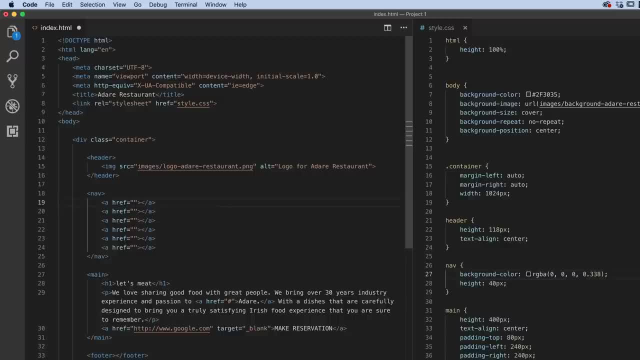 and hit down, down, down, down, down, And then I'm going to type hash. If you're on a PC, it's Control, Alt down, down, down, type hash. I want to get rid of that now. 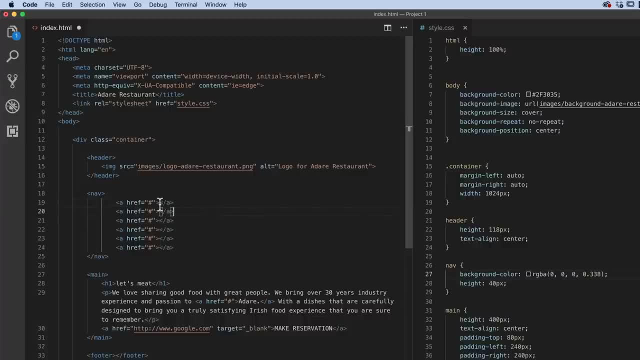 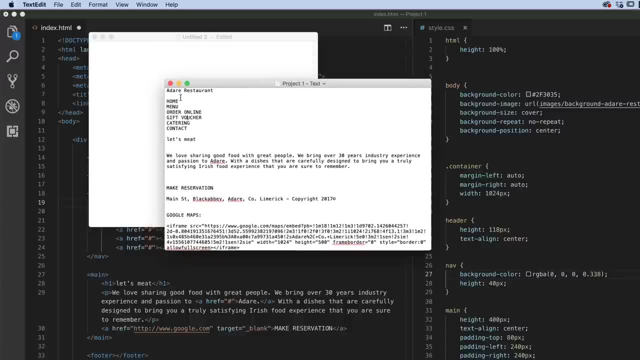 because I don't want Home in all of them, So I'm just going to click once anywhere else. So I'm clicking on the first one and in your text- so remember, in the exercise files, there's a file called Project1.. 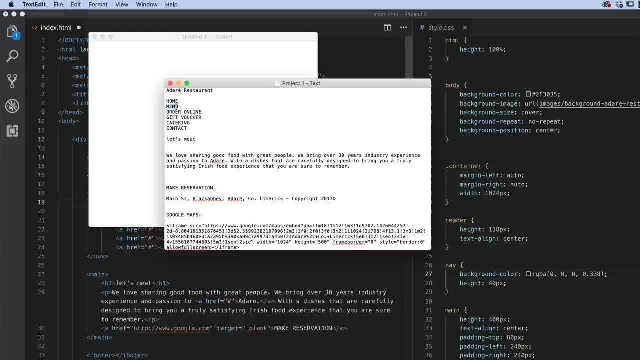 Text. I'm just going to copy and paste it all in Copy paste. you can do the same. If you can type, you can just type it all in. You don't have to put anything in. I'll speed this up. 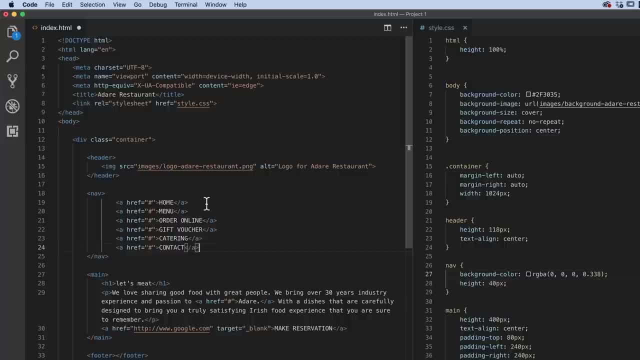 All right, thank you, Editor. It's Jason, by the way. I call him Editor all the time, but his name's Jason and he's awesome. Thanks, Jason. So we'll do a save all and we'll preview it in the browser. 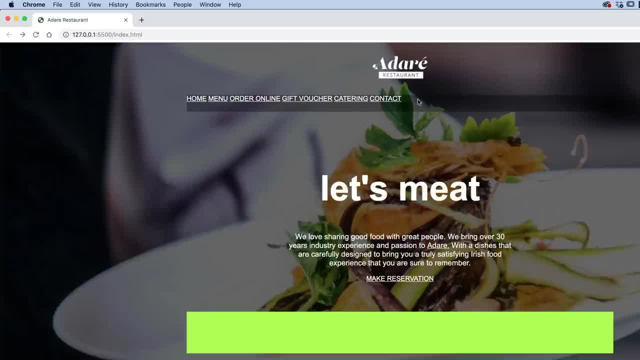 And does this update. It is there. it is there, Cool, so I've got all my text in there. It's not quite right, Because, remember, because this is an A tag and we styled the A tag down here. these guys, hey, we're the same, let's do the same thing. 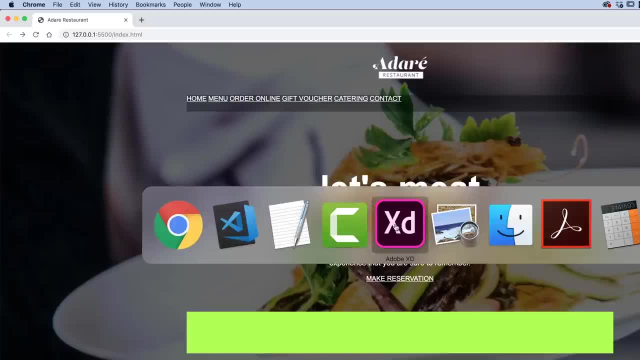 So we're going to have to do some specific styling for this to get it to look like my mock-up here, But we can do that. First thing we'll do, though, is we want to center it, So what we're going to do is we've done this before. 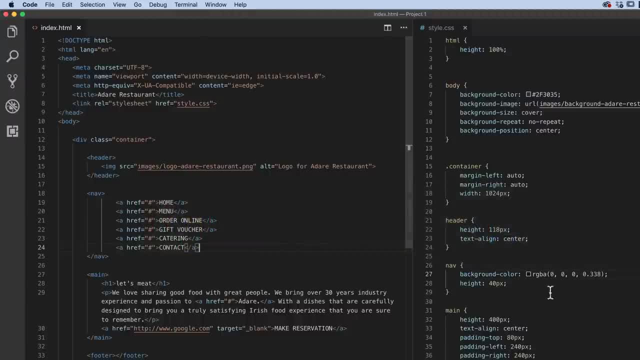 We want to go through and center using Text Center. We'll do it to the Nav. We'll say: all the text inside of me is going to be Text Align Center Semicolon. save. Save all preview in the browser. look at this. 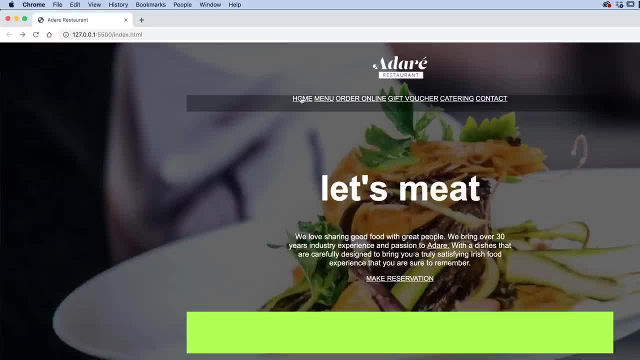 Padding to mess with, underlines to mess with. but that is going to be it for this video. at least We put the Navs in. we learned some shortcuts. All right, I've kind of doubled back. I've finished the video. 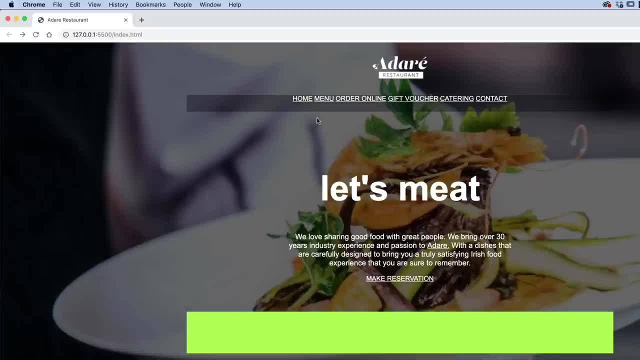 and I was like, oh, I should mention this. So we've started doing shortcuts. now I felt like it was the time to start doing some basic ones. And if you're like, how am I going to remember these things? Or maybe you started writing them down already? 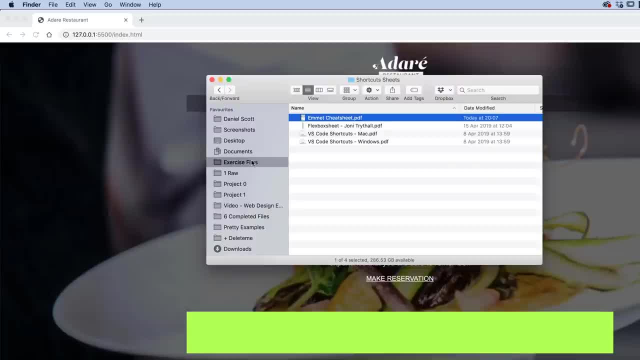 I've created a folder in your exercise files. So exercise files, shortcuts, Open that up and we've got ignore that one for the moment. we'll look at it later on, But these two will be handy. So VS Code, we'll look at first. 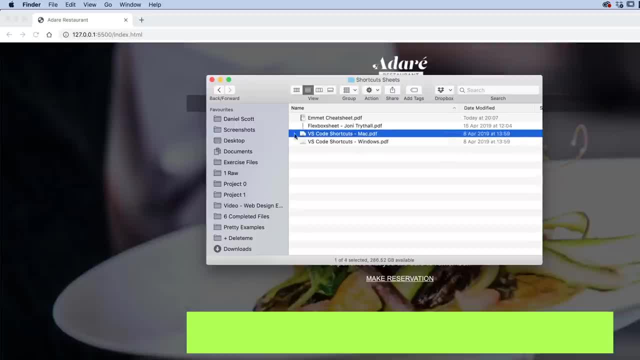 So there's a Mac or PC, depending on what you're using. I'm going to open up my Mac one And let's say it's a nice one-pager. you can print it off, stick it next to your computer. highlight the ones that you find useful. 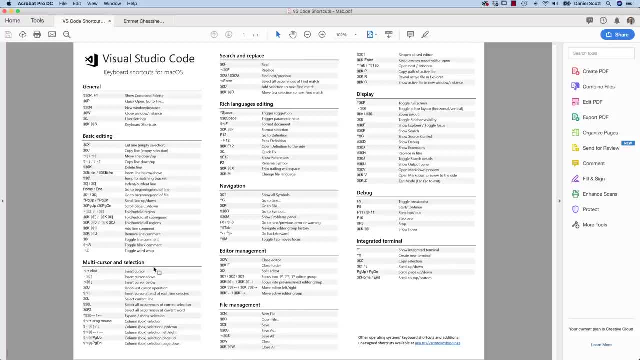 You're not going to remember them all, But the one we just used. can you see? multi-cursor selection? That's the one I used, the insert cursor below. So you might just highlight that one now. print it off. highlight it. 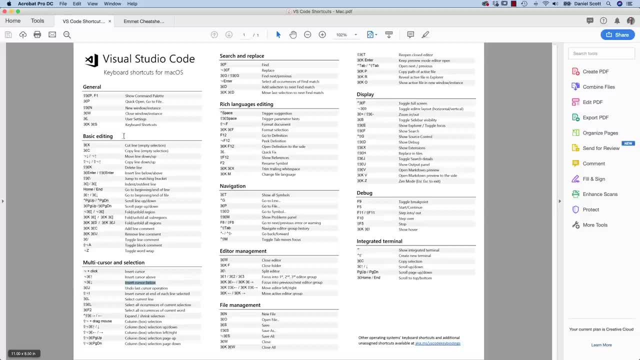 and say that was a useful one. Dan, I'm going to try and remember that one. You might have a read-through, maybe further on in the course you might read through and go: oh, I didn't realize that was the shortcut. 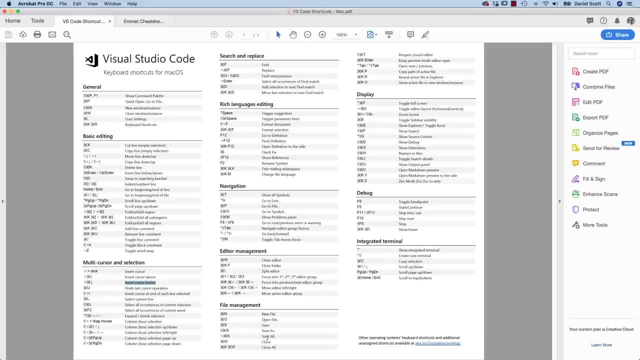 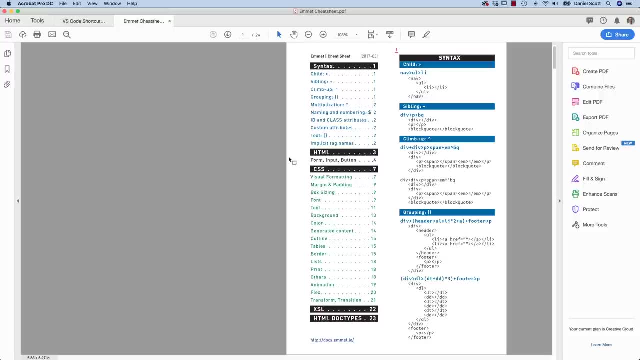 It can be really handy. Or this one here save all. if you can ever remember, highlight that one. So that's VS Code. the other one in there is called Emmet, So Emmet we didn't really talk about. 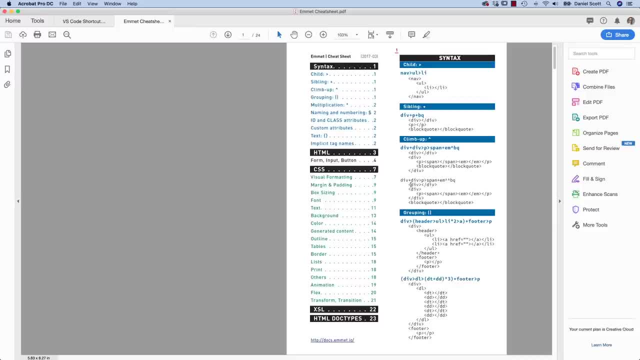 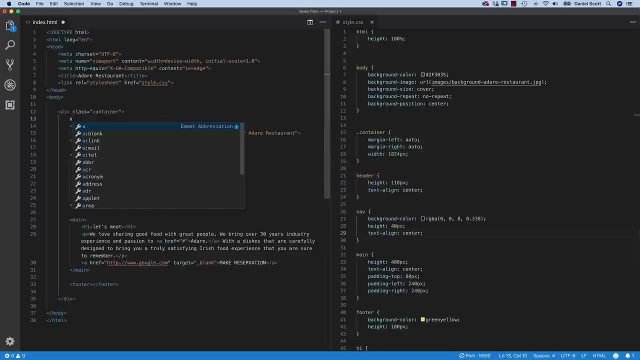 So it's got a separate name, these shortcuts. they're called Emmet shortcuts, But for you it's these ones. it's when we say all the Emmet ones are things like all right A tag If I type A and hit return. Emmet is kind of doing that. 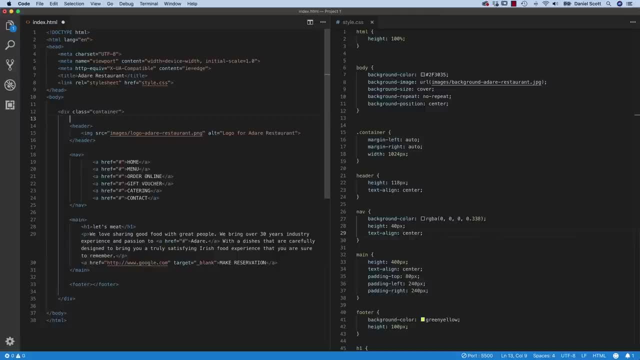 But it doesn't really matter what it's called, But Emmet is what it's called And the same thing before we did A times 6, remember That is an Emmet, or you can see it there, Emmet abbreviation. 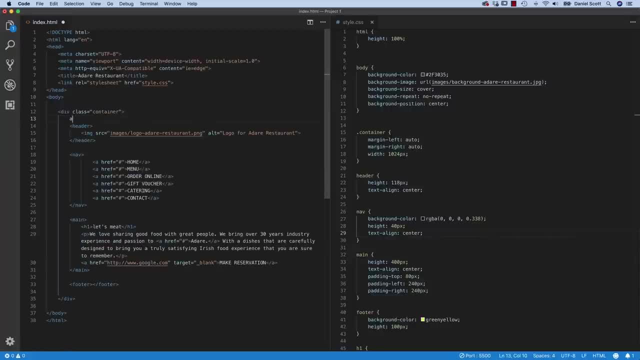 There you go. you probably have seen it, So they call it Emmet, and I've made a little shortcut. Well, I haven't made it, I've collected this for you. So the problem with this one: it's like 24 pages. 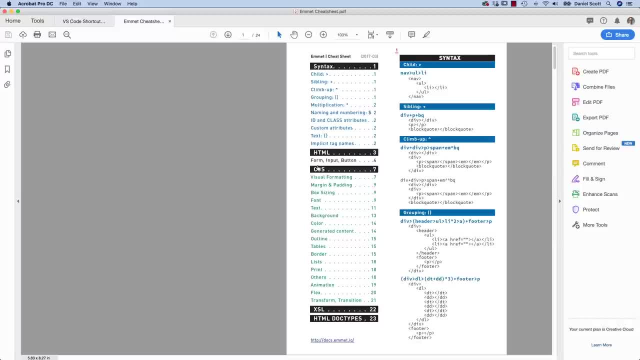 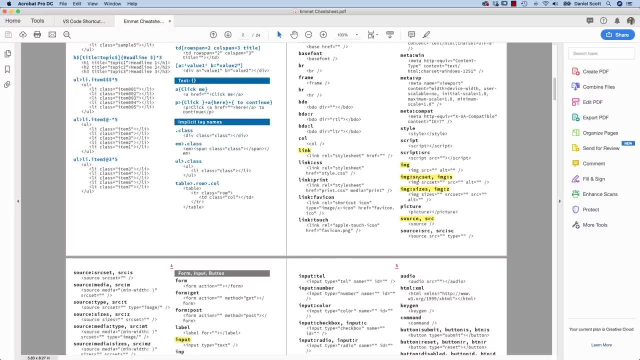 It's got every single thing you might do, And I find it's useful printing off that, The first two pages, because the rest of them, yeah, it's quite hard And they've highlighted the really important ones to the ones that you're likely to use. 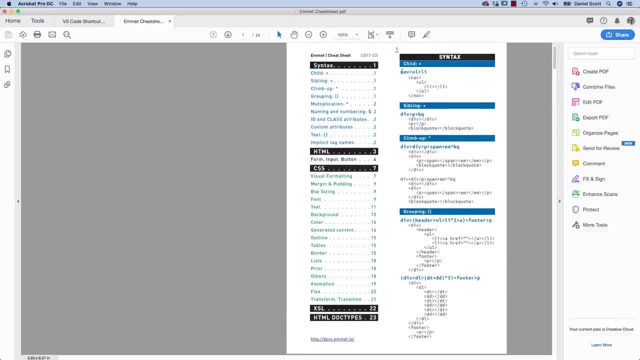 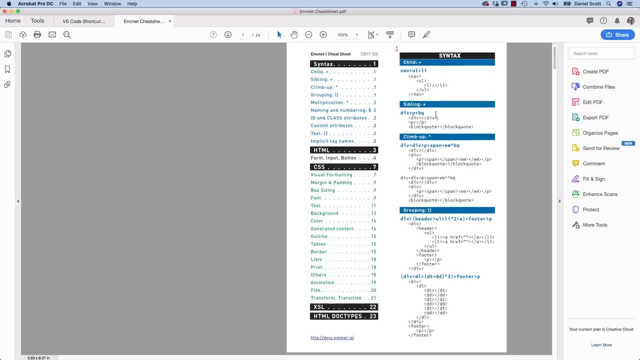 But maybe just print the first two off. I find it really interesting to look at these kind of structures that you can do. We'll get into these further on, but it's probably a good time to print these off now so that you can start scribbling your sweet new shortcuts on it. 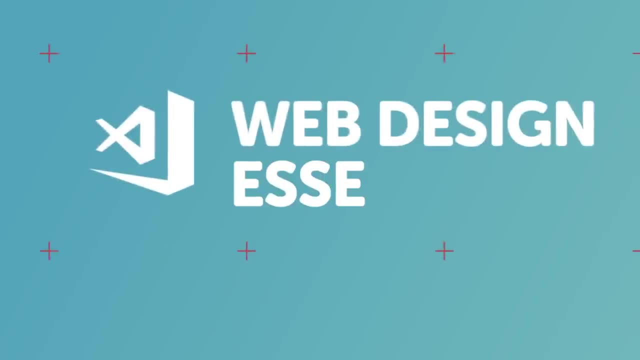 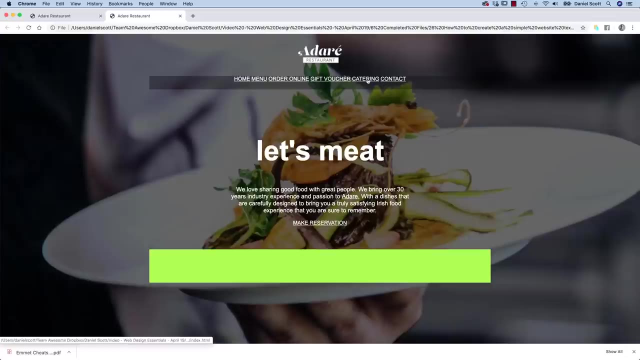 All right, now is the end of the video. See you in the next one. Hey everyone, we're going to take our menu in this video. that looks currently like this: to this: Padding either side: some space between them. font sizes: 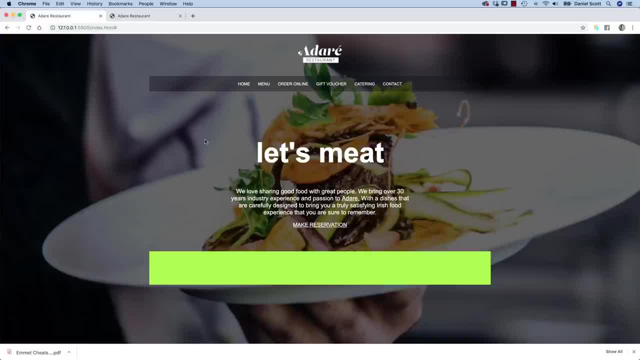 To do all this, we're going to have to learn what a Compound Selector is. It's pretty cool and nice and simple. It's going to allow us to be fancier web designers. All right, let's jump in and learn what it does. 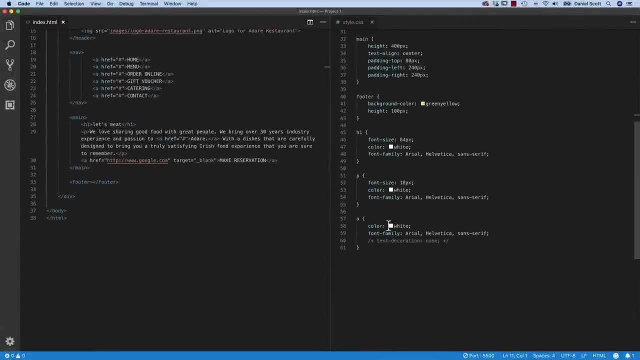 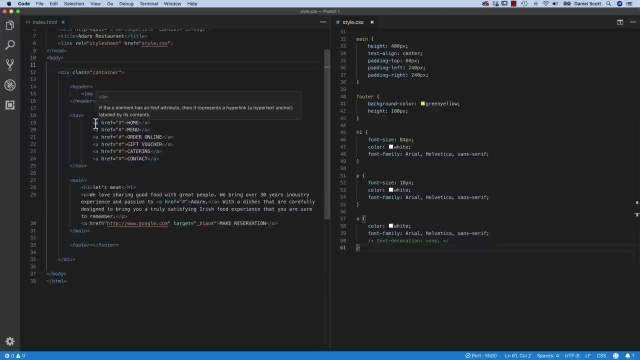 Okay, Compound Selector. What is a Compound Class? It's just more than one. because we've got a problem now, because what I want to do is I want to style these A tags. I want to turn off the underline because I don't want it here. 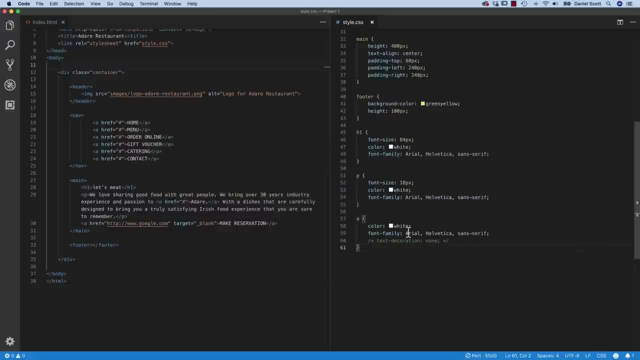 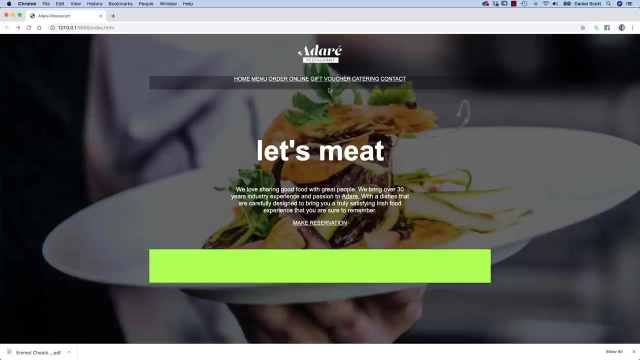 But I've already styled the A tags. remember, earlier on We said A tags we want to leave. We turned that off because we're like, actually we want to leave the underline. So we've got one A tag controlling a couple of things. 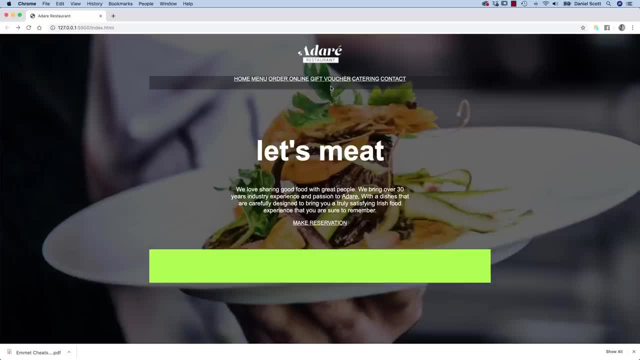 So what we can do is use something called Specificity. It just means the more specific you are, the more it will override if you're more specific. So if I say generally all the A tags do this, but if I say the A tags specifically in the Nav, 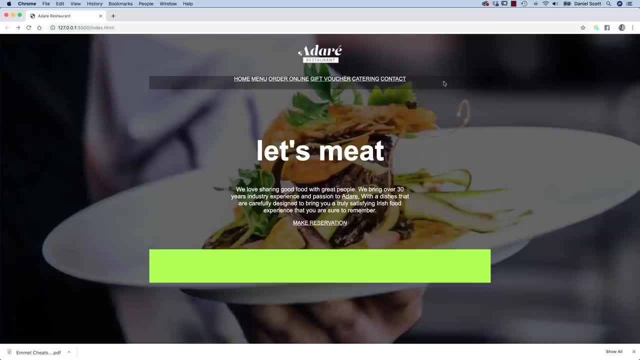 do this other thing, that will win, because it's more specific, Generic, a little bit more specific because we're saying the A tags inside of the Nav. All right, let's just do it, Dan, In Visual Studio Code. 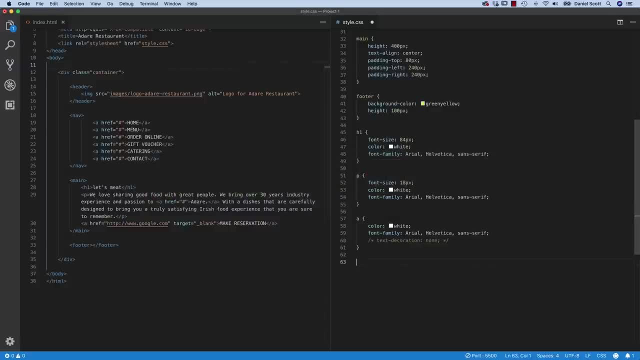 the way you structure a Compound, Class or Compound Selector, Compound- just because there's two parts to it, You can have more than one. We're just going to do one. So what we want to say is we want to say: 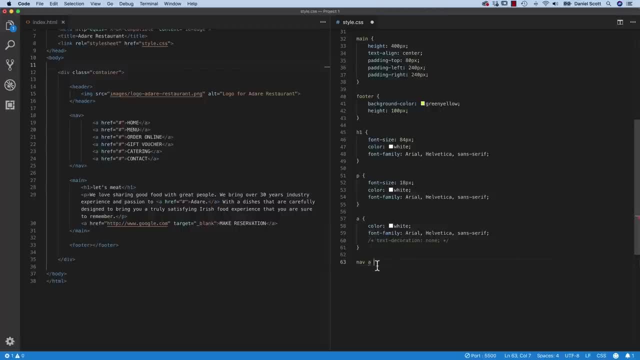 if there's a Nav with an A inside of it, you just put spaces between it, Because we're dealing with Tag Selectors, the Nav and the A. it's not a class. we don't need the full stop, So it does it all by themselves, with spaces in between them, and that's it. 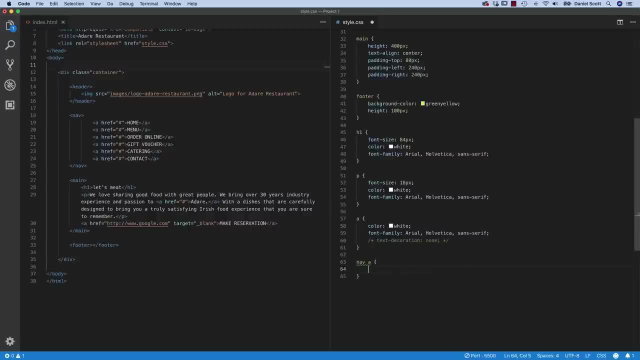 So if there's an, A tag inside of a Nav, do this other thing. And what we want to say is Text: Decoration. Decoration is set to no decor. what's it called? Set to none? It's none cool. 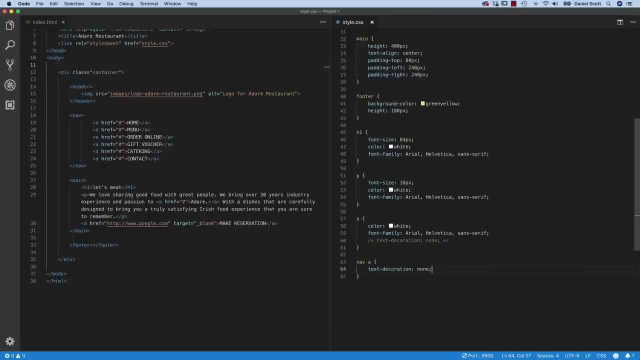 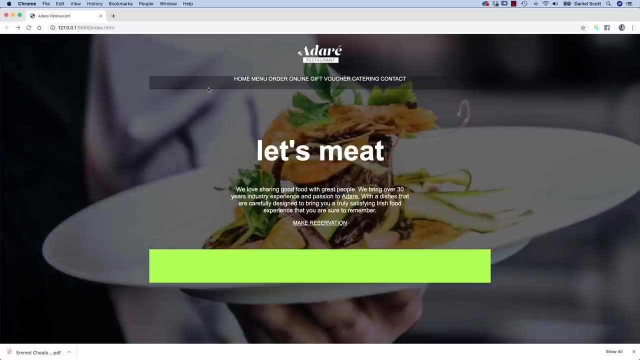 Semicolon done, save. Let's have a little look. is that right Does work? cool, So that one's left fine. but because that one says the A tags inside the Nav, you've got it. Compound Selectors- super useful. 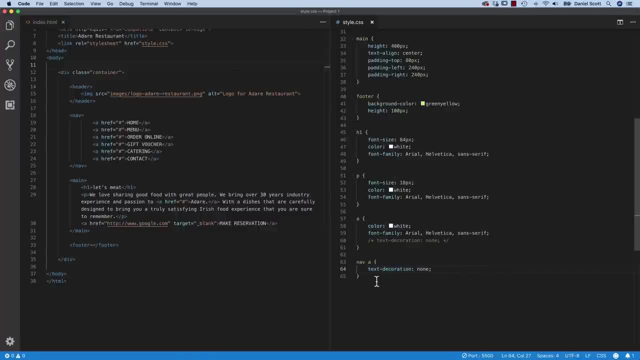 Now, we did it this way because it's the most simple way and it's nice and clean and clear. You could have got rid of this. I'm going to wrap it up in my Command forward slash to comment it out. 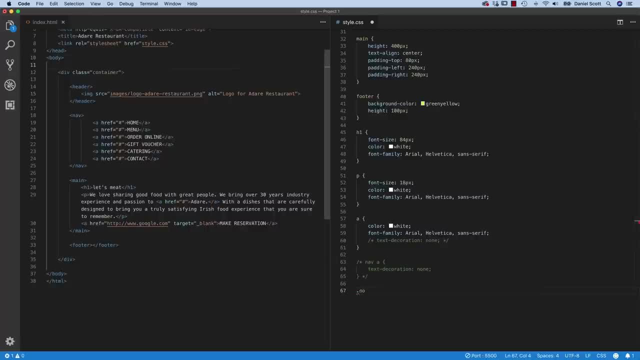 What I could have done is created a class called NoUnderline. I like to show you both ways, because there's nothing really wrong with this way, And over here I'm going to say Text: Decoration is going to be set to none. 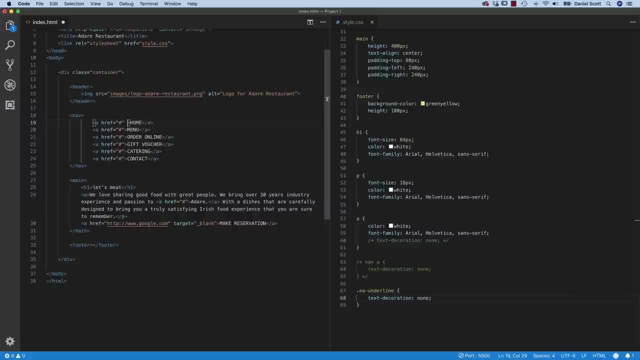 And over here we could say: actually I would like, after the little, after the href there, I'm going to put in a class called what's it called? NoUnderline, NoUnderline, save it, And hopefully just one of them will be working now. 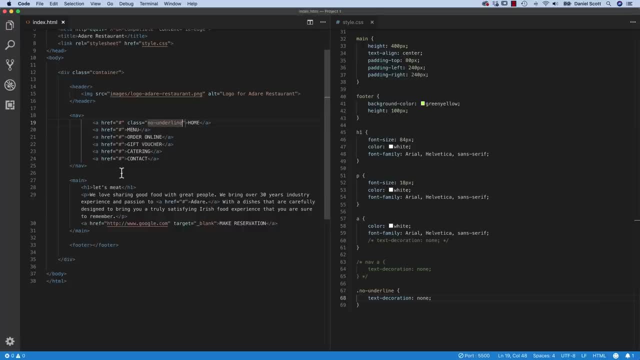 There you go. Now the trouble with that is that I have to apply that class to all of these tags, and that's fine, and if I make another one I have to go and add that class and there's no real problem with it. 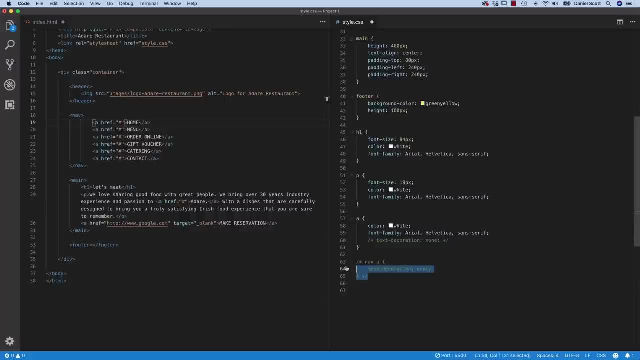 But you can see the elegance of this. first one Is elegance- the word. I feel like it is Awesome. we've learned what a Compound Selector is and the kind of syntax for it spaces. Next thing I want to do is I want to tidy up the padding here. 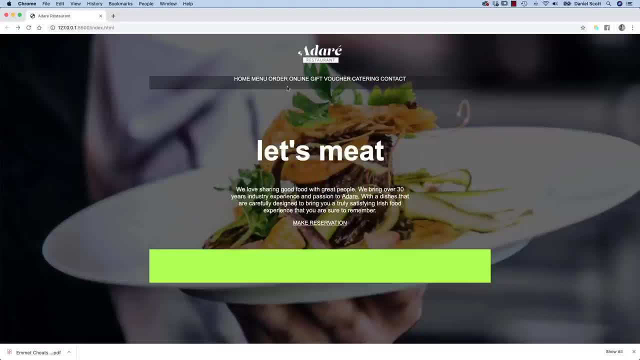 So centering in a box- centering horizontally is perfect, Vertically is very hard, surprisingly hard. Don't ask me why, but it is So. later on in the course, when we look at something called Flexbox, it will get easier. 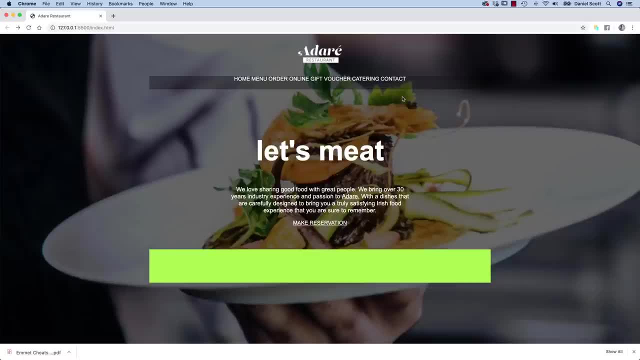 But for the moment, at our current skill level, it's super hard. So what we're going to do is kind of fake it. We're just going to put some padding in the top and the bottom until it looks like it's in the middle. 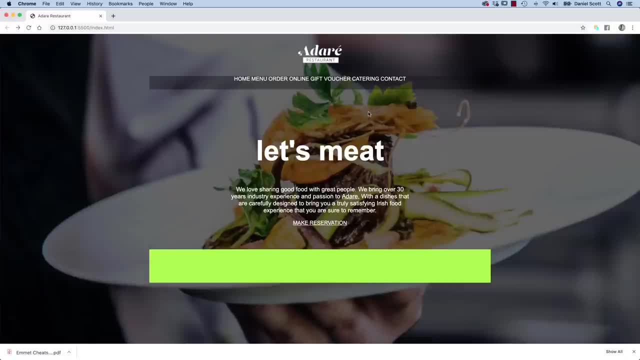 And the easiest way to do this. there's a couple of ways, but the way that we're going to do it is, let's add, we'll add some padding to this nav, Because at the moment it's right at the top. 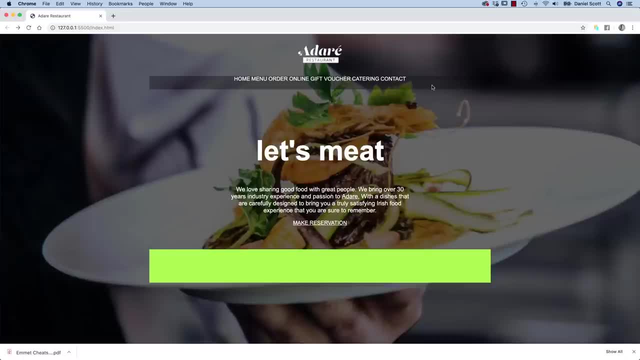 so we'll add a little bit to the top, a little bit to the bottom and maybe get rid of the height. Let's give that a try, So what I mean? So first of all, let's get rid of the height. 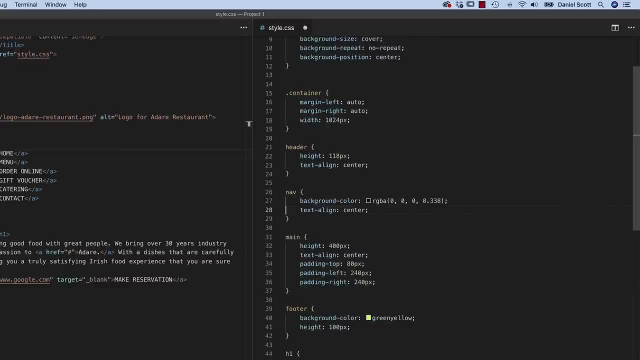 That will make it a bit clearer. So here's my nav height. We can either comment it out or just delete it, because I don't want it. See, it's kind of collapsed, But if I add some padding to the outside of the nav, 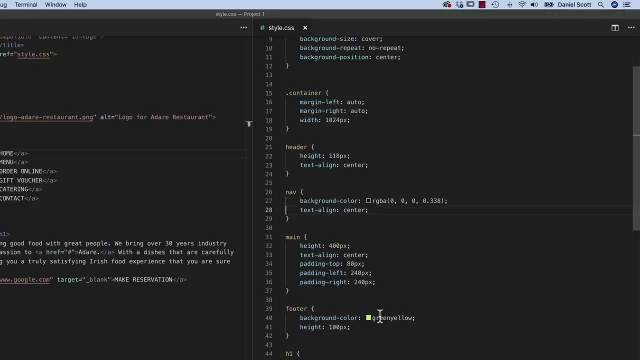 or I could add it to the actual A tags themselves. Doesn't really matter. We're going to do it to the nav just because I feel like it, And we're going to say Padding, and we'll do Padding Top. 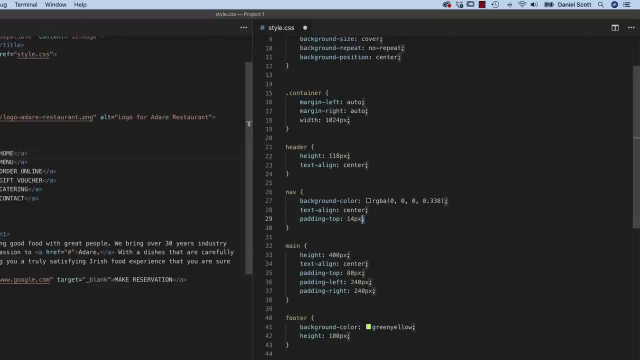 I'm going to make it 14 pixels at the top and the same for the bottom. I'm just going to copy and paste it bottom. Awesome, let's save it and let's preview in a browser. You can kind of see we get to the same point. 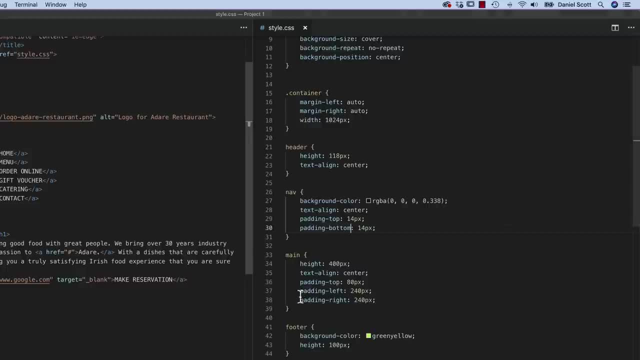 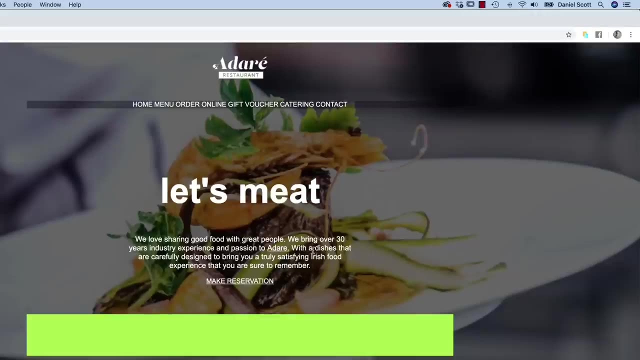 So it was collapsed. now there's padding pushing it out. If we did it with margins it wouldn't work right. I'll just kind of drum this into you: The difference between margins and padding. You can see there is some padding. 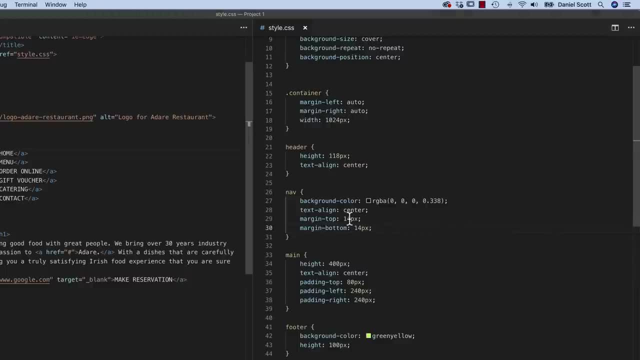 There is 14 pixels above there and below there, because if I crank it up to 140, you can see there's lots of space there. But because it's the outside of the box, it doesn't really do what we need it to do. 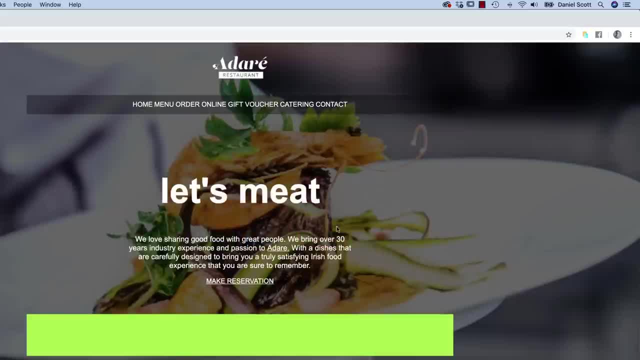 So Undo, Undo, Save Preview. nice, Let's fix up a couple of other things that are bugging me, Like the font size is a bit big and the space between the menu buttons are tiny, So we need to adjust that. 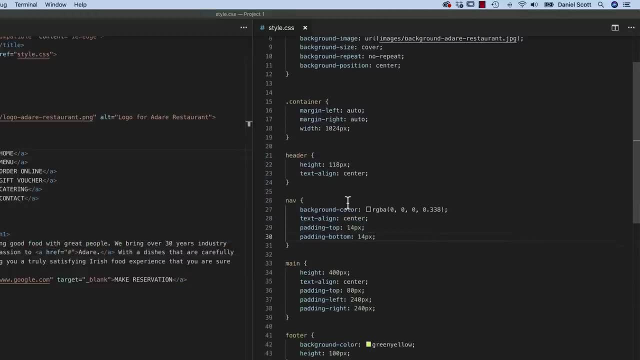 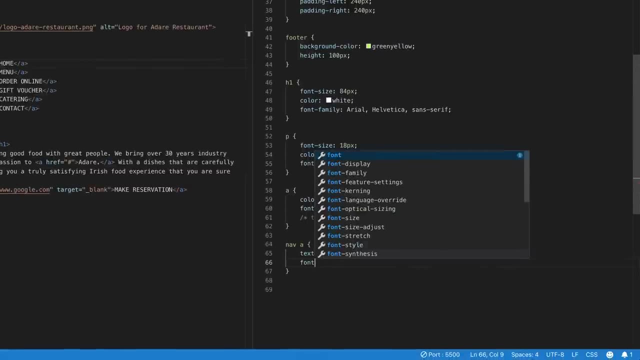 Let's jump into VS Code. what should we do? We'll do it to the NAV A's, Because I want to make this a font size of what are we using? A font size of 12 pixels. I want it quite small, to kind of match my design. 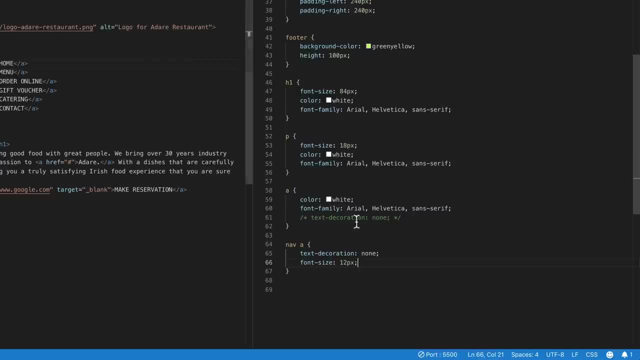 Let's have a look save. that's a bit better. Now let's do the space between them all, And what we'll do is a little bit of padding. It won't matter if it's padding or margin, in this case Padding. 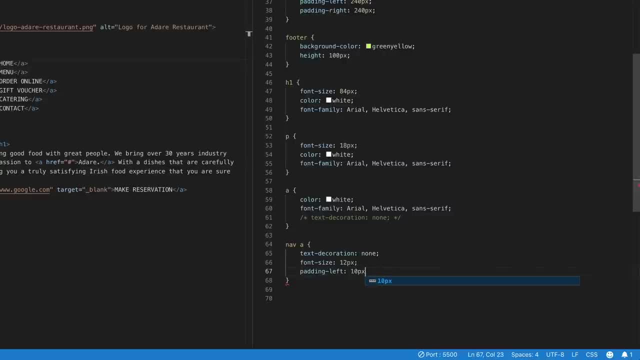 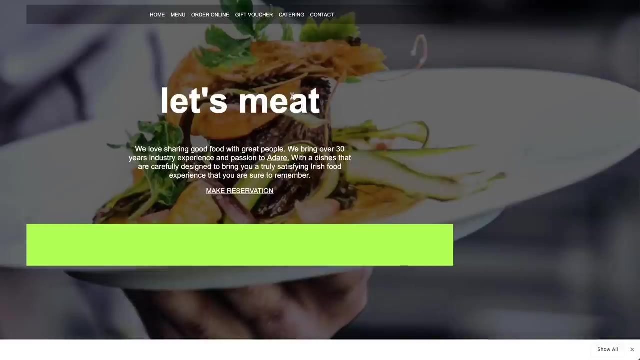 And left. I'm going to put in 10 pixels And I'll do the same for the right Padding right: 10 pixels Have a little look Awesome. Why did I do both? Because if I do that, it's going to be slightly lopsided. 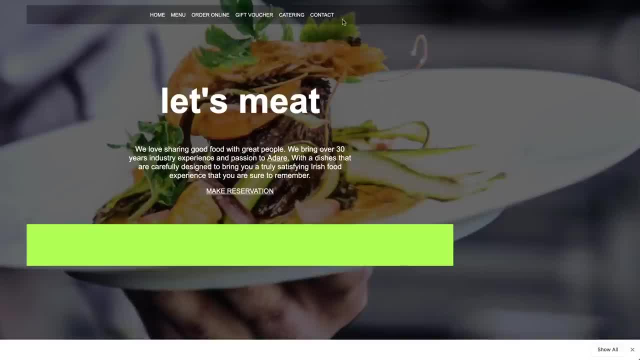 It's going to look fine, but it's going to be pushed one side And I guess you can't really notice it on this. So imagine we've got a bit of padding to one side but not the other On each of these. 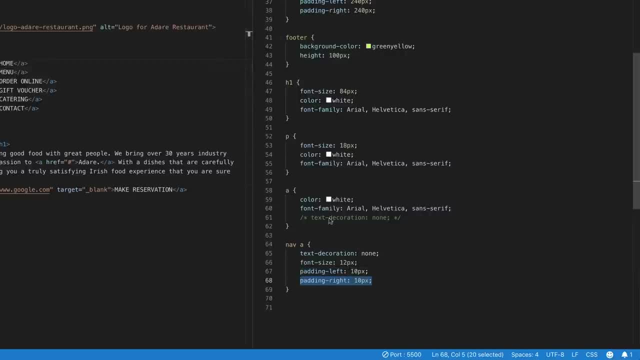 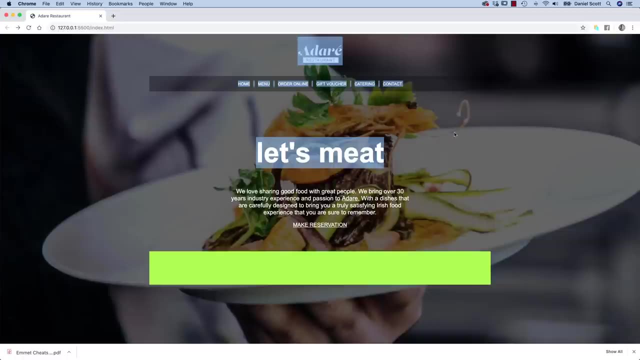 So it really visually doesn't look any different. but you've got padding either side now. I just kind of often do that: I just grab my cursor and click over it and drag to try and highlight it and it gives me kind of a vague. 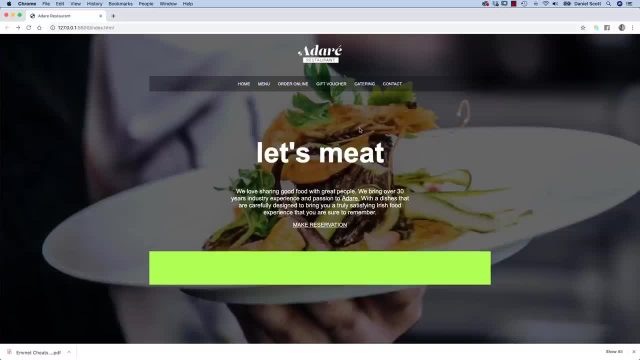 kind of just an idea of what's happening. So that's our basic kind of navigation. they don't go anywhere. yet We've got an index page, so we have to create a menu page and an order online page, but we've only made one so far. 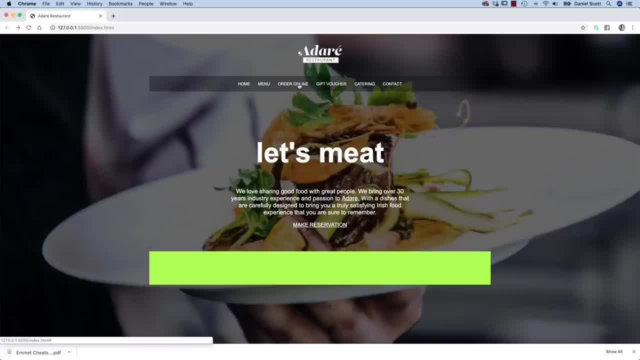 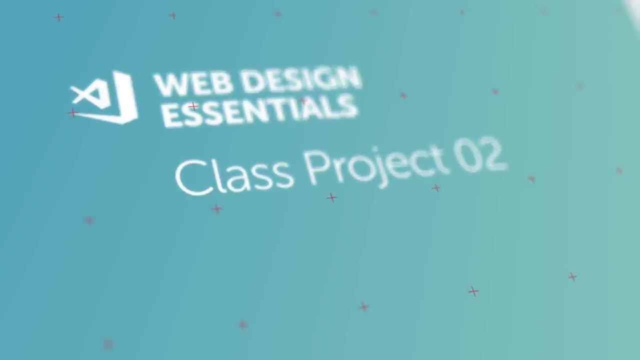 So we're just using those hashes or pound symbols just to kind of make them active, but not actually make them go anywhere yet. All right, that is it for our really simple navigation. Let's get on to the next video. Surprise, it's homework time. 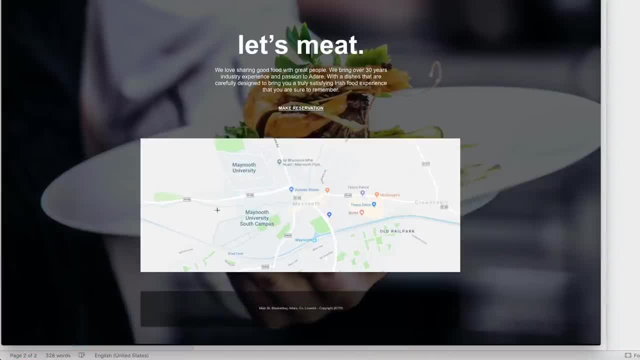 You've got all the skills now to recreate this footer. At the moment it looks like this in the browser: this green thing. Don't worry about this big map in the middle. We're going to do that in a little bit, But I want you to focus on from the map down. 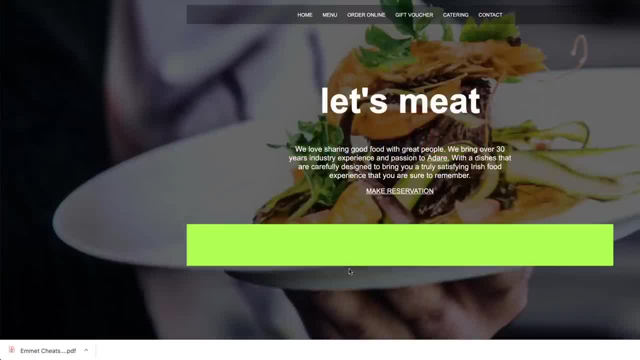 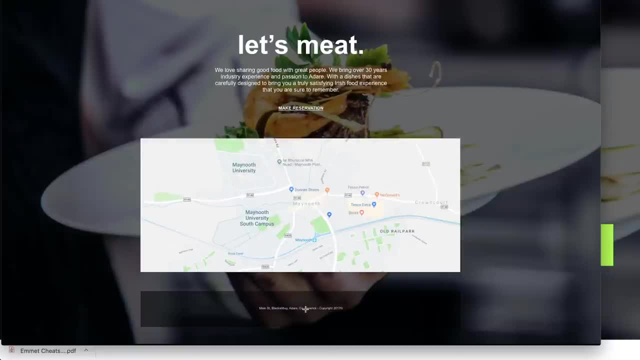 So you're going to be focusing on kind of this part. So what I want you to do is I'd like you to make it look like that: Is it padding? is it margin? How do we get it in the center? How do I make the font smaller? 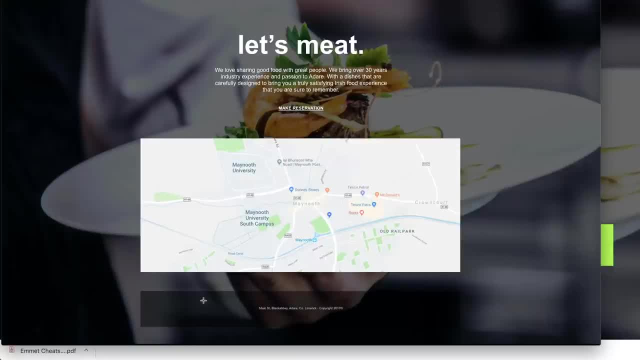 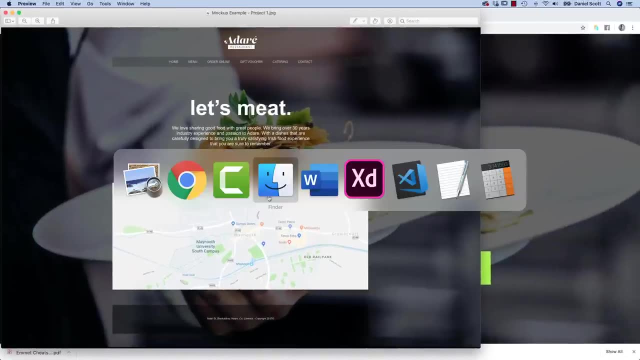 I want you to wrap it in a P tag and I want the background to be black, but transparent, but not as transparent as that, so that's a bit darker. Those are the rules. let me check your remember in your exercise files. 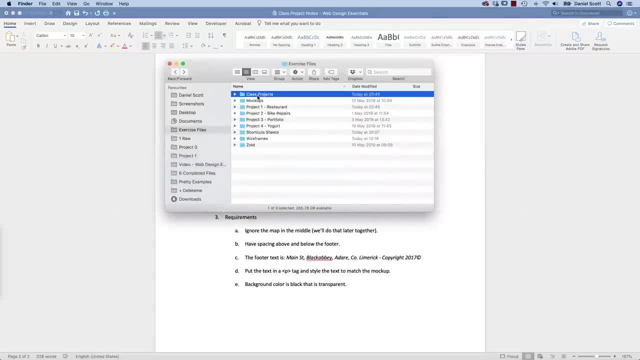 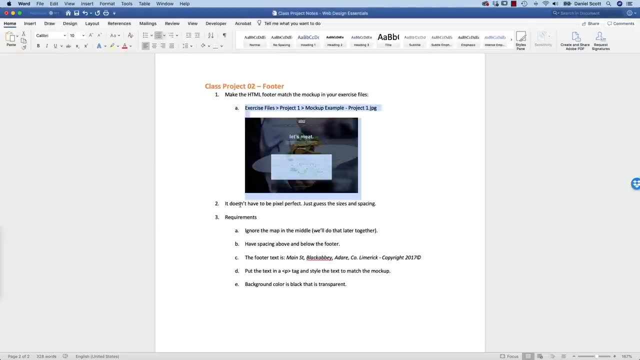 way back at the beginning of the exercise files, there's one called Class Projects and there's a Word doc in here. That's it here and this is Class Project 2, so run through this. There's the mock-up I just explained. 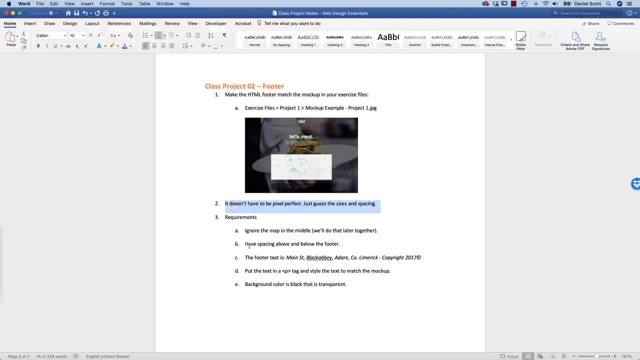 It doesn't have to be pixel perfect, anything else, ignore the map, The spacing. above and below the footer There's the text for it And just make sure it's in a P tag. You could skip that, but let's be proper. 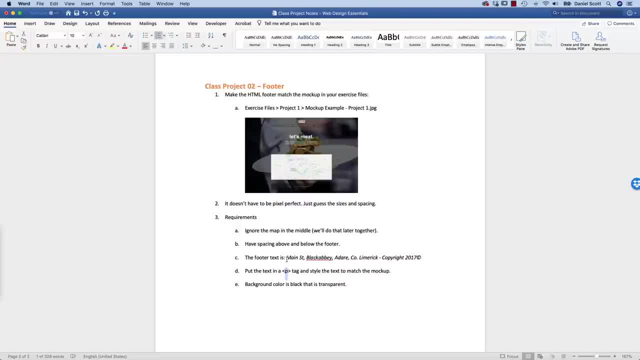 Let's put it in a paragraph tag and then style that And a little hint, you're probably going to need a compound selector. That's kind of what I'm trying to hint and get you to do in this. one Background color is transparent. 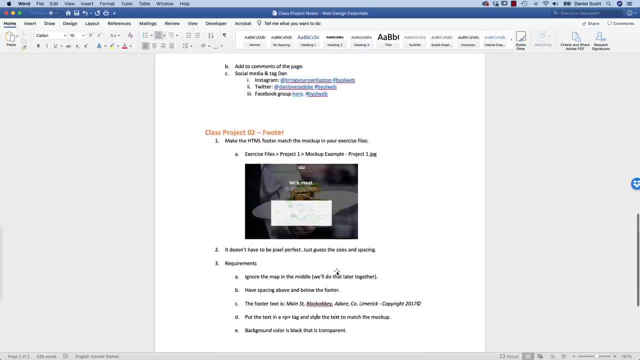 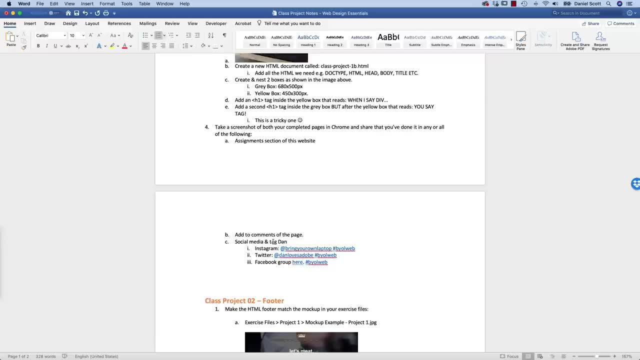 And that's it. Once you've done it, take a screenshot and share it with me on these. so in the Assignments panel, just take a screenshot, stick it in there, If you've, depending where you're watching this. 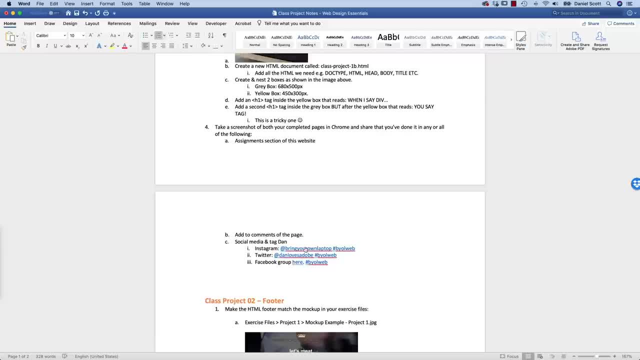 in the comments, in the Assignments and send it to me on Instagram. Keep you honest, Send it to me and say: look, I got this far and I did it without cheating. And what I mean by cheating is opening the completed files. 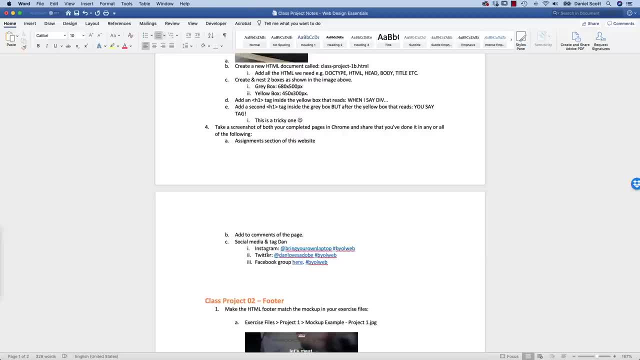 and or watching the next video, where I go through it and show you how to do it. It'll prove to yourself you can do it And share it with me. make sure you use this hashtag, Hashtag, BYOLWeb. And yeah, that is it. 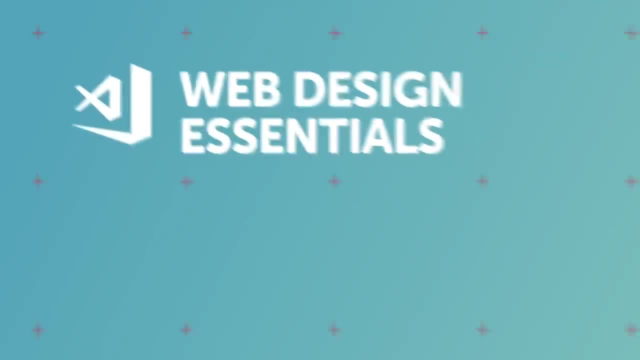 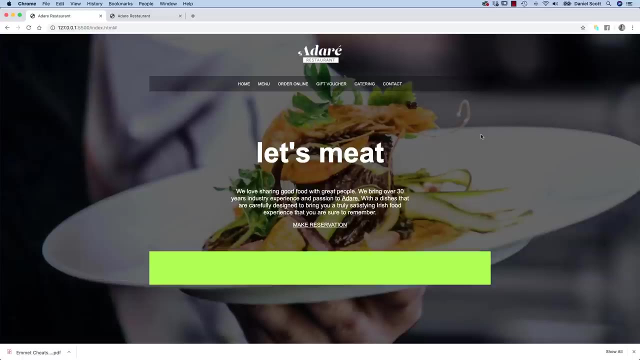 Go to your homework and I'll see you in the next video. Welcome back. How did the homework go? You're either sitting there smug thinking, yep, I did it, I'm a web designer. I smashed out that footer and it looks great. 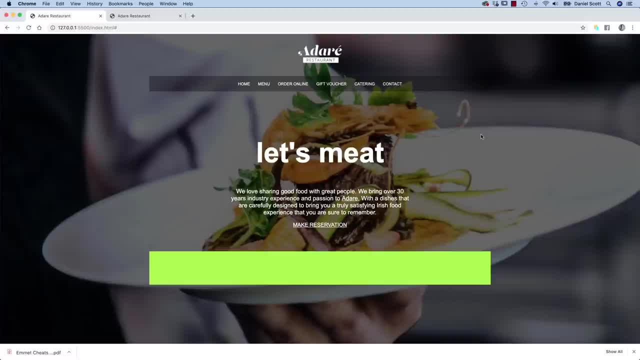 Or you're sitting there going. you're not as good teacher as you think you are, Dan. It went badly and the site doesn't work And my computer caught fire, Which, either way, I'm really happy with, Because this is the beginning. you're new. 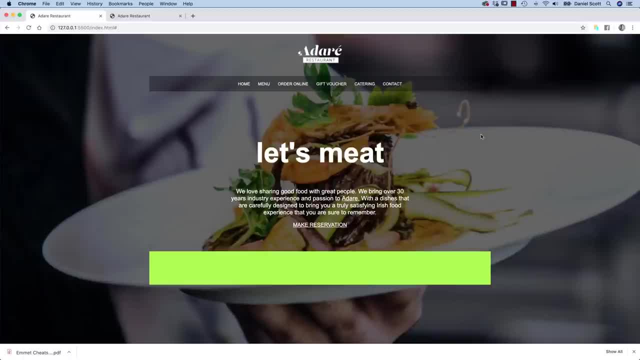 If you skipped it. this is where I'm touching. I'm shaking my finger. You can't see it, but I'm touching, shaking my finger. You should have done your homework, but if you haven't, that's all right. 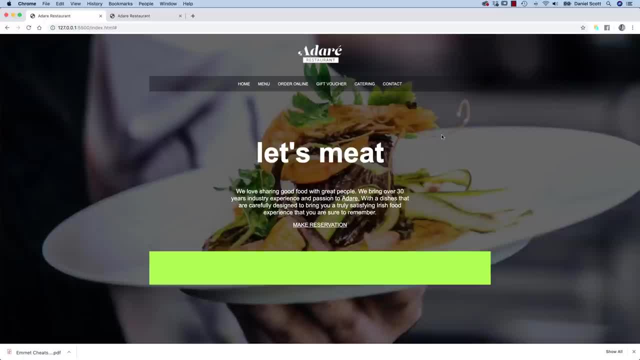 We're all here now. let's go through how I would do it. There's a couple of ways of doing this. Let's do the way I did it. If you got to a good solution, that's perfect. but let's just see. 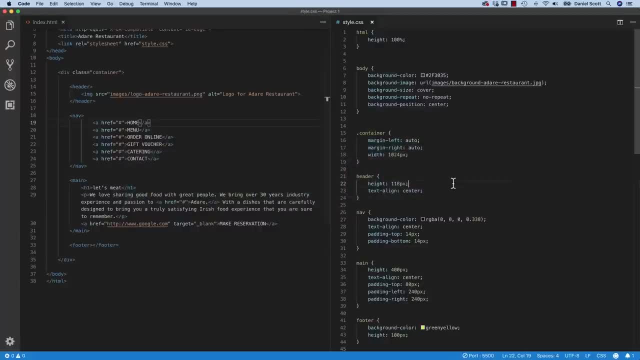 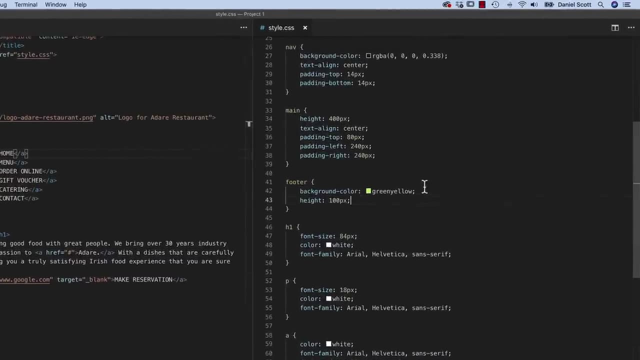 Let's head over to VS Code. and where do we start? I wonder where you started. I'm going to start with. I feel like I want to color the background first for some reason, So let's go to the footer. it's an easy one. 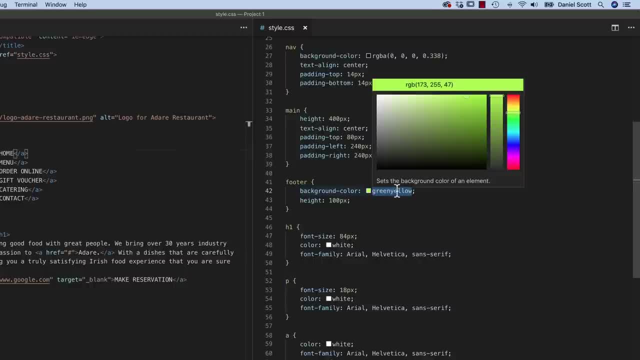 Get rid of this And we could just type in black. but we could actually just hover above this and drag it down to this bottom corner. I'm just dragging it past where it needs to go, letting it go And then coming back and just dragging it down. 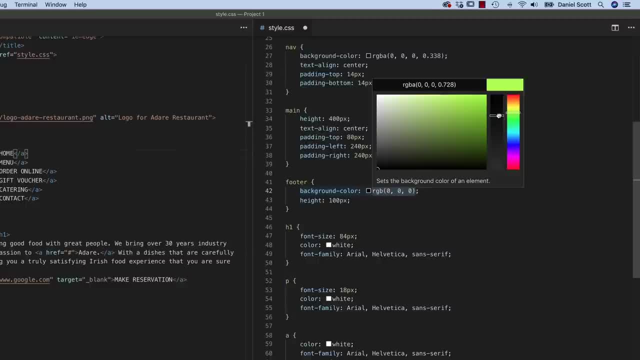 Now I kind of said about 80%, but How about that? save it Preview in the browser. It's kind of see-through. maybe how dark It doesn't really matter, but we got the idea right. There is some black and it's transparent. 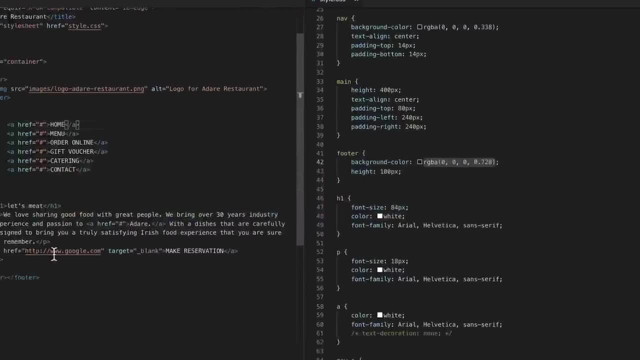 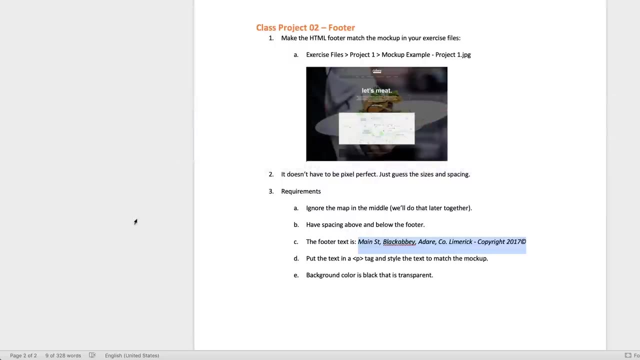 Let's add the text in the hot side here. So let's find the footer, Let's add our P tag, Let's go and find the text There. it is there And paste it. Awesome, save it. see what it looks like. 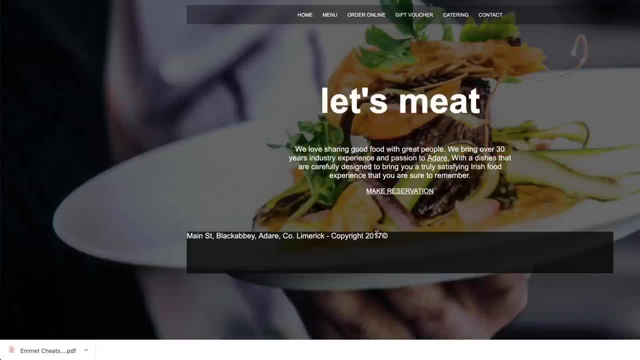 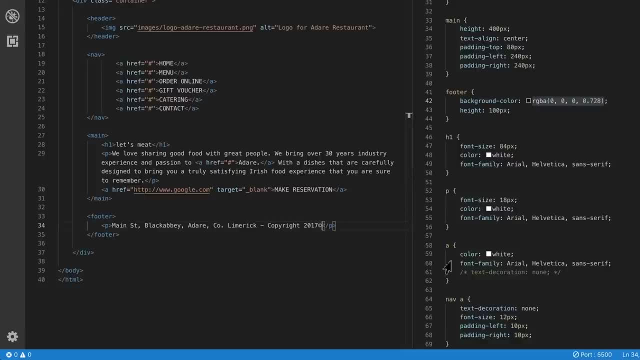 That's where we're at. Let's do a couple of things. Let's maybe make it smaller and center it, and center it horizontally, because that's the easy one to do. So this is where I wanted to. you could actually just style the footer. 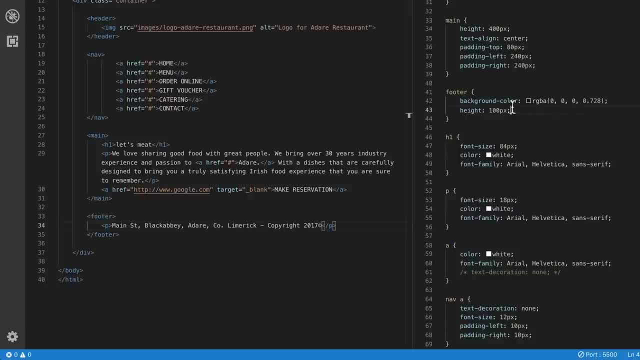 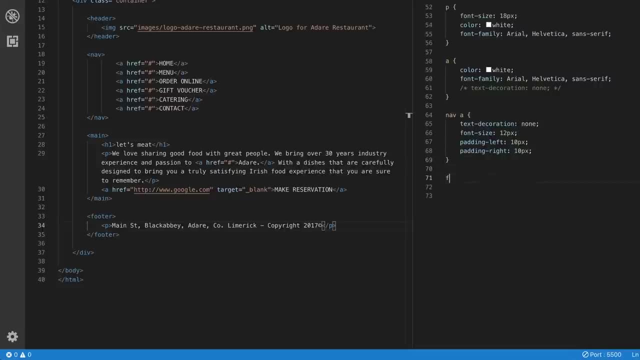 You could say I want it to be a font size here like, say, 10 pixels, whatever you picked, and it would work. The reason I kind of suggested doing a compound selector, so something like footer that has a P tag in it. 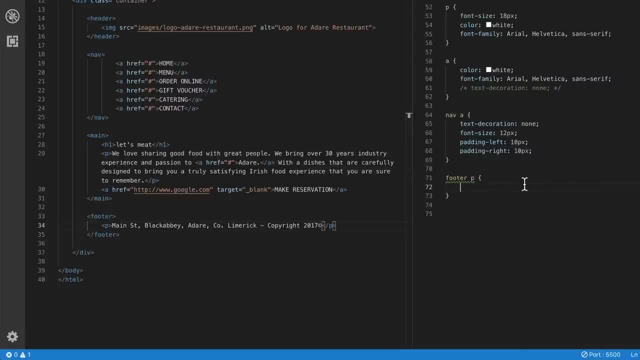 is so that if you've got like an image inside of there as well, or say some links or lots of different things, you can be really specific about it. You can say: I want the paragraph text that's inside the footer. 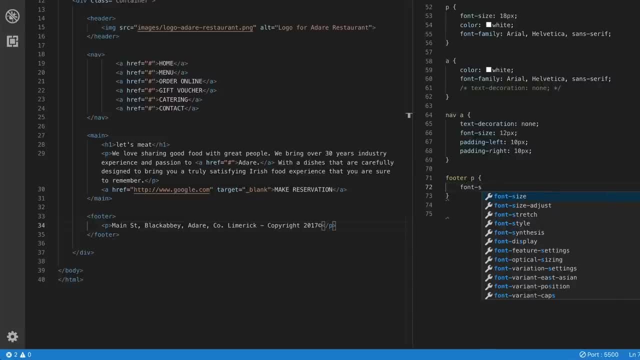 It doesn't really matter how you did it, as long as it worked. We'll do font size. I did 10 pixels. Let's give that a bit of a test. every single time Let's make sure it's working. Let's do a text align center. 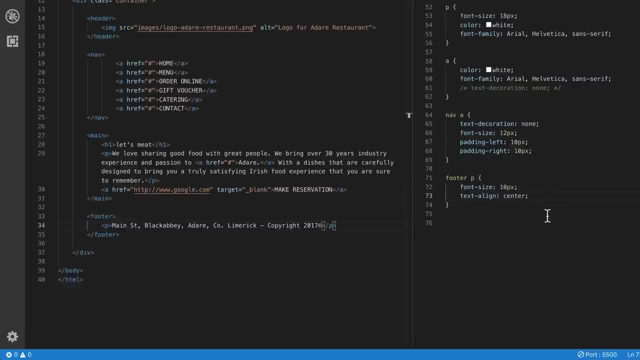 How are you going so far? Is there like moments, or is it like: yep, I did that, nailed it, So we'll look. it looks perfect. I made mine slightly darker. it wasn't white. You didn't know that. 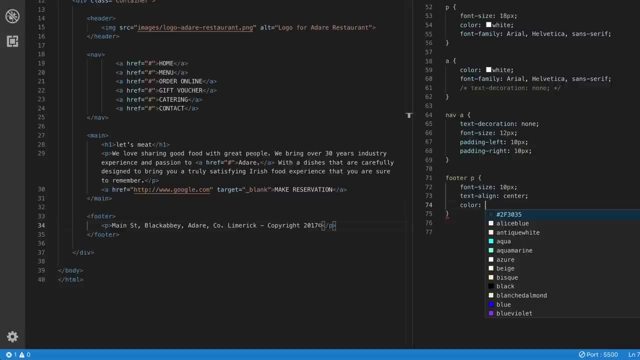 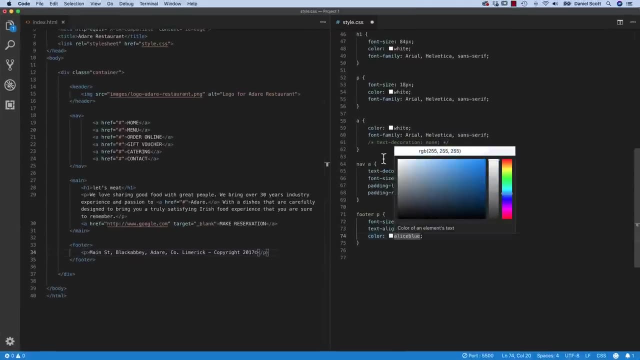 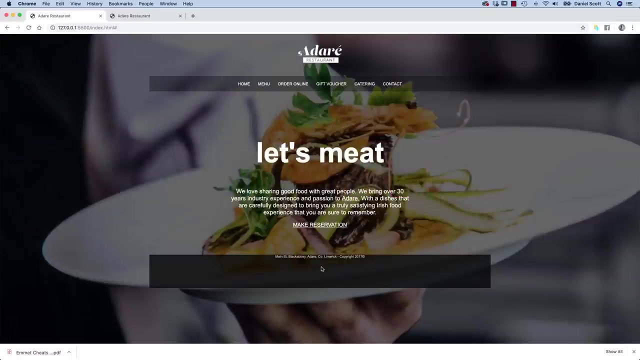 Color. I'm just doing this because I wanted to be a slightly different color. Like it's changing the rules, I want it to be a slightly muted kind of gray. It's too bright down there. All right, next thing I want to do is get the spacing right. 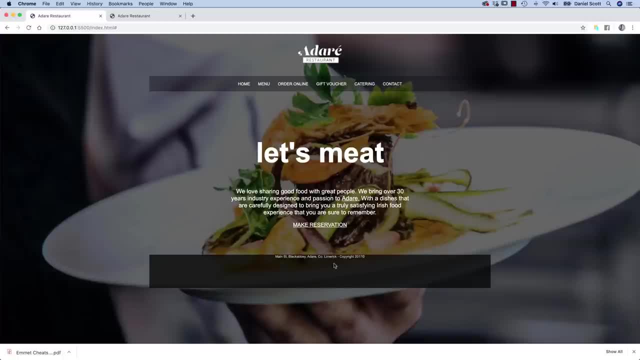 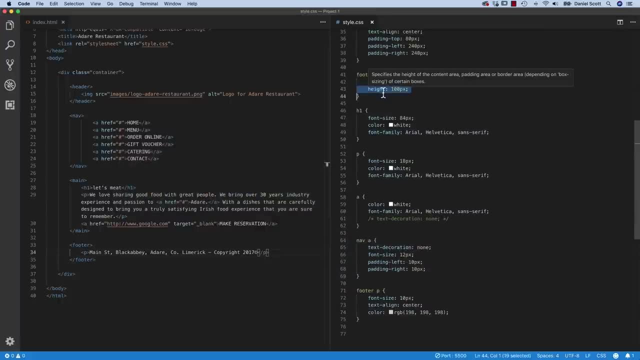 And how did you do it? Did you leave the bottom? play with the heights, play with the margins. This is how I'm going to do it. I'm going to get rid of the height off the footer. Remember, at the beginning, we added loads of heights. 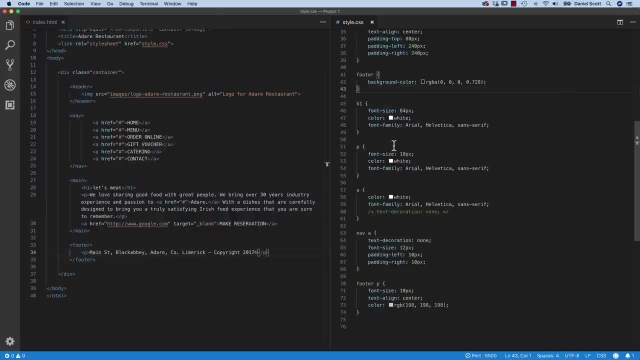 and we're slowly removing it all because they were just useful at the beginning so that while we're learning we can see things. But now it's fine to leave it like that because I know later on, while I'm building it, I can say: 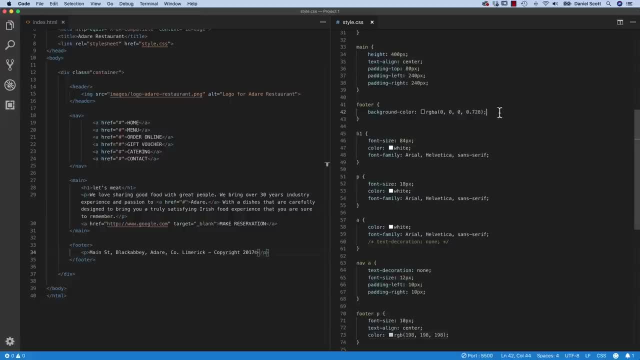 do I do it to footer P or to the footer? I think you can do it to either. I wonder what you did. Leave in the comments what you did, If you're like: hey, I did this other thing and it still worked. 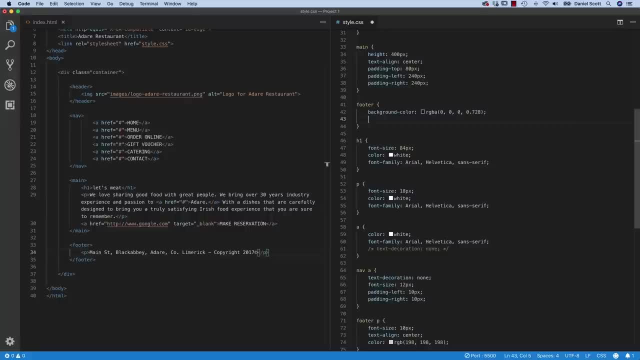 do that because then other people might say: yeah, me too. I did it this other way. There's a better way. Dan's writing it badly. I'm happy for that. So for the moment I'm going to do some padding off the top. 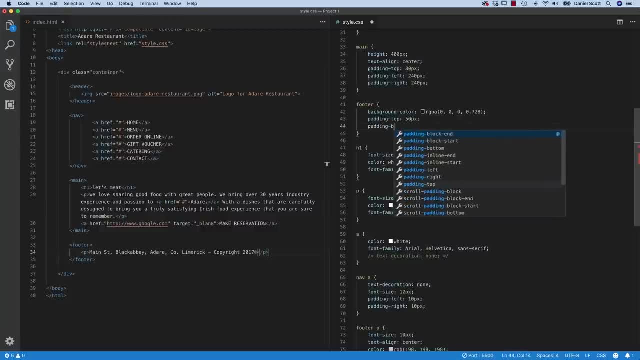 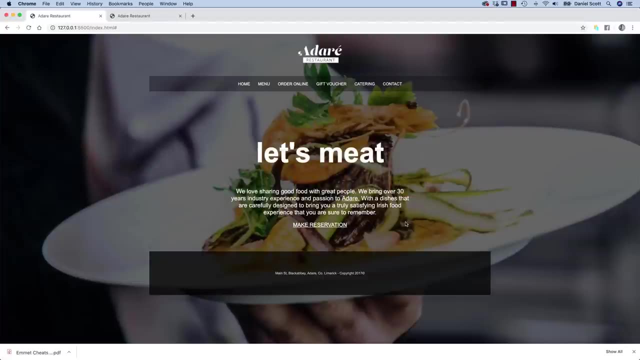 50 pixels and same for the bottom Bottom- 50 pixels. Let's check it. That's kind of where I wanted to get to. Did I fulfill all my brief? Ignore the map? did spacing above and below perfect? 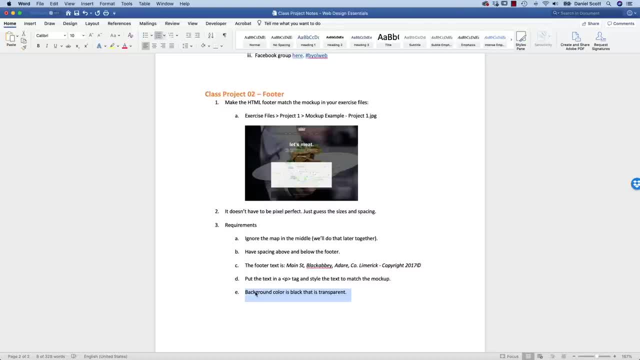 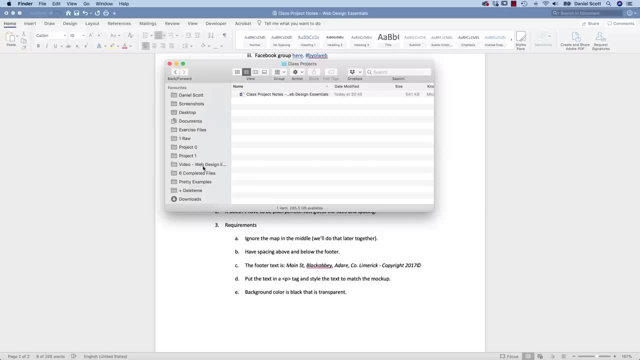 Footer, the P tag background color. we did it. If yours didn't work, I'm going to save this file now and put it into the completed files. Just to recap the completed files, because they're super handy under your exercise files. 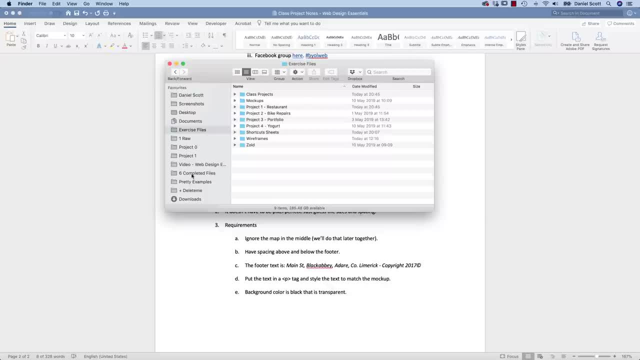 There'll be a folder in here called Completed Files. I'm keeping them separate while I'm working in this course, but I'll dump this whole folder in there when I'm finished. You'll find this one and you can see. these are all the different videos that we've made. 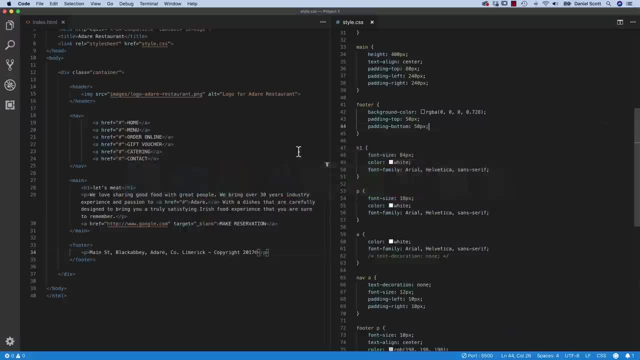 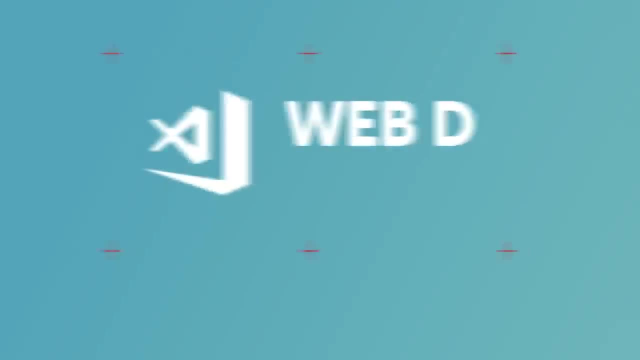 Open them up and you should see the code that I've got here. You can compare. That was our footer project over. Well done you. Let's get on to some new fancy stuff. Hi there, this video is all about adding a really simple email button to a website. 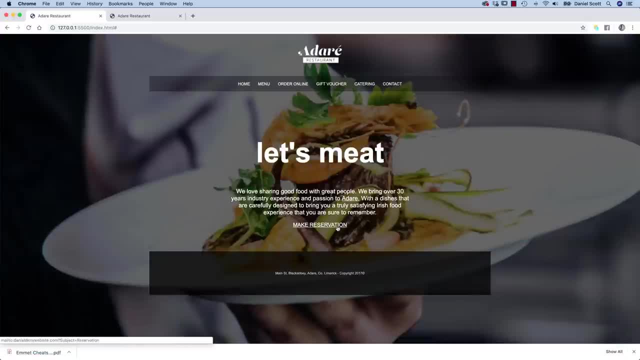 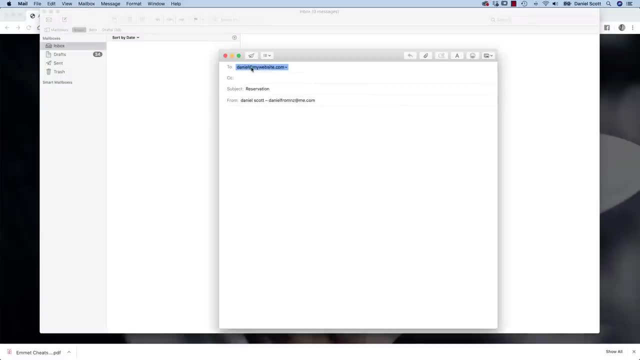 We had this link that we made earlier and when we clicked it it went to Google. That wasn't that helpful. What we want to do now is when we click it, it opens up our email campaign and sends us a website pre-fills in. 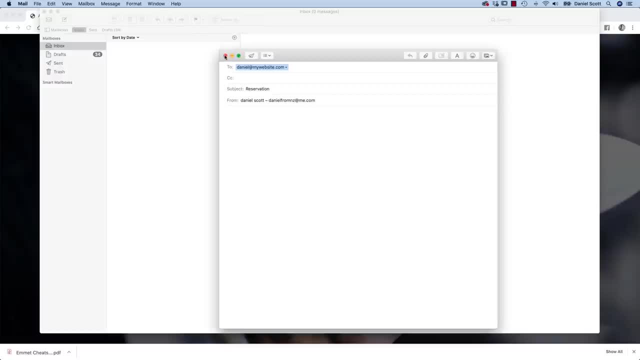 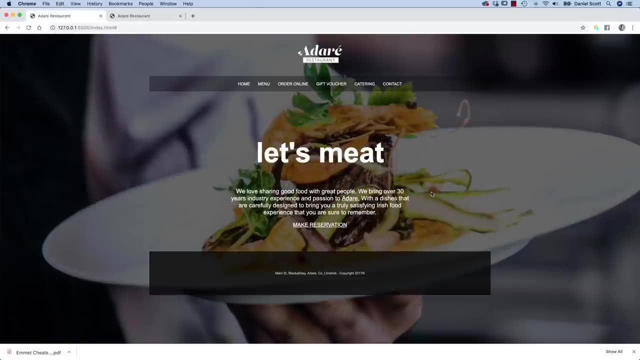 and the subject line's done. It's a nice little handy, quick, super easy, quick trick to add that sort of functionality to your website. Let's jump in and make it happen. To make it work. we're going to do it to the button. 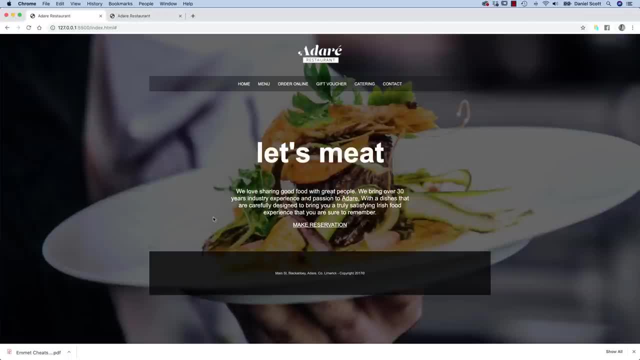 that we've got here. at the moment It doesn't go to Google, It'll go to another web page. I want to get it so that when you click it, so I'm the user, I'm at this website, at Edea. 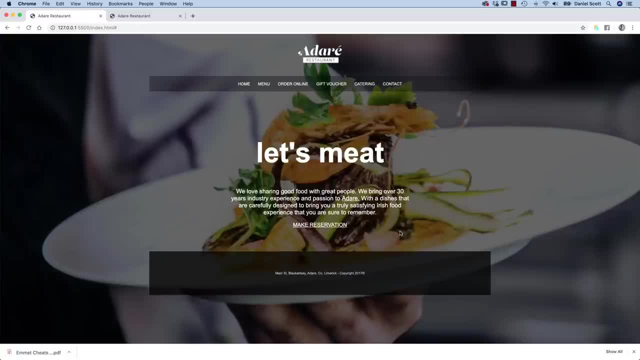 I want to click it and send an email for about a reservation, Doing a form we'll do later on in the course, because it's pretty hard to do, Not pretty hard? yeah, it is pretty hard, We'll do it later on. 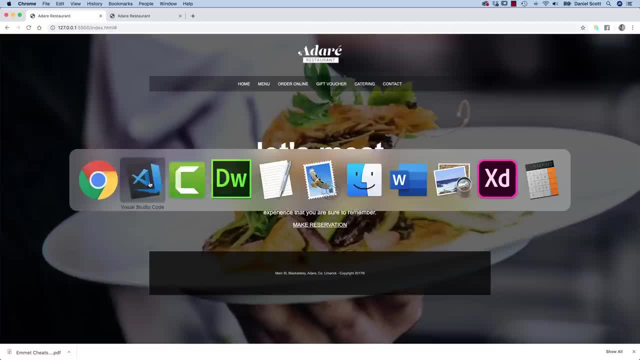 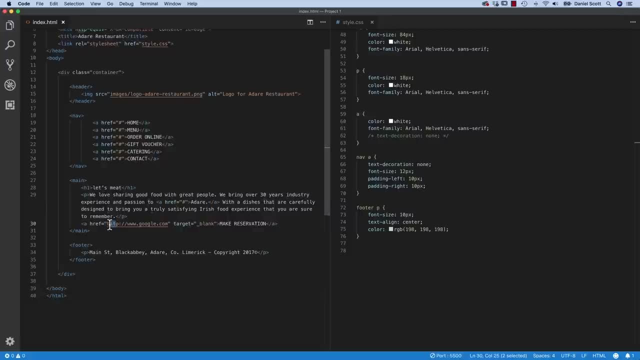 But for the moment, a little mail to thing is going to be nice and simple and quick and easy to do. So all we need to do is we did this href earlier on. If you haven't done this one, look for making a hyperlink video earlier on. 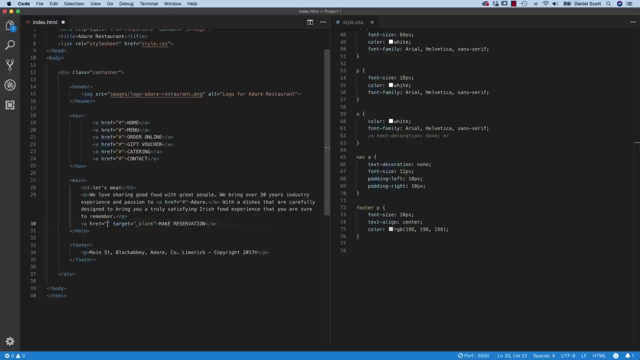 All we need to do is switch out this part. So instead of going to googlecom, we're going to get it to go to mail, to colon. so it has to look exactly like this: Then you put in the email address: no spaces. 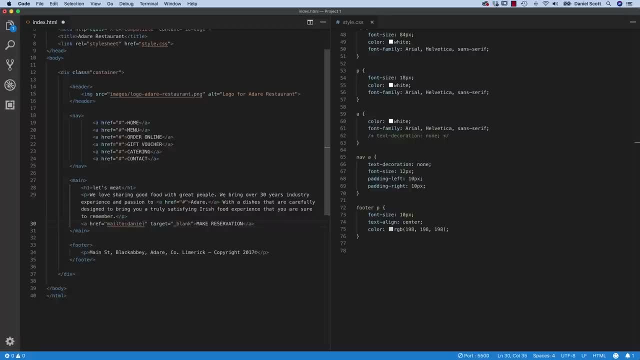 So if you wanted to email me, you'd email Daniel at my email, my website, mywebsitecom. So when somebody clicks that they're going to, we'll show it target blank. yeah, why not? It doesn't really matter in this case. 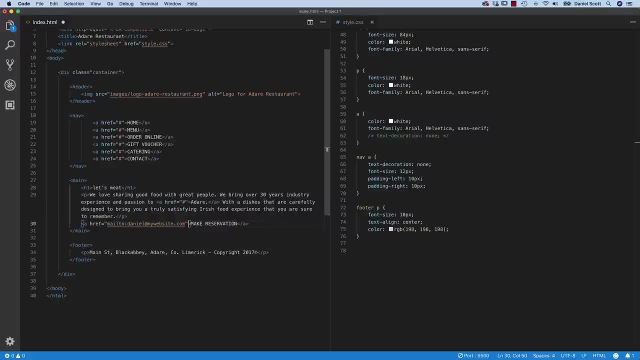 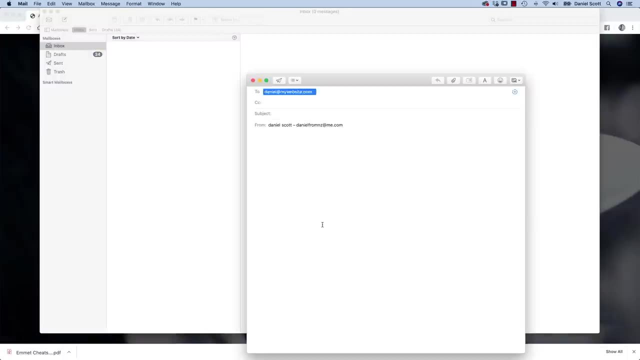 because it will load up in its own blank thing, And that is it that should make it work. Let's save it. let's give it a preview. Let's click it. look at that: It opened up my email system. I'm pretending I'm the client now. 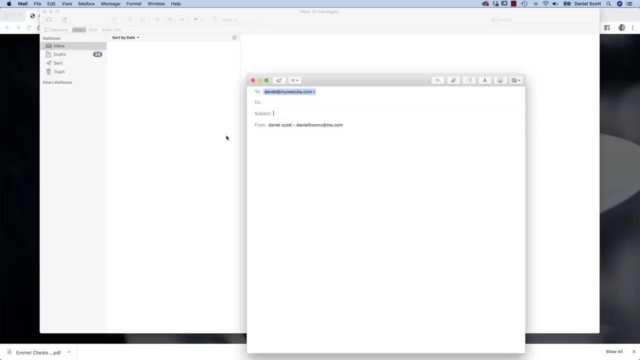 so I'm just searching the internet for a restaurant. I'm like, oh, let's make a reservation. Click the button, this opens up. So it's opening up mail and wants to. I can write a subject and I can say: could I get a booking? 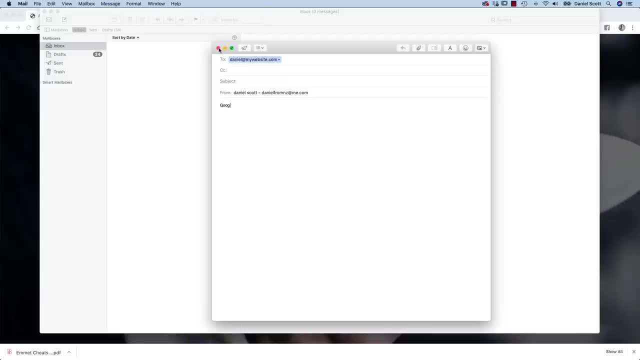 It's a nice, cheap, easy, quick way right, So it's five seconds to implement and heaps easier than a form. A couple of things that might be handy is adding a subject line, like pre-filling it in. 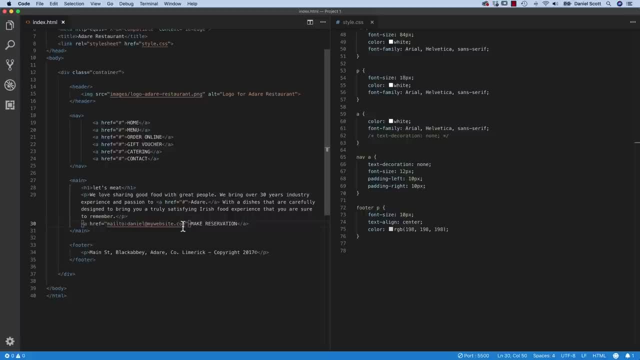 So what you can do, you can add a little bit of extra to the end of this. So mail to is cool, but at the end of the dot com put in a question mark. you got to put a question mark and it has to be spelt like a capital S and it has to be subject: 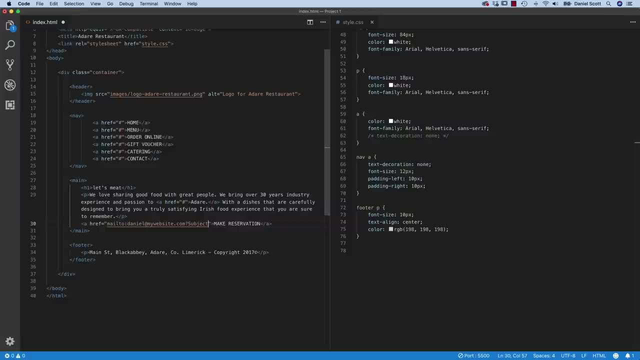 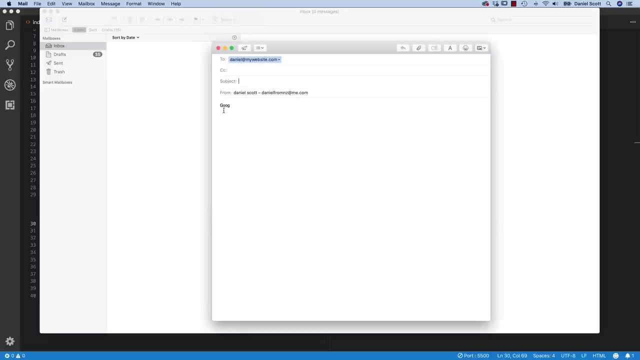 So question mark: capital S for subject, and then you can put in an equals. So it all has to look exactly like that. Then you can just add the subject line So you could say: reservation, Cool, let's hit save and let's preview it. 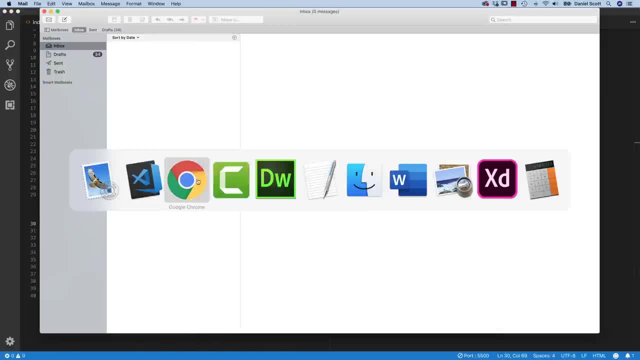 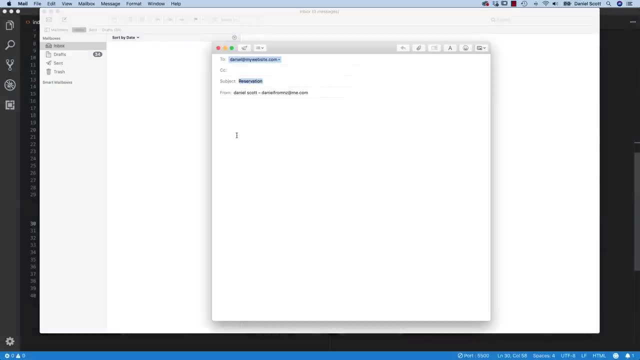 Let's close it down. Yeah, let's preview it in the browser. Let's click on it. You can see it loaded- my email and put the subject in. Cool, you can do some other things, like adding the CC, and can you put body copy in? I think you can as well. 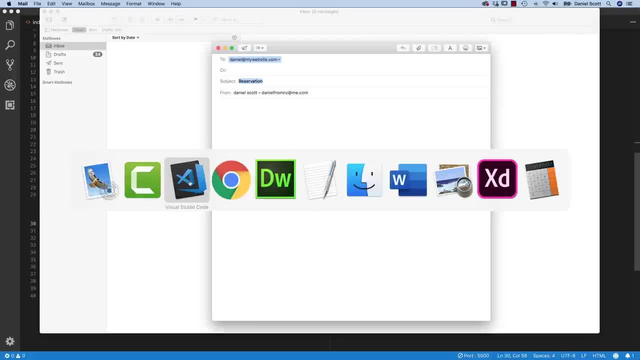 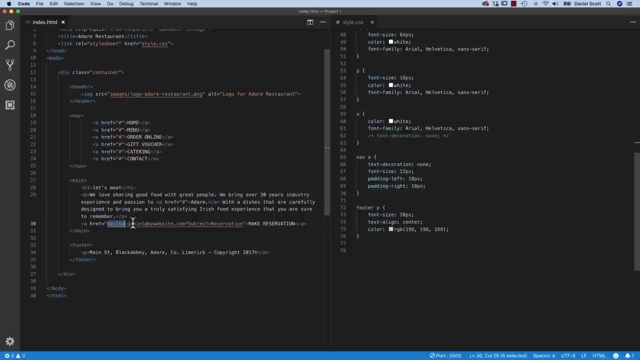 I don't know them off by heart, but you can go and have a look at that yourself now. All you need to really look for is search for mail to in HTML, and you'll find a page on what you can and can't add. 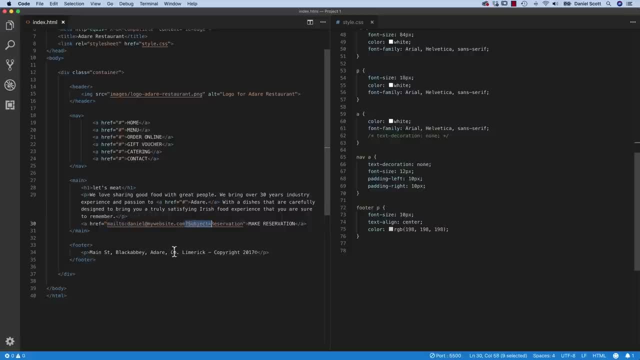 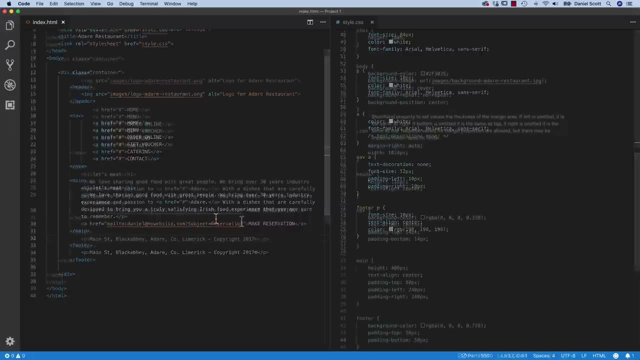 and it'll just be different things like this: I imagine it'll be a question mark, CC equals and you put in another email. But that's a guess and just a nice little cheap trick for adding an email. So that's it for this one. let's get on to the next one. 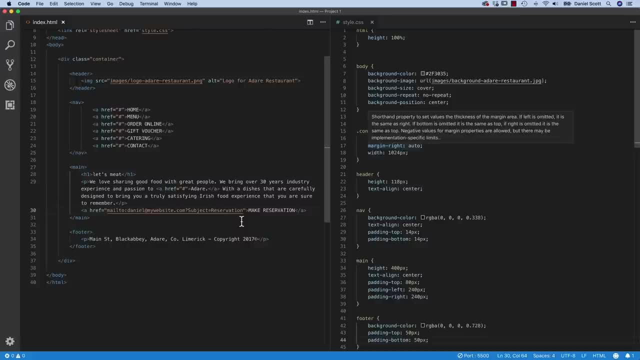 If you're thinking that'll be the last one for tonight, I'll do some more tomorrow. Do the next one, the next one's awesome Embed Codes. it's going to make us look awesome. It's that map. it's not going to take too long. 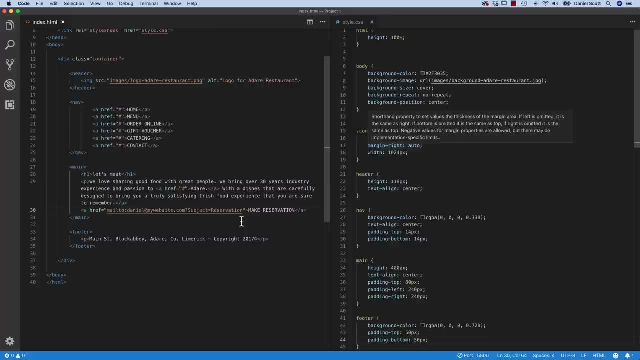 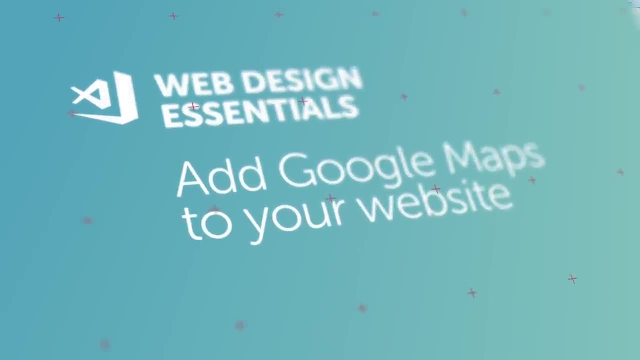 All right, I'll either see you in a few seconds or I'll see you tomorrow when you wake up. All right, bye now. Hello, good looking people, This video we're going to look at something called an Embed Code. 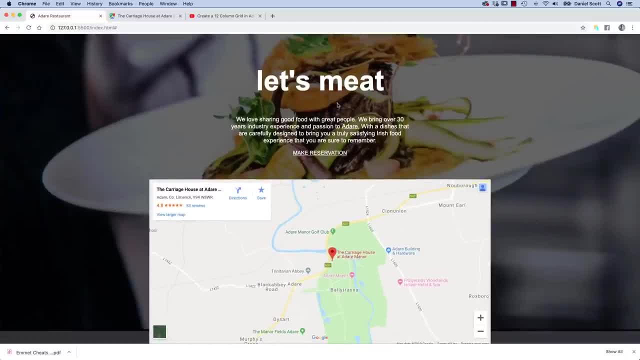 And we're going to start with this one here. See this: it's a map. it's on our website. It's interactive. it shows us where our restaurant is. It's super easy to do. Google does all the work. all we do is copy and paste stuff. 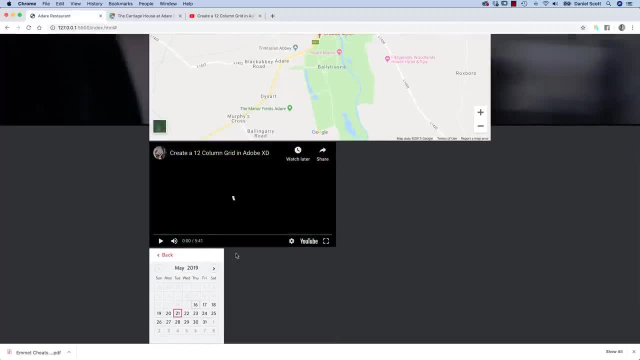 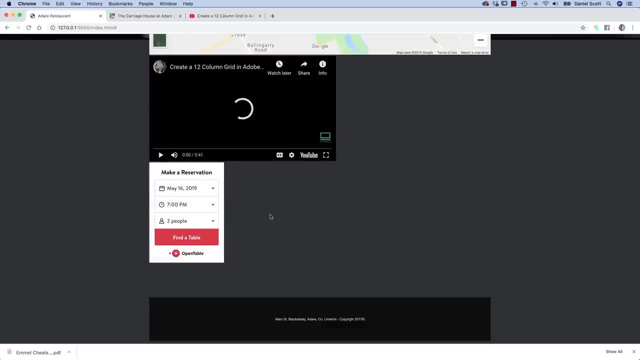 Later on we'll add a video as well from YouTube to our website and we'll add this cool booking thing where somebody can make a reservation. We're not doing it, we're not coding it, we're not styling it. 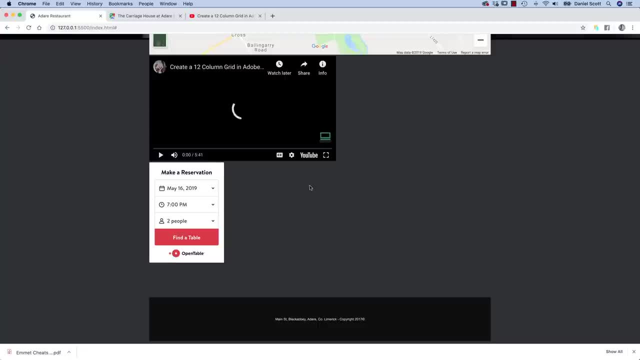 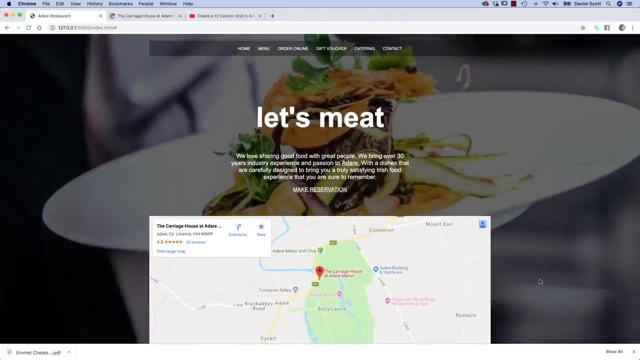 We're just going to these websites like YouTube, Google Maps and OpenTable and they are giving us all the things we need. we just copy and paste it and we look awesome. All right, let's jump in now and work out how. 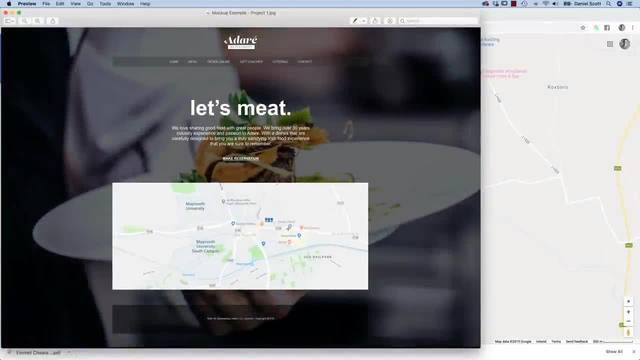 All right, so this is what we want to add, right? It's just kind of a screenshot. at the moment it's not actually working, So we want to add it to our website. And the cool thing about things like this: we're going to do Google Maps here. 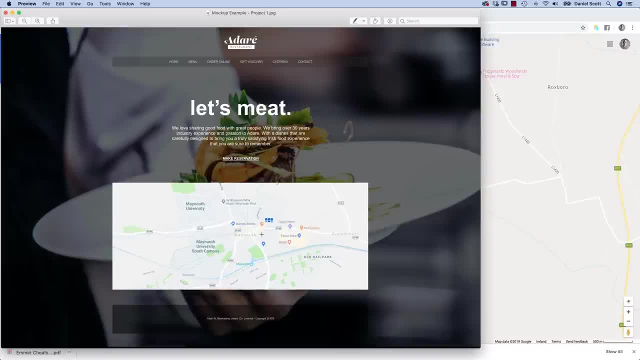 but you could have a calendar from Google Maps here, a spreadsheet from Google. what else? You could have ticketing from Ticketmaster or Eventbrite. You could have Facebook feeds or Twitter feeds. They all use the same sort of method. 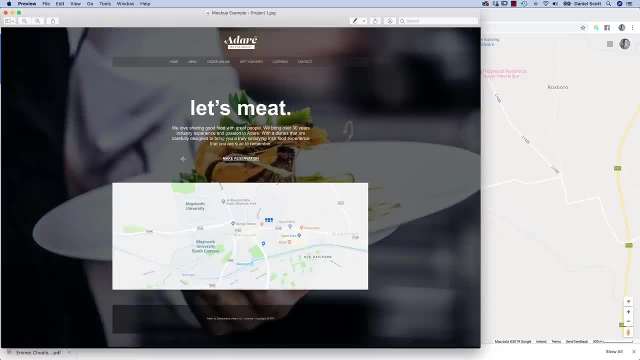 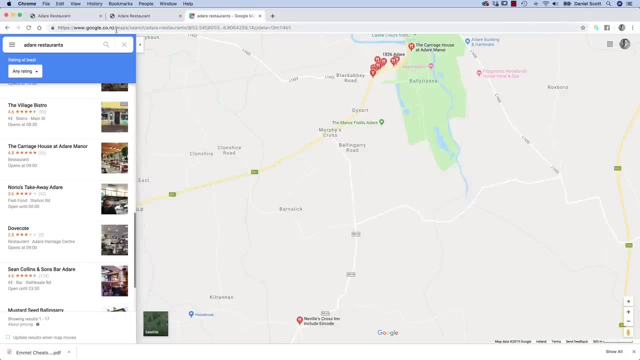 it's called an Embed Code. it's generally in something called an iFrame. So first of all, let's go get the code. So we're going to do. we'll use Google Maps, and I've just loaded up a New Zealand version. 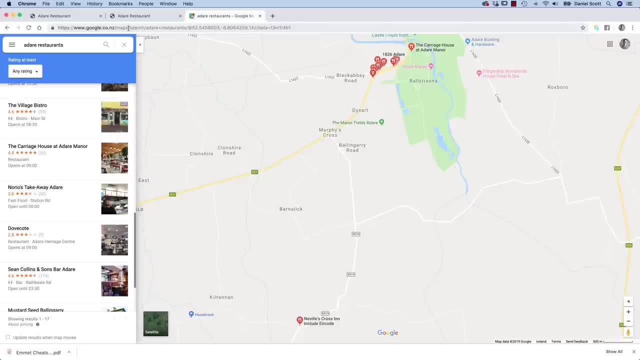 but go to googlecom slash maps- I've gone to conz, but anyway it doesn't matter- And then type in the business that you want to list. So type it in, find it and let's say so. this is where I'm going to move to. I'm pretty excited. 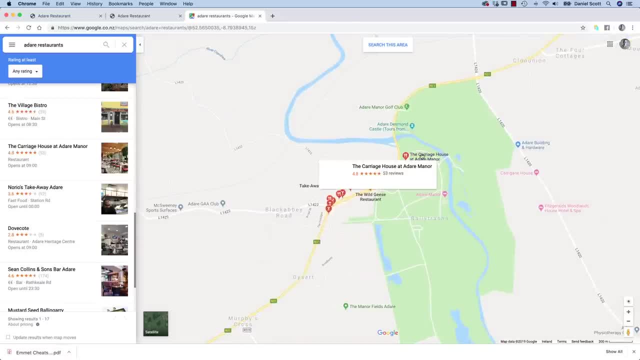 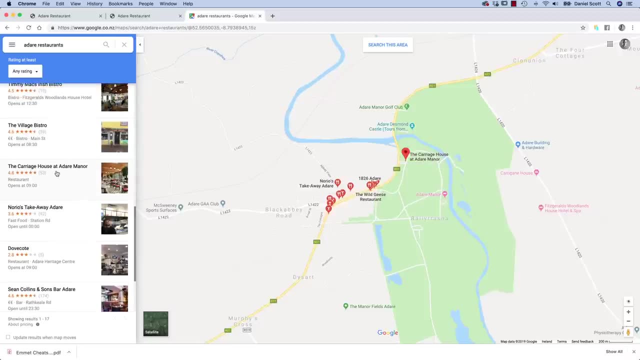 It's a deer. A deer manor is like some fancy big estate manor house thing. there, The carriage house at a deer manor seems like a really cool place to add to my fictional map. So what I'm going to do is I'm going to click on it. 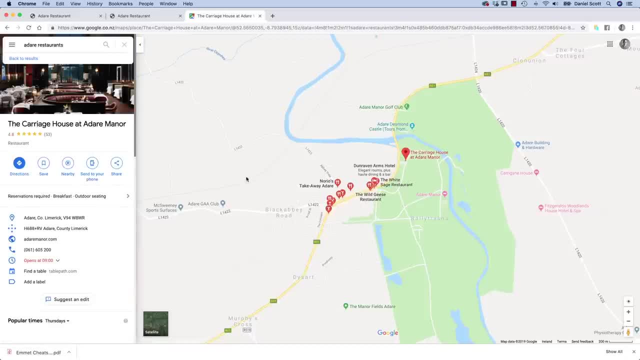 so that I'm just kind of like isolating it over here, because I don't want all of these things over here as well. So I'm just going to find the carriage house at a deer manor, Because whatever you see over here is going to be what's in your map. 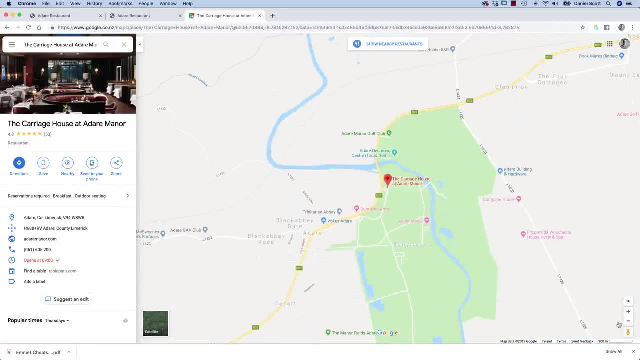 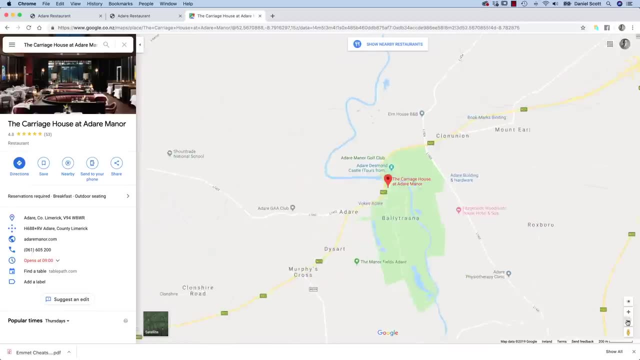 Still showing me the other restaurants. Go away the restaurants. Oh, it has gone away. So a couple of things you need to do when you're doing a map is zoom in and out, because this is the kind of size if you want to show it in relation to like Dublin. 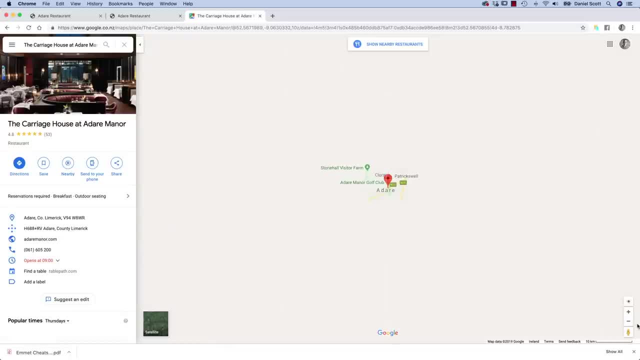 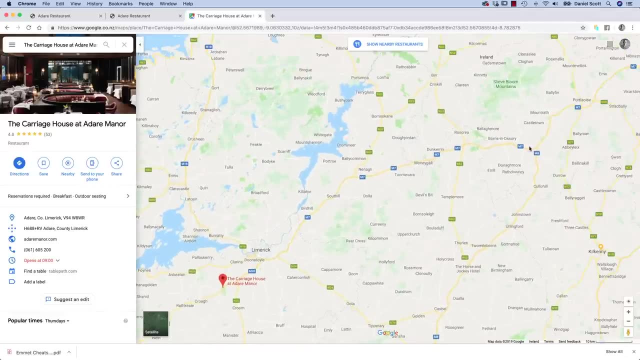 which is miles away. I live in Ireland, I'm from New Zealand, My wife's Irish, Anyway. so you're going to decide the kind of scale Do you want it to be? so you can see the kind of driving distance between Dublin. 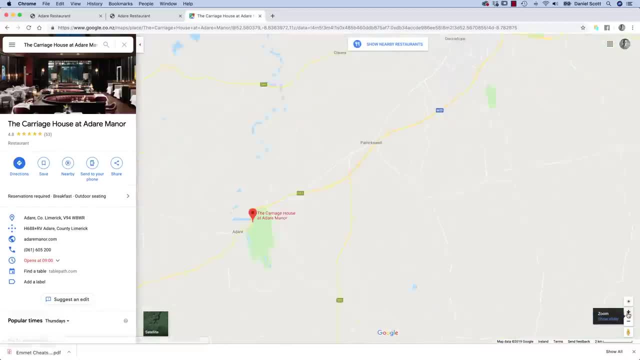 Dublin's up there somewhere, or do you want it to be really kind of localized map so people can see the street that's on very close? Get that right click and drag it in the right position and then what you're looking for. 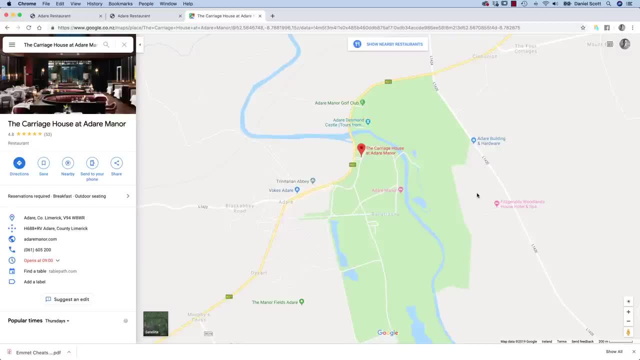 now I'm going to show you as it is at the moment. Every time I teach this class and I make a video, they go and move where this button is. So you're not allowed to complain. Google changes it on me. you just got to dig it out and find it. 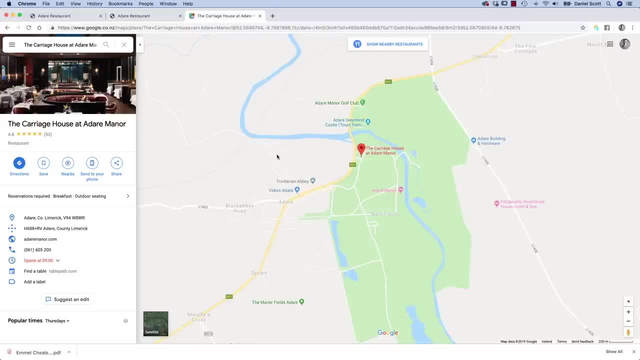 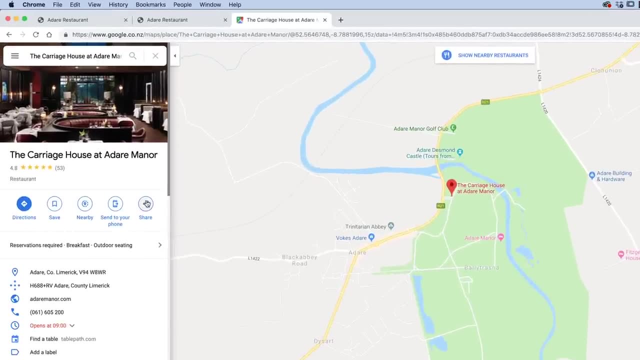 If it is in a different place, write it in the comments so that other students know where it's gone. So what I'm looking for is an embed code. So where is it? at the moment It's under this one called Share. give you options for sharing. 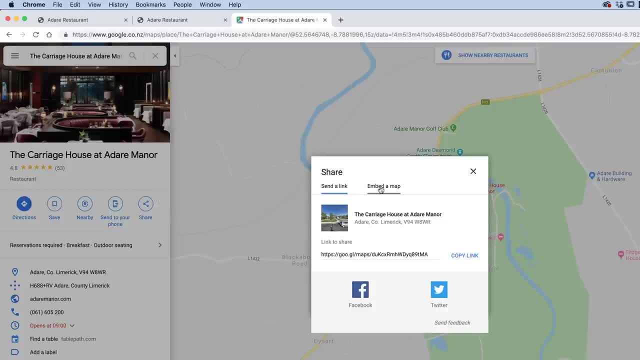 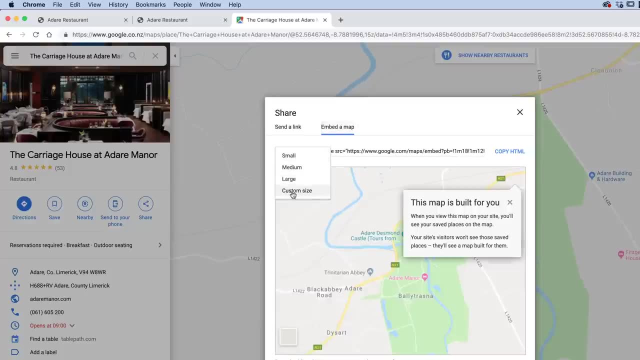 And you're looking for this one called Embed, So Embedded a Map. click on that, And then what I want to do is: you've got the different sizes. I'm going to pick a custom size. You could just pick one of these. click Custom Size. 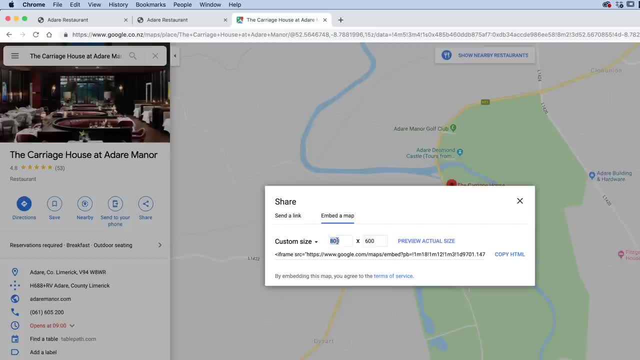 Now, how wide do we want it to be? I want it to be like. I know the width of my site is 1024.. so I might as well make it full width, 1024 even. And how high? I'm just guessing 500.. 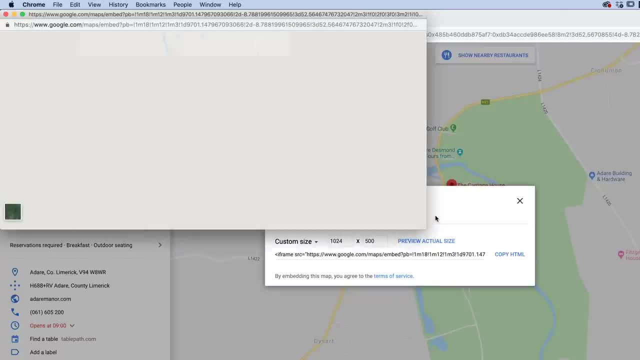 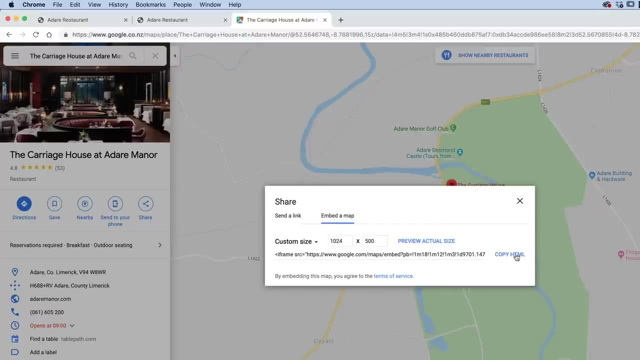 So let's preview it at actual size. So that's what it's going to look like once it loads eventually- Awesome. so all I need to do now is go to Copy Embed Map, copy HTML and paste this on my site. 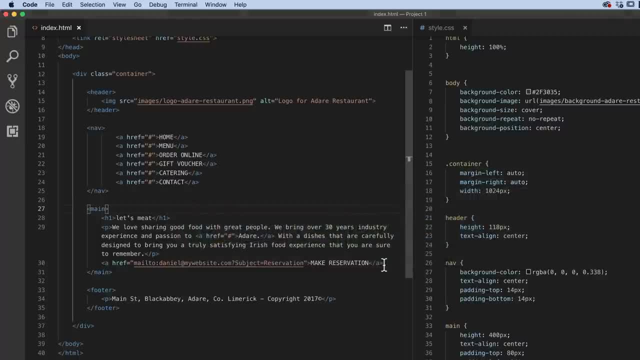 It's too easy, so good. The cool thing about it: it's going to make us look real good if this works. So where am I going to put it? I'll put it inside the main. So, just before it, I'm going to put a couple of returns in. 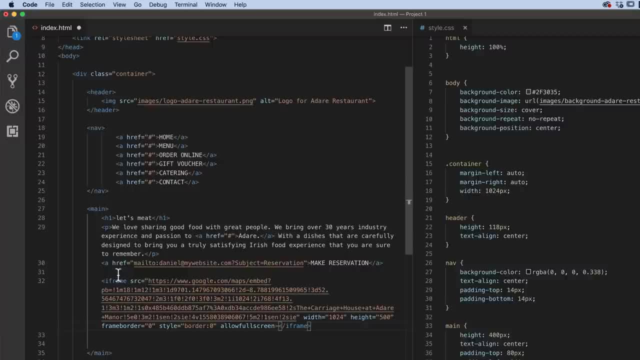 and I'm going to tab across and paste it there. So that's going to be my iframe. Let's see if it works straight without any. sometimes they need adjustments. let's check, I can't remember- And let's preview In the browser. let's see how this goes. 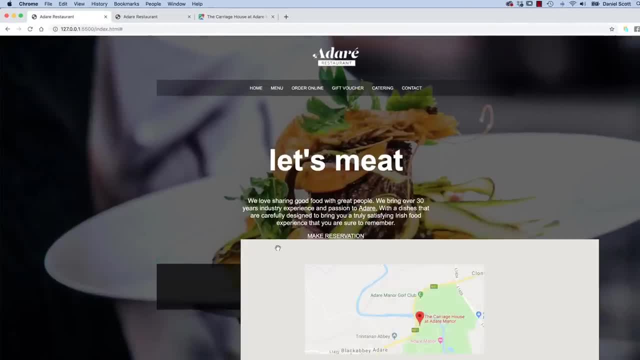 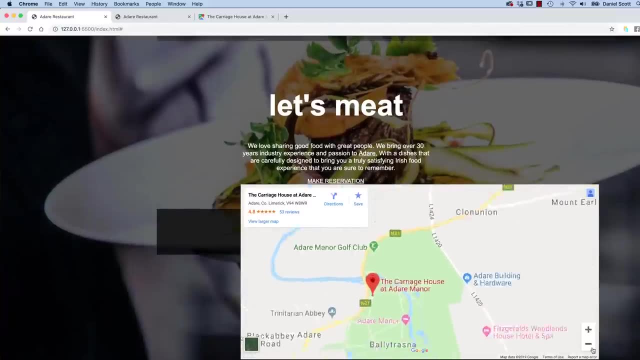 Are you ready? Which one is it? Yeah, it looks great. It's kind of pushed over to the side, but it's there. look at it. You can zoom in, zoom out, people can check it out, find directions and it looks good on your website. 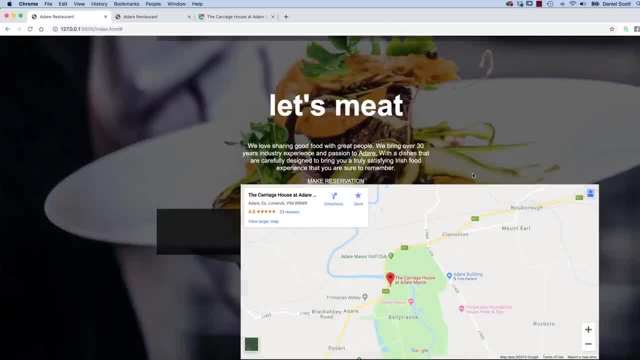 And we don't have to do any of this kind of like hardcore stuff. Google does all the hard work for us. Now, why is it all messed up? It's mainly because we put it. a couple of things. One is: we put it inside. 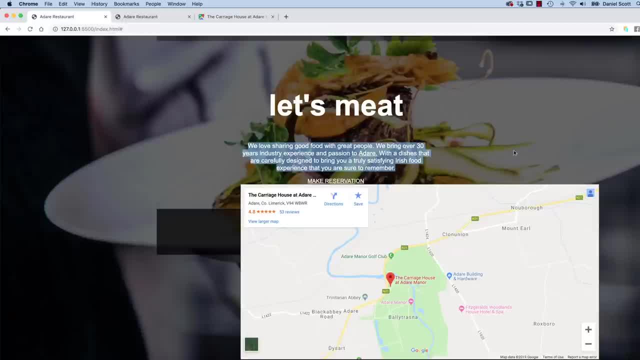 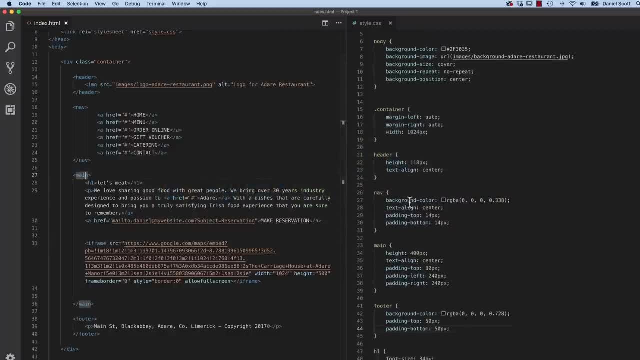 this main tag which I forgot we added padding to. I'll leave this in the course, because these are the things that happen. You're like what happened, Dan, I know because, remember our main we said earlier. later on we said we added giant padding. 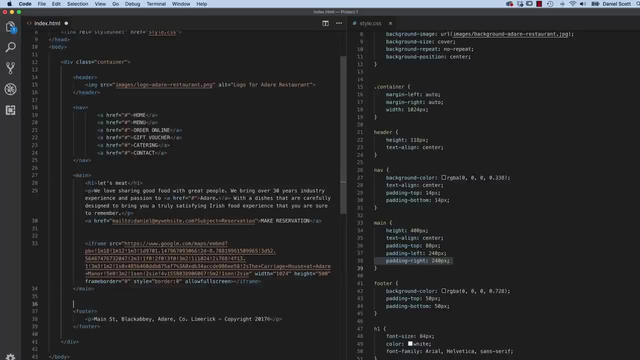 So what I'm going to do is I'm going to say let's not have it in main, let's have it afterwards in our tag. What tag? Let's use a section. We could- yeah, section Section is a nice thing to use. and what we'll do is: 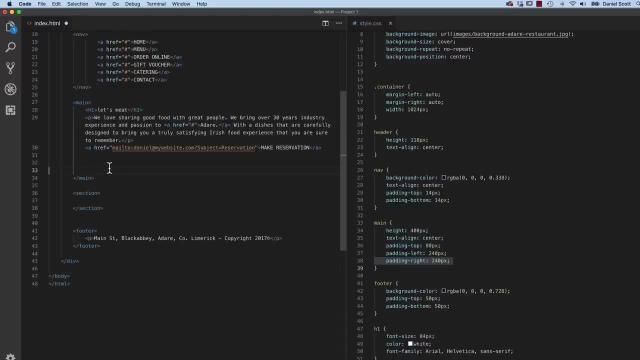 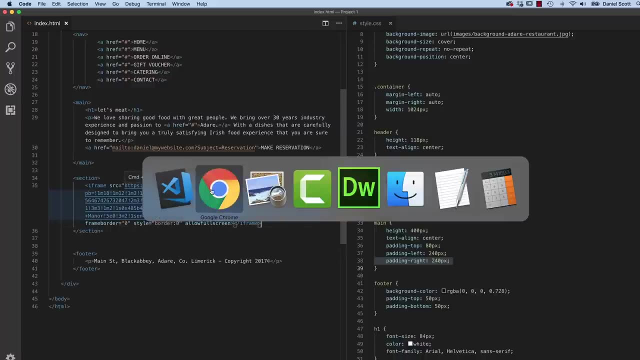 you could just use a div Just exploring using sections. I put it in there. It's going to say: solve some of our problems because it's in a different. the padding is not going to be affected. hopefully, Cool, and that's fixed all of our problems nice. 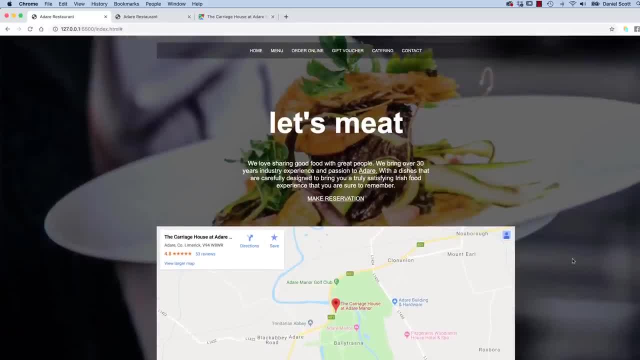 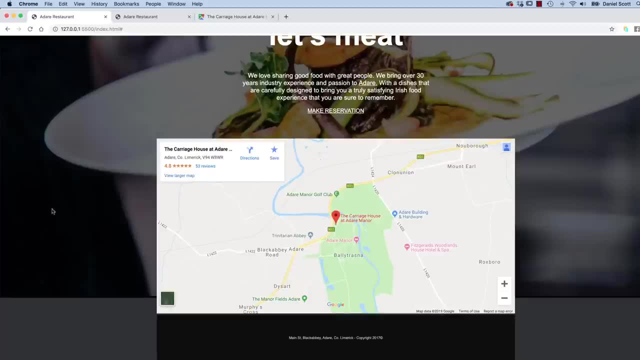 So there's our map. We've got some padding issues that we need to fix, But that's cool, just dump it in and it looks awesome. Let's fix the padding and then I'll show you a quick little run through some other embed codes. 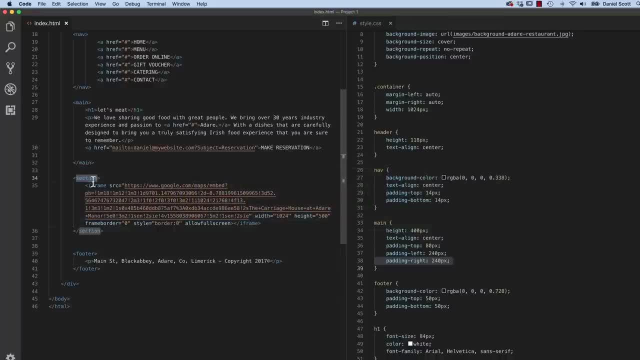 So what I'm going to do is I've got here my section and I'm going to give it a class name. I'm going to call this one, what am I going to call this one? Maps cool, And over here, what I want to do is I want to say: 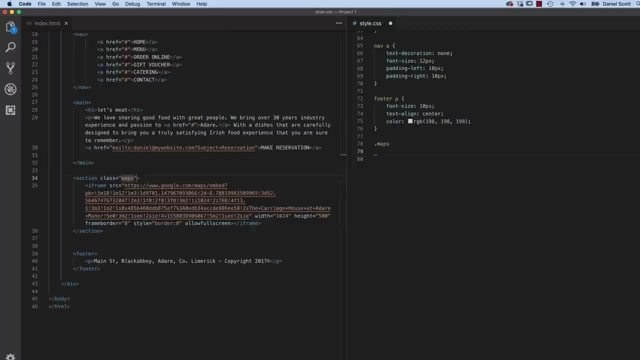 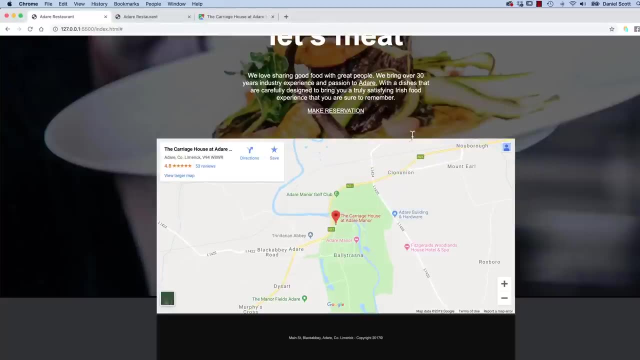 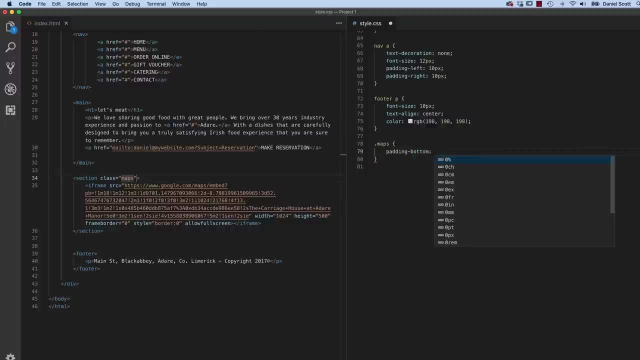 if there's maps, I'd like it to have some. what do I want? Padding or margin? so we'll look. padding or margin will work. Let's do padding. padding bottom Bottom and how many? Let's put in 100 pixels to see what it looks like. 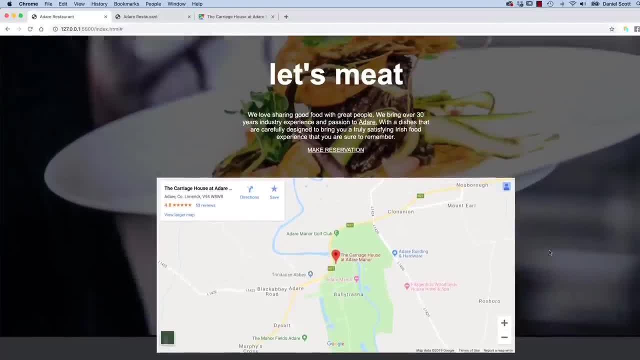 There we go. a bit of a space there My image is getting. it's not big enough to carry it. If you're working on a smaller screen, you're probably not going to run into many image issues, but there we go. 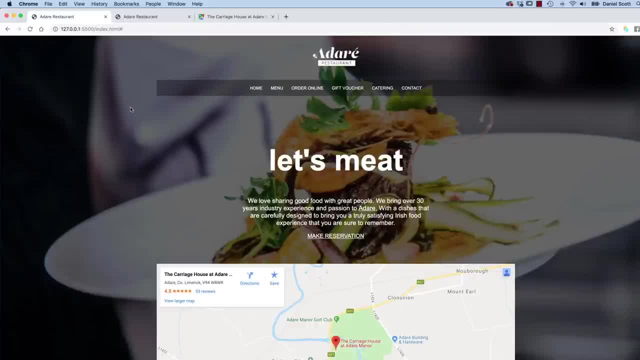 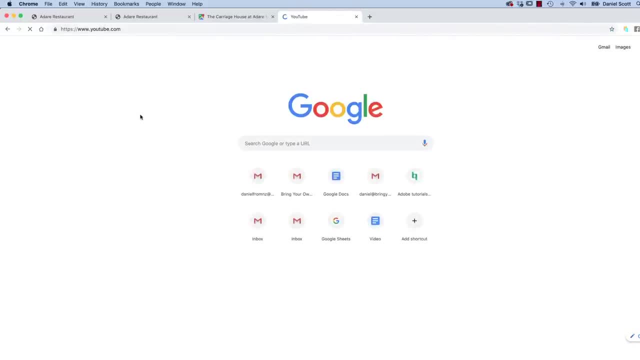 Let's look at a couple of other embed codes, because the process is the same. We'll do two more. a real common one is YouTube. So go to YouTube, find a video that you like. Oh, I know a good video. 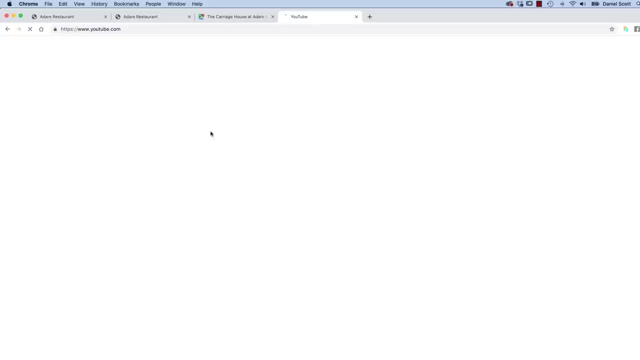 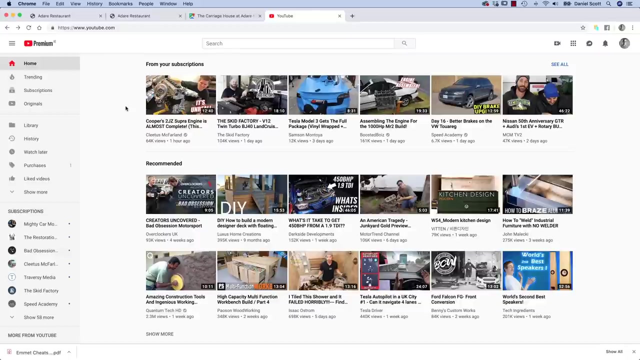 I'm dreading to actually use this to launch, So it's going to show you all my search history. What does Dan like to watch? All right, and it's not too bad. Lots of car shows and home renovation building stuff. 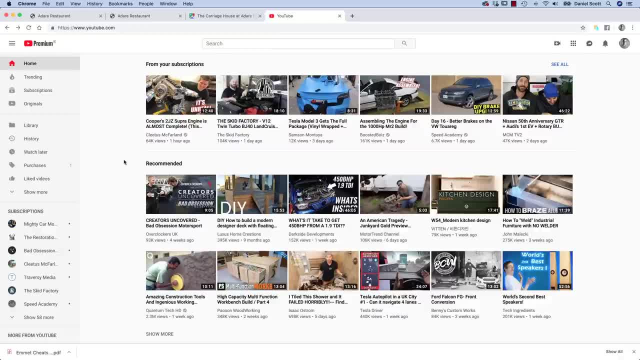 You're like: why aren't there lots of web design shows? Because I like to make web design videos, not watch them Anyway. so let's add a video. let's find: oh, bring our laptop, There's bound to be a good video there. 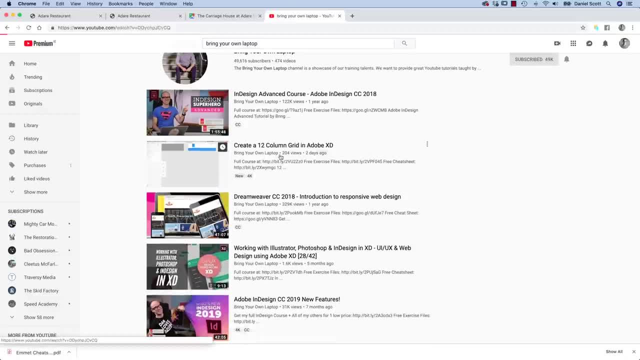 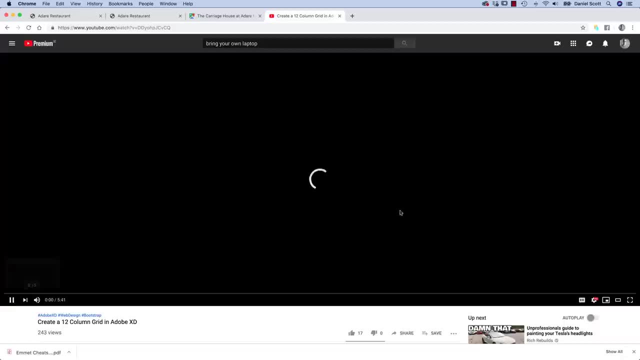 Oh, look at this guy grid in, let's grab this one. It's one of my old videos, my other videos. So what you're doing is you find the video that you want, make sure it's got a handsome Kiwi in it. 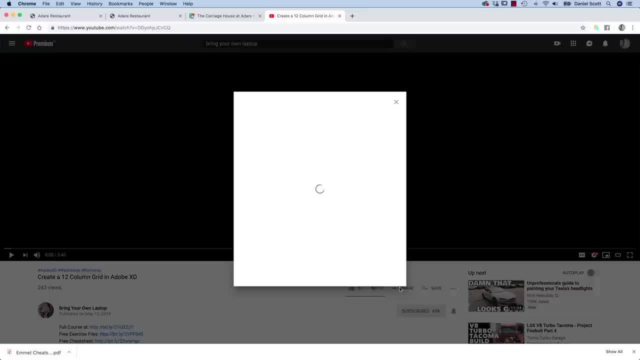 Once you've found that you're looking for the Share button, Now again, this might change. YouTube changes things around all the time as well. So you're looking for Share, it'll be there somewhere And go to where. do I want Share link Embed. 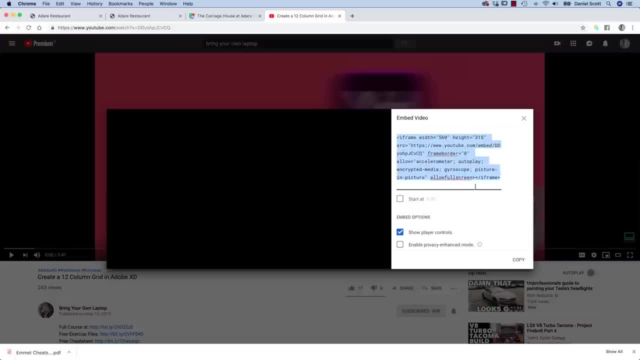 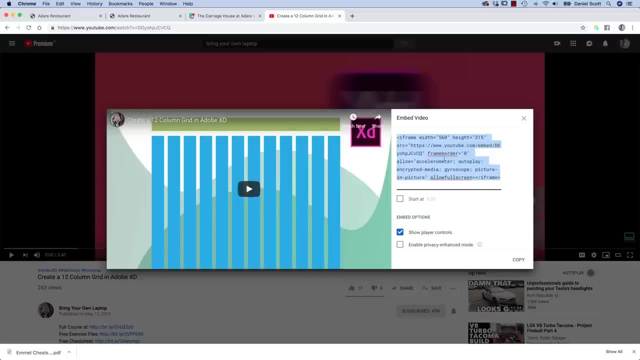 See that one there. click on this. There's our iframe, like before. You can get it to start at a different position. Do you want the Player controls? So, do you want the Play button or not? I'm just going to copy all of this. 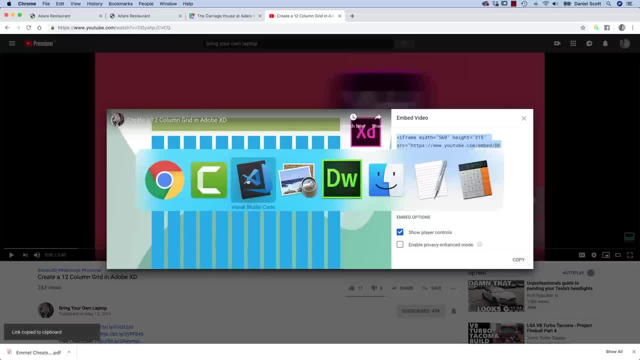 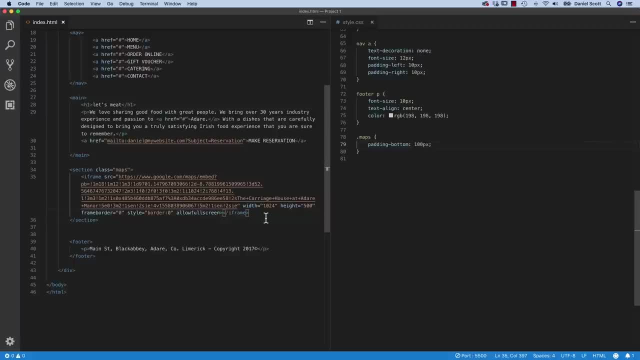 Let's just hit Copy. there you go. I'm going to jump into my Studio Code. Where am I going to put it? I'll put it just underneath this iframe. Yeah, just put it underneath there. I know we're going to get rid of it. 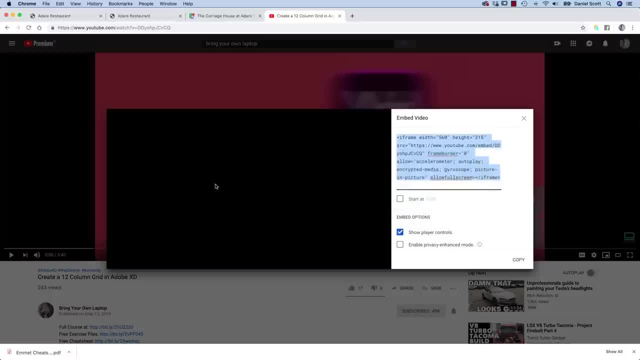 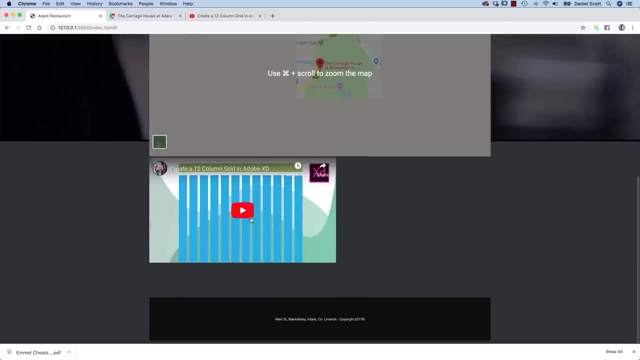 I'm just kind of showing you a for instance. Paste it in. let's see if there's any issues. Let's have a look. that's the old one, The new one. it looks like this: there's a map And there's a video underneath it. cool, huh. 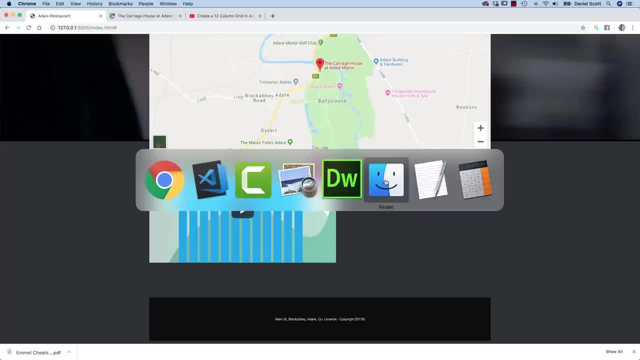 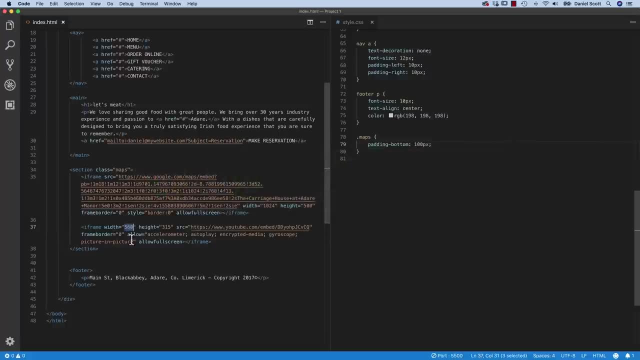 Now you can do things like making it 100% width. What else can you do? Let's have a little look at the code, Because we've said be height and width. I'm going to make it a width of 124.. 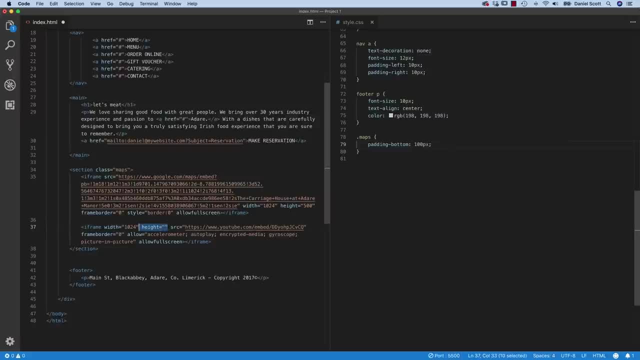 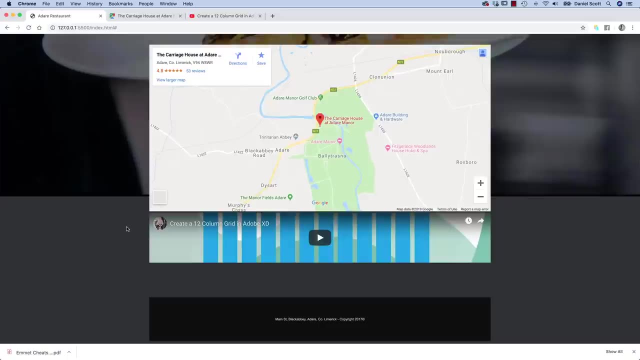 What does that equal? I'm not even sure. can I delete the height? You can just delete the height and let it do it for you. No, you have to work out what the ratio is and make it bigger. It's a really skinny video. 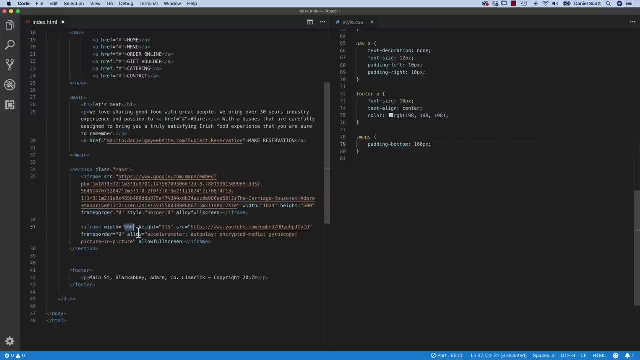 Not sure what it is, so I'm going to just leave it for the moment. It's a mess that my brain can't do. Now it's 10 o'clock at night, it's too late for maths And let's have a little look. 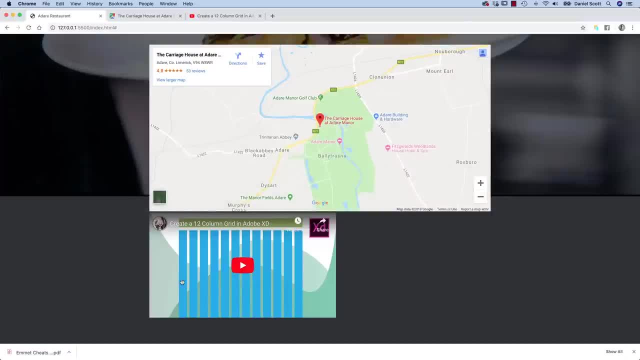 Yeah, adding videos. So I'm just going to mention a couple of other ones. now that you can go off and do, Twitter does the same thing. So if you want to add your Twitter feed to add a little bit of life to your website, 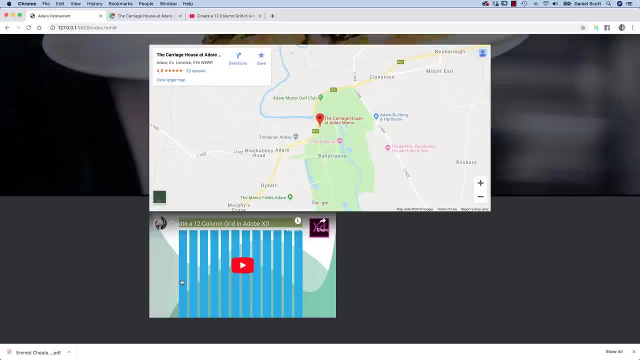 go to Twitter and they have an embed code So you can embed a stream of your tweets. You can go to Facebook and put your Facebook group on here as well, in different posts. What else can you do? MailChimp, have one. 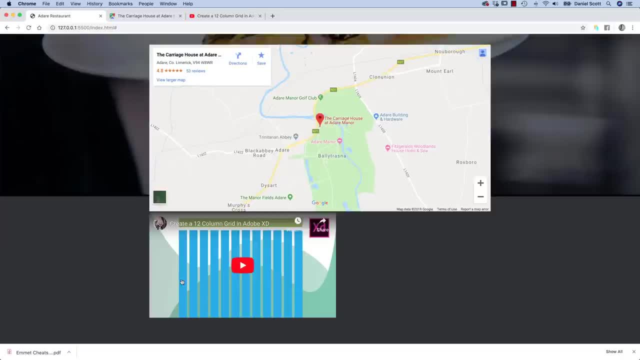 Say you want to add an email, sign up real quick and easy. Go to MailChimp, sign up and they will give you a little embed code that you can just paste on your site and they'll do all the heavy lifting. 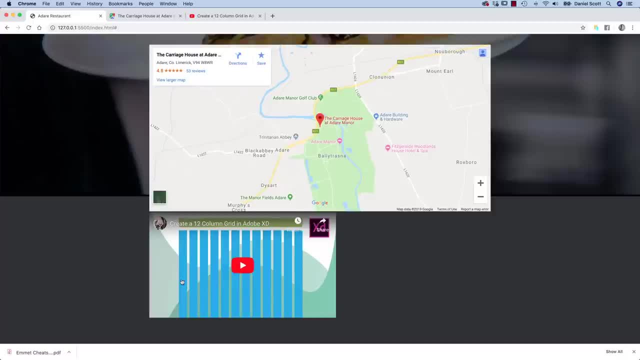 They'll grab the emails, they'll confirm them for you, they'll add them to a list so that you can send them emailers. One other one I wanted to show you was OpenTable. So OpenTable it's not really big here in Ireland. 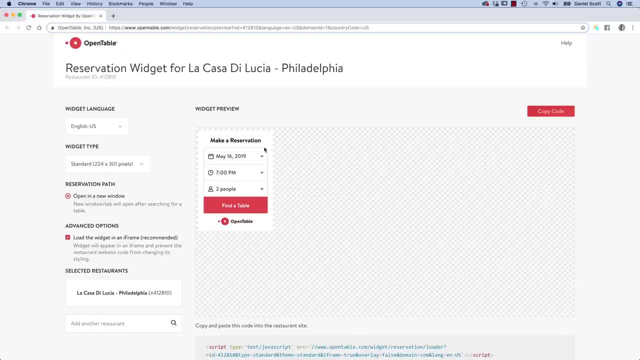 but I know it's big around the world. Anyway, let's say that you want to add a reservation, because at the moment we've just got this reasonably lame thing. Where is it There? we are there, we've got a button. 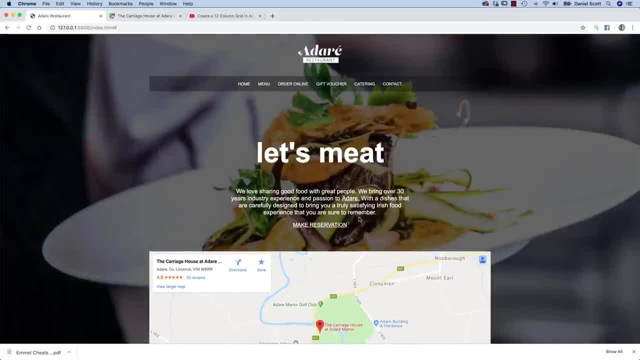 But let's say they actually want to book a time and a place and you don't want to have to code all that, because it can be. well, it's really complicated, it can be. You can go to OpenTable and, if you've been accepted into, 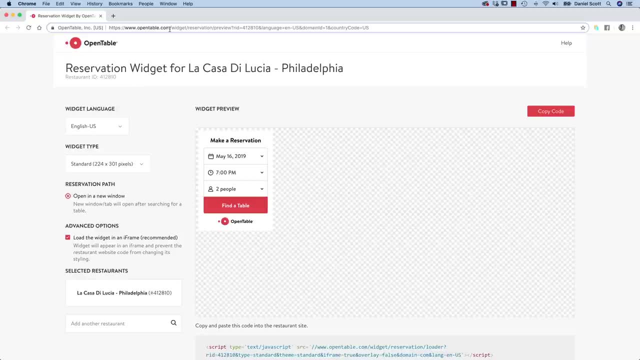 say you're the restaurant owner or the web designer for the restaurant, you're going to have to get them to make sure they add their restaurant and they have to jump through some hoops to say: yes, I'm a restaurant, it's an OpenTable. 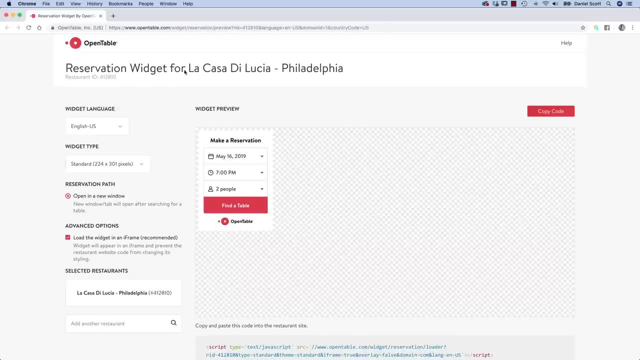 And what you can do then is they've got a widget creator. I found just a random restaurant in Philadelphia. I've never been there, But this restaurant, because it's on OpenTable, allows you to create a really quick and easy widget. 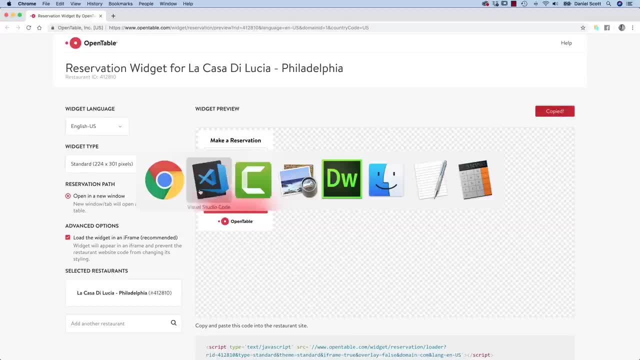 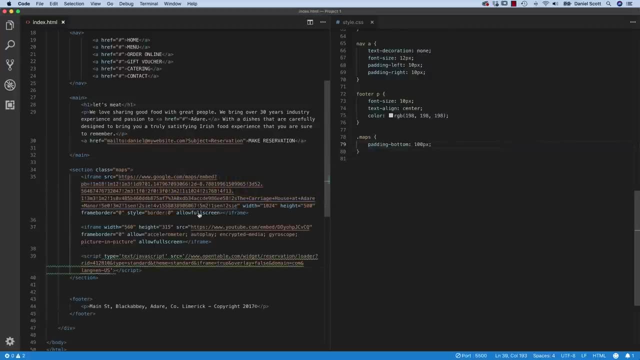 So you can pick the size. do all this, copy the code, dump it into your site and hope it doesn't break it. So where am I going to put mine? I'm going to put it just underneath here: paste: see what it does. 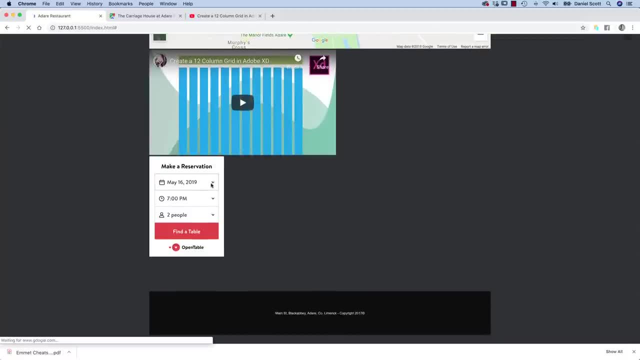 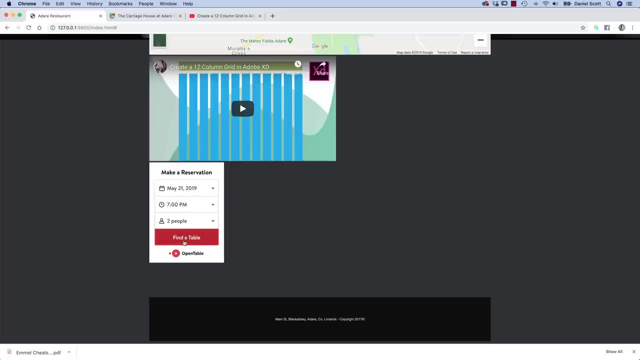 Let's have a look There. it is there, cool huh. So it goes through and somebody can go. I want to make a reservation for now and for two people at 7 PM and click find a table And it will send a booking request to OpenTable. 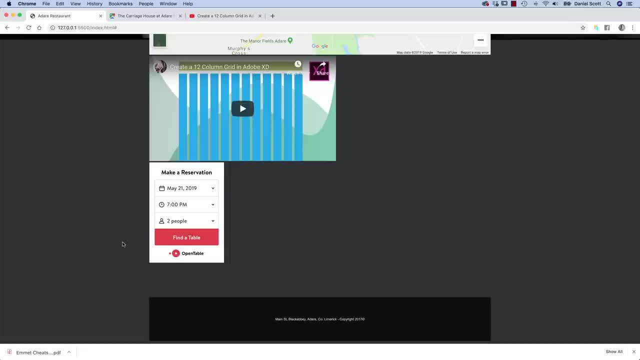 I guess I show you this all. I've said it a few times, but I want to show you this Embed Code stuff because not everything has to be done by you. You can stand on the shoulders of giants that have made cool little Embed Codes. 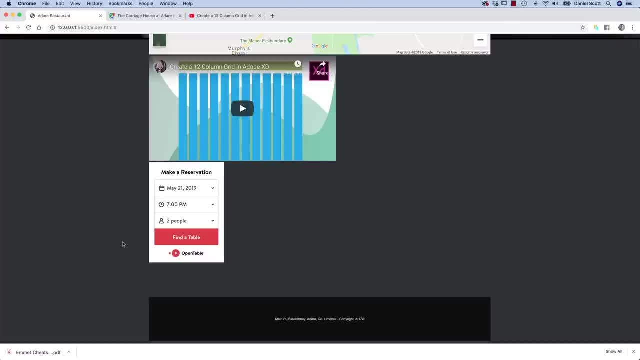 and you can just yank them out and stick them on here. Have we talked about other ones? A couple of other ones that I use is Eventbrite. I created my kind of sit down classroom business based around Eventbrite's Embed Codes. 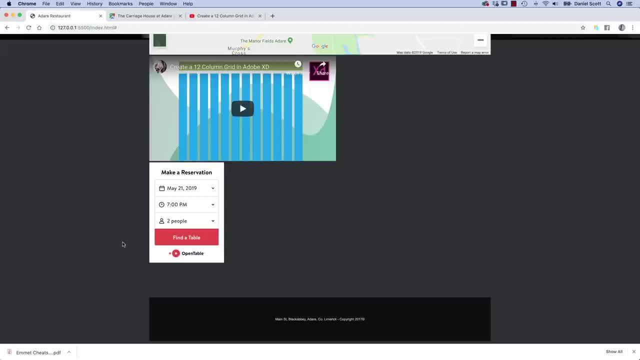 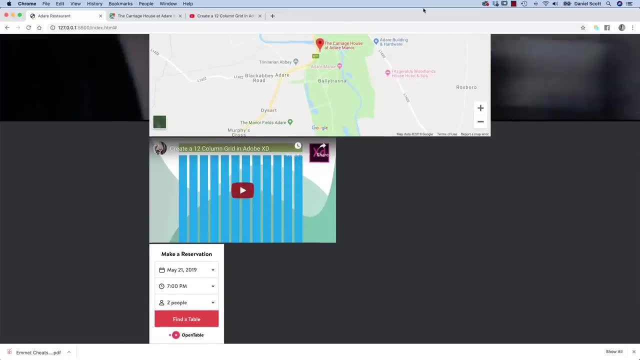 It allowed me to do some people to take tickets and book into my courses without me actually having to do much. All right, I'm going to go through now and delete it. I will save it for this video, but I'll delete it for the next one. 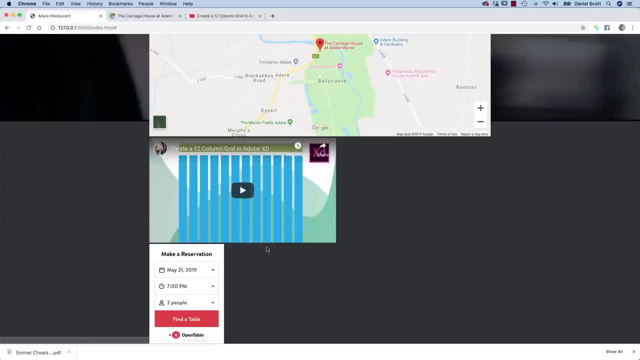 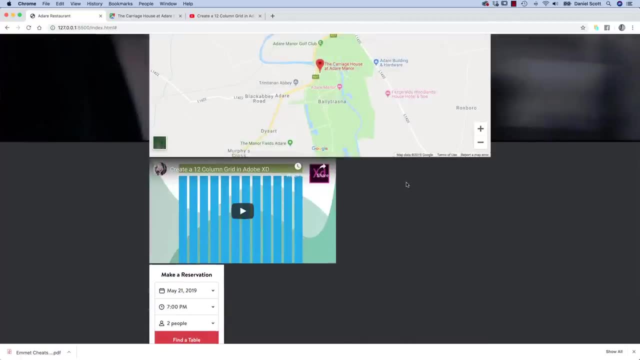 So when I wake up tomorrow and we start our next video, these guys are going to be gone because the map stays, but the rest of the stuff is just stuff we've thrown in for learning. All right, haere rā, good people, I'll see you in the next video. 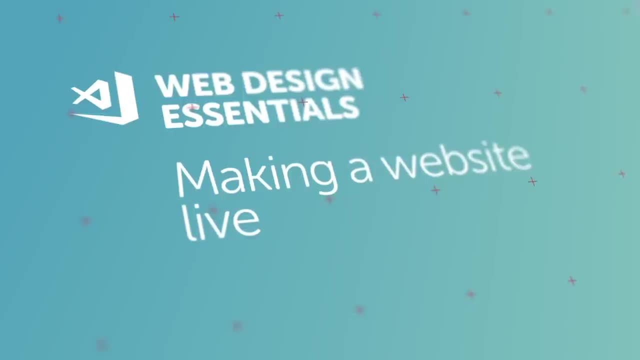 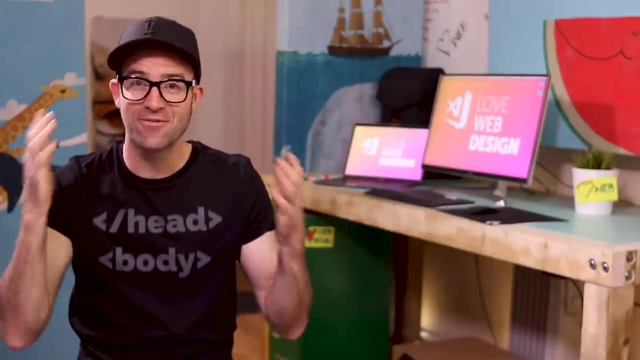 Hey, buddy, It's live me and you. I felt like this morning I'm going to start the day. we're going to do a live video so that, because I feel like we're being stuck behind the screen too long And today's a very exciting day. 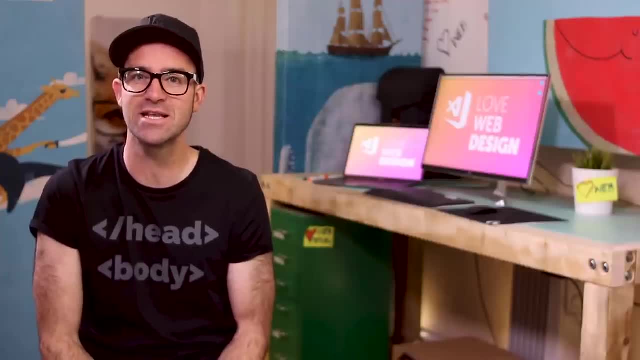 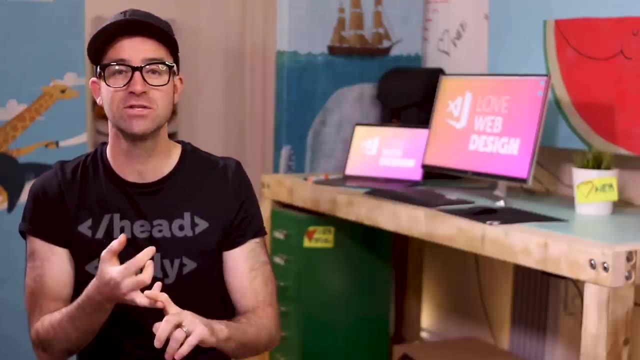 or at least this video is a very exciting video because we get to stick our internet, our website, online. So we're going to do two things: We're going to buy a domain name and get some hosting, and then we're going to stick it up and other people will be able to see it. 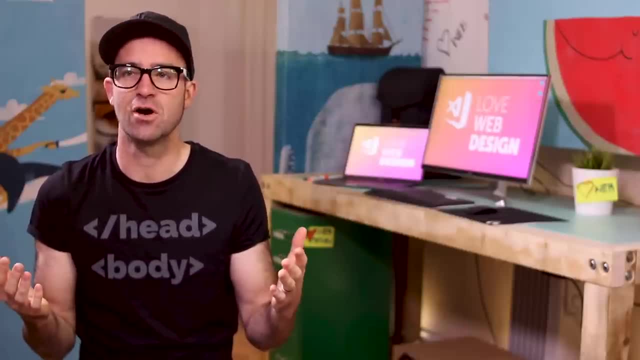 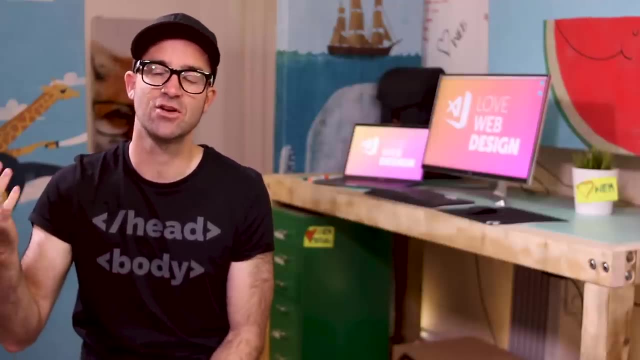 So the domain name is something like wwwadairrestaurantcom. We'll check to see if that one's available and we'll buy that. And then we need something called hosting and that's just a service where they're going to say: we will look after your website for you. 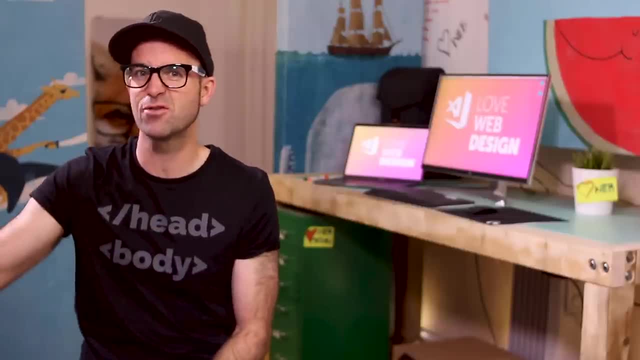 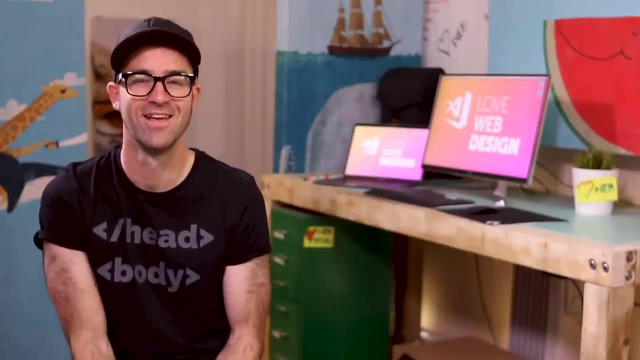 your images and your HTML and your CSS and we'll look after it and we'll make sure it's available to everybody. That's the hosting part And the name, the domain name. it's just the name. All right, exciting times. 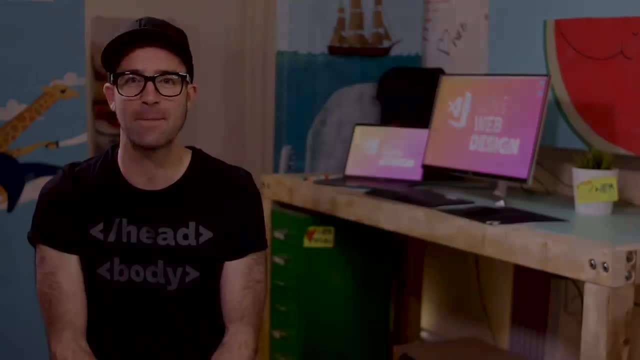 Let's jump in behind the computer again and see if we can get it all set up. All right. before we get started, though, I want to show you what we do at the end. This is it, it's our site, and you're like. 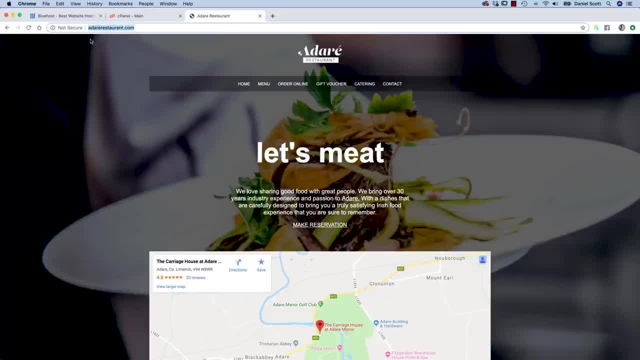 I've seen that before. we've done it. But look, it's now at wwwadairrestaurantcom. It's actually live on the Internet. people can see it. people start making reservations and checking us on our map. All right, that's what we're going to do. 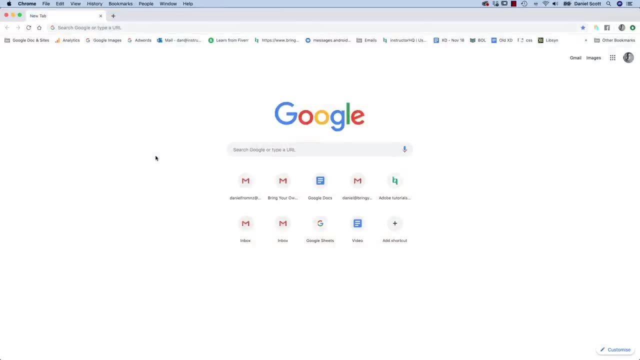 Let's jump in now, All right. so let's get this started. There's going to be two parts. We need to sign up for our domain name and our hosting- We kind of do that together- And then we need to work out a way of connecting our kind of VS Code. 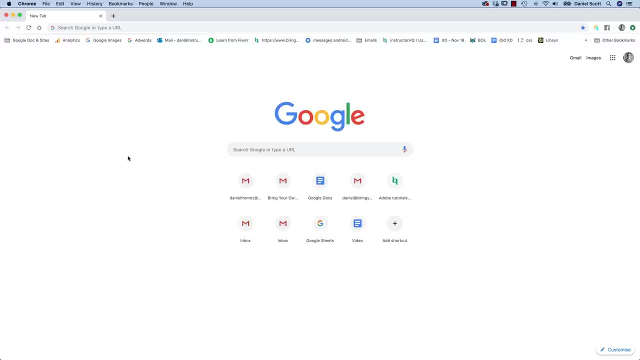 with that hosting to upload it. So where are we going to buy our domain name and hosting? It's up to you. There are lots of sites that do it. My recommendation is a place called Bluehost, and that's what we'll do in this video. 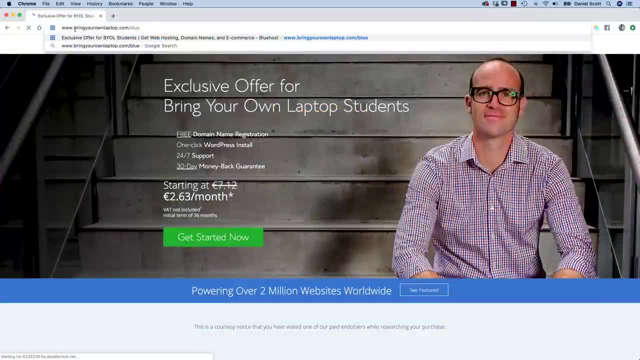 But there are lots of other alternatives. And why do I choose Bluehost? If you want to go to Bluehost, go to bringyourownlaptopcom, slash blue and it will redirect you there. I like Bluehost because it's the one I use. 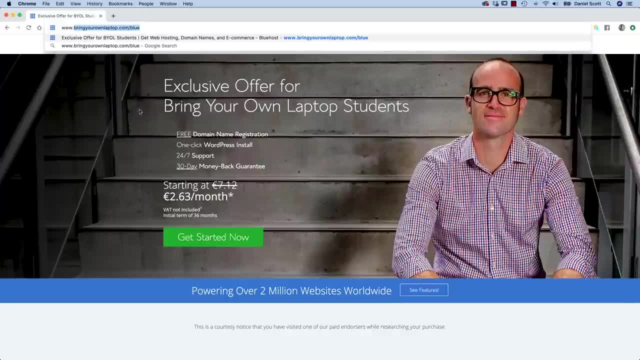 I also like it because of two reasons. we both win. I've got an affiliate deal with them where I get a small cut of your sign up. So when you sign up I get a little bit. You can go around me if you don't want to. 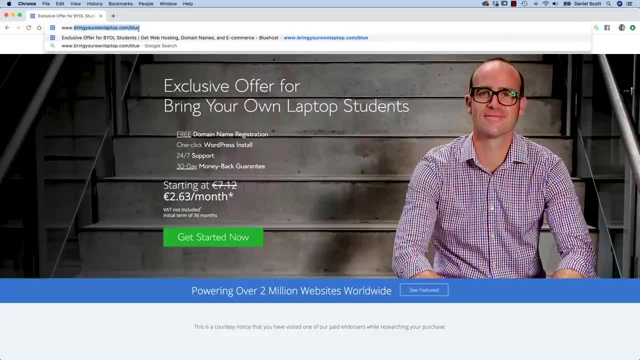 You can go to Bluehostcom, that's okay. But if you use bringyourownlaptopcom, slash blue, two things happen: I get a little bit extra and you get a big discount on your sign up. So if you use this, 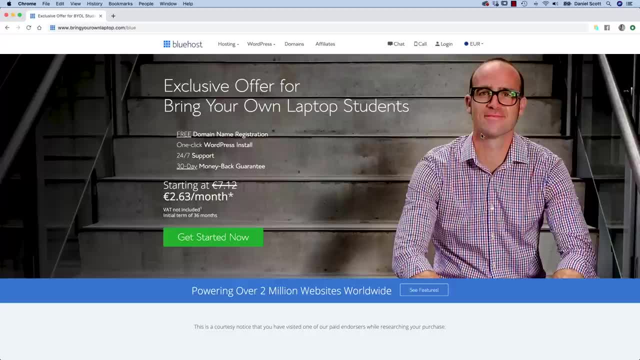 look, it's Bluehost and it's got my face on there. We do some stuff together with Bluehost, so it's a nice little. they made a little website for me, which I can't believe. The cool thing about it is you get your domain name free as part of it. 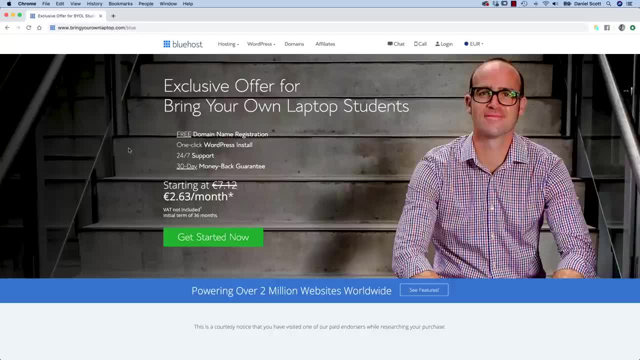 and it has all the things we're going to need for this and kind of future classes that I have planned where we're going to do WordPress. We're not doing it right now. So if you do, if you are looking for other alternatives for hosting, 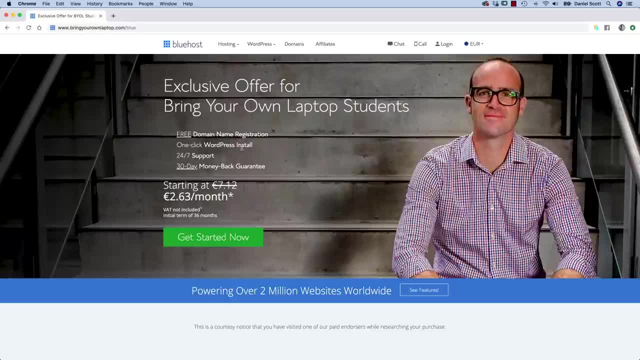 there's a couple of things you just need to watch out for. Not watch out for, just make sure it's included. You need a domain and hosting. those are the basics. After that, it would be really cool if they had really simple WordPress installation. 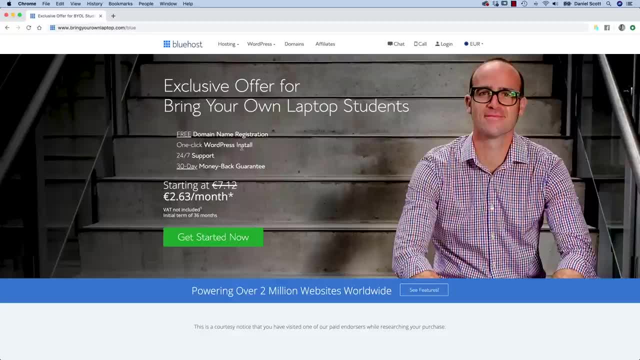 You don't have to for this entire course because we're not doing it, but if you plan on following along to later courses, it'll be super handy. The other little things to look out for is something called an SSL Certificate. Make sure they have that. 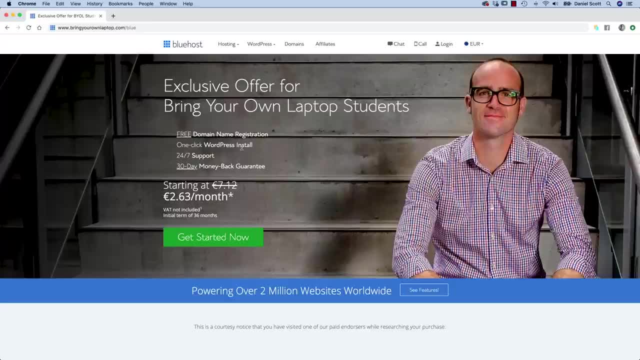 Most of them have it now and it should be free as part of your hosting. This Bluehost one does. Other nerdy stuff is to make sure that it's an Apache server and that you can run PHP on it, because later on in this particular course, 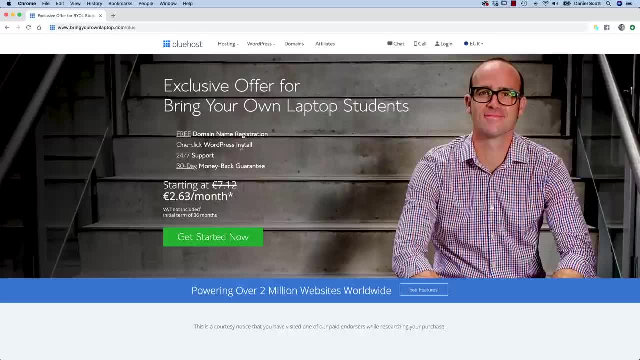 we're going to run some basic PHP to do some cool form validation stuff. If that went all over your head and you're like: what is he talking about, Just use Bluehost and follow me. All right, let's get started. let's click Get Started. 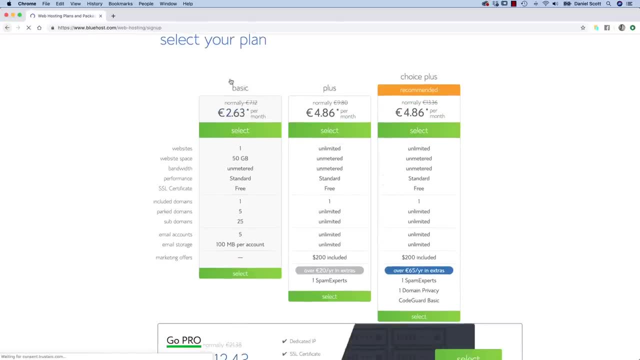 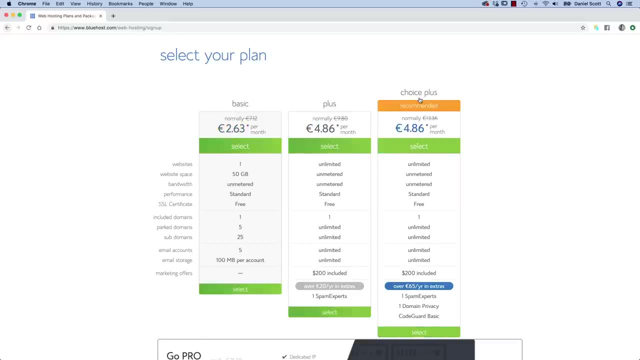 now, all right, we get to choose our plan. Now there's always three. why is there always three For you for this class? all we need is the basic plan. You can do the plus or the choice plus. 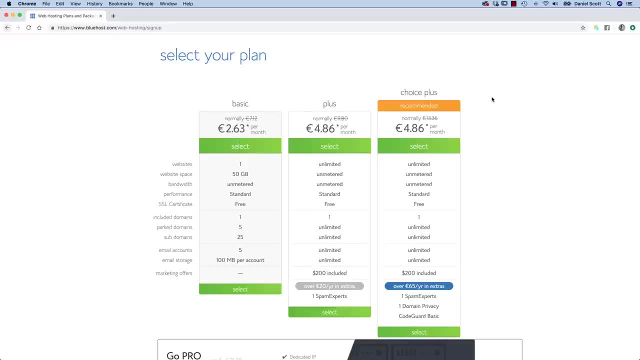 It's not that much more expensive. But the reason you would is if I'm just designing one website- say, I am the owner of Adair Restaurant and I do not need to have 10 other websites. I'll just use basic. 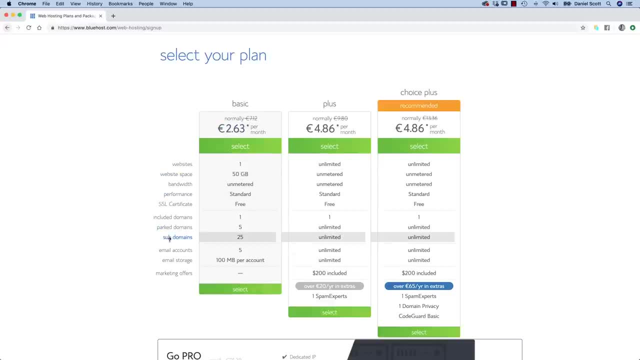 because that's the big thing. that's different down here. Parked domains, subdomains, just means this one. here I can be more of a web designer and go all right. I've got 10 clients and they're all using the same host. 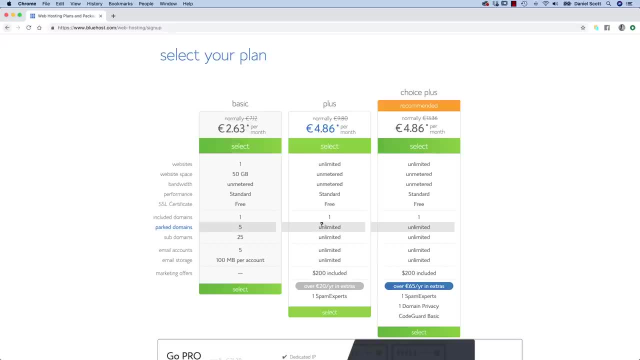 I have to buy 10 domain names, so adairrestaurantscom, and then I'm doing something for Dan's Dentist, and then Dan's Web Design and then Dan's Auto Mechanics. So I'm doing lots of sites for people. 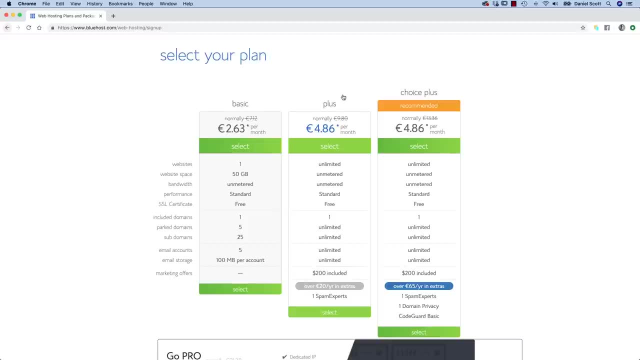 That's where you might decide to use this plus or choice plus, so that you get to do lots of websites using the same monthly cost, rather than imagine I bought one and then I had to buy a second one. I'm already at $5.. 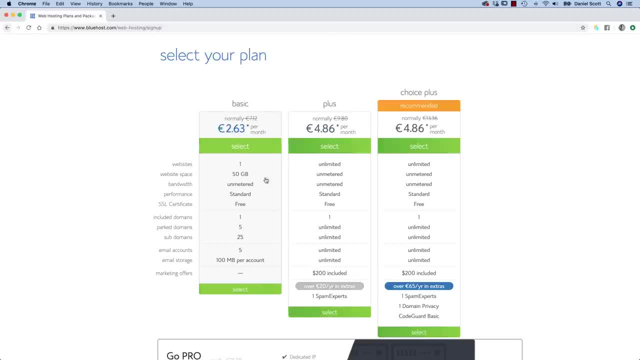 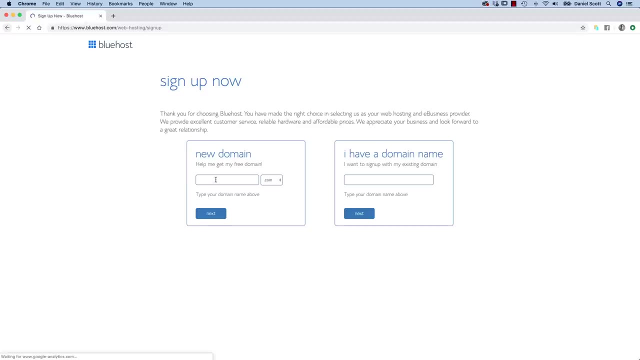 $5 a month, so I might as well go for something like this. You can switch later on, so for the moment, we're going to use Select Now. we're going to pick a new domain name Now. at this stage, you've got two options, three options actually. 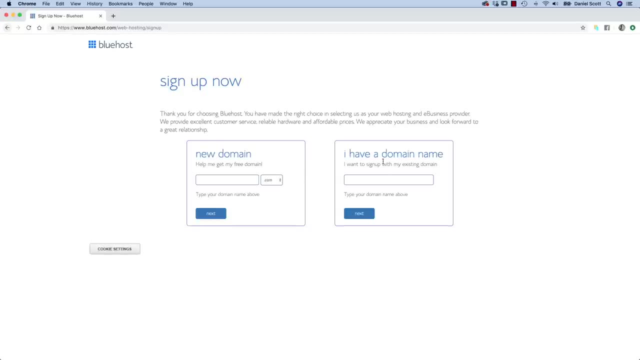 New domain name where you go to pick your com or whatever one you want, and if you already have a domain name, type it in here and Bluehost will help you. basically, they're two separate things. The domain name gets pointed towards the hosting. 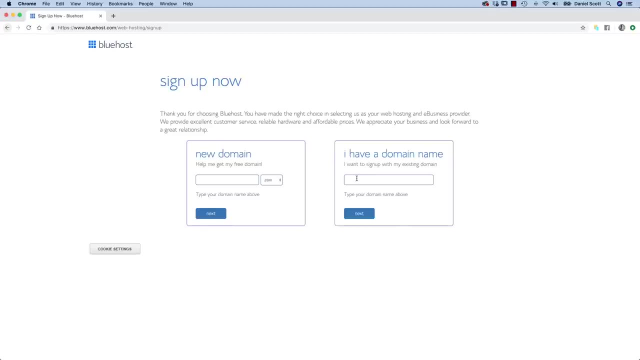 and if you already have a domain name, type it in here and Bluehost will help you point it to the hosting that we're about to sign up for. If you don't have one, put it in here. If you try and leave, where is it? 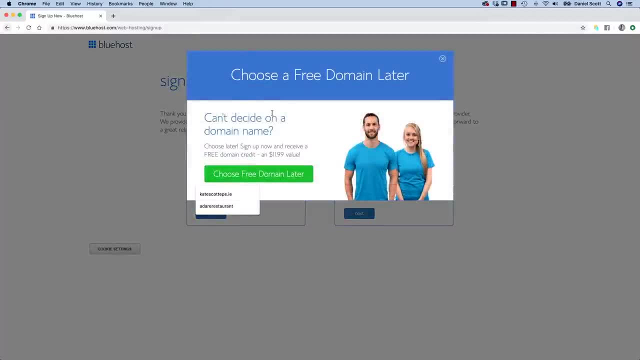 Because sometimes you're like, actually I'm not too sure, there you go If you kind of. I don't even know how to activate this, but it seems when you try and leave this it says hey, can't decide on a domain name. 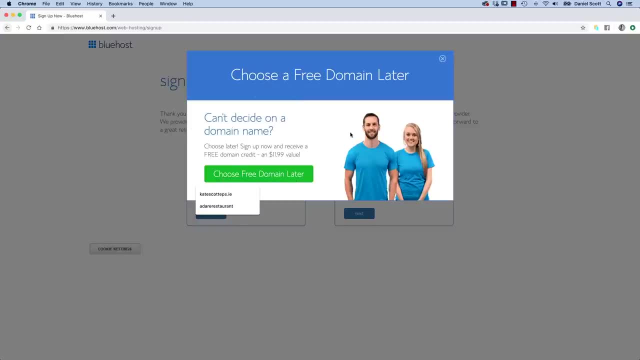 You can do it later. you just get a credit and you can edit later. So if you've spent like already an hour trying to figure out a domain name, come back later and do it. How to activate that little pop-up? No idea. just wiggle your mouse around. 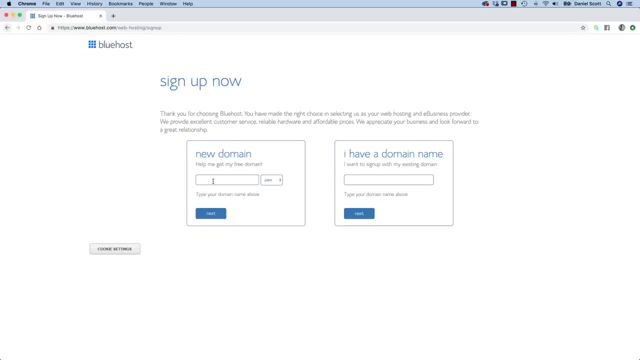 I think if you go towards this, crossing it out, it seems to launch it. Now we're going to check. if Adair Restaurant is available, Let's click Next. I think Adair, it's a weird word anyway. So nobody has it. it's available, which is awesome. 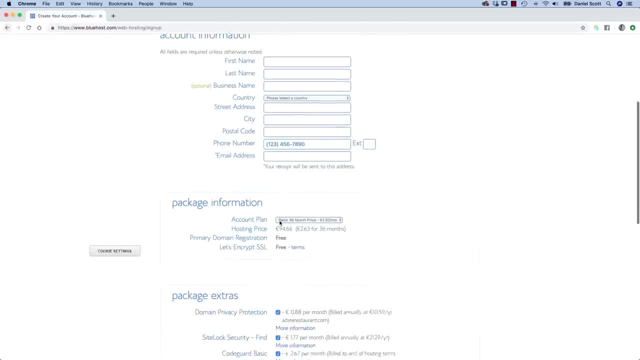 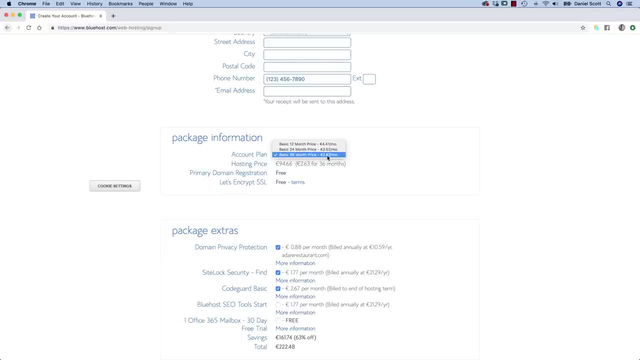 So next thing to do is obviously you know what to do there- Package details. so the price we got I think it's $2.95 for US- It's a little bit less than Euros, but that is based on 36 months, so 3 years. 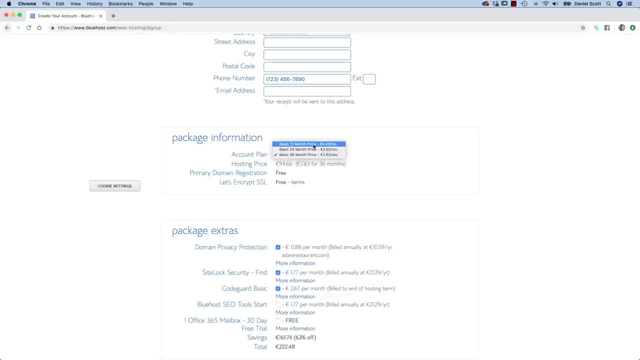 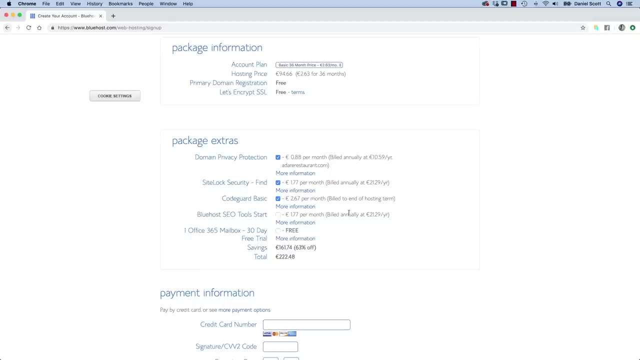 You might be like, wow, big commitment, You can go down to 12, it just costs you more per month. it's up to you. The other thing to think about is these. Now, this is up to you. have a little read through. 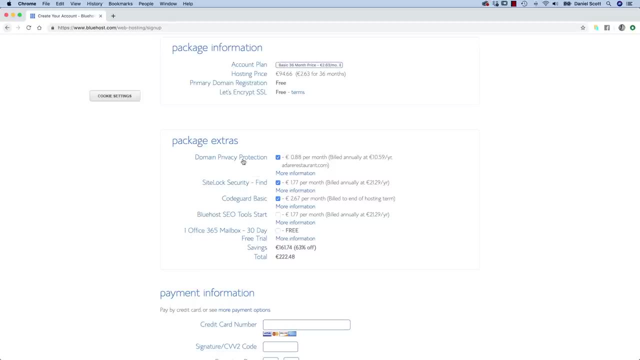 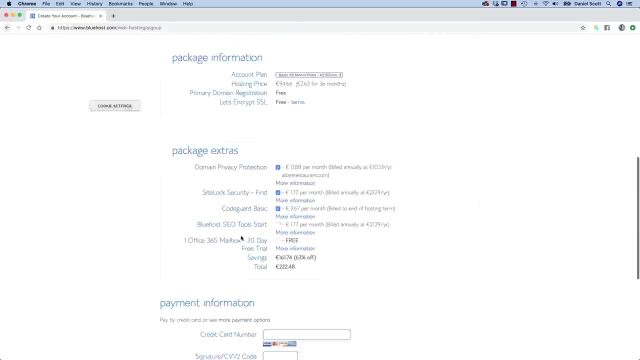 The main one that I'll kind of talk about is the Domain Privacy Protection. So when you fill out the details for a domain name like this stuff, it's actually public domain knowledge, So people can go in and find out who owns the domain name and find out the address. 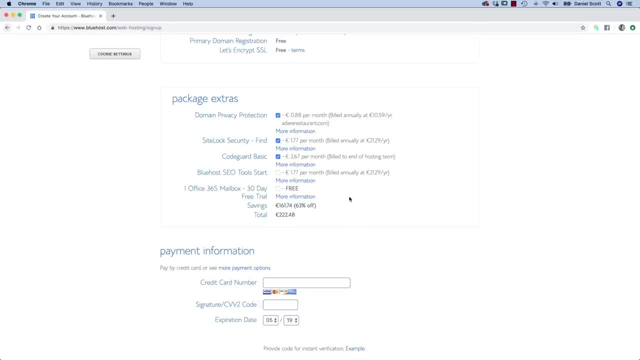 So what people do- not me- is some people just put in a fake address. Never heard of that before. But another way is to do this: Domain Privacy Protection. I have no idea how they do a monthly cost that blocks it from people, but it does. 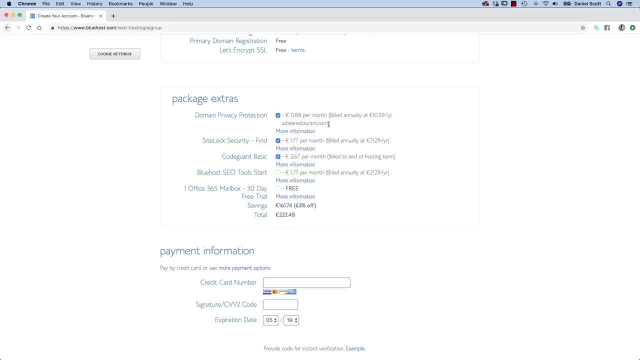 You've got to then kind of reach out to Bluehost to get the information. It's just not easily available. Have a little read of this. I don't use any of these. They're just optional extras. have a read through them. 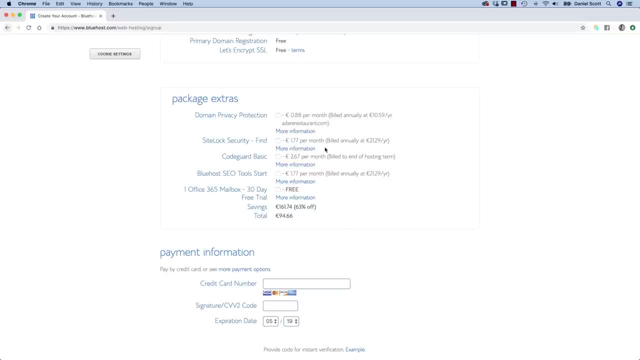 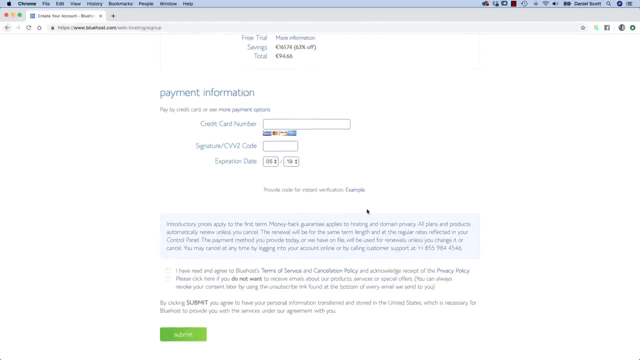 I get a little bit blasé about some of these things, So have a little read through yourself and decide whether they're right for you And what else. I don't need the email hosting Credit card details. sign your life away. 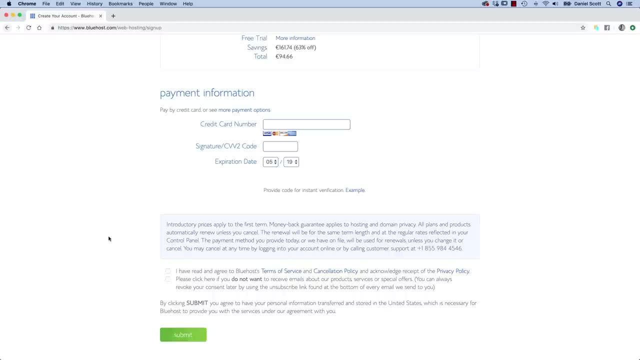 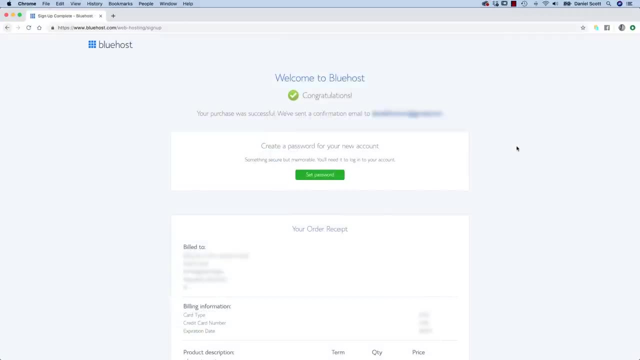 Fill in all that details and I will see you in a second, after you've kind of gone past this page, we'll do the rest. All right, this is the page you end up at, Remember, if you're watching this. in the future, everything might be slightly different. 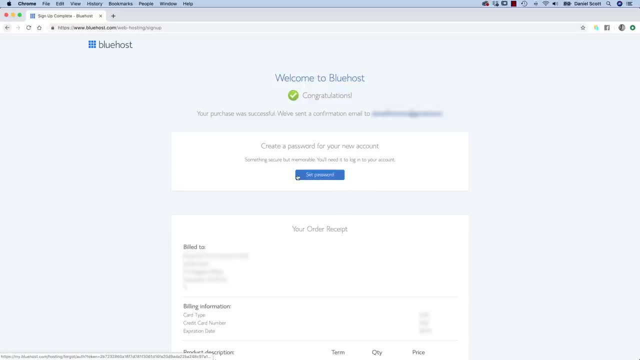 But we should end up in a similar sort of place. so we're going to set our password for the account. I'll do that without you looking. You look away, I promise, and I'll see you in a second Password, complete. let's go to login. 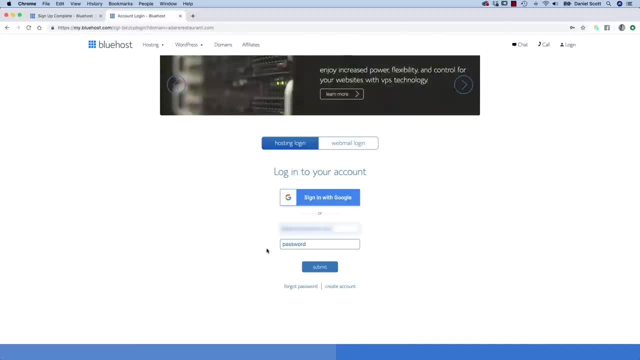 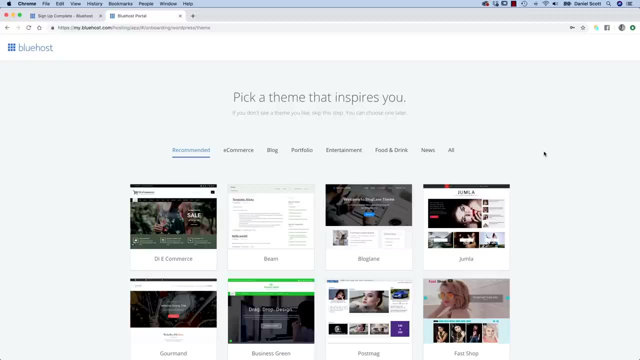 I'm going to go to my hosting login and I'm going to sign in. I'll see you in a sec. All right, it's trying to get us to install WordPress, which is just a different way of building a website. You're not actually. well, you're building it, yes. 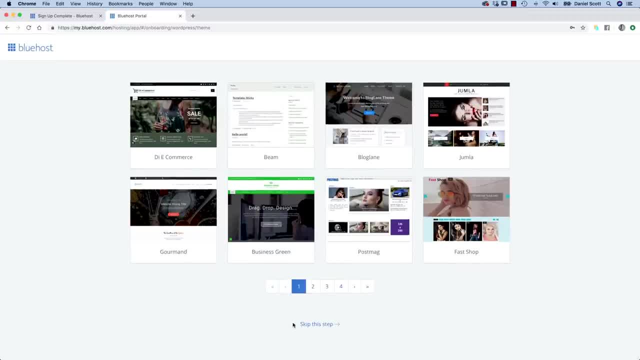 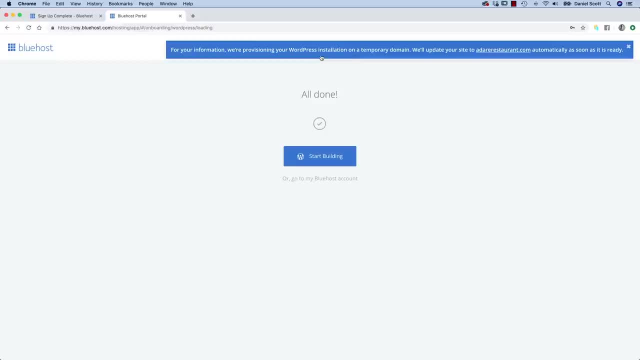 but using kind of templates. So what we're going to do is skip this step down the bottom. Yours might be a little different. They change this onboarding all the time. They're telling us here they're going to kind of put. 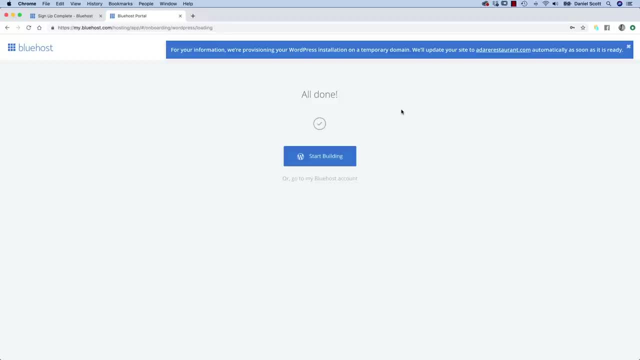 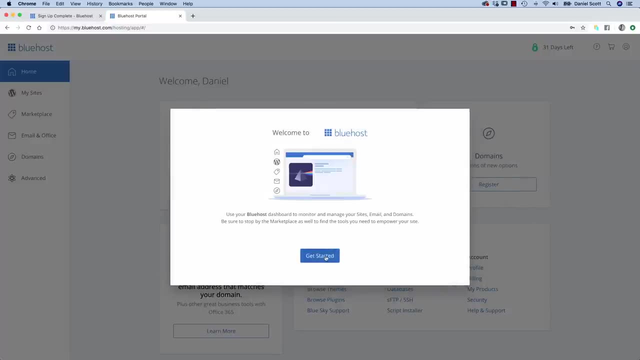 the WordPress installation on a kind of temporary domain. We're not going to use it, so let's skip Start Building, because it's Start Building. a WordPress website was going to go to our hosting account, All right, and this is your kind of like dashboard. 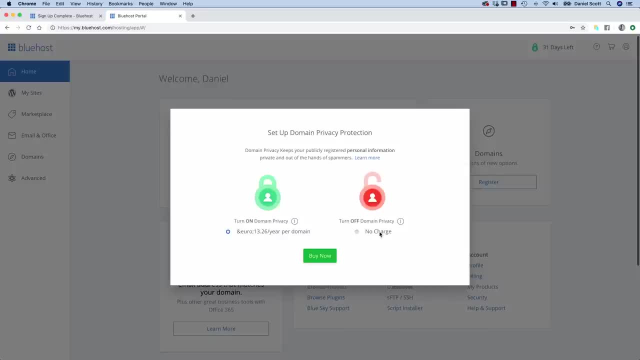 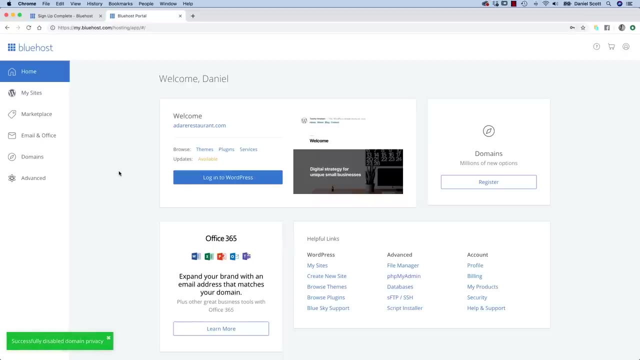 Getting started. there's lots of. I do not want to buy now. no, thank you, I'm sure I don't want it. thank you very much. All right, so what I want to do now is upload my site. Next thing we want to do is: 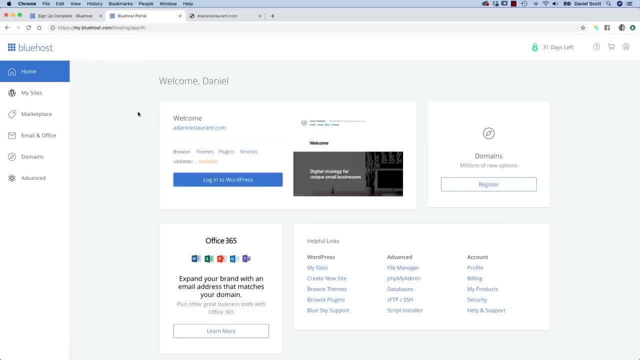 I'm going to show you two ways of uploading your website to your new domain. We'll use the Caveman way, which is super simple and can't be broken, And then there's the way of automatically doing it straight from VS Code, which is helpful. 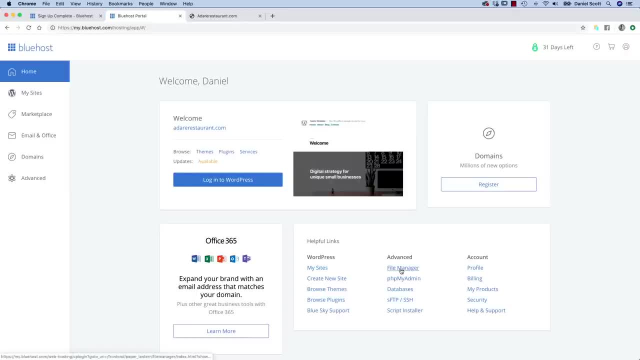 but a little bit harder to set up. So we're looking for the File Manager. It might not be here when you go to here, they might move this around a little bit, but you're looking for the File Manager somewhere. File Manager is going to load up. 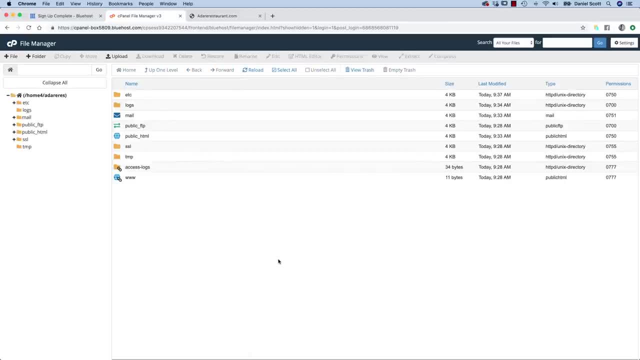 And this big thing opens up And this is looking at. remember before we had something called the local site, So let me show you All right. so on our desktop we created this local folder called Project1.. and inside of that is our website. 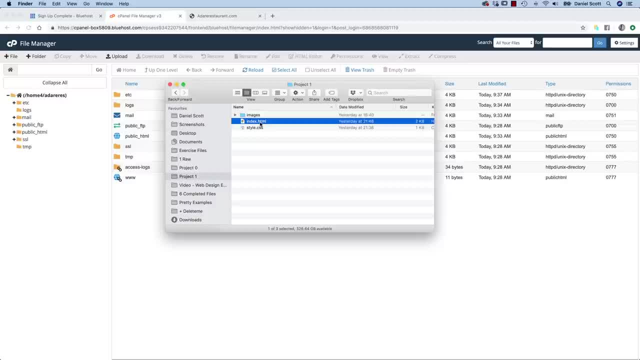 And the only problem is we've got an index page and we can see it, but the rest of the world can't. And all hosting is is that there's a company like Bluehost that says we'll take these files and we'll share them with the world. 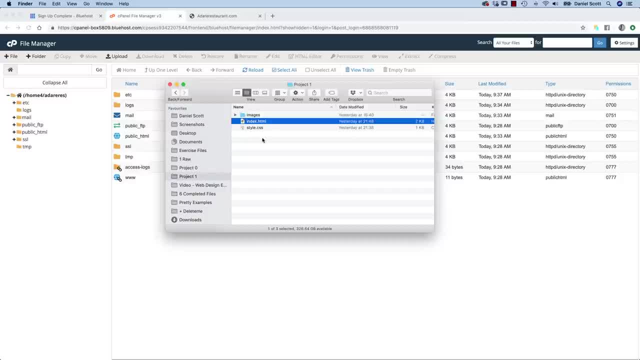 and we'll make sure it's live and connected to your domain name. So when people go to adairrestaurantcom they're going to be shown this index And they promise to always have 100% uptime so that everyone can see it all the time. 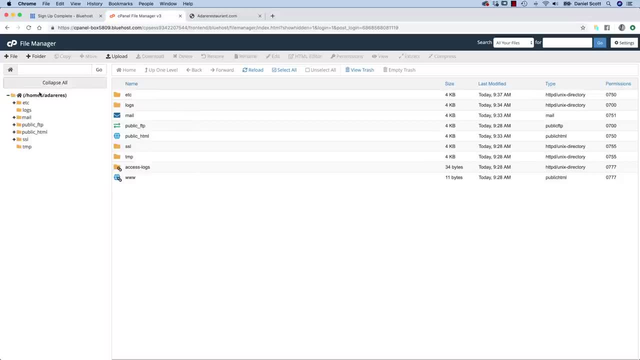 So what happens is this is the kind of like. this is the folder structure that you get. Your website is kept in this one called Public HTML, So double click Public HTML to go inside of it, and this is currently what's in your website. 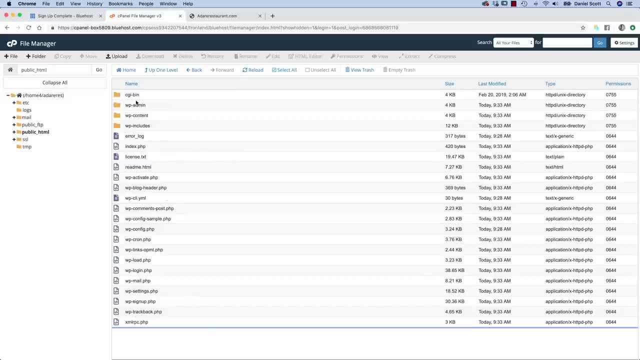 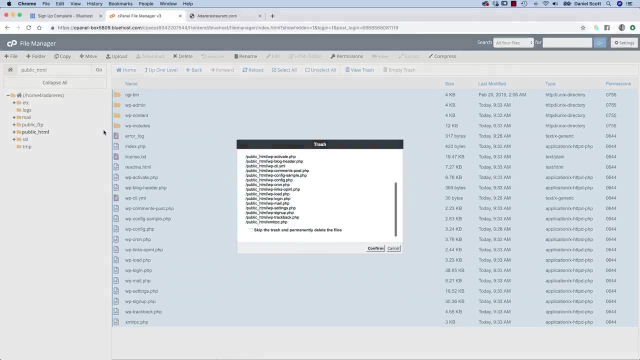 It's not what we need, just it's got a kind of like a placeholder website in here for us. We're going to select it all and delete it. So select all and, on the top here, delete, And we're going to add all that to the delete. 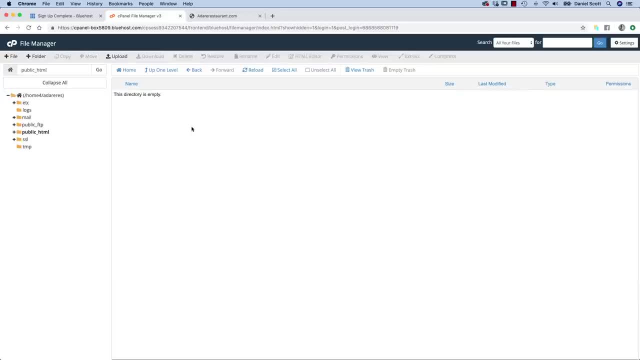 Leave in the trash. you can bin the trash, it's up to you. But now I've got an empty file, so now I want to upload some stuff. Remember, we're in the public underscore HTML, so let's go to Upload. 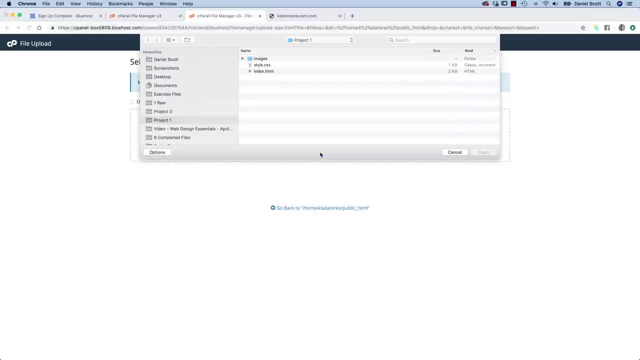 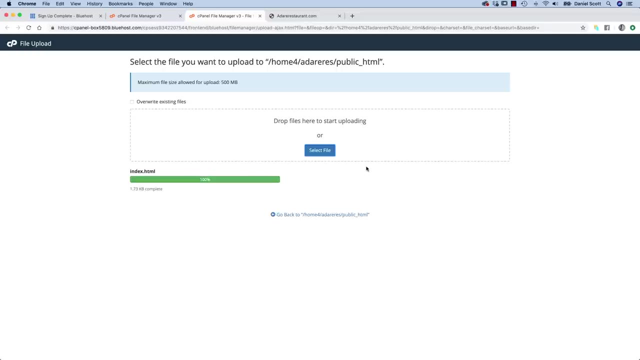 And here we can drag files in or click them one at a time. Select a file, let's do index open. It's not going to work unless we have all the rest of the files. It will half work. so we need to do both CSS and the HTML. 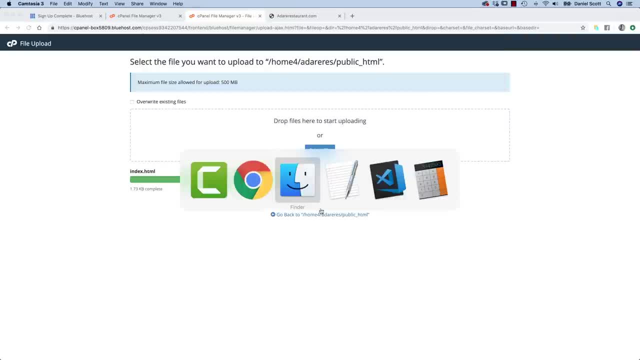 or you can just drag it. It's up to you. You can't drag folders into this thing for some reason. That's why it's a bit caveman-ish doing it this way. But I've got my index and my HTML uploaded. 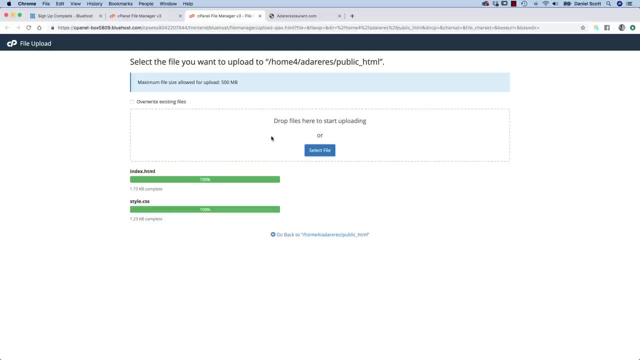 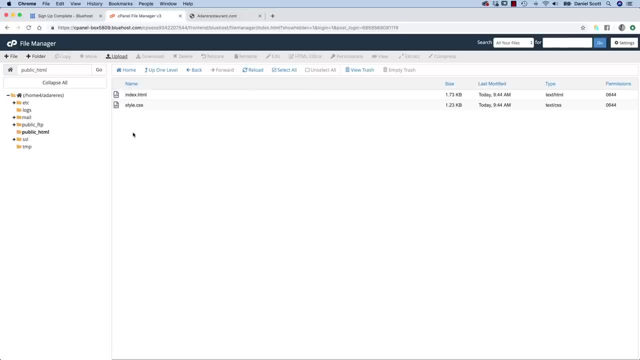 Now what I want to do is I want to add an Images folder and upload them separately. So let's go back. So I've got those two and we just need to rebuild this. So we've got index. so we need this folder called Images. 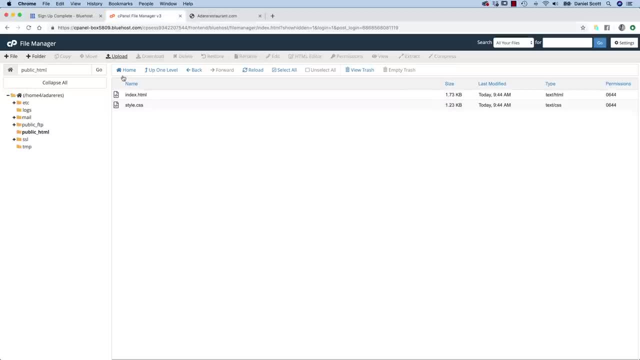 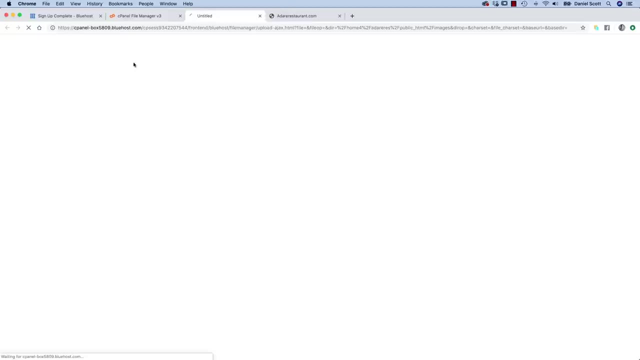 Make sure it's spelled exactly the same. And I'm going to make a new folder. Put them in create folder, Open it up by double-clicking it, Upload some stuff to it. Find all my images. don't have much too. 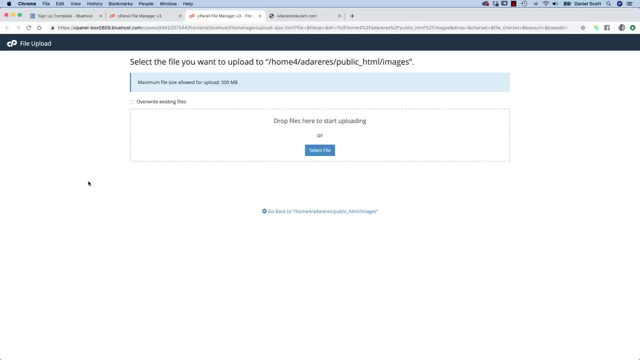 I'm going to drag them across. Images will take a little bit longer to upload. I'm on some terrible internet here, so it's going pretty fast. I'm the web designer who's working out of a shed next to sheep With terrible internet. 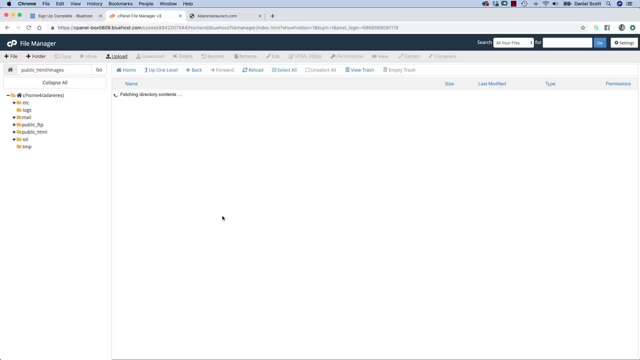 Anyway, fast enough. All right, let's go back And are we inside the? So go back to publichtml just to see You've got all of them in there. Let's go check it out. Are you ready? This is a pretty big moment. 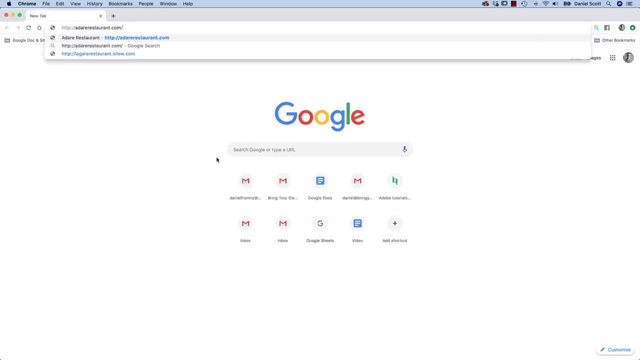 I'm going to go a new window. We're going to type in adairrestaurantcom. Are you ready? Hold steady, Even like this is just a Do it, Dan, and then talk later. go Make it load. Hey, there's a map. 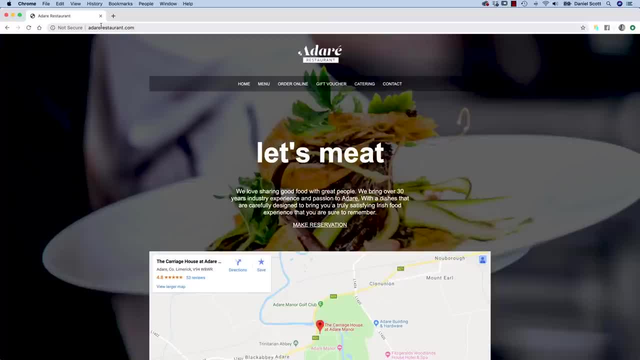 The good thing about it is you right now, as a student, can go to adairrestaurantcom and it'll probably be here. Let me know if it's not because I haven't paid my hosting fees. It might come down at some stage. 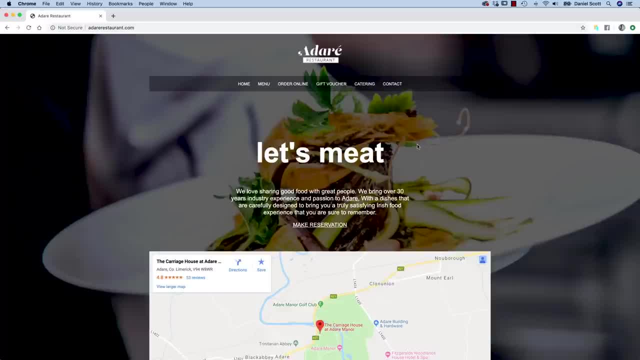 because, as much as I like this website, it doesn't serve any real purpose other than learning. But that's the cool thing about it is that now anybody can go and see it. You can see it to your mom, you can send it to your friends. 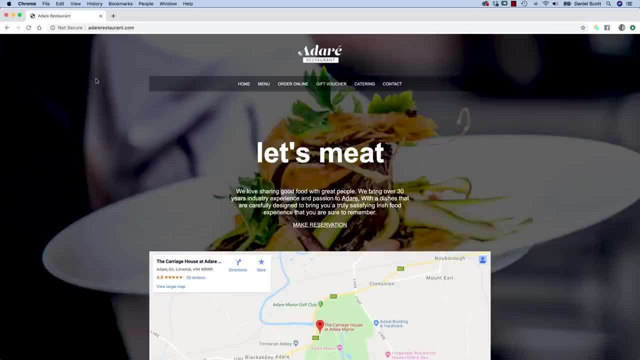 and say: go check out my website, Start posting it on social media. I made a website. Anyway, I get excited because, even if it's like just my like, I've made a zillion sites and it's just that moment. 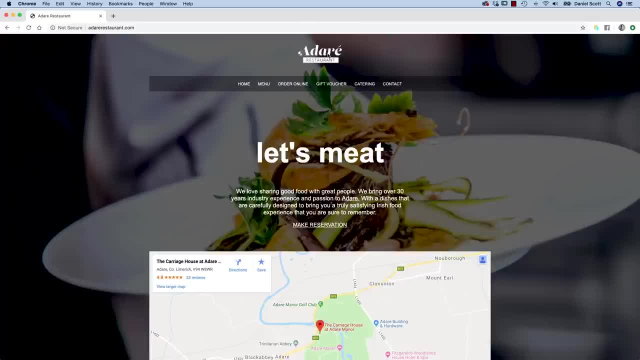 it's like the birthing of your website. It's alive. all that hard work, other people can see it. The trouble is is nobody's really going to see it right? Nobody's going to find this website unless I start sharing it around. 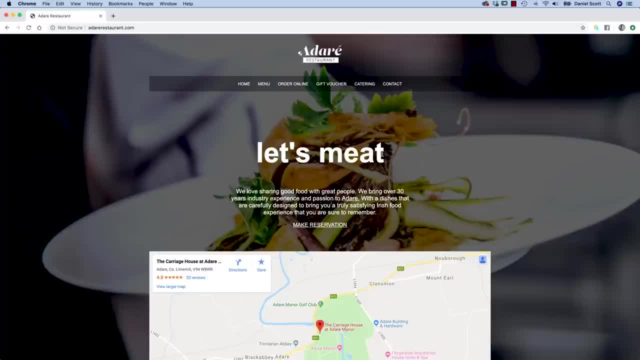 and telling people and adding it to lists and that sort of stuff. But it's alive. it's exciting. One thing you might find is when you get started is that surprisingly? I assume during this course we were going to go and 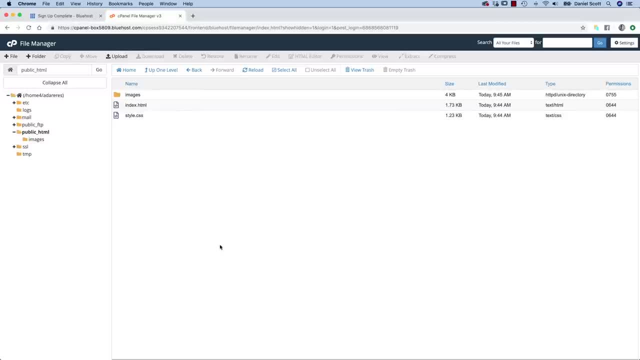 where is it? We were going to upload it here. buy our domain name. and the domain names take a long time to populate. So often you need to wait for a day or a few hours for adairrestaurantcom to work. 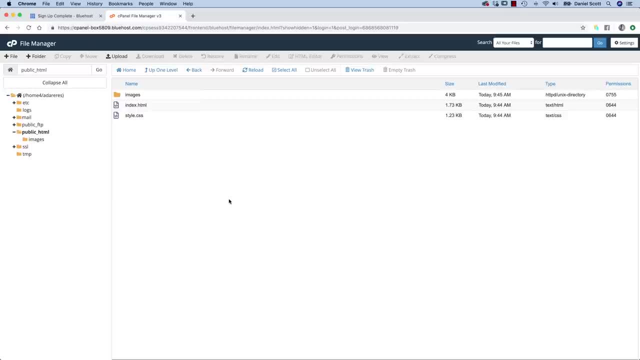 I'm really surprised at how fast Bluehost got that up, And I don't know if it's just like because they're awesome or it's because, yeah, like it's taking me between recording this and actually doing that launch there. 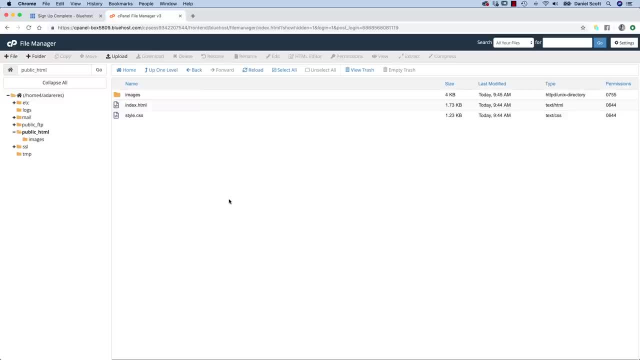 I don't know about 15 minutes, so that's pretty amazing. If you go to your host domain name and it's like you've got danswebdesigncom and it's still not loading, it's coming up with not recognized or can't find it. 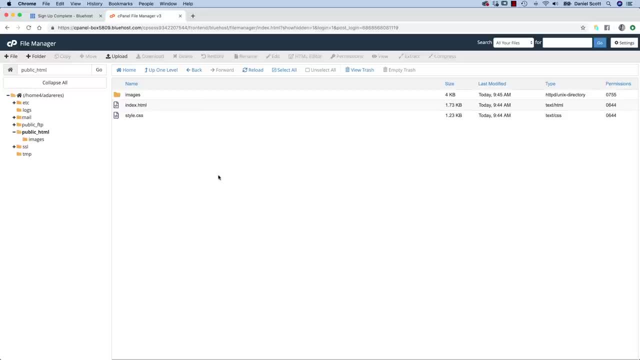 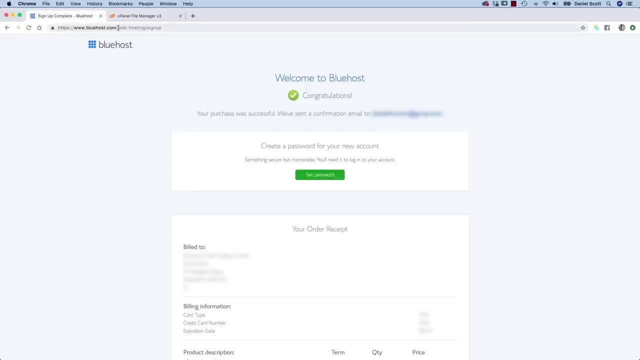 give it- at least give it the maximum of a day. If it's still not working after a day, contact Bluehost. Bluehost are awesome at just customer service They are. that's the reason I'm real happy to send people their way. 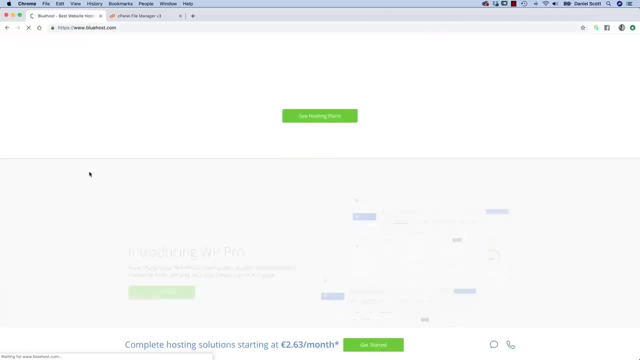 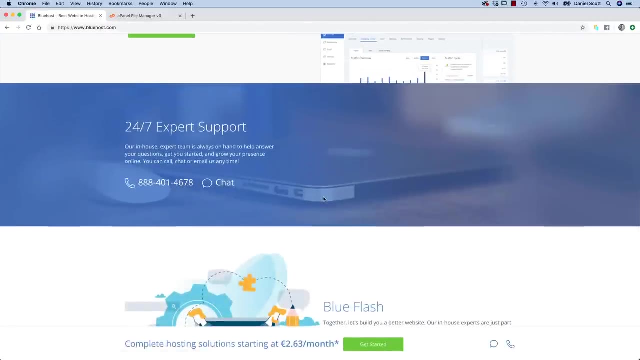 because Bluehost's 24-hour support is really amazing. So where are we? Yeah, these guys, you can call them, you can use live chat, you can email them and they're crazy fast at getting back to you. It's not a pitch, I guess it's just more of a. I don't know. 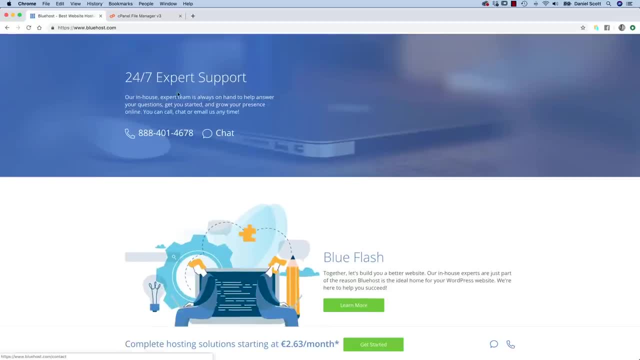 not all businesses are as good as this. I wish more were, but anyway. So the domain name came through. you might have to wait a little while. I just want to jump in here real quick, because I said: just wait a little while. 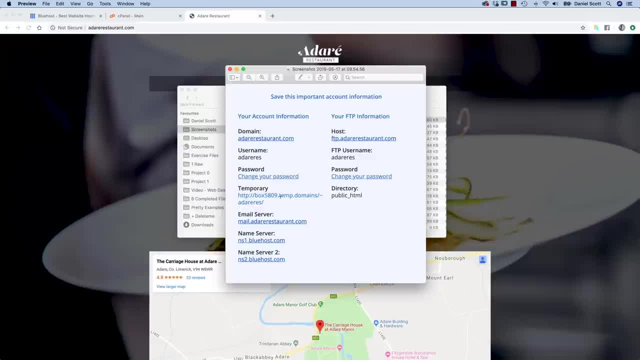 Actually, you don't have to. you do have to wait a while for the domain name to get populated, but there is a temporary domain name that you will get, So they'll send you an email saying they'll send you probably three emails. 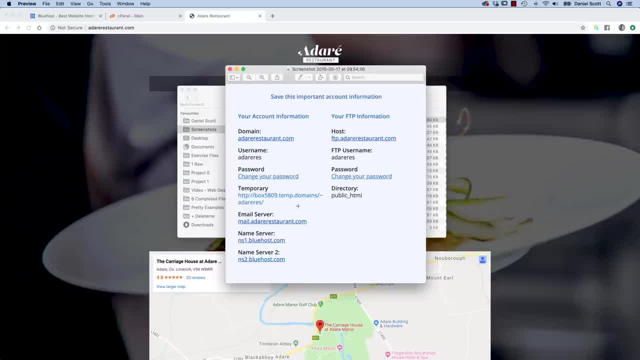 Your account, sign up some details like this one. So check through them all and you'll find one of them that has this important account information. This is the one that you can use temporarily Because if you're like a bit deflated, because you're like 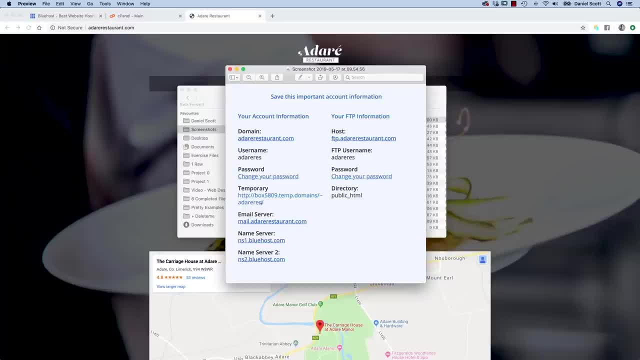 I've got a domain name and it doesn't work. Use this, copy and paste this into the browser and this is like a temporary holding for your domain name that will later on become live, so just use that. Yours won't be Adairis. 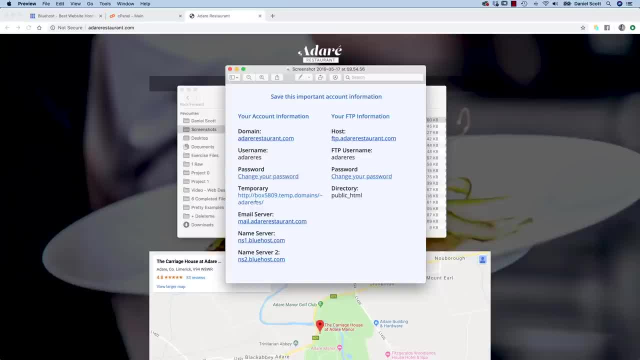 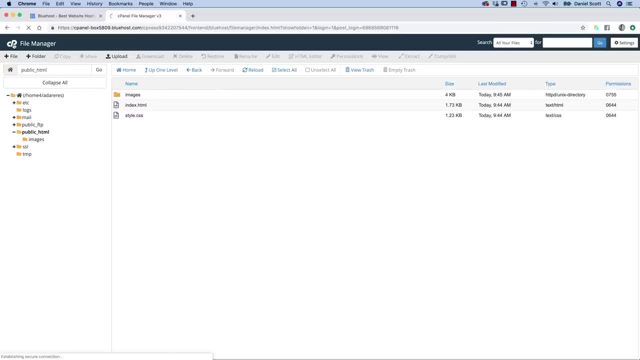 Yours will be whatever domain name you're using, so this will be different for you. But anyway, let's jump back into the video. And again, if you run into any problems with this, with the hosting, you can contact me and I'll help you as best I can. 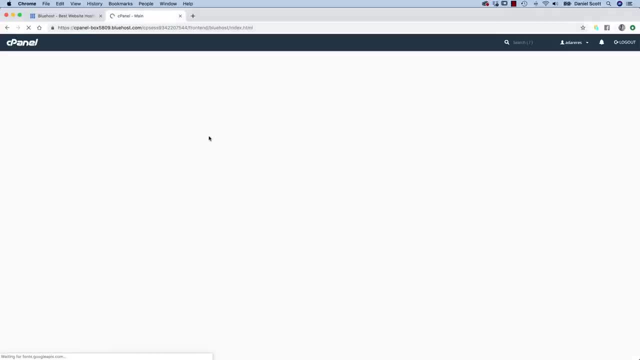 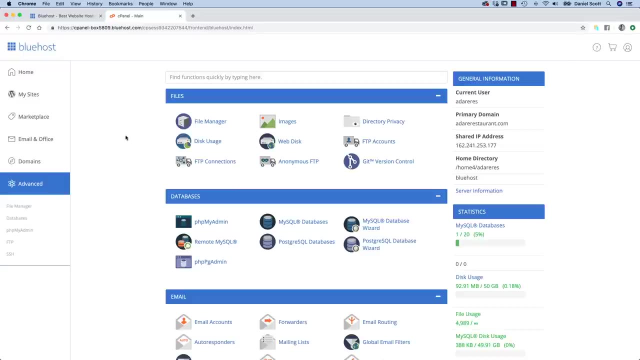 but because this is kind of more Bluehost's thing and they change things and move things around, it can get a little bit well. it'll be easier for them and quicker probably for them to help you. So home is where we kind of start. 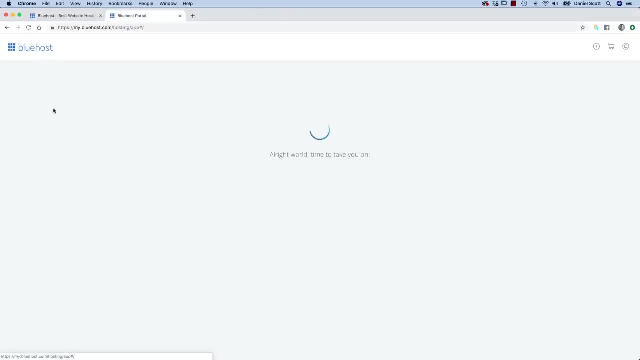 Let's just recap: What Bluehost wants you to do is sign up for WordPress. So we ignored that and deleted that kind of templated stuff from the site, And what you want is File Manager and just kind of recreate the folders and upload it manually. 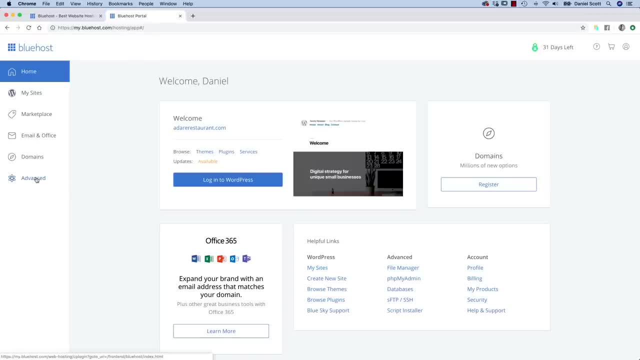 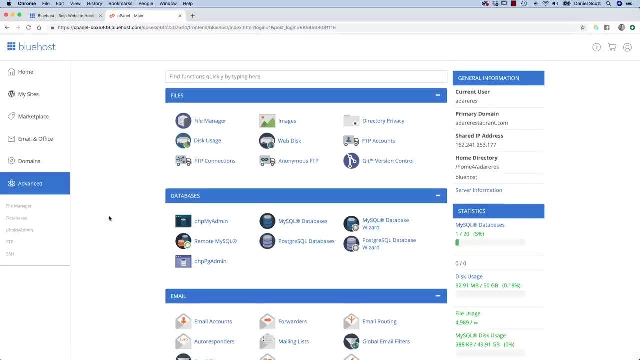 Other interesting parts about your host is under this advanced one. Click on that. you'll see all of these again. but there's some other useful things in here. Depends on how nerdy you want to go. You can set up your email address from in here. 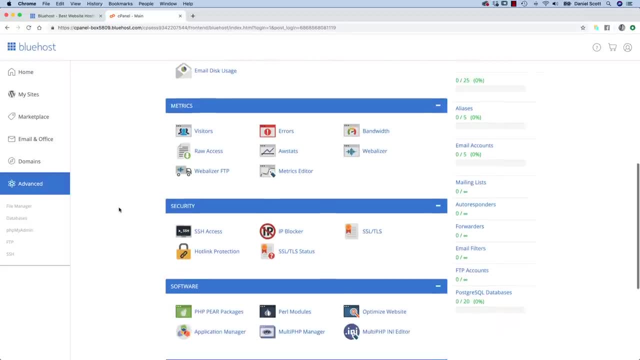 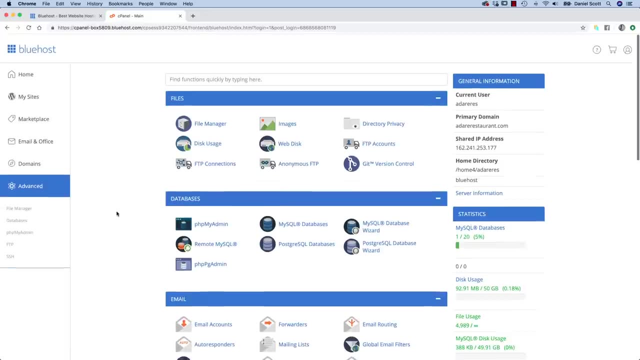 You can set up kind of tracking- how many people have been to your site, all sorts of cool stuff, And the other thing is something called an SSL certificate will get created and applied to it later on. At the moment, if we go to adairrestaurantcom, 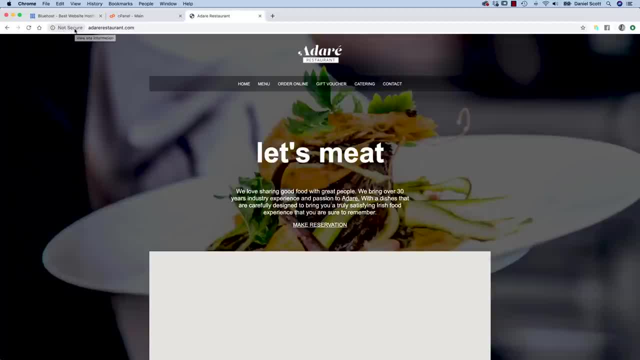 you'll see that it says not secure, That's just because it hasn't been made and done yet. That will become secure later on. So if you go to your site and it says: hey, this is a dodgy looking website. 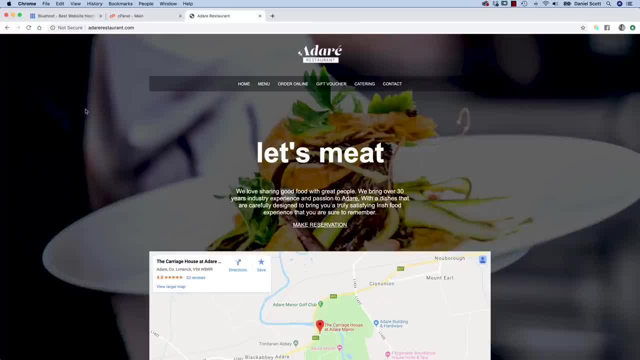 it's because the security hasn't been put on it yet And it's fine for you to look at, it's fine for anybody to look at, it's not malicious, but it will need to be there eventually because Google doesn't like unsecured sites. 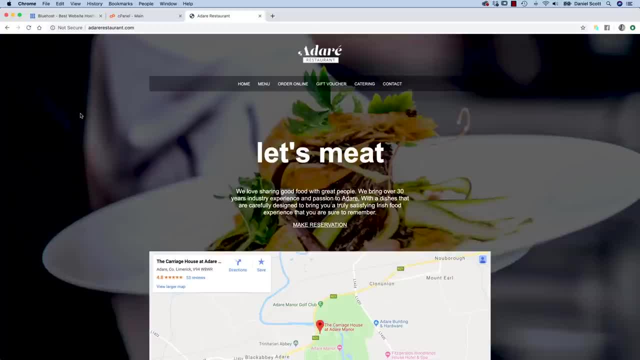 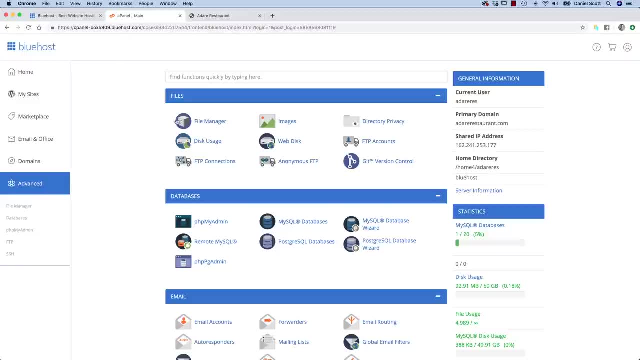 but that will happen automatically for you If it doesn't reach out to Bluehost and ask them to help out, but it seems to be an automated process with them. Now I promised you we'd do the long way, which is kind of using cPanel and File Manager and manually updating it. 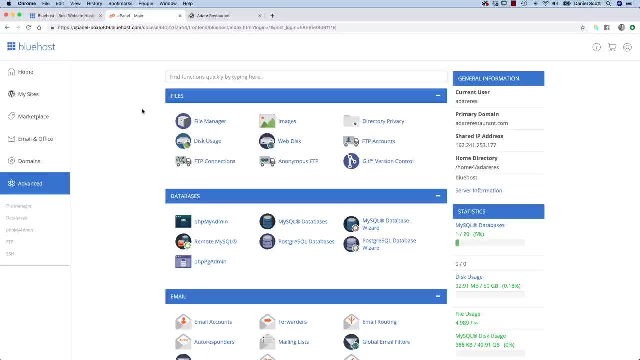 Now it would be nice just to kind of be in VS Code and just kind of automatically send it. So let's do that now. and this video is epic, right, It's pretty long. Let's do it In the next video, kind of separate it out. 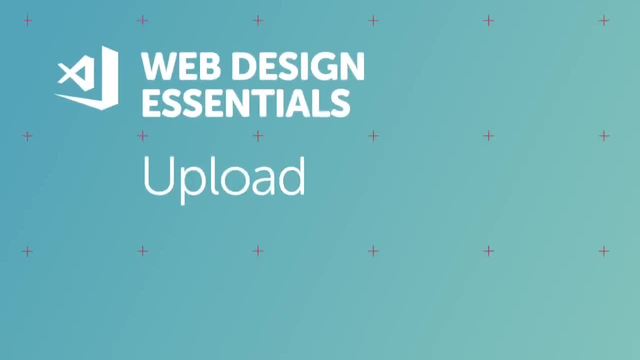 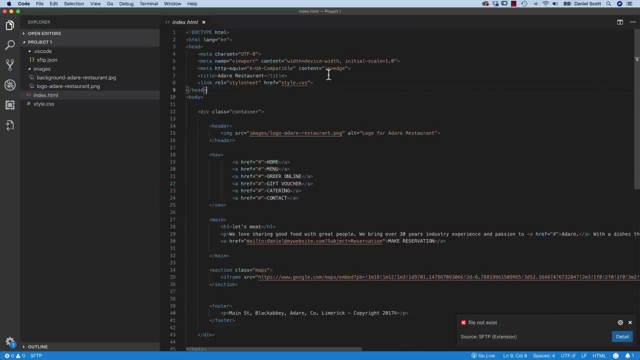 All right, I'll see you in a sec. Hey there, in this video we are going to use VS Code to connect directly to our host, rather than using kind of anything else or using their website. It's all done within VS Code. 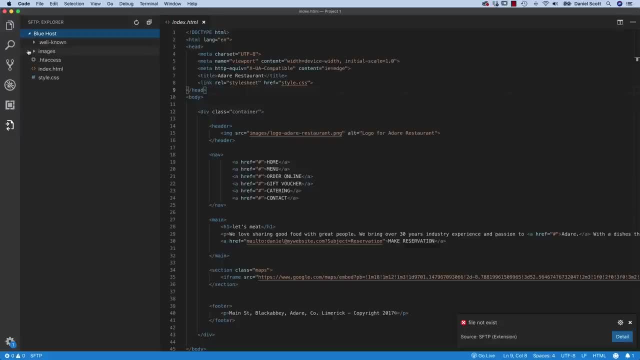 We're going to install this plug-in called SFTP and it's going to show me everything on my site nicely, And when I want to upload stuff I just right click it and say Upload, and it ends up on my website, simple. 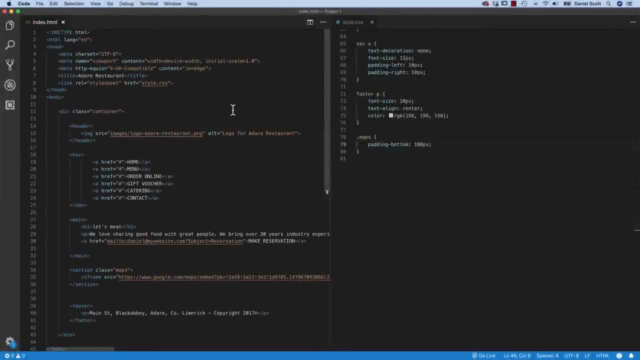 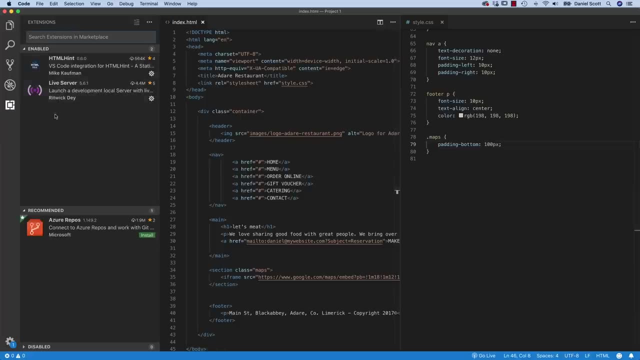 All right. so in this video we're going to connect directly from VS Code. We're going to use something called SFTP and it's one of the extensions, like we did earlier. Remember we did extensions for HTML, Hint and Live Server. 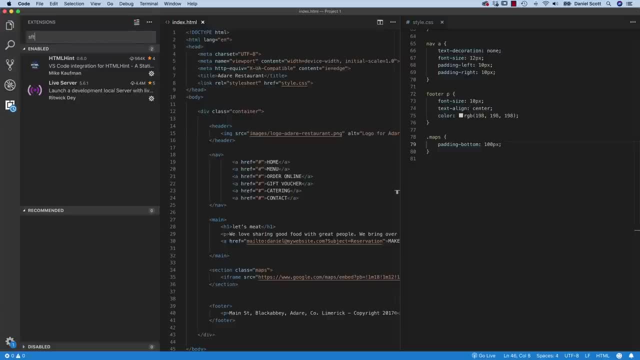 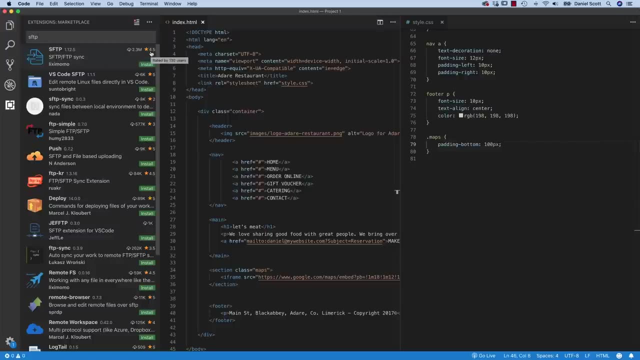 Like the other ones there is, so SFTP is the most common one at the moment. It's the one that I use and it seems to work real good. It has 4.5 stars and has a chunk of downloads. 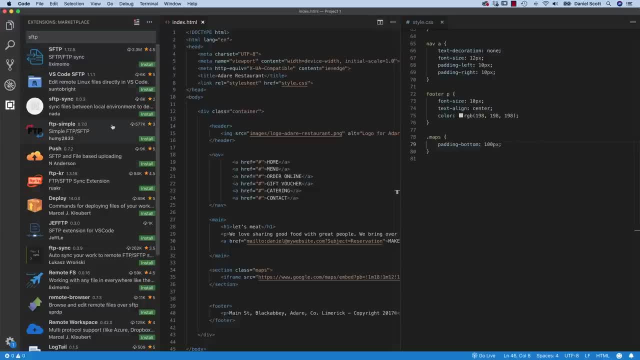 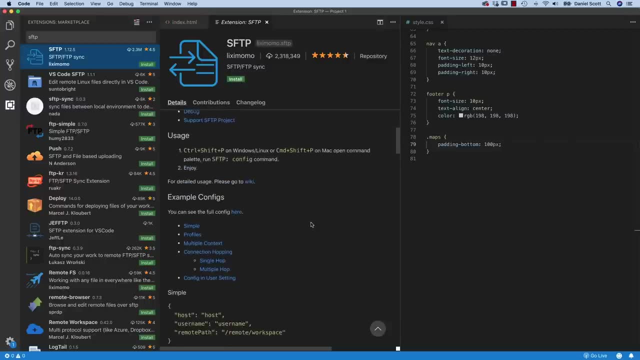 So you will check when you're doing it. There's other ones in here that one's got less stars. That's the one we're going to use for the moment. Have a little read through how it works. I'm going to show you how to do it. 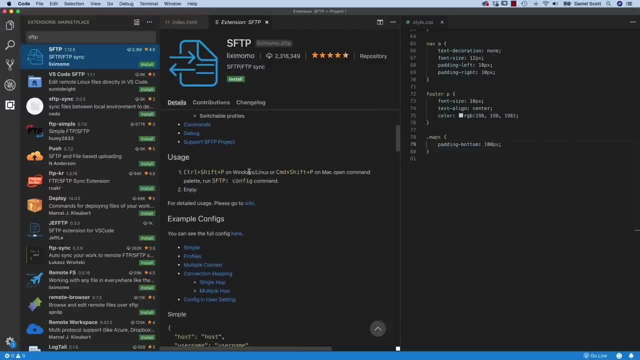 The main one for this one is usage. It says: you need to do this thing. You need to open the command line- sorry, the command palette- and run this thing, and I'll show you how to do that in a second. But basically, there you go. 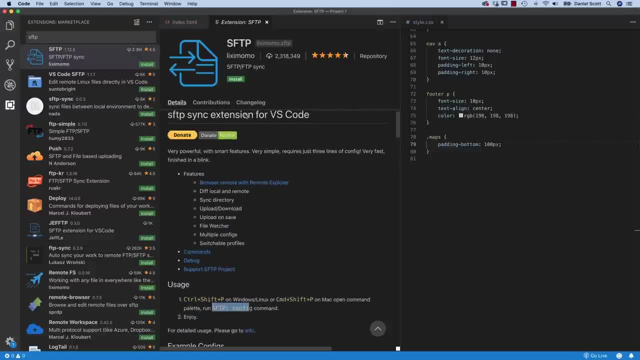 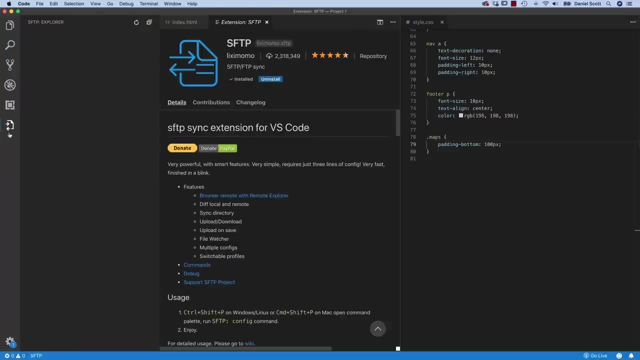 That's what we need to put in the kind of details. So let's install it first. Give it a sec, All right, it's installed. Nothing really happens. you might have noticed there's a new little icon over here which doesn't quite work yet. 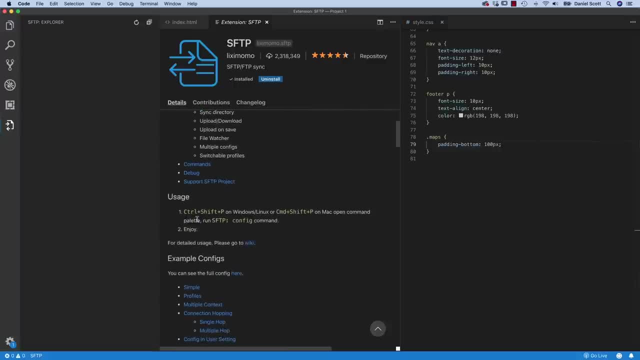 We've got to set it up, and that's what they say in here. They say: do this, run this shortcut on Windows Or on Mac and then type this in. So we'll do that. The long way is under View and Command Palette. 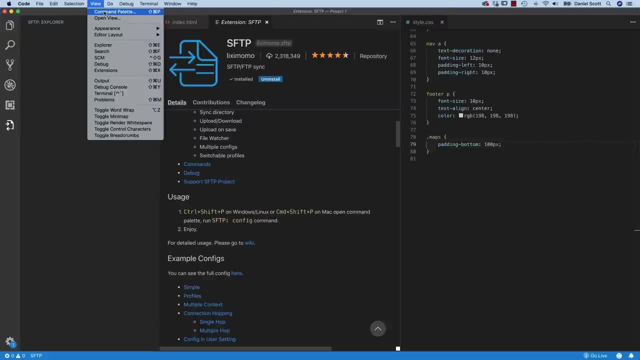 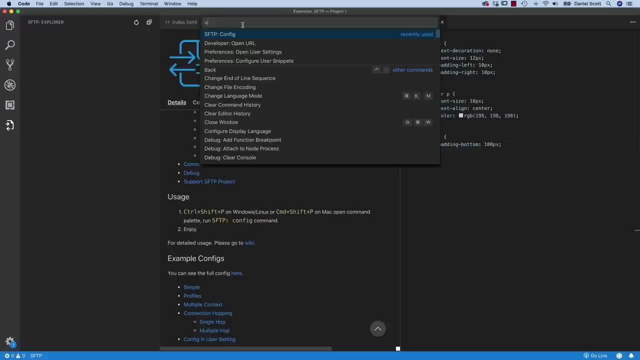 So Command Palette is you're able to tell the give kind of commands to these plugins. It's kind of a crude way of doing. it depends. You might be happy with Terminal or Command Line. some people aren't. So what I want to do is I want to type in SFTP. 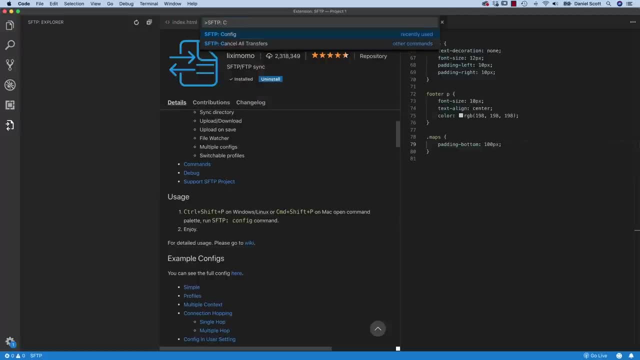 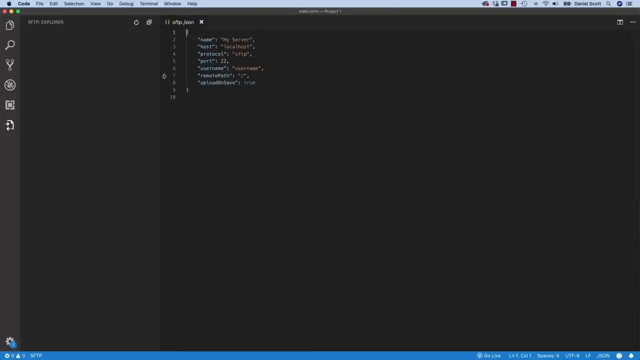 It should pre-fill it in And to configure this bit of software. this is what we need to type in. Let's go. what ends up happening is: let's close it all down to make. I'm going to close down my HTML and my CSS. 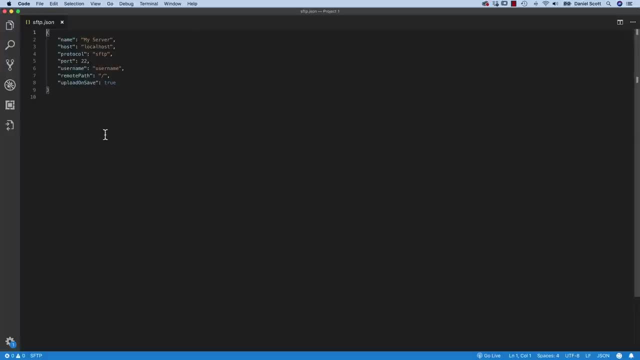 I'll even close down this by double-clicking it, so it's nice and clean. So this little JSON file is the kind of details that you need to populate for this thing to work. Now you're like: where do I get all of these details? 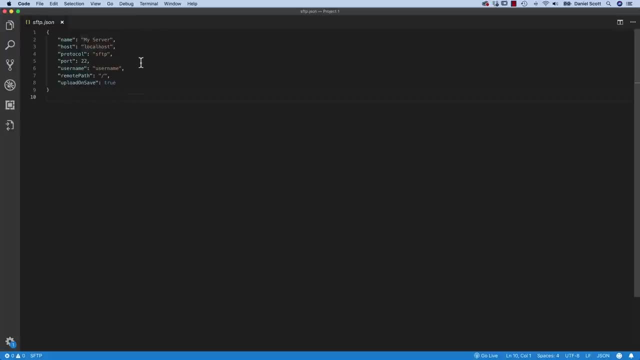 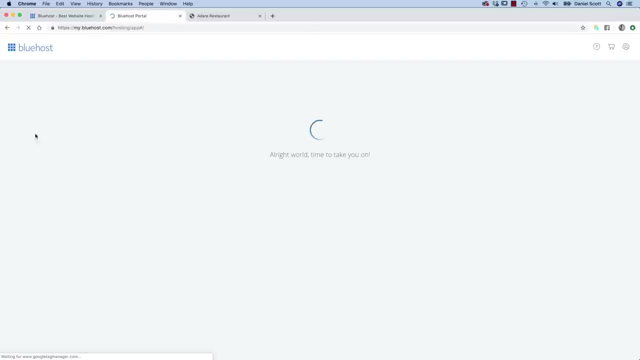 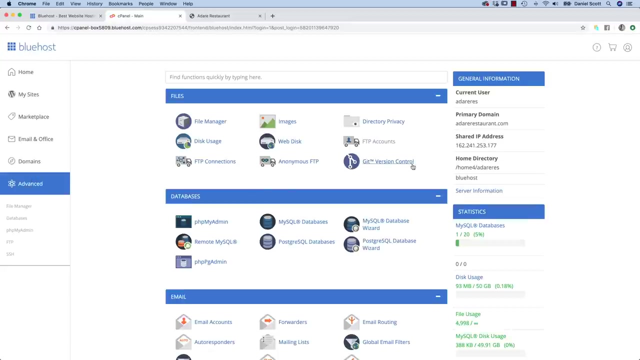 So they are the things that came through in an email. So they either come through from an email from Bluehost or if you go to your Bluehost account, you'll find them from home. go down to Advanced, Advanced, Go to FTP Accounts and you'll find them at the bottom of this. 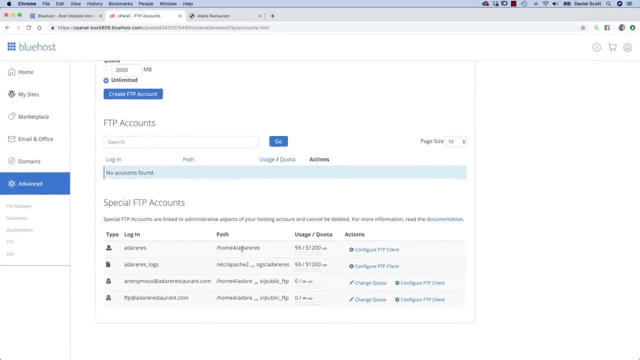 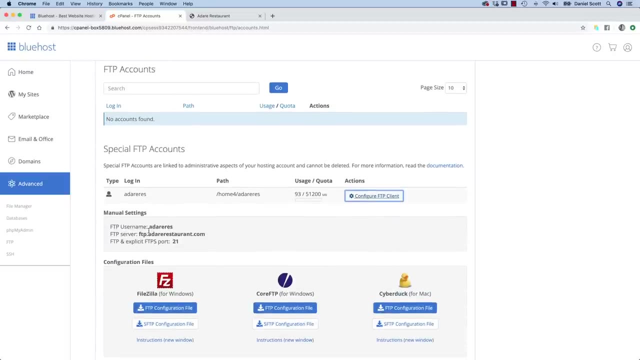 So this top one here is the one that is automatically generated And it's got all of our details in it. You click on Configure FTP Account and here are the basics that you need, So the username, the server that it's going to and the port. 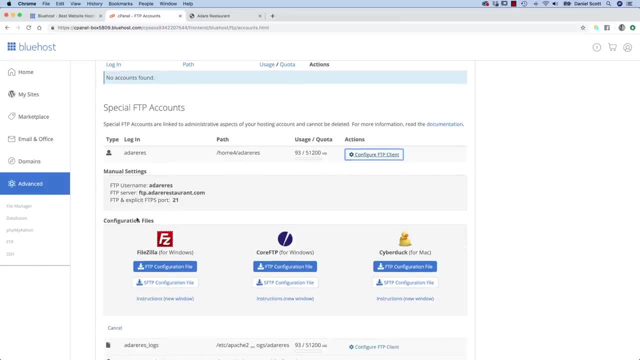 Alternatively, if you don't want to use this plug-in that we're using in VS Code, you can use. if you're more familiar with FileZilla or Cyberduck for Mac, you can use those cool instructions of how to use it. it's just another way. 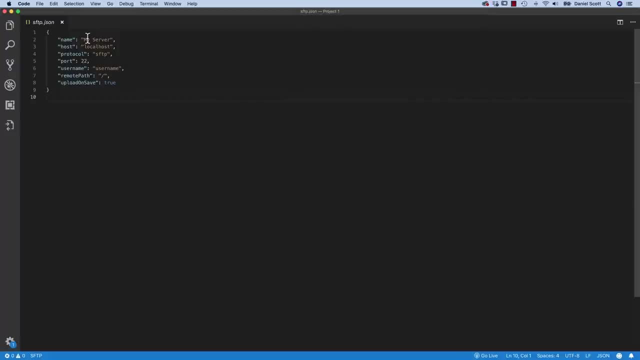 So let's copy and paste them across. so what do we got The name of the server. it's called Bluehost. This doesn't matter, you can type in anything there. This next one, the host address, is really important. At the moment it's local hosting. so on my machine, it's not what I want. 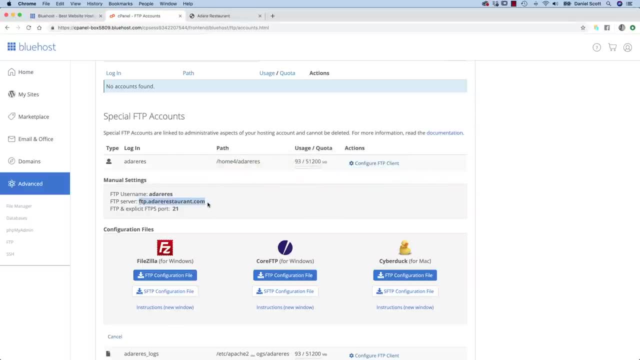 So I'm going to grab this one here. FTP Now, if you're using something other than Bluehost, sometimes it can not have the FTP in front of it, and sometimes it does. So if you're using some other hosting company, you can just. 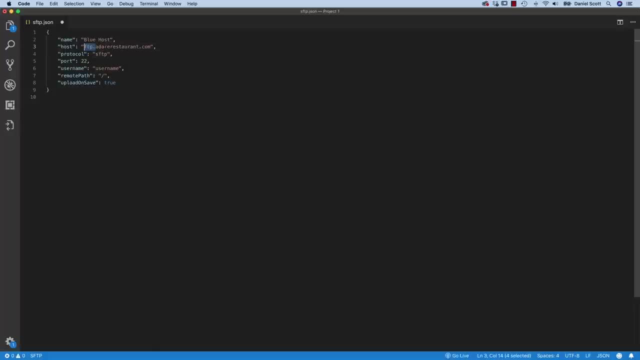 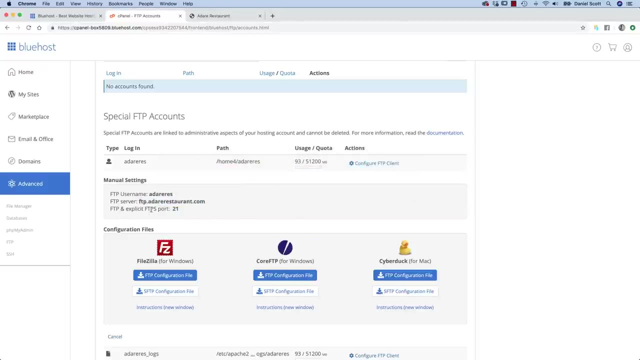 sometimes it's FTP, sometimes it's not. in this case it is. Now, I think in this case we're just using FTP, not SFTP. let's check. I think you can use either. in this case, I'll put in my password. so where's my password? 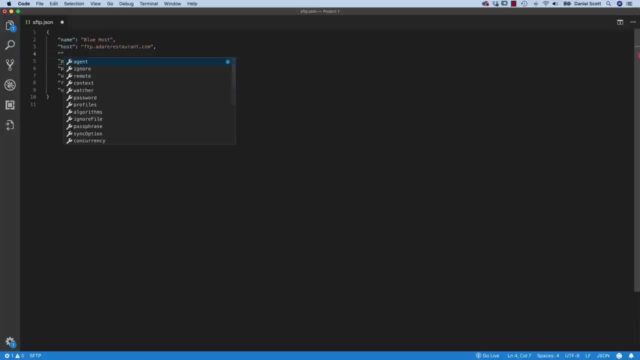 Weirdly it doesn't have it as an option. I remember this when I was setting it up first. So this needs a password to get in password. So you just type it in inside of the quotation marks colon. Your password goes in quotation marks as well and ends with a comma. 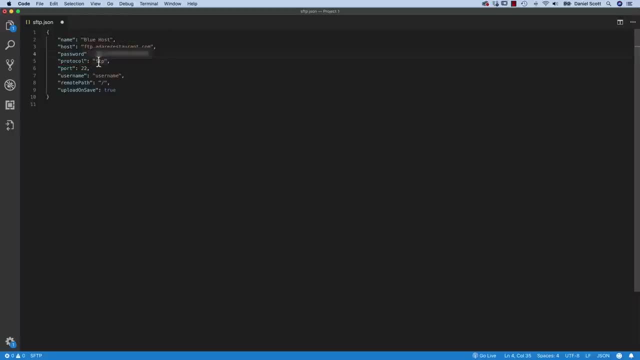 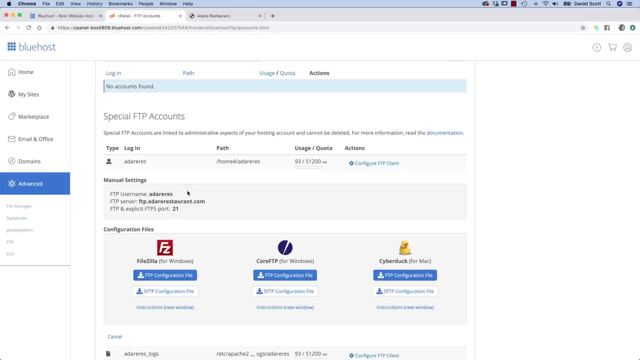 So we've got our name, we've got our host. we've got our password. We've got FTP the port number: Often it's 22,. in case of Bluehost, they are 21,. they are Your username. where's my username? 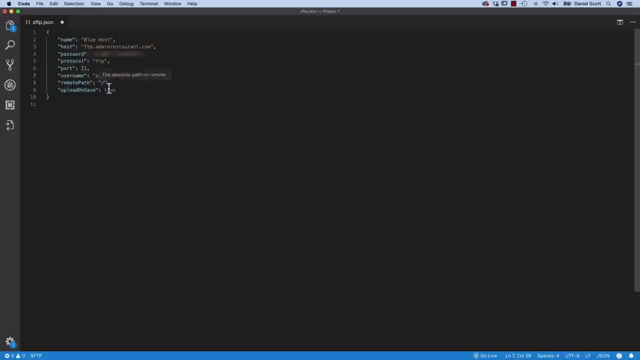 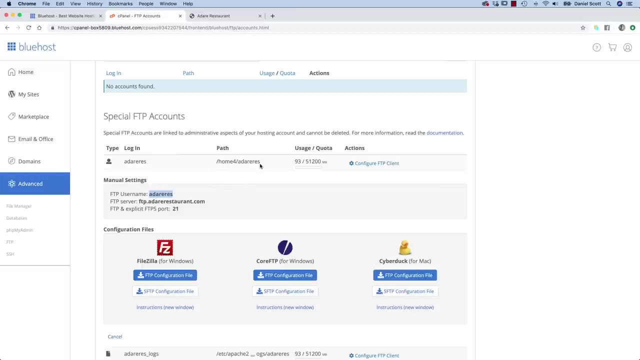 There it is, there AdairRes And the remote path. in this case they say my remote path is Now that's not it Generally for pretty much all hosting companies that I've ever dealt with. it's remember when we were in. let me have a little look. 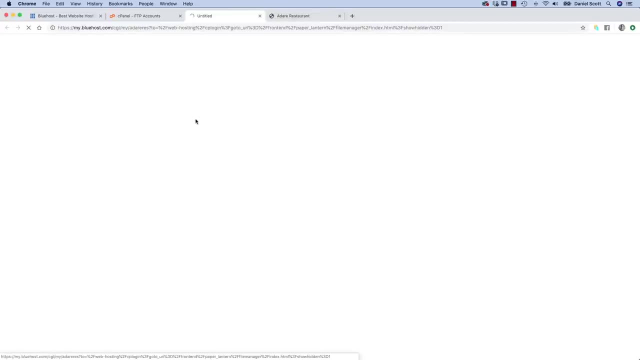 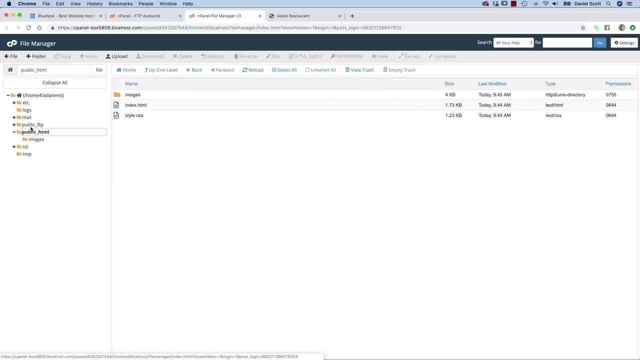 We're in File Manager, remember public underscore HTML. That's the one we want. Remember this one. that's the folder, Because at the moment we're logging into this kind of like big, this big directory with all the stuff we don't need. 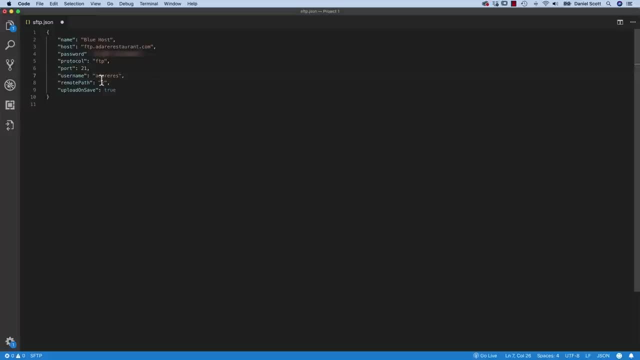 We want to find this public underscore HTML to get to our website. So in here we go to public underscore HTML and this one is up to you. So upload on save. I turn it to false just because, And the problem with having it as true. 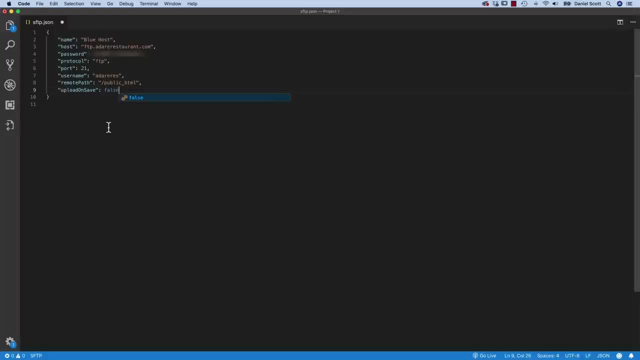 it means every time I hit save, remember, File, Save All. it's going to then try and push my website live to adairrestaurantcom And if I'm messing about with it and it's all broken and half working, the website is going to be half working on the site. 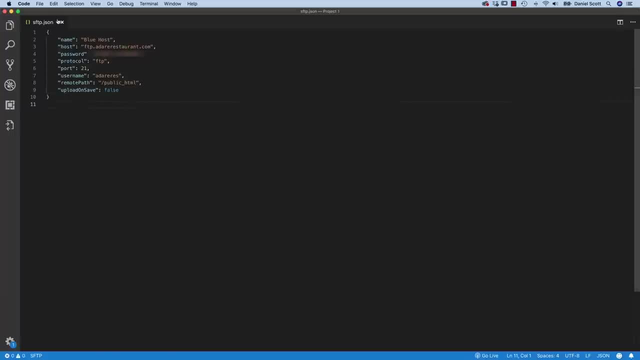 So I set mine to false. Anyway, that's what that guy needs. So we're going to save it and we're going to close it and we're going to go to this option here for our SFTP. You can see our little host there. you're going to drop it down. 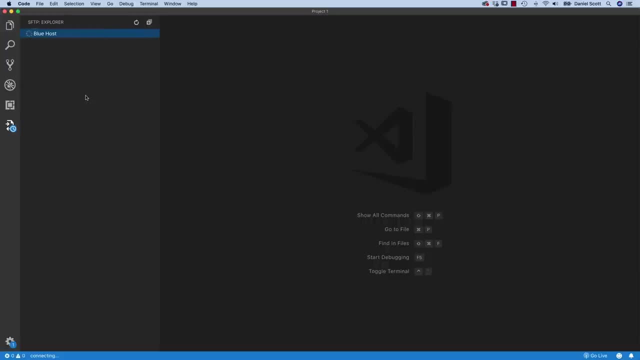 This little blue bar is going to run across for a while until it connects to your server. fingers crossed it does. There you go. so it has found my index and my style and my images, And the thing is, this is not on my computer. 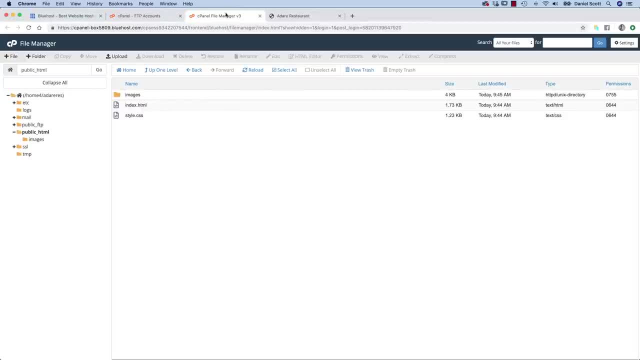 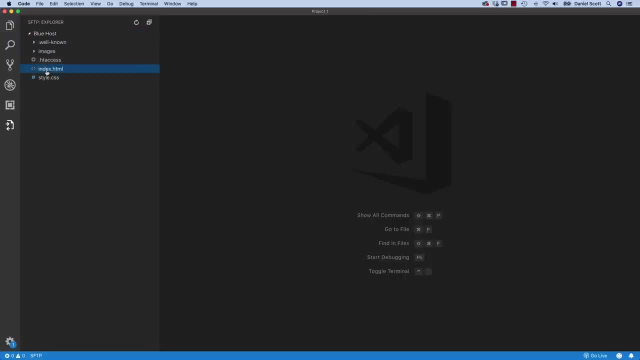 This is actually looking at this folder here on Bluehost which is connected to my URL, which is this: So yeah, that's what that is. So if I go in here now and I click this and I right click it and I say Delete, 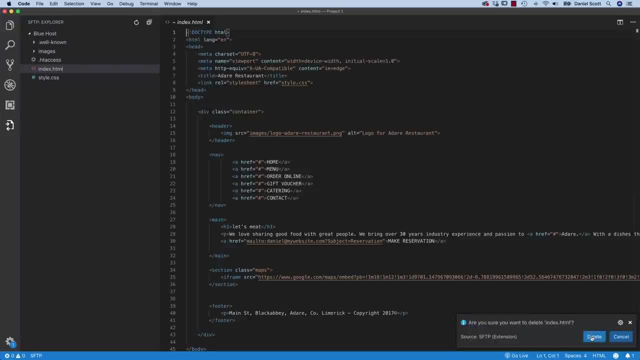 Be very careful. you see down the bottom here. it says: are you sure you want to delete your index page? I'm okay with it because I'm going to stick it back up in a sec, But because I've deleted it here, this thing's going to. 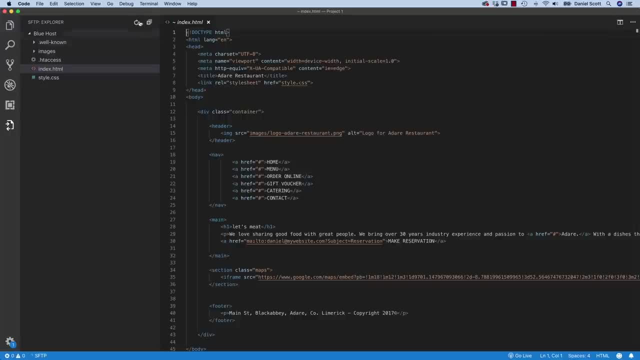 my website's going to freak out because it doesn't have an index page, I'm going to hit Refresh. Let's have a little look Down here as well. you see it kind of humming away. It's thinking about it, it's checking the server. 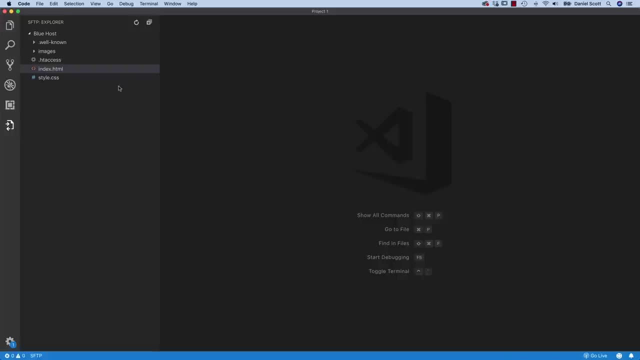 It's never a fast process. This thing's gone. Did it delete? Delete? Are you sure Delete File does not exist? cool, This thing could take a little bit to update. even though I clicked Update, it still was listing there. 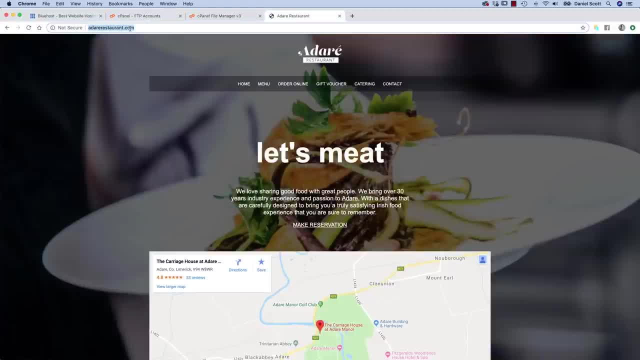 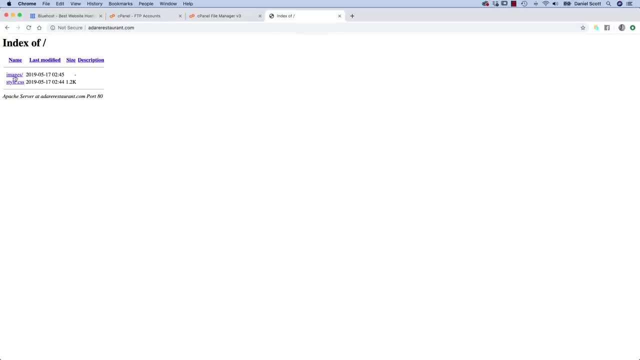 There it is, it's gone. So now if I go to Adair Restaurant, it goes: hey, freaking out. I've got no index page. That's the reason we need indexhtml, And it's showing me other stuff in here. 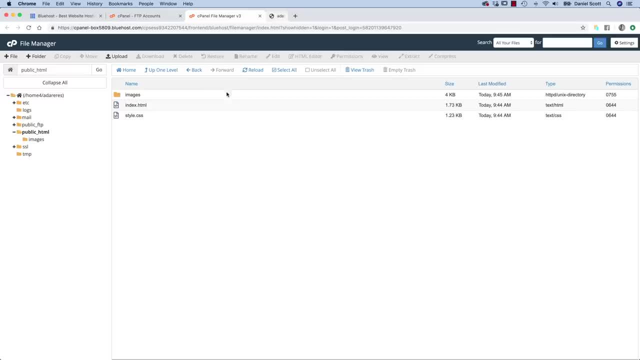 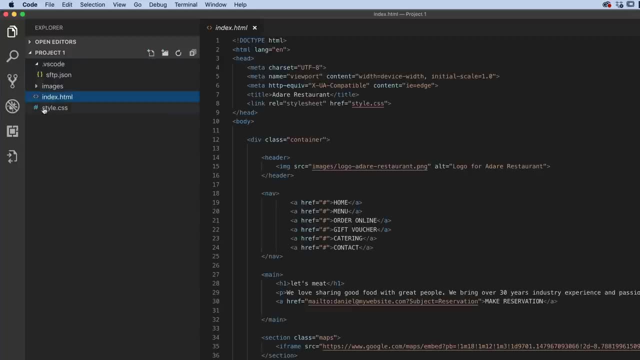 I've got a CSS sheet and some images, but that's not very helpful. So how to get stuff back up? Let's say that I'm in my File Explorer, so this top one, And in here I'm going to open up my index page and I'm working on it. 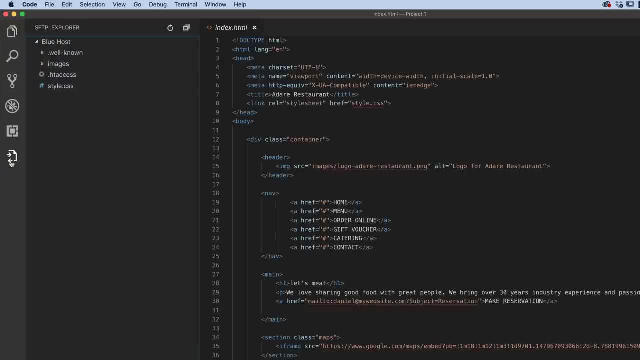 So this is my local Explorer, is my local stuff. This down here is the remote, So remote's considered their Bluehost's hard drive. That's where your site is for other people. this is you, So you do all your work locally and then you push it live. 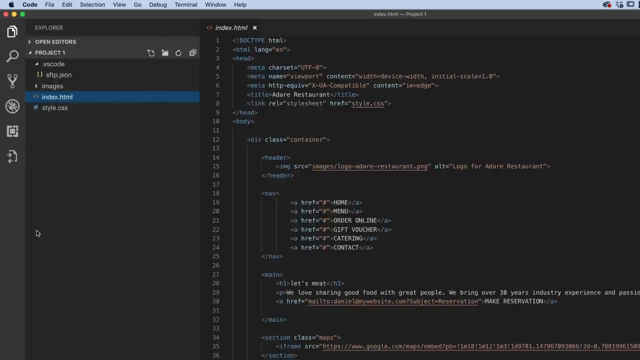 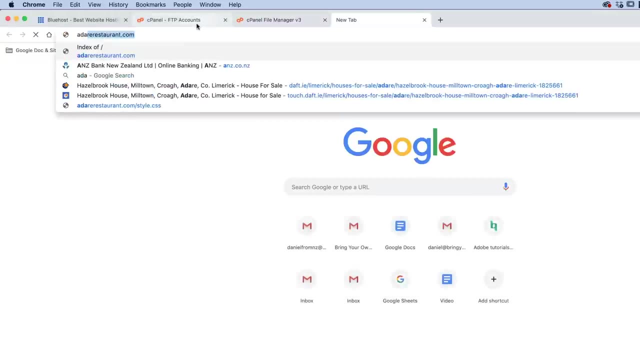 To push it live. you right click it and say Upload And off it goes and it should be uploading And hopefully in a second I can go to adirrestaurantcom and it should be back Nice, Now that is going to work fine for like half of you. 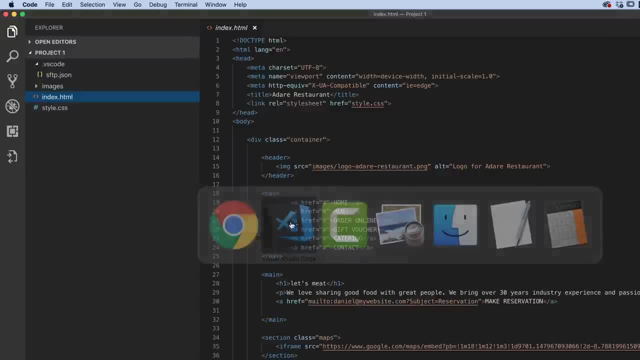 And the rest of you who have got hosting other places are going to be like man, it's not working. we're so close, So how do we fix it? A couple of things: is you need to open up the same thing as before? 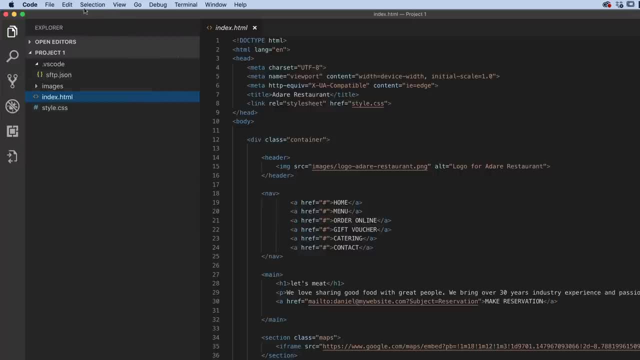 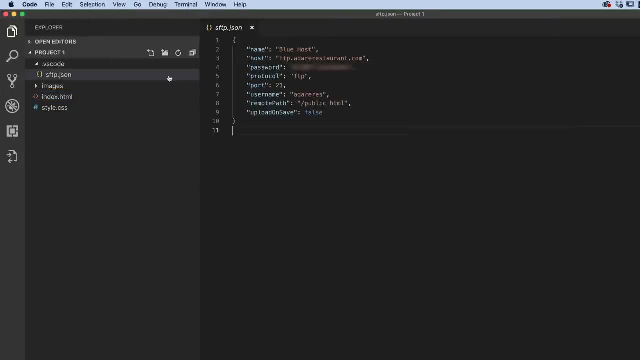 to get back in to do the settings, And that's really weird because like, yeah, Anyway, it's just the way plugins work in VS Code. I can go to Secure View, go to Command Palette, and that's the last thing I did. 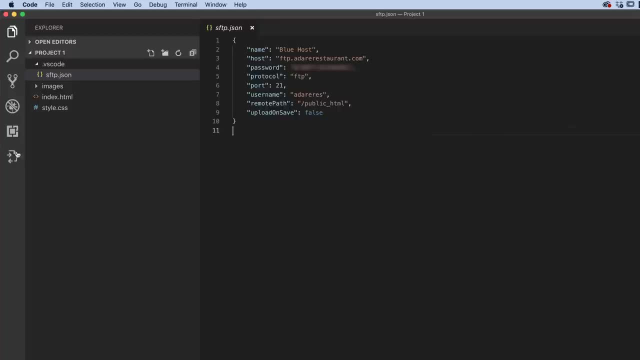 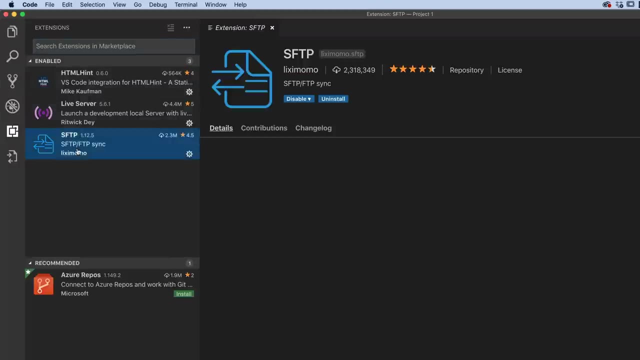 And I can open up this JSON file. If you can't remember how to do it, you go to the extension and then you find I'm going to close these out- and it shows me the ones I have enabled. I can click on it. 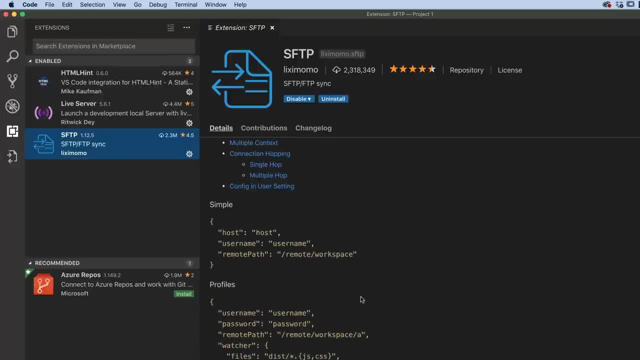 and then kind of read through the documentation again on how to do it. You can see we've just done some basic stuff. There's a lot more that can go in there. You can do Watch Folders, which is cool. There is lots of stuff that you might need to do. 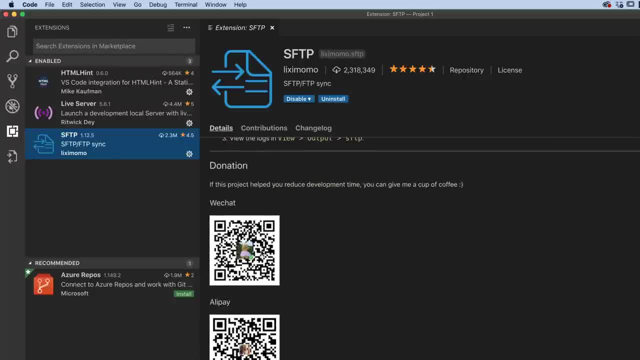 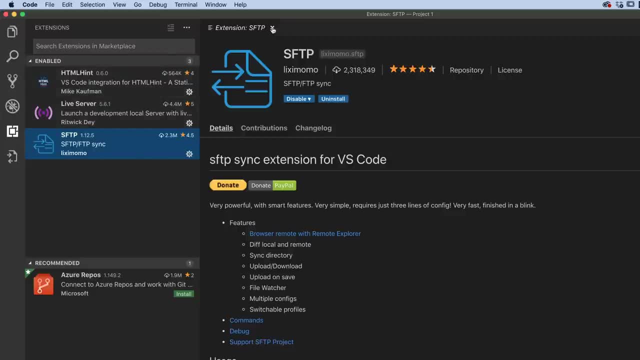 to make it work, maybe your school or your university or your work. All right, so what are we doing? Oh yeah, problems. So we wanted to open up. I'm going to close all the extensions down and I want to go to View Command Palette and open up this again. 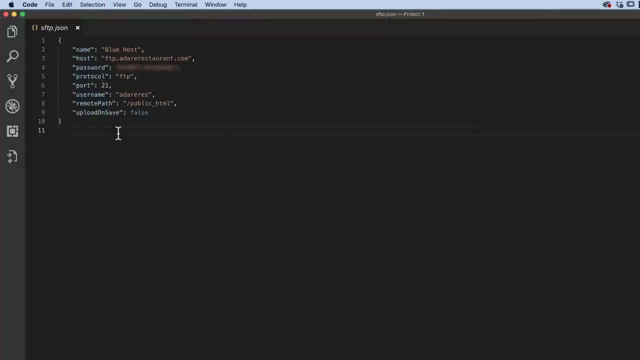 So if it doesn't work, a couple of things you can try easily yourself is sometimes that your username has an email address, So it could be it might be this at adiarestaurantcom That sometimes can get some hosts do that. 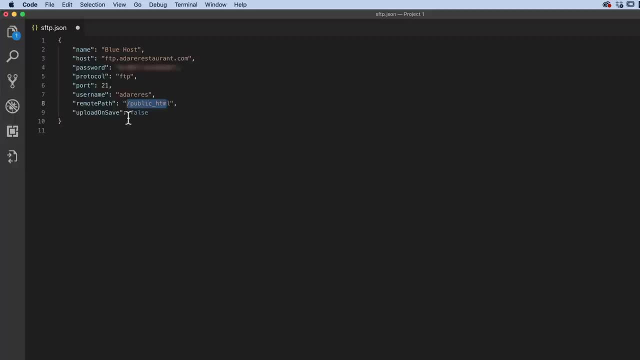 Sometimes you don't need that. You can delete the public slash underscore. it can just be left by itself. Just leave the slash there. sometimes that works. Sometimes it needs to be SFTP. Sometimes you might got your password wrong. 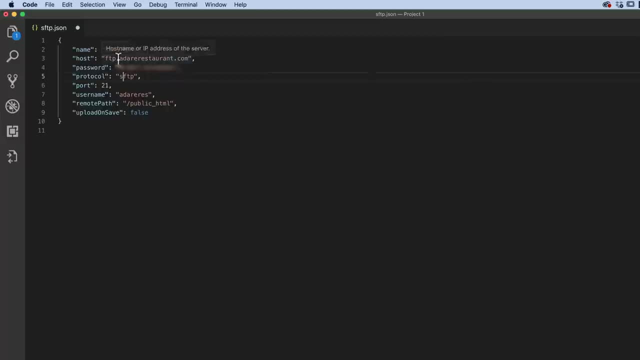 We talked about the host. sometimes it doesn't need the FTP at the front. You can delete that. sometimes The host name doesn't do anything. Just get listed in this little folder here And if that still doesn't work, copy this: 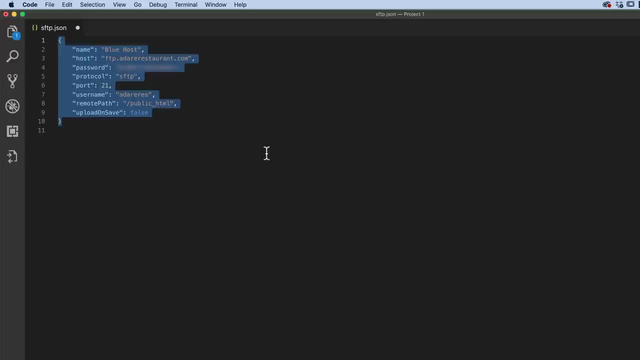 I'll actually copy and paste this into a Word doc right now and stick it in your exercise files. And what you do is you contact your host, Say you're with GoDaddy or HostGator or somebody else, Just send the support ticket and say: 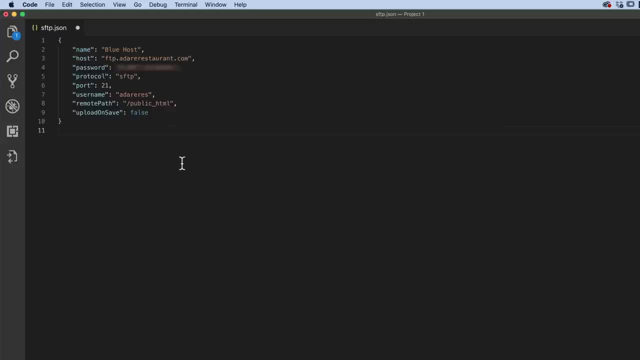 hey, I've got an account with you and I can't connect it. Can you tell me what to put in this And they might go? oh yeah, you're doing it wrong. You've got to put in port 23, or 22, or something else. 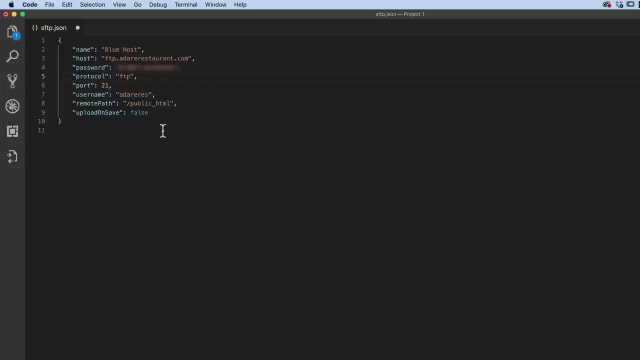 Or they'll tell you how to kind of change it around And the way to test it is. once you've done it, save it. That might be a thing that you've done wrong as well. Let's go File Save, click on this and click on Bluehost. 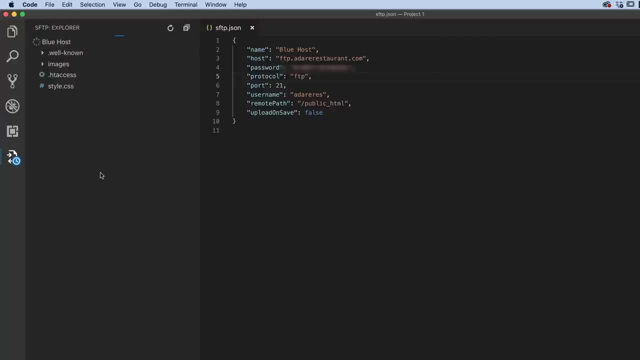 Hopefully this eventually will populate with the things on your site. Now what else can you try if it's still not working? FTP can be blocked by your internet provider. Not your internet provider, but your say you're at a- I don't know a coffee shop. 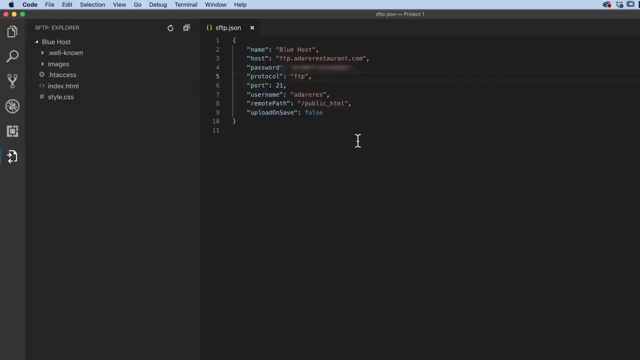 or a hotel that you're trying to do this in. Sometimes the infrastructure there- the Wi-Fi network- will block kind of weird stuff like this, because you're trying to connect with a server online and they freak out sometimes. So if that's happening- or at least yours is broken- 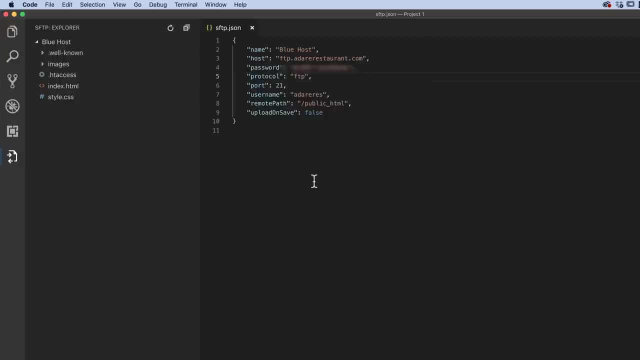 try connecting to a different Wi-Fi. Say you're at work, try it at home. If you're at home, try it at a friend's and try the exact same thing, because sometimes it's your internet that's wrong, It's not the details, it's not EVS code. 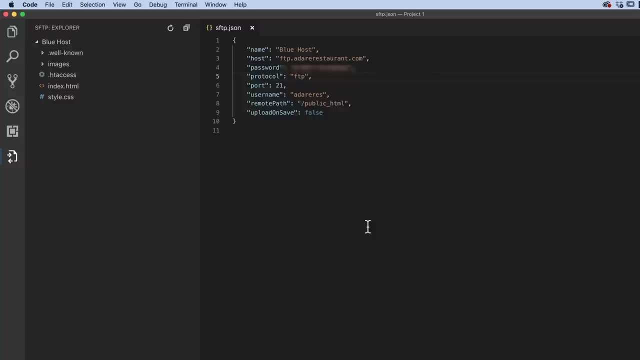 I've got around it sometimes by doing a hotspot on my phone- Like what do you call it tethering- on an iPhone or a mobile hotspot on my Android phone, and I connect my laptop to that and go and try it, and it works fine. 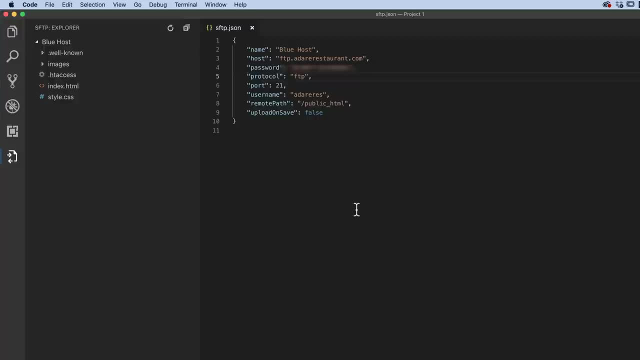 And if it's still not working, contact your host. They're there, they're real quick. Bluehost are really good at getting back to you and helping you out. Same thing. I'll put this in a Word doc now. Try and remember. come on, Dan. 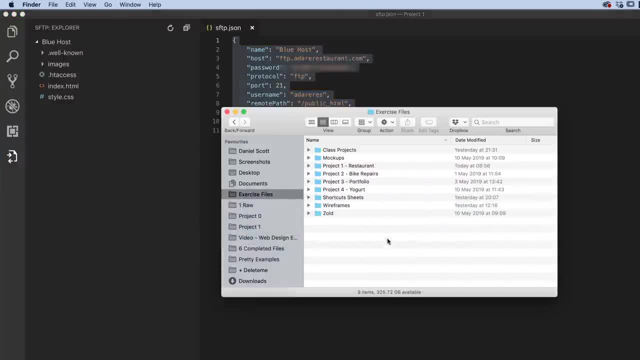 I'll put it in your exercise files in a second and it will be under Project 1, and I'll call it FTP code. And that's it. we've connected it. it's online. It's exciting, people can see it. we can update it. 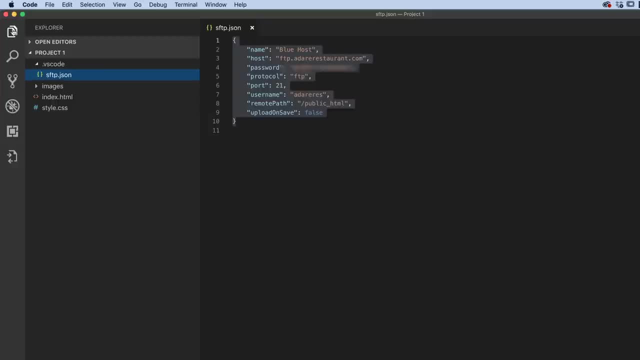 And if we need to make any amends, we'll upload it to our site. all we need to do now is click on it. You can actually grab a chunk of stuff. You can say: I want images and all of this.